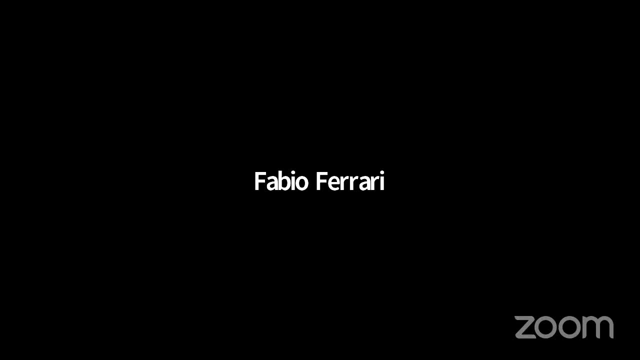 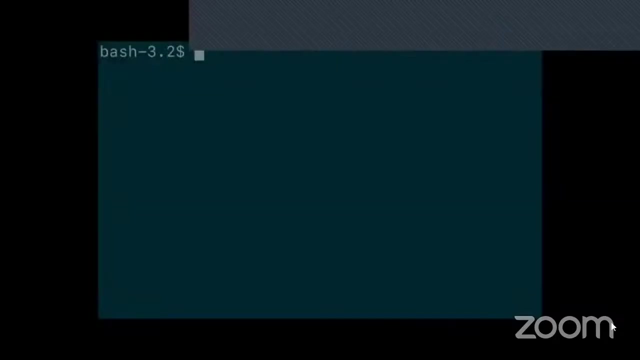 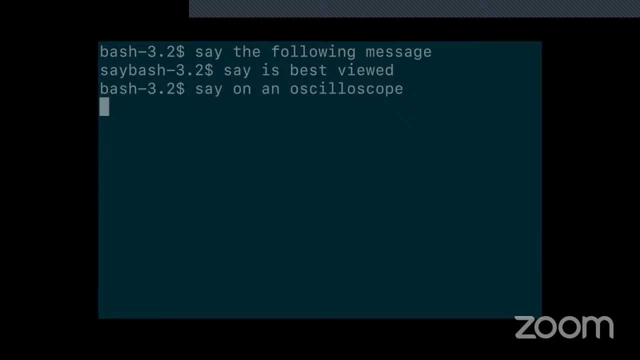 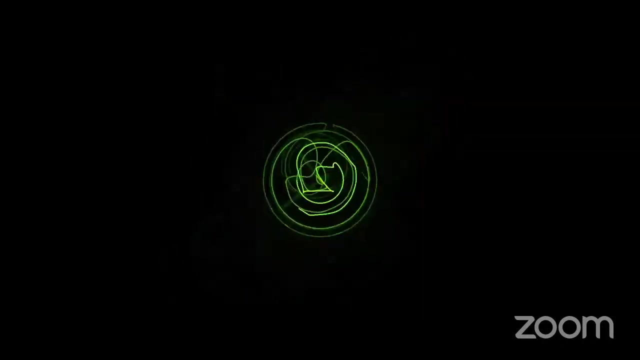 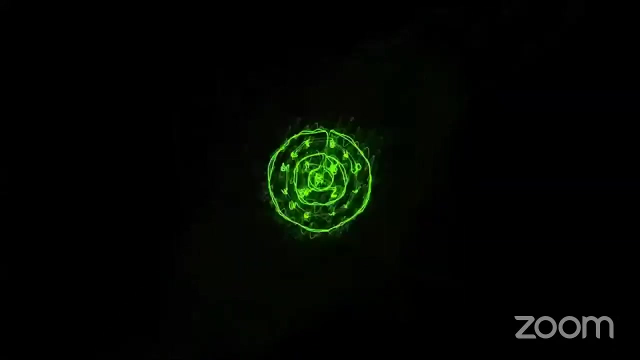 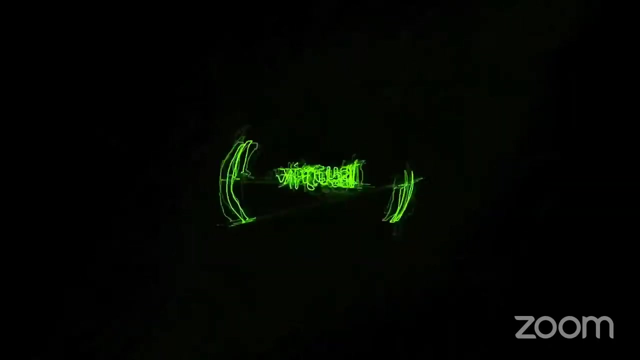 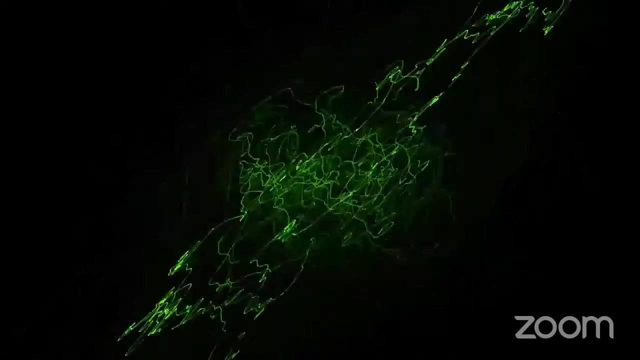 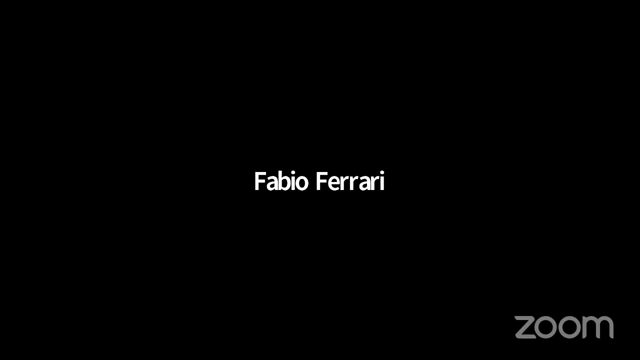 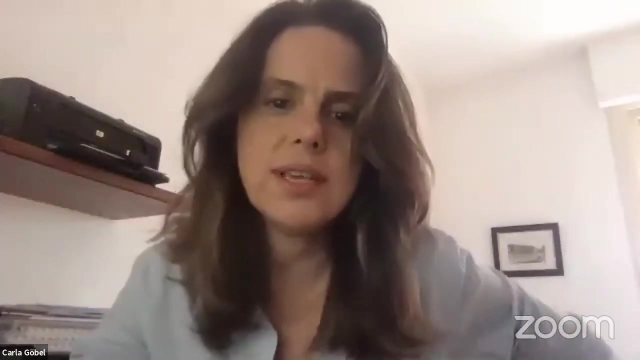 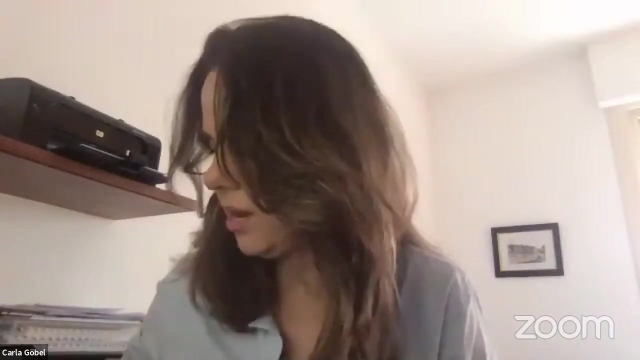 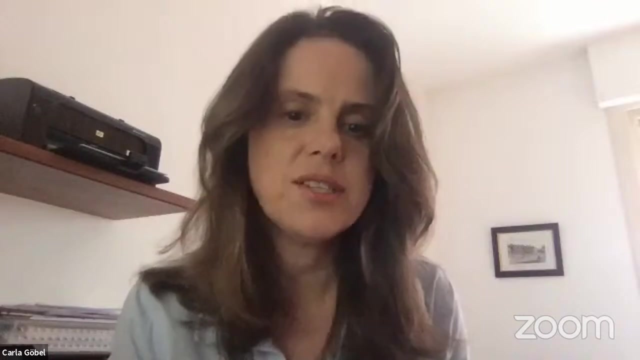 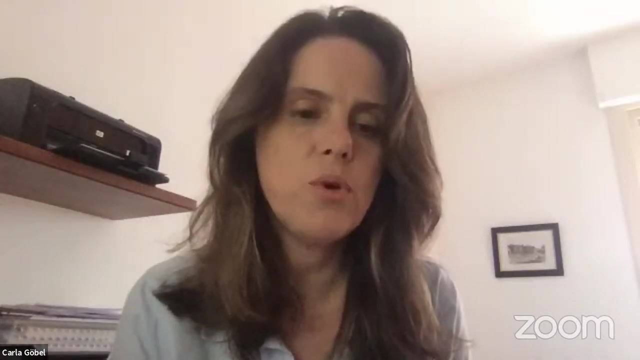 Thank you. The following message is best viewed on an oscilloscope. Thank you for watching. Thank you for watching. We and me and Karin will be sharing the session and we'll let you know when you have five minutes less and then two minutes. 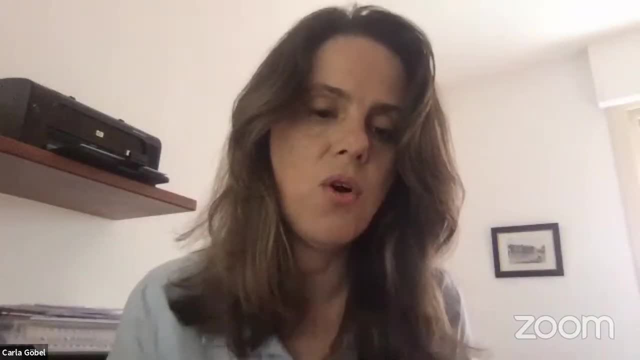 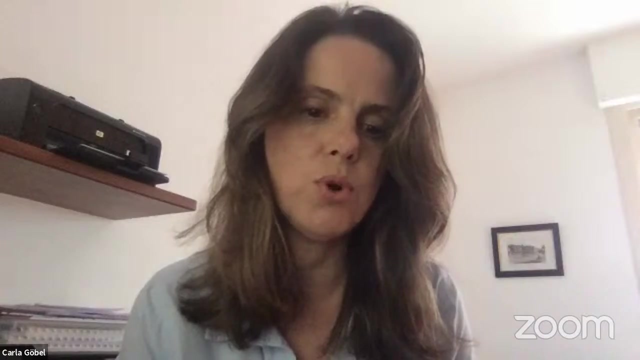 As I said just now, we prefer that you broadcast your slides and your image. So, if there are no problems with connection, this is best And, please, if there are more questions, If there are more questions that the time allow us to use, we encourage people to use the Mattermost channel, which is open. 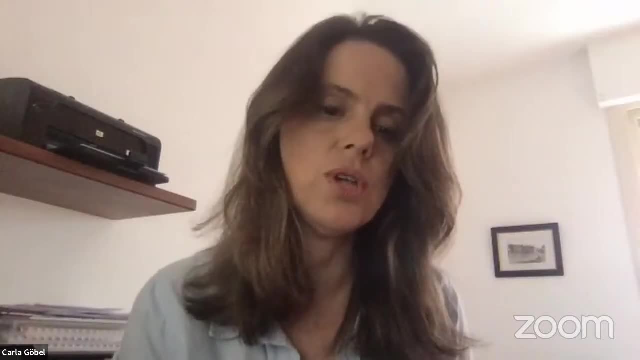 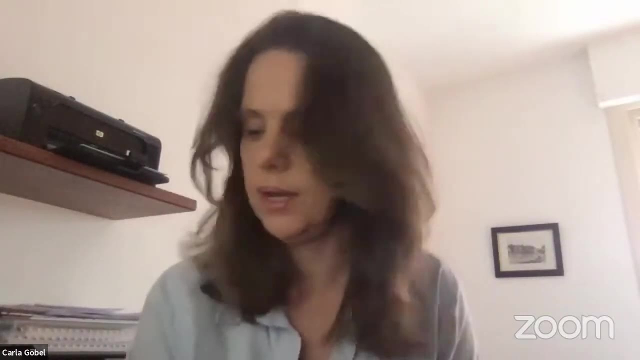 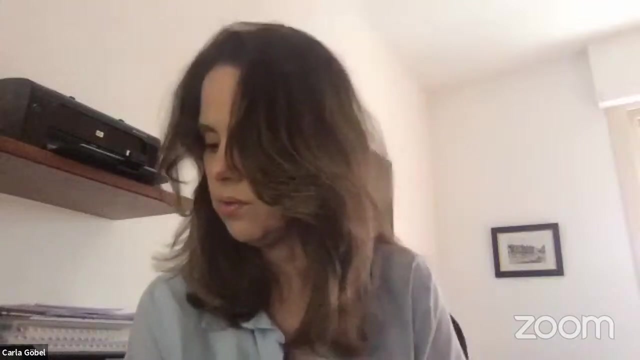 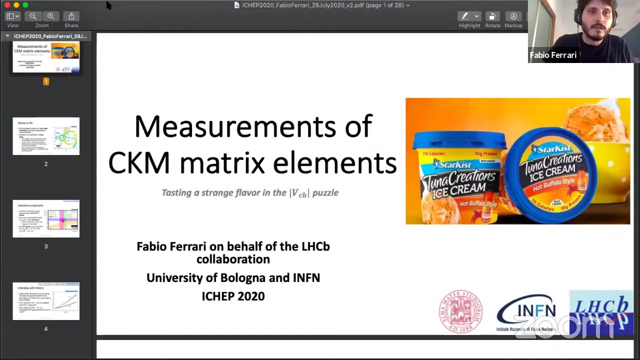 And at the end of the session today we also let the space for speakers to continue discussions if they wish. So I think we can begin. So I invite Fabio to start. Measurements of CKM metrics elements. Hello, So you should see the slides now. 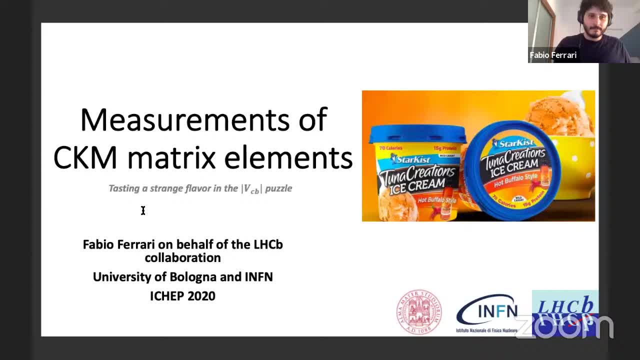 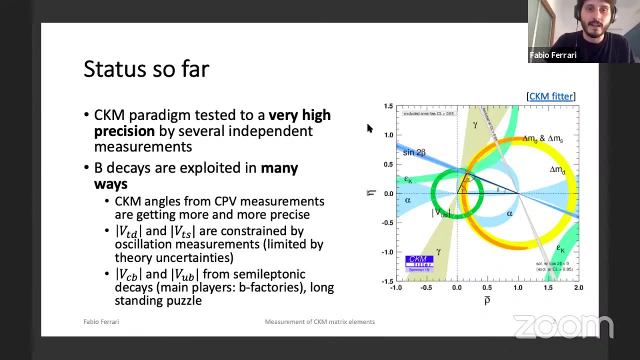 So good afternoon to everybody. Today I will report about measurement of CKM metrics elements on behalf of the CKM collaboration. So the CKM paradigm has been tested to a very high precision by several independent measurements, as you can see from the results of the CKM. 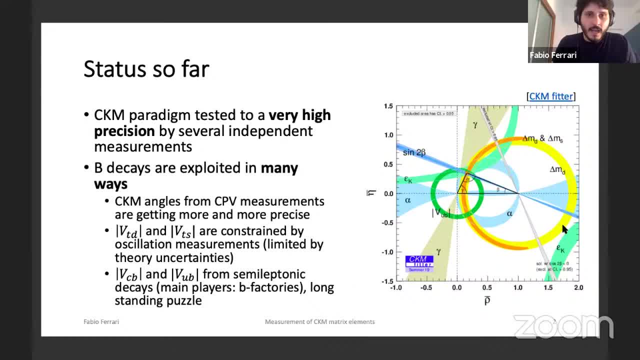 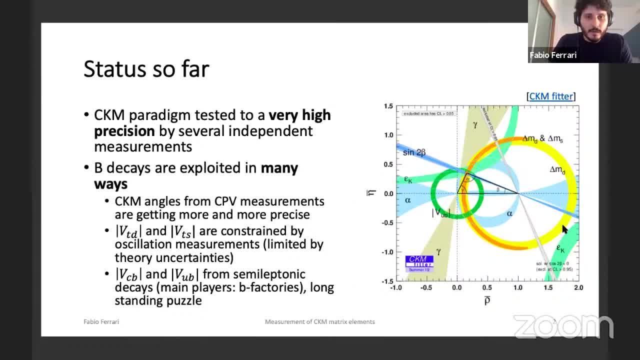 For example, CKM angles are obtained from CPB measurements, and these angles are getting more and more precise. The model of VTD and VTS are constrained by oscillation measurements, And the model of BCB and VUB are obtained from seelotonic decays. 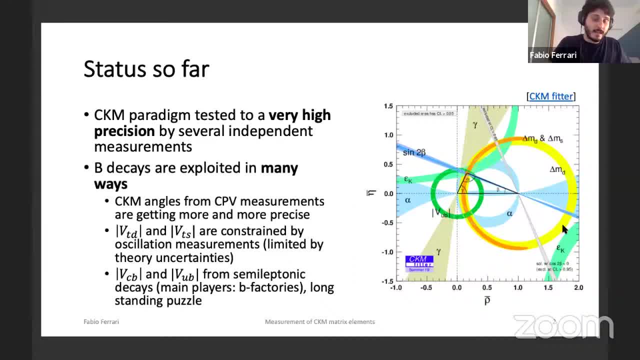 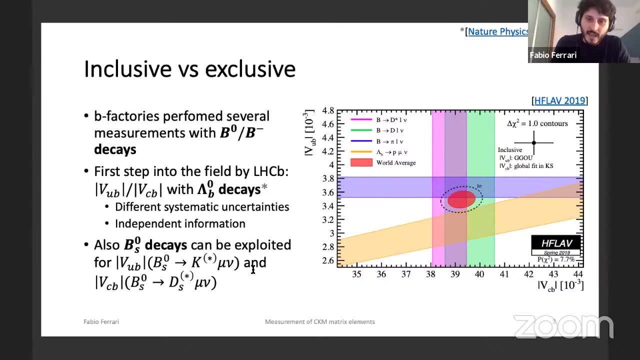 And in this case the main players been the b factories. and regarding bcp, there has been a long-standing puzzle that we'll try to summarize in the next slides. so, as you can see, in the right plot there is a tension of about three sigma between the, the, the exclusive and the inclusive determination of bcp. and, as you can as 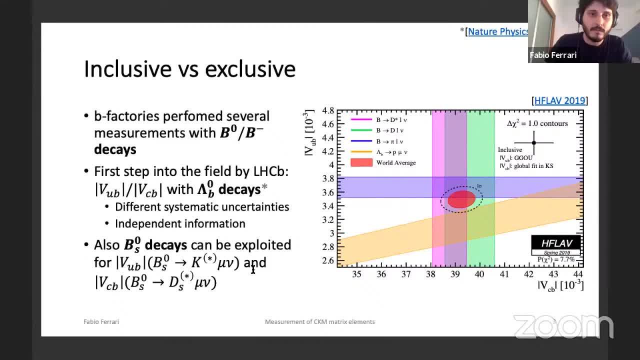 you can see from the bands, there are several measurements and the b factor performed. lots of measurements would be zero and be minus the case then. uh, some years ago there was a first step into the field by the cb collaboration with the measurement of bup, of the model of bup over pcb. 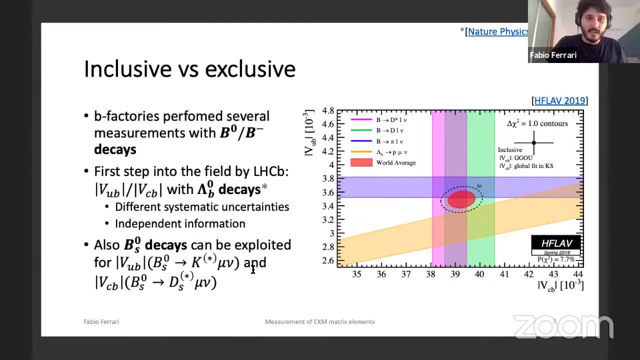 with lambda pdks. in this case, the measurement is affected by different systematic uncertainties and brings up independent information. so it's a very important measurement. but what they want to stress is that also b sub sdks can be exploited for the measurement of the model of ub and the and the. 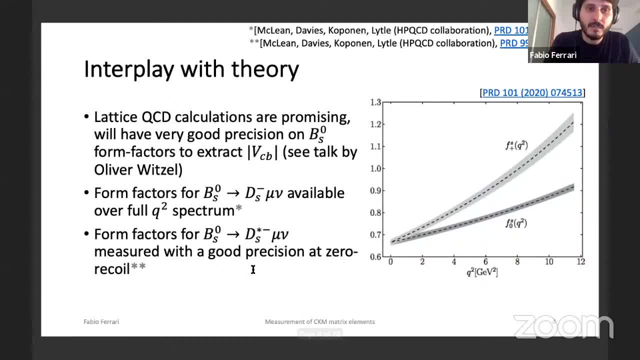 model of pcb. there is a a big interplay with with theory. uh, for example, uh, lattice qcd calculations are very promising and will have a very good precision on this best form factor to extract the model of pcb. and invite you to to follow the next thought by oliver uh, in our case the form factor for the b sub s to the best. 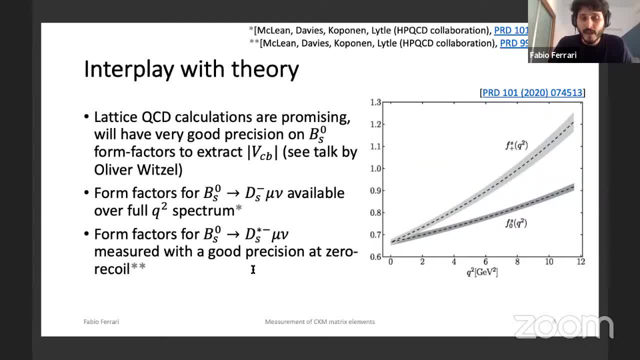 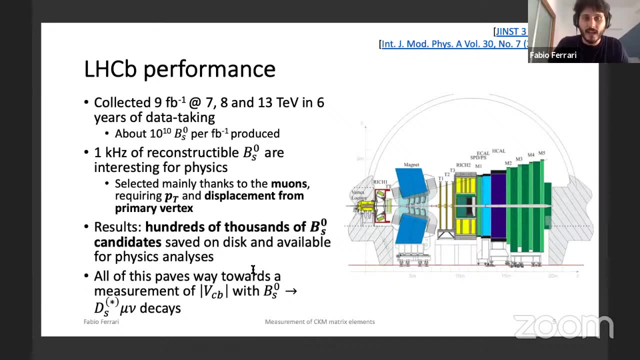 menu: uh are available. uh, over the future square spectrum. uh, whereas the different factors of the b semester- this is the best time we knew- are measured with a good precision only after zero. uh. going to the cb experiment: uh, the experiment collected about nine inverse phantom bands at the 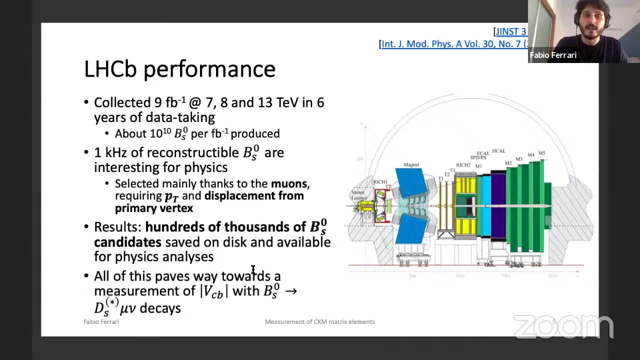 seven, eight and thirteen tv uh center of mass energy in uh. six years of data taking and we have about 10 to the 10 b sub s produced per inverse phantom. but uh, uh, we, we have one kilo else of reconstructed, reconstructible b sub s that are interesting for physics, and these uh. 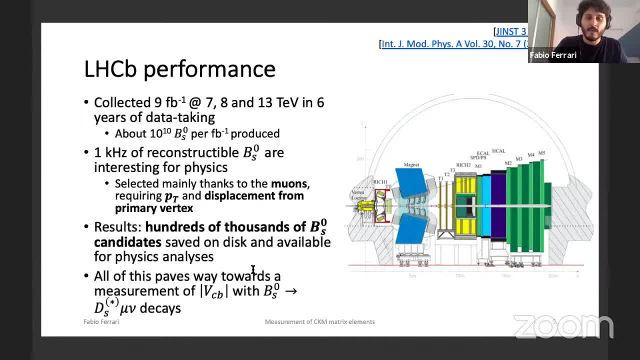 b sub s decays are selected mainly thanks to to muons, by requiring uh thresholds on the transverse momentum and displacement from from the primary vertex, and these uh results in a hundred of thousands of sub-s candidates that are saving on this camera are available for physics analysis, and all of this paves uh the way to towards a measurement. 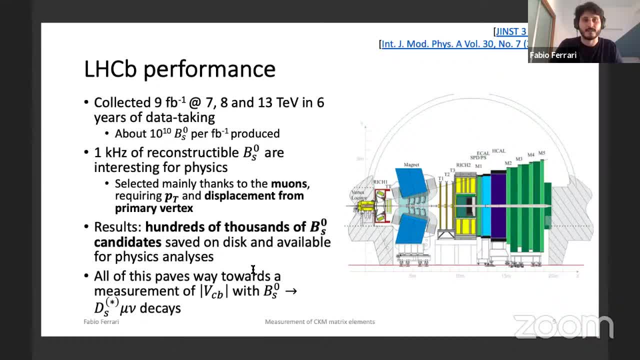 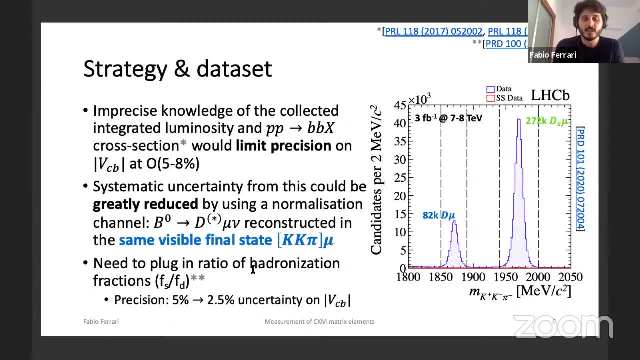 of pcb with the visa best to this abyss and this is the best time in the case. so just a few words on the strategy and the data set. so, uh, the, the, the implicit knowledge of, of the collective, the integrated luminosity. uh, end of the pp to bbx cross section would be a limiting factor for the. 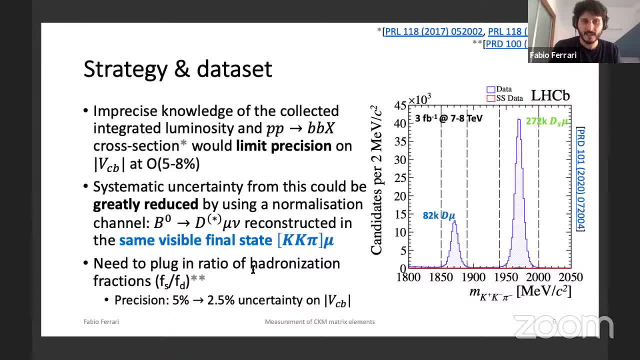 measurement of the model of pcb at the order of five to eight percent relative uncertainty. but this systematic uncertainty uh can be greatly reduced by by using a normalization channel and in this case we decided to use uh the b0 to d menu and the p0 to this time menu. 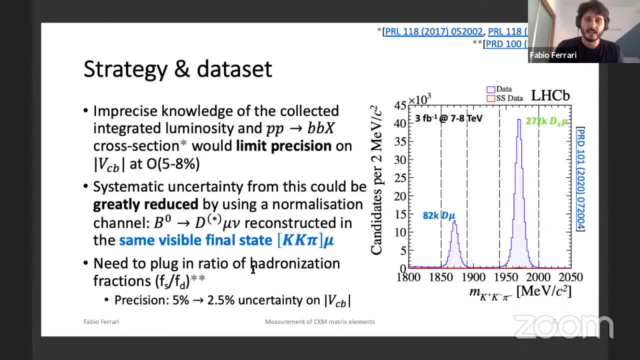 the, with the d reconstructed in the same visible final state as it is the best. so is the kk, pi final state and uh. but in this case we we need an additional ingredient, that is, the, the ratio of the organization fractions, uh, that is called the fs over ft and this is measured with a precision. 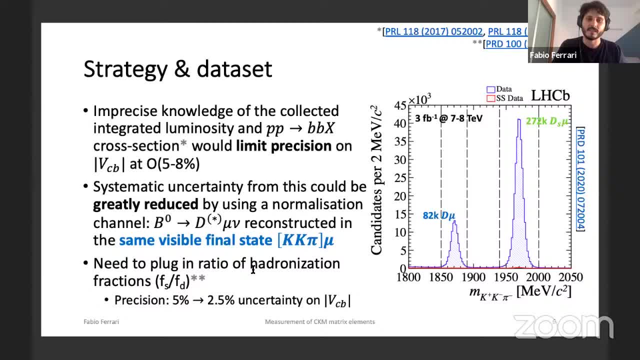 of five percent. that translates into a proceed uh 2.5 percent uncertainty on the model of pcb, and on the right hand side of the slide you can see the, the kk pi invariant mass spectrum. on the left side you can see the, the class with 82 000 uh signal candidates, and on the on the right side you. 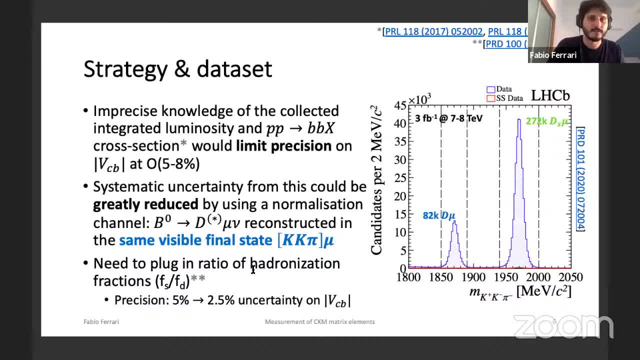 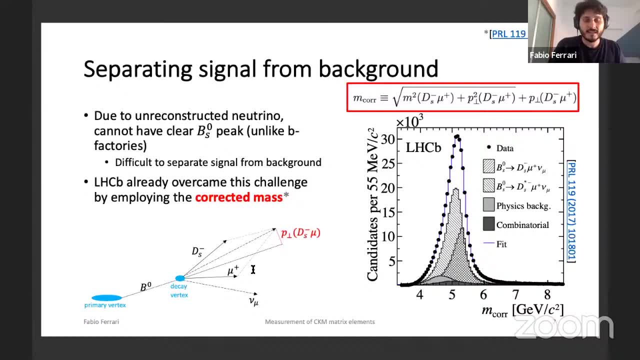 can see the the class with a 272 000 signal cabinets. uh, one challenge of this, this analysis, is to separate signal from background, and this is a very hard due to the reconstructed neutrino, since we cannot reconstruct a clear b sub s peak, unlike, for example, the b factories and and and. 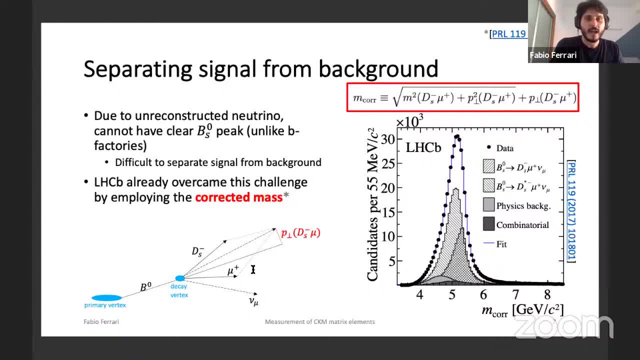 that is very difficult to separate signal from background, uh, but lacb already proved to be able to overcame this challenge by out by employing the cross-section of the signal from background to the correct mass. the definition of the correct mass is reported in the right rectangle in the. 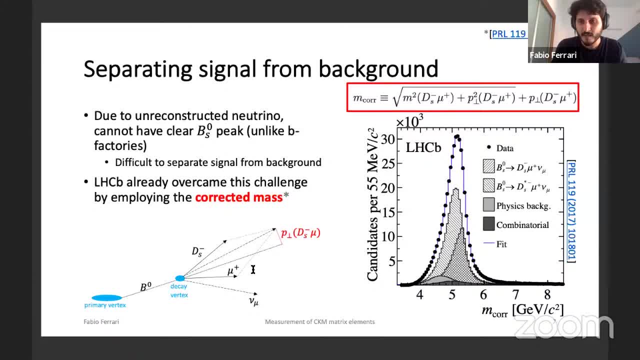 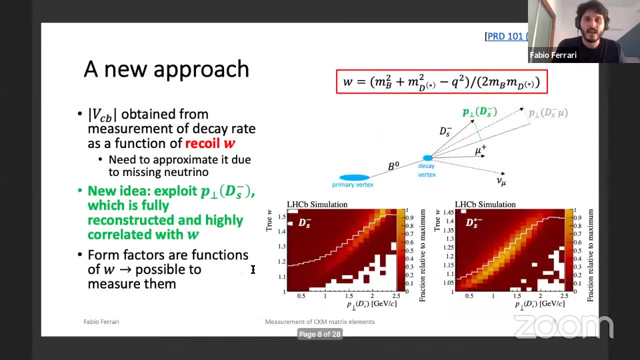 top right corner, and you can see here, for example, one previous analysis in which the the two b sub s decay channels can be separated both between themselves and also uh from from the physical physics and combinatorial barriers. uh, in this case uh vcps, can be obtained from a measurement. 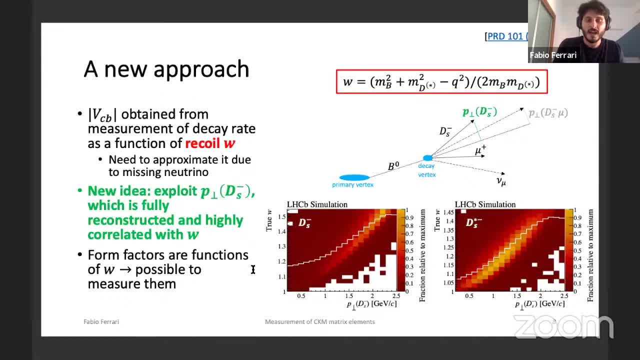 of the decay rate as a function of of the recoil w? uh. but this recoil w needs to be an approximate quantity, uh, because we have a missing neutrino in the decay chain. so the idea, uh, the novel idea of this analysis is to exploit the perpendicular component of the momentum of this disabase with respect to the b zero, uh, or this best. 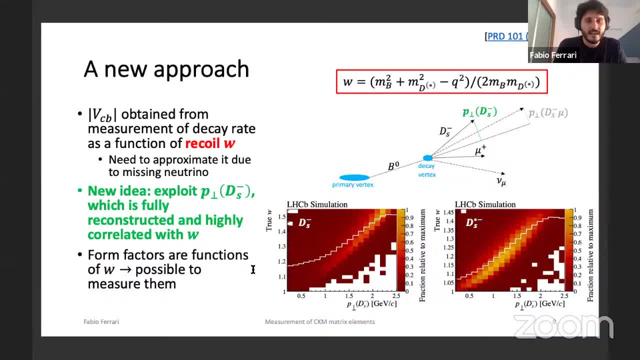 flight direction, as you can see from the sketch, and this quantity is fully reconstructed, so is a very good, goodly known and and it's uncorrelated with the w, as you can see from the, from the, from the top, from the, the bottom right uh plots where uh you can see the true w from simulation as a. 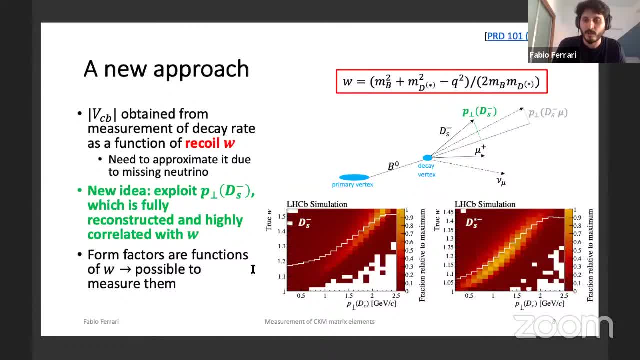 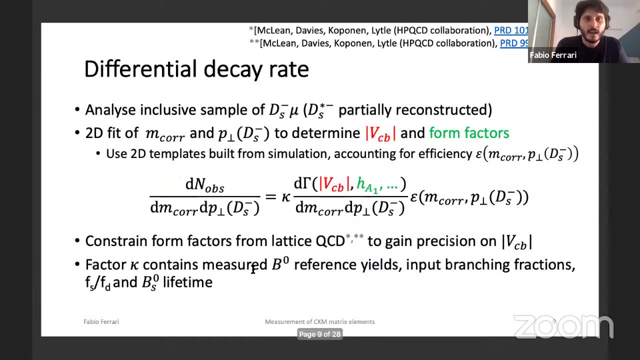 function of this uh, uh perpendicular variable, uh in a two-dimensional plane, and also the different factors are functions of w. so it's it's since we are sensitive, sensible to, to to w, it's also possible to measure the different factor of the decay uh. so we need to analyze the inclusive sample of this best new uh candidates, where the disabase 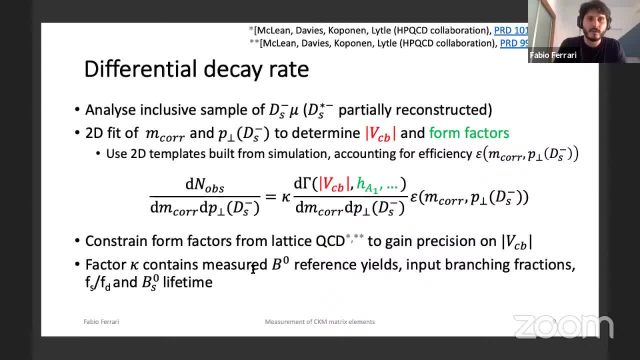 star is partially reconstructed and we perform the two-dimensional fit, the corrected mass and the perpendicular of the disabase in order to determine, uh, the model of bcb and the form factors simultaneously. and to do this we use two-dimensional templates that are built from a simulation and that, in that, account for efficiency, for the efficiency on the two-dimensional 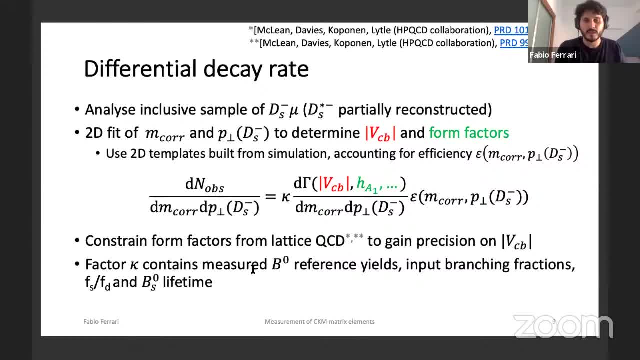 plane and and you can see the relation between the between the differential uh observant yields and and differential decay rate. that contains vcb and the four factors uh. we decided to constrain the form factors from lattice qcd in order to obtain uh, to gain precision on the model of bcb. 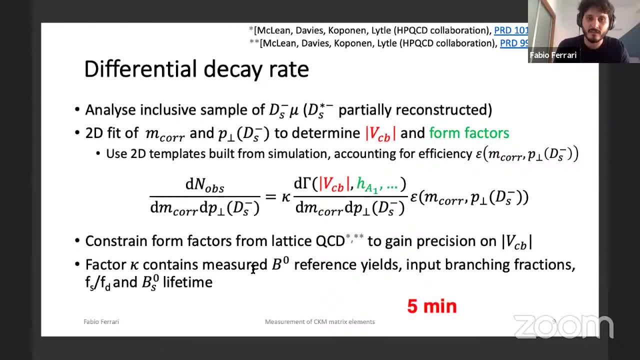 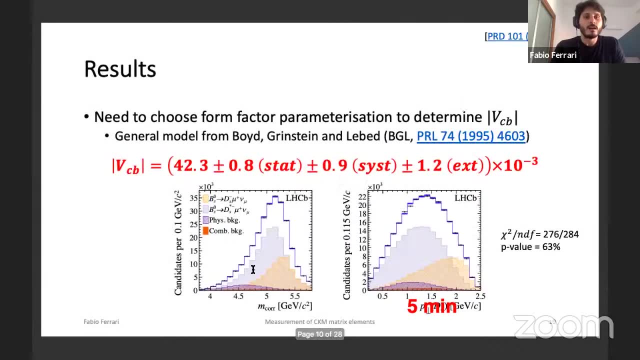 and the. the factor kappa that you see in the, in the formula in the middle of the slides uh. uh contains the measured with zero reference yields, the, the important, the, the input branching fractions, uh, the ratio of the transition fractions at s over fd and the bsfs lifetime going to the results. so we needed to choose a factor. 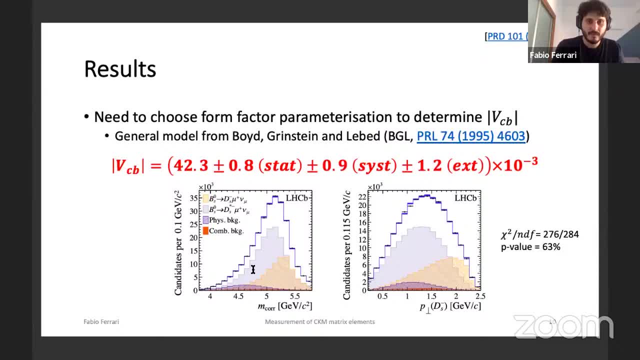 parameterization in order to determine bcp and we the first choice was was a general model from boyd greenstein and lepid, that is, a commonly called bgl, and here you can see the the results for the model of vcb and the two fit projections, on the left for the corrected mass and on the right for 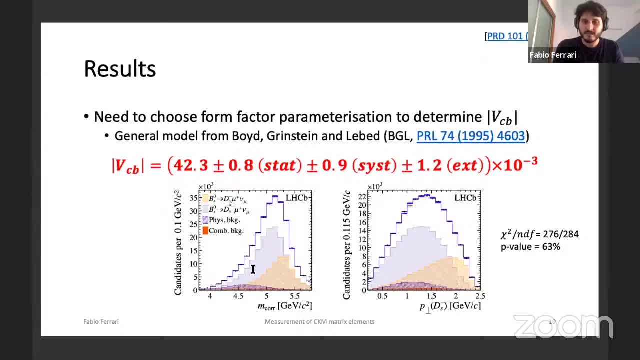 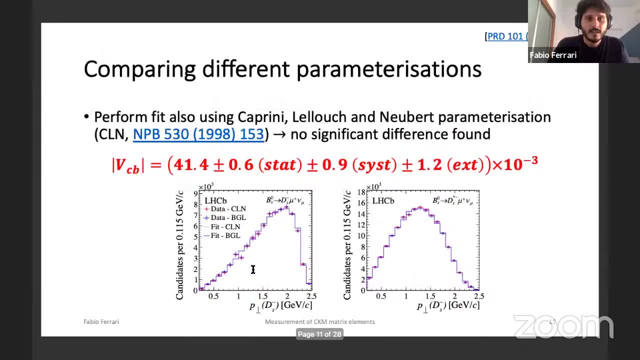 the perpendicular uh uh momentum and you can see that the fit quality is pretty good and we have a p value of 63 percent. then we also performed analysis using a different form factor parameterization. in particular, we decided to use the caprini-lelluk and neubert parameterization. that is called cln, but as you 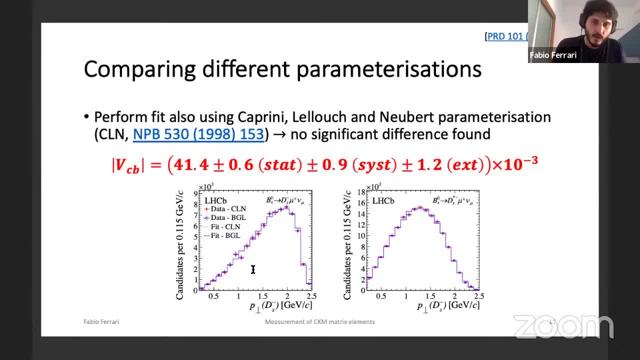 can see from the projections in the two bottom plots. uh, the one on the left is for the b sub s to the sub s menu and the one on the right is for the b sub s to the sub s star menu. you can see that the fit results and and the data compared between cilin and bgl, they are almost 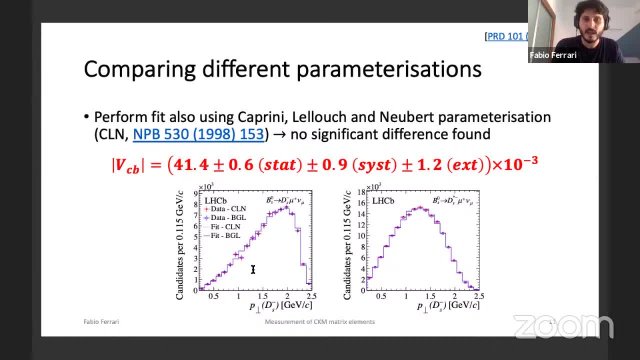 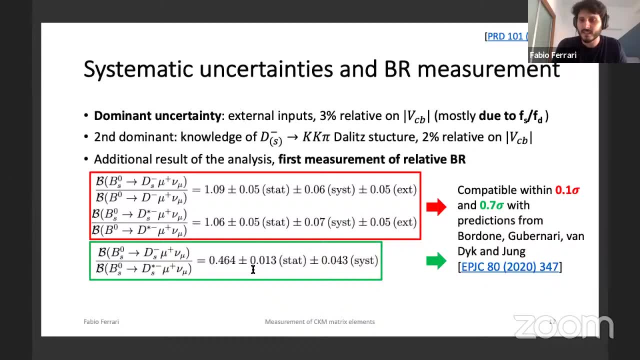 identical, so that there are no significant difference found between the two parametrizations for the measurement. the dominant uncertainty is due to external inputs and is a three percent relative on the model of bcp, and this is mostly due to fs over fd and the second one dominant. 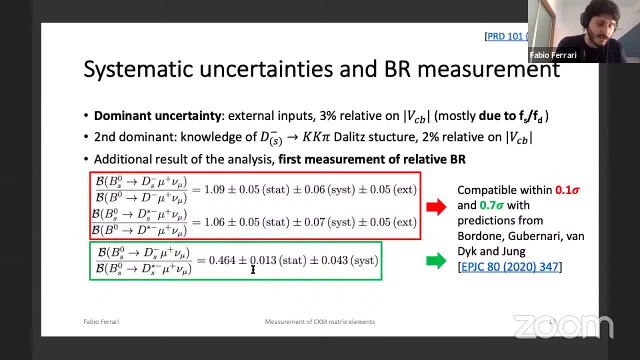 uncertainty is the knowledge of the d and the sub s k k pi by a structure that brings up two percent on PCB. Some additional results of the analysis are the first measurement of the exclusive branching ratio, that that you can see here, and also the the ratio of the two estuaries. branching ratios. 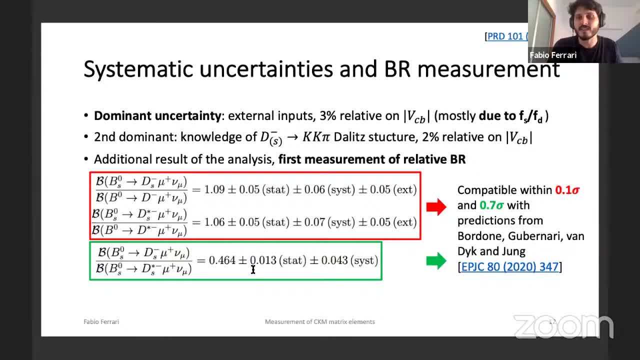 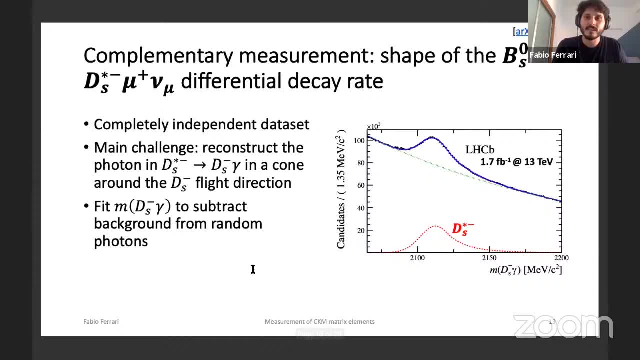 and these results are compatible, within 0.1 and 0.7 sigma, with prediction from Bordone-Gruenari and Van Dyck and Young. Now I go to another complementary measurement, that is the shape of the Bissabeste-Bissabeste time-renewed differential decay rate. This measurement is: 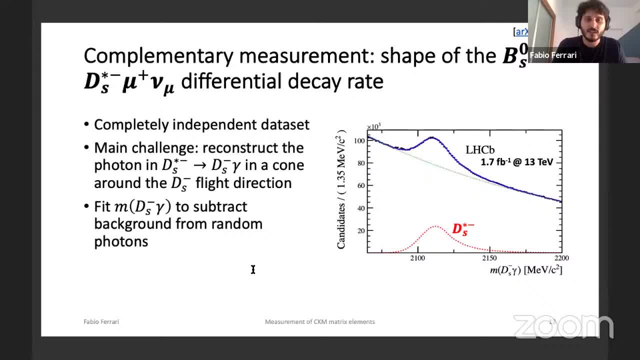 performed in a completely independent data set, and the main challenge in this case is to reconstruct the photon in Bissabeste star to Bissabeste gamma decays in a cone that is around the Bissabeste flight direction, and then one performs a fit with Bissabeste gamma in variant mass in order to 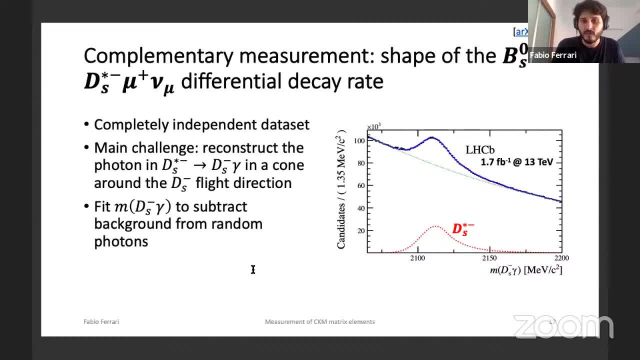 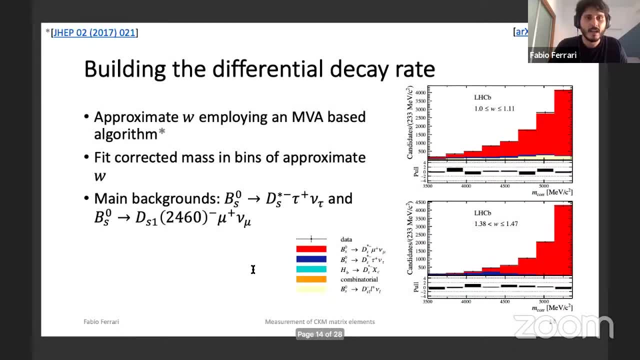 subtract the background that is due to random photons in the vents, and on the right part, on the right plot, you can see the results of this fit. Then one needs to approximate the W by employing some MVA based algorithm and fit the correct mass in means of. 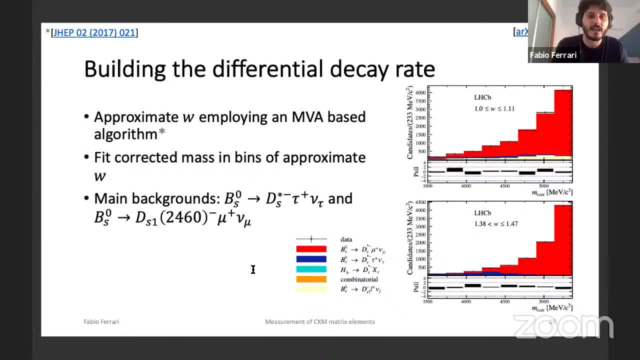 the approximate W in order to obtain the differential decay rate. and on the right part of the slide you can see two fit projections for two different bins of W and you can see that in these cases the main backgrounds are due to the Bissabeste star tau new decay. 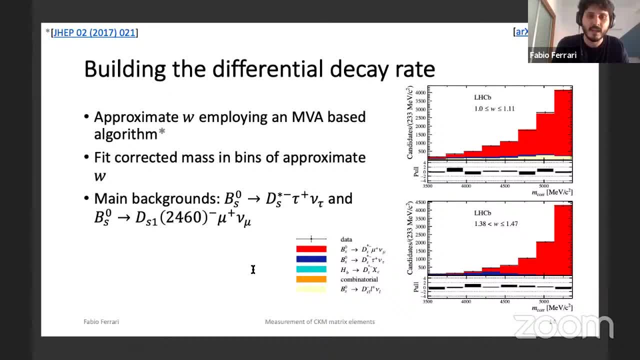 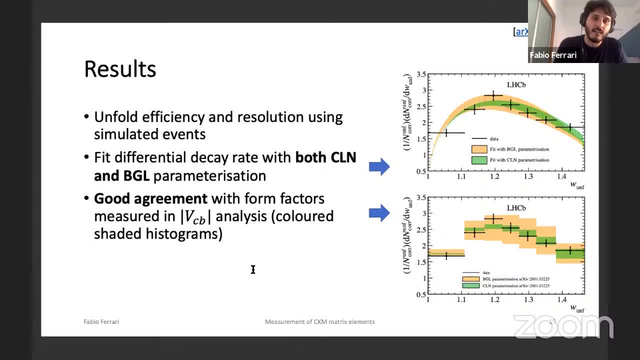 and this Bissabeste to this ds1 2460 minimal decay. The result for the analysis can be obtained once one unfolds the efficiency and the resolution by using simulated events, and then one can fit the differential decay rate with both, with both the CLN and the BGL parameterization, and you can see the results of this fit in the top right plot and 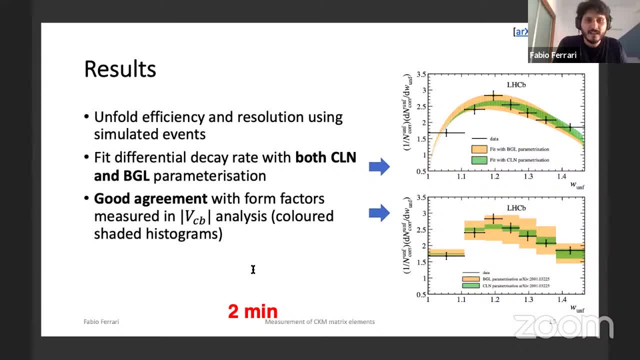 also another important thing to notice is that this analysis shows a good agreement with the four factors that are measured in the in the analysis that I presented Before, so the BCB analysis that are represented as a shaded histograms in the in the bottom right plot. 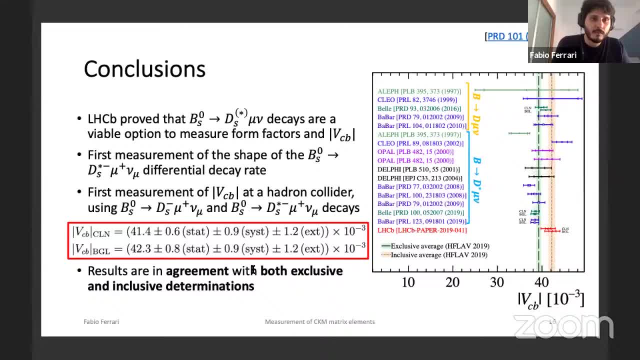 So, coming to my conclusions, the LCB collaboration proved that the Bissabeste to ds minu and Bissabeste to ds star minu decays are a viable option to measure the form factors and the model of BCB In particular. today I presented the first measurement of the shape of the Bissabeste to ds star minu. 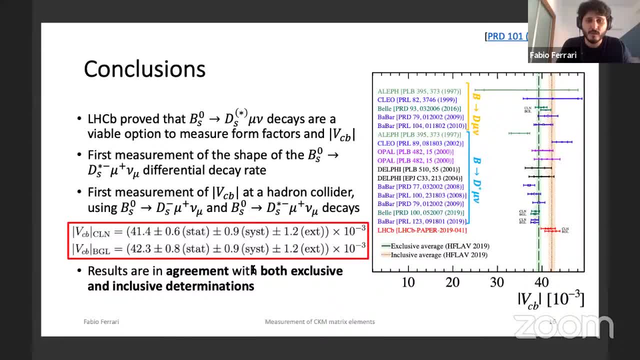 differential decay rate and the first measurement of the model of BCB at the Hadron collider using Bissabeste to ds minu and Bissabeste to ds star minu- decays. and in the red box you can see the the results obtained in the two different parameterization, the CLN and the BGL parameterization. 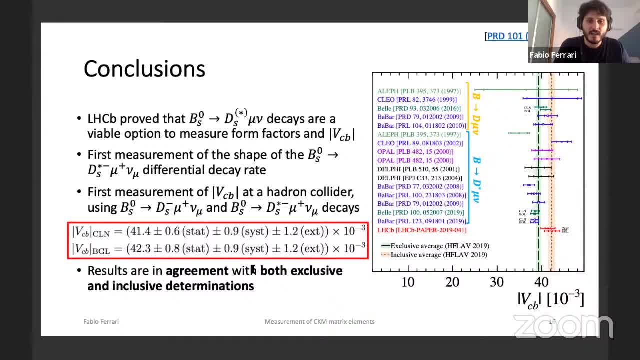 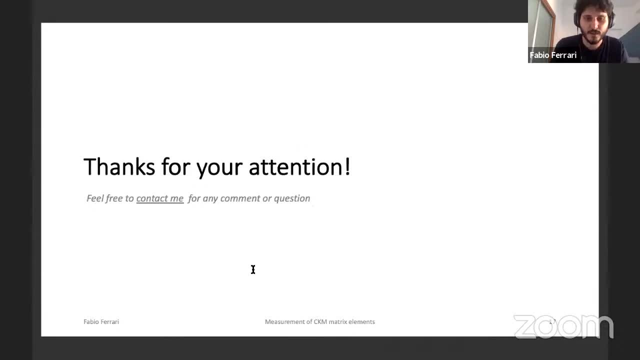 and those results that we obtain are in agreement with both the exclusive and the inclusive determinations, as you can see from the right plot that collects all the measurements of the Bissabeste to ds star minu As to this measurement of BCB performed in the last 20 years. and that's all from my side, thank you. 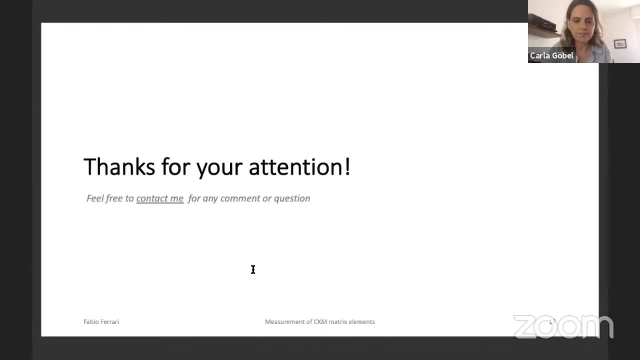 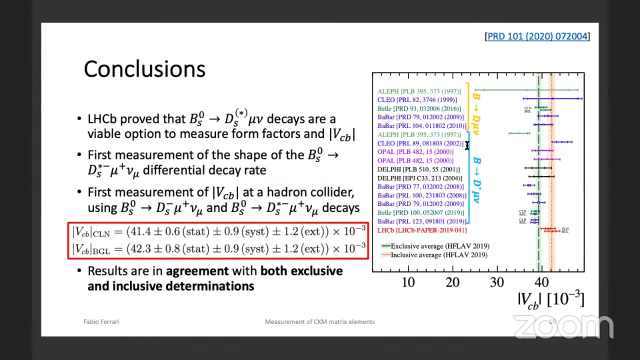 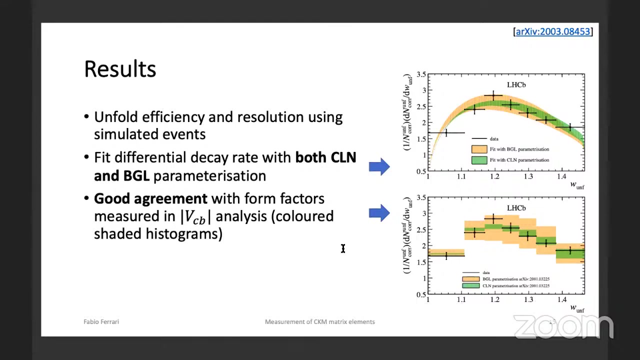 Thank you, Fabio. Questions for Fabio. You can raise hands or just jump in. Yes, Doris, go ahead. Can you go back to page 14? Where we show the distribution of over recoil? yes, 15. sorry, I was talking about yeah, it doesn't matter. yeah. 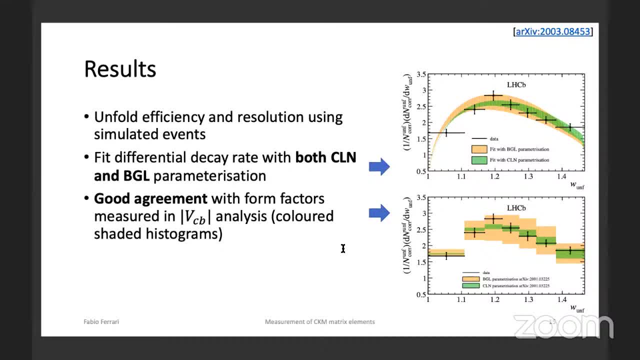 I was wondering how you are, how, whether the lattice people will give you a distribution similar to these plots. Sorry, that is QCD, that is QCD. so when we will get the prediction from lattice QCD on this? Yeah, in this, this recoil variable. 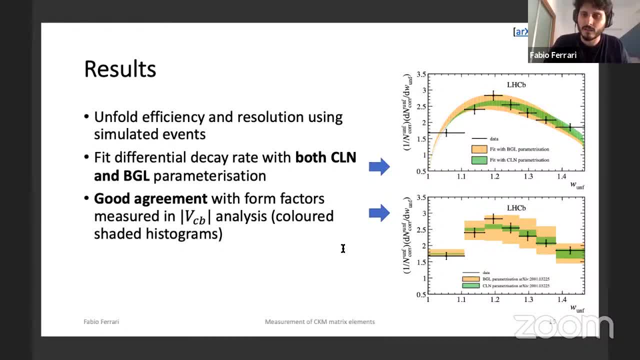 I'm not sure that on the timeline of this or if we already have a prediction on this. actually, I'm not sure we have prediction for sure on the form factors that we have and and by comparing them with the with predictions, they agree pretty well, but I have. we have also to say that uncertainties are. 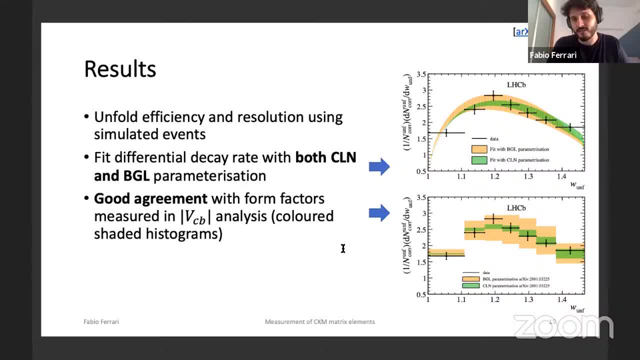 pretty big at this stage. so it is not a very precise that but, but, but but the prediction from four factors. they agree with the, with the LACD results, but that I can tell you. okay, thank you. Okay, you can go to the next question, someone, okay, oh, yes, Christoph. 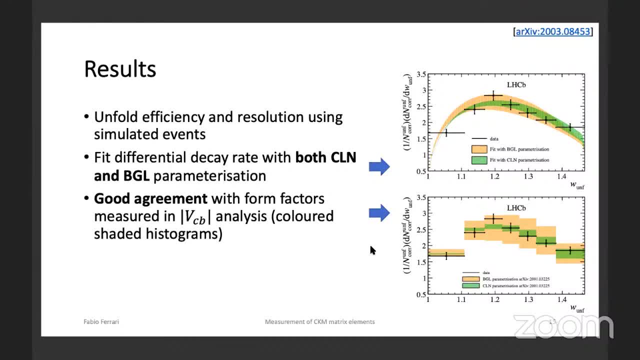 Yes, can you hear me? so I have a similar question. This measurement of PS to DS mu does it cover the whole Q, square or W range, or is your sensitivity concentrated in a particular range and does it match the lattice prediction? do you have a good overlap or do you have to make an assumption to connect the poles? 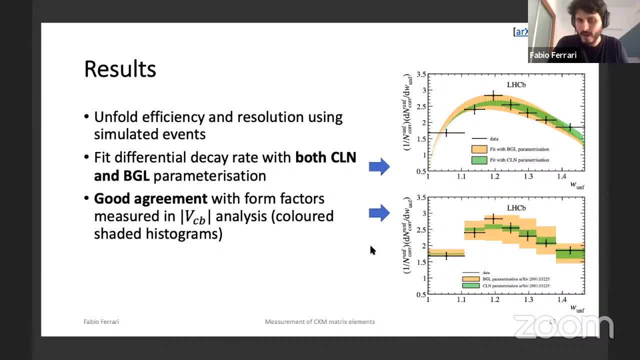 So so you are referring to this spectra in Q square? Yes, exactly, Okay. so as far as I know, the the W range is from 1 to 1.5 approximately, and this can be translated directly to Q square. so I would say, yes, this is a measurement of the full spectrum of Q square. 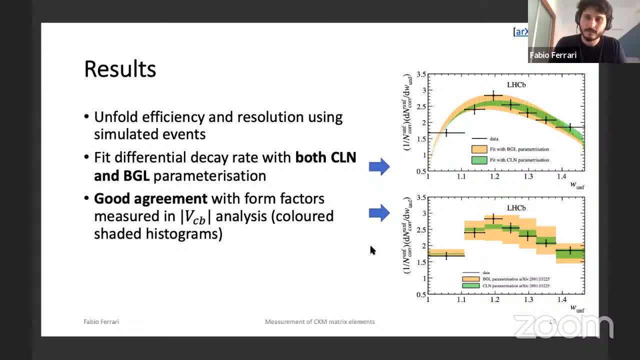 that you that that you can have? yes, And the lattice prediction is also over the full range. or is it only in a particular For the for the B sub s to D sub s style menu? Yes, yes, Yes, yes. not sure if we have lattice prediction just at zero recoil, that is q squared equal to zero. 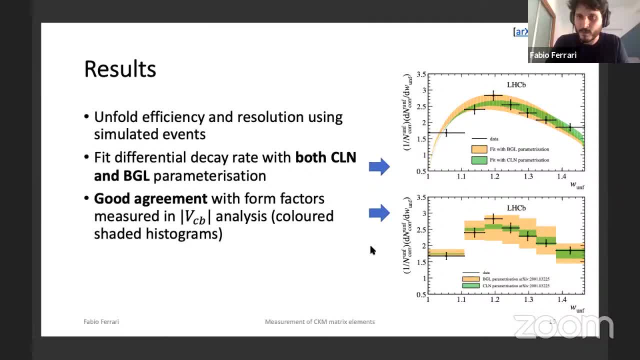 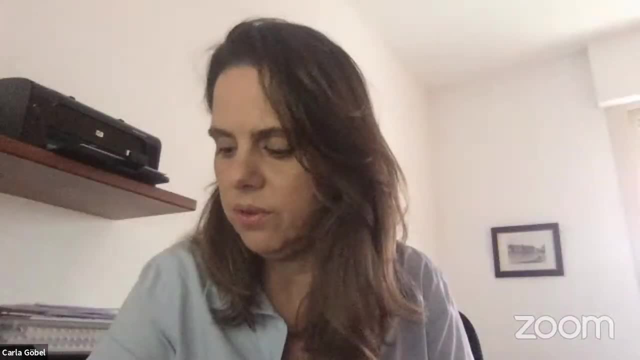 or on the plus pattern. probably Oliver in the next talk can be more precise than me, but but I'm not completely sure on this. thank you, no problem. okay, thanks, Fabio, again, we can move on. the next talk is from Oliver Witzel on non-pertubative calculations of form factors. 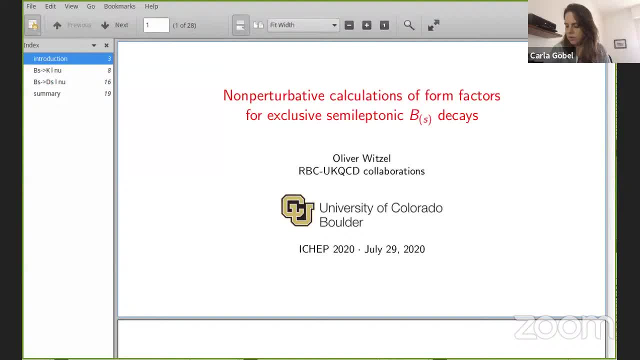 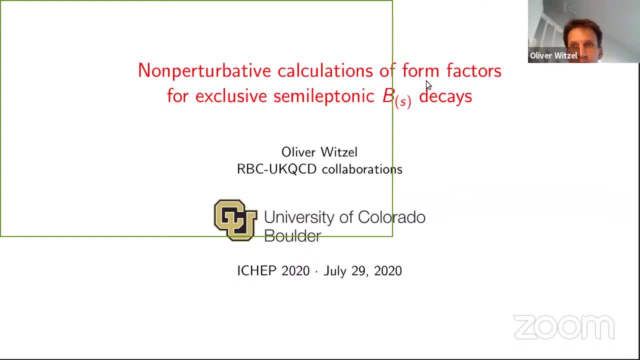 for exclusive semi-leptonic v sub sdks. okay, can you see my screen? yes, okay, so sunny greetings from Colorado and thank you. thank you, Fabio, for the nice introduction. so I will continue talking about v sub sdks, but from the latest perspective to calculate. 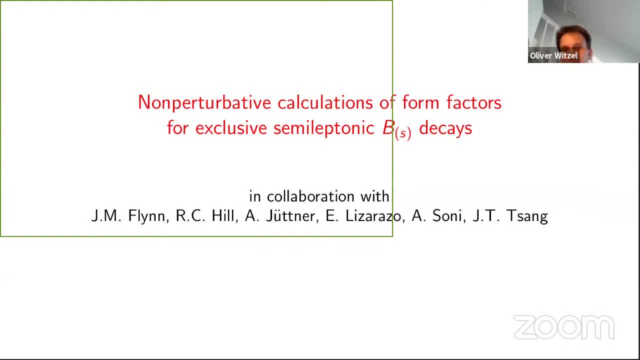 the non-perturbative contributions and, first of all, I would like to thank my collaborators on this project, in particular, Jonathan Flynn, ryan hill, Andreas Jutner, Edwin Lidhra, Zu Amirjeet Sonny and Tobias Zang. so, as you all know, we are. 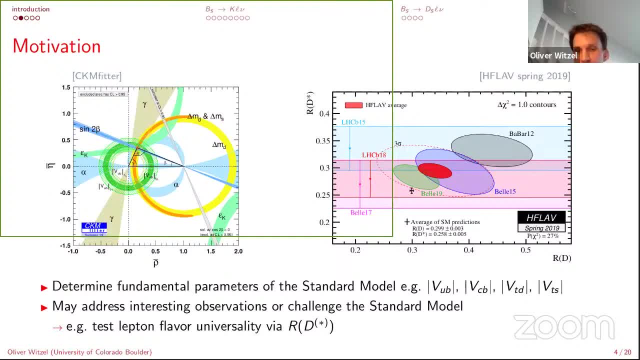 interested in determining fundamental parameters of the standard model, like the ckm matrix elements. we are also interested in addressing observations or challenge challenging the standard model which are interesting. so in particular the laptop flavor, universality And the ratios Rd and Rd star have caught a lot of attention. 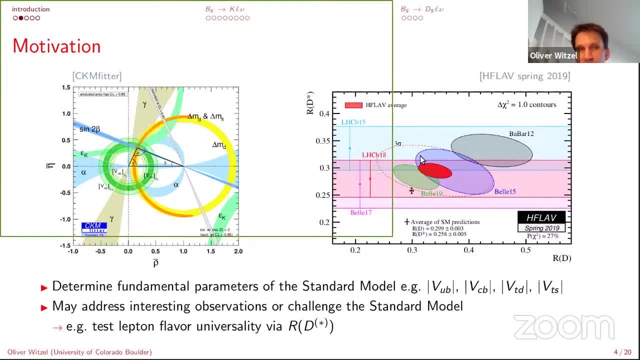 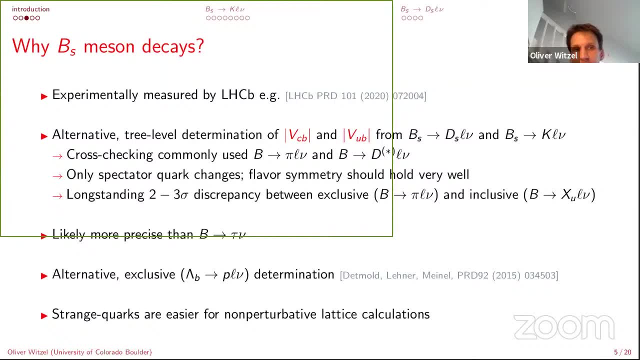 recently And so far we are looking at this typically for semi-laptonic BDKs, but we can also look at that for B sub SDKs And, as we just learned, LHCb can do a wonderful job in measuring these DKs. 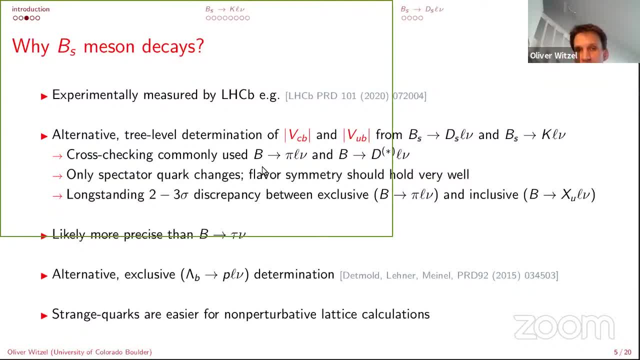 And so we get an independent cross-check on the commonly used channels B2 pi Lnu and B2 D star Lnu. if we look at Bs2 dslNu and Bs2 klNu, for example, Since we are only exchanging the spectator quark. 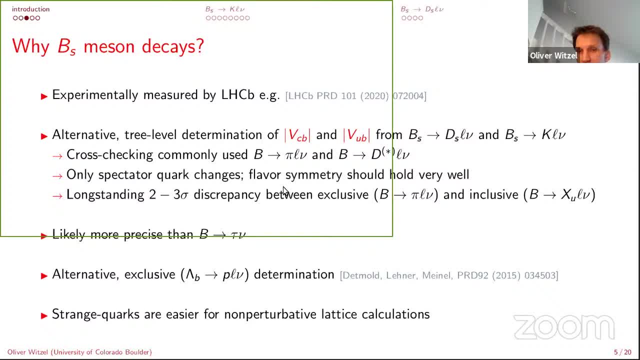 flavor symmetry should hold very well And we expect that this is really a good cross-check on what we have And we can also hope to address these longstanding discrepancies between exclusive and inclusive determinations. Likely, looking at B sub SDKs will be more precise. 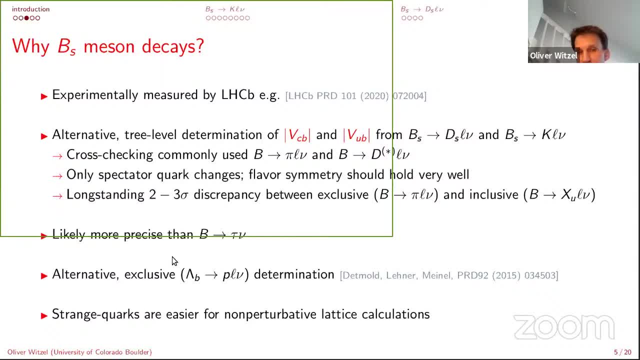 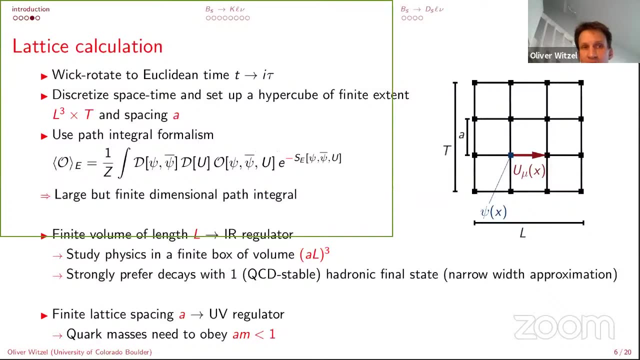 than B2 tau nu DKs, And it's. a further alternative is to look at the baryonic DKs of a lambda B going to a proton. From the lattice point of view, looking at strange quarks is definitely favorable because they are making the lattice calculations easier. 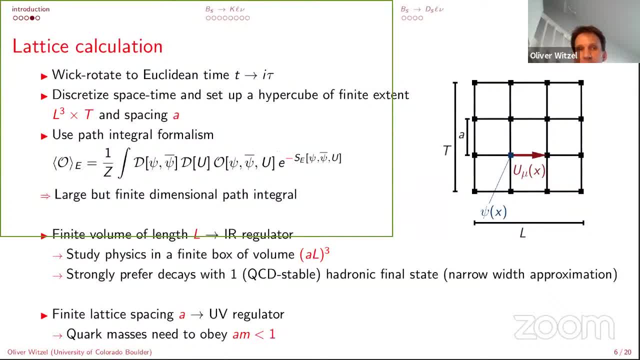 Now basically a one-page summary of the lattice calculations. We work in Euclidean time, So we do a wick rotation and discretize space-time to a rectangular grid, And then we can turn the path integral into a large but finite dimensional job, which we can. 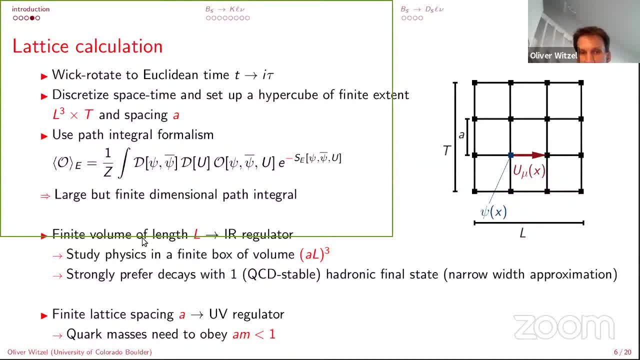 tackle with statistical methods. However, we do have the length of the box as an infrared regulator And at the same time the lattice spacing works as a UV regulator. So we have to obey constraints, that the light quarks are happy, not feeling too squeezed in the small box. 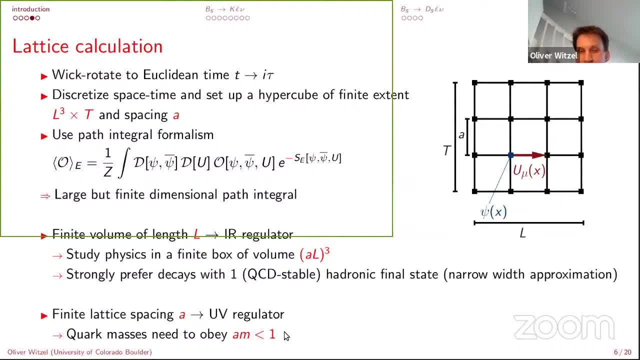 But at the same time we do need to have high enough resolution to deal properly with the heavy quarks, in particular with the bottom quark and the general rule of thumb That the quark mass and lattice units needs to be less than 1.. 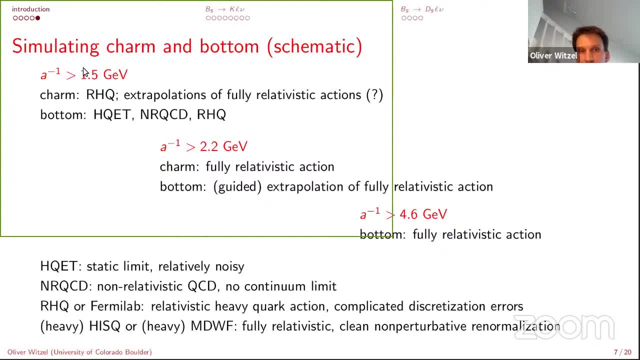 So, depending on the lattice spacing, whether it's coarse or more fine, we have different concepts on how to deal with a charm and bottom quarks, And while for the bottom quarks I'm going to refer to a relativistic action in this work, 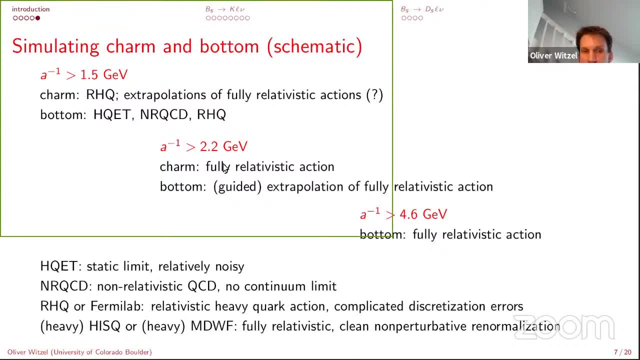 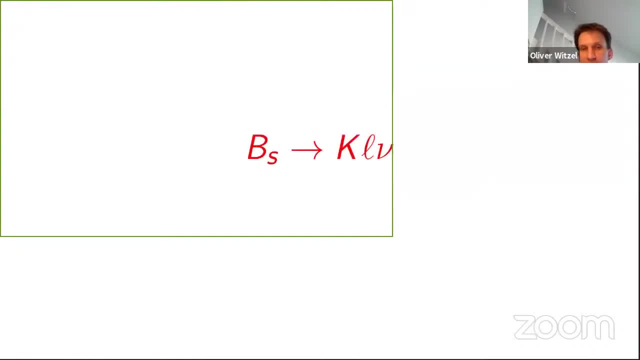 we are trying to, we are using a fully relativistic action for the charm quarks in the B-sub-S2DS case. Now let me jump right away. So the first decay. so looking at B-S going to K-L-NU. 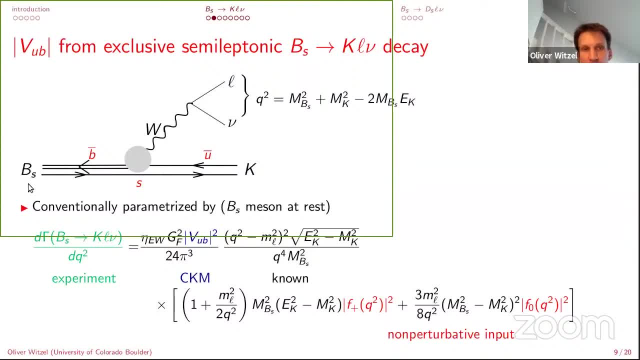 And the process is sketched here. So we have this range quark which just goes unchanged, And then we have the bottom quark which, on the left, forms our B-sub-S state, And it decays under the exchange of a W to a U quark. 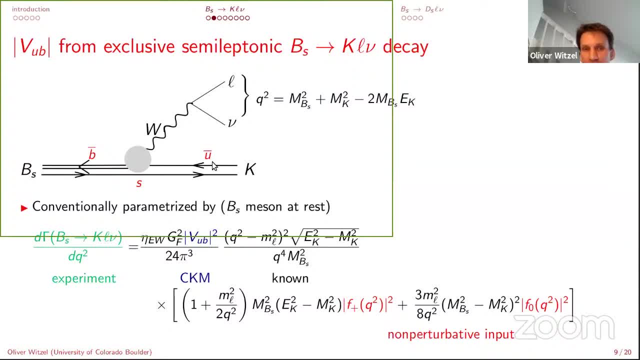 and forms the kaon. The W itself will give us a lepto-neutrino pair. So this is the charge, current decay Tree level in the standard model, And the experiment will determine the branching fractions And then we can parameterize that. 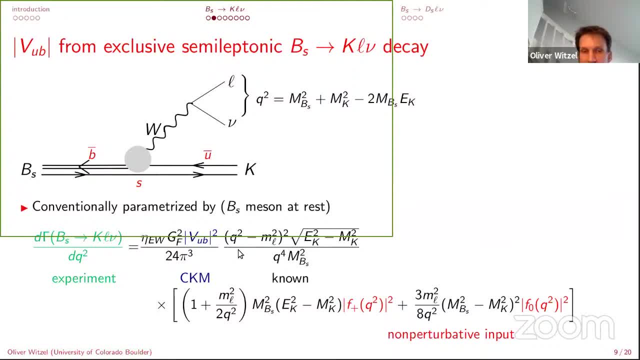 in terms of known coefficients, plus the CKM matrix elements highlighted in blue VUV. And in addition we need to have the form factors F plus and F naught, which are the non-perturbative inputs, So they parameterize the contribution. 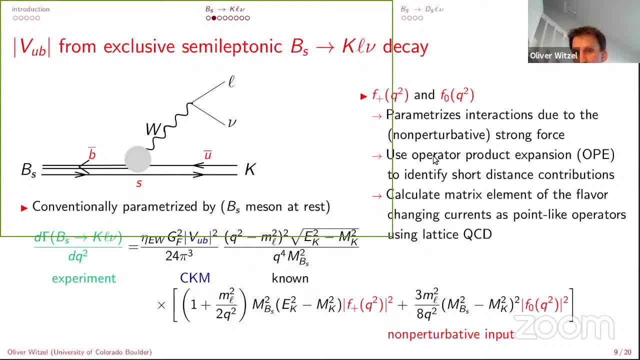 due to the strong force, And we use an operator- product expansion- to identify the short distance And then we can calculate the contributions. And these we can calculate on the lattice by determining matrix elements for the flavor-changing currents, And that's basically a point-like operator. 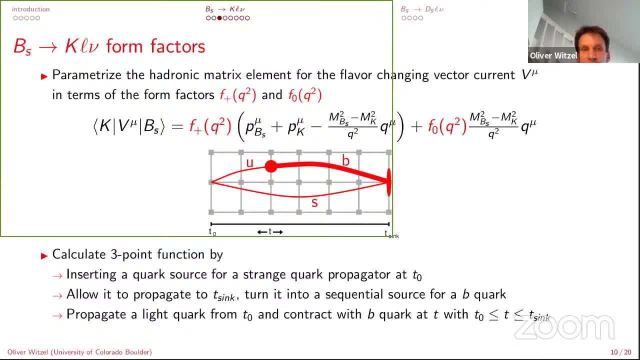 Schematically. this is then how we really enter the lattice calculation. So we want to calculate this matrix element a, B-S changes under the vector current to a kaon That can be parameterized by the two form factors we defined earlier. 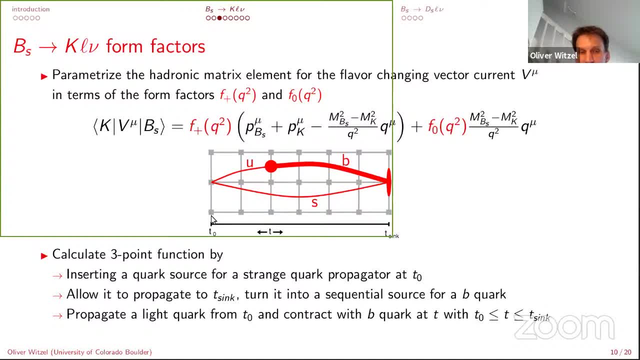 And in the picture it's shown as we have a source on the time slice, T0. We let the strange quark propagate in time to a time later- T-sync. At that point we create a so-called sequential source for the B-quark which goes back in time. 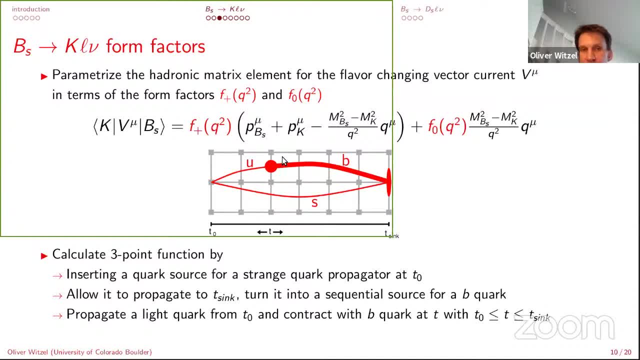 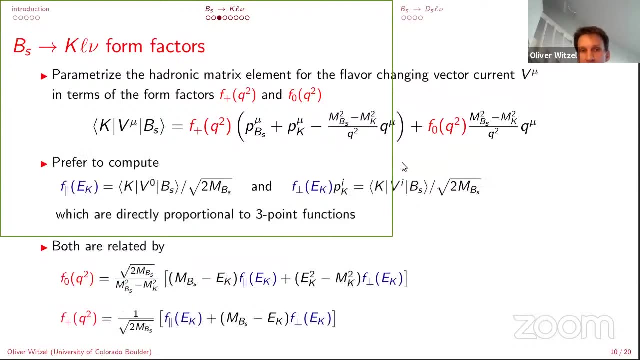 and is contracted with a light quark also originating from T0. And at this point here we have the operator insertion And we can then compute the signal and vary the range between T0 and T-sync to determine the signal of the three-point function. 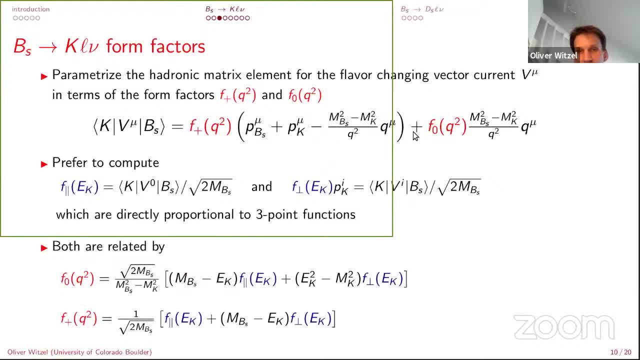 Now on the lattice, we are having discrete symmetries. So instead of directly computing F plus and F naught, we prefer to compute F parallel and F perpendicular, which are then just the temporal and the spatial directions in the three-point function. 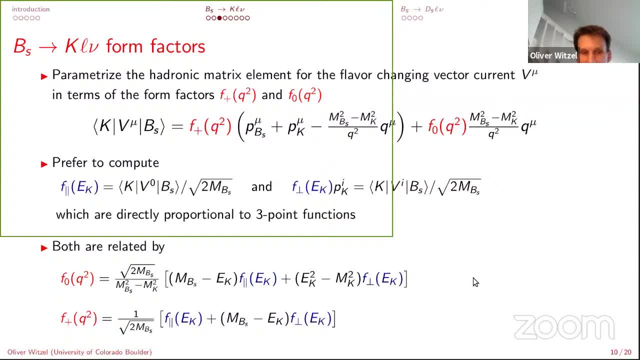 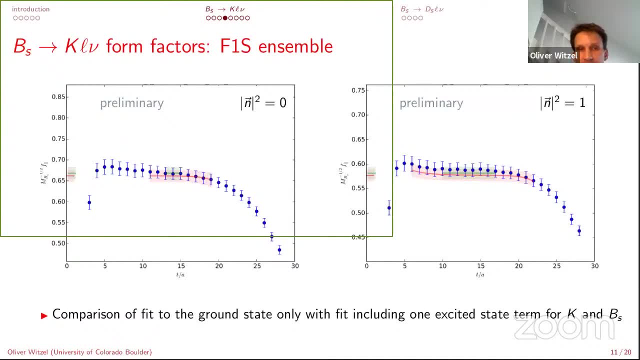 And both are, however, linearly related to F0 and F plus, which are then on the bottom, And to give you a picture of how this looks like, this is an example for our finest ensemble. In this case, the B meson is on the right. 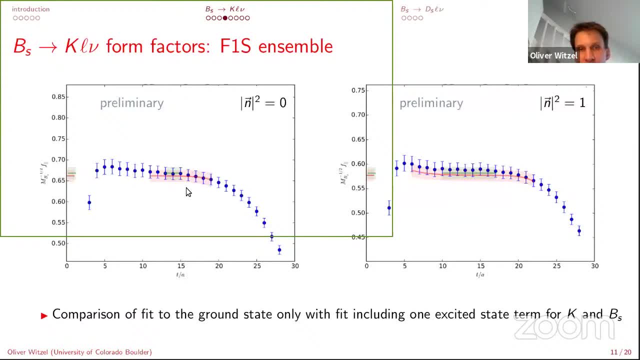 The kaon is on the left, The blue data points are the signal we are observing, And then we are looking for the flat range in between. And on the left this is F, parallel at zero momentum, And on the right it is at one unit of momentum. 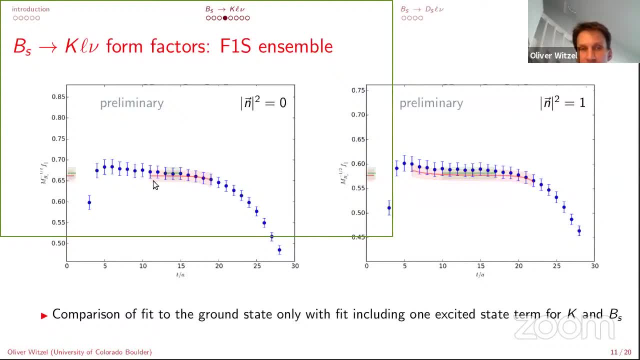 We then look for the flat range And we can account for so-called excited states contributing. So you see a little bit of curvature. It's better resolved on the left, where we account for these additional states in the fit function to determine the plateau. 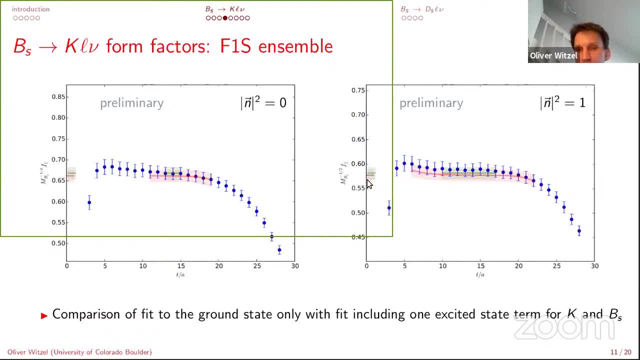 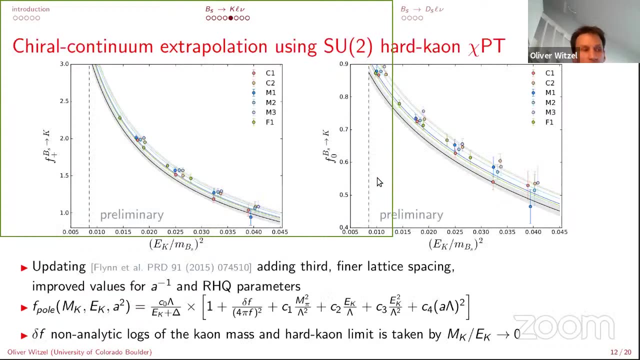 And what is shown on the left here are how the two determinations of just fitting the ground states or including the excited states perfectly agree, which gives us a handle on the systematic of the signal we are determining. Now we have to do this exercise for all the ensembles. 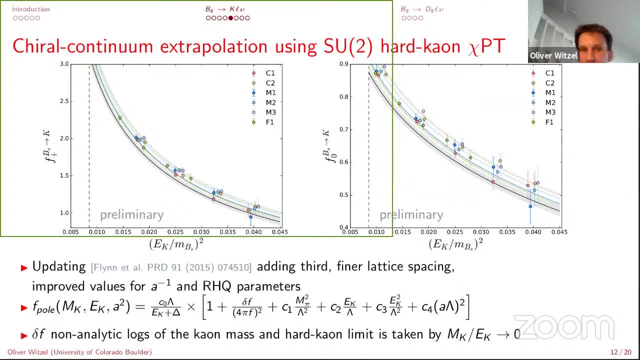 we are using and for different momenta. So what you see here are now a set of six different ensemble. Each ensemble is given by the same color and is statistically independent. The red colors refer to the coarsest ensemble, the blue ones to the medium ensemble. 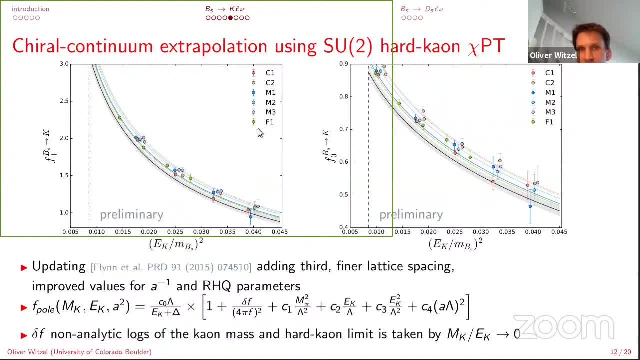 and the green one is our finest ensemble. So we have three lattice basings And then we have on the coarse and the fine different values of the light sea quark mass, which gives us a handle on how to estimate the effects due to having unphysical heavy pions in the sea at this point. 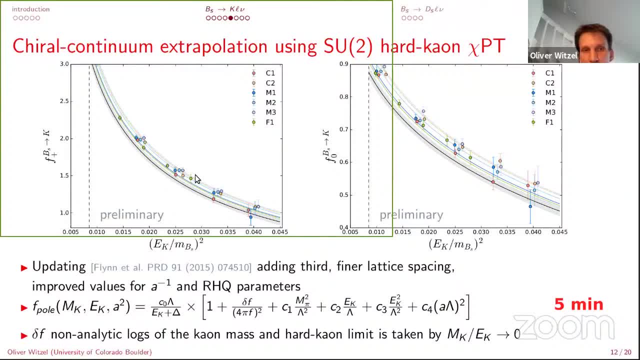 What you see is that we could determine the values for different momenta of the kaon, And these data points of the same color are now correlated. So what we do is to obtain a chiral continuum limit. we fit all of these data points together. 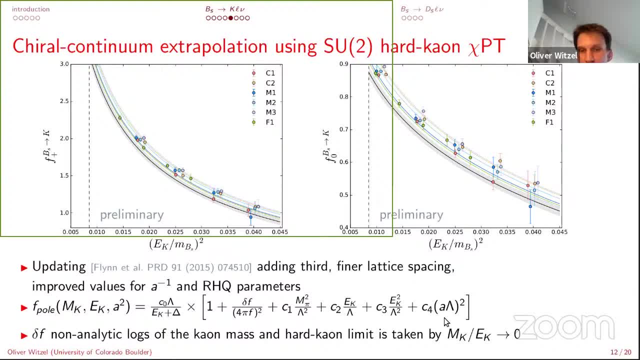 using an ansatz inspired by heavy meson, chiral perturbation theory, given on the bottom, And then we obtain the colored lines which are supposed to pass through the same colored data points And, in addition, the chiral continuum limit where we are extrapolating all quark masses. 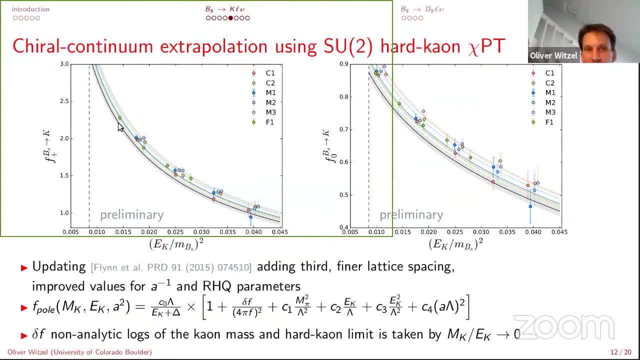 to their physical value and the lattice spacing is sent to zero. That is the black line with the gray arrow band, And this covers the range where we have data in our simulation directly, And on the left, this is the result for F plus. 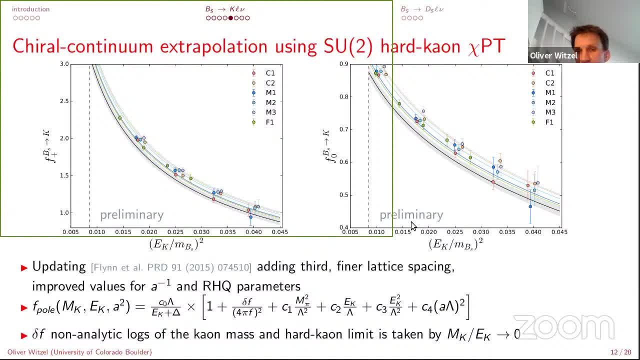 and on the right it is for F zero. Now, once you have done that, this result only shows the statistical uncertainty on the chiral continuum limit, But we now have to estimate all sorts of systematic errors, And I have a long list here. 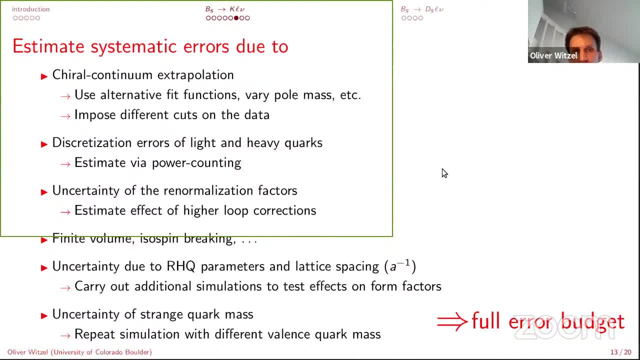 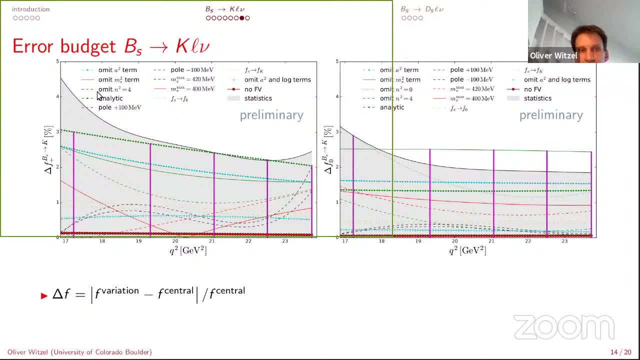 And instead of going through this list in detail, let me just show you a few plots. First of all, we need to Address the systematics due to our fit ansatz, And this is done by doing variations, And in these plots you see the gray background. 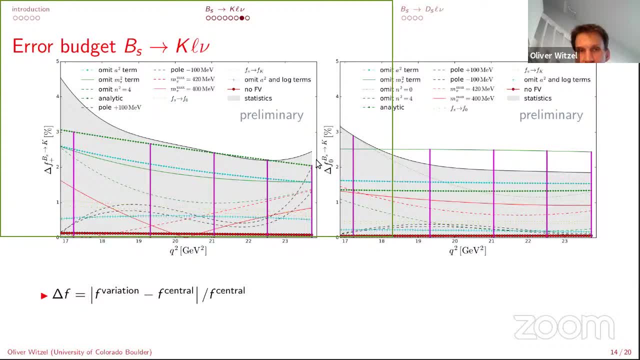 is our statistical, is our preferred result, with a statistical uncertainty. And then the colored lines give us different systematic effects, from varying the fit function by omitting terms or by changing the pole term and so on, And basically what we see is that everything. 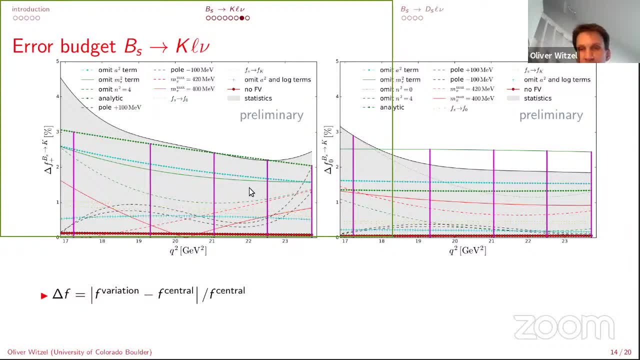 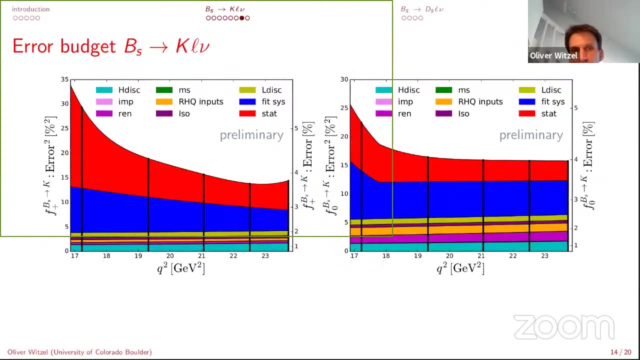 is on the same order as our statistical precision for F plus, whereas there is one uncertainty which is relatively independent of Q square, which is a little bit larger for the higher Q squares in the case of F zero. Now, in addition, we have to estimate the uncertainties. 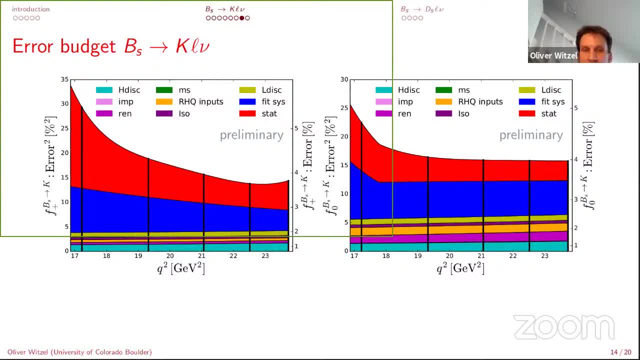 which we cannot get from just varying the fit function. We need to look at discretization effects and uncertainties of the input parameters, et cetera. And this gives you then the layout plot where the statistical error is on top. The systematic due to the fit is given in blue. 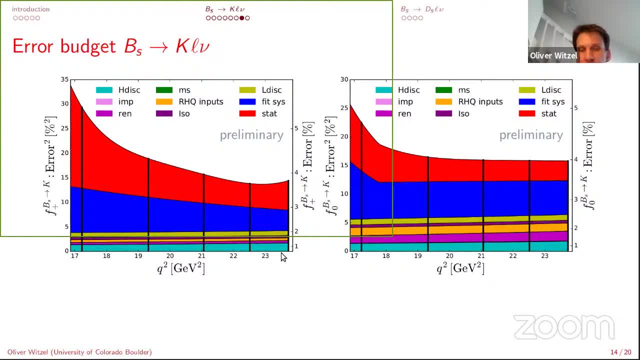 And the other uncertainties are then color coded on the bottom. All in all, we get a result of around 4% for both form factors in the range where we have Q square. Now, as Christoph was asking in the last question, this is a restricted range in Q square which we are studying. 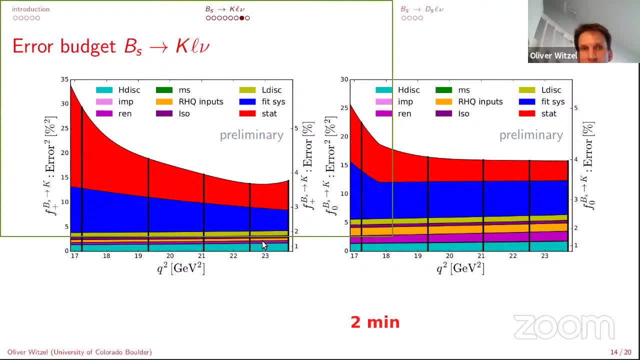 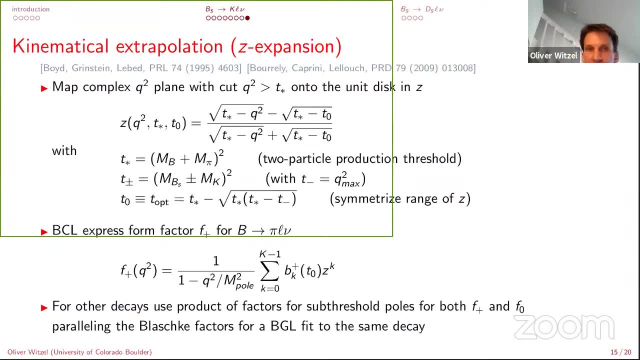 And we want to extrapolate that over the full range, And for that we need to refer to the kinematical extrapolation or that expansion, going back to Boyd Brinstein and Leavitt, And later we find from Borelli, Caprini, Lelouch, 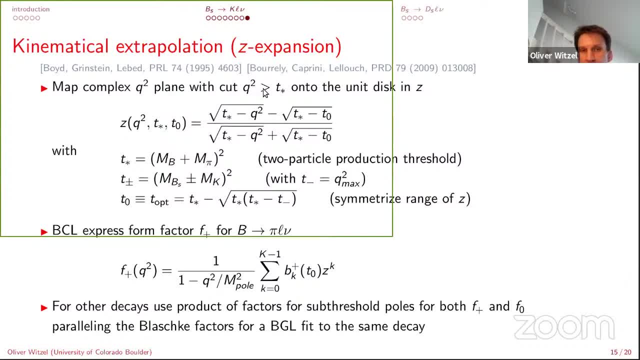 And it is basically mapping the Q square plane with a cut onto the unit disk in Z space. And this is the equation you do. The basic philosophy is that you are converting the parameter range from Q square to a well-defined range on the unit disk. 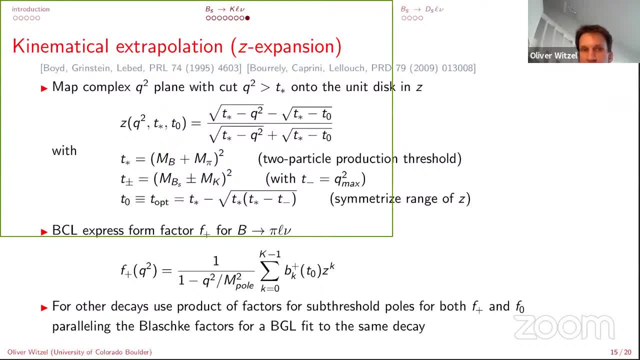 And you symmetrize the fit range to improve the kinematic extrapolation, And so you can just go forth and back between Q square and Z. It's just easier to perform the expansion in the Z parametrization space. Specifically, we are using BCL right now. 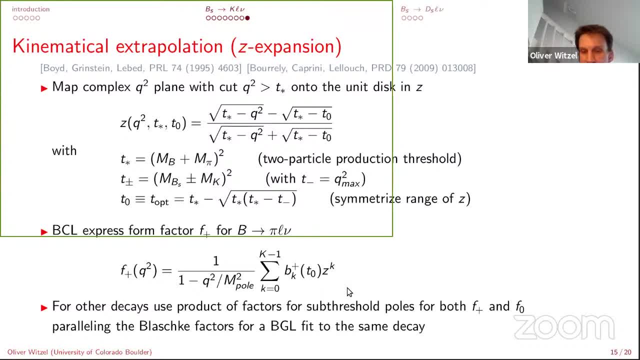 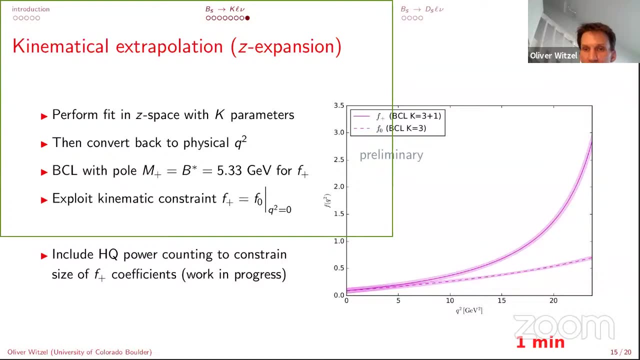 for testing out our fits. So the equation is given up here, And then we need to account for the product of factors for subtraschle poles in the case of BS2K. This is now a first look at our BS2K expansion over the full range. ,, ,, ,, ,, ,, ,, ,, ,, ,, ,, ,, ,, ,, ,, ,, ,, ,, ,, ,, ,, ,, ,, ,, ,, ,, ,, ., ,, ,, ,, ,, ., ., ., ,, ., ., ., ., ., ., ., ., ., ., ., ., ., ., ., .. 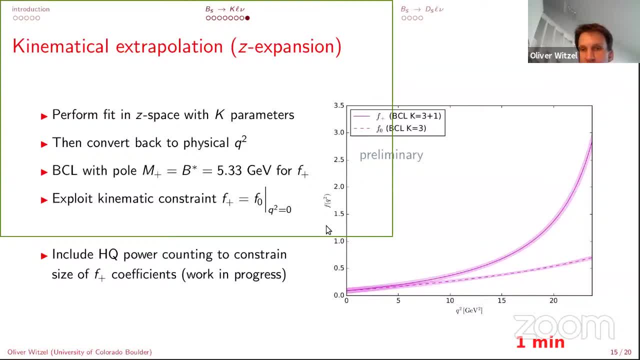 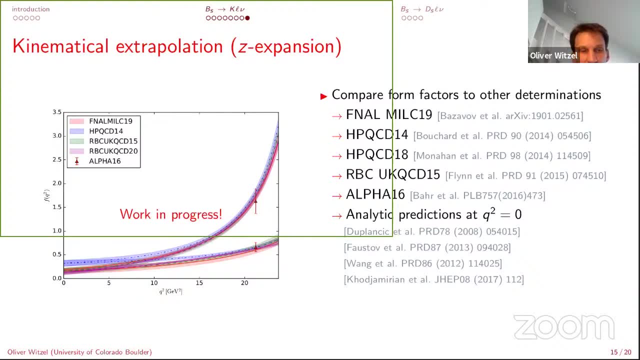 expansion over the full Q-square range. And since I'm running out of time, I can just show you a quick comparison to other lattice results. And all in all, there is good agreement with this still persisting discrepancy at 0 Q-square to the HBQCD14 result, But we are still. 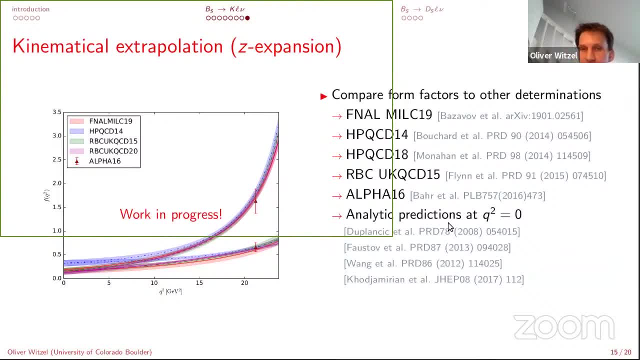 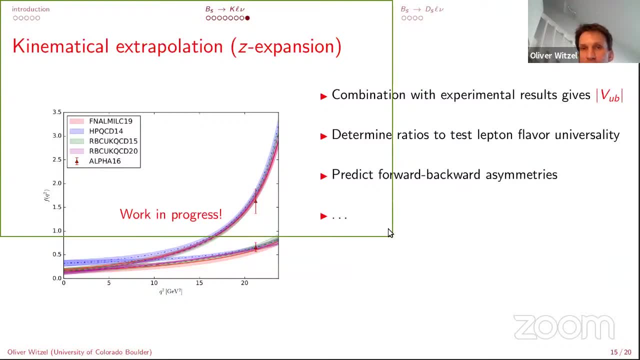 working on making the comparison here, We are also working on including analytic predictions. So in the last minute let me quickly jump to BS, to DS, which basically has the same equation, except that we have to deal with the charm quarks here. 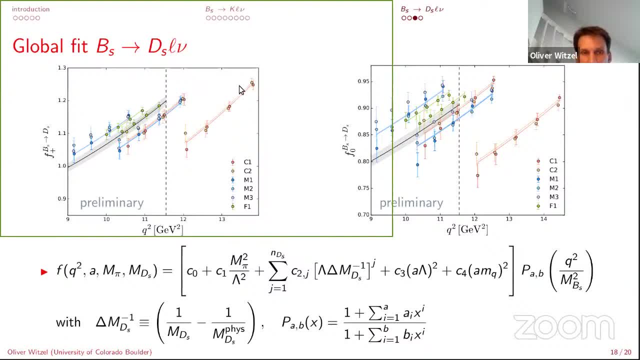 And this is the status of our result. We have the chiral continuum limit implemented and we have a good result here And there. you can see that the range in Q-square is significantly smaller because the DS is eating up much more of the energy. 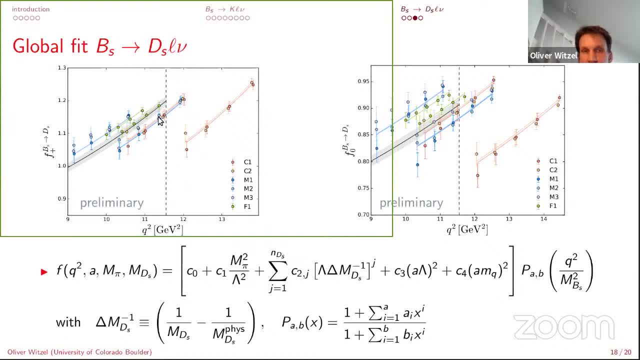 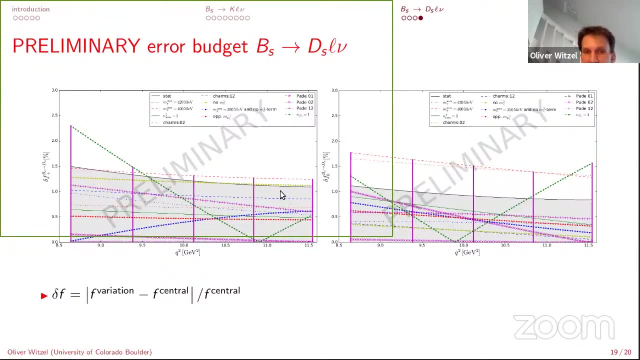 And what we are doing here is either an extrapolation or a small interpolation to the physical DS meson mass. Now we are still working on estimating the full error budget And what we already see. it is a harder task because the statistical errors are significantly lower. 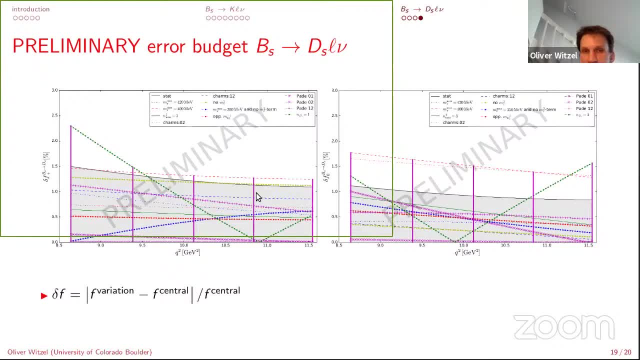 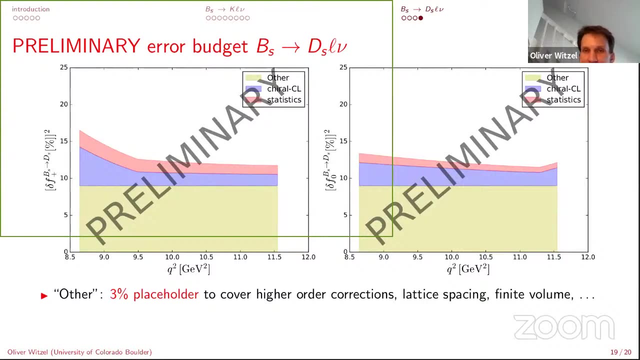 They are off the order of 1%. So you have to be more careful in considering all the systematics because they can be more easily be significant And at this point we hope to have a final result of a few percent, but that is still under heavy discussion. 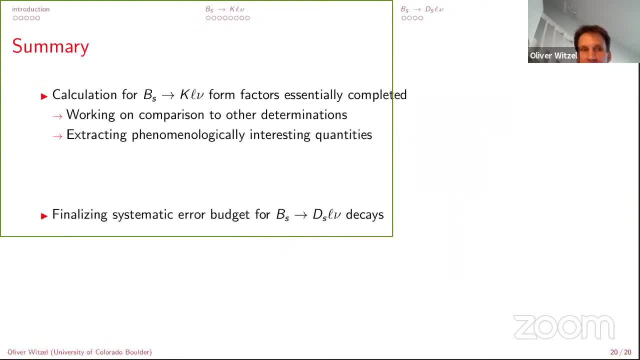 within the collaboration. So let me briefly summarize: The calculation for BS to KL mu is essentially complete and we are working on the comparisons and extracting phenomenologically interesting quantities, Whereas for BS to DS L mu decays, we are still finalizing the systematics. 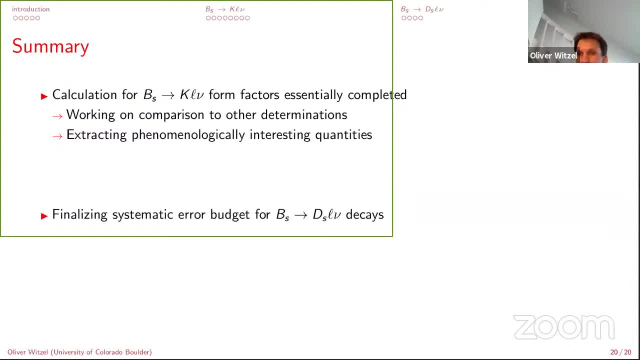 but we are hopeful to finish the result very soon now, Thank you. Thank you, Oliver. We have time for one question, maybe, And we encourage people to make questions of the Two, So any question OK, so I see no raising hands. 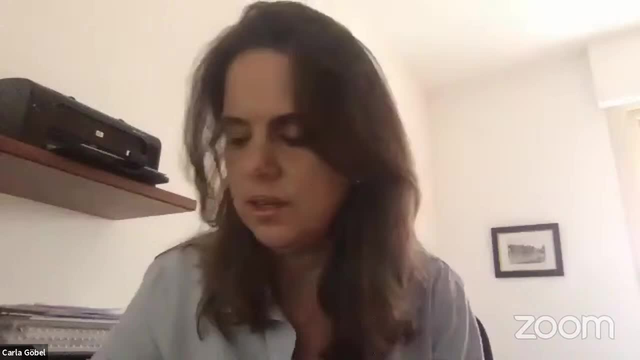 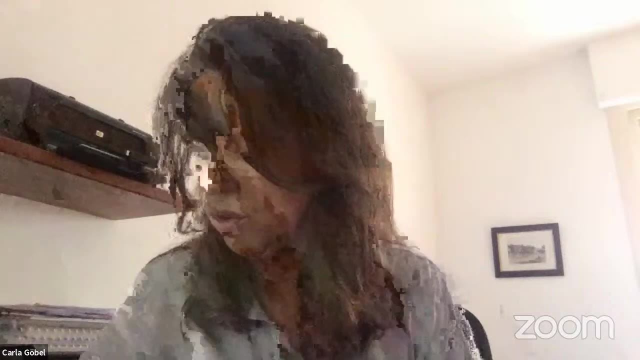 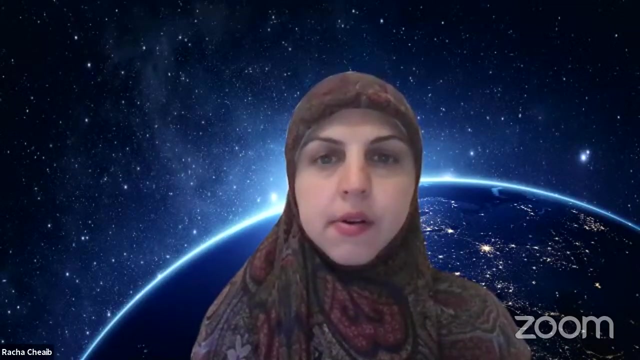 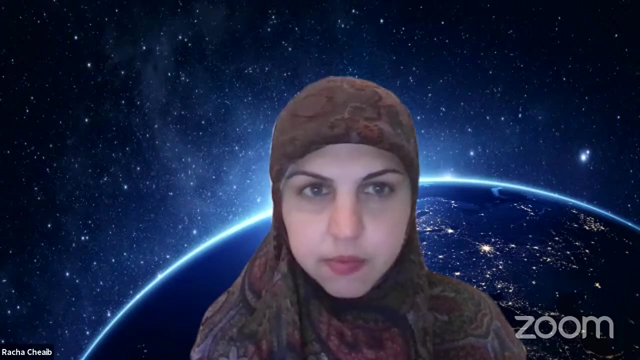 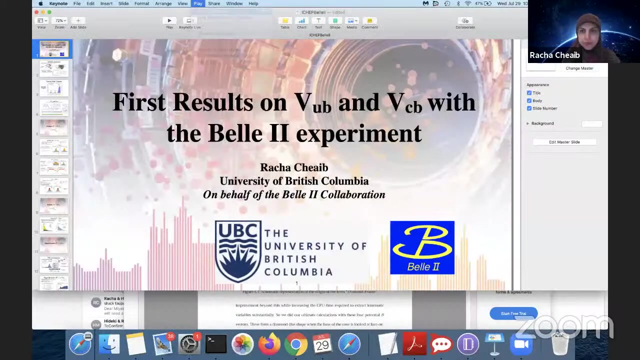 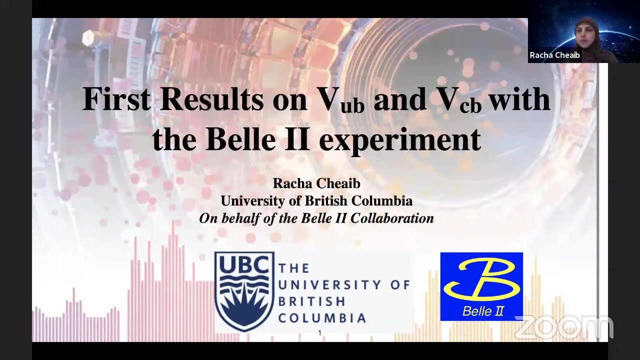 So thank you, Oliver. again. We can move on to Russia. First results on EUB and VCB with the BEL, BEL2.. OK, should I share my screen? Sure, All right, OK. OK, so I'm going to share my screen. 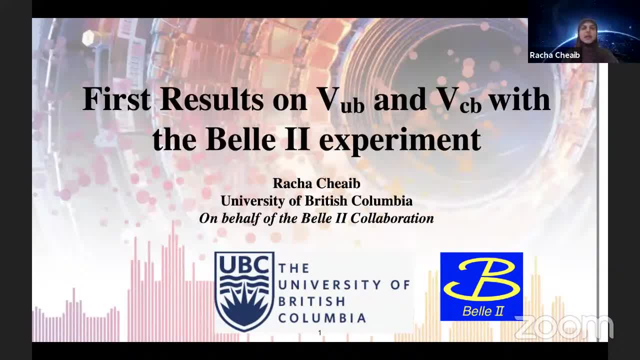 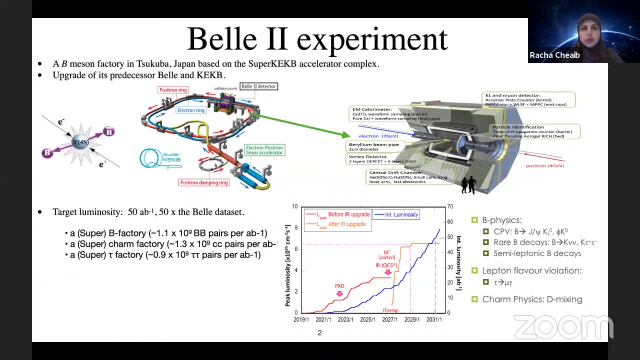 All right. So I don't know how to get rid of this Zoom, but anyways. So this is a talk on the first results on VUB and VCB with the BEL2 experiment. So the BEL2 experiment- brief intro: it's a B-Mas on factory in Tsukuba, Japan. 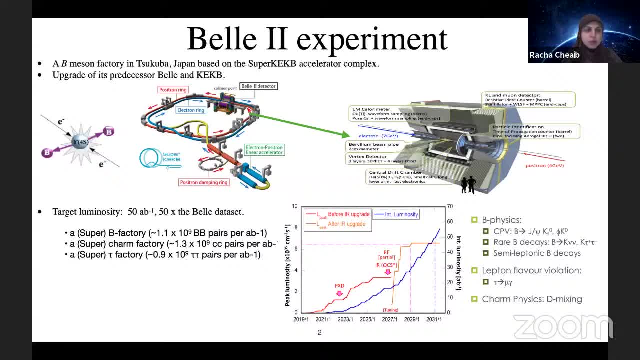 We collide electrons and positrons at an asymmetric energy And we produce B-Mas on pairs, And the 1800s are a few years old, And so what we do is we use a B-Mas and the BEL2 to call in B-Mas. 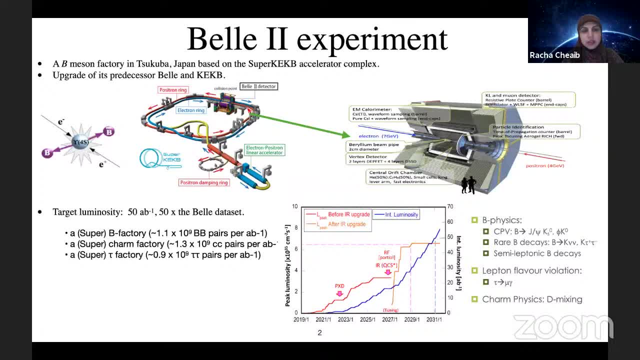 And we use this B-Mas to put the B-Mas together And we use it in the B-Mas And we're doing a MenS test with some of these two of these B-Mas. So this is a test that we do. 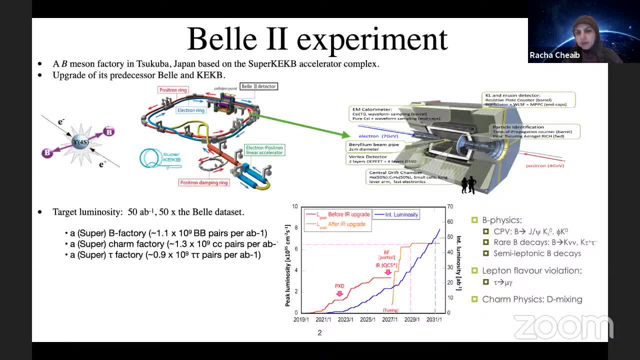 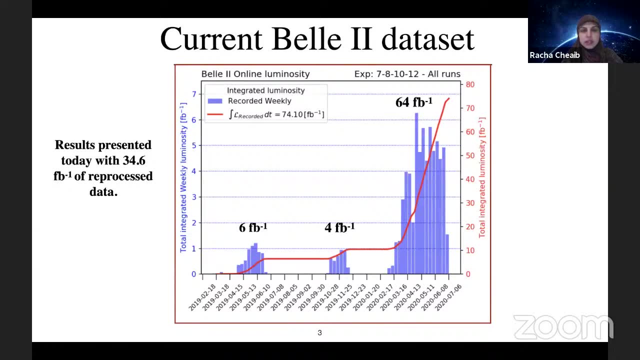 And it's fundamentally we're doing this to have these two B-Mas in the same atom. OK, So if you don't want the B-Mas to collide with one another, then you don't want to do that. So our current BEL2 dataset- we recently started data taking. Our current dataset is around 74 inverse femtobarons. For today, our results are presented with 34.6 inverse femtobarons of reprocessed data. 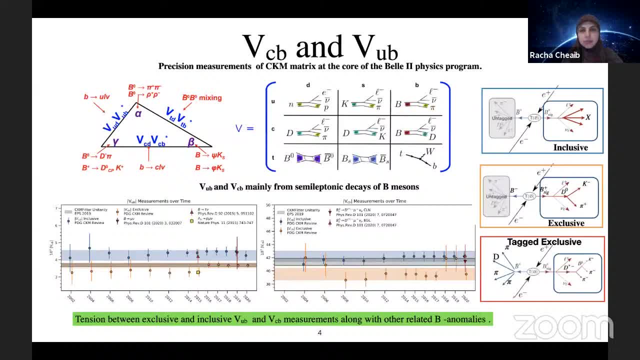 So VCB and VUB, as presented by Fabio. you know, precision measurements of the CKM matrix elements are at the core of the BEL2 physics program. We're a flavor factory, and so we will be planning to determine these elements precisely. 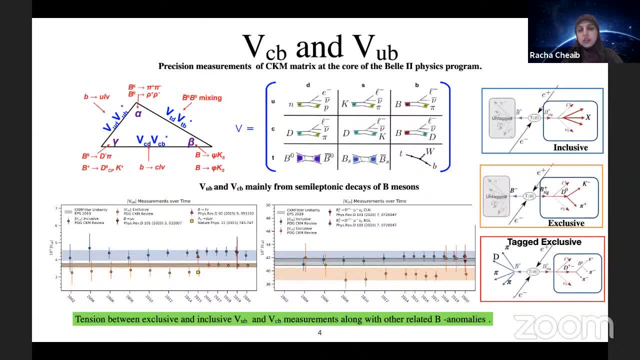 And for VUB and VCB, these are determined primarily from semileptonic decays of the mesons And you can see here there's this tension between X-cludes. So we have inclusive and inclusive VUB and VCB measurements which we want to, I guess, investigate and measure, along with other related B anomalies. 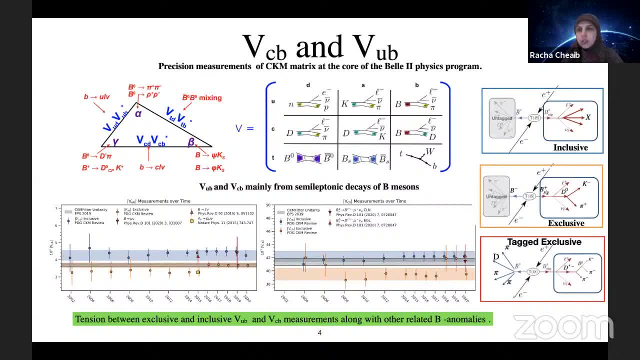 And so for inclusive decays, you know there are a couple of ways to target these. So inclusively is where we don't fully reconstruct the X system which is seen, And then exclusively is where we fully reconstruct the X system which is seen. 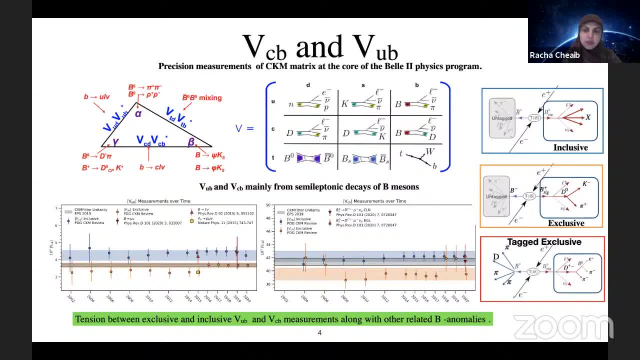 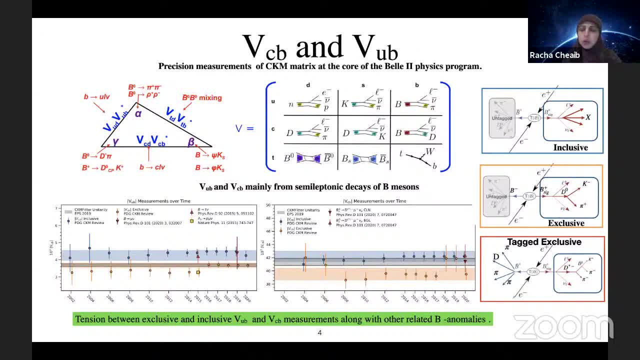 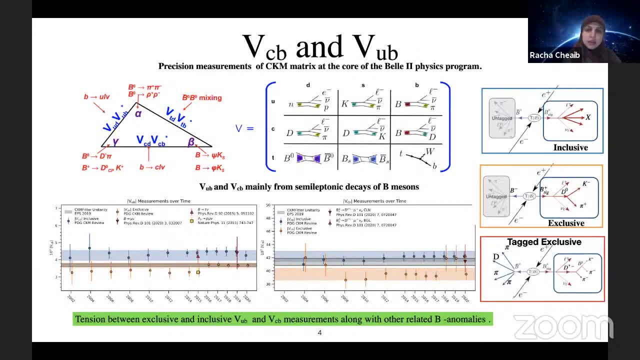 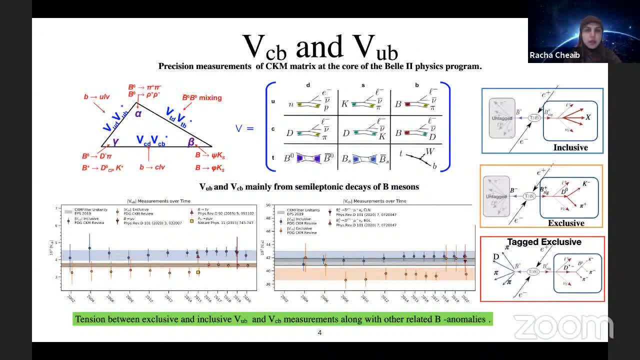 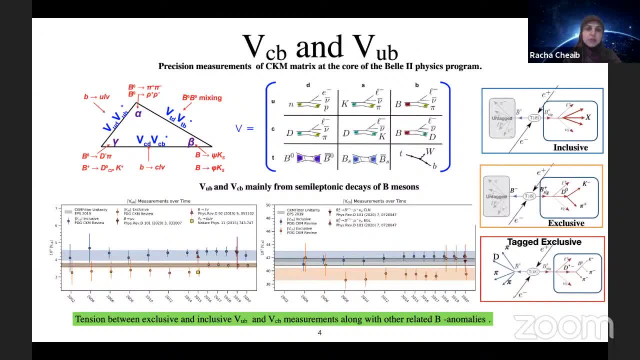 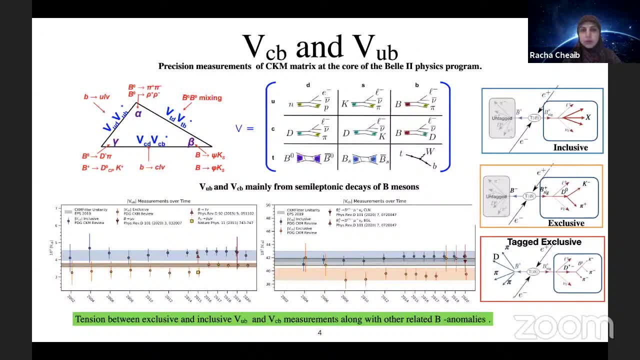 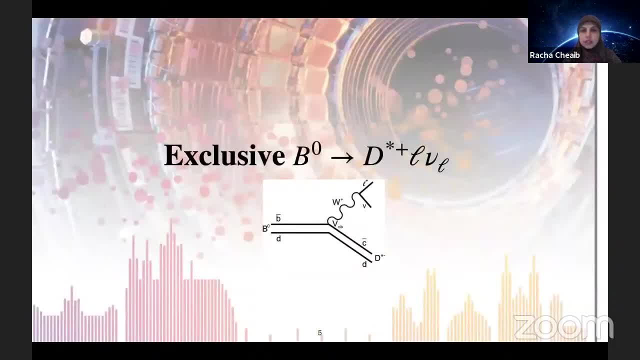 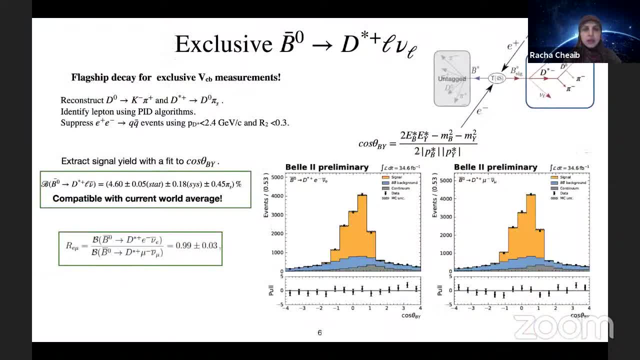 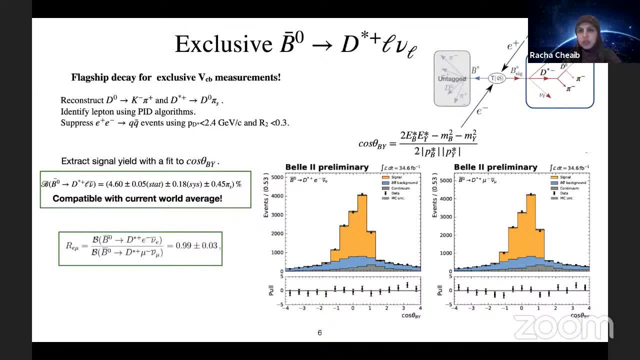 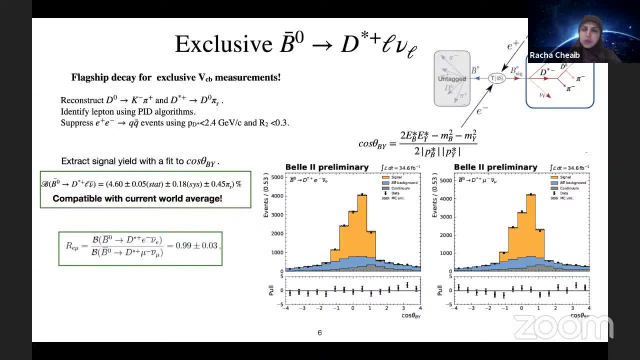 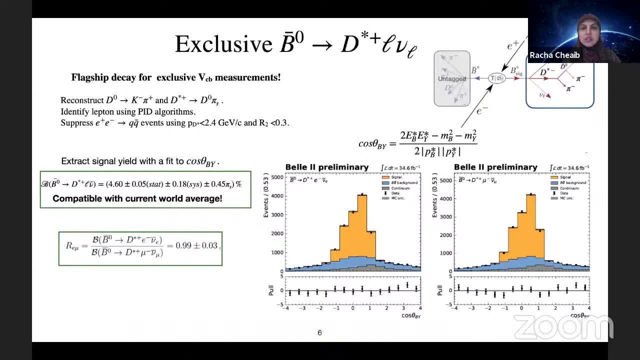 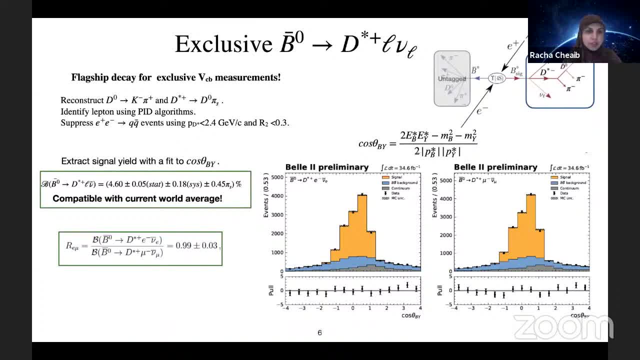 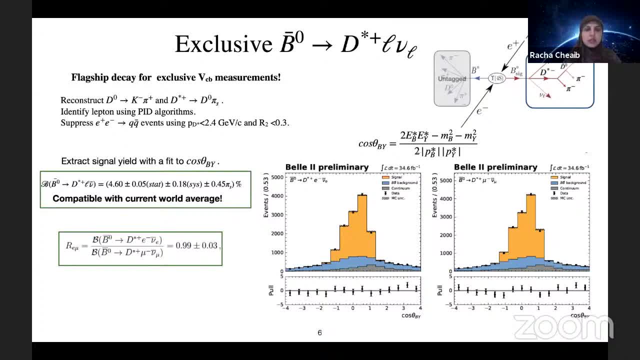 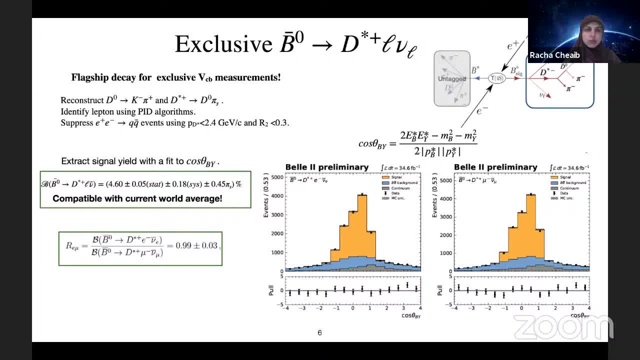 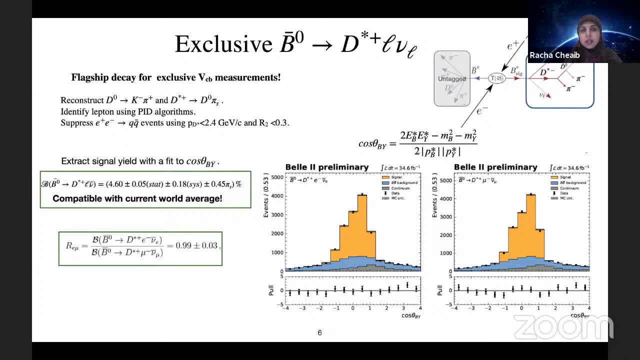 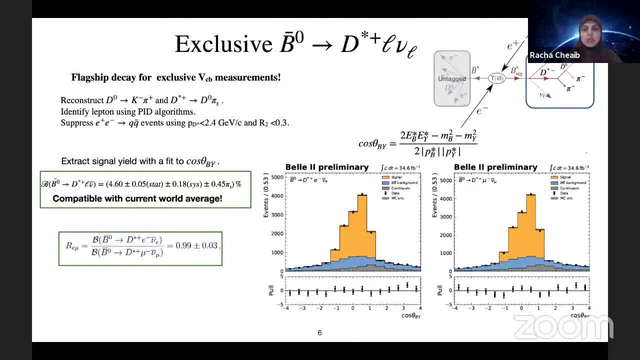 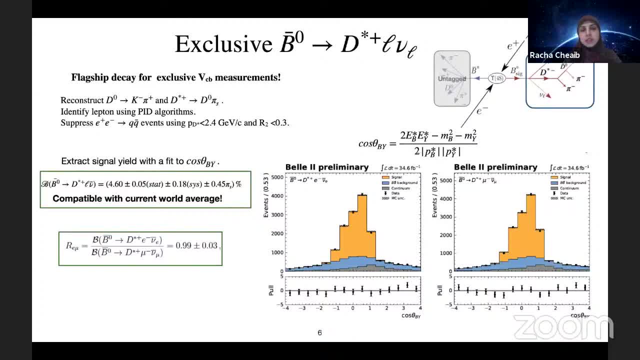 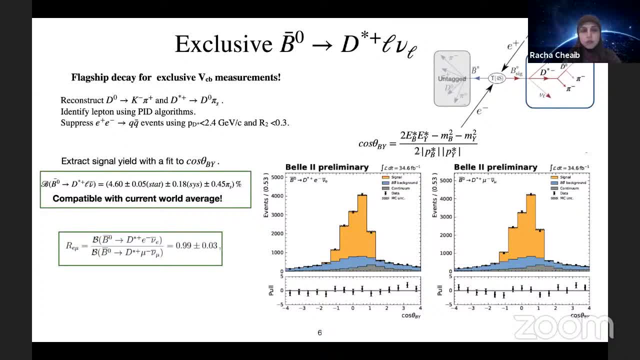 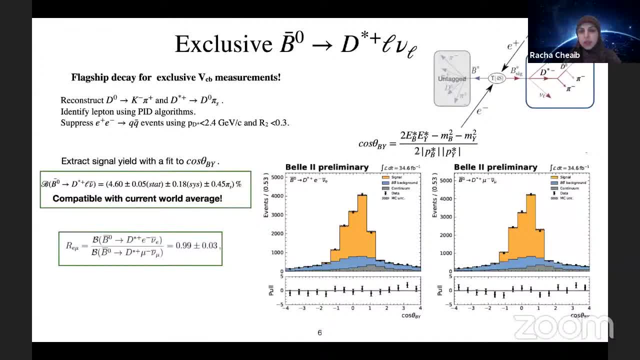 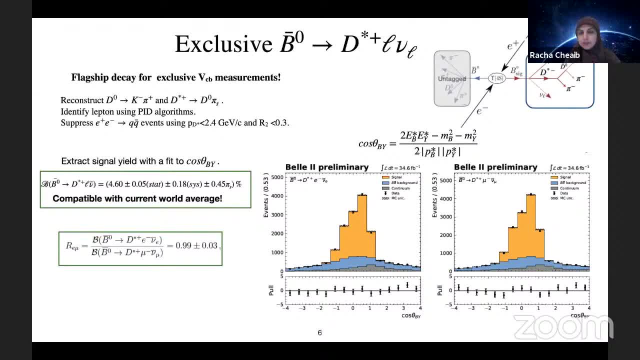 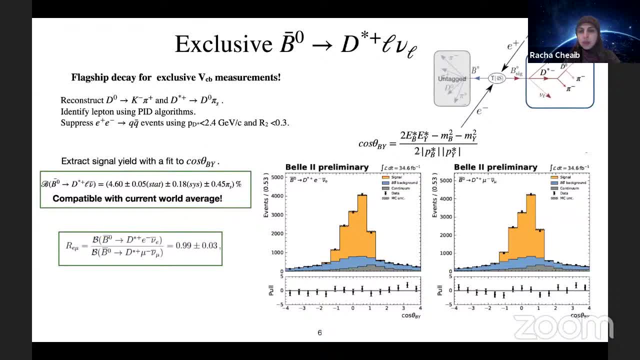 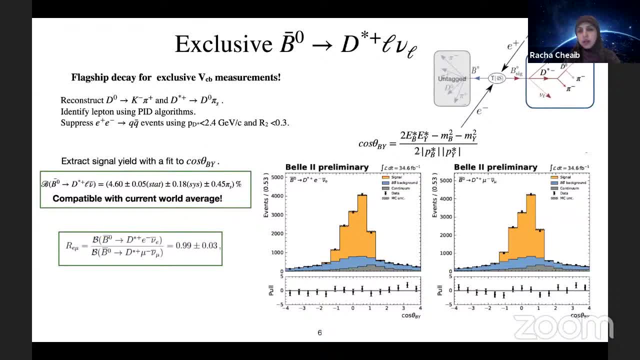 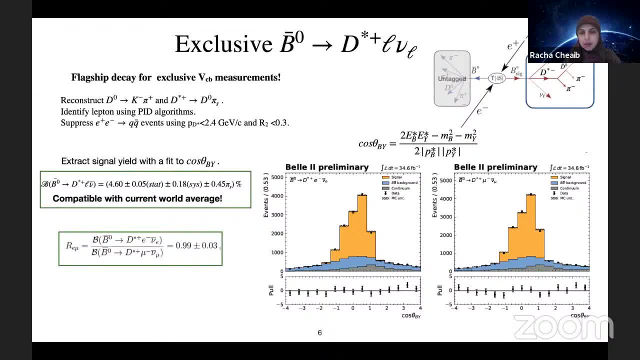 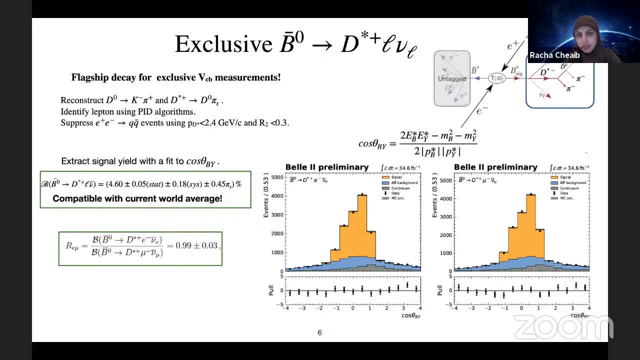 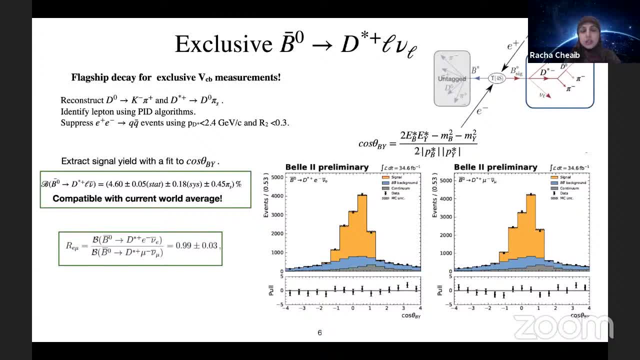 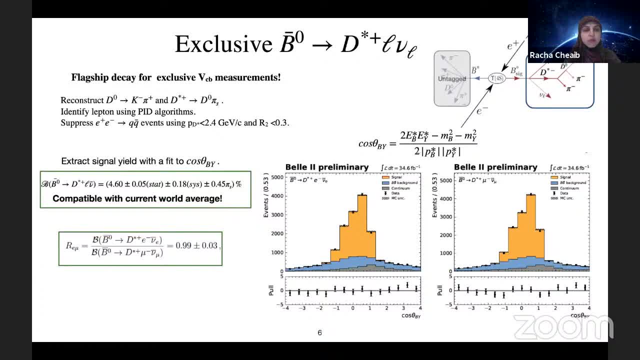 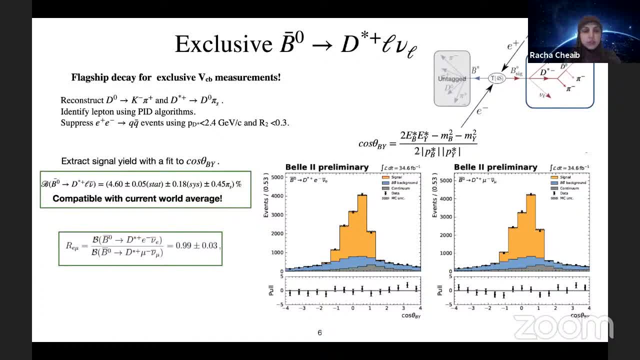 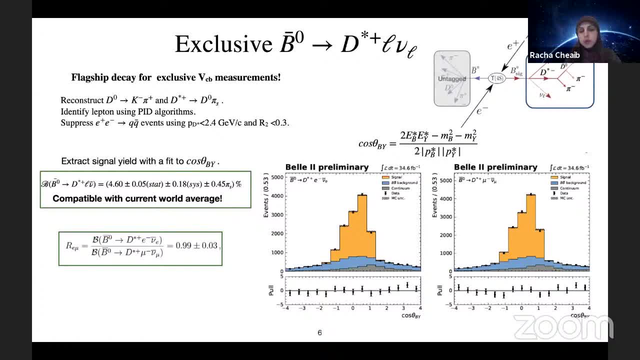 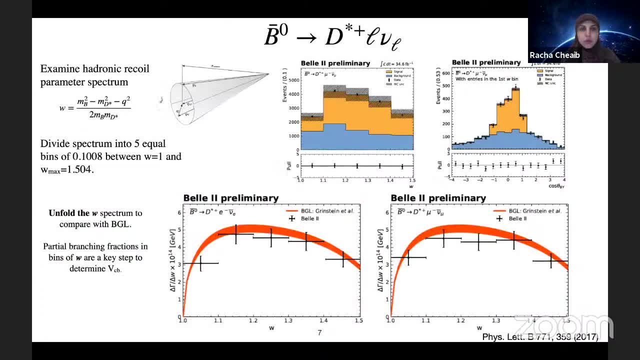 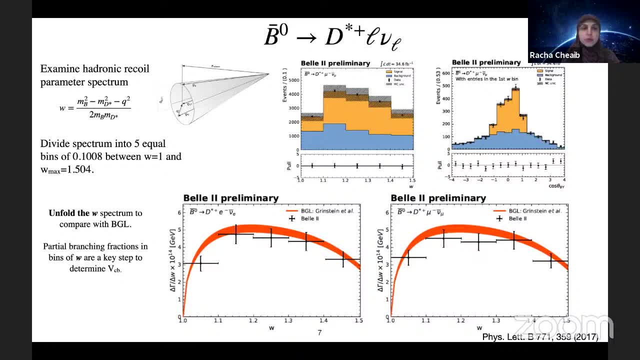 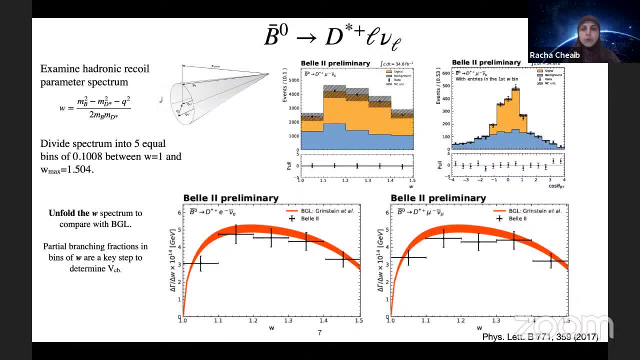 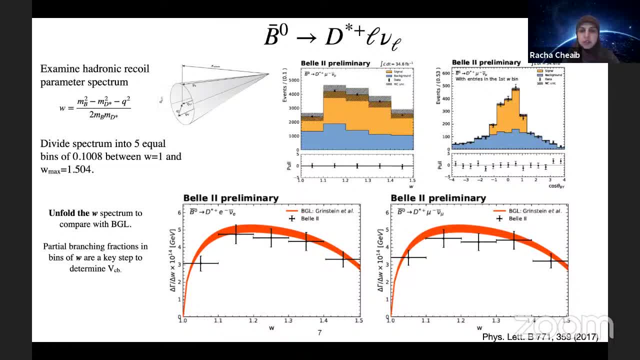 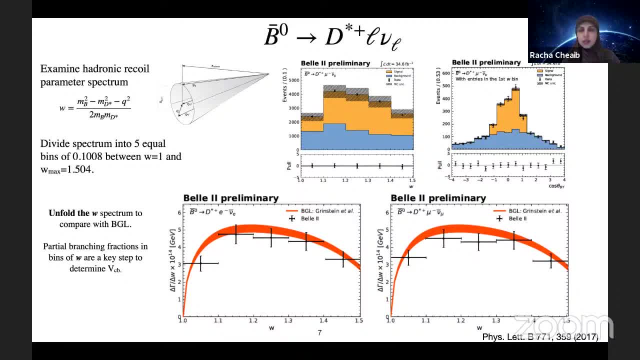 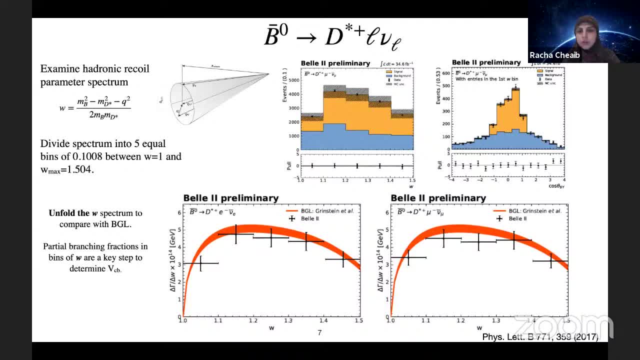 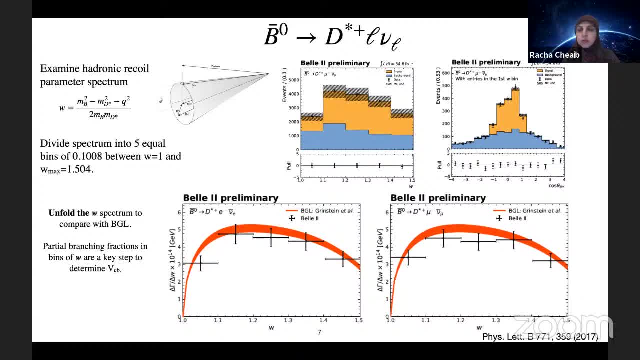 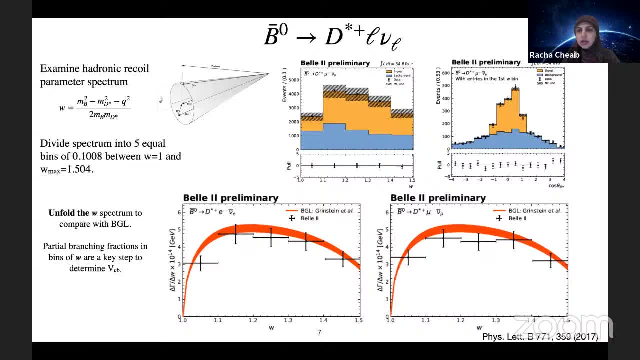 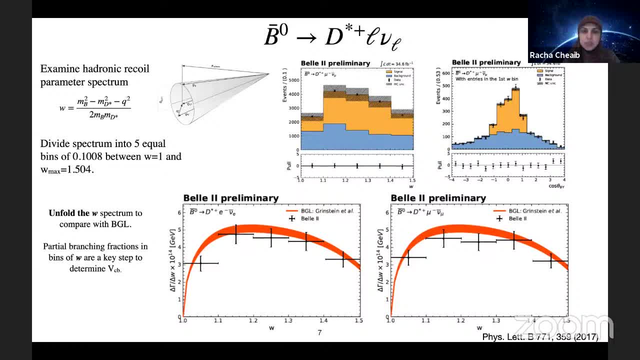 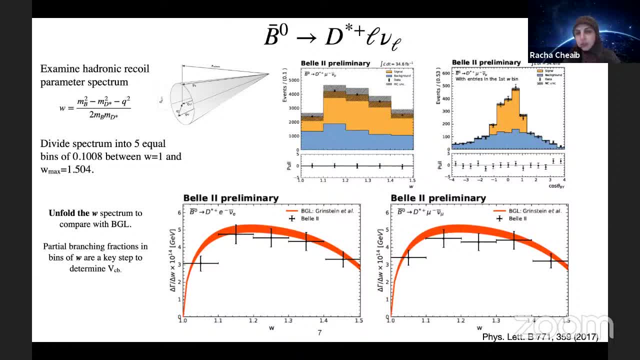 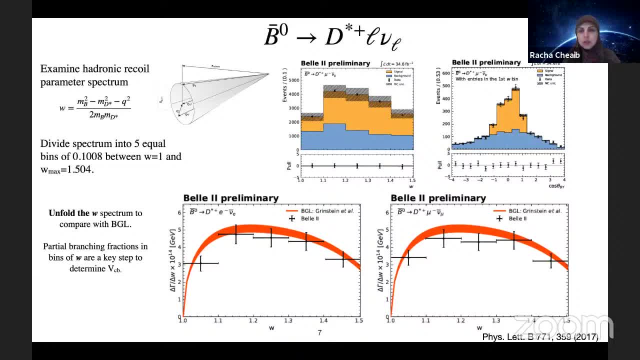 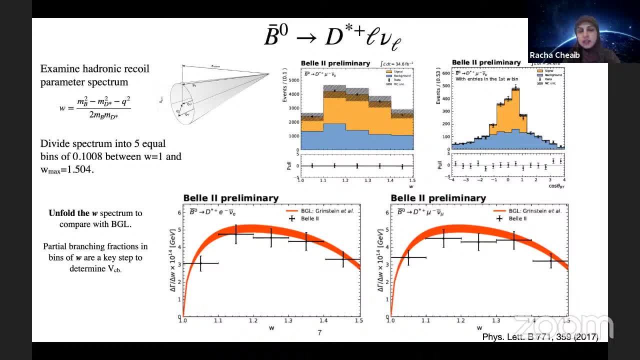 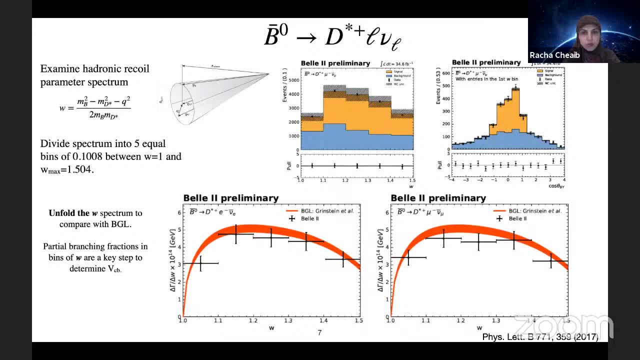 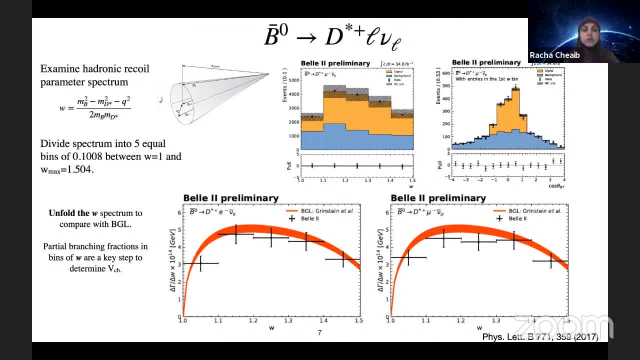 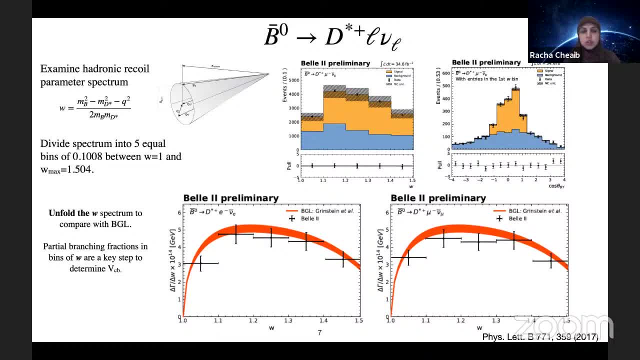 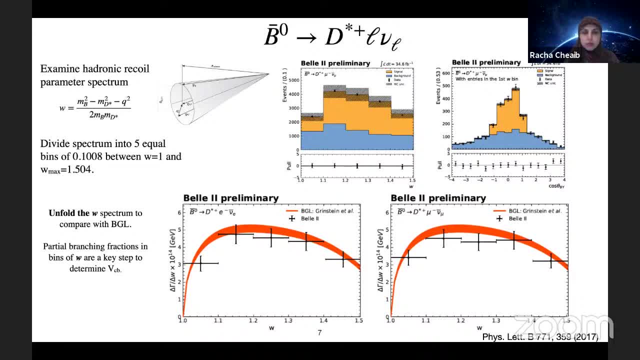 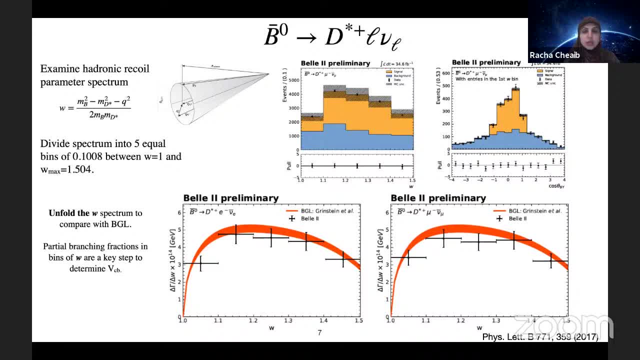 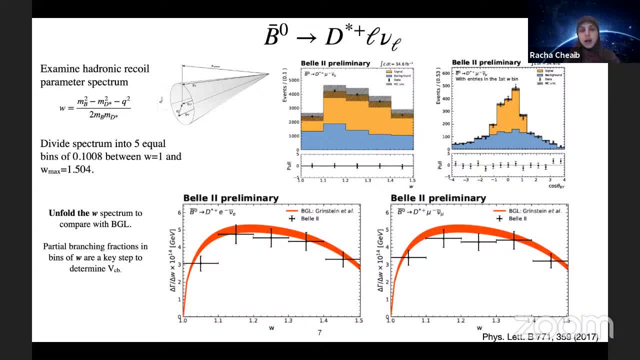 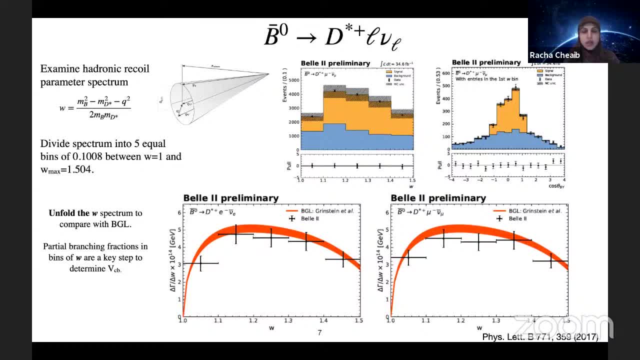 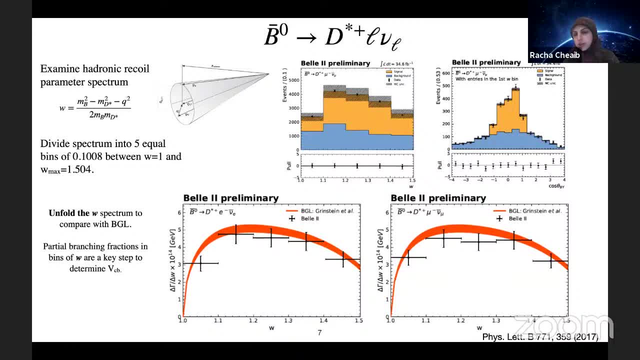 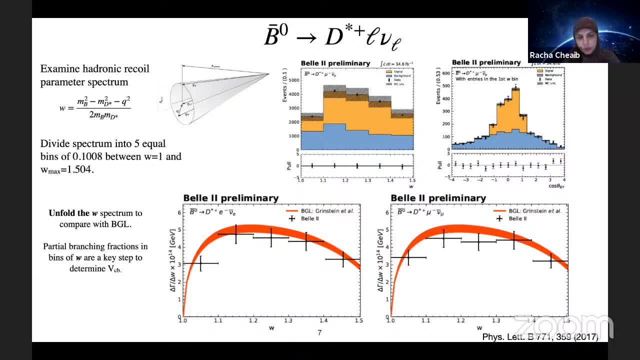 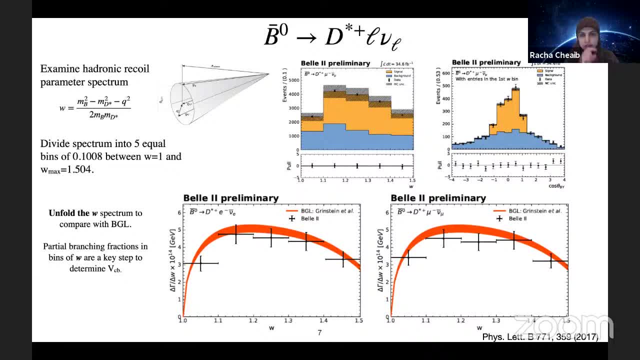 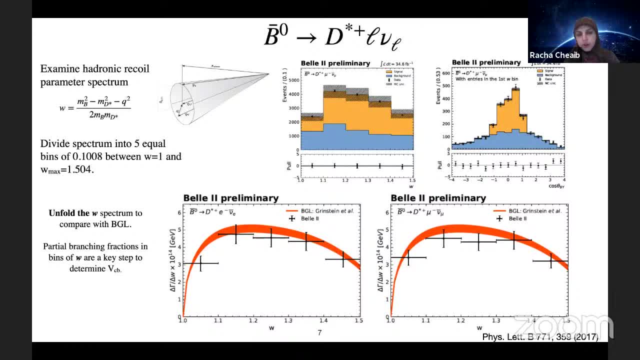 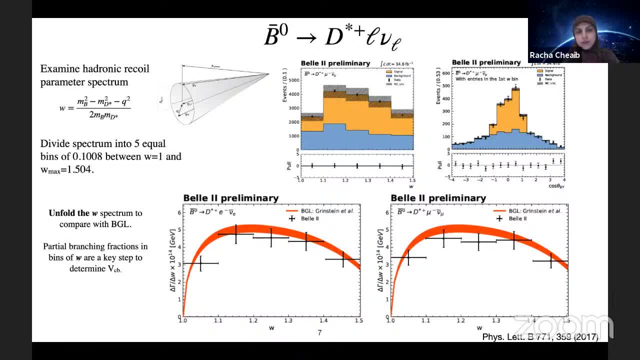 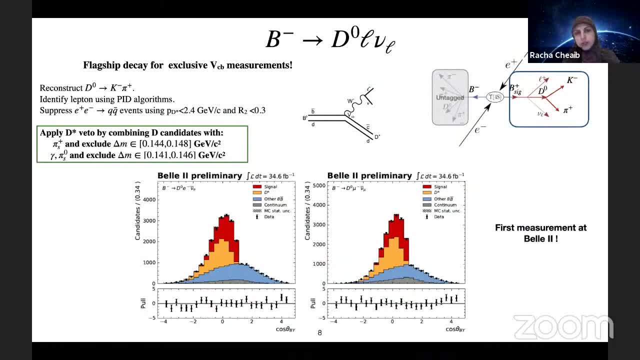 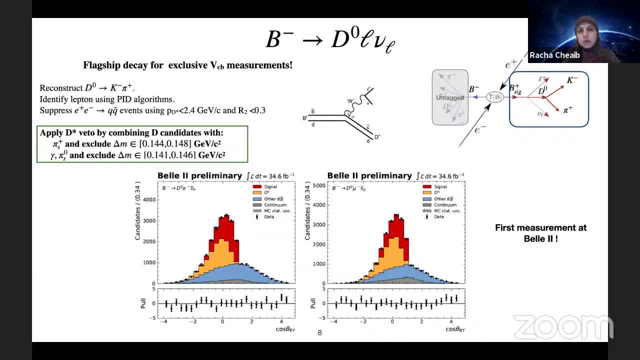 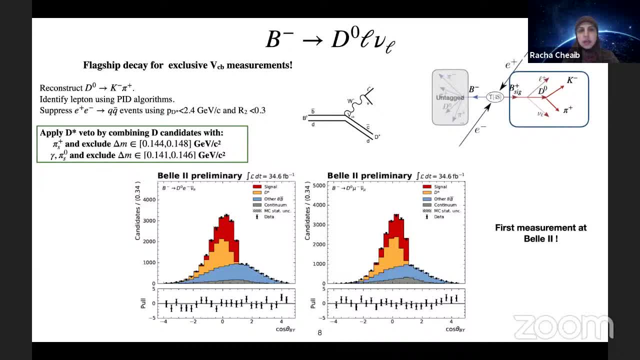 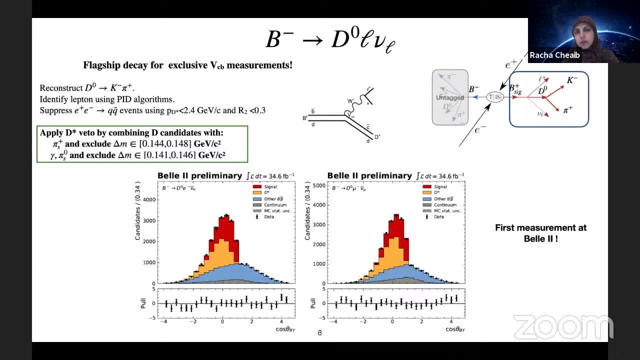 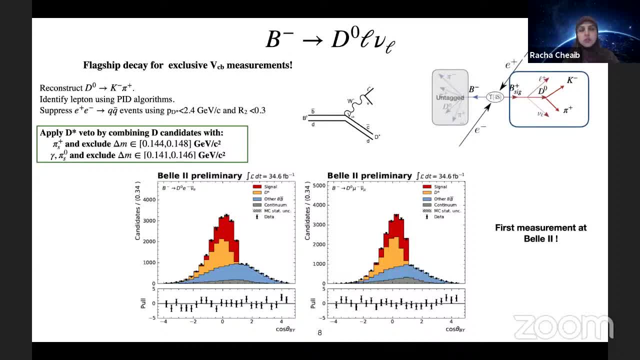 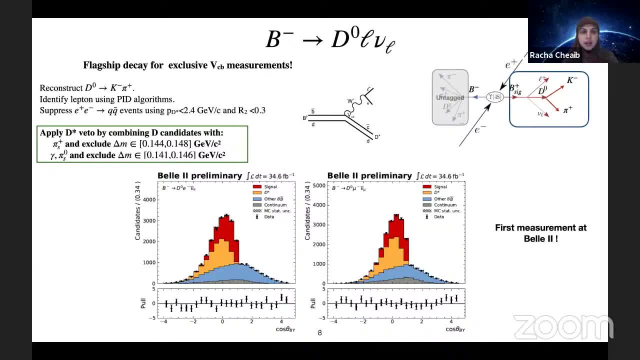 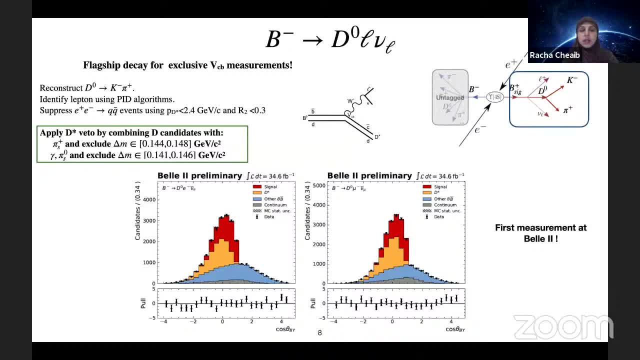 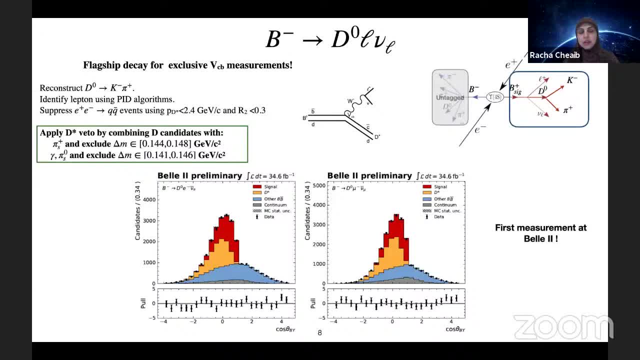 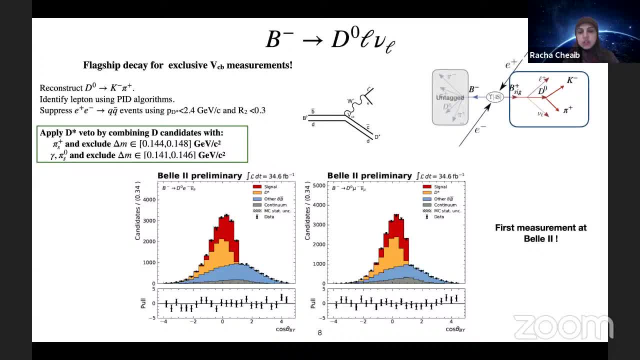 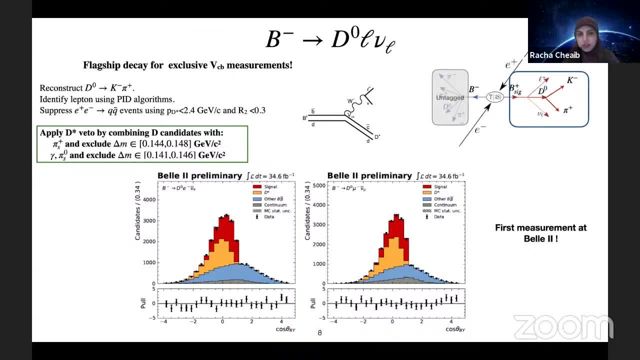 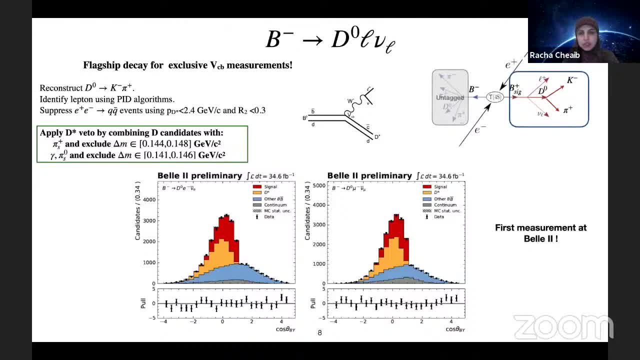 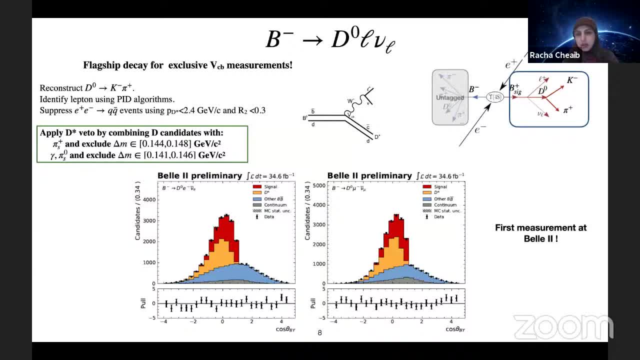 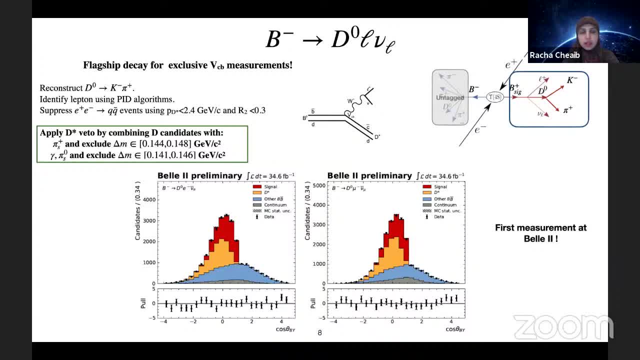 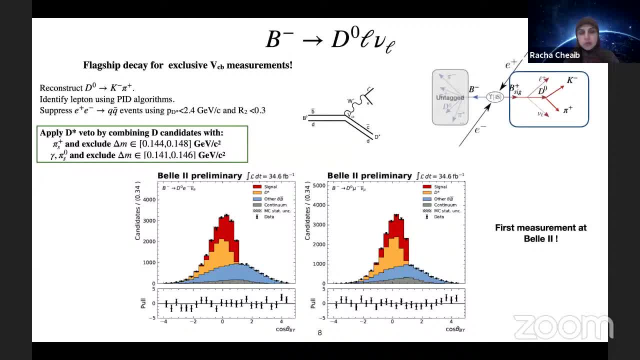 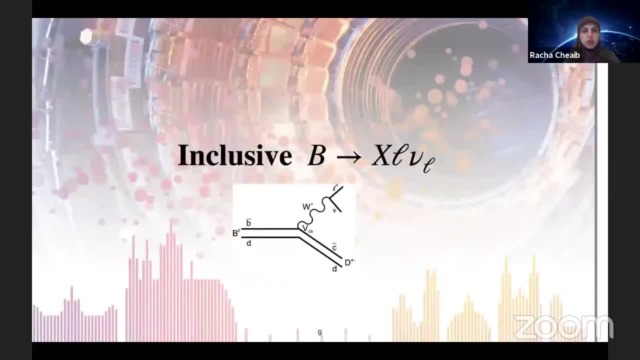 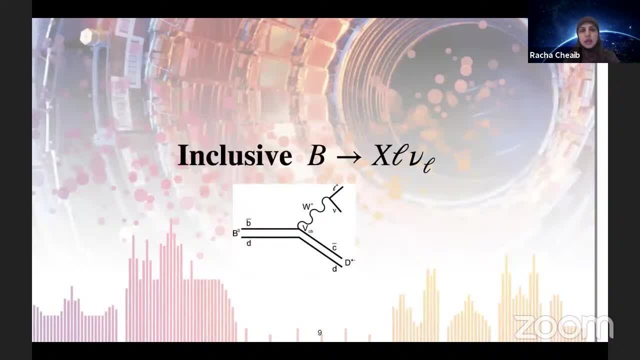 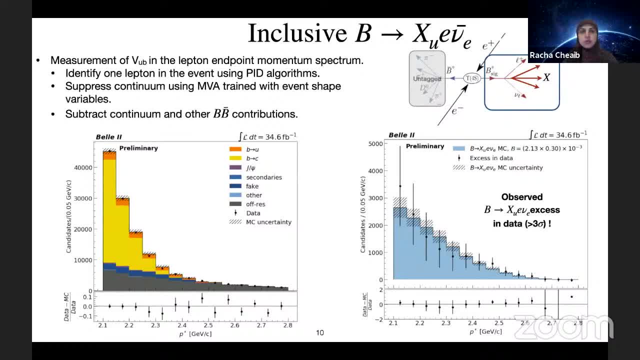 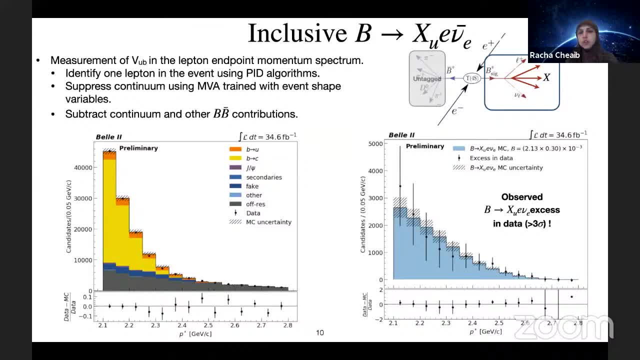 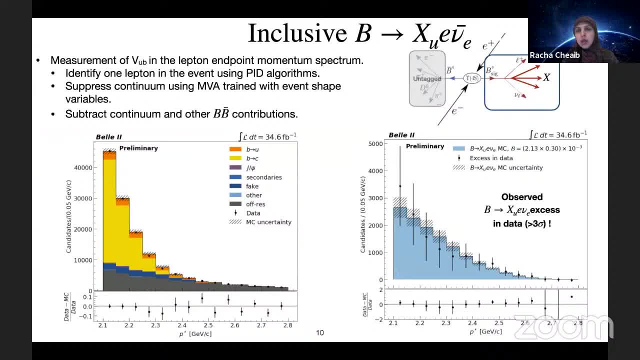 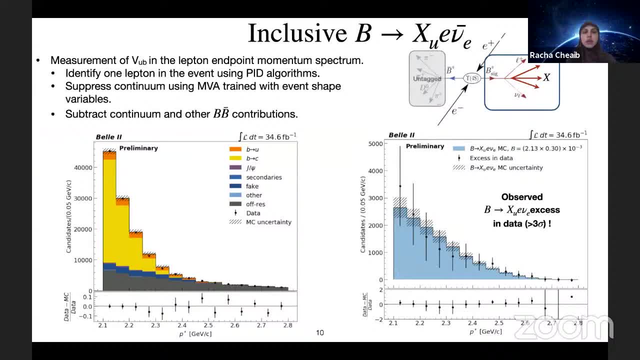 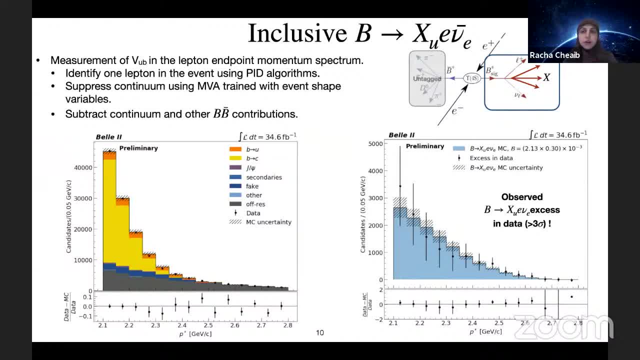 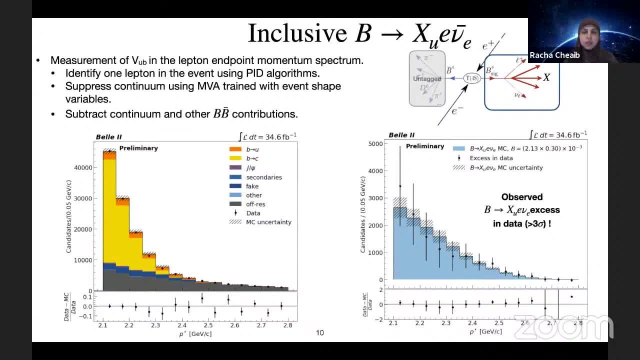 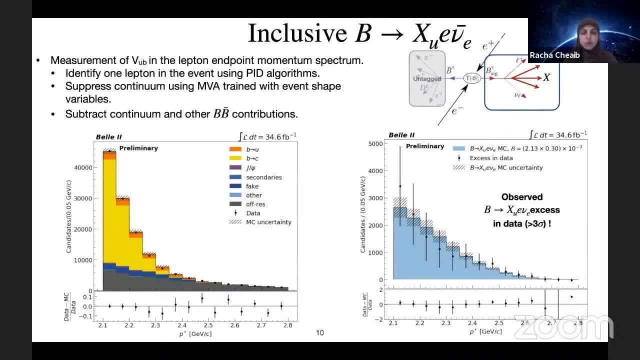 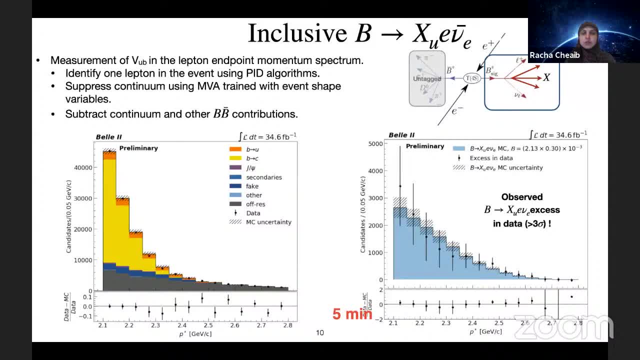 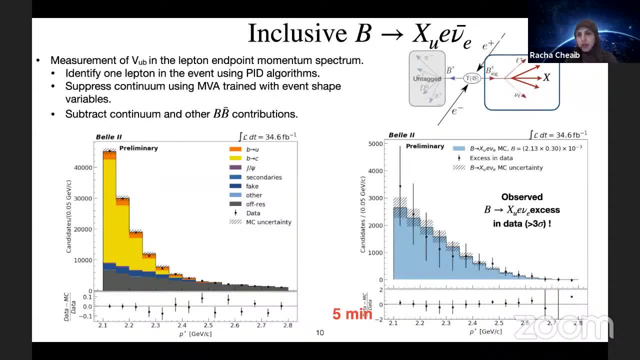 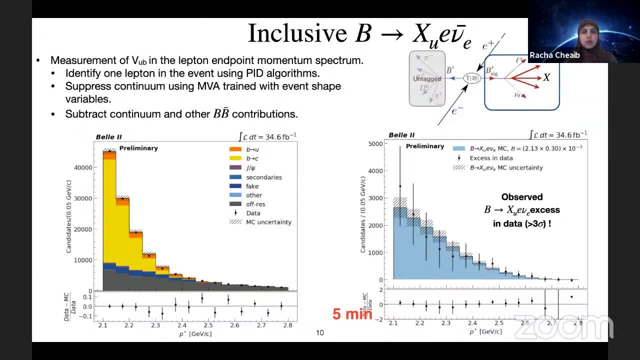 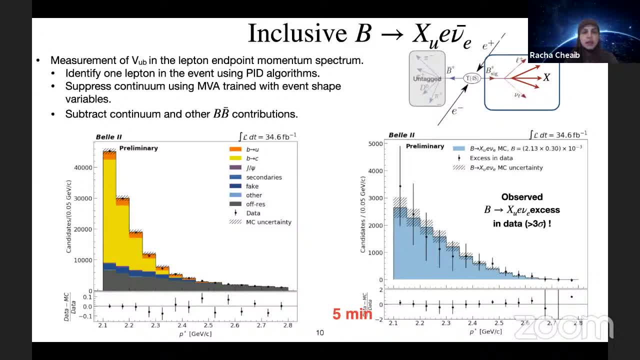 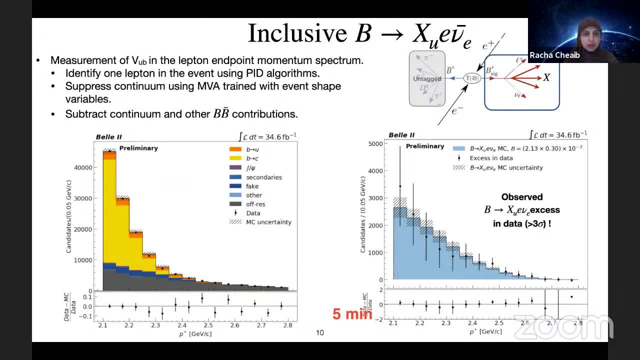 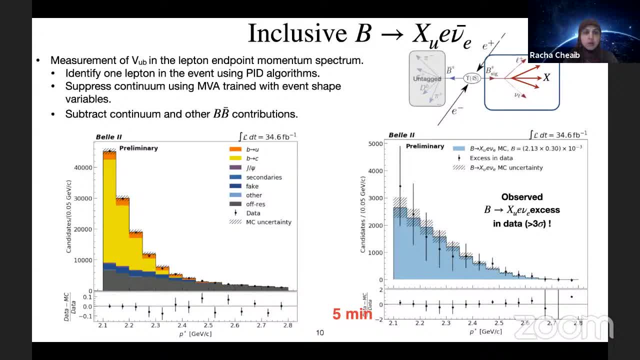 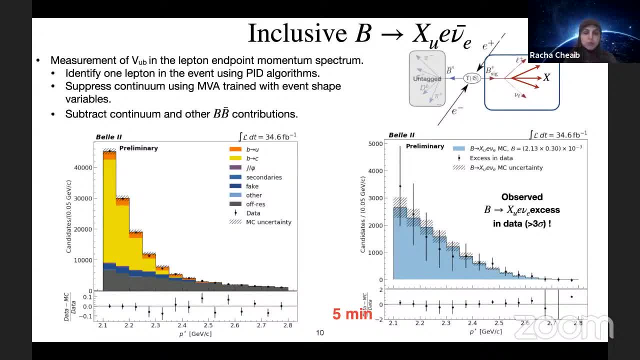 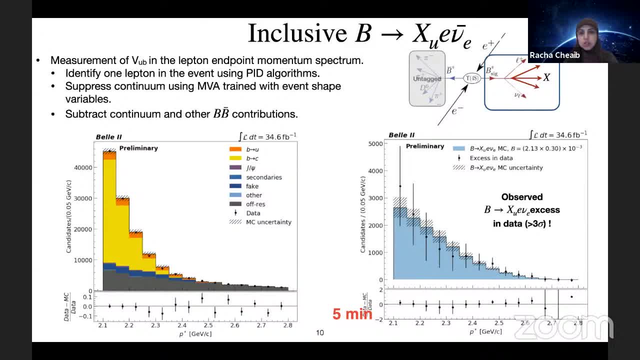 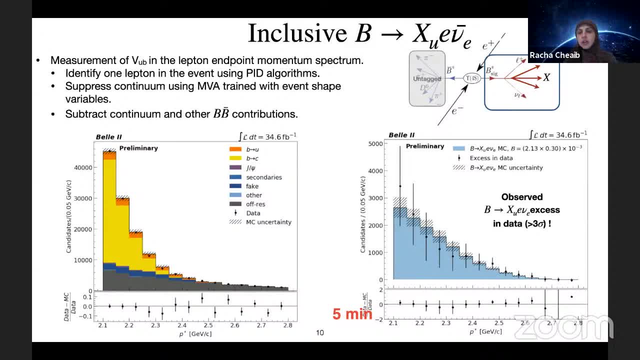 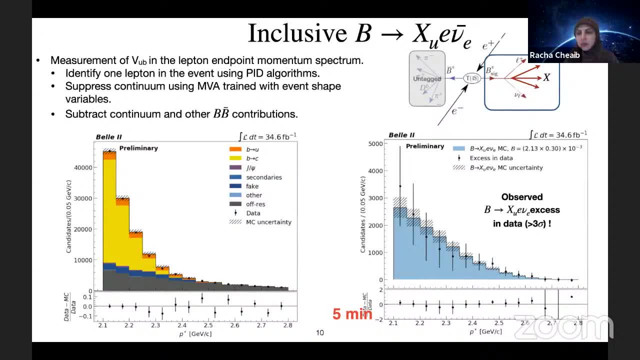 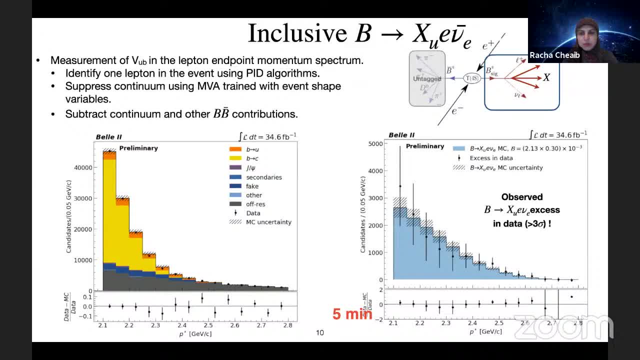 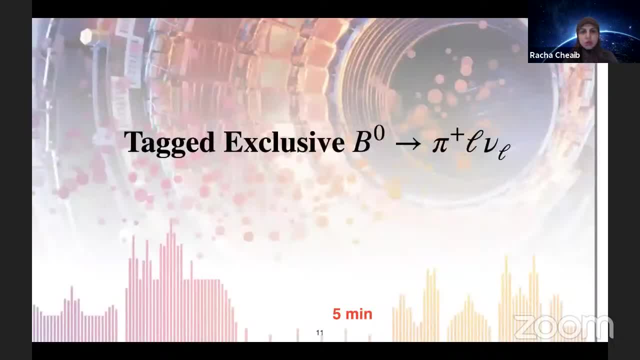 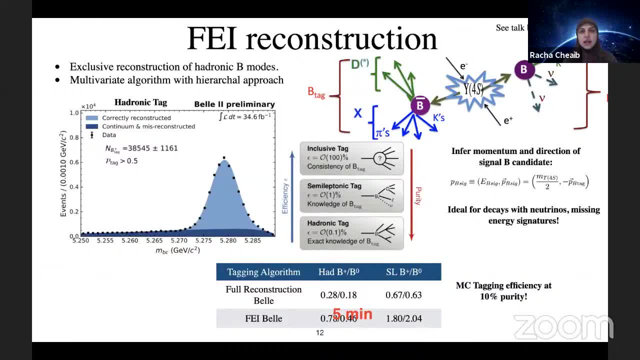 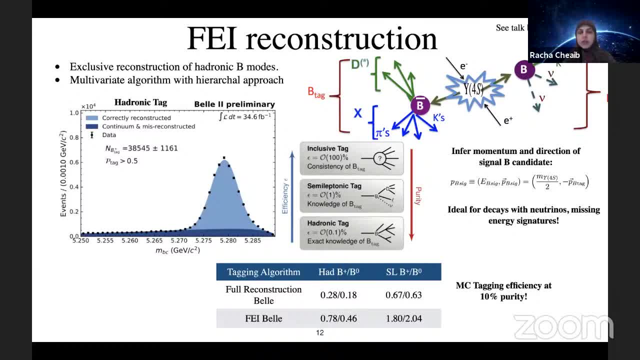 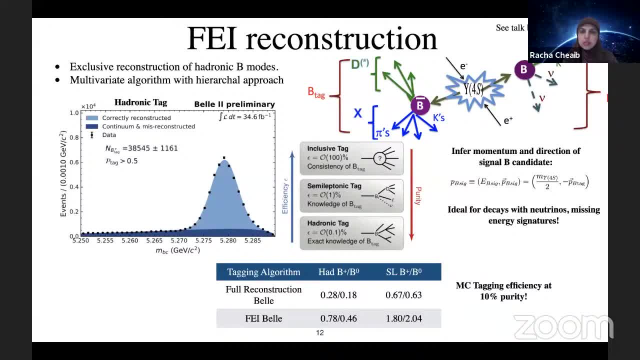 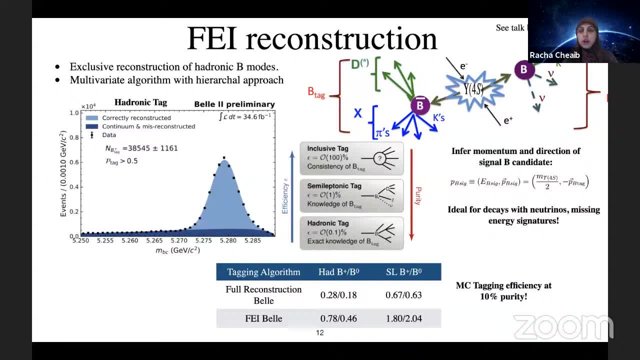 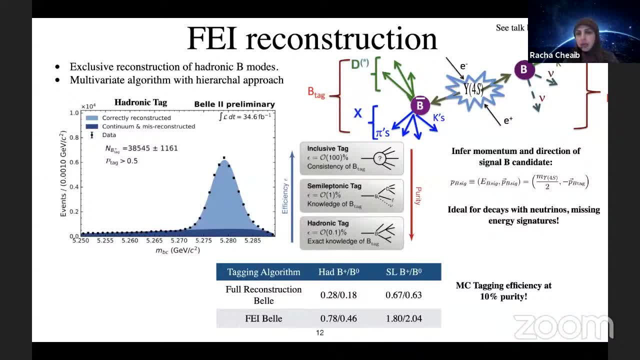 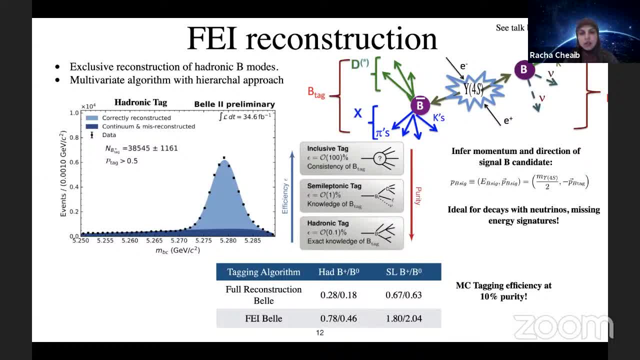 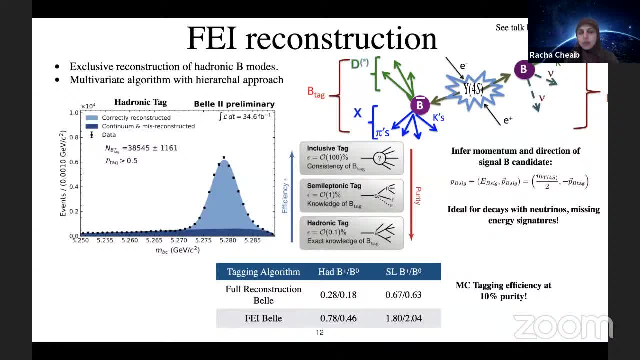 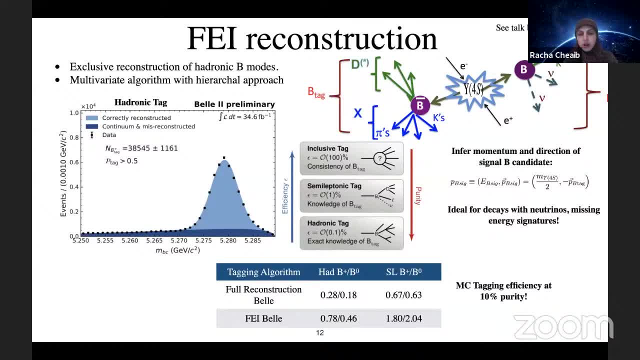 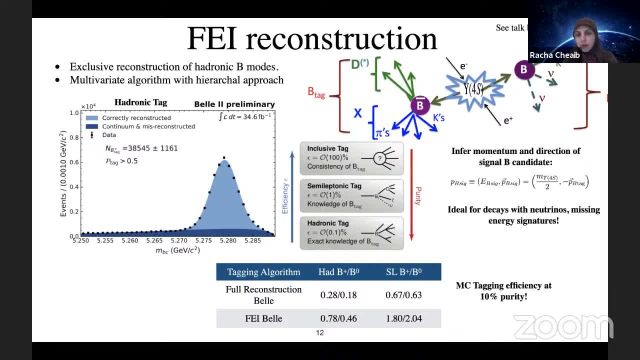 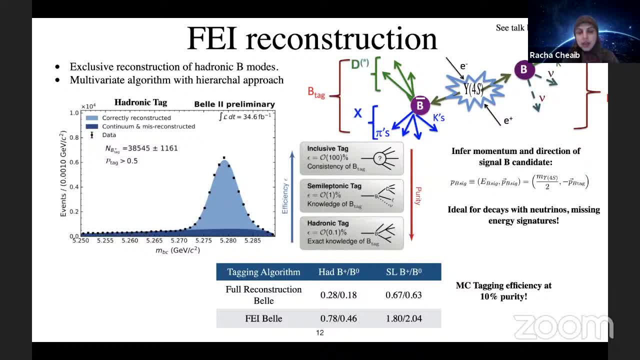 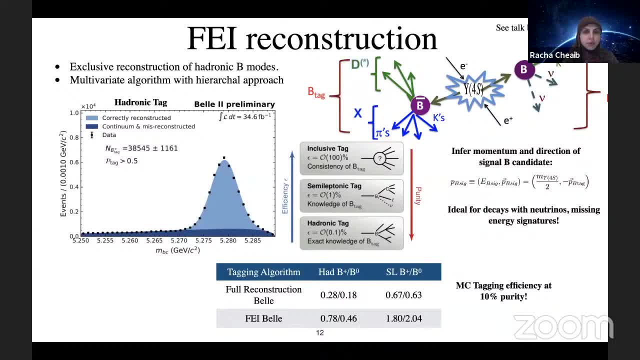 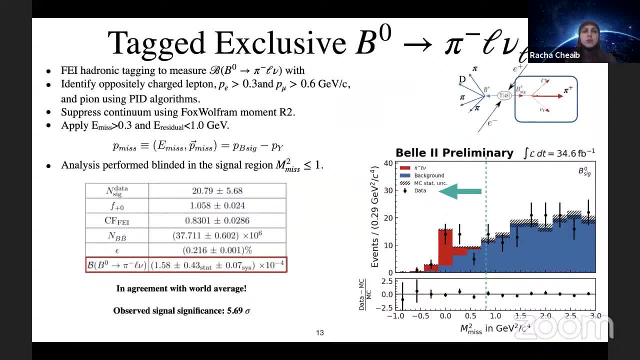 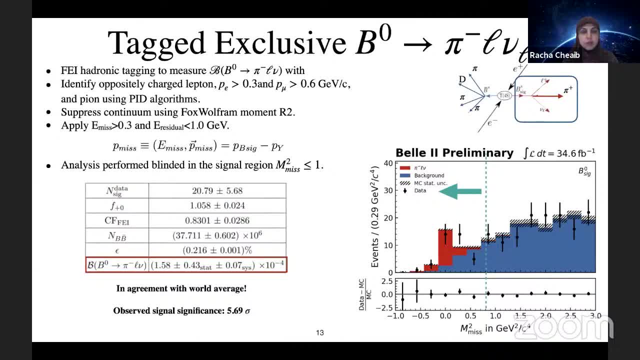 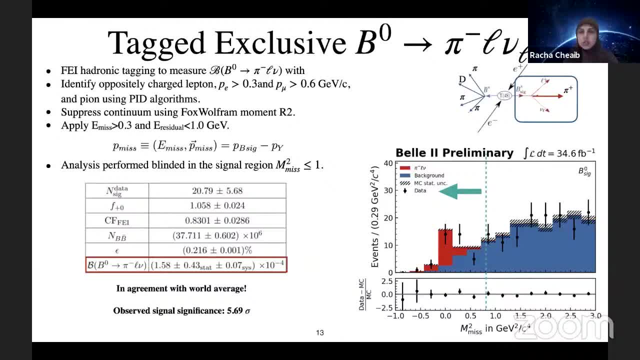 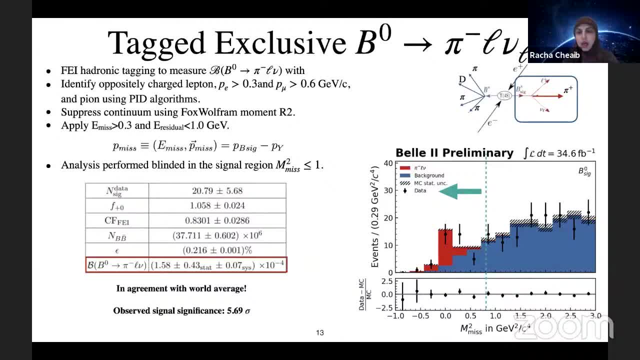 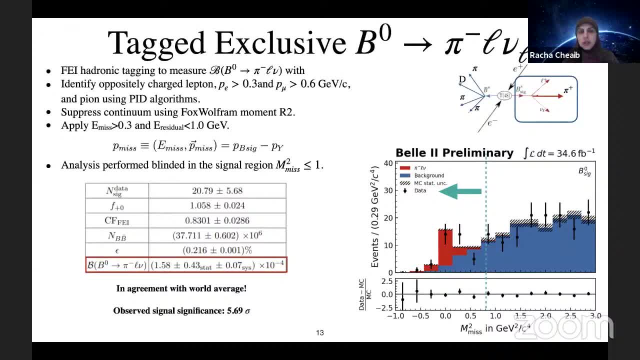 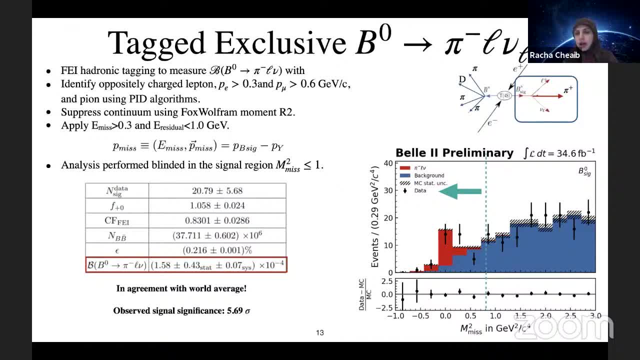 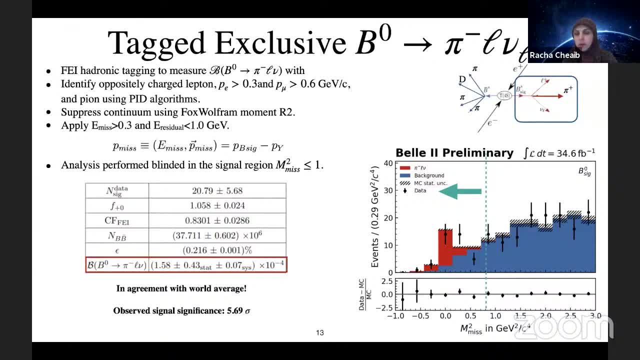 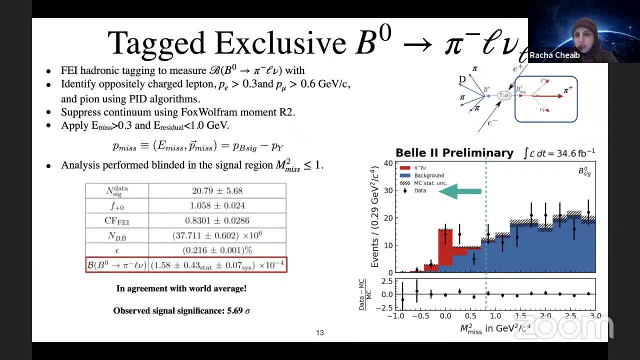 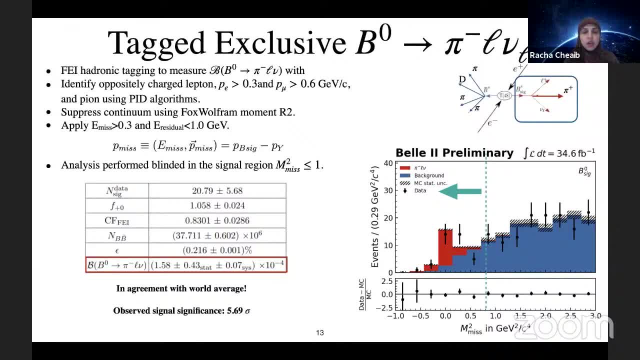 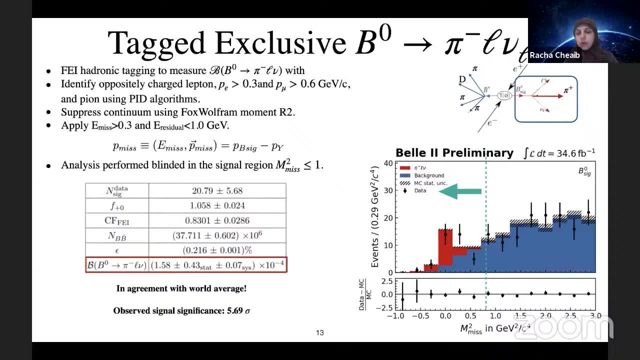 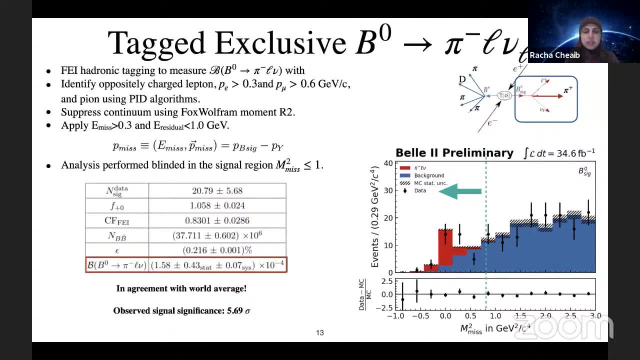 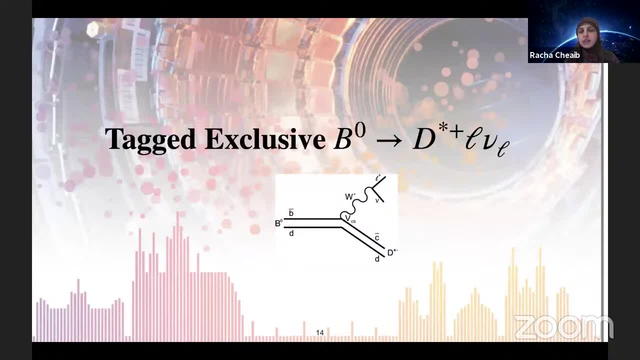 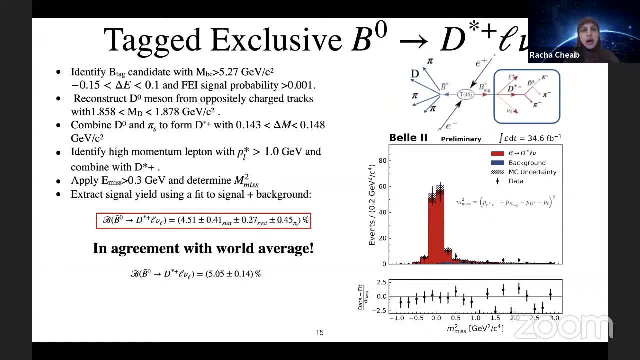 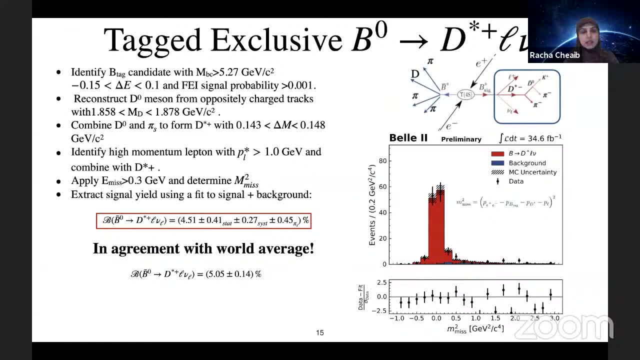 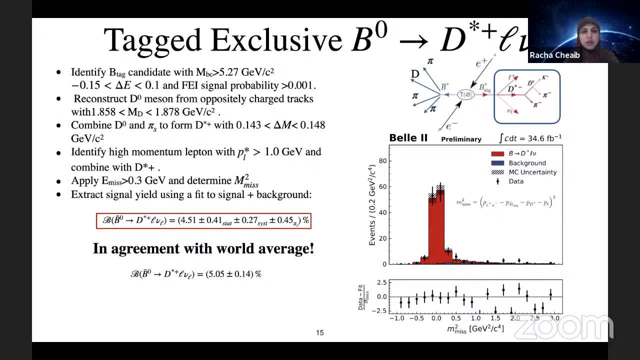 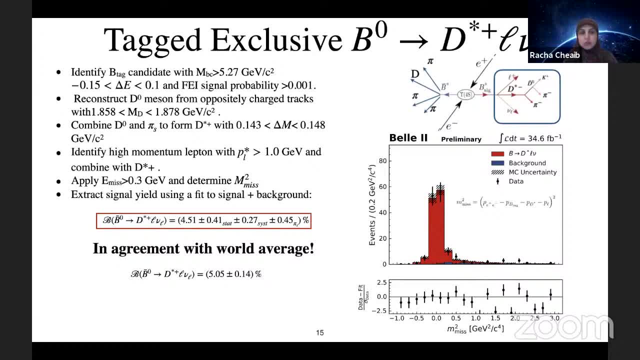 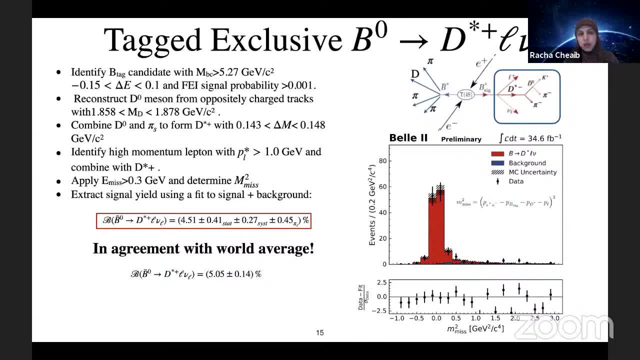 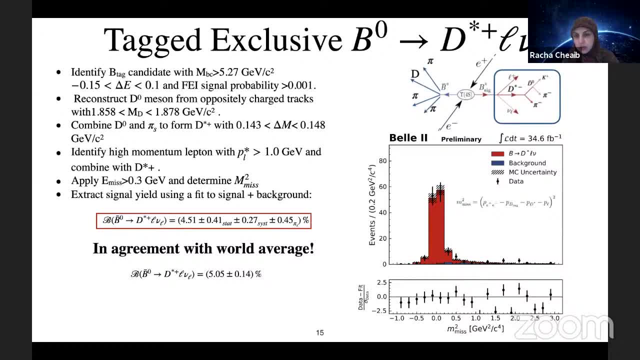 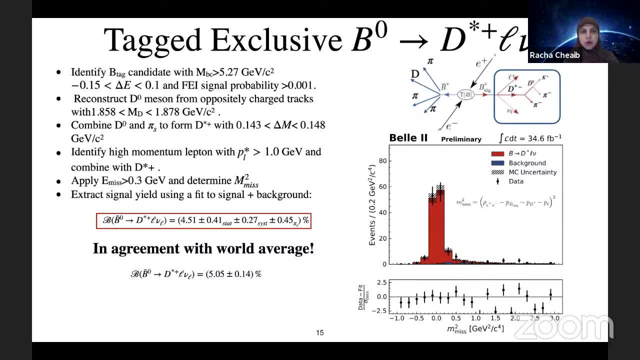 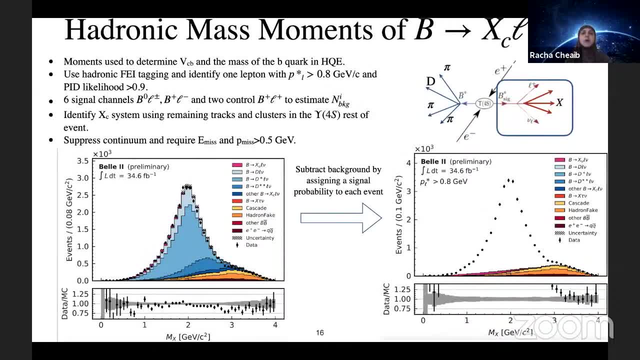 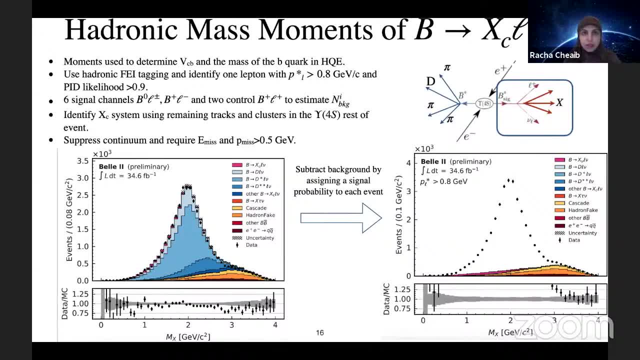 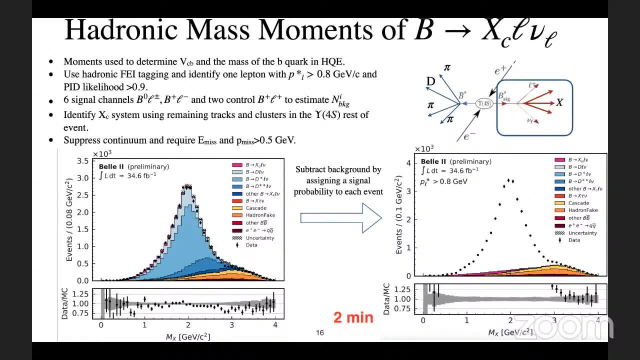 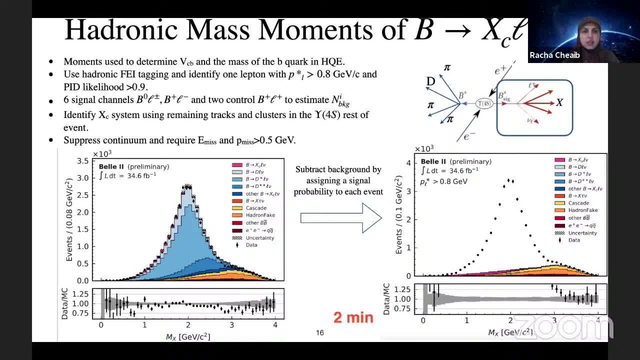 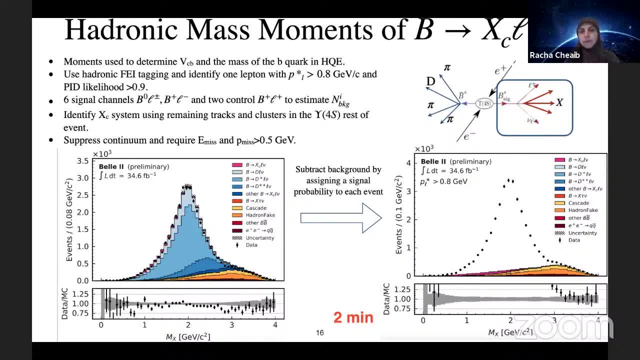 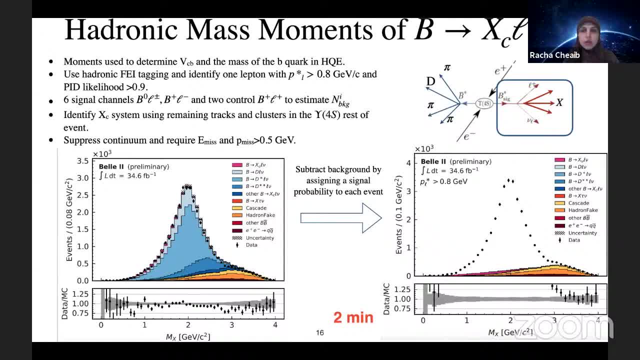 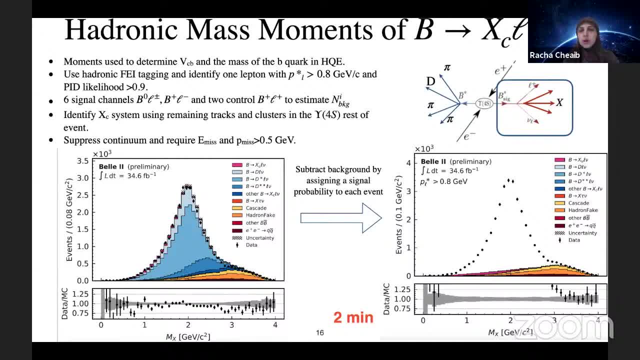 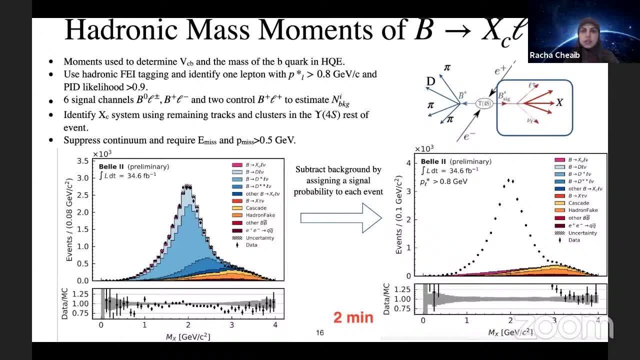 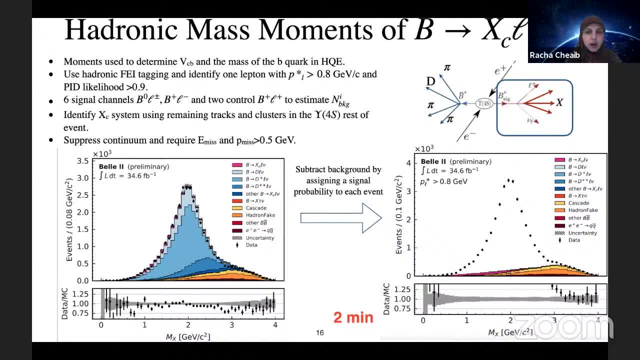 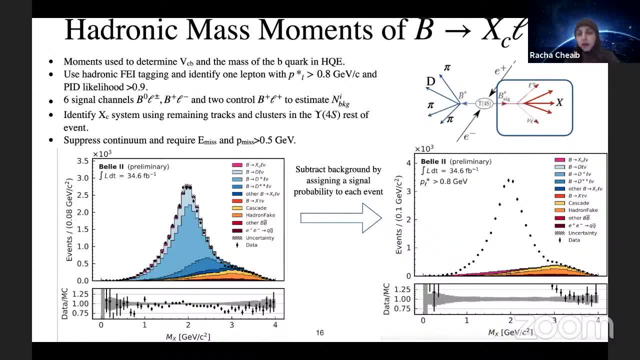 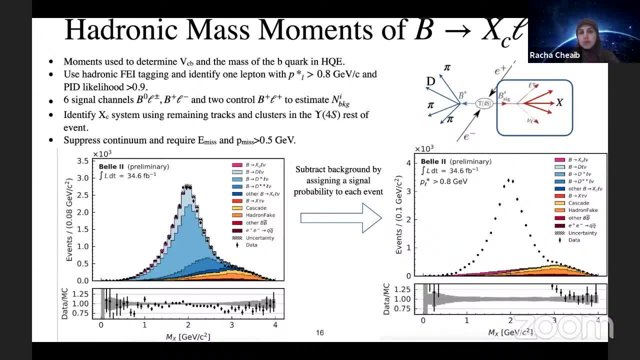 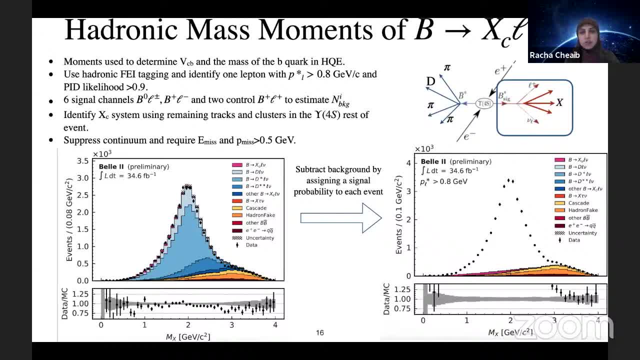 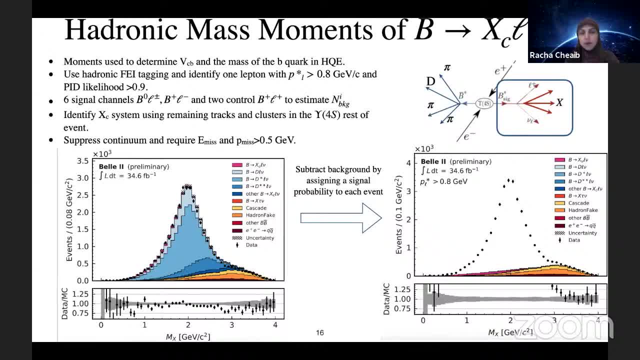 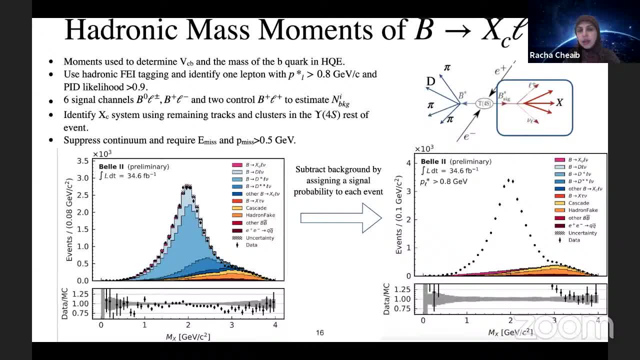 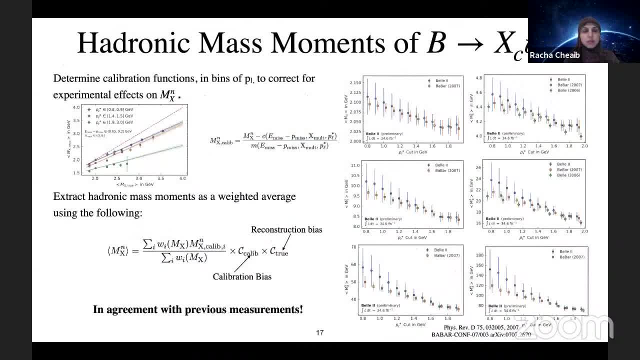 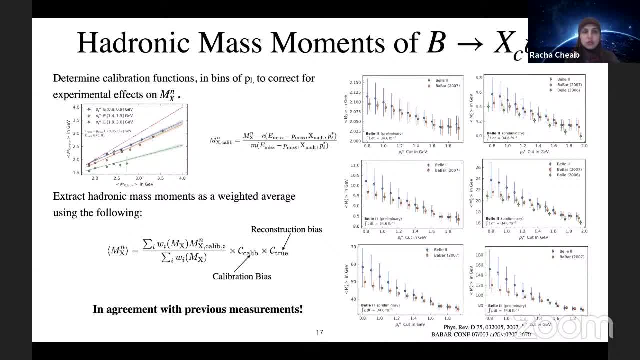 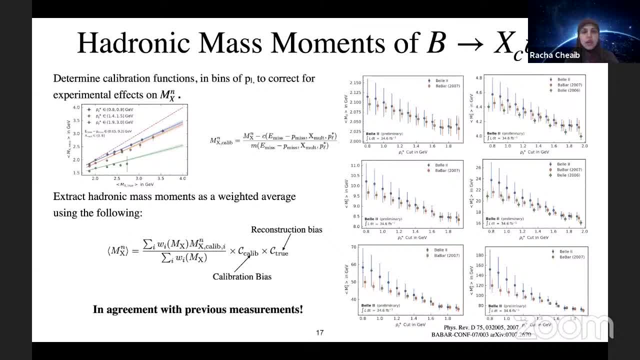 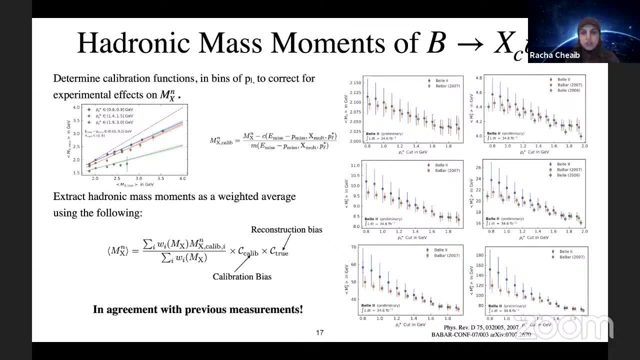 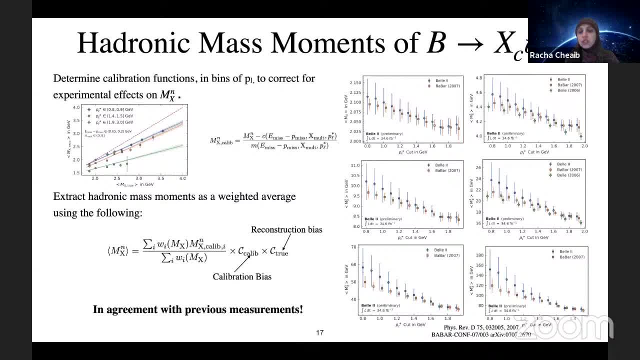 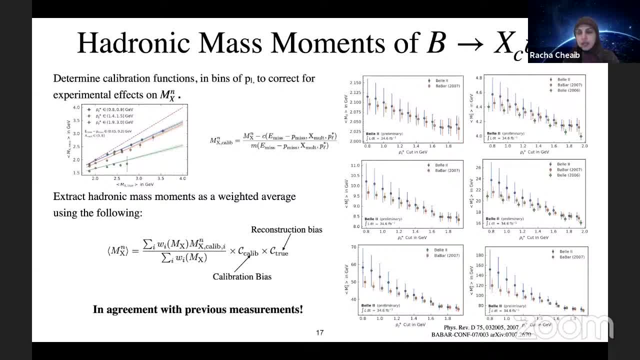 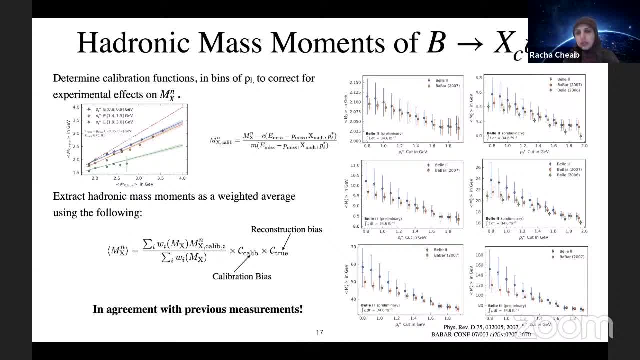 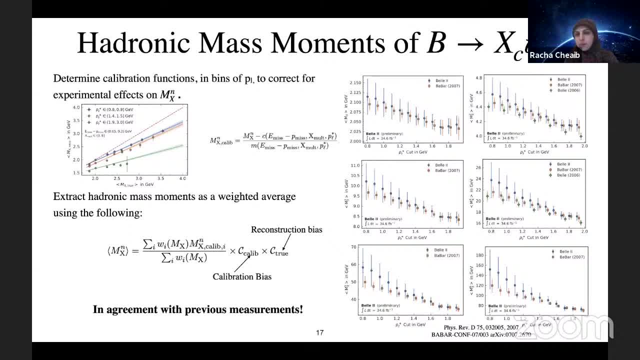 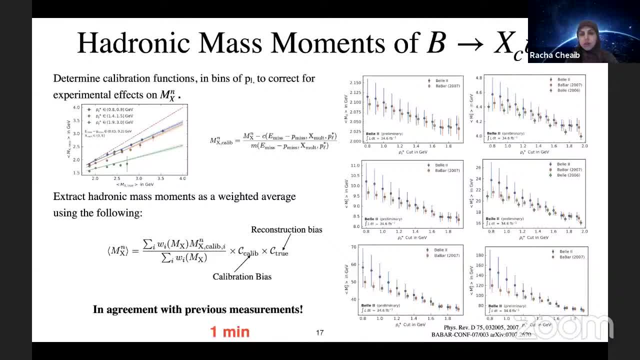 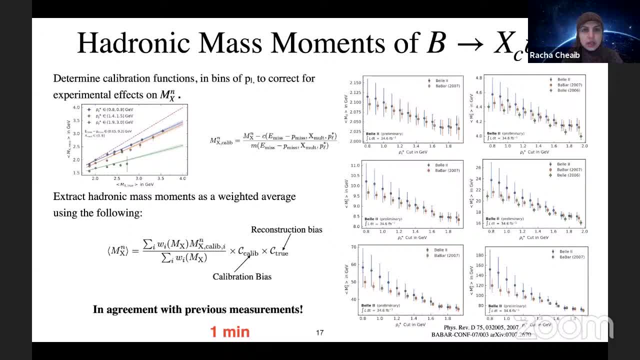 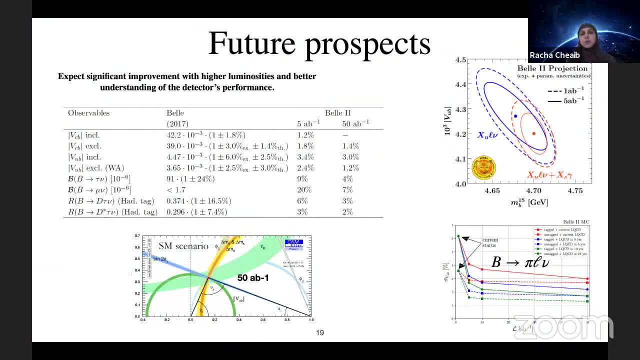 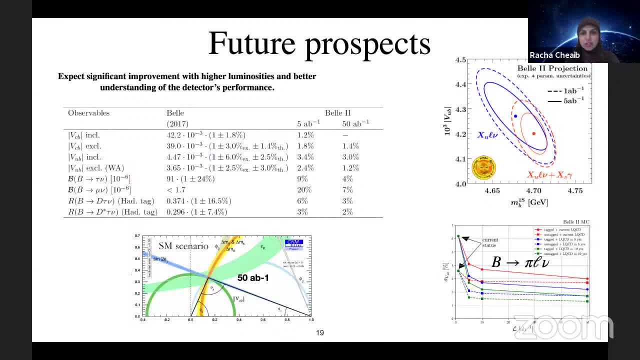 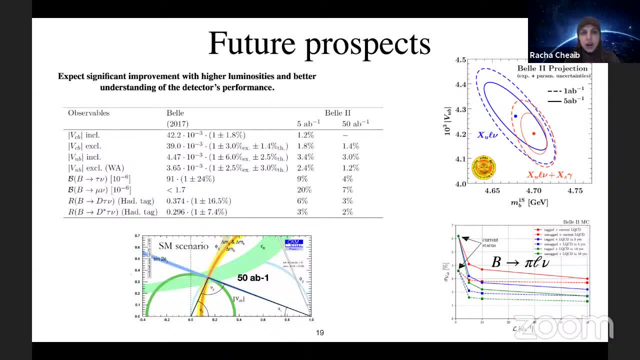 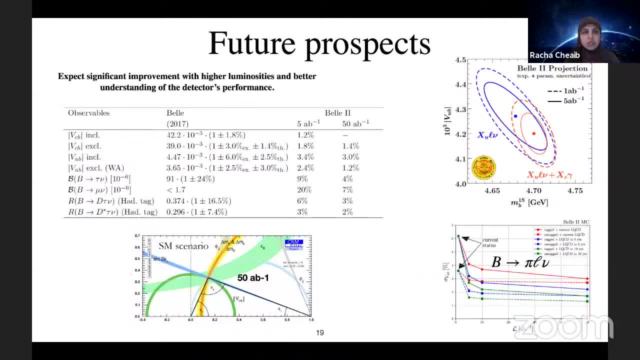 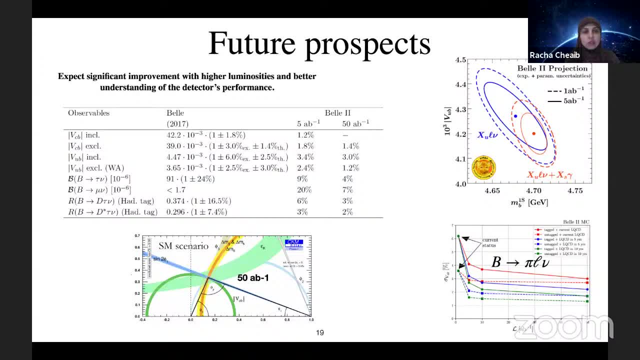 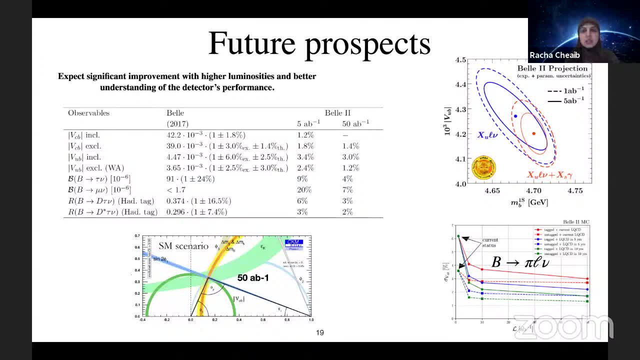 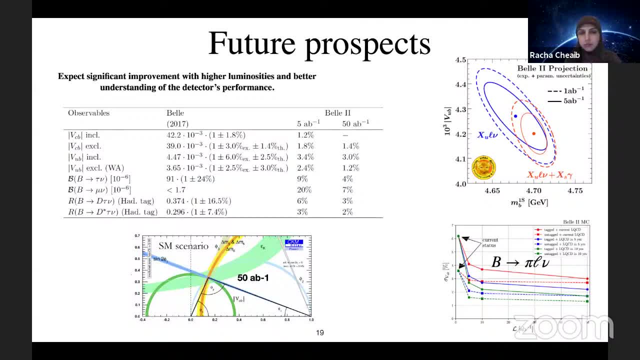 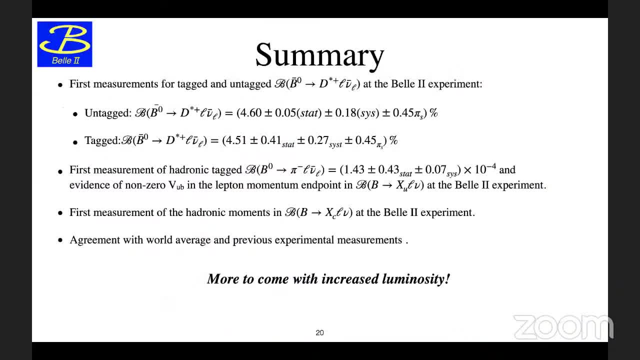 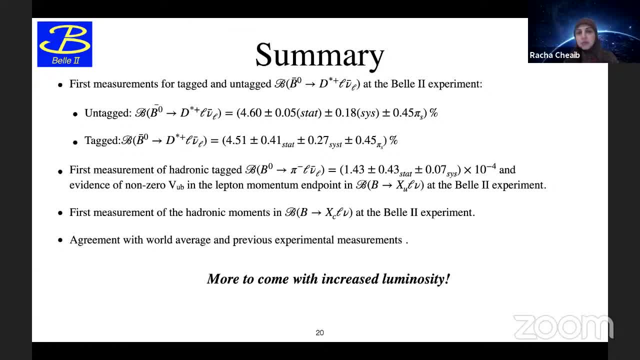 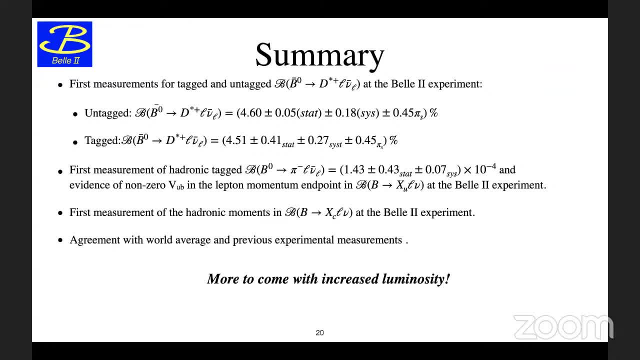 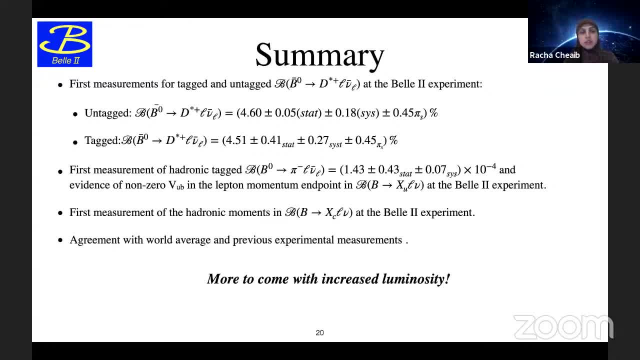 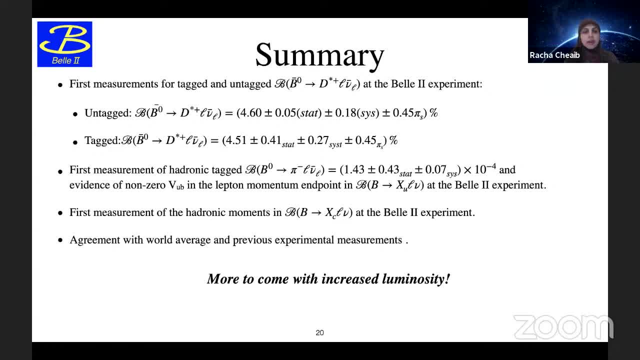 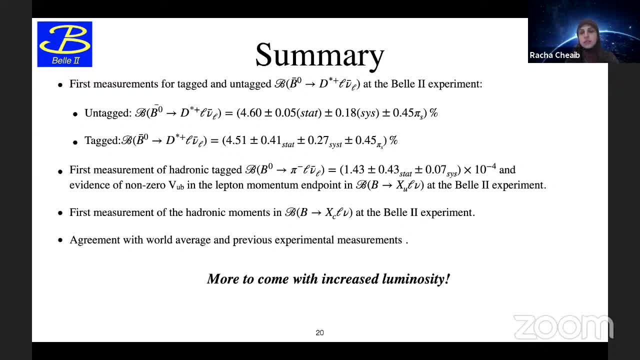 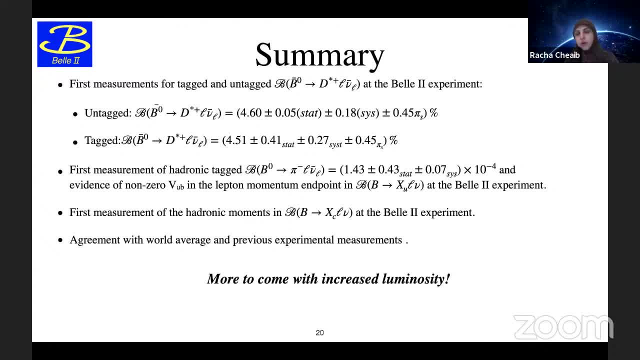 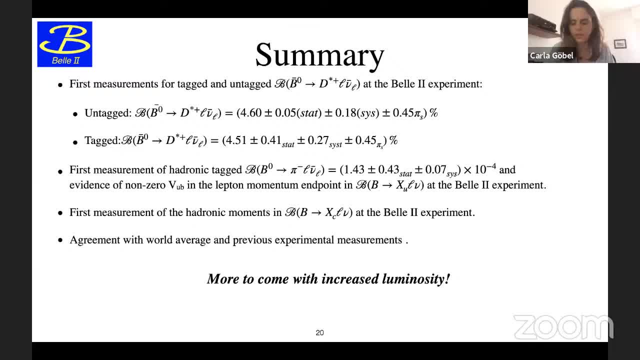 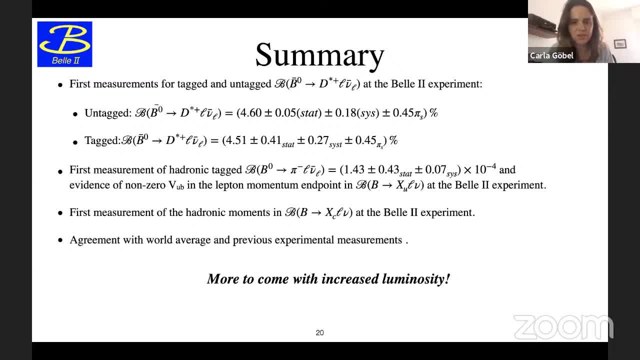 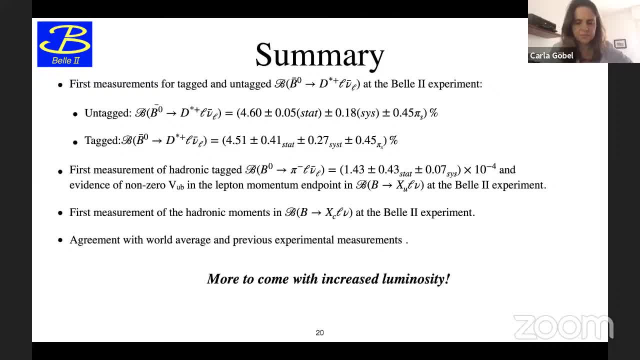 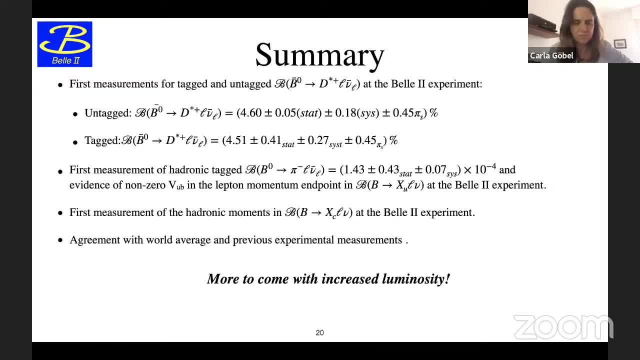 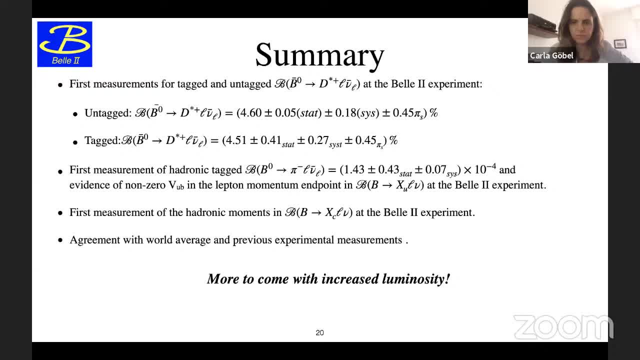 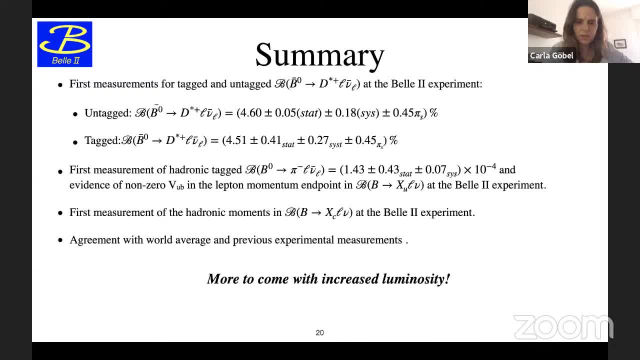 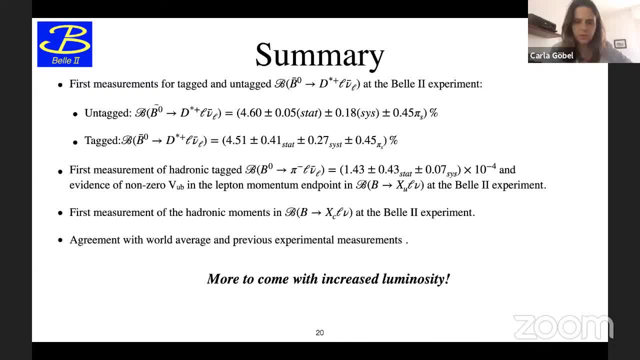 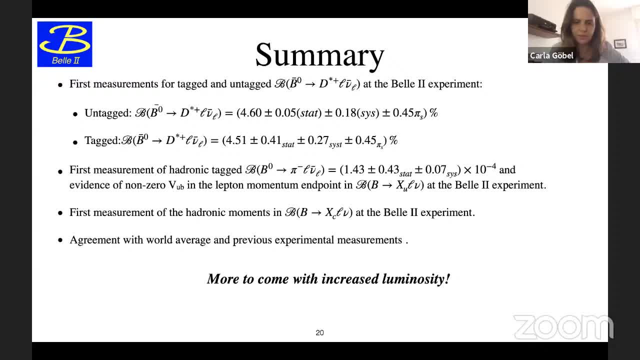 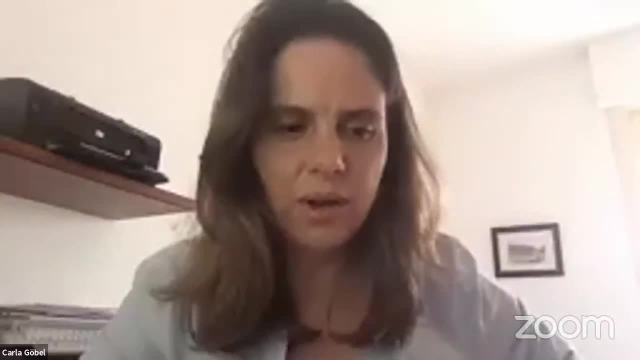 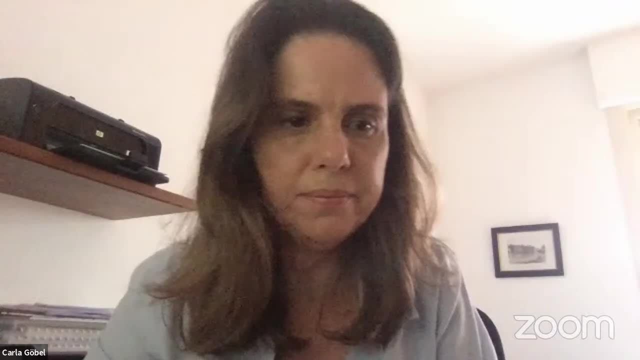 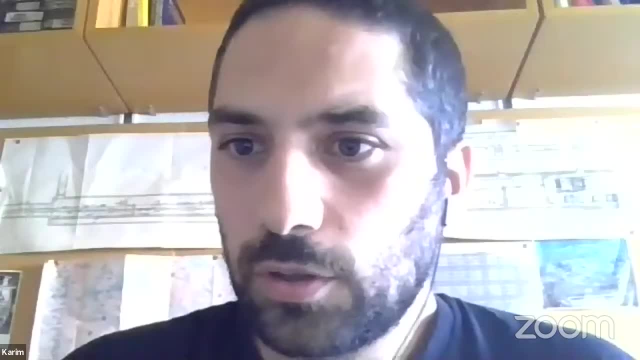 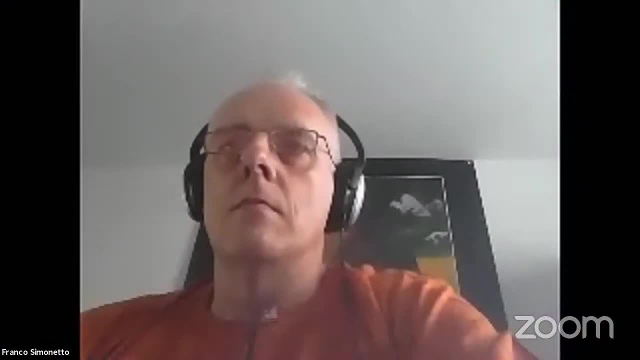 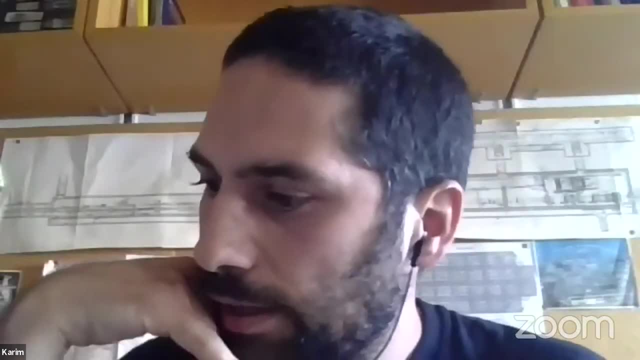 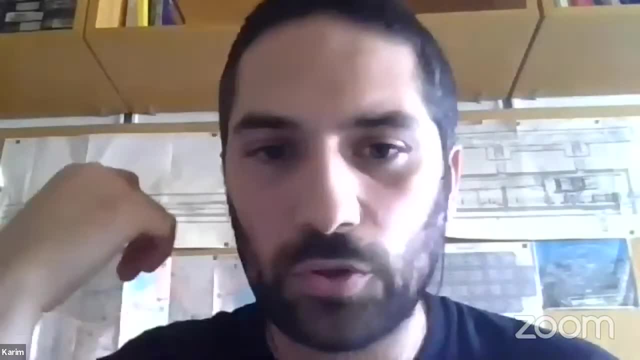 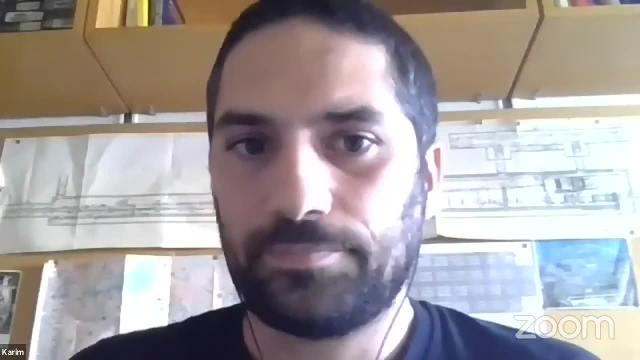 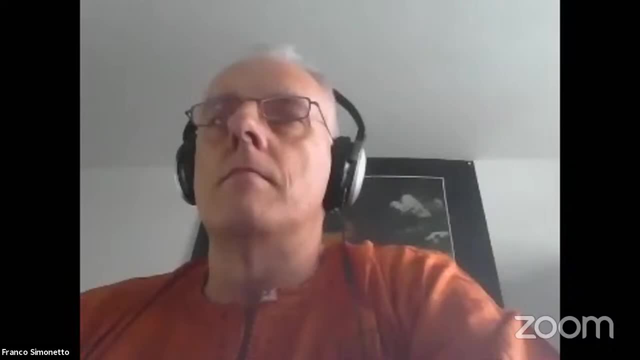 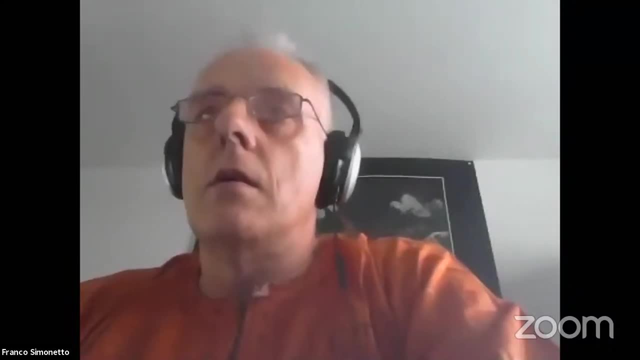 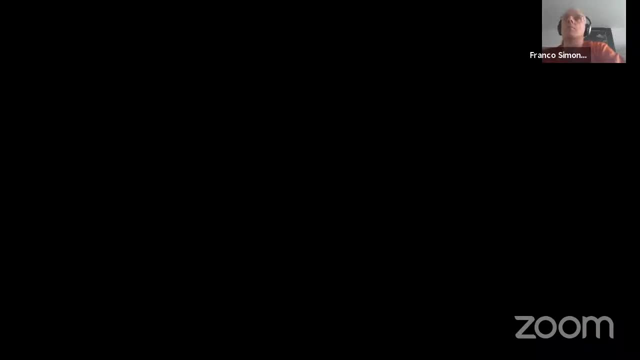 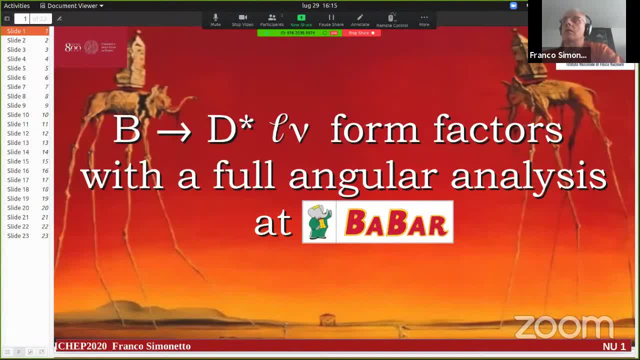 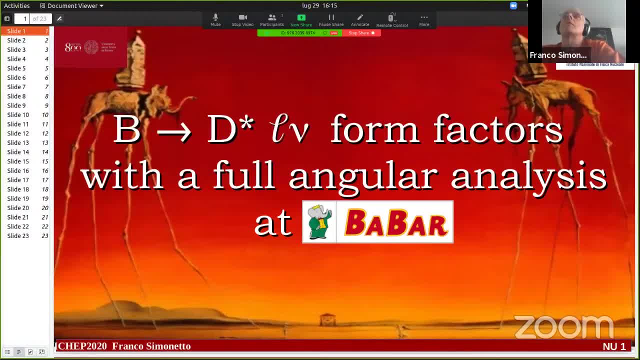 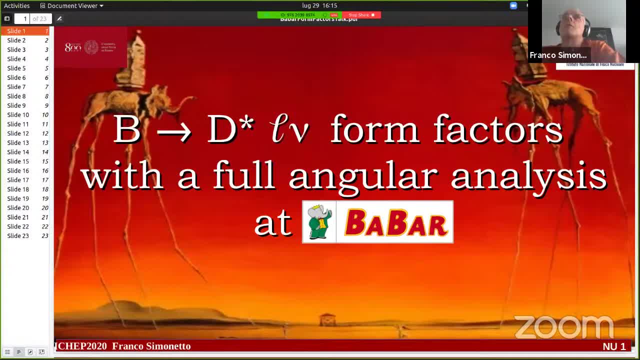 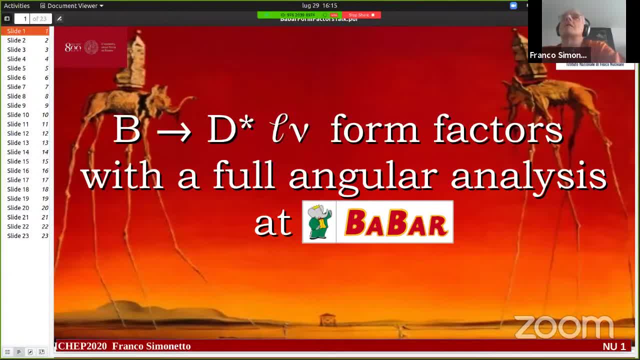 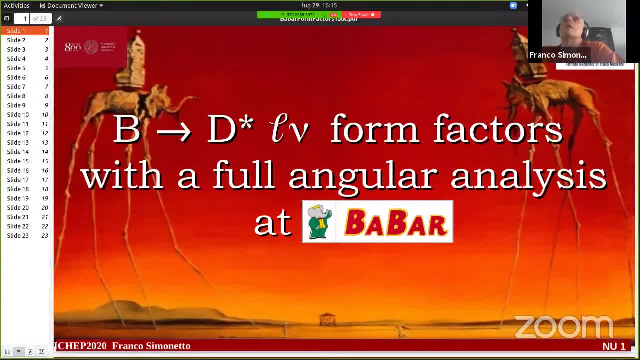 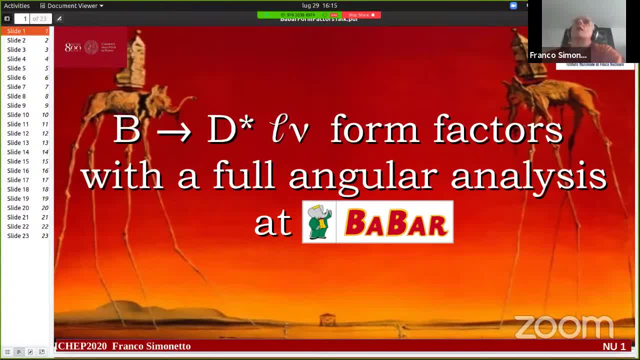 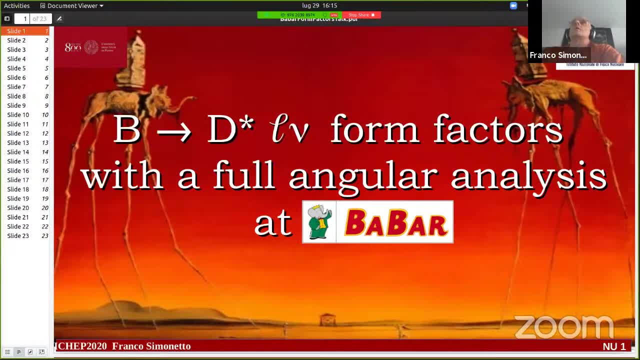 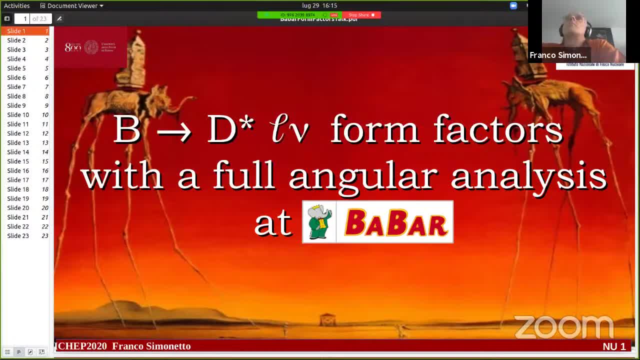 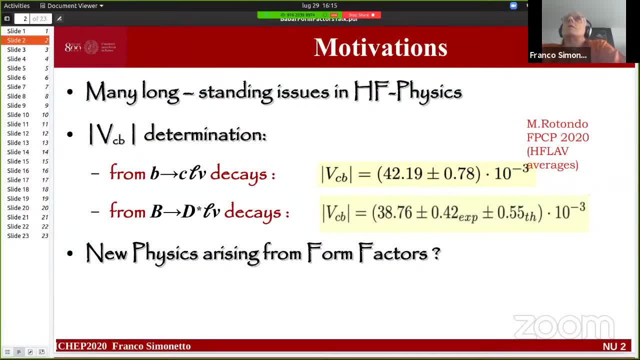 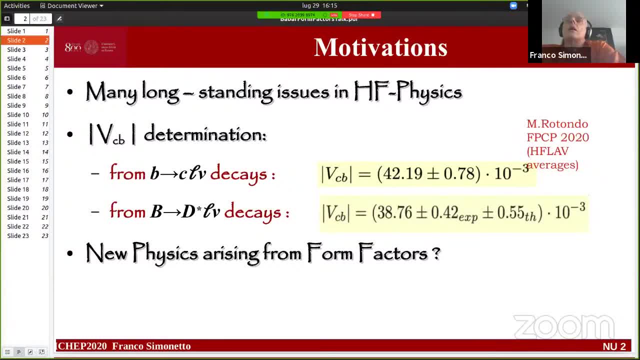 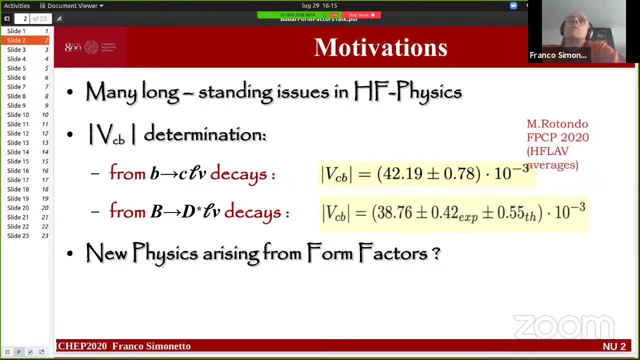 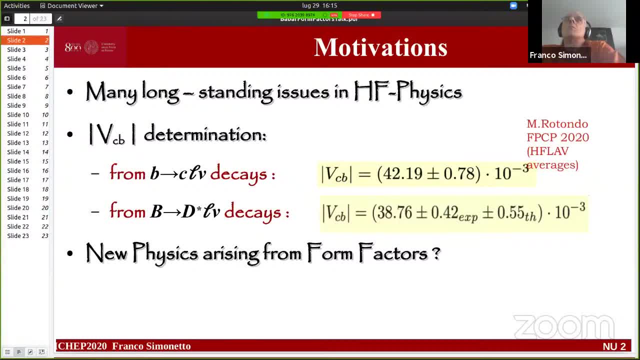 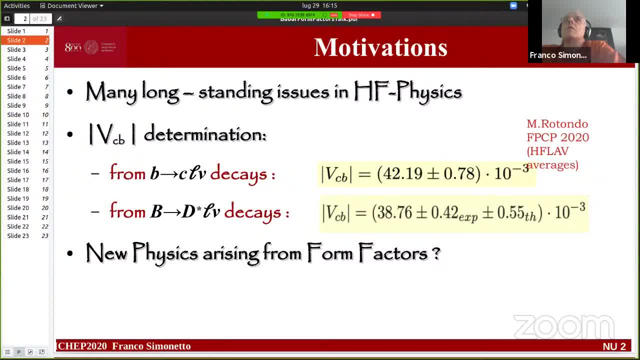 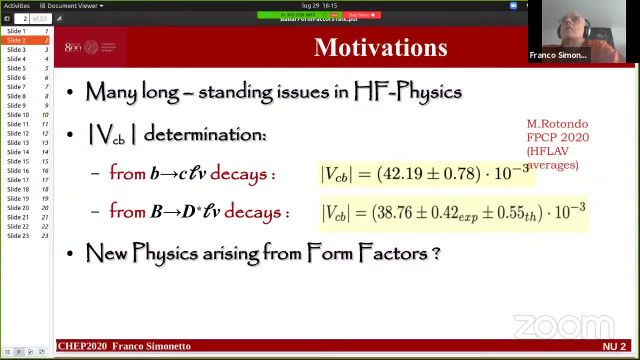 And then exclusively, is where we fully reconstruct the X system which is seen, which might either be a sign of some problems in our understanding of the decay processes which bring to these final states, or maybe could even be a hint that there's new physics. 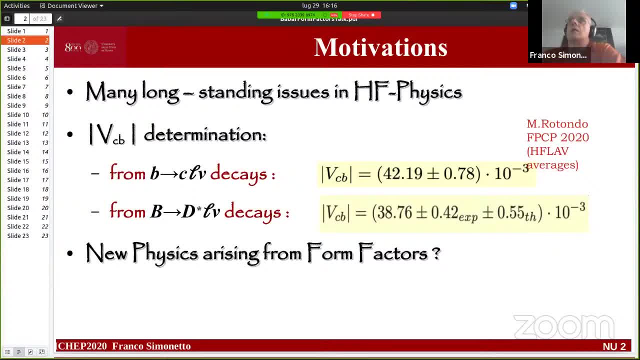 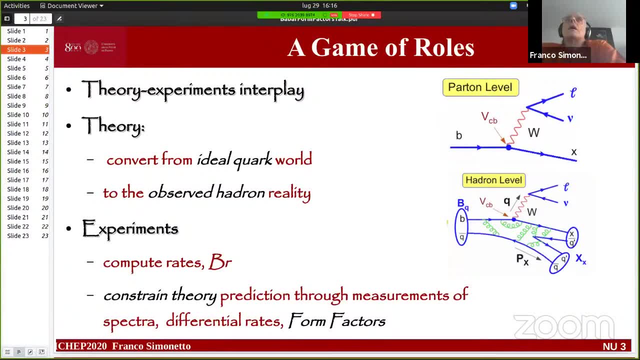 in the form factors which describe the decays. Let me briefly remind the game of roles. by one side, this is a measurement which exploits a deep interplay between theory and experiments, because the role of theory is to convert from the very beautiful ideal and easy life at the fourth level world to the hard reality. 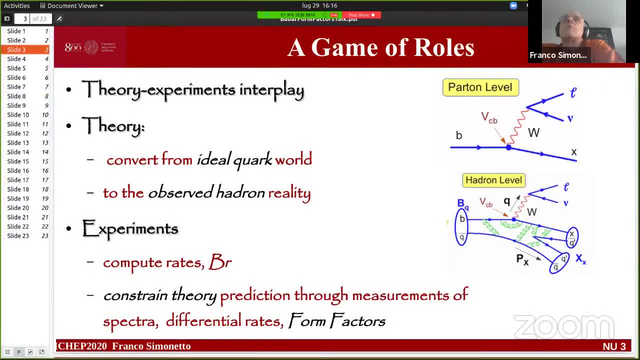 of the absurd hadrons, Then the role of the experiments is, of course, to the computer. In addition to that, they can provide constraints to the theory by measuring spectral shapes, differential rate and particularly form factor, as is the case for this talk here. 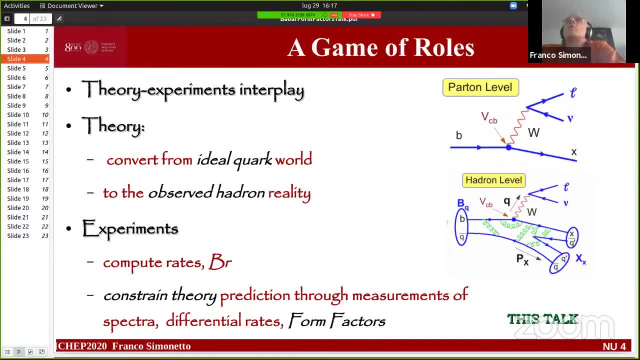 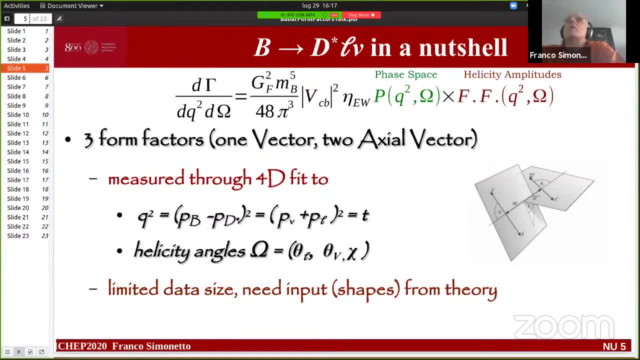 So you have already seen this formula before. you know that we can decompose the partial decay rate in terms of well-known parameters and so on. In fact, it can be measured as a Fermi constant, then some electroweak correction, VCB, which 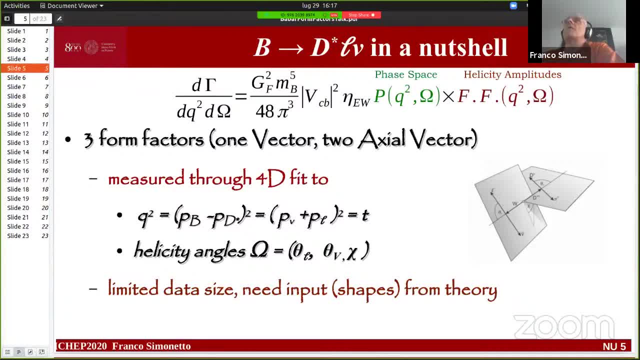 is the name of the game, then phase-space factors and a term which is connected to the elasticity amplitudes which describe the decay, which can be also formulated in terms of three form factors, one vector and two axial vectors- And in fact, they can be measured or, I should say more correctly, constrained. 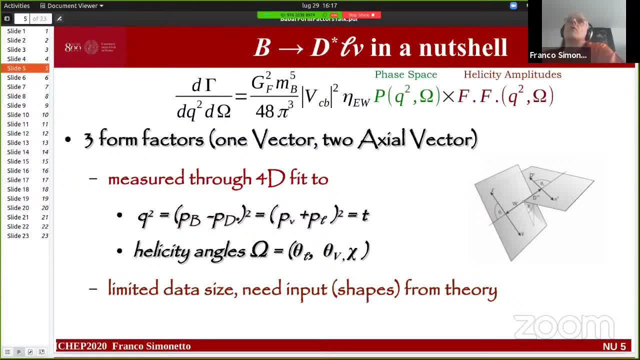 And in fact they can be measured, or I should say more correctly, constrained. And in fact they can be measured, or I should say more correctly, constrained To a four-dimensional fit to well, the Q square, the square of the momentum carried. 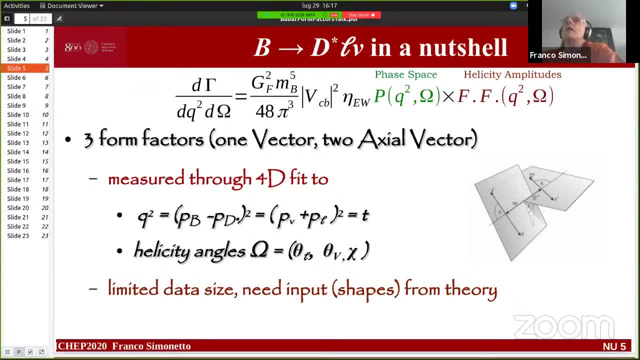 by the W-mason and then three-elicited angle which parameterize in detail the details of the decay of the W and of the discharge. Due to the limited data size, however, you cannot really determine the shapes of full factor just from the measures. 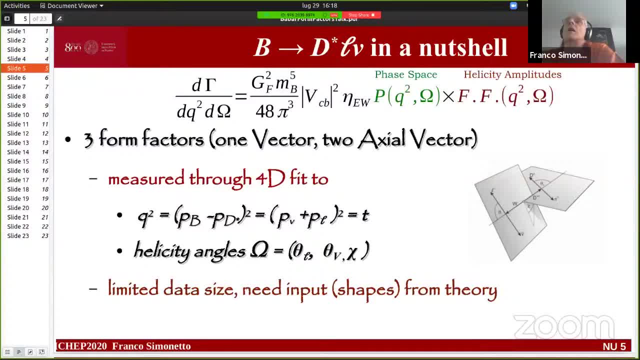 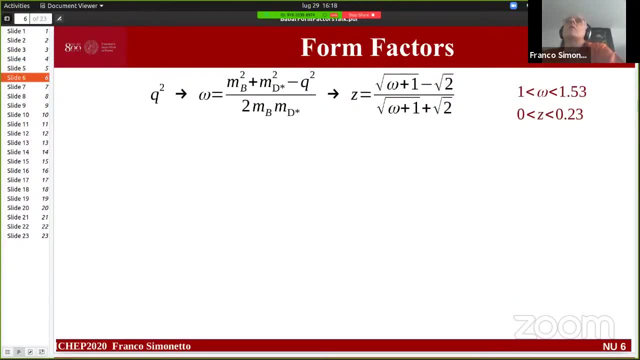 But you need some input from theory and then you can interpolate the theory prediction, determining a few free parameters. So the first step in determining from factors is redefining the variables in such a way that they are easier to be dealt with. So we move from Q square to the omega, which is in fact V times V and which is related. 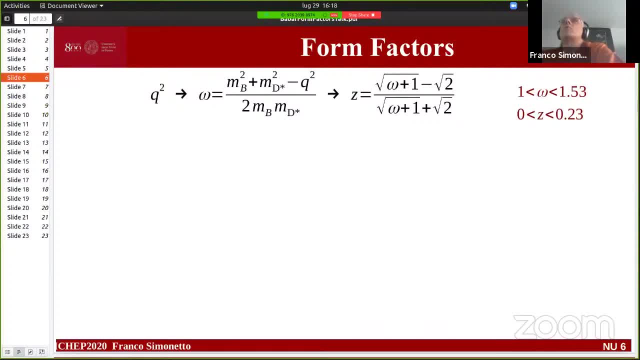 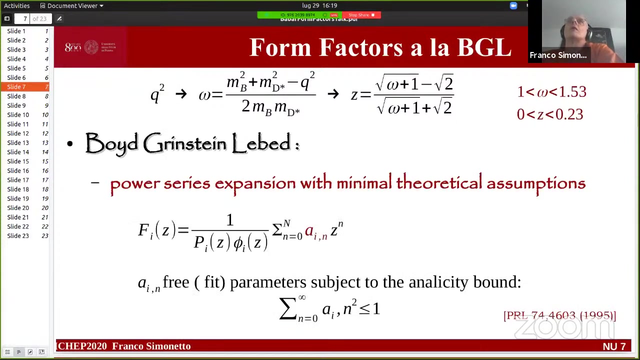 to Q square. in this way, Then omega can be mapped to another variable, Z, which has the quite proactive feature of being contained in a very small region. So perturbative expansions can be done in this parameter, And that's what, for instance, I'm done with the parameterization of Voigt-Greenstein-Lebed. 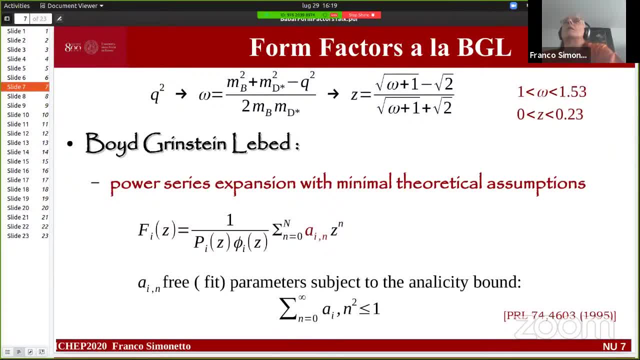 which expressed the form factors in a power series: expansion with a really minimal expansion. And then omega can be mapped to another variable, Z, which has the quite proactive feature of being contained in a very small region, So perturbative expansions can be done in this parameter. 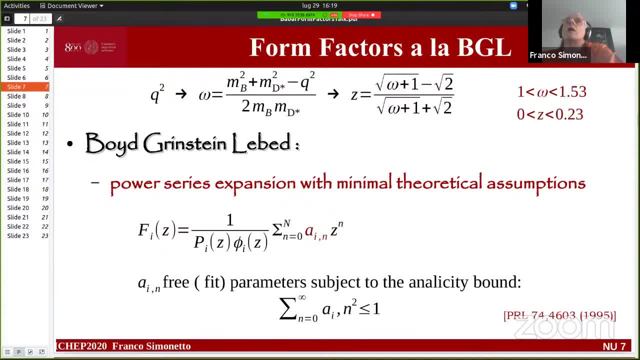 And then omega can be mapped to another variable, Z, which has the quite proactive feature of being contained in a very small region. And then omega can be mapped to another variable, Z, which has the quite proactive feature of being contained in a very small region. 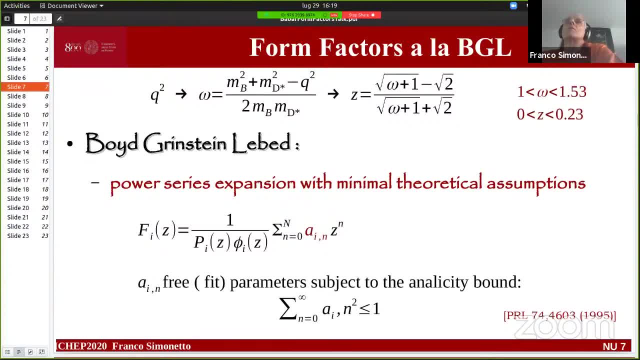 And then omega can express the form factors in terms of well-known functions, and then a power series in Z which depends on Q, unknown parameters that lie in this AI, While they are free parameters, but they have an unani-city bound which limits their maximum. 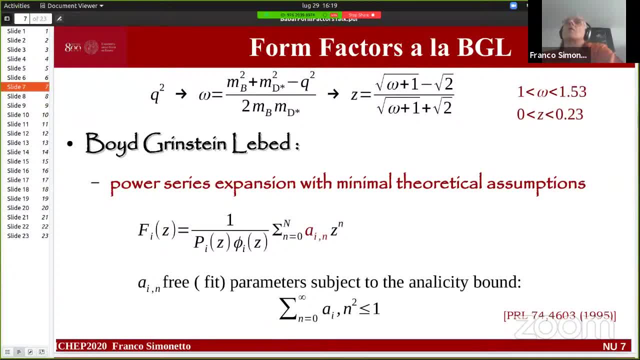 possible values, Or they should be a small. So where's the route D었어요, Any way, OK, All right, All right, Ok, All right. sum of a: i must be less than one. okay, so in practice, then, for this measurement we will not. 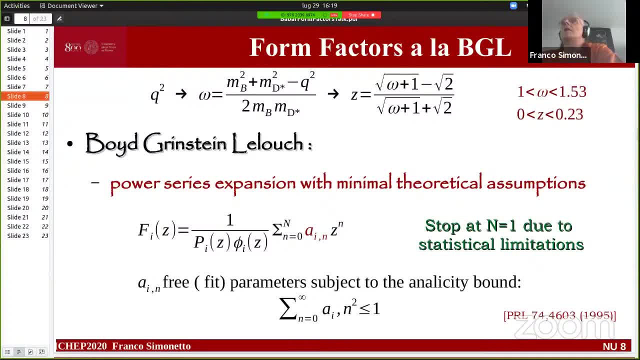 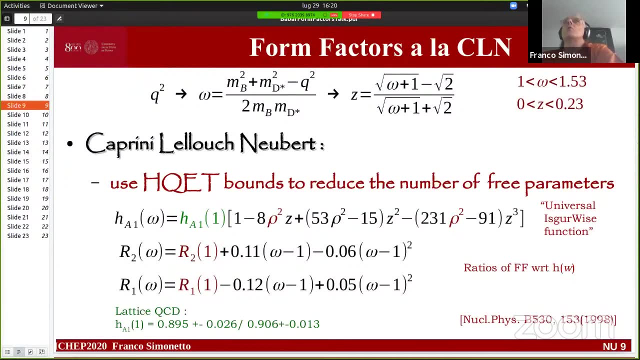 push the fit, the development to infinity. stop at 10. 1 equal to 1. due to statistical limitations, an alternative approach has been proposed by caprini, lelouch and albert. this is a bit more aggressive than the other one in the sense that it uses hqt bounds to reduce the number of free. 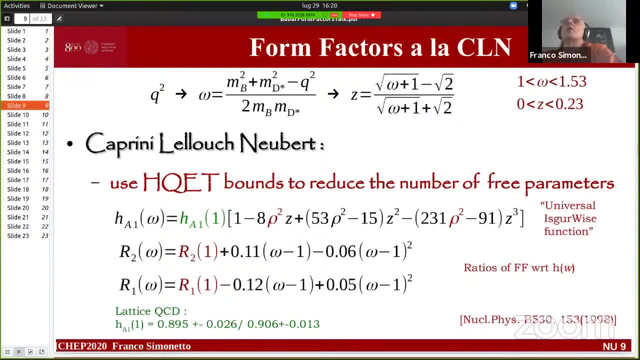 parameters, so that we have this expression for the form factor, the one of the actual from factor, which is expressed in terms of a normalization term produced, produced by light, sqcd and the slope. and then we have the other two perfectors that are expressed as ratios to the first one. 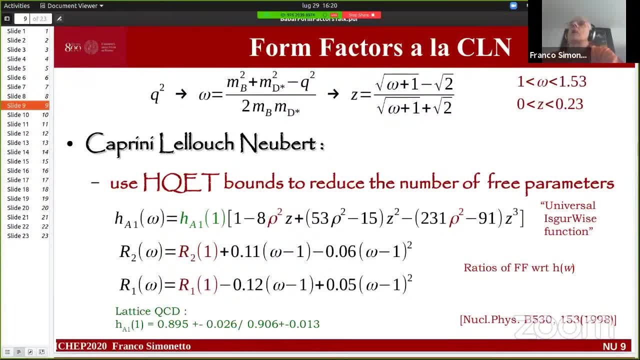 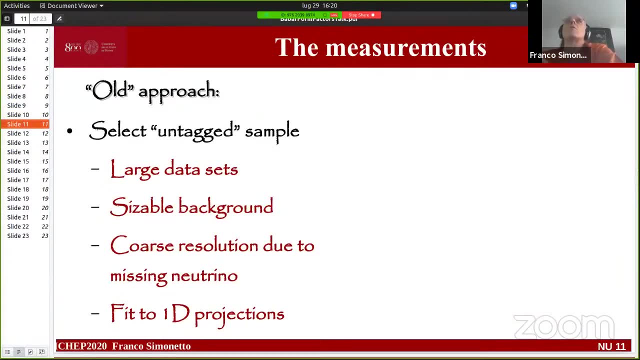 and the only three parameters are the normalization of the two ratios. so basically, for with this approach, you need the only need to fit a slope and two normalization parameters. coming now to the measurement, we have seen in the previous nice talk what we i would like to call an old approach, the 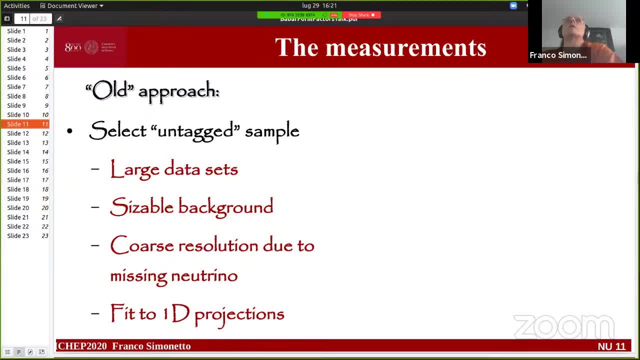 first approach that all experiments has been following since the time of clio and glap and basically you select what: an untapped sample which provides you a larger like a set, however with a sizable background, with a course resolution, because you missed the neutrino and up to now all experiments didn't perform a full fit, but they fitted to one. 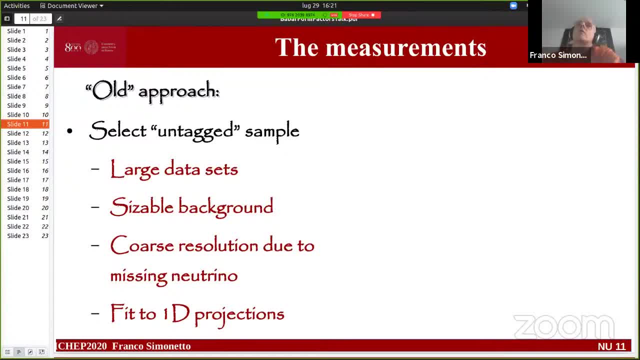 bit projection and then take it and cut into account correlation to get to the result. what i'm showing here now instead is a new approach based only on paged event, which gives, however, a small data set but, as we will see, with the algebraic background, with the two. 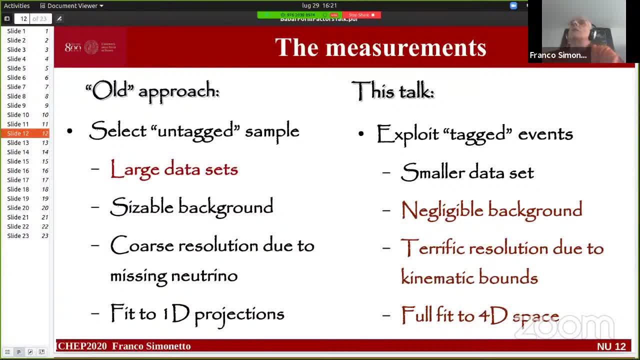 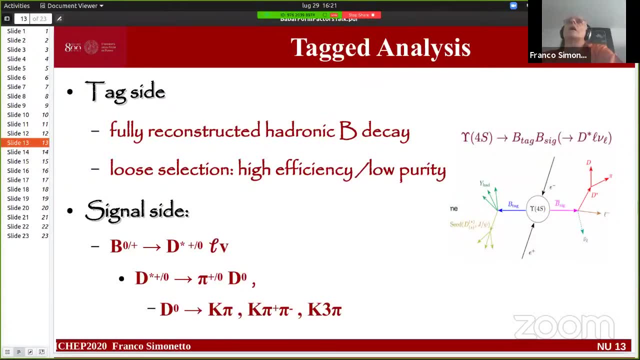 rific resolution in each of the parameter due to kinematic bounds which allow these two facts allowed to a full effect to the 4d space. so it's a type of analysis. so we have the tag side and the signal side. the tag side consists that we've seen before in folder reconstructed that don't be the. 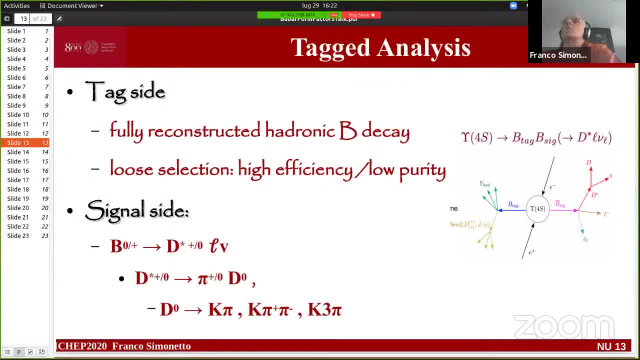 case we use a 10 000 modes or less, which gives a very loose selection with high efficiency and low purity. but we don't care about the low purity because the signal side is practically here. we have a fully reconstructed semi-leptonic decay where only the neutrino is missing. so in the end we have 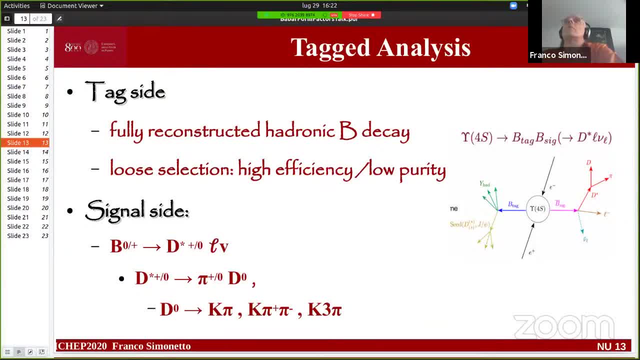 very clean data sets. so as for the selection, i wish to underline that we have a very constrained system because we know everything about the two. i've been fully going to select and i constructed one of the bees. we know everything about the other. then we have max constrained. so it's an over constrained system which allows us for. 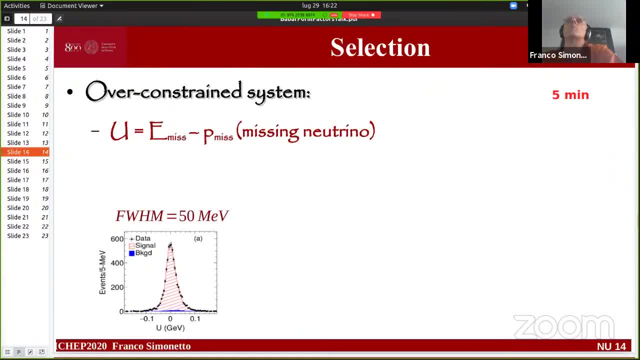 instance, to reconstruct both the energy and the momentum of the missing neutrino and compare the two of them. and so you see what's the resolution that we get when we make the difference between the missing energy and missing momentum. it's of the order. sorry, i wrote the error. yes, yes, the full. 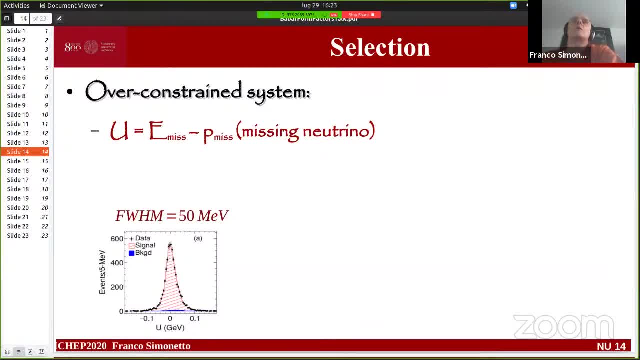 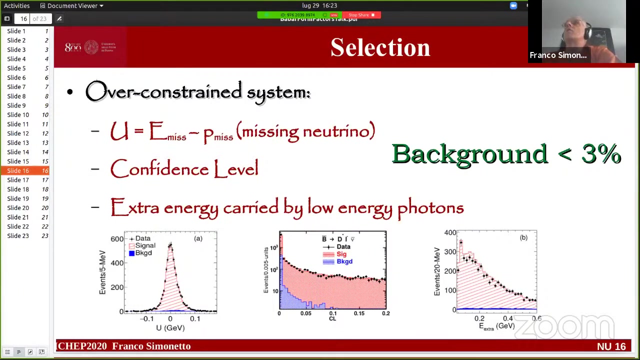 resolution is about 50 meb, which is quite a score for neutrino reconstruction. in addition to that, you can use the confidence level of your overall feet in order to further decrease the background. and then we also have a time, a light cut on the extra energy carried away by low energy photons. 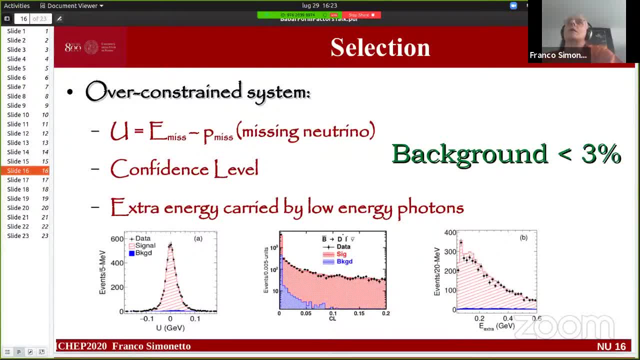 all in all, as you can see, by inspecting these plots which complete the reconstruction of the system, we can see that we have a very good signal-to-noise ratio. so if we maintain all the cuts, apart of those for the variable we are looking at, you see that we have a wonderful 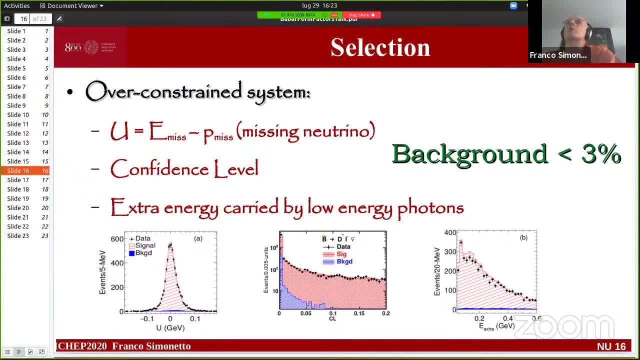 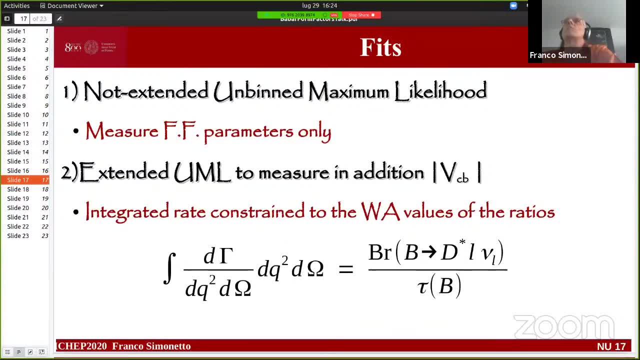 signal-to-noise ratio background is below three percent, which is quite a score for semi-leptonic measurements. so, as fits, we perform a couple of them and not extend the mean maximum likelihood, in order that you know that to determine just the shape parameters can we also perform an extended and being maximum likelihood. where, however, we feed our feet from? 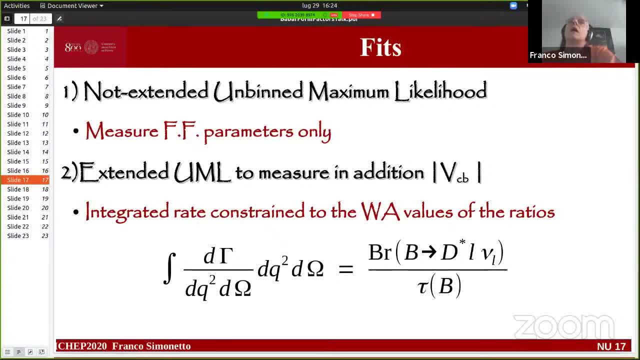 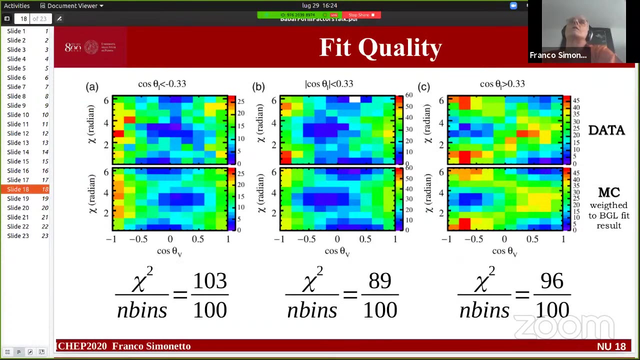 with information from outside. in fact, we ask that our integrated rate be equal to the ratio of the branching ratio and the lifetimes of the b involved, as provided by the h club working group. so first, before coming to results, i show you the fit quality. it's not easy to compare, but on top you have the data. 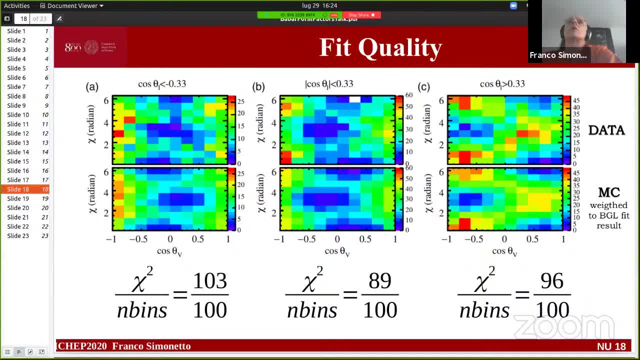 distribution for the chi versus cos theta v. i'm integrated along the q square in three means of cos theta l, so this is a an attempt to make a full description of all the variables employed in the. on bottom you have the how to compute of our monte carlo, reweighted to the fit results within two parameters corresponding to the. 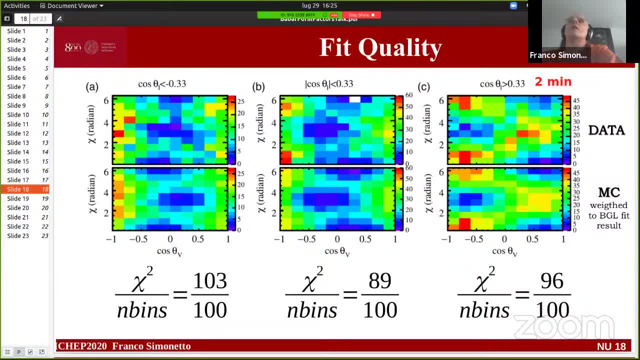 fit results and you should try a 2d comparison of the two plots. if your eyes are not well trained on that, you can look at the chi square over n bins which is coming out for each of these three plots to say that, all in all, we have quite a good agreement. 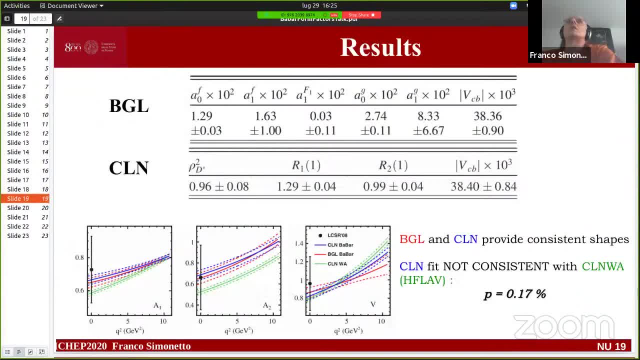 so now let's come into the results here i have, on top you see the results for the boy, the child, parameterization. on bottom you see the results for the caprini, lalu schneiber. well, these numbers are not going to tell you much. the value of bcb, you can see, it's quite consistent with the one. 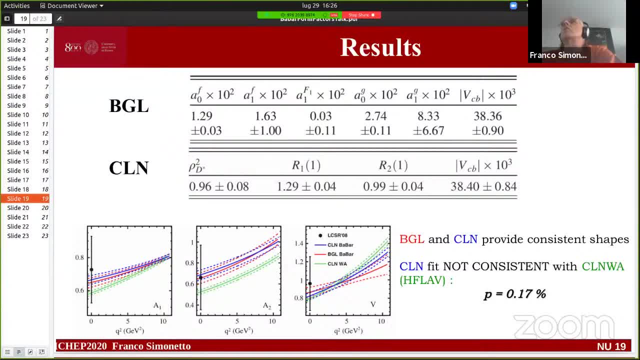 you have already seen in the past the statistics. the overall error, which includes statistics and experimental systematics, is small, but not as small as in other cases because of statistical limitation. what is worth to underline, however, is that you should look in the three plots where we show the form factors in the 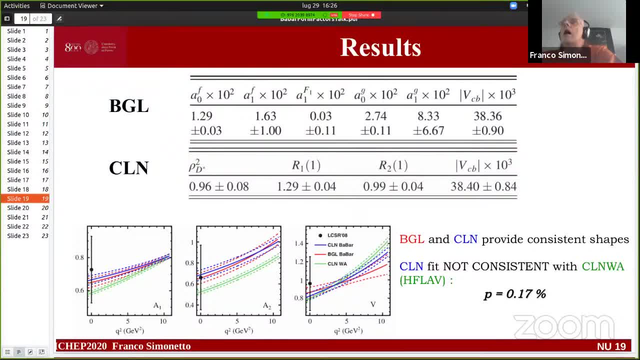 caprini parametrization. you can compare the blue line to the red one, showing that these are our experimental results and they simply confirm that our data are both consistent with both parametrization. boyd and caprini provide a similar result, even if they have different. 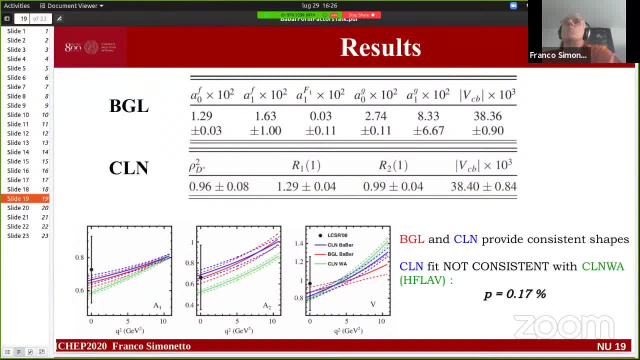 structure. what is more striking is the comparison of the blue line with the green line, because the blue line is our result, which are the mind you is much less dependent, for instance, on background and is driven by a much better solution with the word average, which is the green line. you see here. 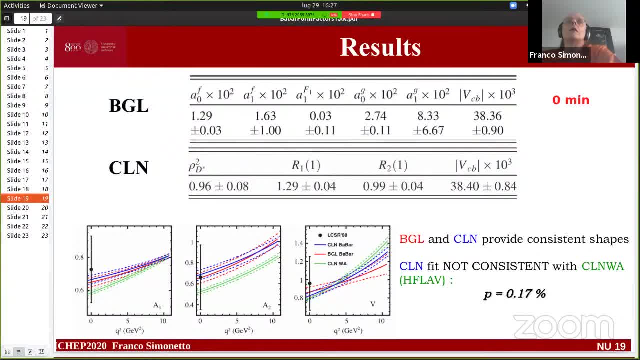 and you can see that in all the three cases, the two, the two curves don't match well. and this is particularly true if you look at the second actual vector from factor, where the difference between our feet and the world and the world average is quite striking if we perform an overall comparison of our results. 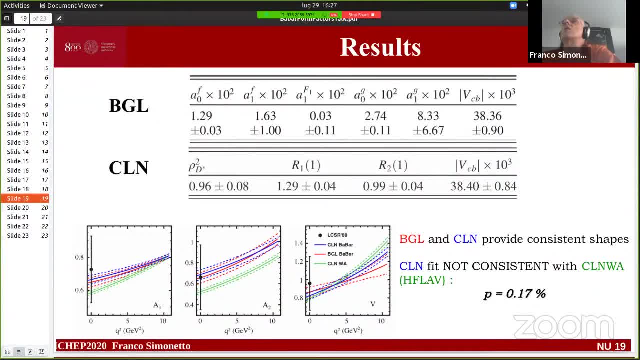 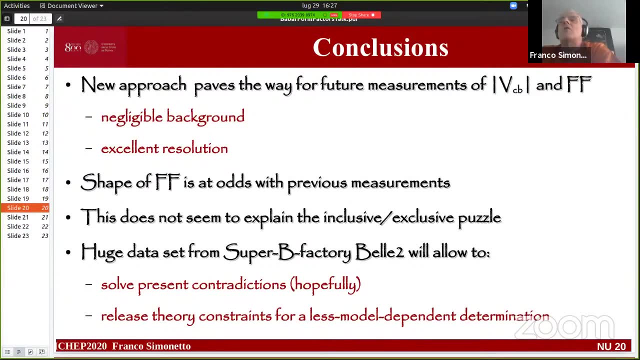 with those published by hflav, we see that the compatibility value is less than two per million. so, coming to conclusion, i have shown you a new approach to measure, to make a very old measurement nowadays, which i'm sure is paving the way for future measurement of vcb and for factor, thanks to the fact that it has negligible background. 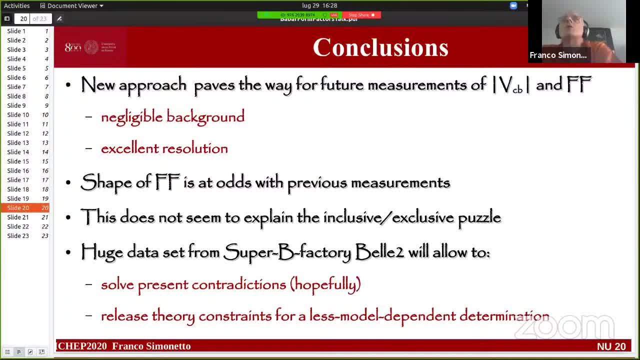 and excellent resolution. the main, most striking result of this analysis is that the shape of four factors is not consistent with what is tabled from a previous measurement, even if, apparently, this is not explaining the the difference between inclusive and exclusive results on bcb. so clearly, babar is over for this game, but we have just heard that. 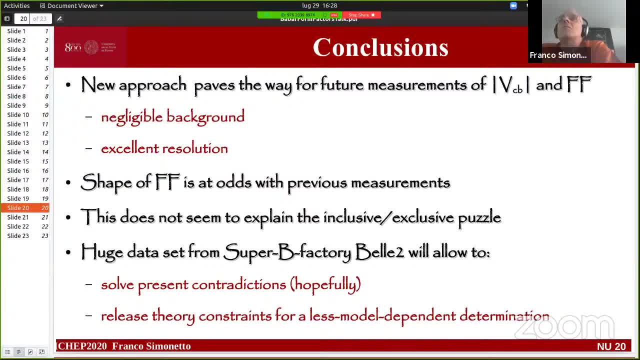 batu is entering the game, and so we can be practically confident that quite soon, if batu will apply this same technique to its, to the huge amount of data that they are going to collect, we will probably solve all present contradiction, or at least hopefully and maybe. 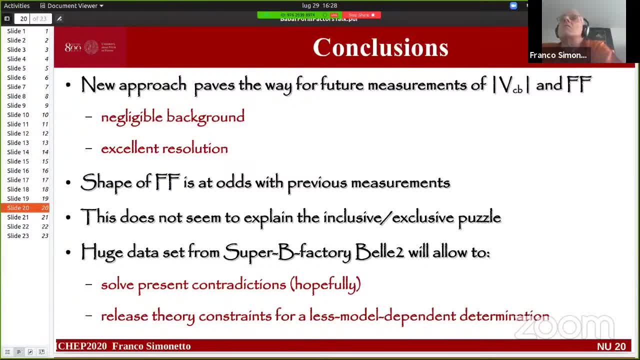 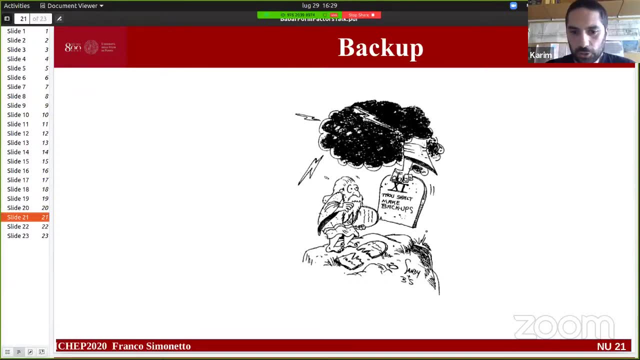 be able, or also to release theory constraint in mother in order to provide a less modern dependent determination. okay, with this, i'm over and i thank you. thank you, uh. i think we have time for one question. i see already. well, okay, i see two. if uh, let's see if uh. 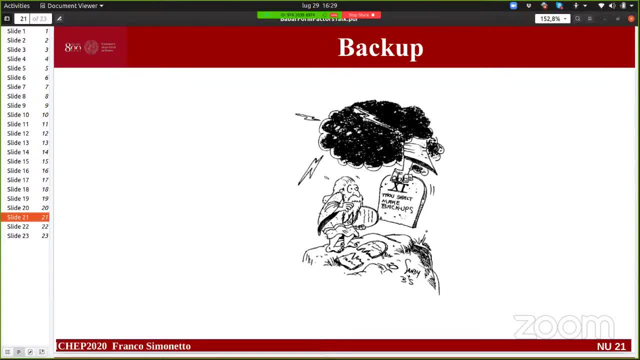 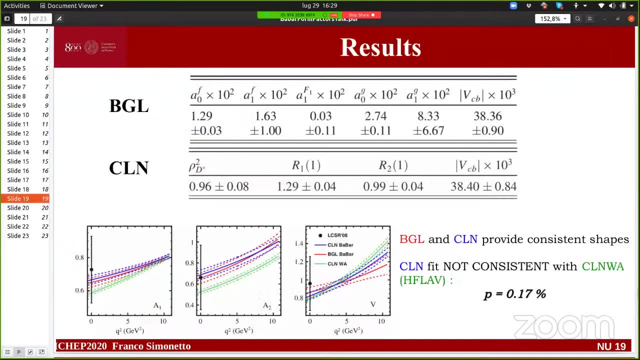 they are quick enough. so, christoph, yes, i hope it will be quick. so i'm a bit puzzled by your claim that your shape, that you measure, is not consistent with the world average, because in principle you use the world average, at least a new branching fraction, to get a value of vcb. 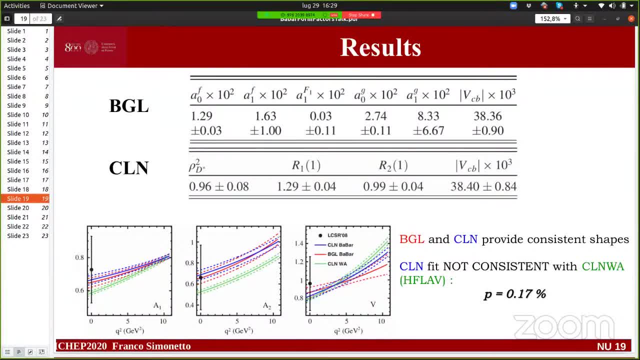 you must extrapolate to the zero recoil point and the result is consistent with the world average. so if your shape would be inconsistent with the world average, how can you get a consistent value of vcb? so that doesn't seem to well, uh, first of all. uh, you should notice that. 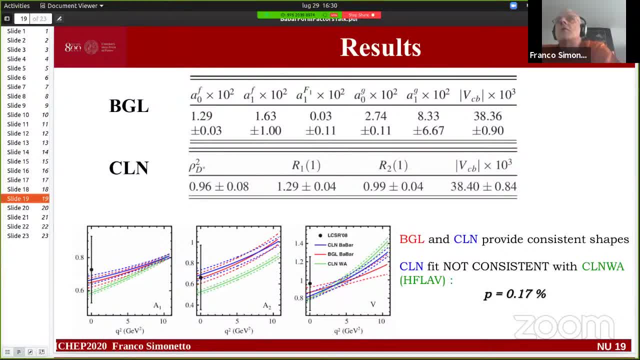 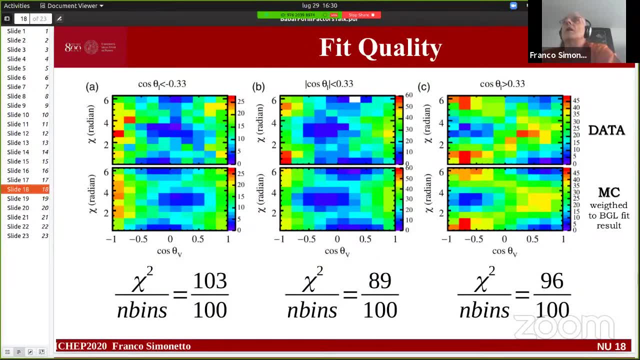 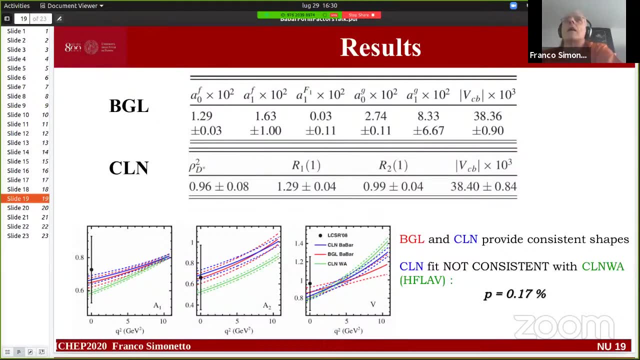 the main discrepancy is coming from one of the three form factors and you remember that one of the meters that we are fitting is the normalization of one of the form factors to the other one. if when i saw, i don't know if i have in the- uh, yeah, i already have- you can maybe appreciate. 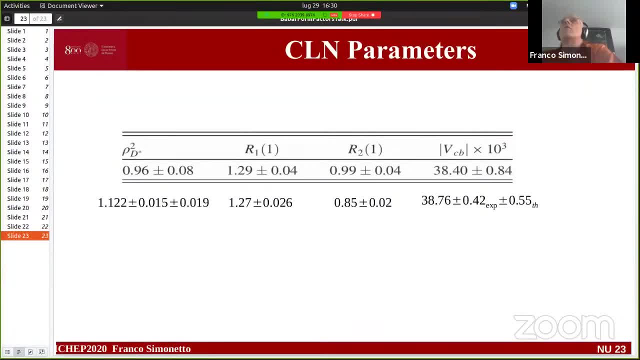 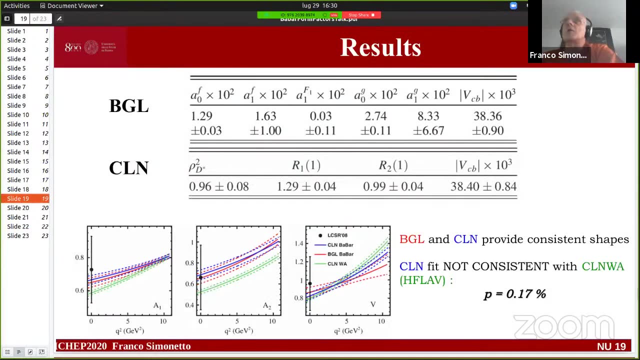 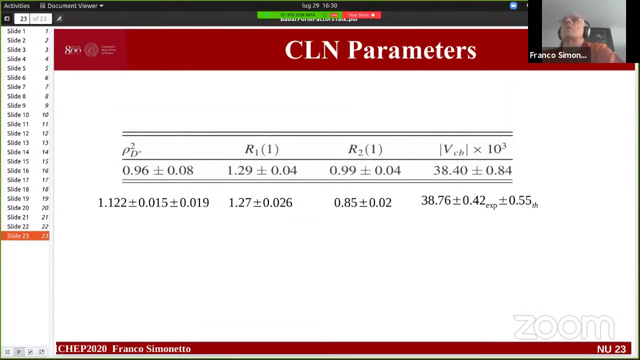 the fact that the main discrepancy we have from the world average is, in fact, on the normalization of the second uh form factor. you can also say that the slope is not very different. slopes are quite consistent, but the normalization of the second form factor is quite different. so here is that where we have the problem, apparently. however, this is you know. 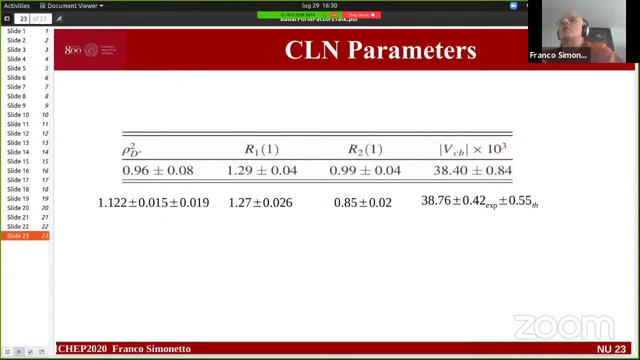 it's very difficult going from one projection to a four-dimensional adjustment. apparently this is not affecting the overall rate, but just the shape on one. just the well, the normalization of one of the compactors. okay, thanks, okay, if, if the other question is uh much faster, then i would uh also take the other. 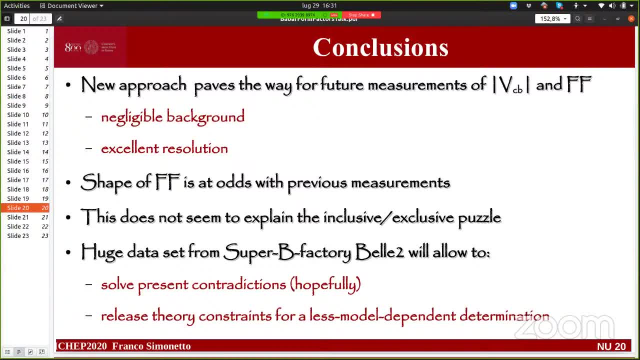 yeah, so this is uh following up essentially from from the previous question, so it can be very fast. so i i want to just to notice that the, the actual h5 combination for for this uh measurement has a pretty poor consistency as a pretty poor p value. so i wonder whether the 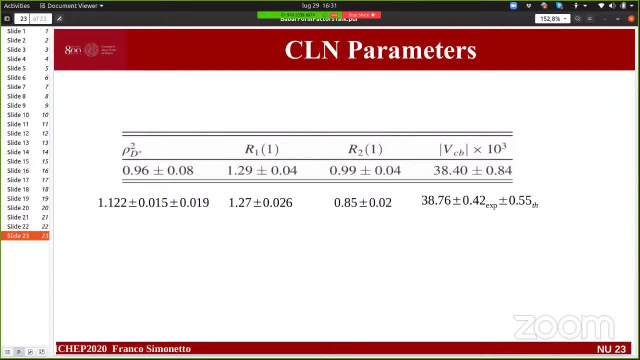 discrepancy is with any of the specific measurements that that enters the, the combination, or or i mean, if you looked into a little bit more details and not just the overall combination, but even at the individual measurements, there are a bunch of measurements by bar and bell that enter the determination of this world average. okay, of course, sorry, i. 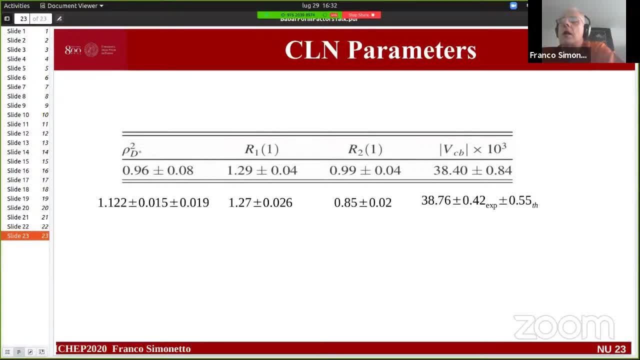 cannot answer to your question, but i take the point and we will make a comparison. i could also just go through the parameters measured by all other collaborations and let you know the answer in not a long time. okay, thanks a lot. so for any further discussion, please use the mattermost channel. now i would say we go on with the last talk before the coffee break. 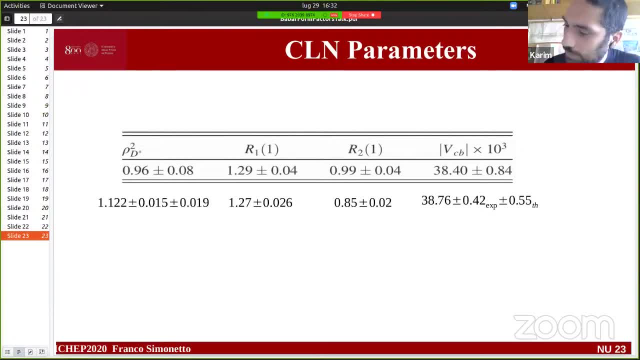 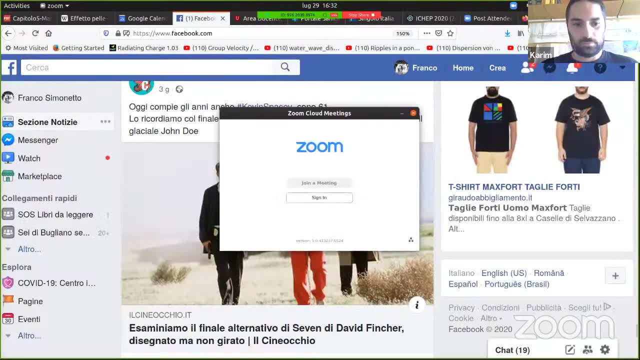 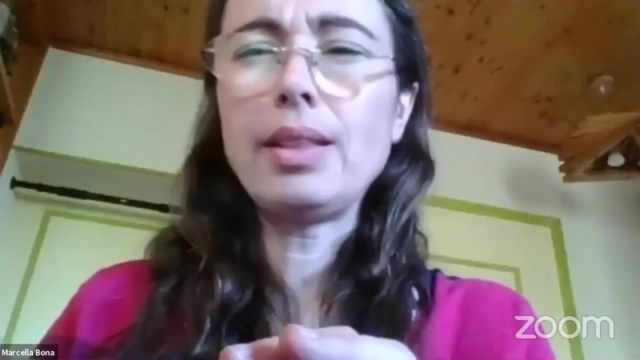 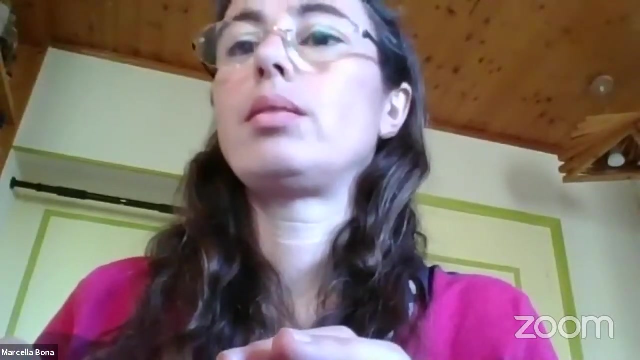 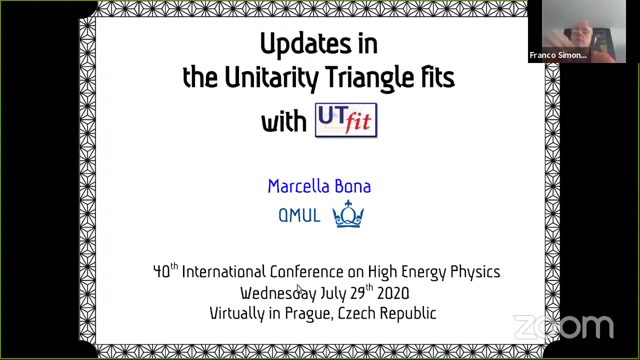 marcella bona. uh, we'll discuss about the updates on the unitary triangle by the ut fit. i need to share hello everybody, hello okay. OKAY, YOU CAN START. OKAY, SO I'LL GIVE YOU THE USUAL UPDATE ON THE ON OUR FIT WITH THE USUAL FIT COLLABORATION. 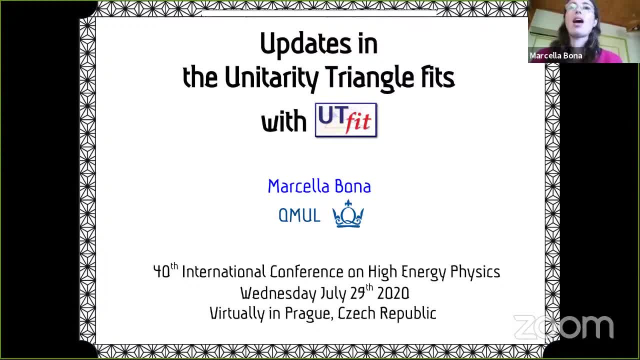 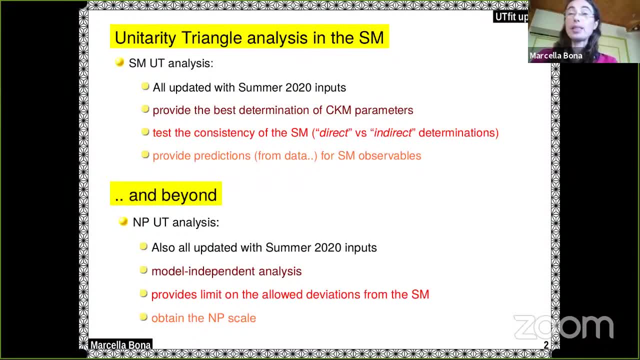 AND SO I'VE UPDATED THAT, THE ANALYSIS, WITH NEW INPUTS, SO EVERY SINGLE PLOT AND SINGLE NUMBERS UPDATED WITH WHAT I LABEL THE CALL WITH ME. RIGHT NOW IS THE CALL WITH ME thou. I'VE WENT THROUGH THE TOPIC AND THEY DIDN'T. PROPHESIS ON THE IT IS THE EXTRA PRIMARY. 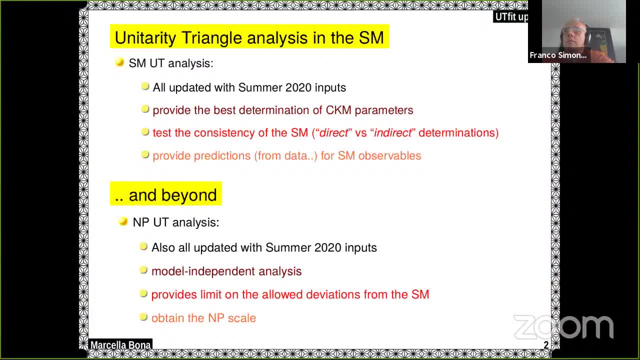 I GREW UP WITH THE SOCIAL PROCESS. Menschen sehen das andere in das aller großen. hmm der hier sind das andere101.. label: the summer of 2020 inputs and I'll go through the model analysis and the new physics analysis for with the different properties and interests. so this is just a reminder of our 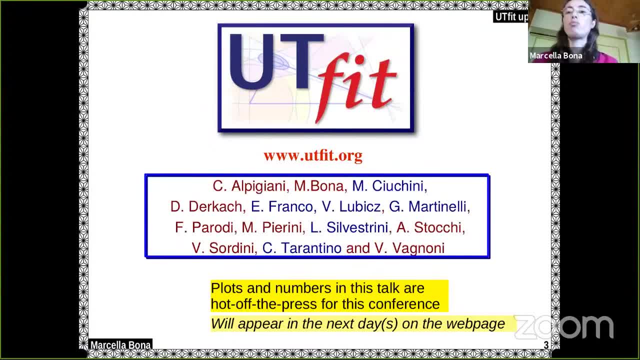 website as the plots and numbers, as I said that they are really just a hot topic for this conference, so they are not on the website yet. I expect I need to do a little bit more statistics, but in general they they will appear in the next days again. I'll just remind you what. 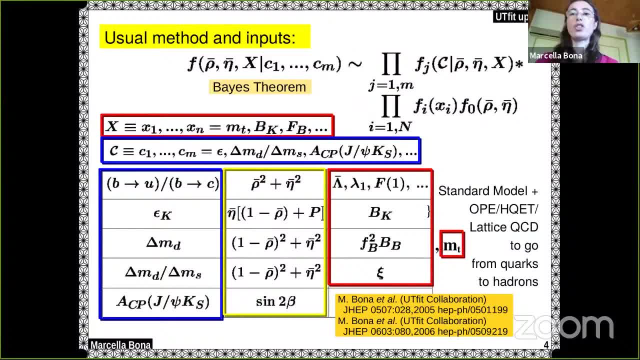 we use and we use the variation approach and we need to have the observables. so we need to have the connection there, the functional connection with the theoretical parameters, and then we need some parameters that that allows us to go from the hard-on level to the port level that we are operating at. 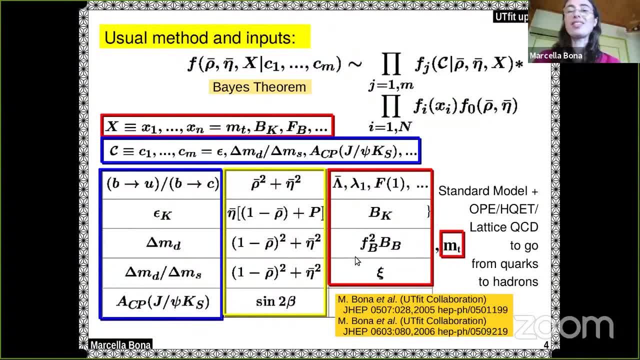 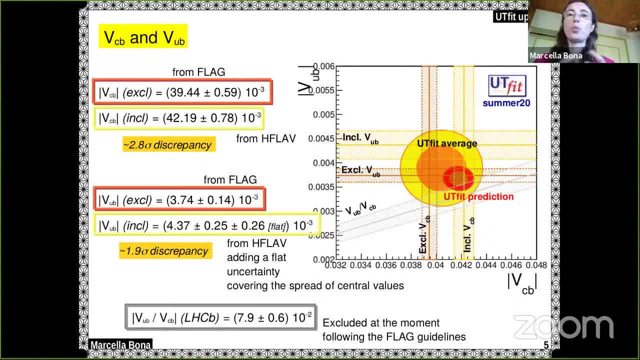 so we have heard already a lot, so that's good that I included this slide. so I have, we have our own. so, from our point of view, we try to use VECB and VUB as inputs and of course, as you know, there is a little bit of a discrepancy. so these are the latest numbers that we could cook up for a. 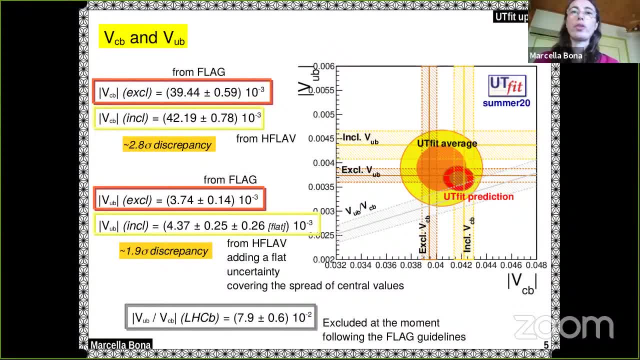 little bit. so the exclusive numbers both for from you and VUB and VECB are from flag and that was the the latest updates that we got. and then the inclusive results are from hflav. but you see that for the VUB we we noticed that there was a spread in percentile outflow. so in the case of all the 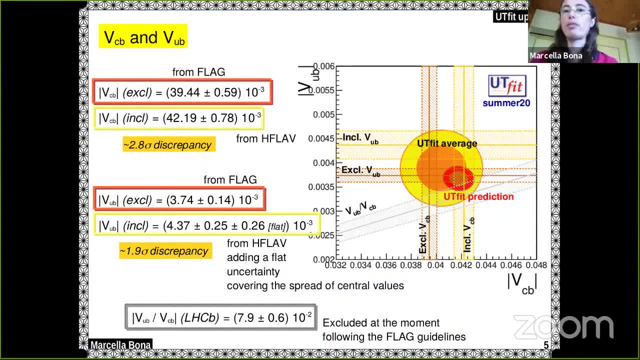 data we had, there was a trend. we had a trend of a wave of equilibrium for the entire university, so there was a trend of some sort of shift in frequency. we had a trend of a flight of the, the central values, and so we took a flat error to cover that given spread. 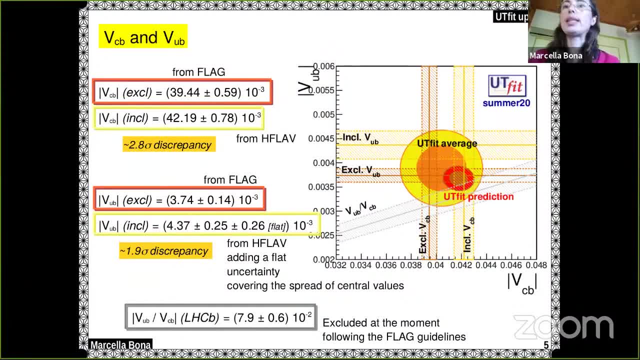 The other thing. so in the plot you see the various visualisation of these numbers and their errors. and usually we heard about LACB and their measurements of UV over VCB. We have nothing against LACB and these measurements. however, we followed the flat guidelines and 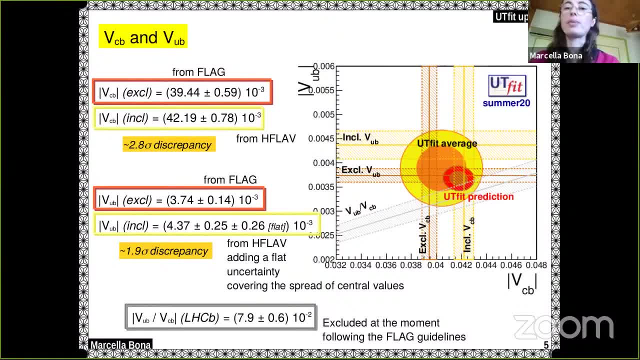 because the lattice numbers are coming from a single collaboration. they are not included in our average so, regrettably, we took it out from our average. However, what we did is also to do a PDG inflation a la PDG inflation of the averages. so you: 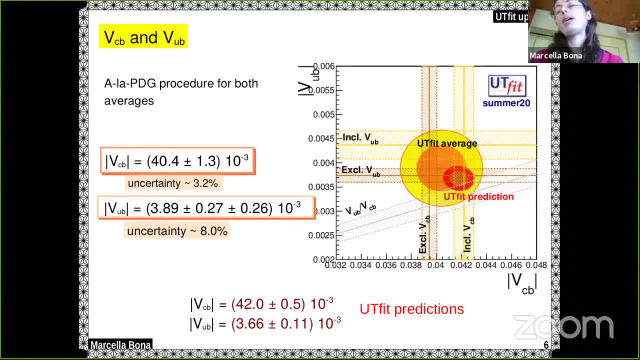 see that The blob- the orange and yellow blob- of the UCFIT average in the plot is really covering all possible intersection of the inputs and basically these are the numbers that we get with this procedure. on this page At the bottom you see also the comparison with the UCFIT prediction that I mean I call. 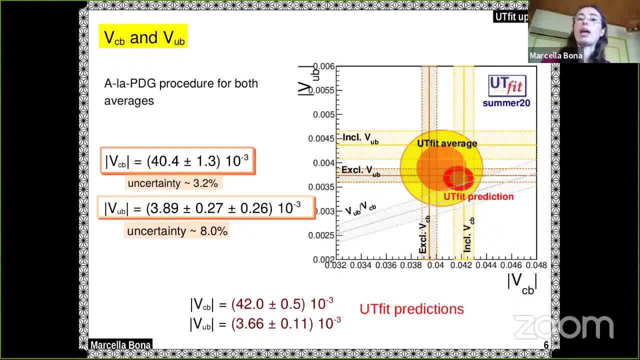 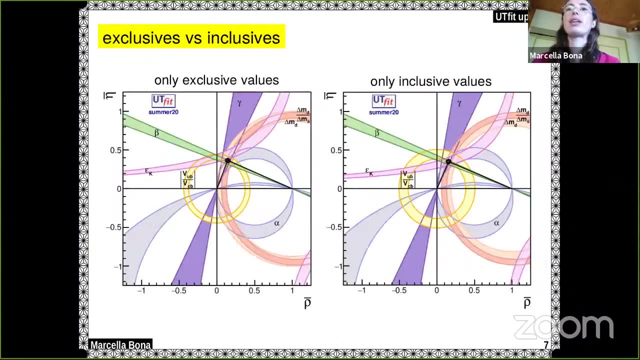 them prediction when I run my fit, and then I remove the inputs that I'm interested in looking at. So this is my fit, This is what the numbers that fit prefers, without using VCB or VUB respectively. So then the other game we do is run the full fit to separating the exclusive and inclusive. 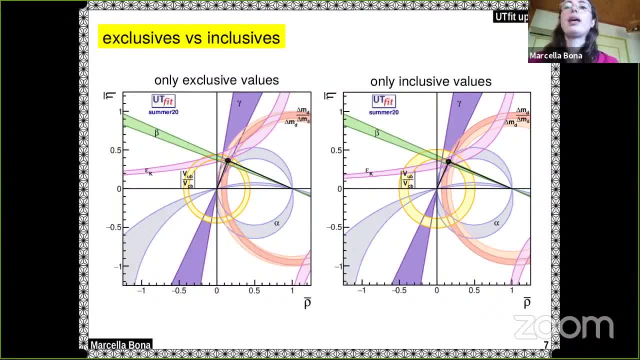 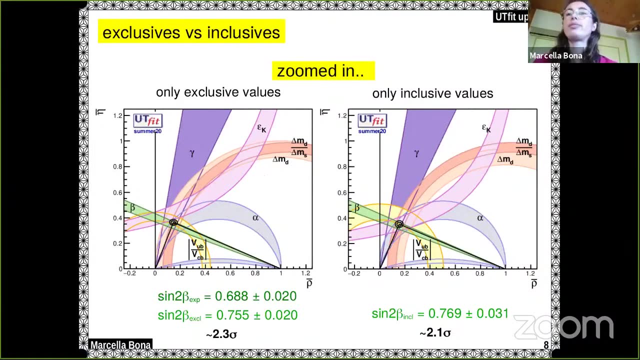 values. So I run this with VUB and VCB only exclusive on one side and only inclusive on the other side. Now the fit is becoming very precise, so I need to zoom in and then this is the zoomed in version And you see there is a little bit of confusion, especially in the exclusive part where there 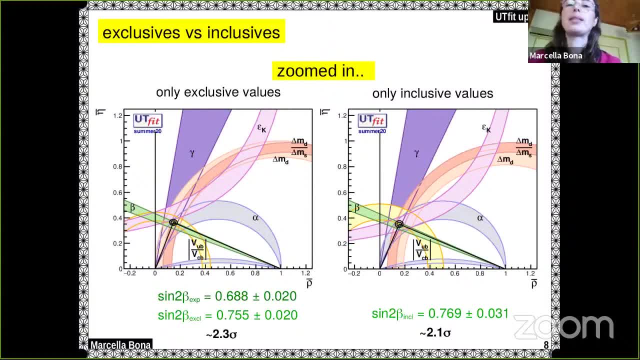 is a little bit. there are tensions, especially with epsilon k. I report here the tension that we see with sine 2 beta, which is the usual way we look at this type of tension, and that we are at the 2 and 3 sigma level. 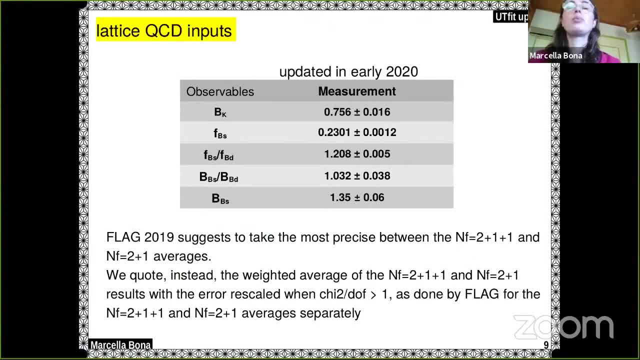 So then the other update I did with these is the lattice QTB input. So this is the QTB input. There has been some updates and also some different choices in calculating the average by our lattice colleagues. I don't have too much to say on this, just to make sure that people know what we are. 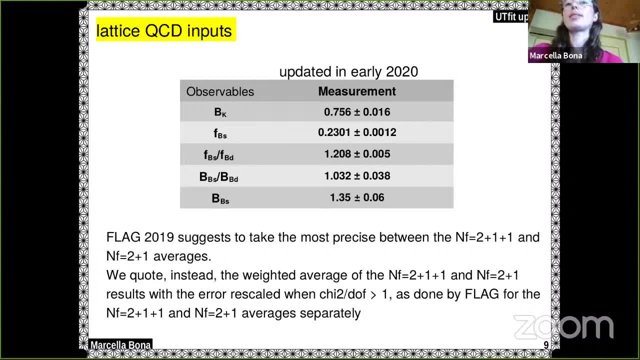 using as input. So most of the results are similar to our past update because of this different way of calculating the error. So this is the QTB input. So this is the QTB input. The error has gone down a little bit in the first three lines. so the dk, the df, the. 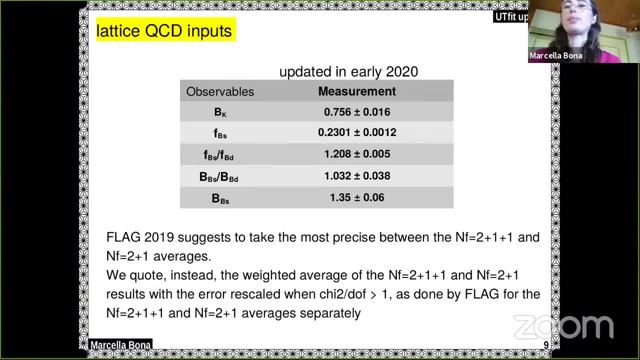 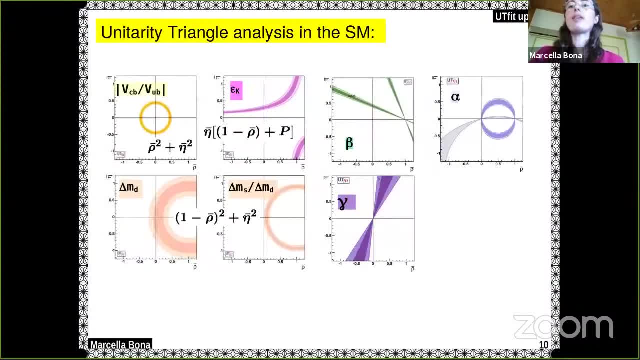 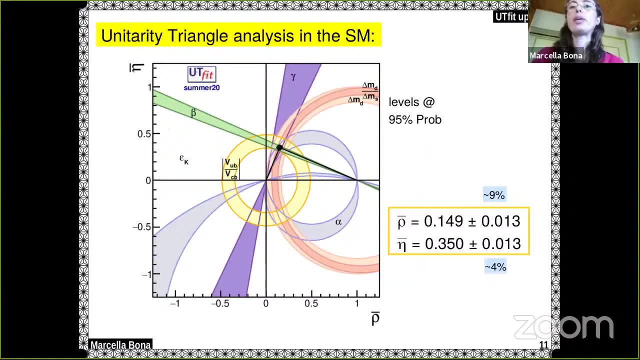 f, the bs, and then the ratio, the bs- bd. So that's a little bit to be effective with respect to our last update, And then we put everything together. This is just the summary of the main constraints And we get to the full standard model picture. 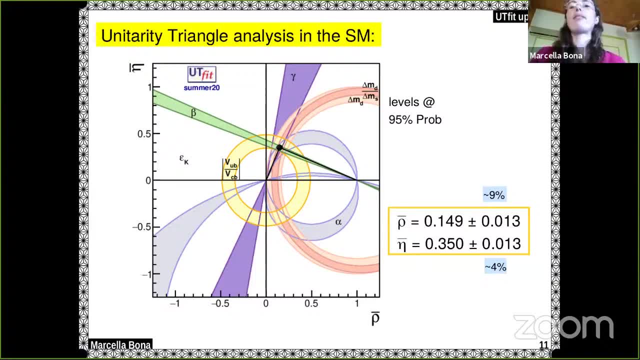 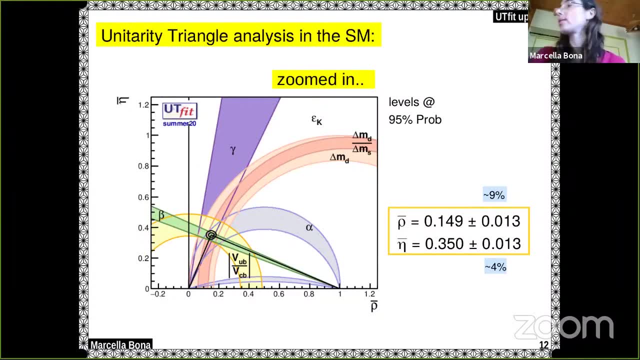 And with this number again it's getting hard to see the area. So I zoom in And this is showing quite a nice agreement And of course you can clearly see that partially this nice agreement comes from this a little bit bigger band, from the bub bcb, the yellow band that you see there. 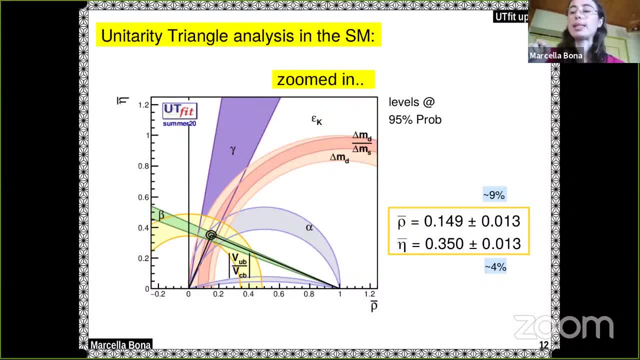 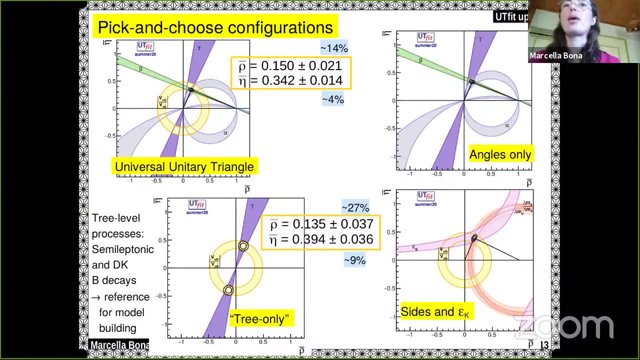 And that's clearly one effect that we can see. Now, then, what we can do: we can do several configurations, So I chose this, The plastic ones that we've been looking at, And so at the top left, you have the universal, the Duras universal, entire triangle. 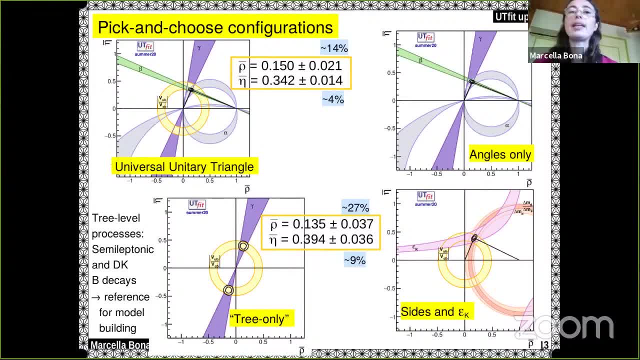 And then the bottom left are the three only caves where you only use three-level processes, so gamma and bub over bcb. And you see, there for those I also put the values for rho and etas, with a little bit increased uncertainty. 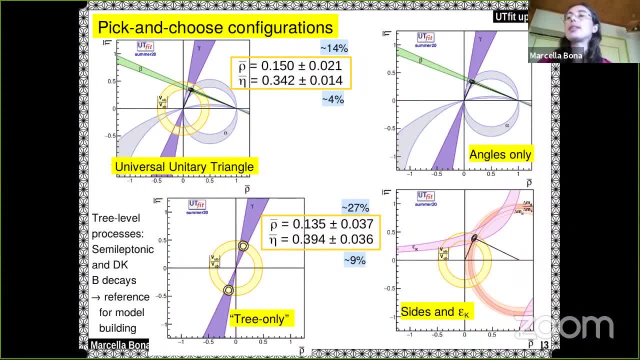 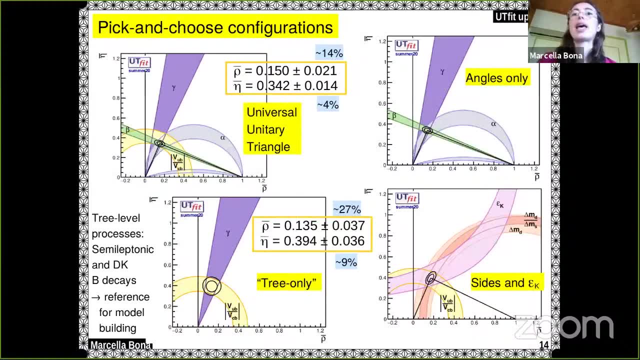 Of respect to the full fit, clearly. And then on the right, you see the case of the angles only and the size. Again, it's good to zoom in, So I do the same for this slide. You have exactly the same structure as the previous one. 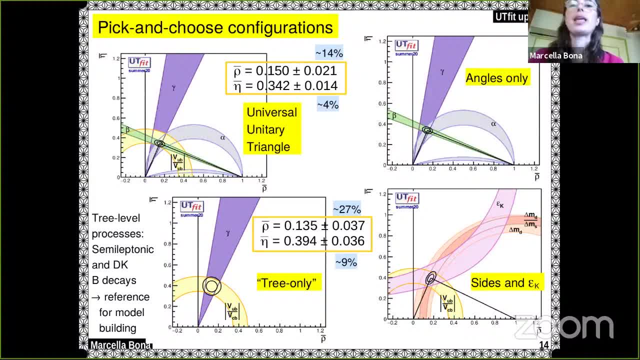 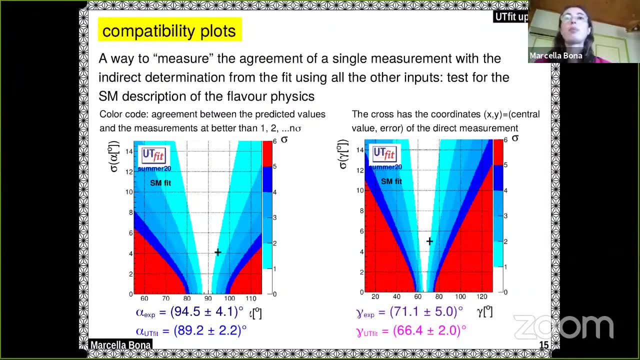 But it's just zooming so that we can actually see the area that is selected by the fit. The other way, we have to look at how the inputs are compatible with each other. Is this compatibility plot? And basically we run the fit without the observable that we're interested in. 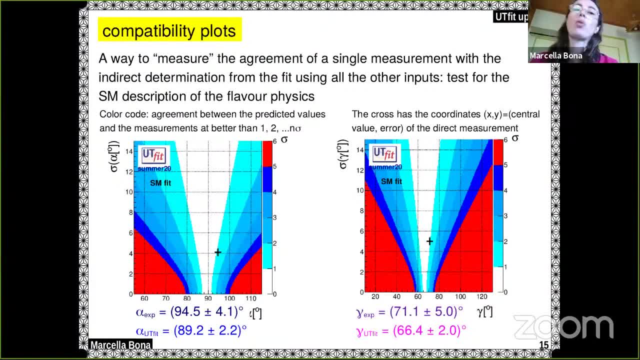 And then we plot the on a two-dimensional plane: the observable and its error, And then the experimental value that we usually use as the input. it will become just a point in this grid, And that's what you see here, And this is the case of alpha and gamma. 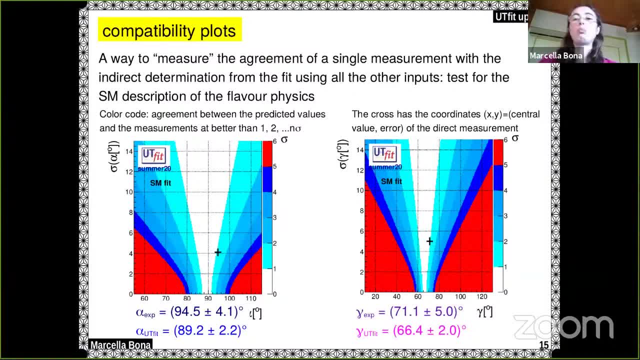 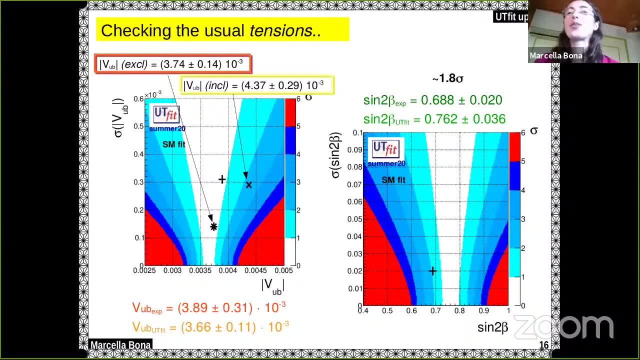 Where we have a rather good agreement at the level of 1, 1.1 sigma, If you go next, we usually then check the usual tension that we expect in a way. And so there is the UV, as I've already mentioned several times. 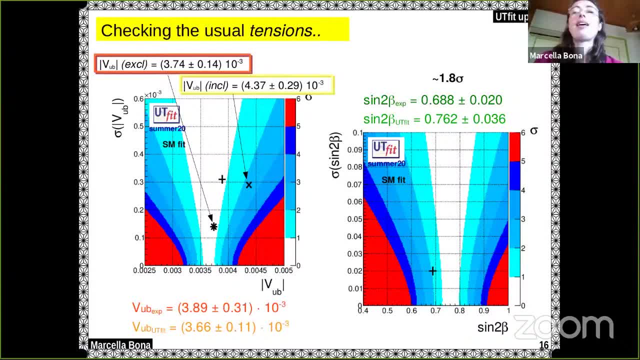 Here you have the cross. Here is the input value that we use And, as I already mentioned, it has an inflated error. So you have no tension there. But then if you split into the exclusive or inclusive values, you see that the inclusive is the one that's less agree with the rest of the fit, as we already know. 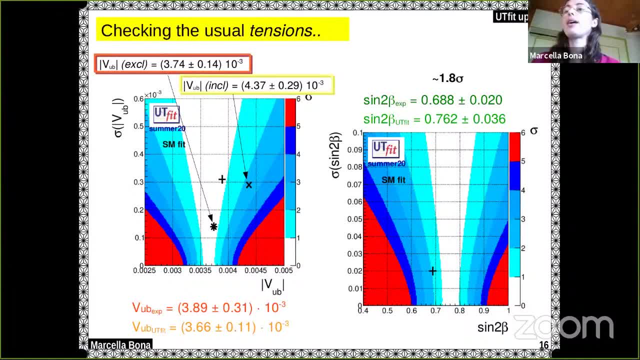 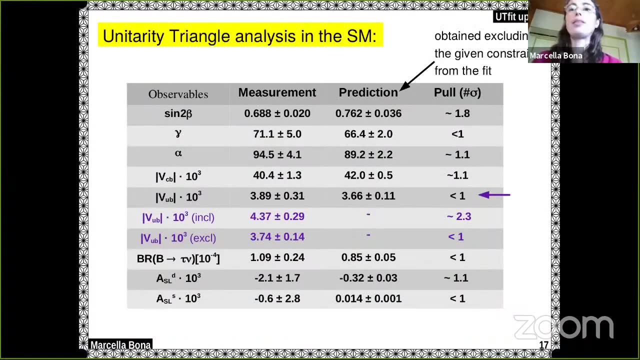 On the right, you have the sine 2 beta And again we have a 1.8 effect, Sigma effects of tension with the fit. This slide shows a summary of all this And you have again the measurements of the inputs that we use and also the prediction that comes from the fit without using the given input. 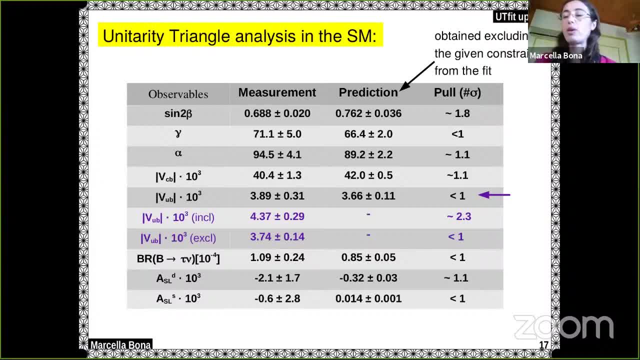 And then the last one. the sigma of agreement is somewhat, And then again you have the error. It's not matching. But anyway, you see that 2.3 from the UV inclusive and then the 1.8 of sine 2 beta are the main highlights here. 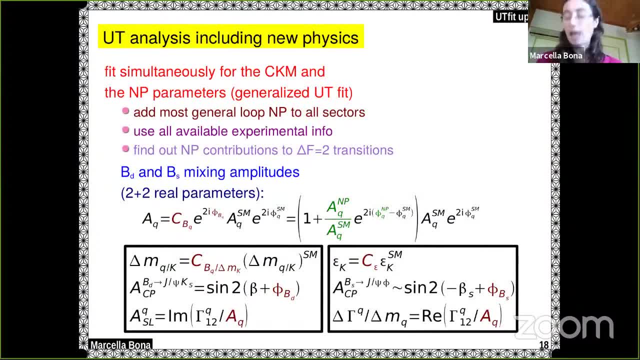 Then the other things that we can do. we can revert our fit- Not really reverse, Just add extra observable- And basically saying, because we have, we are over constraining at the moment, because we have a distance amount of constraints, We can even push it a little bit more and add extra constraints. 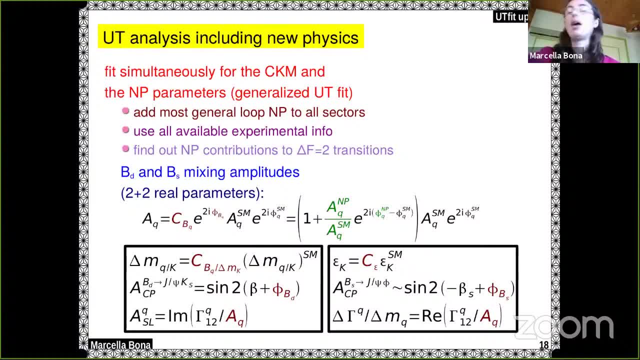 That represents new physics Spaces. So, for example, we can imagine to have an amplitude from new physics and a phase coming from new physics, And that's the most generic characterization. And that means, though, that you need to reinterpret your observable in line with this extra amplitude and phase. 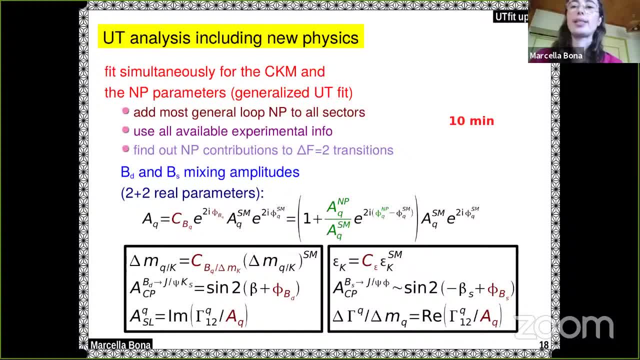 And you see how we reinterpret the standard constraints At the bottom of the page. And then we can look at this- The new physics parameters- two ways: Either as a multiplicative Factor to the amplitude, Or you can also look at the ratio between the new physics over the standard model. 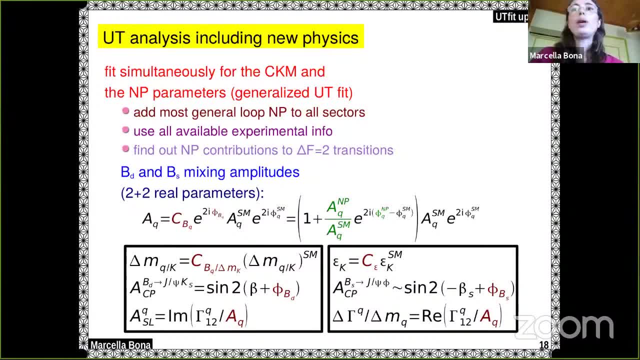 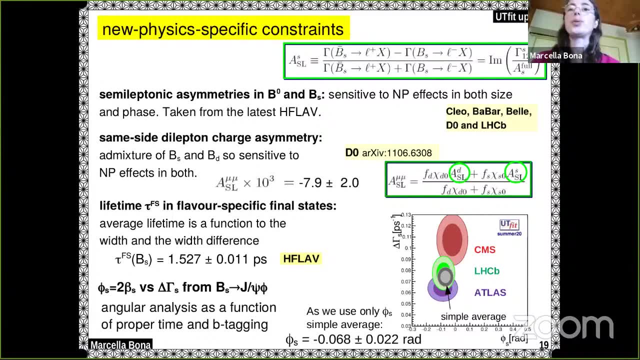 Amplitude. So To do this We are also helped by new Other other constraints that are not particularly using the useful in the standard model one, but they are useful to To constrain Also the best sector and also to have the constraints that act on both the size and the phase of the new physics that we implemented. 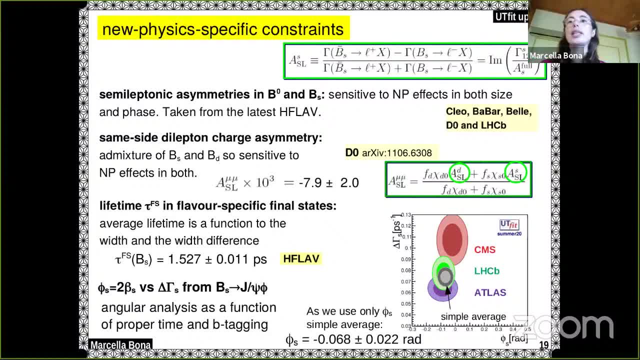 And so this is typical. For example, the semi-electronic asymmetries are giving you this kind of constraints. At the bottom of the page I mentioned five, So now We used to. We had different types of inputs, But at the moment, 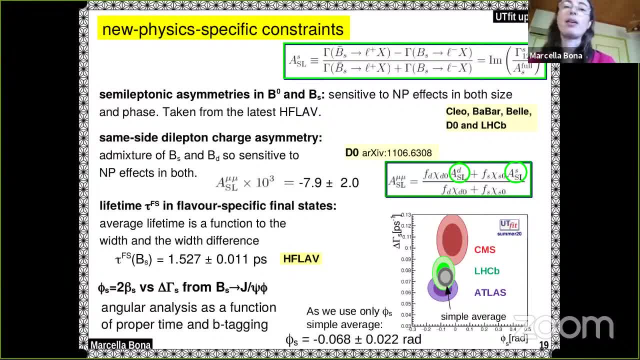 For our Analysis We use the only five Yes And so not. We don't use Also Delta gamma At the moment, And so, basically, I We did A Utility With The current Situation. 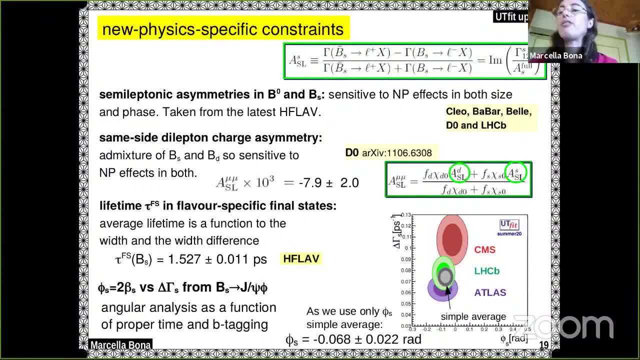 And if you Project On the wall On the exact This, So you Look at From the point of view of Yes, The Measurements Are not Particularly In Tension And so we can do. 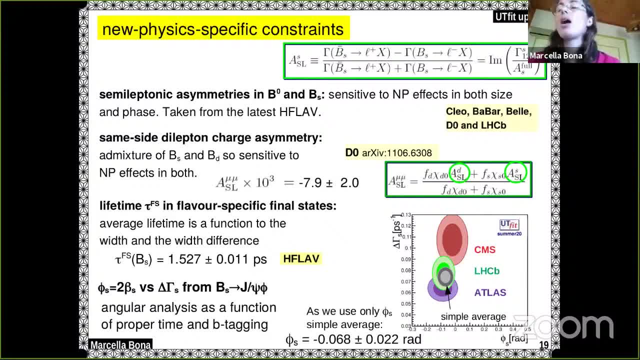 What Simple average, Which is the The Blade blob They have there. Of course, If you want to use Delta gamma, So then You need to think A little bit About it, And that's what We're going to do. 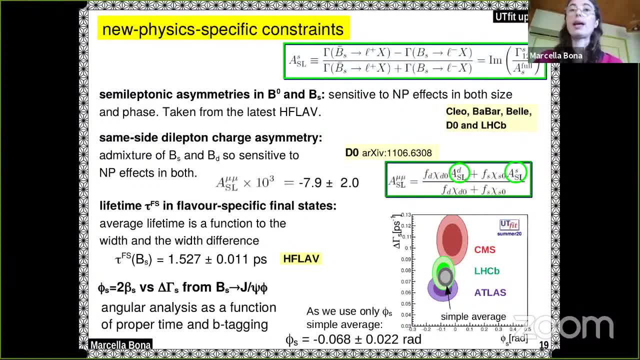 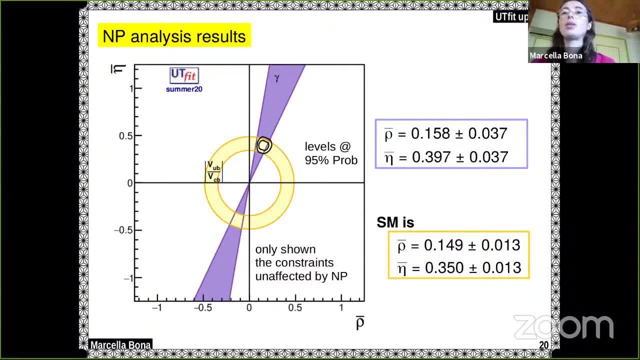 In the next Month, Because clearly There is Some. So If Then We Run The New Physics Analysis And The Fit And We Get Out So The Usual, 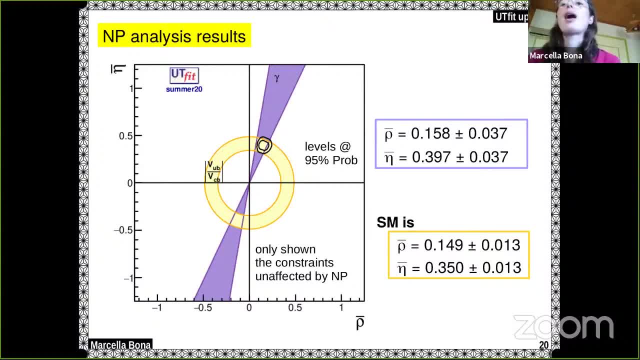 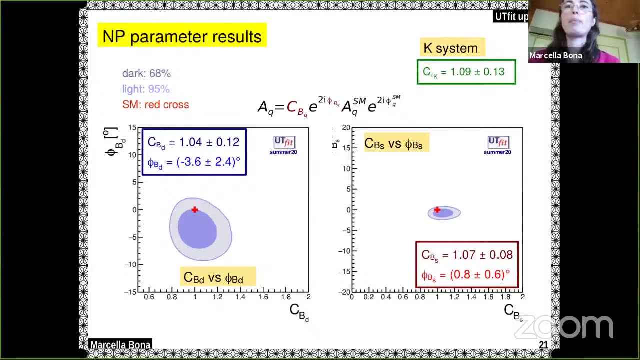 Role And Eta Values. And This Is The Role. It's A Part Of The New Physics Parameters, As I Implemented Them, And Here You Have. 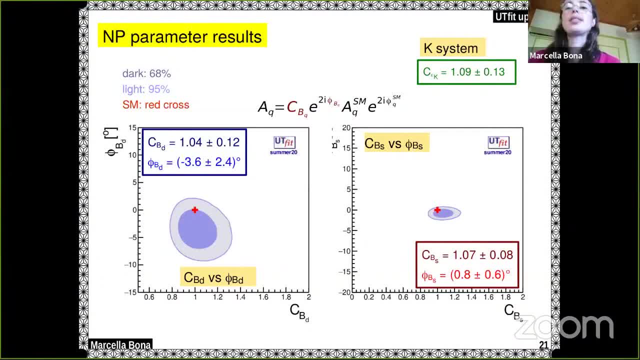 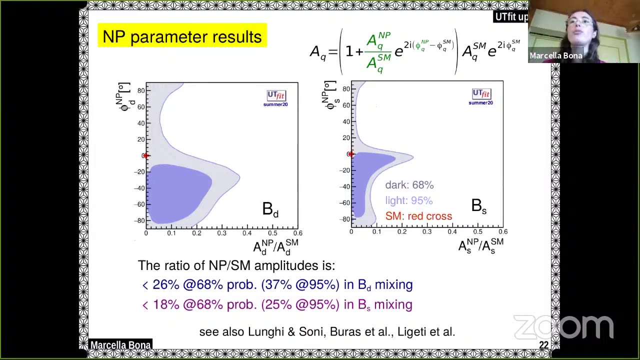 The On The Left Side Of The Subject System, And Then You See That To The Phase Is Not Too Much In The Amplitude Another. 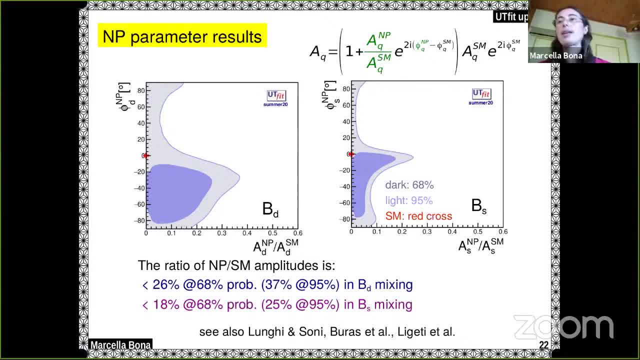 Way To Look At This And Is That Judging The Amount Of Physics Amplitude Still Available With Respect To The Errors Are Reducing So 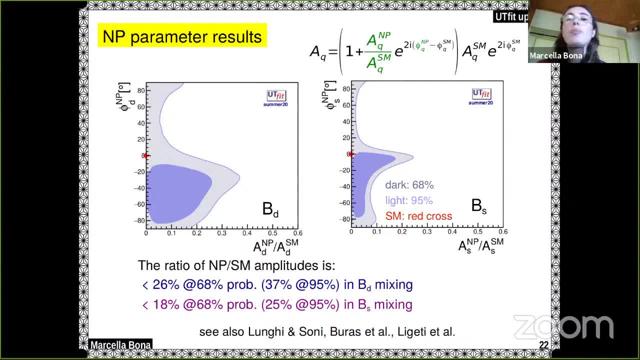 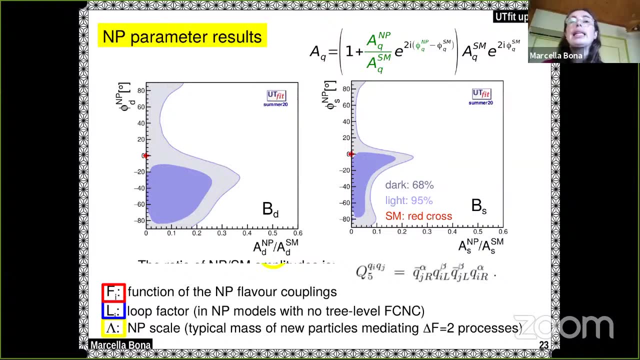 It Becomes Quite Constraining Of Your New Physics Space, But Still You Still Have 25. 35% Of Of New Physics- That Is Still Possible. 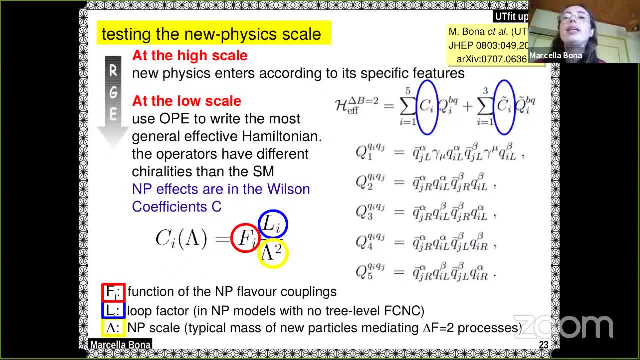 In The Space. That Has To Be A Very Important In The Space And That Is A Very Important In The Space And That Is A 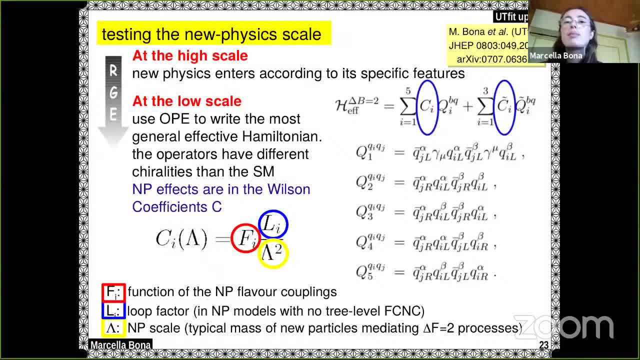 Very Important For The Space Is Coming From The Flavor Coupling Of New Physics, A Loop Factor. That Is The How The New Physics Couples. 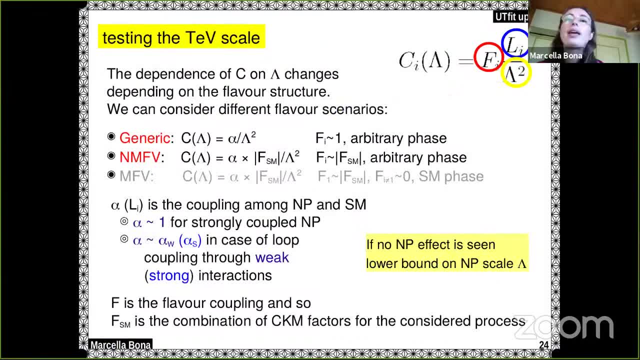 With The Standard Model And Then The Lambda, Which Is A Different Assumption In Different Scenarios. You Can Extract A Constraint On Lambda, And That's. 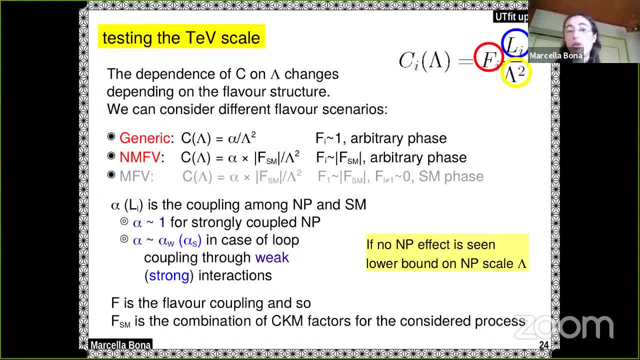 What We Want To Do. If You Don't Have New Physics Effect, You Have A Standard Model. Now The Default We Take Is As One. 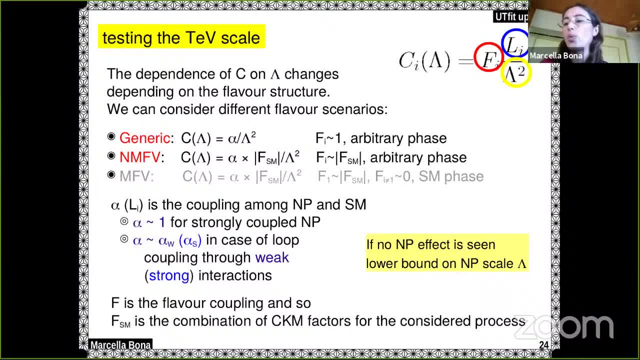 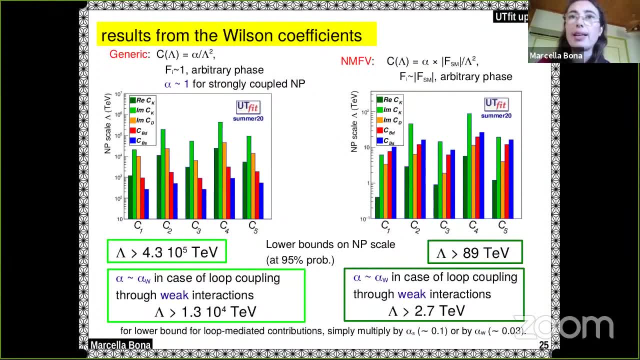 So A Strongly Coupled New Physics System Model, Although It's Realistic. But It's Not Important, Because Whatever Stronger One This Is Usually And 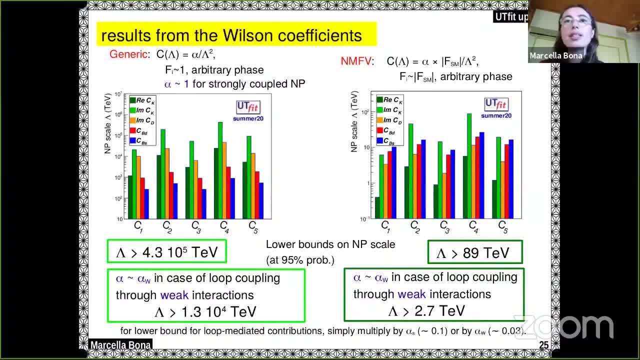 It's Okay The Case With This Results: On The Left You Have The Generic Scenario Where You Have A Generic Flavor Structure On The For. 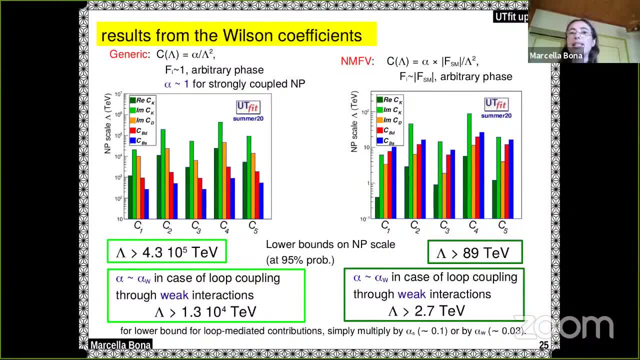 As The People At Four Point Three Tends To Be By: TV For The Generic Case And 89. TV For The Next, Next Immune. 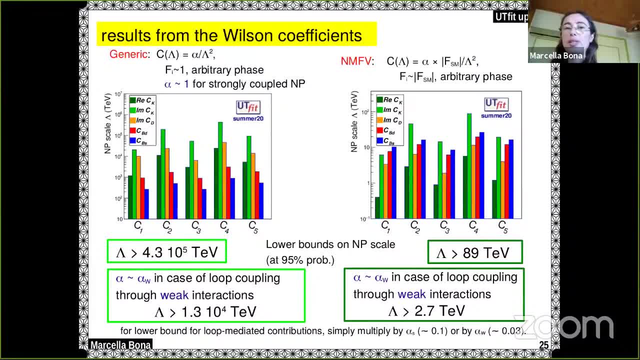 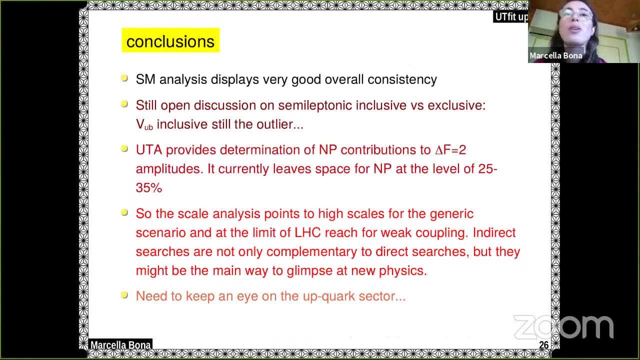 Flavor Variation Case In That, Something That, For Example, In The Next Meaning Of Flavor, Flavor Violation Scenario, Is That Getting Us Closer To The? 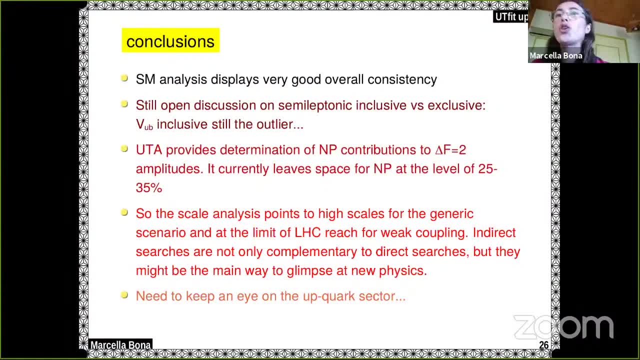 Lhc Rich. So To Conclude, This Is The, The Inclusive That Is So Like Liar. We Showed Also The Business Contribution. That Still. 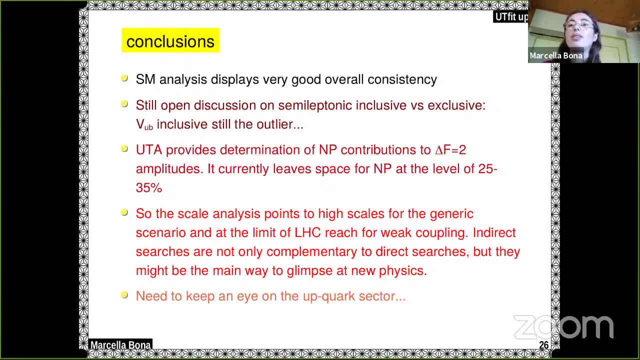 Allowed The Current Precision Of The Fit And Then The Scale Analysis That Shows Once We're Looking, And Of Course I Talk So Only About. 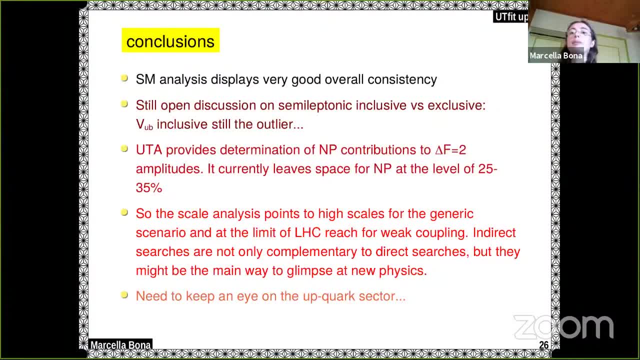 Bottom Quarks. But But There's, There's Still An Eye To Be Kept On The Work. Thank You Very Much. Thanks, Hi, Very Nice Talk. 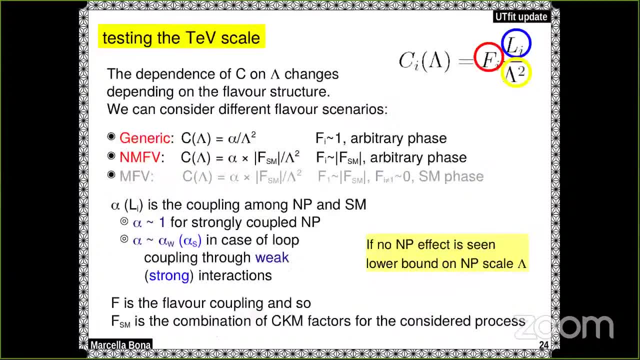 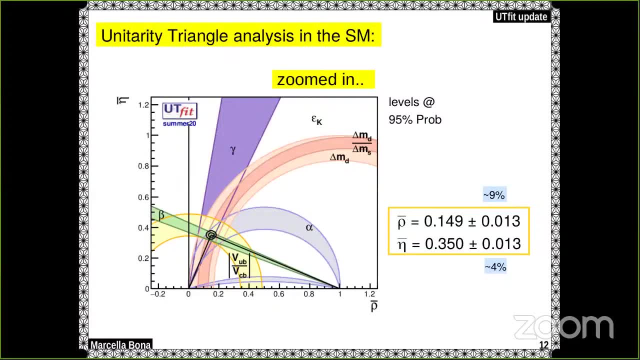 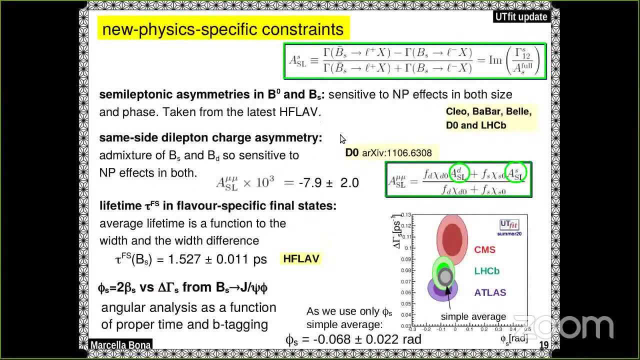 Marcella On Slide 12. In The Standard Model Fit I Thought You Had A Value For ASl Of Point Three, Two Plus And Minus. 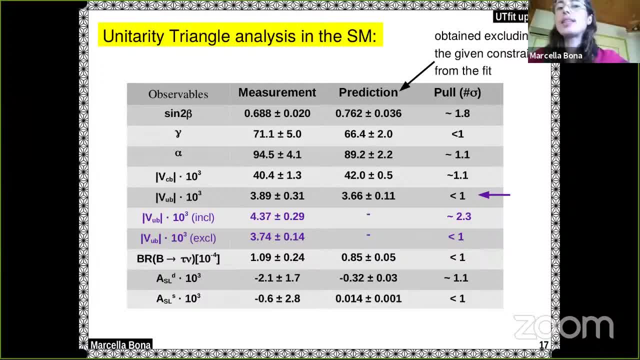 Point Oh Three. This Is The. So This Is The Experimental Measurement That We Have. No, The Measurement Is Input. Your Measurement Is Minus 2.1.. 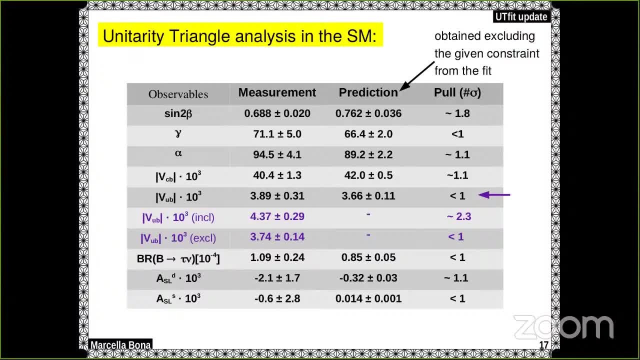 Plus Or Minus 1.7.. Your Fit Is The Standard Model Physics Here. If We Were To Believe This, I Can Check I Might Have. 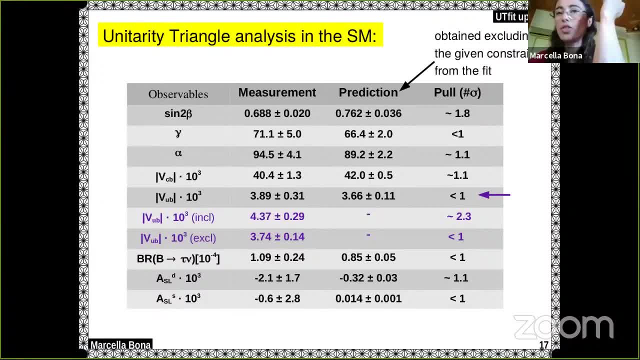 Done This One Late At Month, But It's True. I Just I Don't Know If That's What You're, What You Predict, Which Is What. 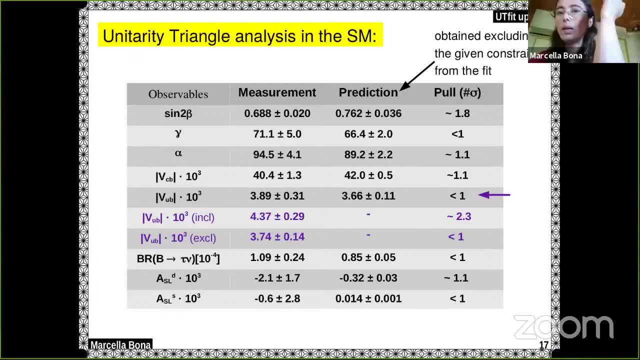 Means That You're Getting Out Of All The Data And The Prediction Is 10. Times Smaller Than Your Prediction. From Your Prediction, Okay, I. 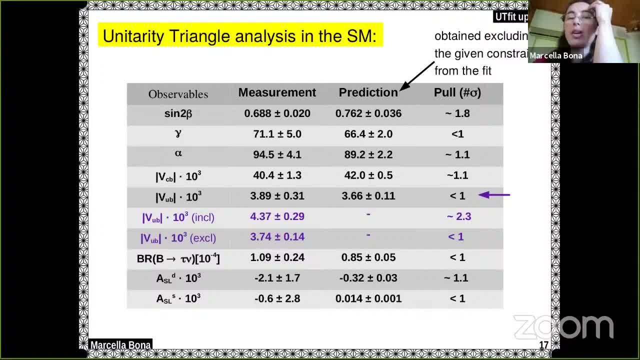 Mean The. I'm Not Super Excellent On Asymmetry, But If You're Saying That The Prediction Is In Line What We're Seeing from your overall fit, which okay, but but if it's within the error, it means simply that 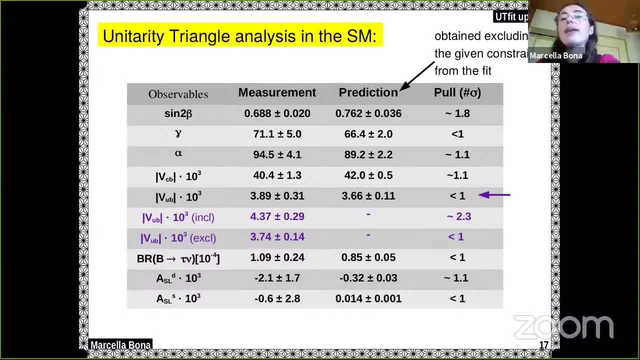 it's not within the error, okay, okay, i'll check that then. okay, now understood, took me a while. okay, you're in sigma above, yeah, yeah, yeah, okay, i'll check that. um, i might i have done a miscalculation of the error. excuse me, but isn't this number multiplied by 10 to the 3? 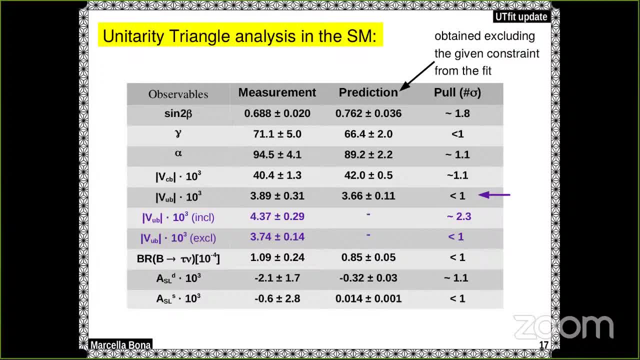 so, so in fact, the 10 to the minus 4 is 3.2. 10 to the minus 4. that explains it, thank you, oh, okay, okay, oh, i see, yes, yeah, yeah, it's 10 to the minus. that would definitely explain it, okay, sorry. 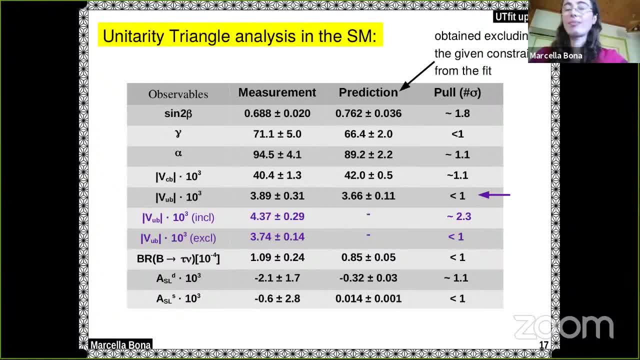 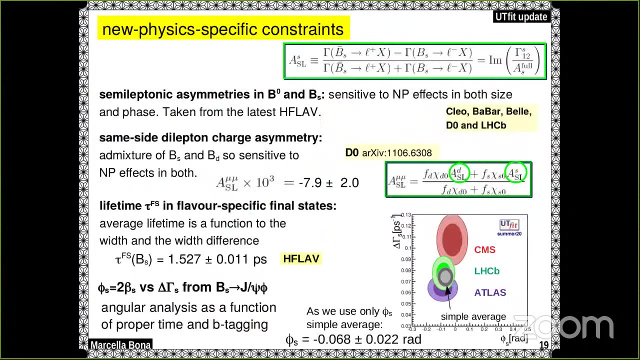 okay, okay, i think we we have uh time for one last question. i see there was already uh dory scheme who wanted to to ask something. yeah, uh, can you go to page number 19? hello, yes, i'm in my, in my view, i'm on page 19. okay, you have to go three, three more pages. 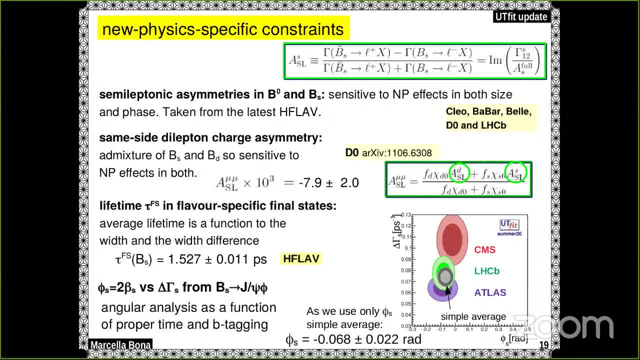 you have to go three, three more pages. yeah, there, uh. here you are showing uh the flat of uh. yeah, there, uh. here you are showing uh the flat of uh. yeah, there, uh. here you are showing uh the flat of uh psi s and gamma. uh, i heard that, all three. 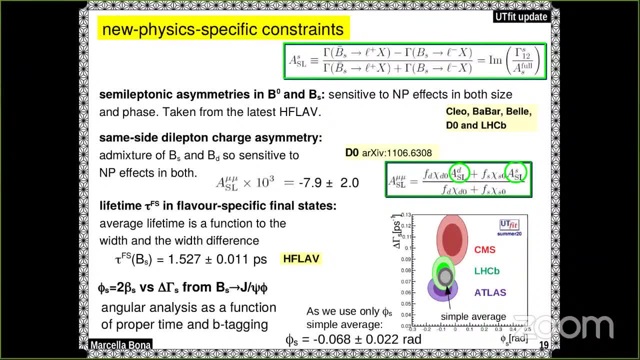 psi s and gamma. uh, i heard that all three psi s and gamma. uh, i heard that all three experiments updated their numbers during july. experiments updated their numbers during july. experiments updated their numbers during july. so i was wondering which version of numbers you. so i was wondering which version of numbers you 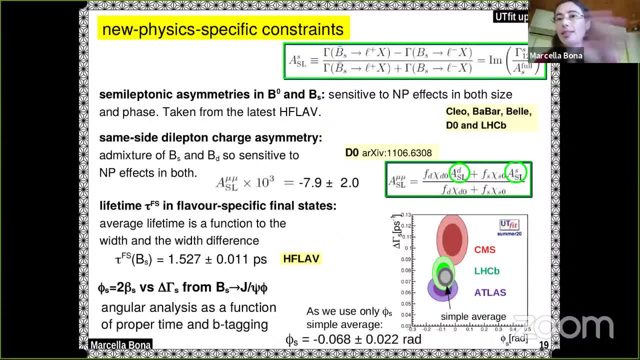 so i was wondering which version of numbers you are using, are using. are using so this idea this sunday, so it should be so. this idea this sunday, so it should be so. this idea this sunday, so it should be the latest one for all the three of them. 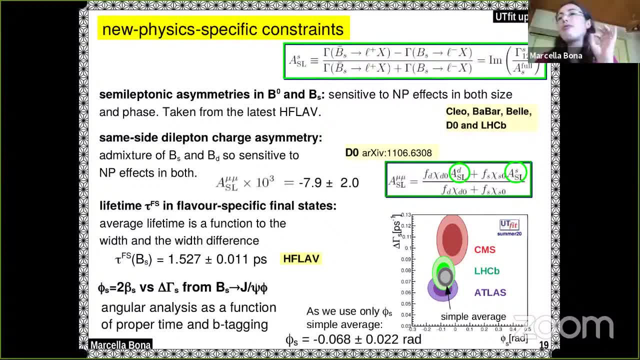 the latest one for all the three of them. the latest one for all the three of them, because, yeah, i see i wouldn't put my hand, because, yeah, i see i wouldn't put my hand because, yeah, i see i wouldn't put my hand on the on fire, on the fire, because i 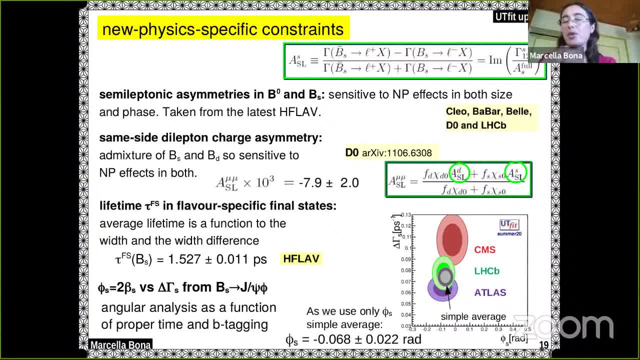 on the on fire on the fire, because i on the on fire on the fire because i really like um it. it's complicated to really like um it. it's complicated to really like um it. it's complicated to uh, disentangle some, some of the of the. 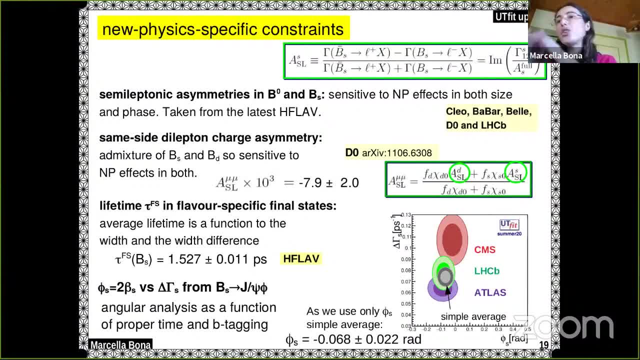 uh. disentangle some some of the of the uh. disentangle some some of the of the numbers, but numbers, but numbers. but what i did, i this don't don't use this. what i did, i this don't don't use this. what i did, i this don't don't use this one. this is really just. 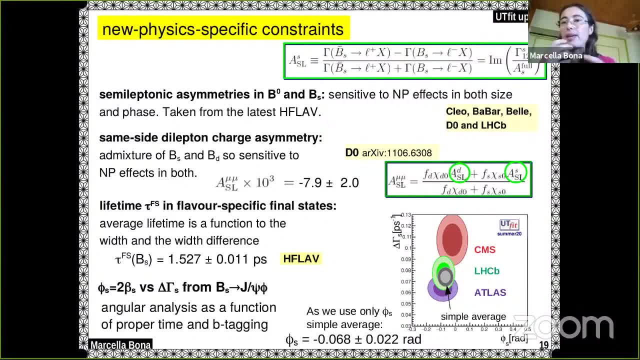 one, this is really just one, this is really just me- to help me visualize and help me me to help me visualize and help me me to help me visualize and help me make the average and then compare with make the average, and then compare with make the average and then compare with some other average. 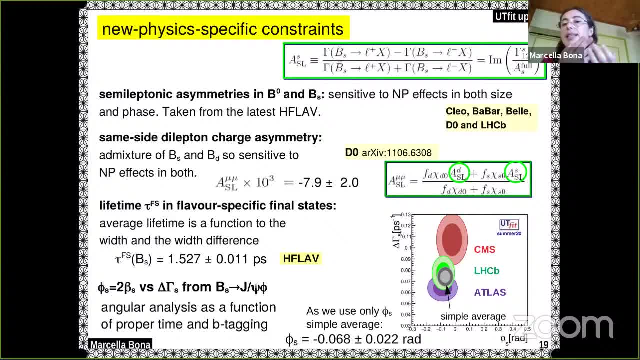 some other average, some other average, uh. then i decided that i mean the the lac uh. then i decided that i mean the the lac uh. then i decided that i mean the. the lac uh uh group is working on on averaging. uh uh group is working on on averaging. 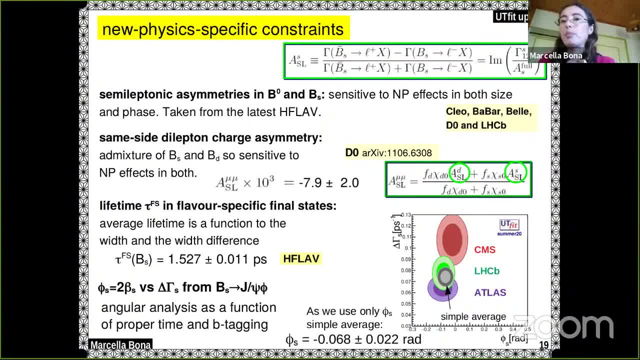 uh uh group is working on on averaging that and so that they will at some point that and so that they will at some point that and so that they will at some point they will be um talking seriously about, they will be um talking seriously about. they will be um talking seriously about this, as we are only using fias. 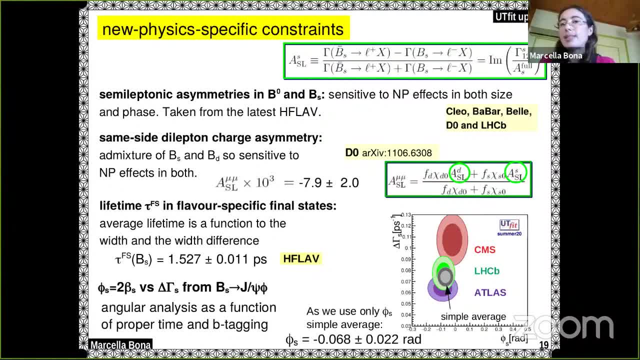 this, as we are only using fias. this as we are only using fias, even with uh a pdg inflation, i guess, even with uh a pdg inflation, i guess, even with uh a pdg inflation, i guess i still get this. so there's no, there's. 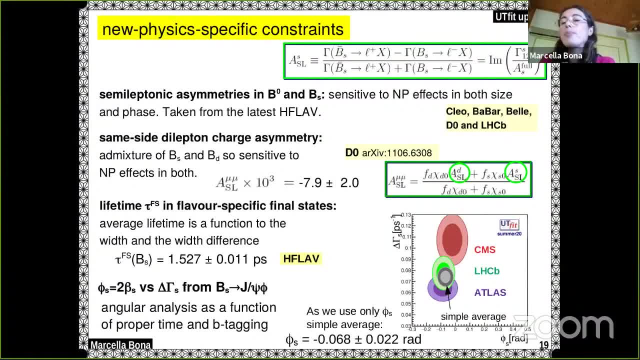 i still get this, so there's. no, there's. i still get this, so there's. no, there's no difference, no difference, no difference. but clearly there is there is an issue, but clearly there is, there is an issue, but clearly there is there is an issue at. yeah, i think, i think um. 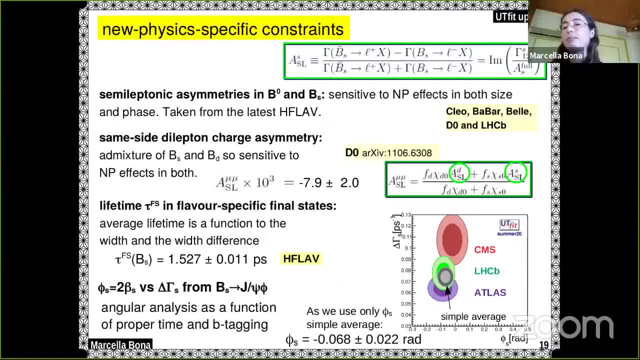 at yeah, i think i think um, at yeah, i think i think um, yeah, i'm not sure about lacb because that, yeah, i'm not sure about lacb because that, yeah, i'm not sure about lacb because that lcb, lcb, lcb published an update on. 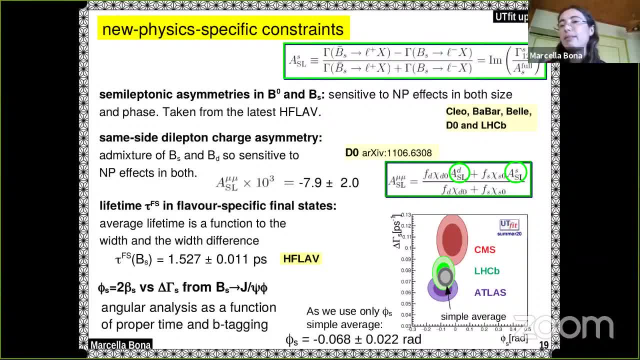 published an update on. published an update on recently, and i'm not sure if i if i'm recently, and i'm not sure if i if i'm recently and i'm not sure if i if i'm using this one, so i haven't um using this one, so i haven't um checked, but i can easily check and yeah. 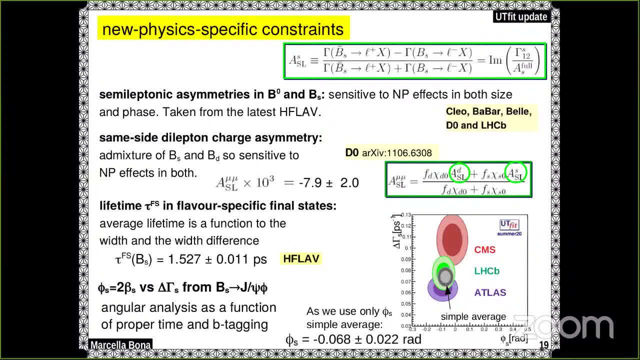 checked, but i can easily check. and yeah, checked, but i can easily check. and yeah, yeah, i i sent you an email. i think, yeah, i i sent you an email. i think, yeah, i, i sent you an email, i think. atlas, atlas, atlas to their number a couple of days ago. 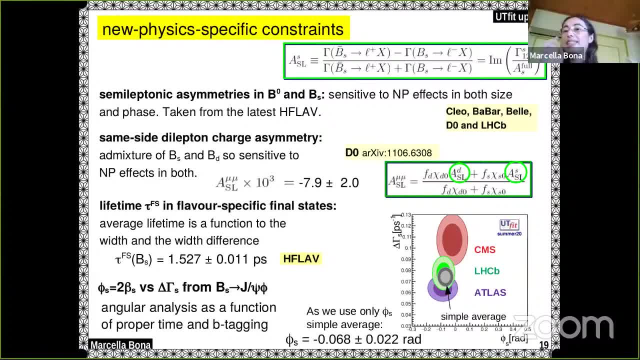 to their number a couple of days ago. to their number a couple of days ago. yeah so atlas of course, because i'm yeah, so atlas of course, because i'm yeah, so atlas of course, because i'm also in atlas. but i didn't do that with also in atlas, but i didn't do that with. 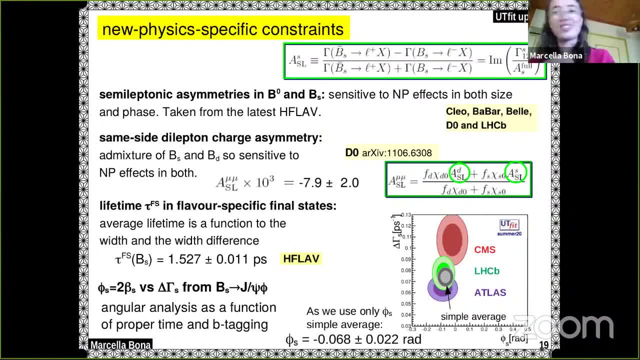 also in atlas. but i didn't do that with any atlas information. i just uh any atlas information. i just uh any atlas information. i just uh use public numbers just to be sure. oh, i use public numbers just to be sure. oh, i use public numbers just to be sure. oh, i see. 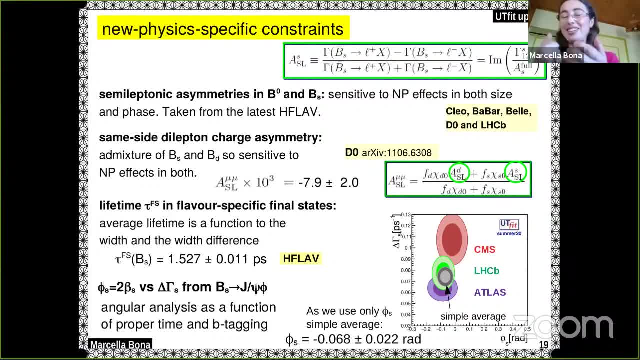 see, see, so i know that atlas updated, so i, i, so i know that atlas updated, so i, i, so i know that atlas updated, so i, i, because i, i, i knew the updates, i updated, because i, i, i knew the updates, i updated, because i, i, i knew the updates, i updated numbers. 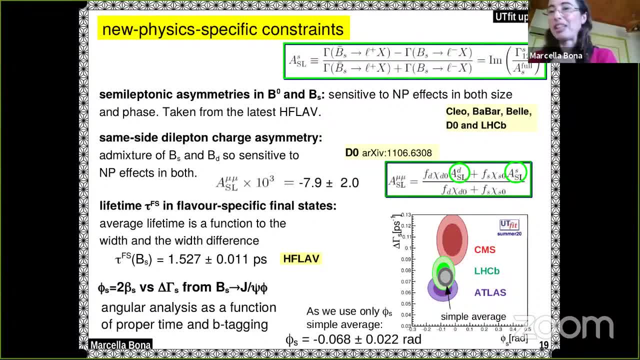 numbers, numbers, uh, they are not public, so there's, uh, they are not public, so there's, uh, they are not public. so there's there's no conflict of interest, but i, i, there's no conflict of interest, but i, i, there's no conflict of interest, but i, i have to admit. 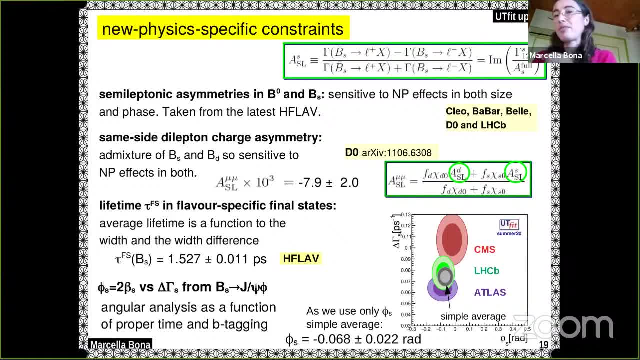 have to admit, have to admit, i'm not sure: 100 sure that i'm using the. i'm not sure 100 sure that i'm using the. i'm not sure: 100 sure that i'm using the latest from alice to be, because what i latest from alice to be, because what i 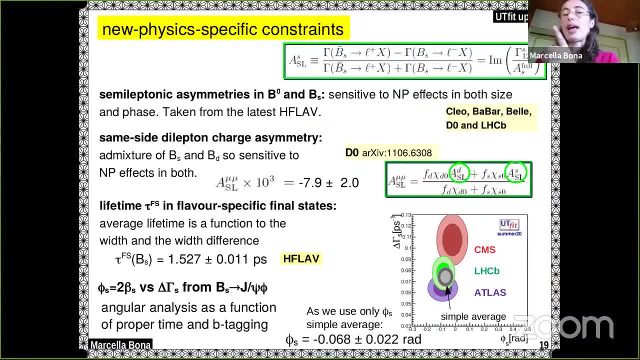 latest from alice to be, because what i want to use here, want to use here, want to use here, is the kk only. uh, oh, i see, is the kk only. uh, oh, i see, is the kk only. uh, oh, i see, i don't want to use the pi pi as well. 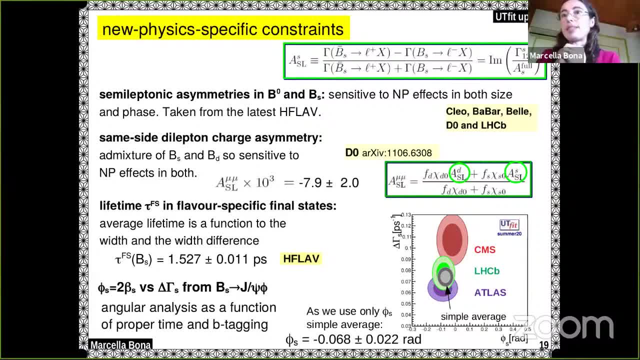 i don't want to use the pi pi as well. i don't want to use the pi pi as well because, in principle, because in principle, because in principle, friends and theoretical uncertainty: the friends and theoretical uncertainty, the friends and theoretical uncertainty: the company, company, company. um, okay, yeah also, what we plan to do is: 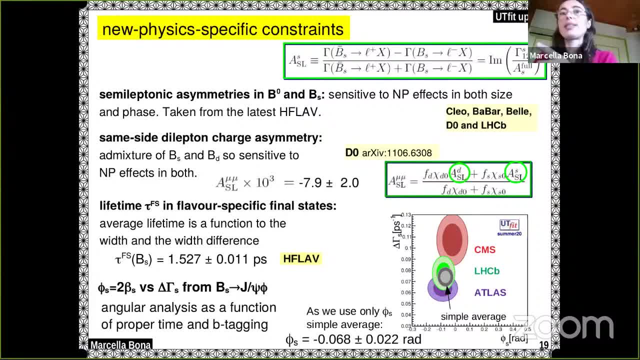 um, okay, yeah, also. what we plan to do is: um, okay, yeah, also. what we plan to do is to do, to do, to do, to add a theoretical uncertainty, uh, once to do to add a theoretical uncertainty, uh, once. to do, to add a theoretical uncertainty, uh once we. 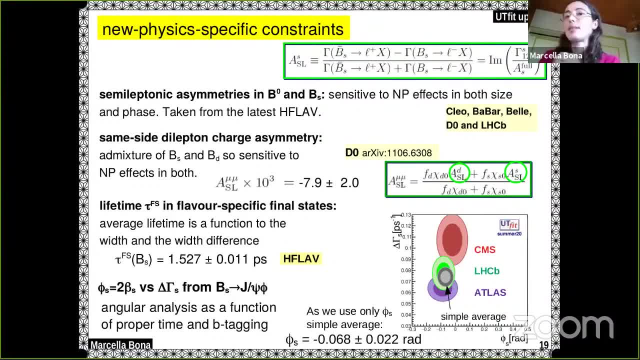 we, we. we have an estimate for this uh two. we have an estimate for this uh two. we have an estimate for this uh two, bit by s, bit by s, bit by s. measurement okay, thank you, thank you very. measurement okay, thank you, thank you very. measurement okay, thank you, thank you very much. 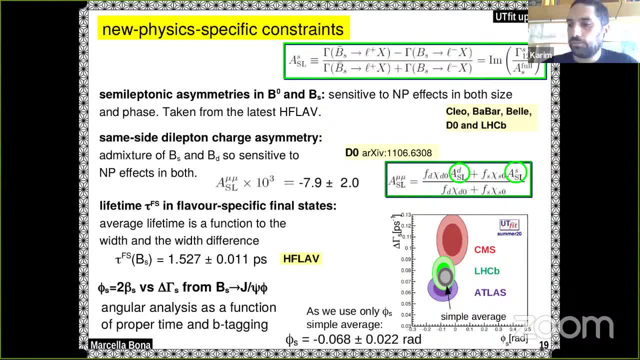 much, much. okay, thanks a lot for the discussion. okay, thanks a lot for the discussion. okay, thanks a lot for the discussion. i think now it's time for the coffee. i think now it's time for the coffee. i think now it's time for the coffee break. 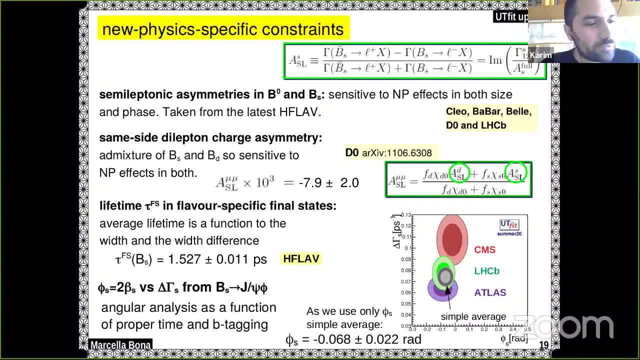 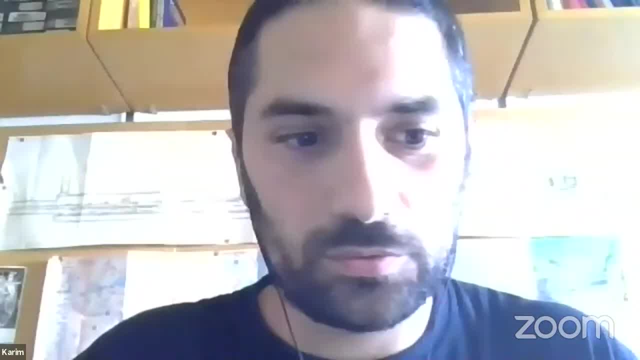 break break. i would propose to resume at. i would propose to resume at. i would propose to resume at five past five, since we are a bit a five past five, since we are a bit a five past five, since we are a bit a few minutes later. okay, so, 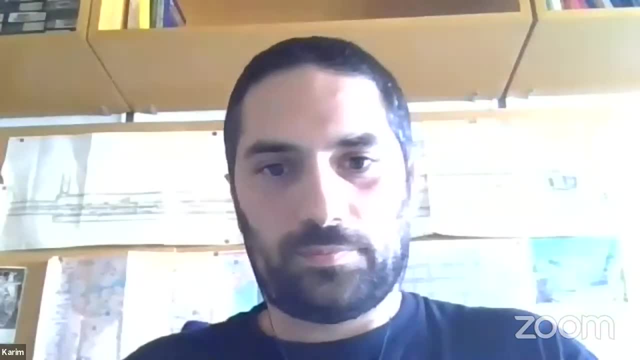 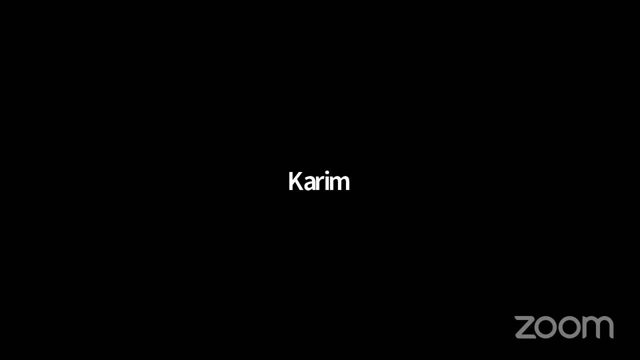 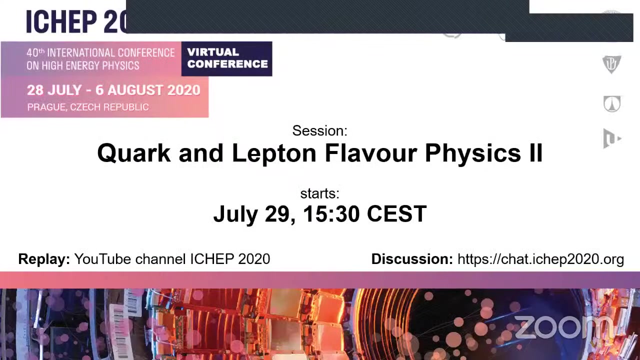 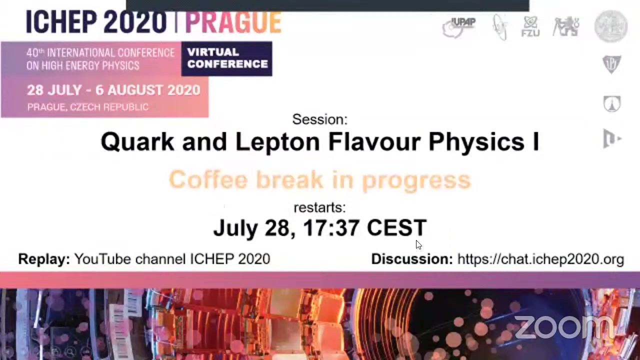 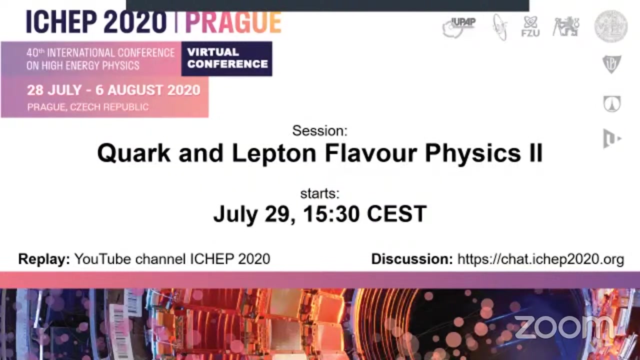 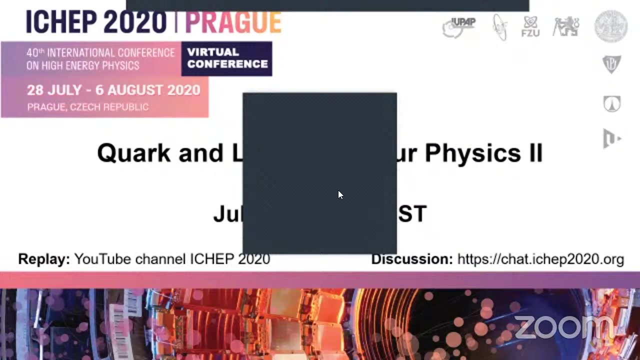 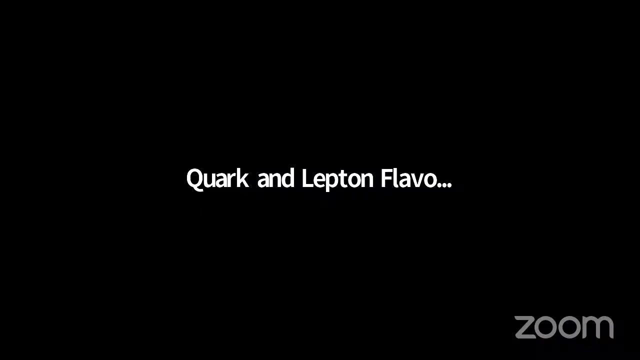 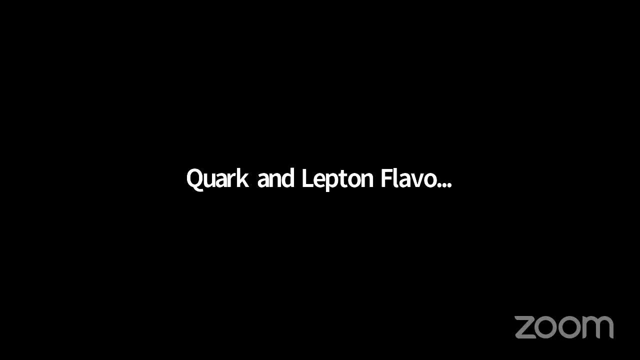 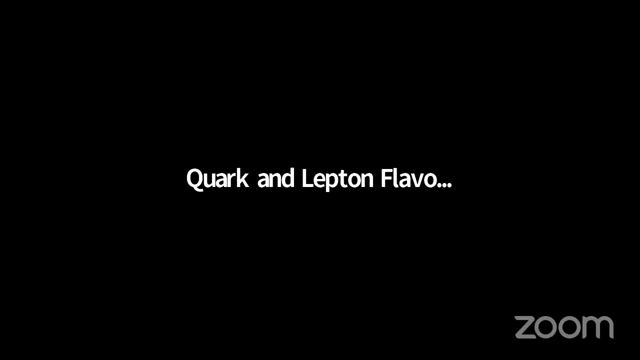 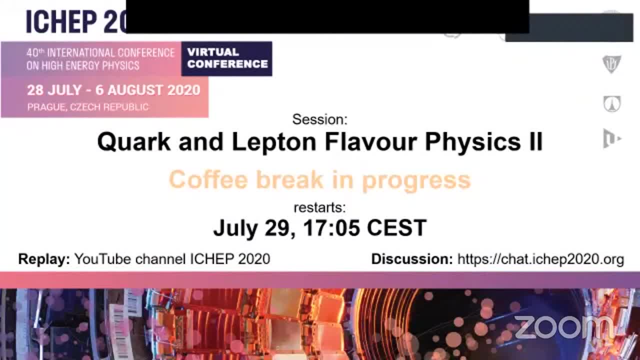 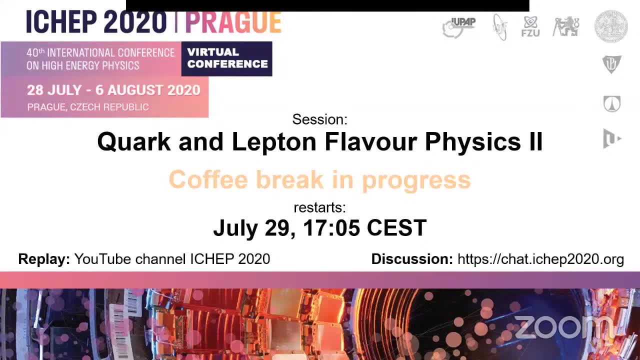 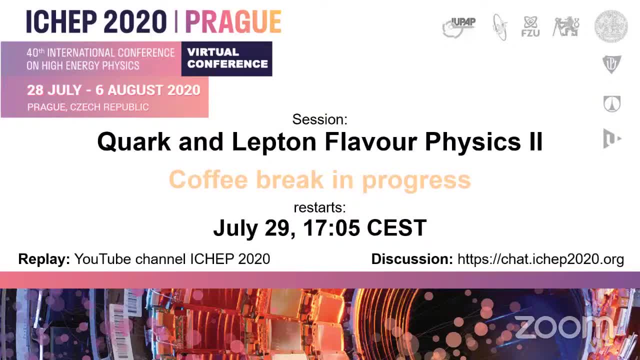 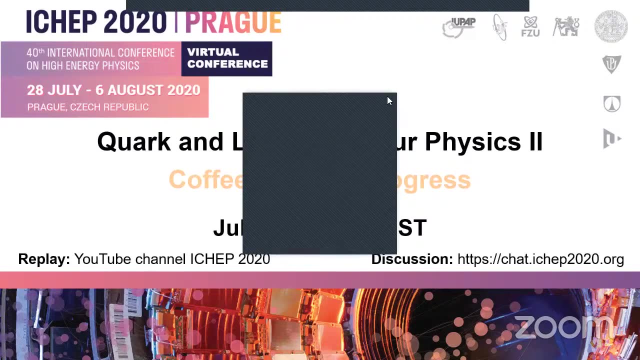 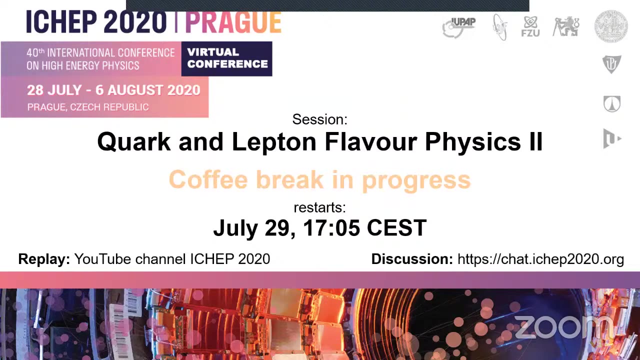 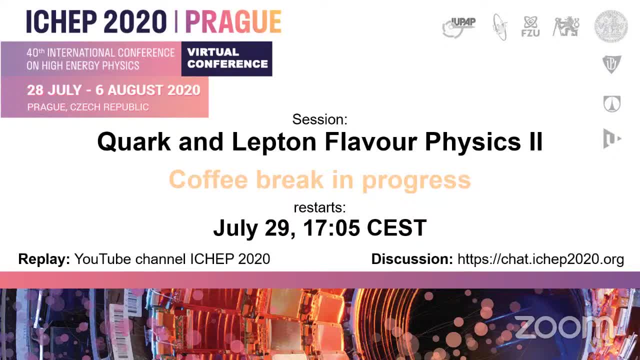 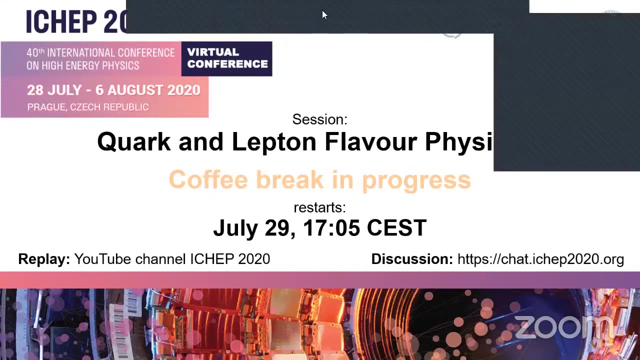 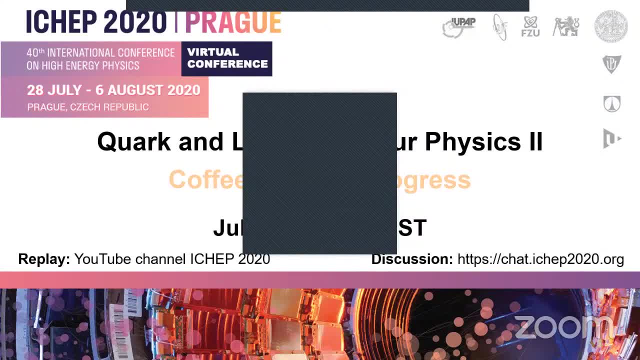 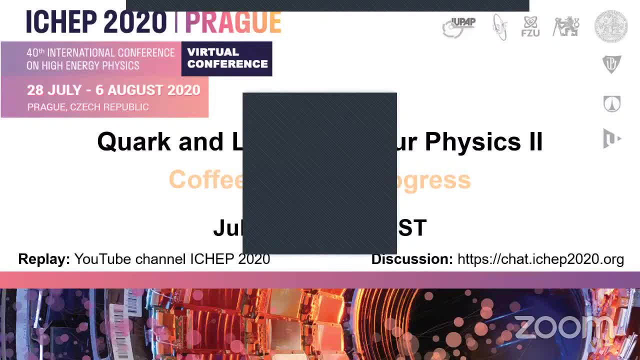 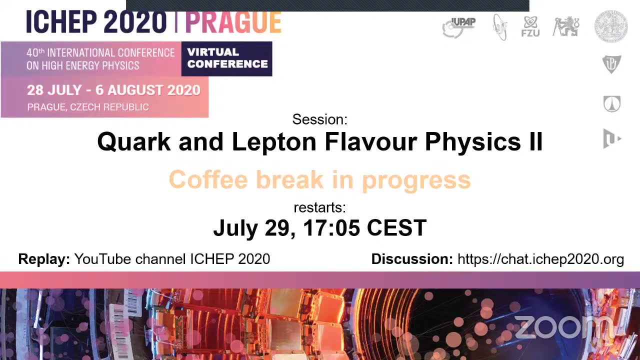 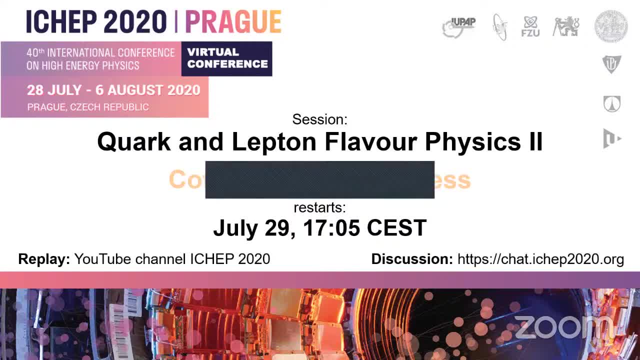 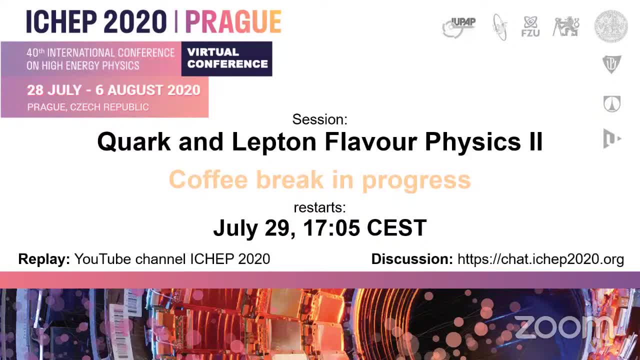 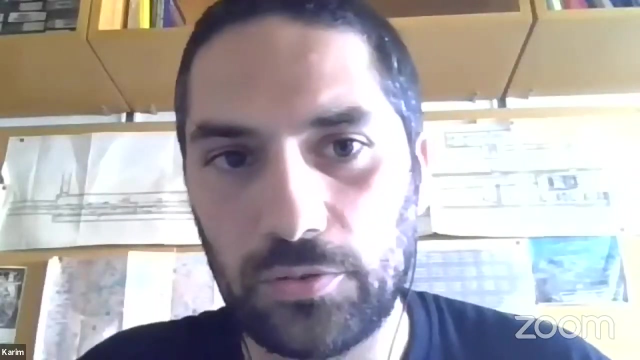 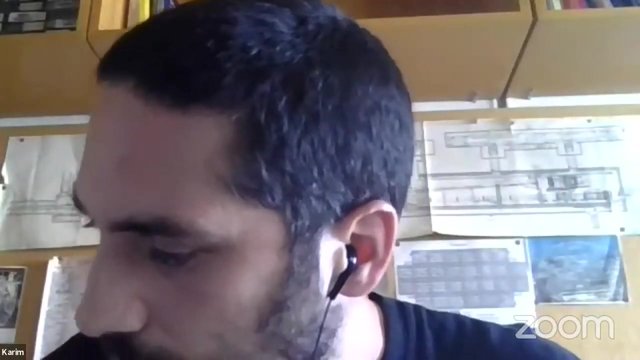 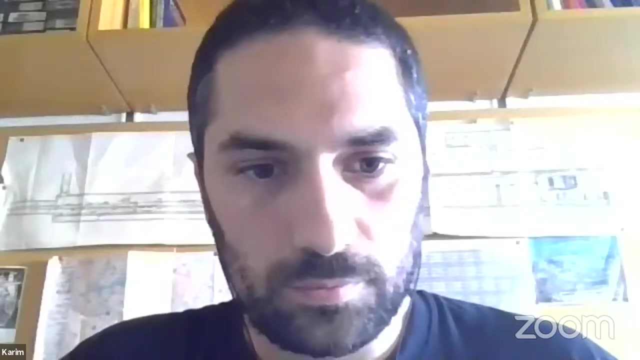 okay, welcome back. I think we can start this sub session, which is mostly dedicated to leptin flavor violation and leptin universality. leptin flavor universality: so the first talk is by stefan weber on the leptin flavor violation at lhcb. so please, stefan, yes, hello. 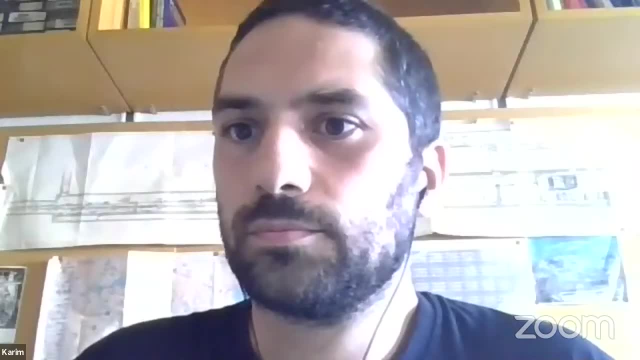 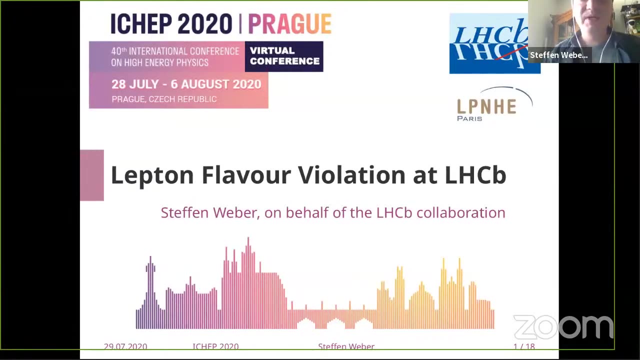 let me share my slides. i think you can see them now. yes, you can hear me. well, i hope, okay, thank you, yeah, thank you, so welcome to my talk. i will talk about leptin flavor violations and i will do this on behalf of the lhcb collaboration. 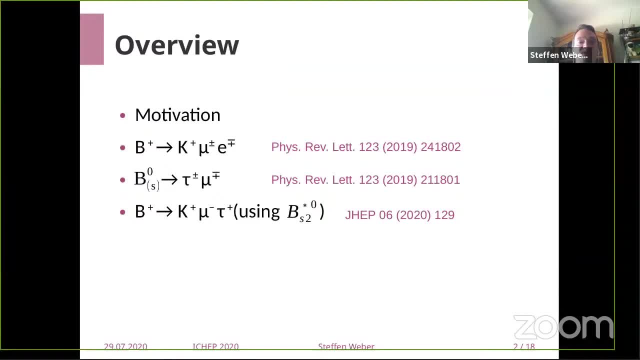 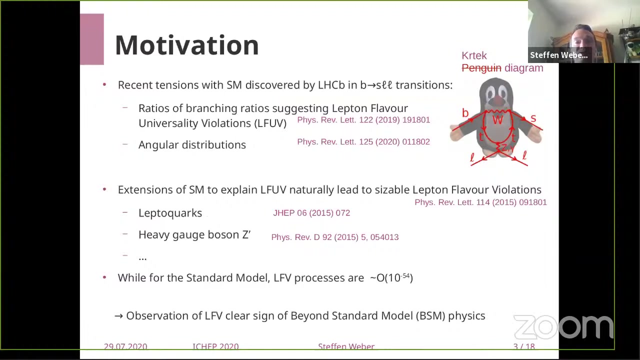 in my talk i will first give a brief motivation and then i will basically present three searches for leptin flavor violation. this is a b2k new electron, then b0 and b0s to tau mu and finally b2k mu tau. so recently there were some tangents with the standard model discovered. 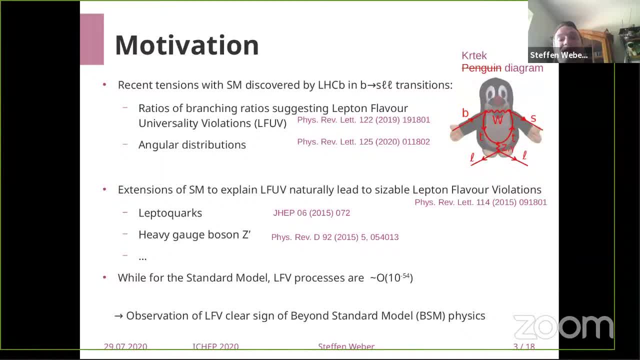 for example by the lhcb collaboration, and this especially within b2sl transitions. so examples are the ratios of branching ratios, which suggests that we see leptin flavor universality violations, and then we also have, and then we also have particular distributions of these decays and in general one one can say that 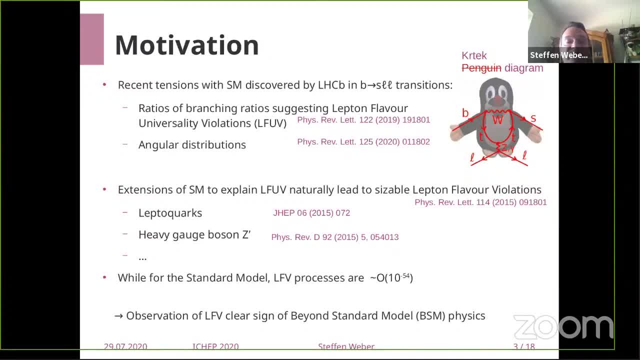 extensions of standard, of the standard model which are able to explain this, these effects. they quite naturally should lead to sizable lepton flavor violation contributions also, and examples for these models involve laptop quarks or heavy gauge bosons and many others. and on the other hand, in the standard 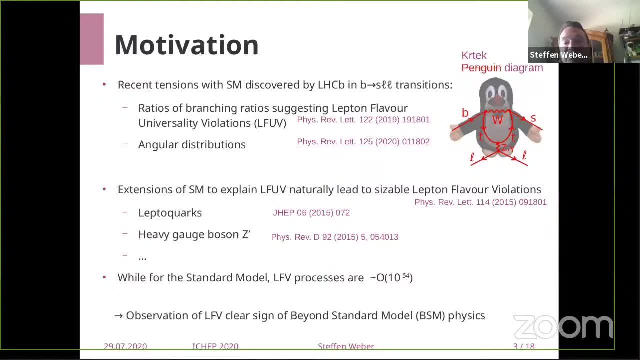 model. this lepton flavor violation processes are very much suppressed. so on the order of 10 to the minus 54, and this means this is unobservable within the foreseeable fetch up. this means an observation of lepton flavor violation would be a clear sign of beyond. 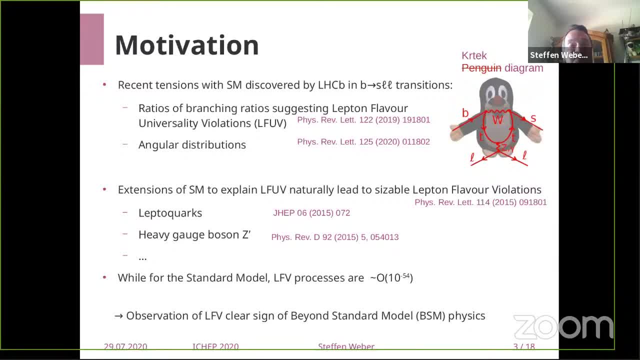 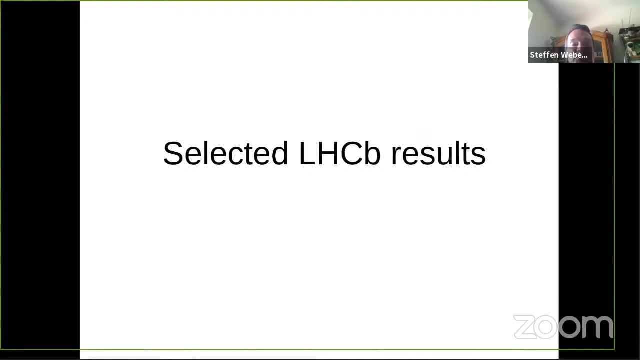 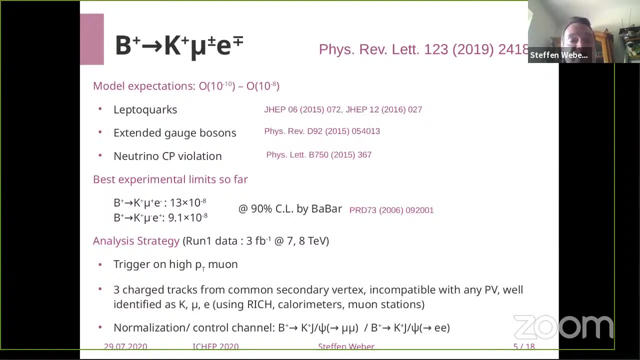 standard model physics so that's why we are looking for them and let me present some selected lhtb results the first one is the decay B plus to k plus so here on the left is oneullated k plus this is the � and then a neuron and an electron. 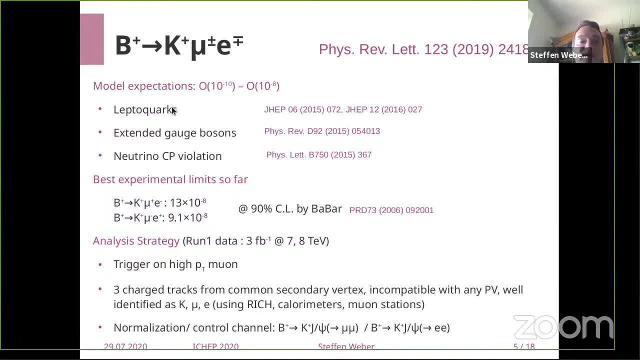 There are various models make predictions for this and they range between several orders of magnitude and this can go up to 10 to the minus eight. The best experimental limits so far come from the BABA experiment and one can distinguish between two chart configurations and the limits are on the order of 10 to the minus eight. 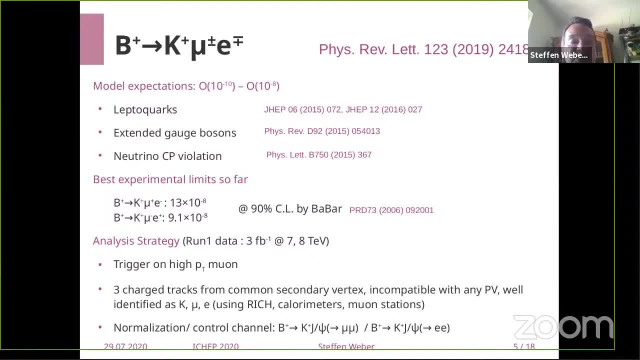 In our LHCb analysis we have been using run one data. These are three inverse femtovarn at seven and eight TeV. The basic strategy is to trigger first on a high momentum, high PT muon, Then, as the next step, require three charts. 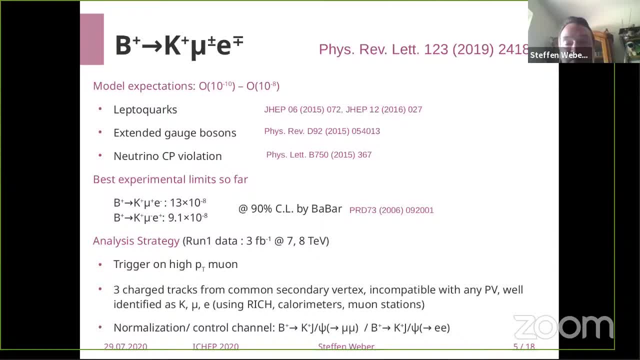 chart tracks which form a common secondary vertex which is incompatible with any primary vertex of the event and which are identified as a Keon, muon and an electron using our PID detectors that we have To calculate the branching ratio. we don't usually do this in absolute terms directly. 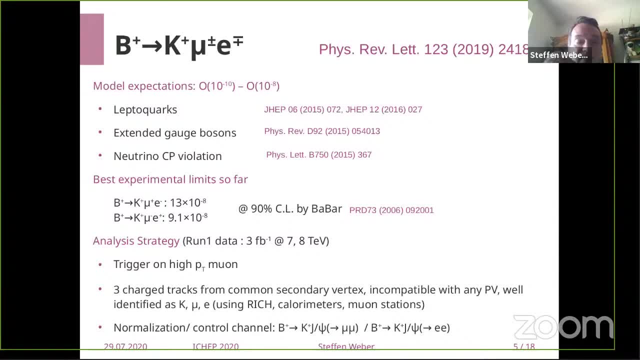 but we normalize this to a well-known decay channels, And in this case this is the decay B plus two K plus and the gypsy, with which then decays further to a di-muon pair, and as a control channel we also use the di-electron pair. 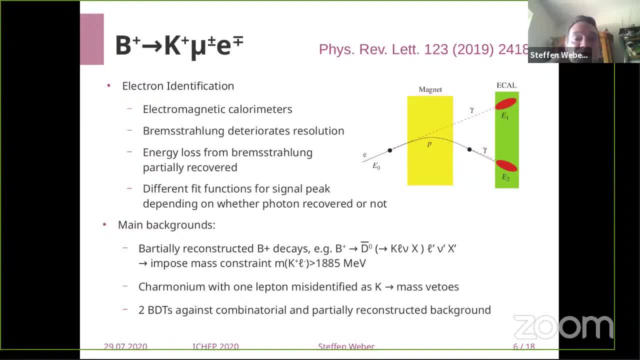 So in the analysis we have to reconstruct an electron. This is a bit complicated because this can radiate bremsstrahlung, But within our calorimeters we are also able to recover partially the energy loss from bremsstrahlung. 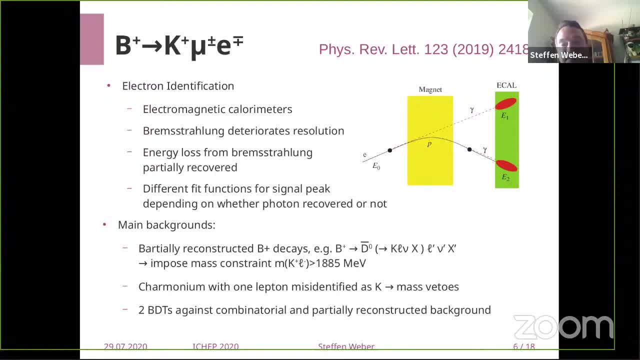 This does not work perfectly, but with this. so we lose a little bit of resolution, but we can partially resolve this And within the analysis then different fit functions can be used for the different cases of whether we have photons of bremsstrahlung recovered or not. 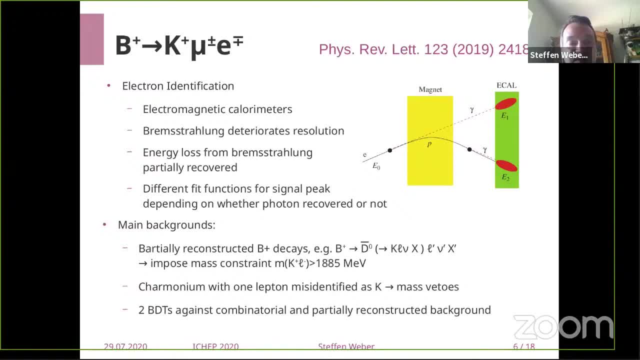 In the analysis the main background consists of a partially reconstructed PD case. So you can have this case where you have a double semi-leptonic decay which can produce this pair of leptons, And for this one can impose mass constraints on the combinations of the decay products. 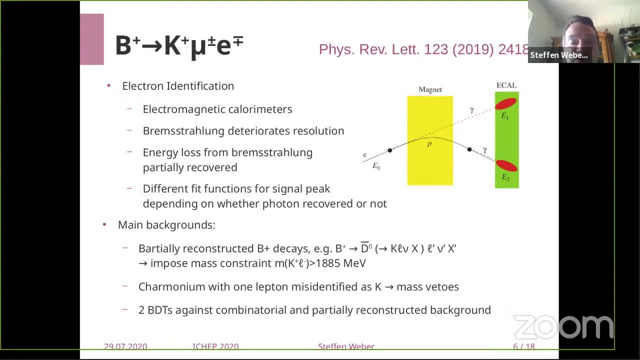 It's possible to have a germanium decay with one of the leptons misidentified as a kaon, and this can be cured with mass V2s. Then in the analysis we also employ two boosted decision trees against combinatorial and partially reconstructed background. 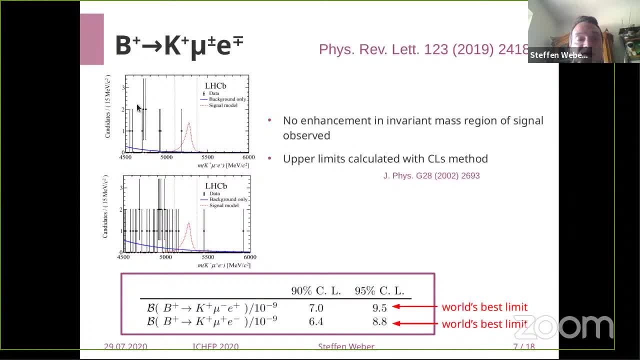 Yeah, these two invariant mass distributions here then show that we do not observe any signal in the region where we look for it, And that's why we can give upper limits for this decay. And we arrive to a value of seven times 10, to the minus nine. 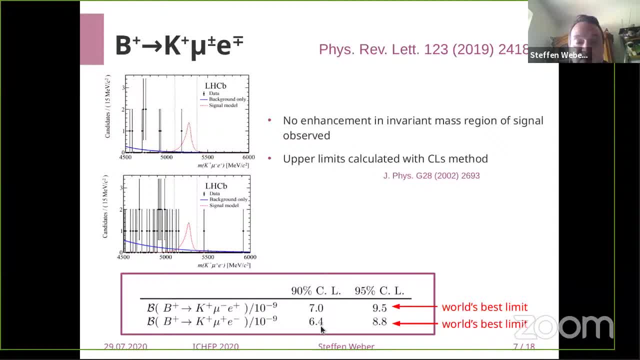 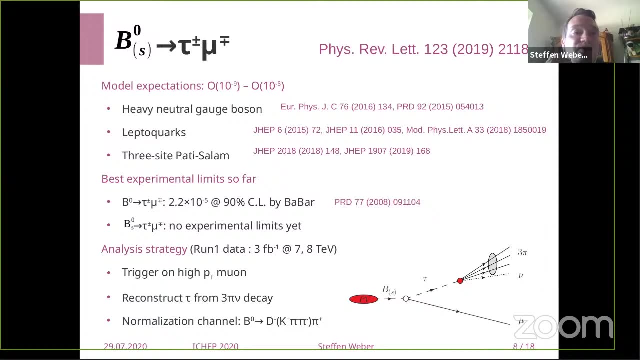 for the K plus mu minus E plus charge combination and 6.4 times 10 to the minus nine for the K plus mu plus E minus, And both of these are the world's best limits so far. Next decay which I want to present is the V zero. 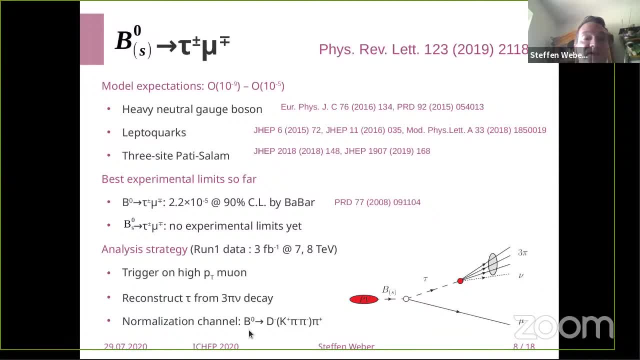 or V zero sub S, two tau mu on pair. They are the model. expectations go up to the order of 10 to the minus five. The best experimental limit on the V zero decay comes from the Baba experiment. It's 2.2 times 10 to the minus five. 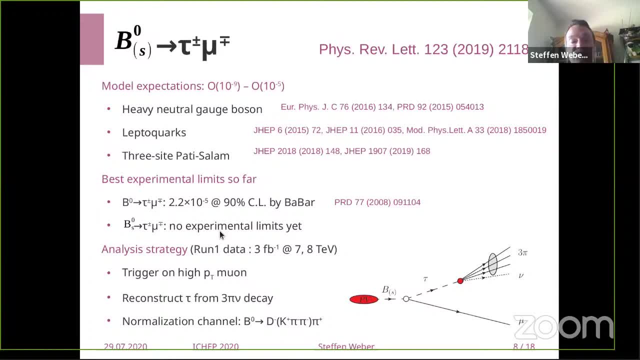 While for the V zero sub S, there is no experimental limit so far. The analysis strategy is a bit different. Again, we use three femto bonds from run one. Again, we trigger on a high PT muon, but in this case we have to reconstruct the tau. 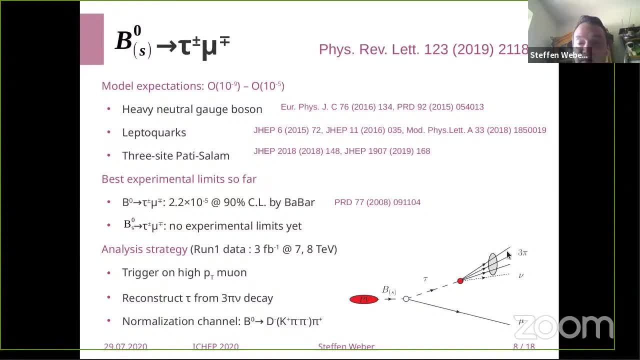 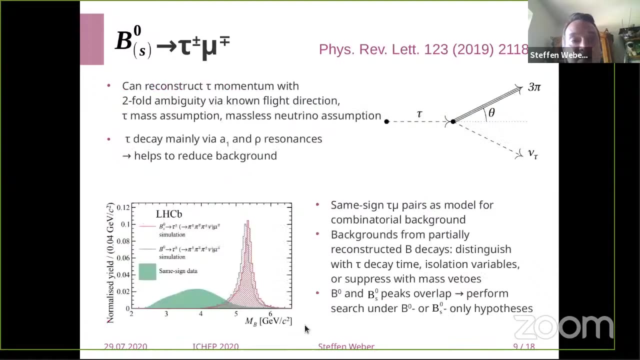 from it's decay products. For this we use the three pion neutrino decay of the tau on, And then again we normalize to a well known normalization channel which has a similar topology. as our signal decay We can reconstruct the tau momentum. 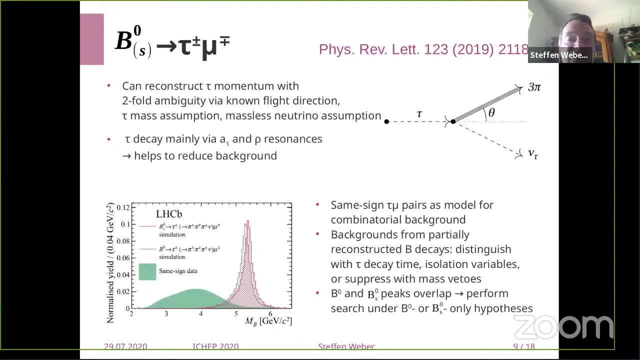 with the two fold ambiguity from the known flight direction and under the assumption that we have tau mass or massless neutrinos. And one can also use the fact that the tau in the case mainly via the A1 and row resonances, And this helps also to reduce the background. 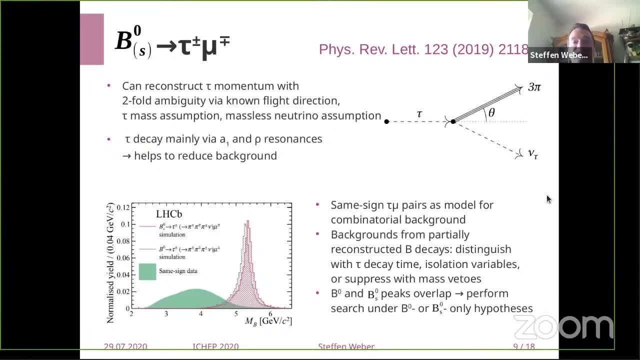 from other particles. We can also use same sign tau mu pairs as a model for the combinatorial background which is then used for the training of the BDTs- An important background, also partially reconstructed BDKs. This can be distinguished from the signal. 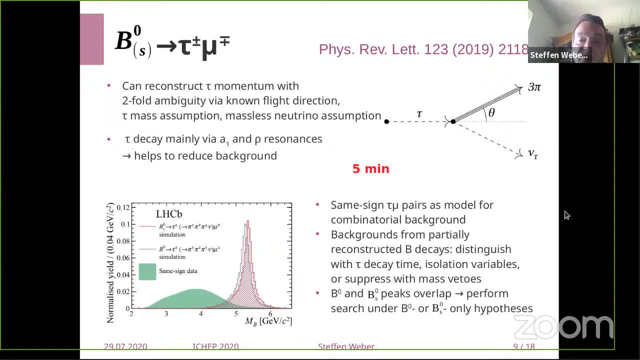 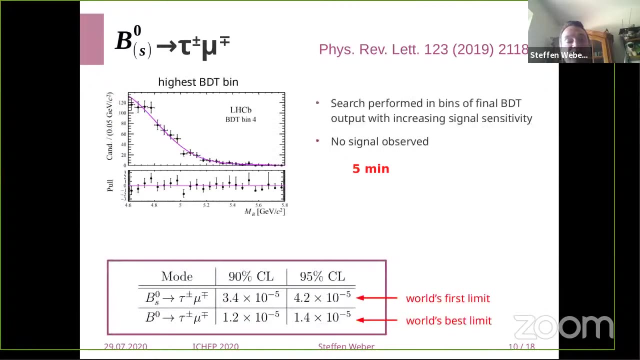 with help of decay time isolation variables and can be suppressed with mass vetoes. Here I illustrate that the two, the B zero and B zero S, the peaks, overlap, and that's why we perform all search for the hypothesis that we have the one or the other. 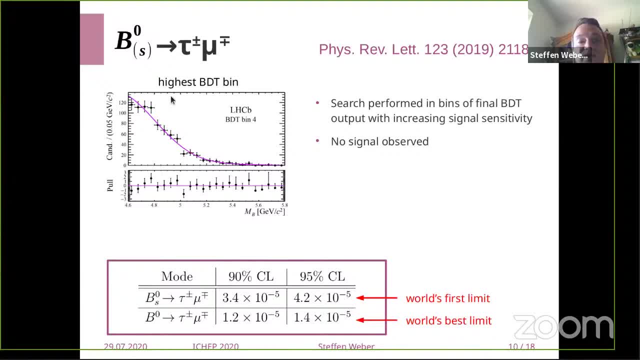 Search is performed in bins of a final BDT. Here for illustration I show the bin with the highest signal probability. Again, we don't see a signal. That's why we can give confidence limits. So for the B zero sub S we have a 3.5 times 10 to the minus five at 90%. 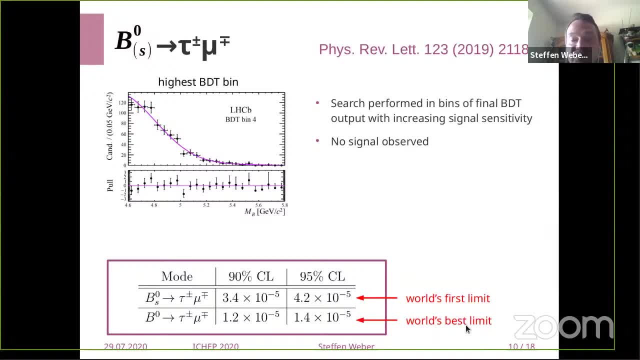 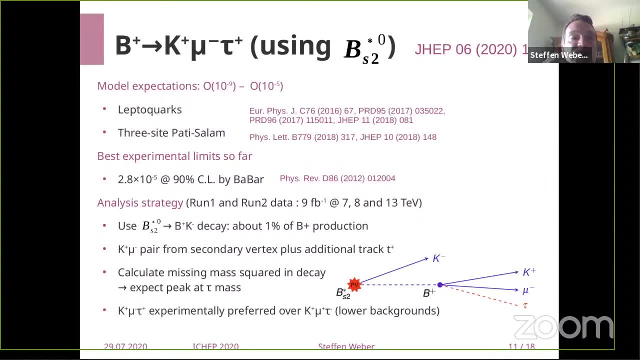 And for the B zero, 1.2 times 10, to the minus five, which is the world's best limit, And the other one is the first limit so far. Then the final decay which I want to demonstrate is the B plus two, K plus mu tau. 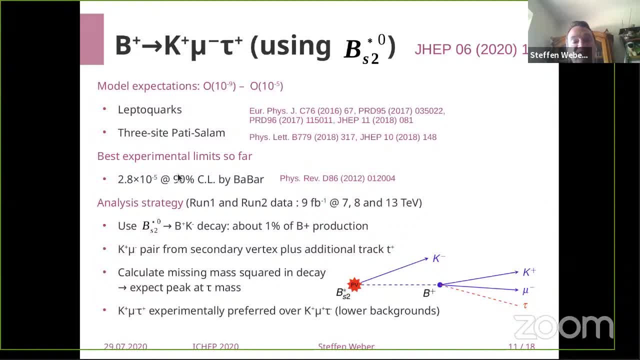 Again, the model expectations reach up to 10 to the minus five. The best experimental limit 2.8 times 10 to the minus five. Here the analysis strategy is a bit different. We use both run one and run two data. So this is nine inverse femtovans. 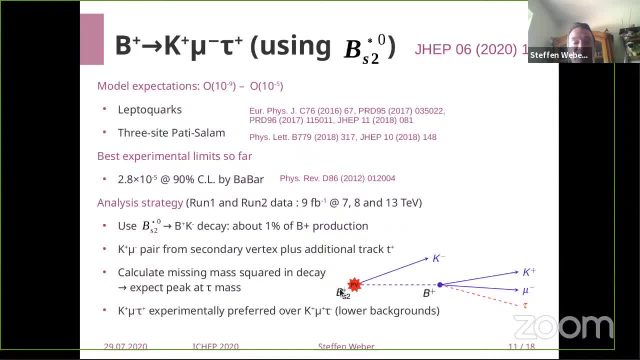 And we actually consider B plus from the decay of the B star sub S two. This means we require a pair of a K on the muon from the secondary vertex plus an additional charge track, And then we can calculate the decay of the muon. 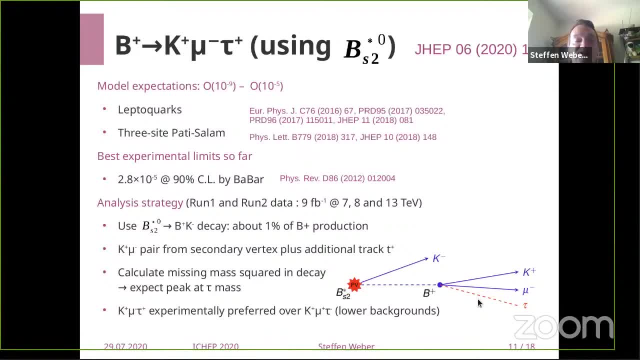 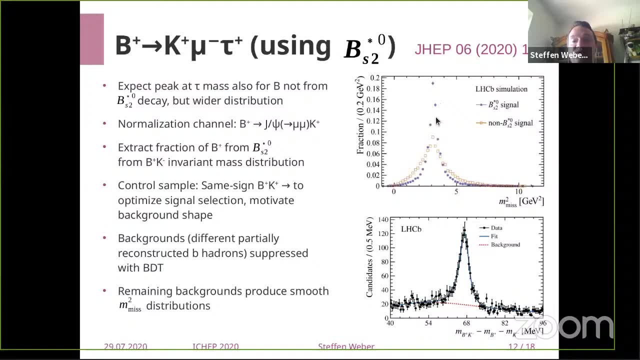 We calculate the missing mass squared of this track And we expect the peak at the tau mass for the signal. This is illustrated here. So for a signal we expect a clear peak as a. again, we use a normalization channel which is B plus two J psi, K plus. 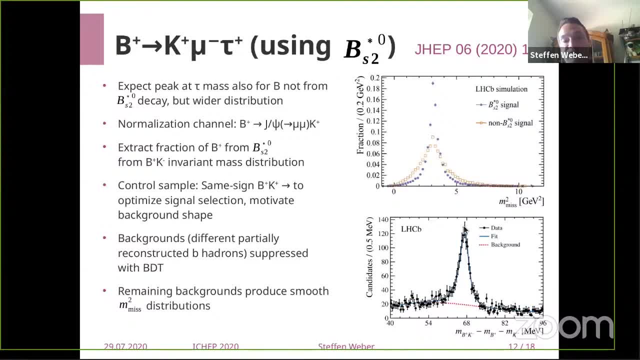 We can also extract the fraction of which of the Bs come from this. B star S two decay And which are independent of this. And then we have several backgrounds which can be suppressed again with the help of boosted decision trees And the remaining backgrounds. 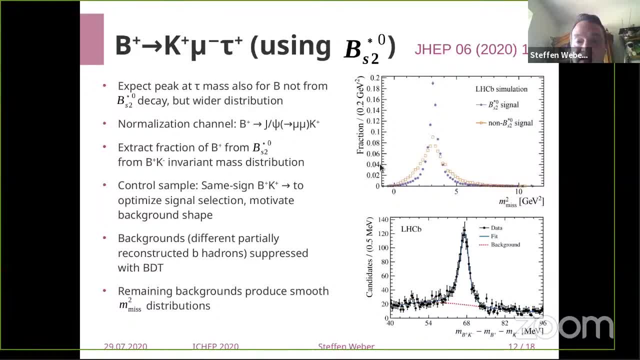 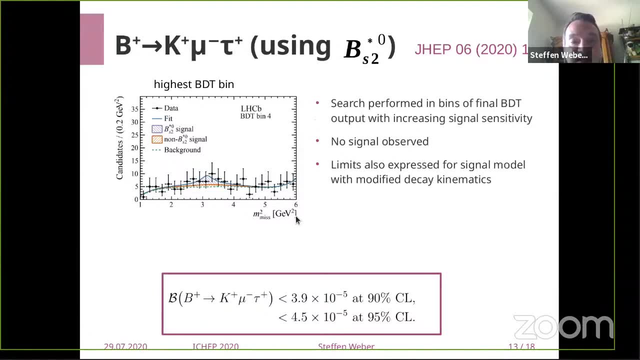 we don't. we expect a smooth distribution in this missing mass squared distribution And also in this case, we don't observe any signal And we can extract. Okay, We have a few limits from this And our limits are 3.9 times 10 to the minus five. 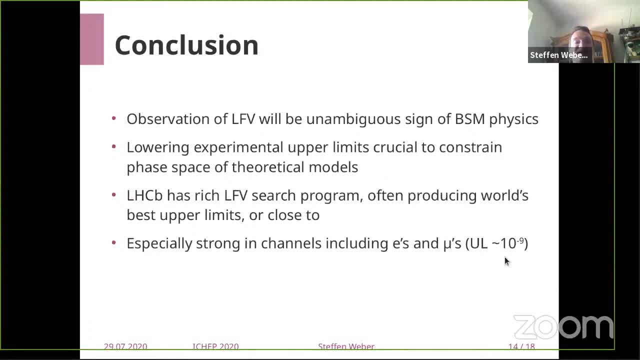 which is comparable to the world's best limit. In conclusion, we can say that an observation of laptop play violation would be an unambiguous sign of beyond standard model physics. So lowering the experimental limits is very crucial, also to constrain face base of theoretical models. 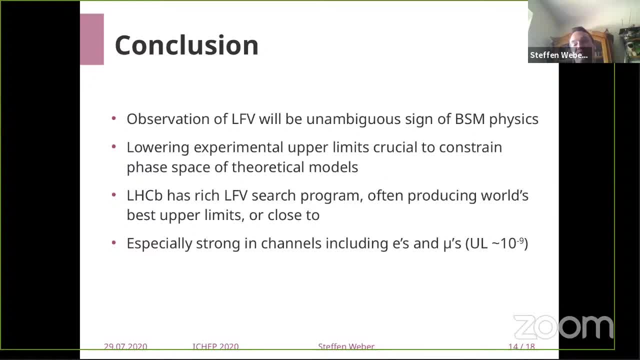 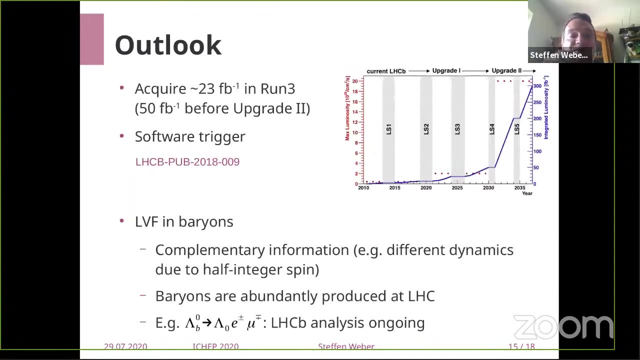 And LHCB has a very rich search program for this laptop field violations, of which I presented to you few examples. and often we are able to produce the world's best upper limits or we are close to a little bit of outlook. so of course, in the future, we want to 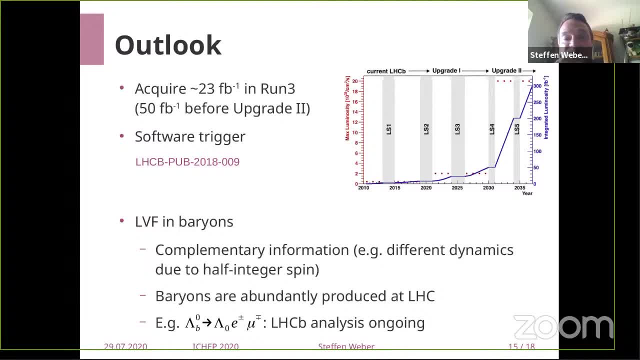 collect more data. this is about 23 investment ones in run three. we will use a purely software trigger in in this run which will help us to cope with the higher luminosities, and another aspect which i would like to mention is that we are also able to measure lepton field violations and 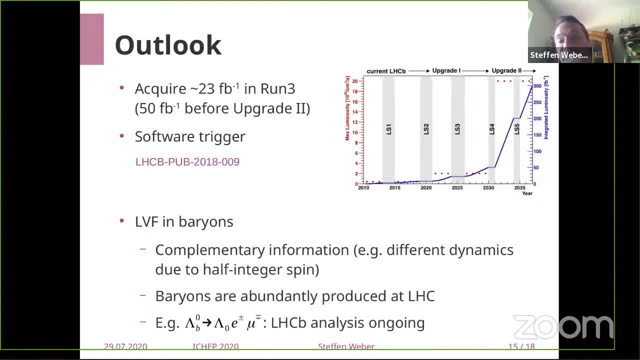 variants which can give complementary information. so, for example, we have different dynamics due to the half integer spin of the variants, and these are abundantly produced and, as one example, the lambda b to lambda e mu decay is currently being analyzed by lhcb. so thank you for your attention. 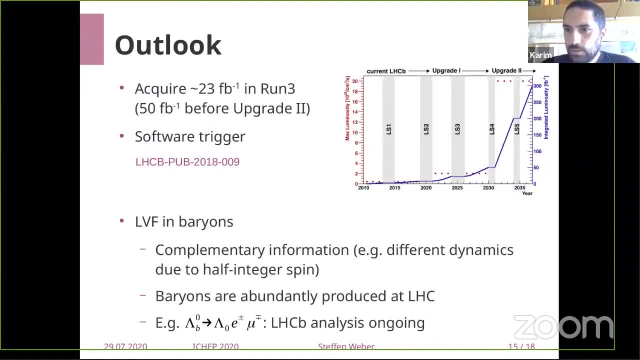 thanks a lot, so let's see if there are any comments or questions from the audience. i do not see any, but okay, i have one. i've seen that you have. among other things, you have presented the upper limits on the branching ratio of the b0 to mu tau. 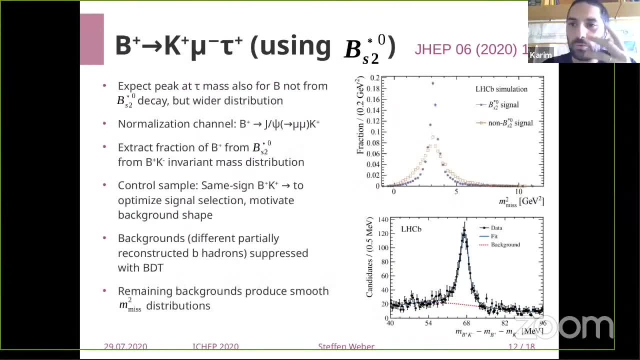 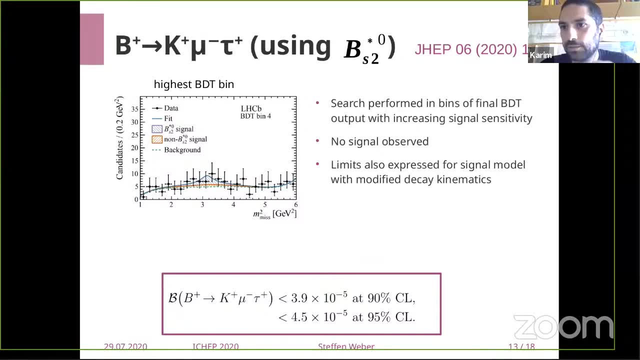 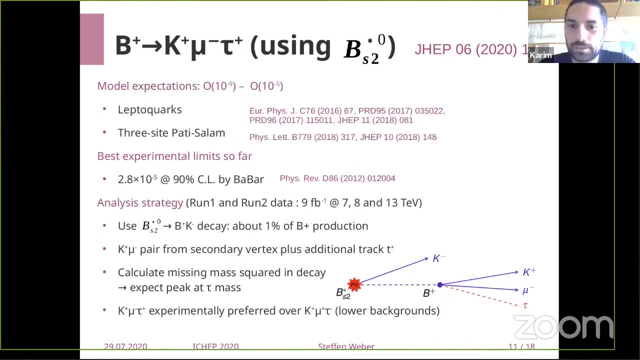 and the b plus to k mu tau. but i was wondering, regarding the theoretical interpretation, which one should you consider for the qs? one would be more sensitive between the two, for instance on laptop work or new particle, Or if there are different models which are, let's say, shared. 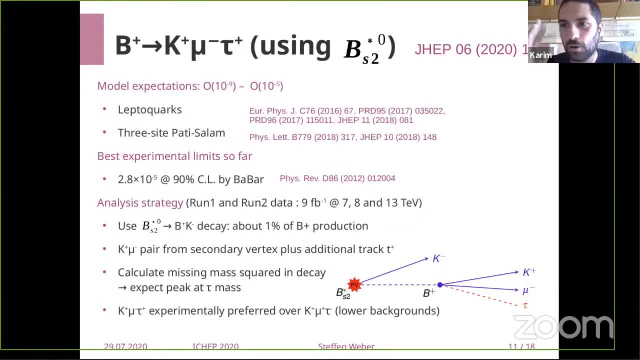 like there is one model in particular for which the B0 mu tau is more sensitive rather than B plus. If you could comment a bit on this. No, I'm not really an expert on the models And I think they give vastly different limits depending. 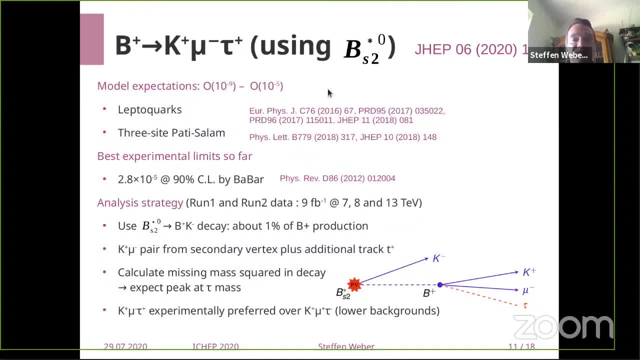 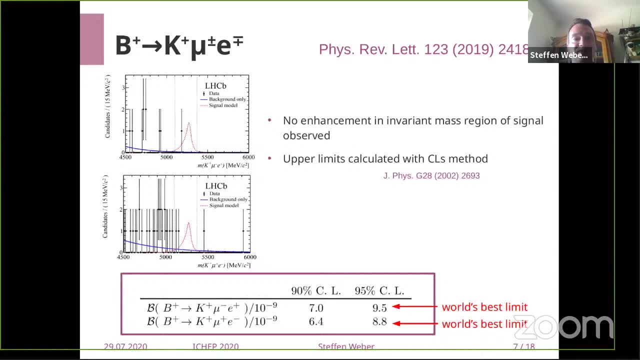 on the flavor of your models. But I think one thing: one can say: that really, for this decay involving mu and an electron, we go very deep. We go in the order of 10 to the minus 9.. While model expectations, indeed, they reach up. 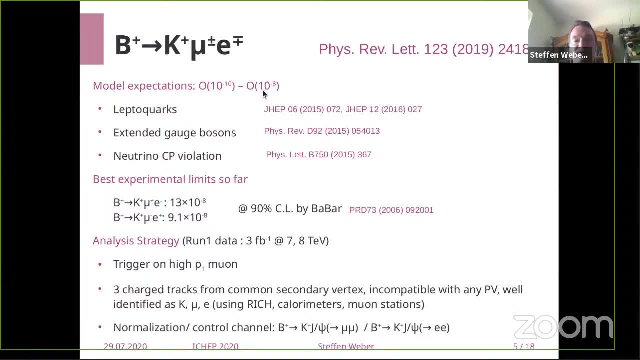 to 10, to the minus 8.. So I think there we are indeed doing quite some restriction of the phase space of these models. OK, yes, OK, no. my question was more about the mu tau, But in any case, it's clear that the searches are. 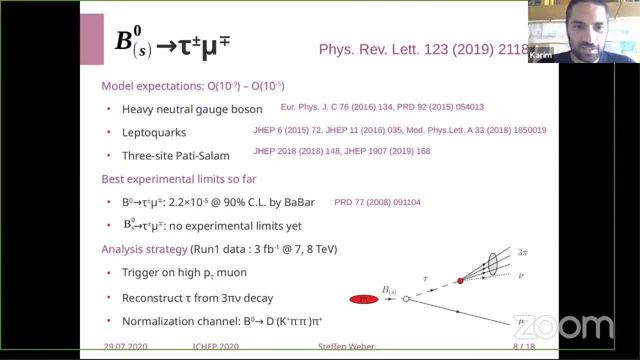 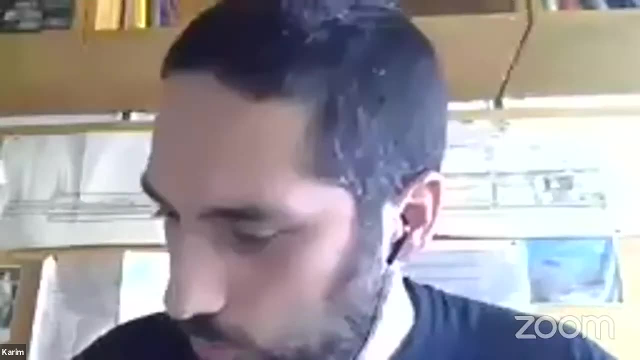 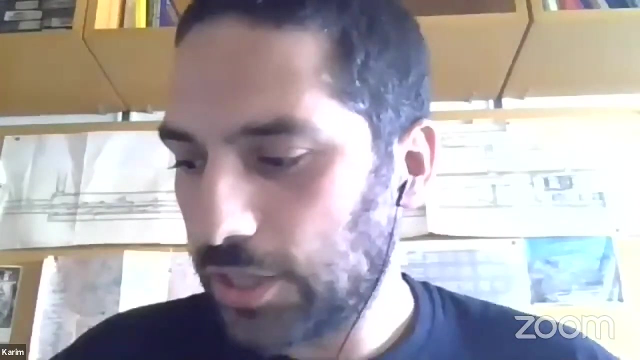 very nice and interesting all the ones that you have presented. OK, so there are no more Any other comments or questions on these. Thanks again, Stefan, And we move on to Altsir, who will present a review of the leptin flavor violation at LHC. 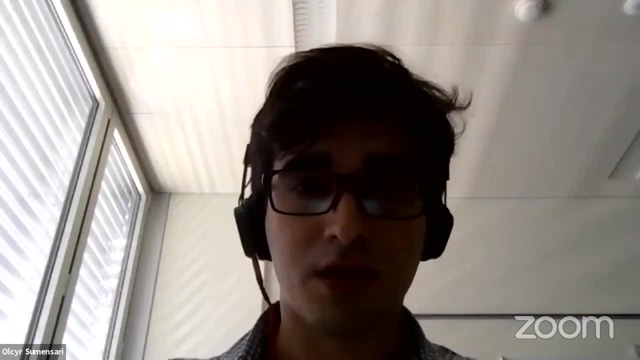 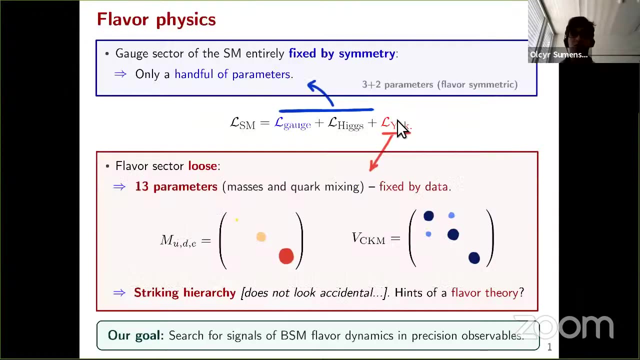 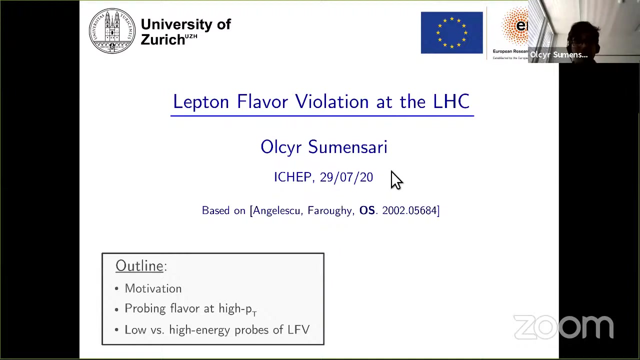 OK, can you hear me? Yes, OK, very good. so let me share the screen, OK, so can you see? Yes, OK, very good. OK, thanks a lot. My name is Altsir and I'm very happy to tell you a bit today. 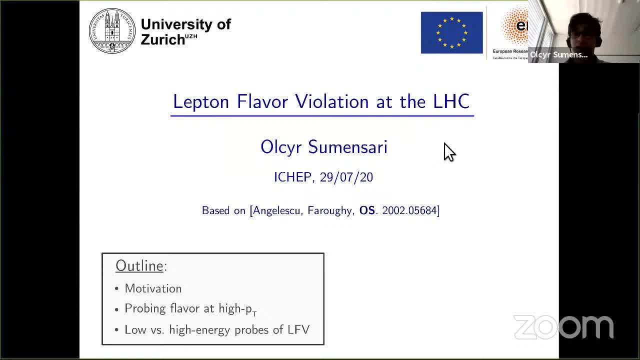 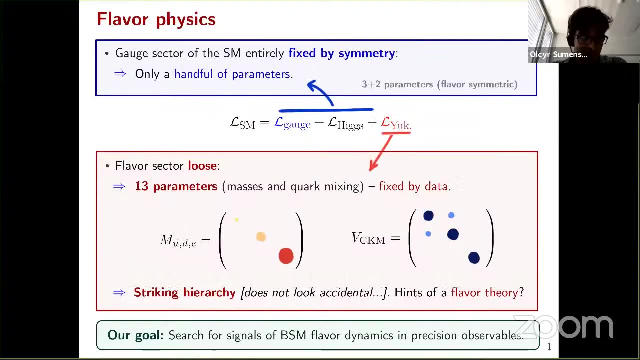 about flavor physics. that can be done at high PT, And particularly I'll continue the discussion on leptin flavor violation, And so I'll present these results from this recent publication of ours, And I'll start with a brief introduction, which is our motivation here. 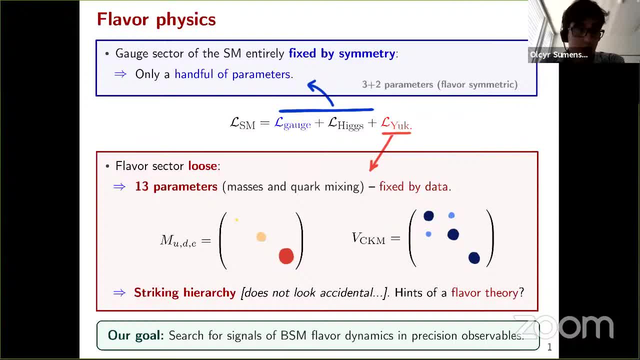 So, basically, when you do flavor physics, you're going to get a lot of information, And when you do flavor physics, the ultimate question that we would like to answer is the flavor problem, And the flavor problem is basically the fact that in the standard model, 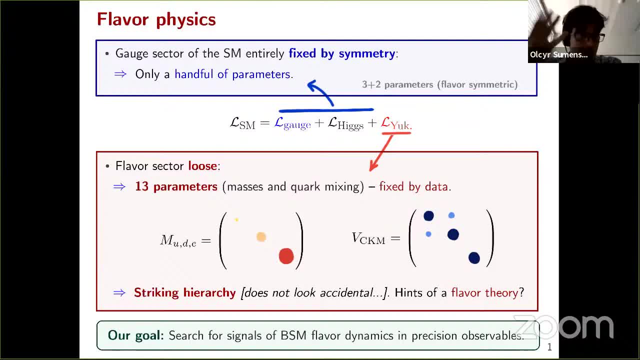 we don't have flavor symmetry- That would be equivalent to the gauge symmetry, the gauge sector. So that flavor is pretty much unconstrained And the consequence of that is, as you know, is that we have many parameters in flavor. so the fermions, mass and mixing, which 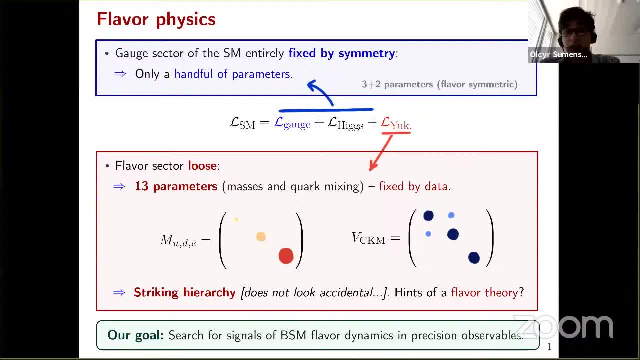 can be described by means of interactions, But then we have to extract this information from data, And this is a problem, not only because flavor becomes then highly non-minimal, but most importantly by the fact that, when you look at these values for the fermion, 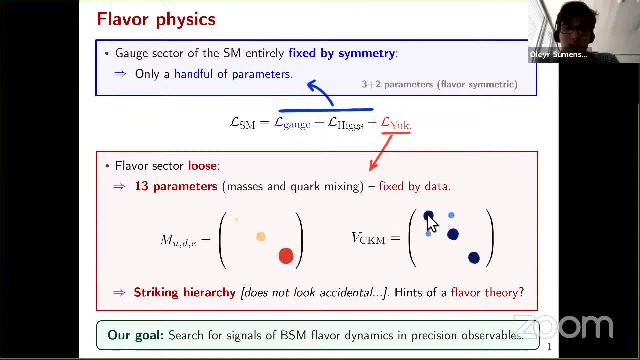 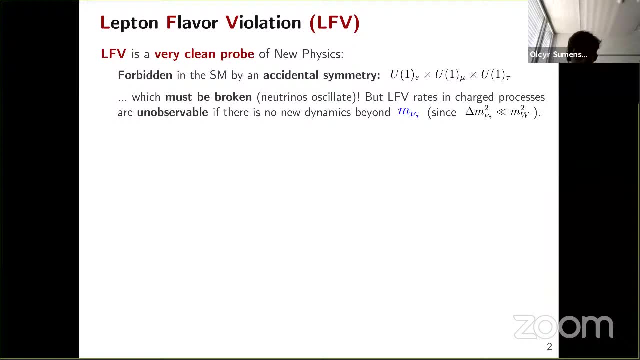 masses or the mixing parameters, we see clear patterns that suggest something beyond the standard model. So our goal, then, is to look for any signals of these beyond the standard model. flavor dynamics by using low-energy observables, And the key observables are the ones where flavor is violated. 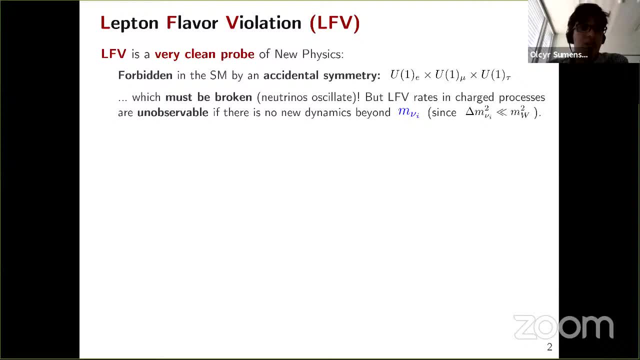 And lepton flavor violation, as we just heard, are particularly interesting. They are interesting because they are forbidden in the standard model by accidental symmetry. We know that the symmetry should be broken because neutrinos are massive and oscillate. But even if you plug in the neutrino masses, 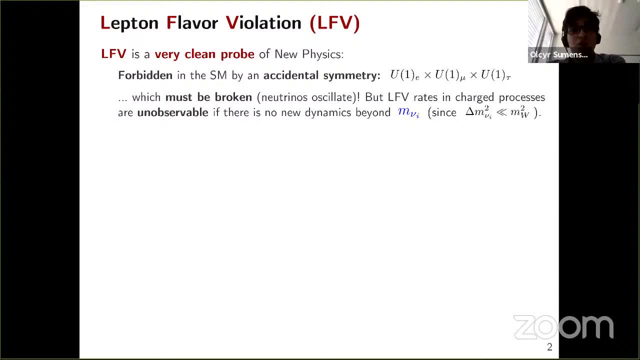 assuming that there is no, No other dynamics. we see that all these processes are completely unobserved. So that's why we say that they are very clean And that's why it's important to look for them experimentally And from the experimental prospects. 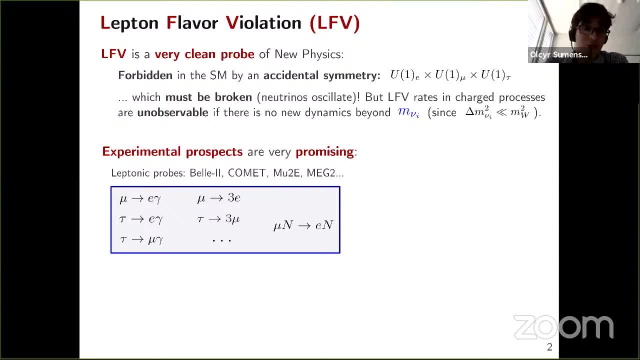 we also have a very promising scenario for the coming years as well. So these decays, they can be in purely leptonic observables, such as the tau and mu decays, And here there are many experiments that are pushing in this direction. 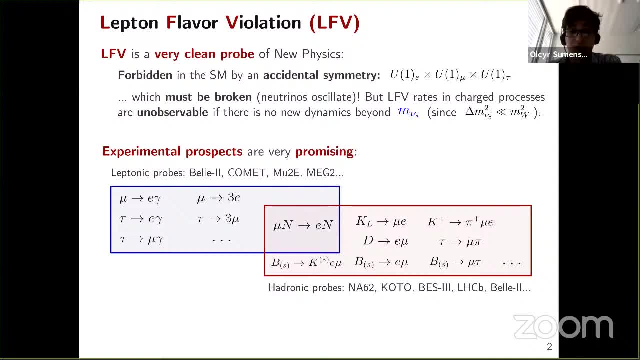 And we also have the hadronic probes with decays of k-ons, d- and b-mesons, which are quite interesting, And these are the ones I'll be talking about today. So the goal of my talk is to tell you what can we learn by using proton collisions. 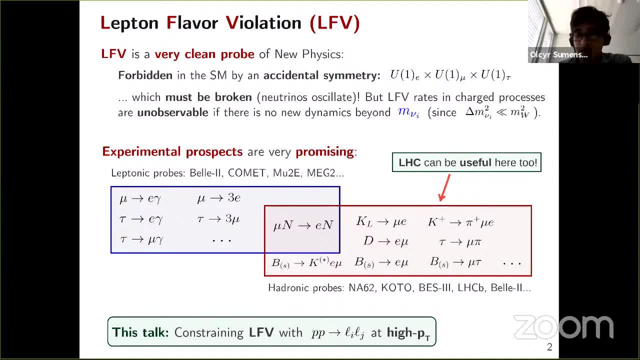 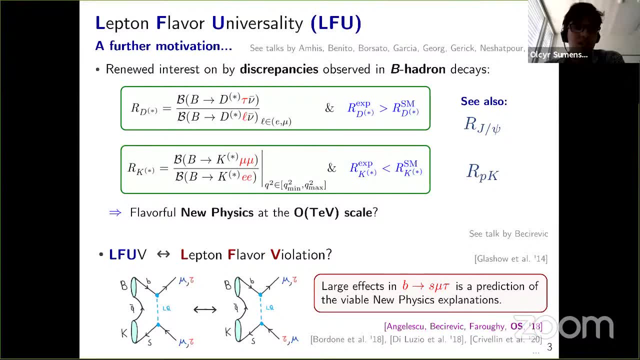 How can we get some indirect information on these decay modes? And a further motivation for that that I'll mention very briefly are of course these b-physics anomalies, Because here It suggests that there is new physics around the corner with lepton flavor dependent couplings. 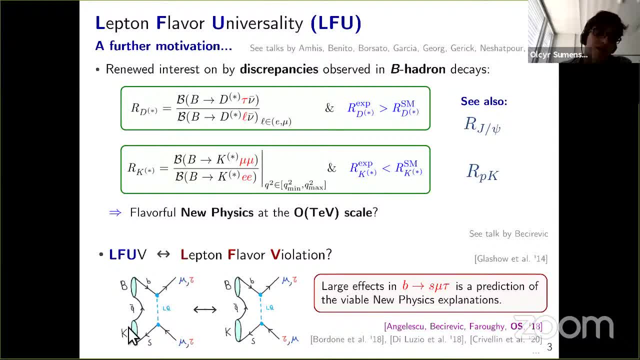 And nowadays we know that the only particles that can actually explain these discrepancies are the so-called lepto quarks, And they must couple to muons and taus. So here, if you just swap the flavor in one of these legs, you see that's almost unavoidable. 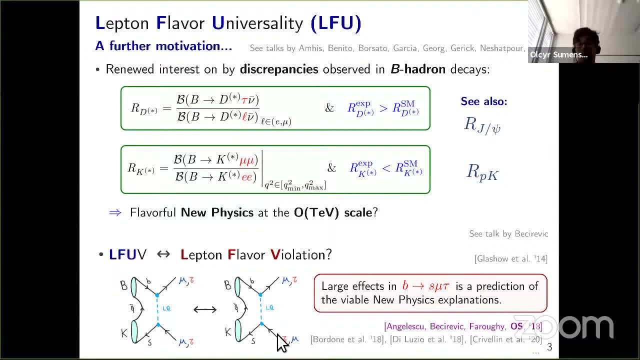 to have lepton flavor violation to some extent. So there's a common prediction of these viable models And that's why it's so important. So to push in this direction, like we're doing now with LHCb and Bel2.. OK, 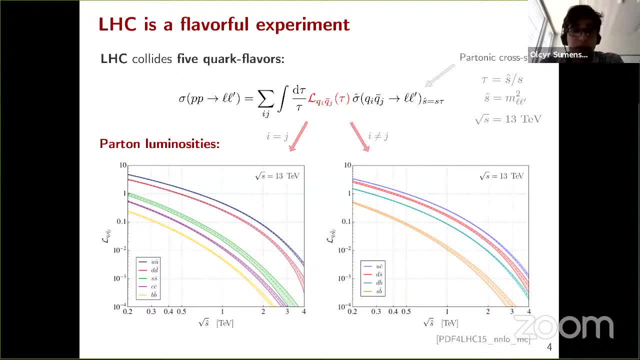 But today I'll be talking about LHC, And the main idea behind this talk is the following: when you collide protons, that's also a flavor physics process, So actually the cross-section for proton-proton into di-leptons that can be factorized. 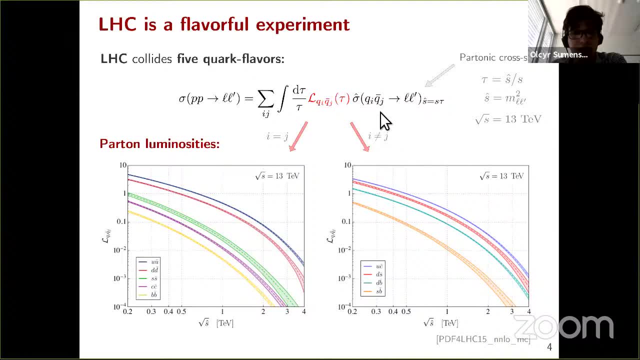 into a partonic cross-section where we can have five different quark flavors And then we have these luminosity functions which depend on the quark PDFs And that weight the different contributions to the total cross-section And, as you see in these plots, these luminosity functions. 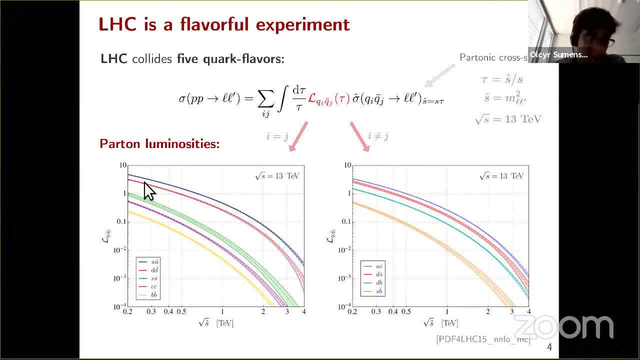 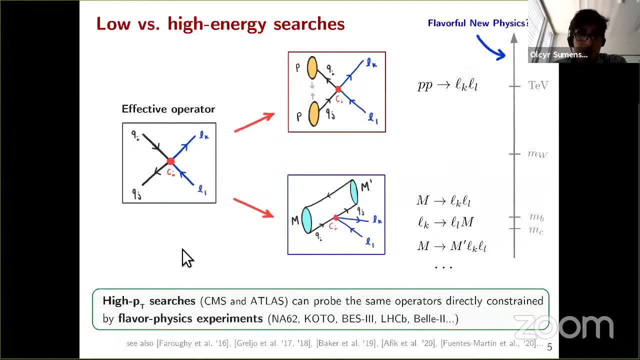 are bigger for the first and second and third generation- first and second generation- And then they are smaller for the big quark, for example. And the approach we use is effective in theories, because this is the most economical one that we can have. 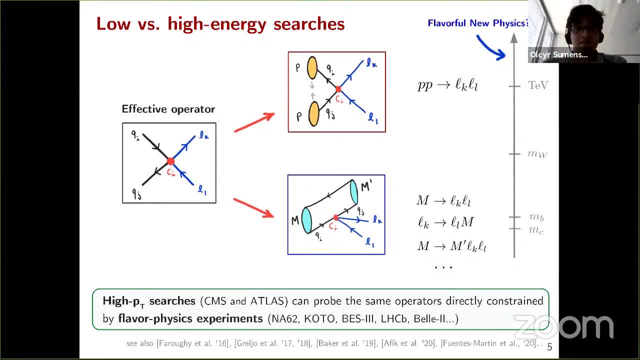 And the only assumption is that new physics is sufficiently heavy. And then this effective operator here with two quarks and two leptons can be constrained either by flavor, by some specific mass on the case, or by looking at proton-proton collision. 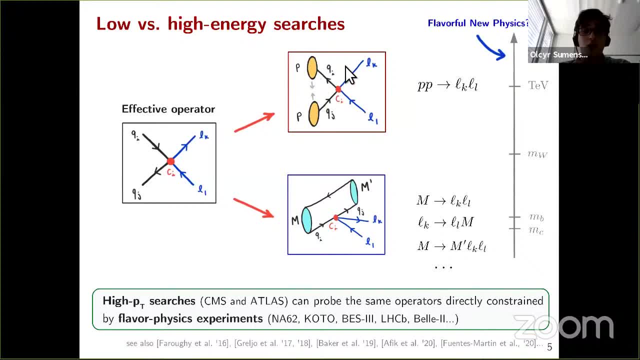 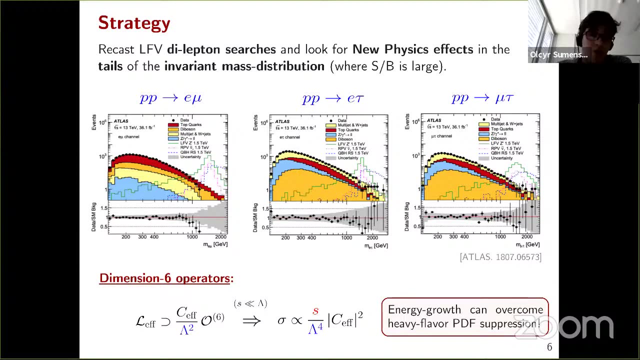 by this partonic interaction here, And then in the following I'll show how these two results can be very much complementary to each other. So this kind of analysis at high PT is possible because of a very simple argument, which is that when you have a dimension 6, 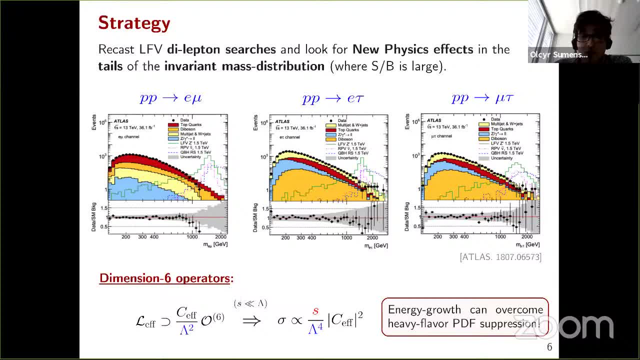 operator like the ones I mentioned before. if you compute this cross-section- assuming that the EFT is valid, you get something that grows with the square of the energy, And that's, of course, different from all the standard model backgrounds, since the standard model is renormalizable. 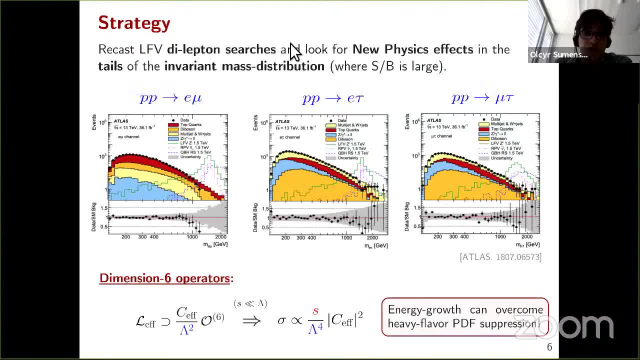 So what we do is to take data from proton-proton going to the different lepton combinations, and then let's say, we have a certain amount of energy And then we look really at the high energy beams, because here we know that signal over background. 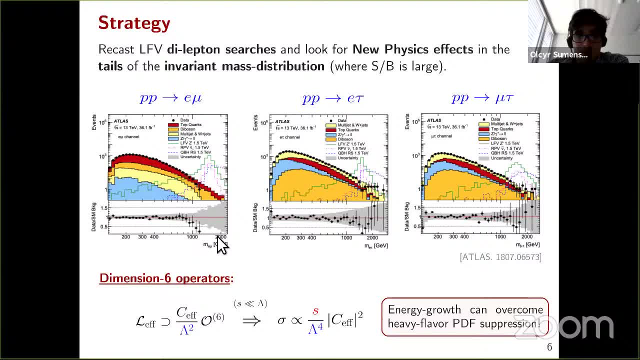 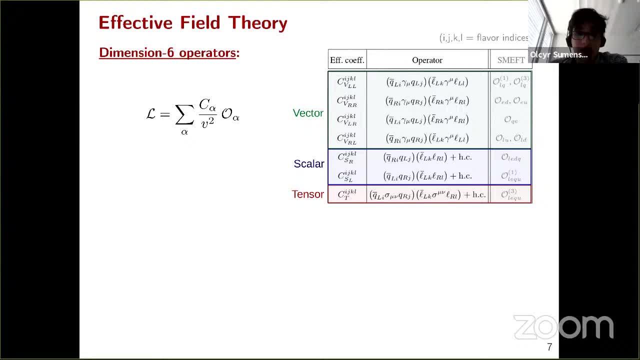 will be the largest possible And when you look into this, there are many operators that can contribute to these partonic processes. They are listed here in this table. So we think there's a standard model, EFT and also the broken phase, And basically you have vector operators, scalar operators. 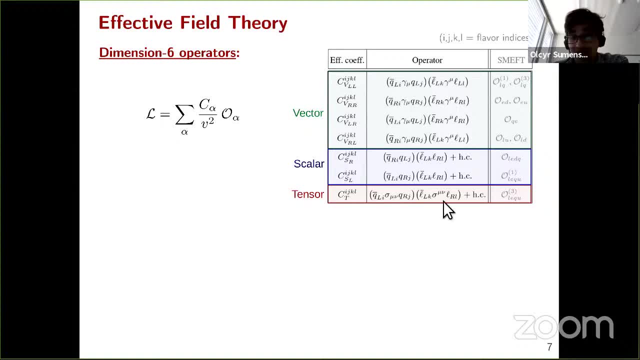 and tensor operators with the different chiralities. So you can try to compute this partonic cross-section And then you get this formula here. So we have this energy enhancement that I mentioned before for all these operators, And the funny thing is that they do not. 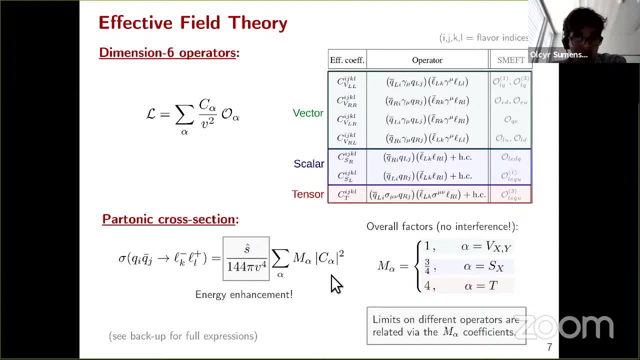 interfere with each other at high energy. That's useful input that I'll use in the following. So the only thing we're left are these multiplicative factors here that tell you how the limits on each of these operators scale when you compare them. So just a proportion. 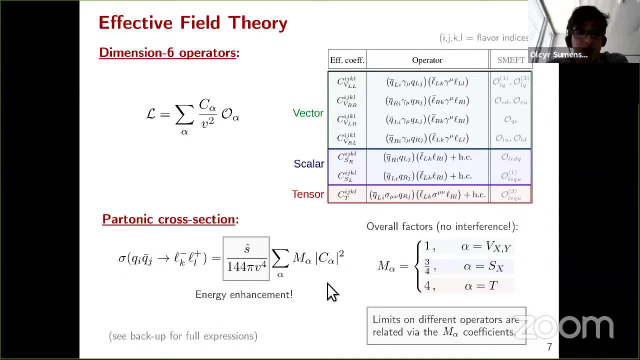 Just a proportional factor. This was for total cross-section, But then we have of course checked that when you impose the selection cuts from this experimental analysis, the total cross-section changes, But this proportion between the different contributions remain more or less the same. 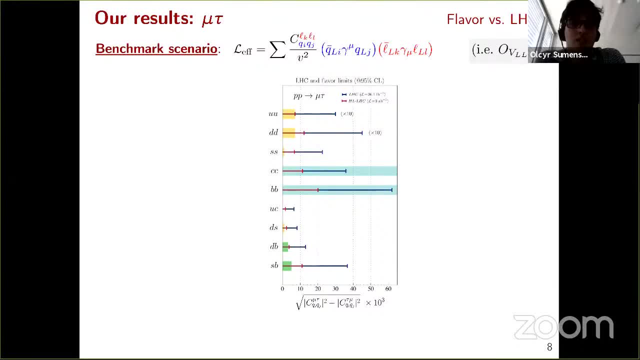 OK, so now let me show you some results. So I'll consider the tau to mu lepton flavor violation And I'll pick one example of operator, which is this: v minus a v minus a weight one, So factor with left-handed fermions. 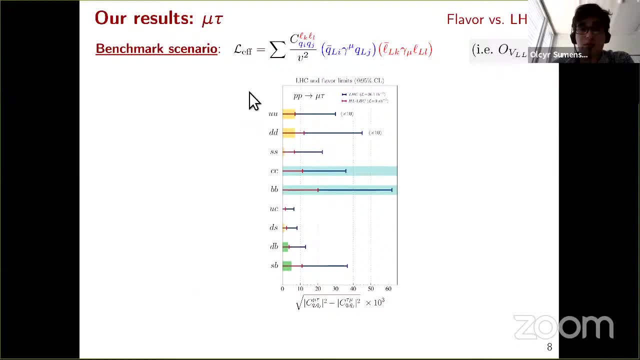 And here I have a Wilson coefficient with two quark indices and two lepton indices which are mu, tau. And then here you see the LHC limits that we get with current, in blue and red, future data for each quark transition And the colored bands here are the limits. 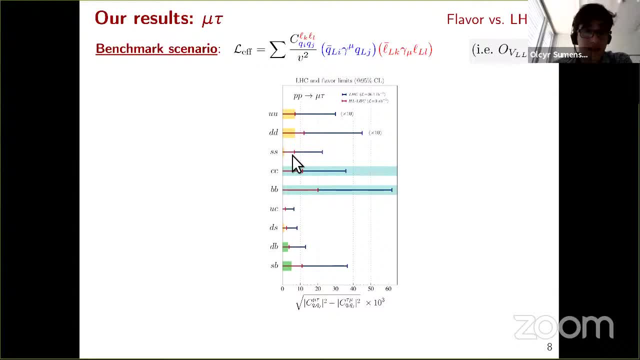 that we get from flavor physics observables. So what are these limits from flavor? So here for the light quarks, they come from tau decay, So tau to mu and some meson. So in the case of the B2S and B2D transition, 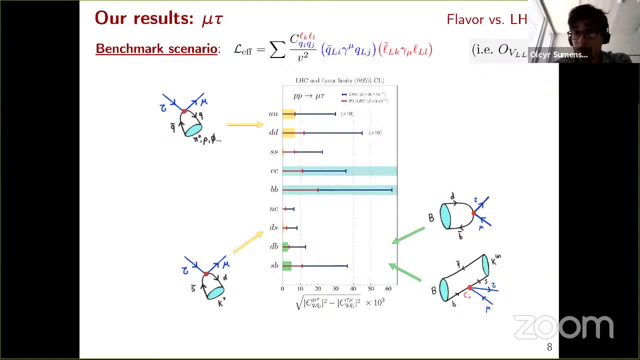 these are the case we just heard about in the previous talk. So leptonic and some other leptonic B decays, And there is also the quark flavor conserving transition. Here we have to use quark-coinean decay. so J psi. 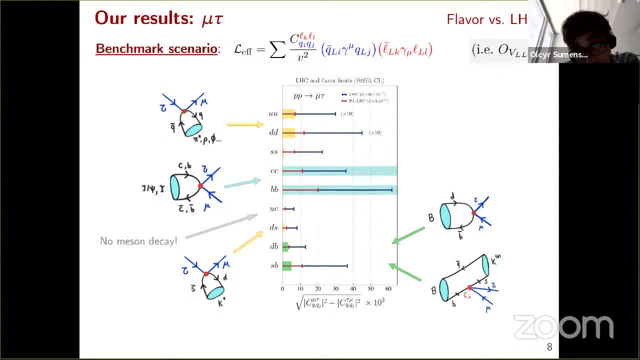 and oops And finally there is the Cu coupling And here actually there is no meson decay, just because it's not kinematically allowed. So the D and tau mass are too close So to allow you to have a decay. 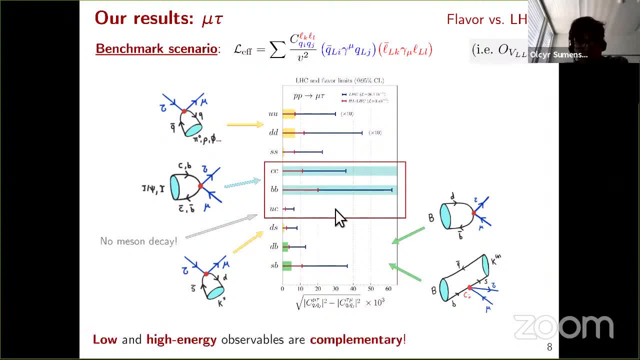 And what is interesting is that the limits are very complementary. So in many cases, like down here and up here, flavor does much better than LHC, But there are situations where LHC limits can be much more constrained than flavor. So these blue bands here, actually, 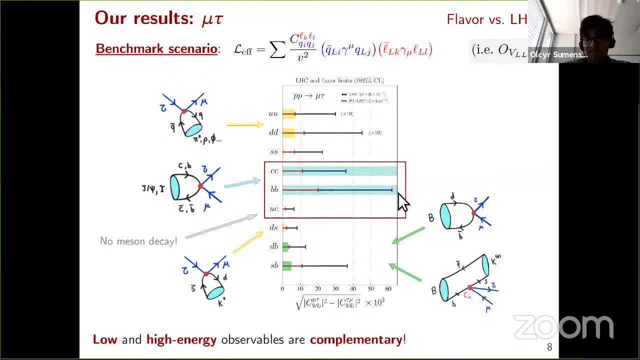 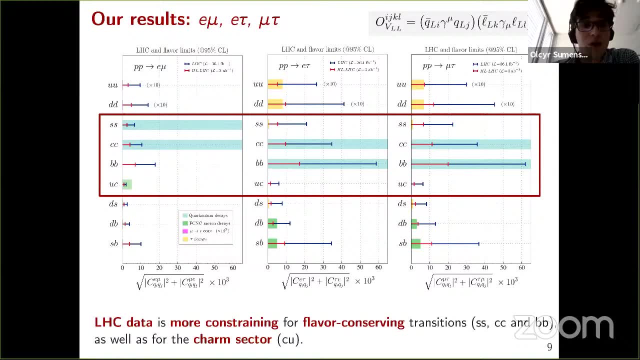 they extend beyond the picture so you don't see them. So they're very complementary And this remains true when you look at all the lepton transitions: E mu, E tau and mu tau, as you see here, Here in this plot. 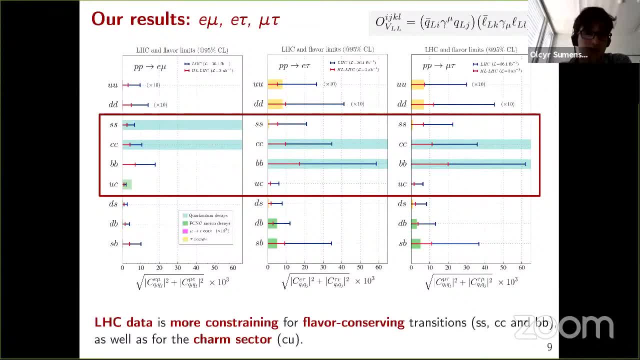 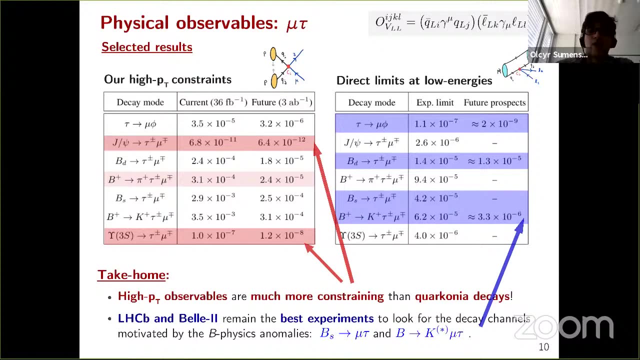 So the ones where LHC can give you some useful information are the flavor conserving transitions and also the charm quarks, sometimes because we don't have a meson decay, OK, So now just to give you a feeling of these results. 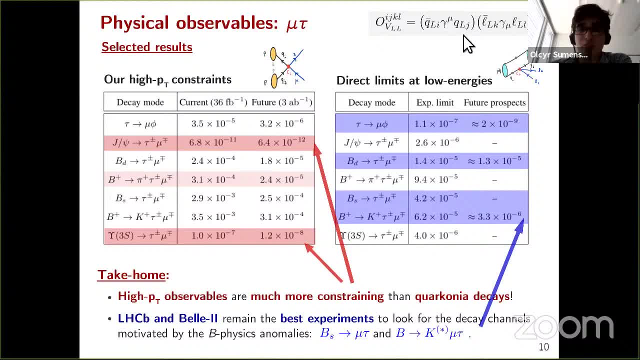 let me make a small exercise here. So again, let's assume this operator, And then let's take the limit that we get from high energies, the proton-proton collision, and let's just take this coefficient and compute a branching fracture that you can try to measure experimentally. 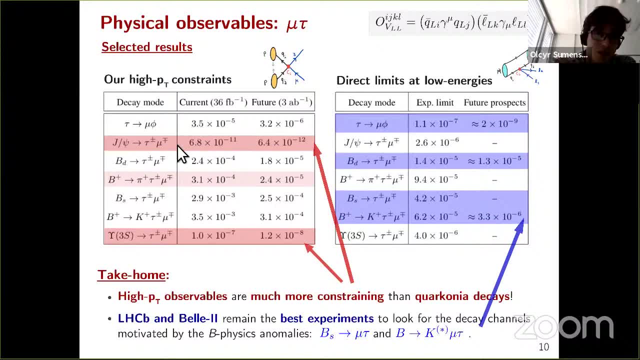 So for each of these decays here, we took the LHC limit and we saw what is the sensitivity that we're getting with LHC, assuming keeping this assumption. And these are the results that we compare here with the experimental limits today and the future prospects. 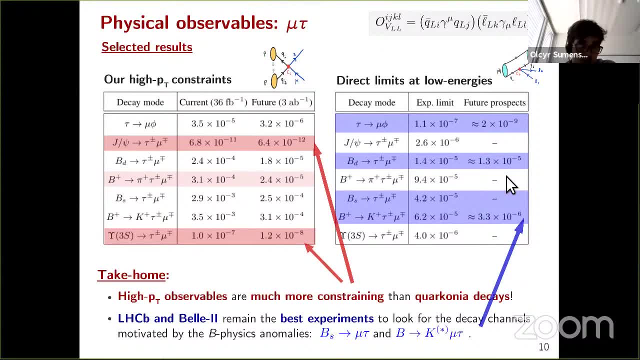 that we were able to find And the way to read this is: for example, if Bell 2 wants to improve the flavor violation test in oops non-decays, so they have to push these limits 4 to 10 to minus 6. 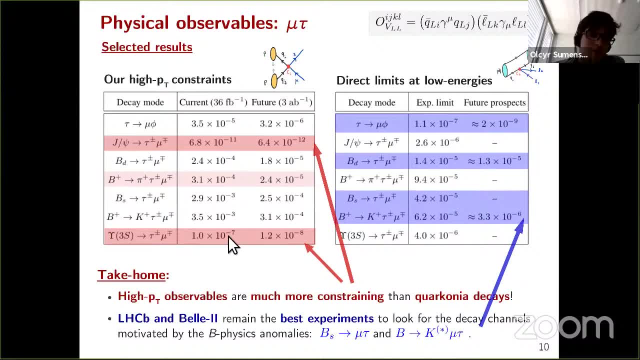 to be 10 to minus 7 to be competitive with what we have now, and then 10 to minus 8 in the future, And the color are actually the limits that are the most constrained ones. So you see, the things are very complementary. 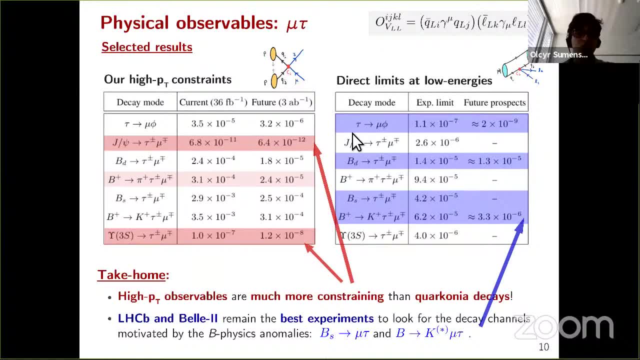 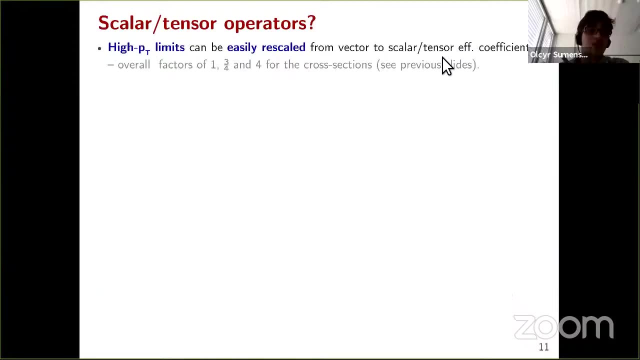 And it's very important to have both pieces of information. when you want to constrain your physics, OK, And of course, here there is an assumption, which is that I only have this operator, which is left-handed, And then you might ask what happens. 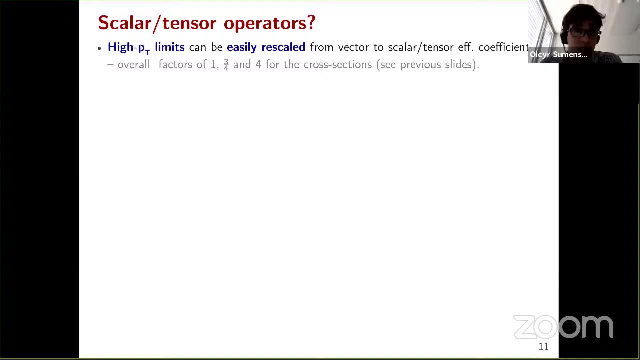 if the other operators are present, such as the scalar and tensor ones. From the point of view of LHC, it doesn't change much because, as I said, the cross-section changes by a factor of 1 to 3, fourths or 4.. 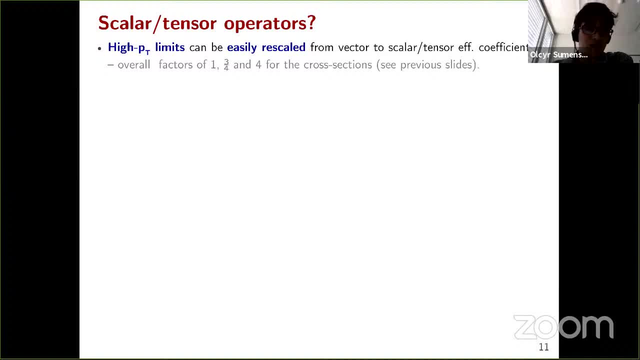 So there is small numerical factors that can be taken into account And we give you the number. OK, This is the full prescription in our paper. But for flavor things change a lot. So the choice of vector operators here was intentional, because here the comparison was easier. 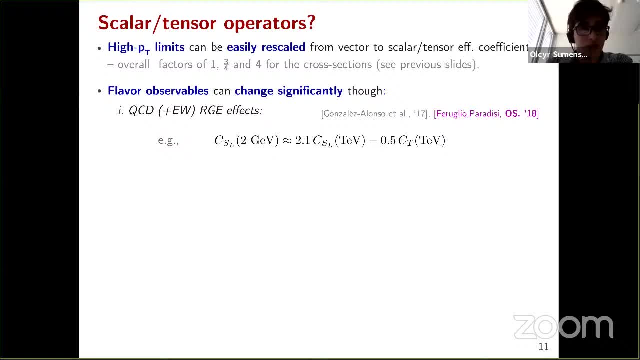 And we knew that in this case LHCb had a better chance to give meaningful results. But for the scalar operators the situation is a bit different. First, because when you run these operators from the TV, scale down to the few GV, but you 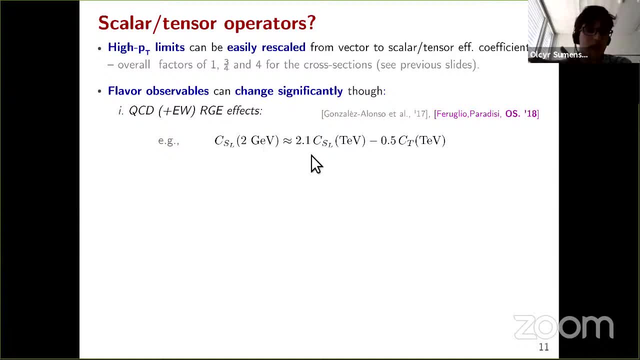 try to measure these decays, you see that for the scalar operators we have an enhancement, And also scalar and tensor operators can mix by an electric run. So that's one factor And the second one is chiral enhancement, because when you look at pseudo-scalar mass, 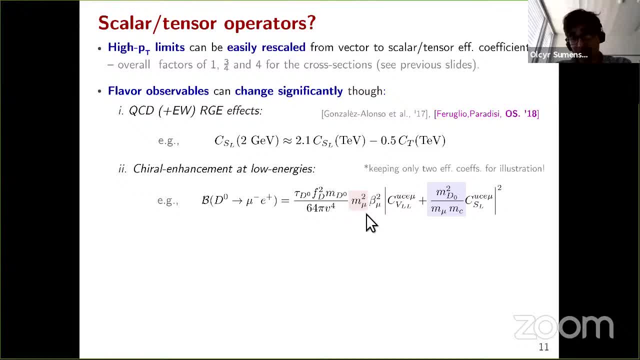 on the case with a vector operator, they're going to be suppressed by the laptop mass. But as soon as you turn on the scalar operators, there is a chiral enhancement of order md over mu, which is huge and that can improve the signal. 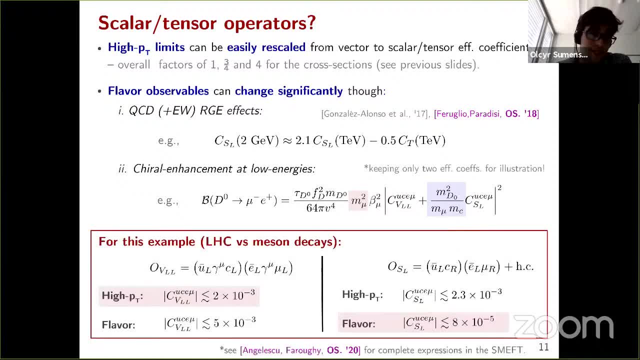 So just to give an example, if you look again, this d0 to mu e decay for the vector operator. we found that high PT was a bit more constraining than flavor. But for the scalar one flavor is much better. so a factor of 10 more. 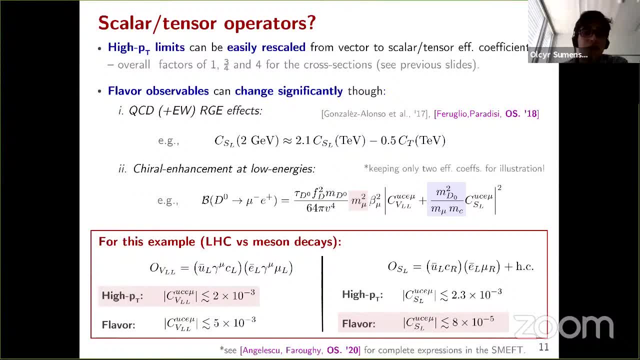 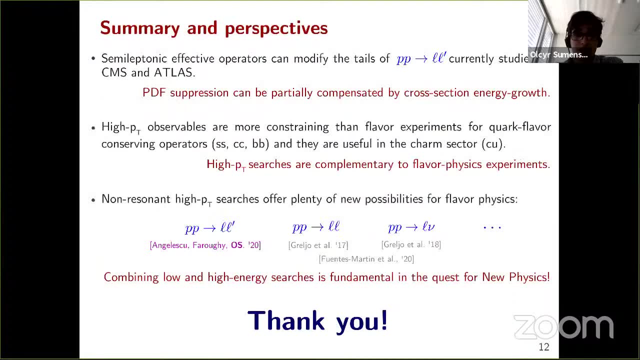 So this tells that flavor and LHC are complementary, not only about the transitions that you can probe, but also the chiral structure of these operators. So that's one factor. Thank you, And that's all I wanted to say. So the brief summary is that there 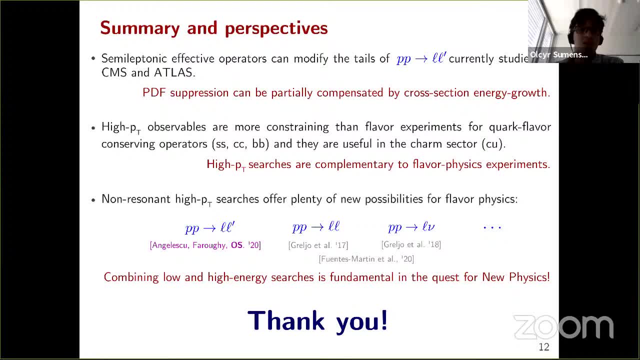 is a lot of possibilities to do flavor physics at the high PT. So today I spoke about this PP tool- leptons with different flavors. But there are other publications that studied dilapidons with same flavor or the monolapton signatures, and they 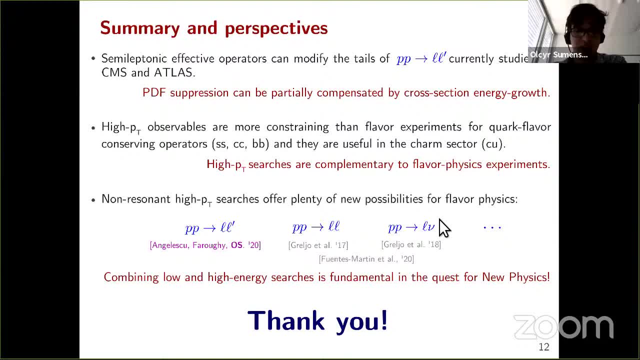 were motivated by other problems, such as the B anomalies or charm physics, And so these are all meaningful constraints that should be combined, And also combined with what we have for flavor when we try to look for new physics, in order to be the most sensitive to it. 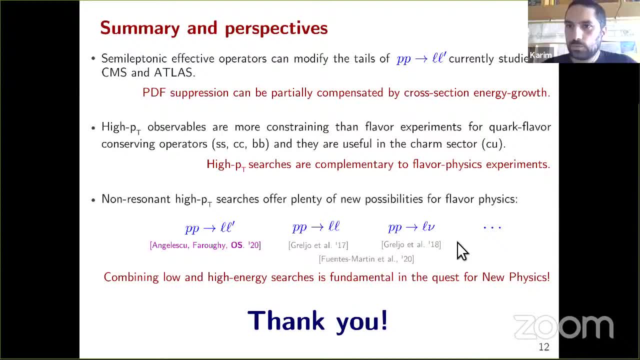 Thank you very much. Thank you. So any comments or questions from the audience? I do not see any, OK, so maybe I can ask you something. So I think, OK, everybody, given the anomalies, let's say, is focusing mostly on the mu tau because, of course, 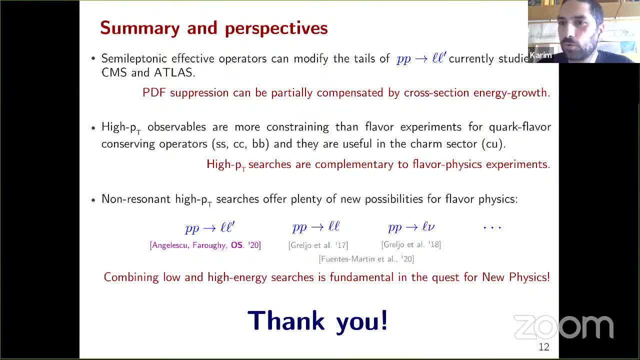 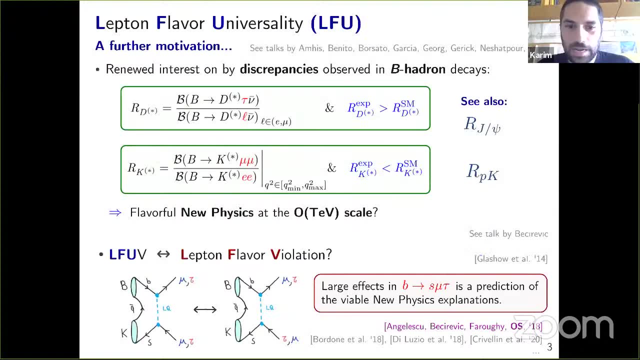 it should. if there is any lepto, quark or similar, it should couple, let's say, more likely with the heavier leptons. But I was wondering how suppressed it would be if you said that it would couple. Yeah, So, for instance, I mean looking at the same particle- 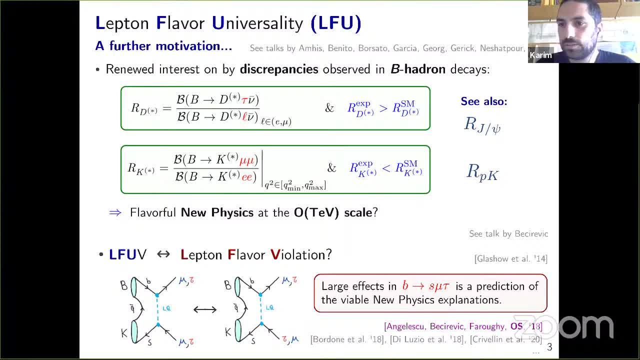 with the muon electrons instead of muon tau? is it that strongly suppressed? How much So? yes, the point here is that to explain the B anomalies we need a large coupling to the tau and a slightly smaller coupling to the muons. 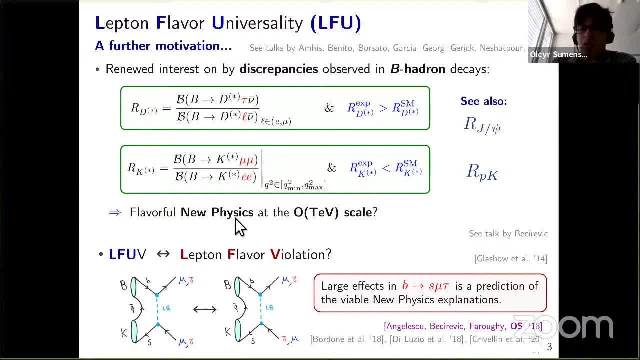 So when you compute these rates, you get not only an upper limit on this B2S mu tau, but also a lower limit. Now, when you think about the electron and muon transition, there, we have also an upper limit that you can compute. 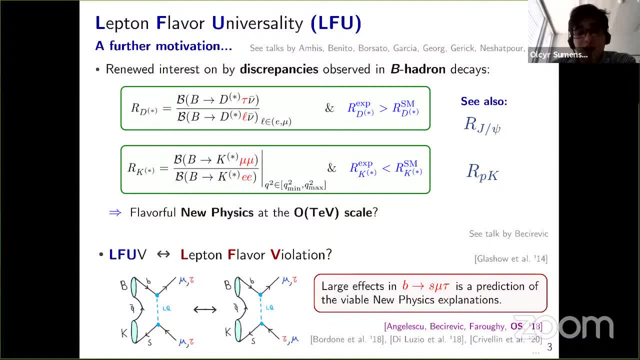 if you assume that you have a coupling to the electrons, But there is no lower limit, because the couplings to electrons could be super suppressed because we have no hint of muon physics there. So I think it's important, of course, to push these limits, because they're always useful to have. 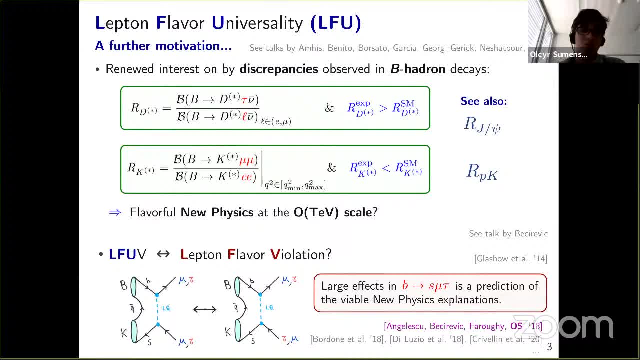 a feeling of, if the anomalies are confirmed, what is the pattern of labor that we should have in these lepto quark couplings? OK, But it could be that super suppressed that we've never observed. OK, But let's say it would be a kind of fine tuning I guess. 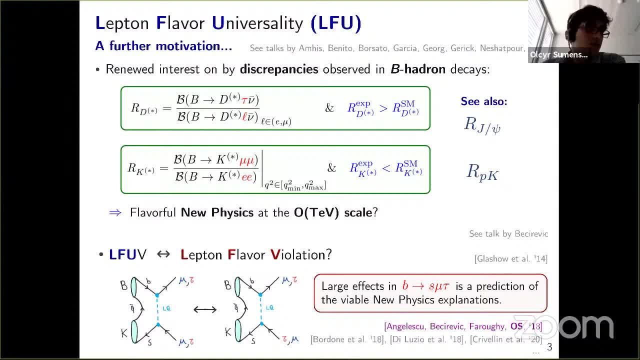 In any case, OK, Well, not a fine tuning, because I mean so. look the UCAOs in this under model. they're very hierarchical and they're bigger to the third, second than first generation, So you could have something similar here. 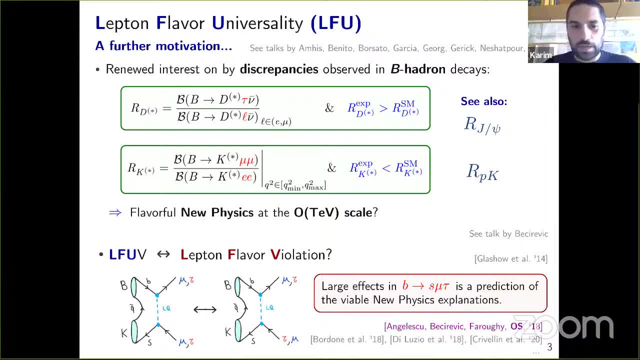 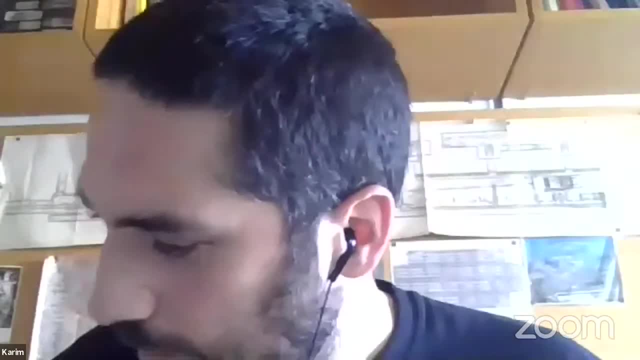 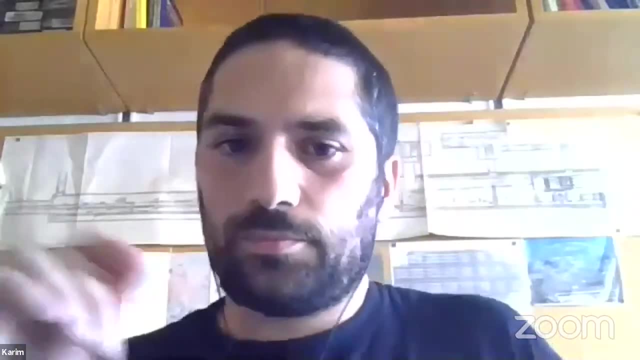 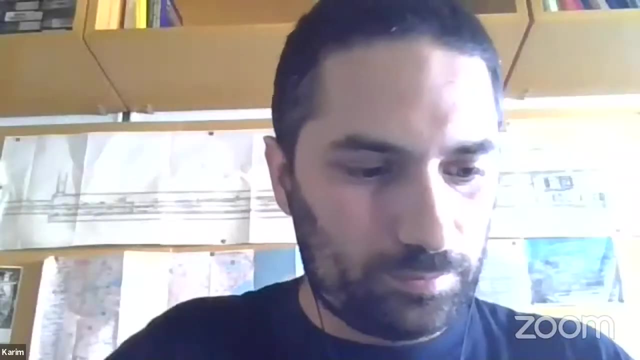 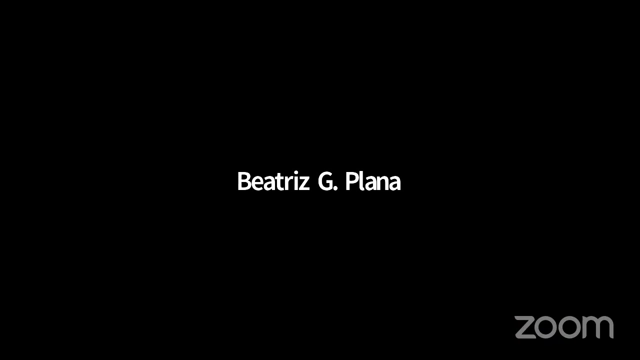 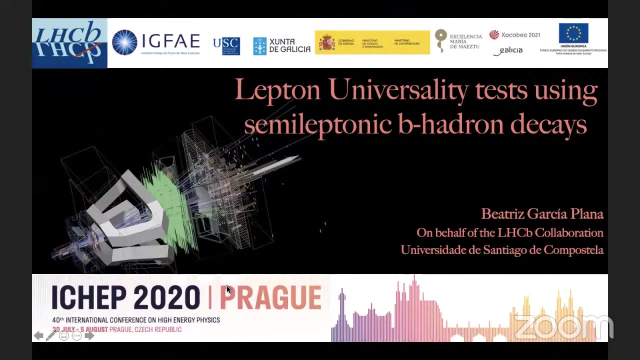 OK, OK, thanks a lot. OK, so I would propose to move on. And now there is Beatriz Garcia Plana with the universal, with the semi-electronic BDKs at LHCb. Yes, hi, Hello, do you see the screen? 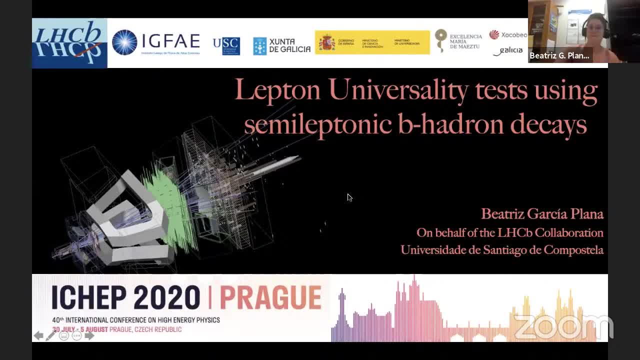 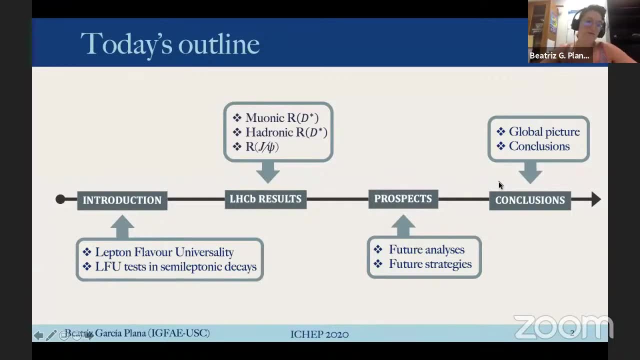 Yes, OK, OK, you can start. So good afternoon to everyone. Today I will talk about lepton universality test using semi-leptonic B hadron decays. This is the outline of my talk. First I will make a small introduction. 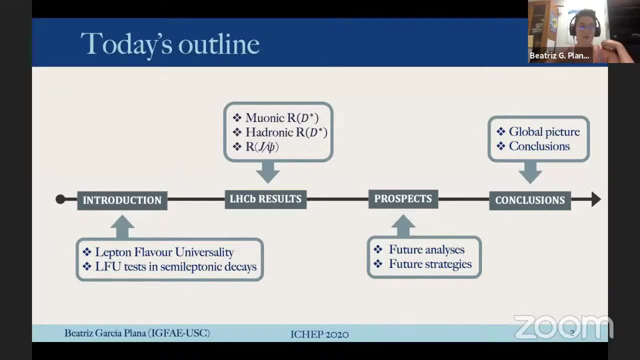 about the concept of lepton-flavored universality and how we can test it in semi-leptonic decays. OK, Then we will move on to LHCb results. In particular, we will see the muonic RD star, the hadronic RD star and the RGF side. 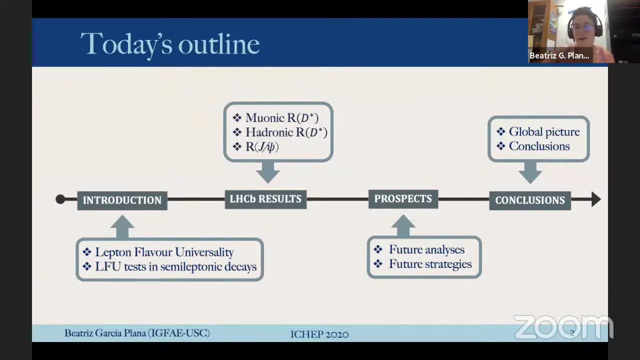 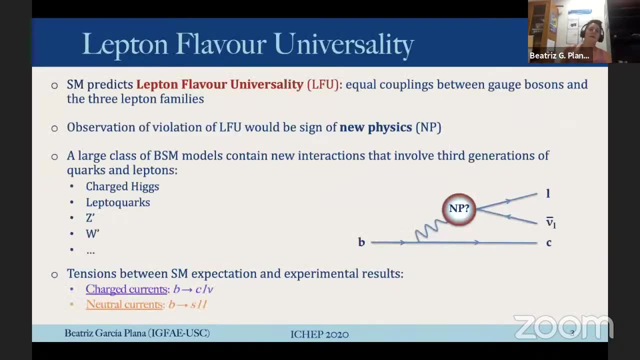 Then we will see some future analysis and future strategies And we will end up with the global pictures and some conclusions. So within the standard model, the electroweak coupling between the gauge bosons and the leptons are independent of the lepton family. 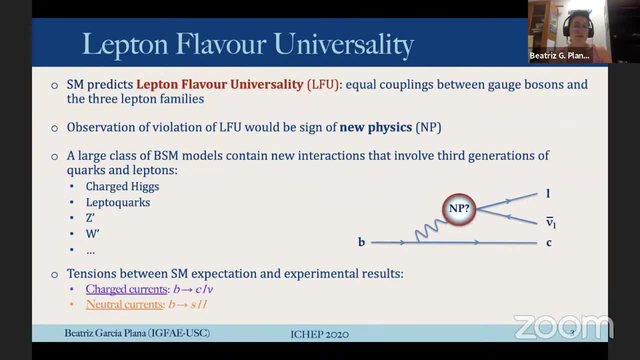 And this is called lepton-flavored universality. OK, OK, LFU is one of the main ingredients of the standard model And therefore any sign of violation would be a sign of new physics. Actually, it exists many models beyond the standard model. 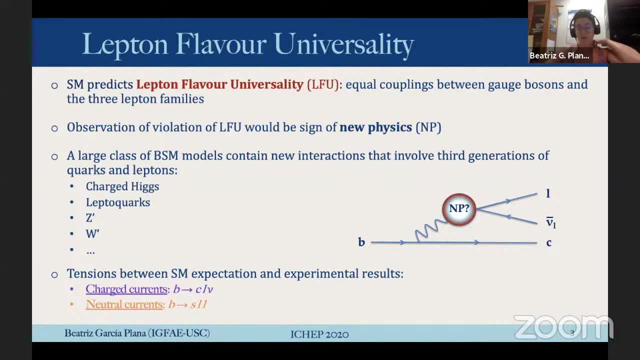 that contain new interactions that involve the third generation of quarks and leptons, such as chart hits, lepto quarks, Z-prime or W-prime. There have been done many searches of this violation And, in particular, we studied two different kinds of trials. 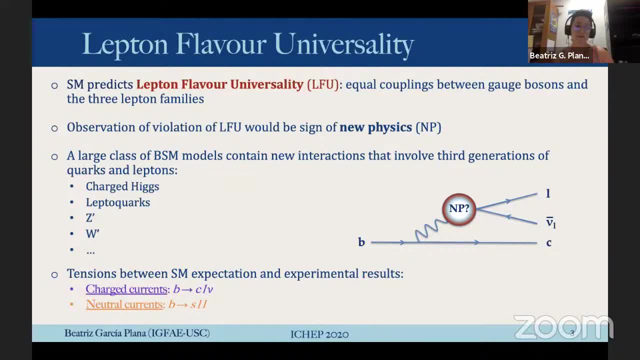 We have a theory of some kind of transitions within charge currents, So B2C, lepton neutrino, and in neutral currents. we studied a B2S LL transition. In this talk I will just cover the charge currents one. 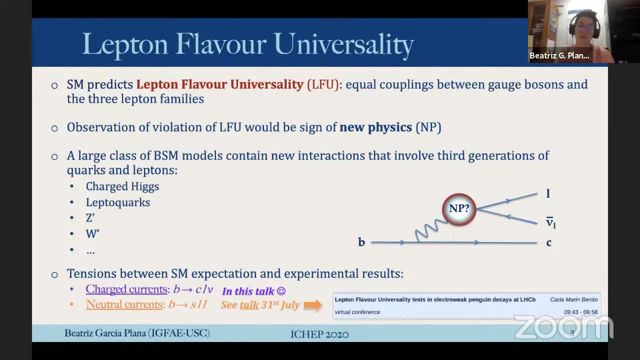 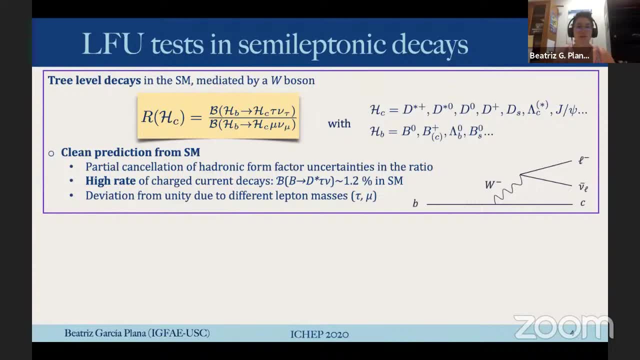 But if you want to learn more about neutral current, don't miss the talk of Carla on the 31st of July. So why semileptonic decays? Semilitonic decays offer us a good scenario to test leptons, to test the electron-free universality. 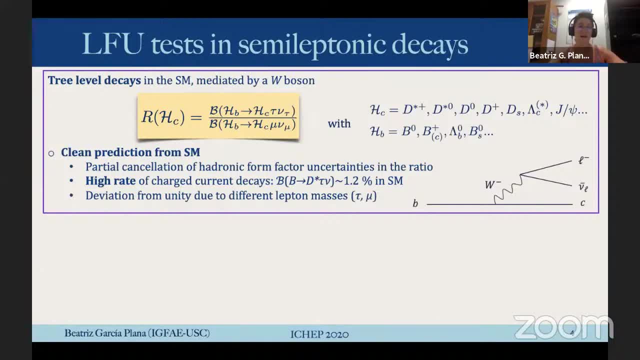 And this is done by means of the coefficients R, H, C, which is defined as the fraction of a B Hadron going to a C Hadron tau nu, with respect to the branching fraction of the same B Hadron going to a C Hadron mu nu. 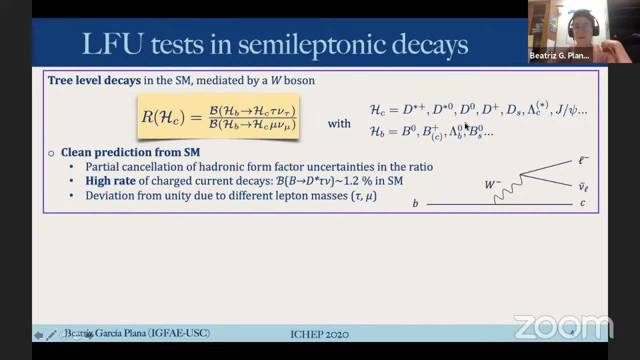 Where a C Hadron could be D or D star D zero D plus D S lambda C, gypsy, and a B Hadron could be a B zero D plus lambda B, et cetera, And this is a tree level decay mediated by a W boson. 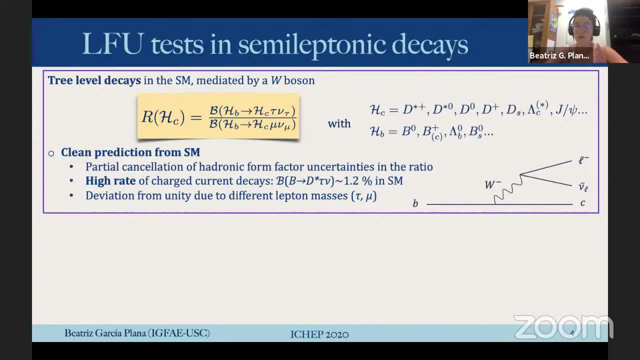 And therefore if new physics, coupled just to a third generation, this kind of transition, are sensitive to new physics component at the tree level. There are many advantages from the standard model. First, it's partial constellation of Hadronic fault factors in the ratio. 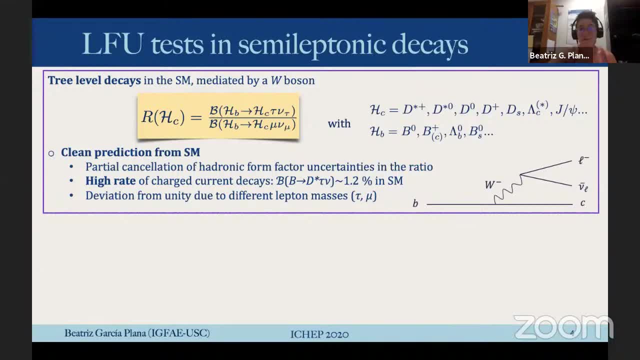 Then the high rate of charged current decays. for instance, the branching fraction of B going to the star tau nu is about 1.2% in the standard model. Then another aspect that I want to comment about these coefficients is the deviation from unity. 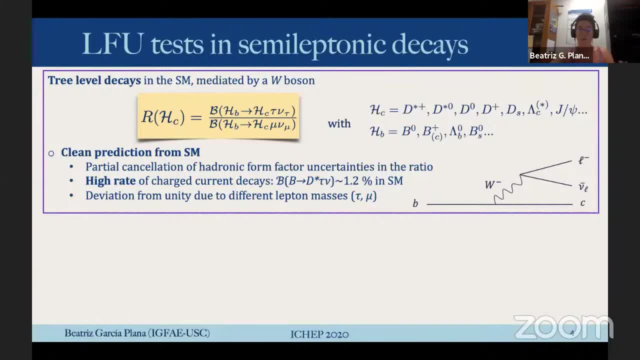 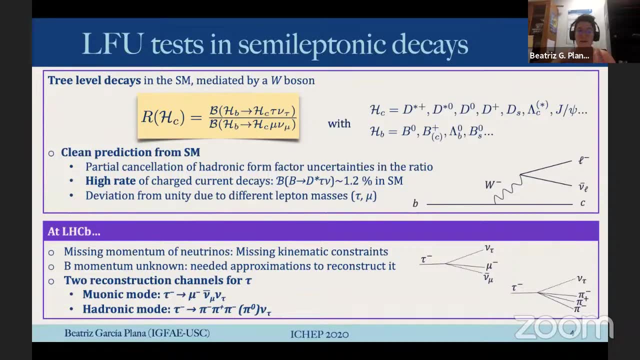 due to the different lepton masses between the tau and the mu. What happens at LHCb is that these kinds of measurements are very challenging because we are dealing here with neutrinos and therefore with missing kinematic constraints. So in order to obtain our beam momentum, 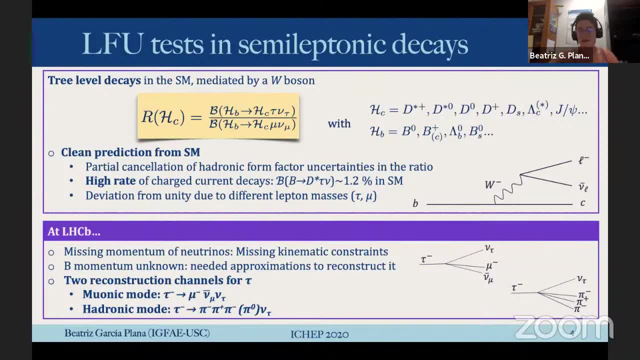 we need to make some approximations And we will see in the next six slides how do we do it. So basically we have two reconstruction, two decay channels for the tau, the muonic mode in which the tau decays in muon, and two neutrinos. 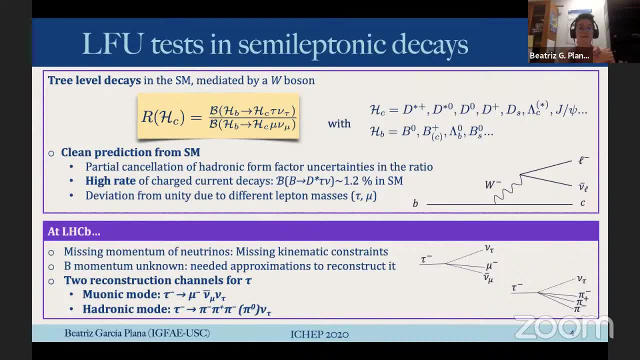 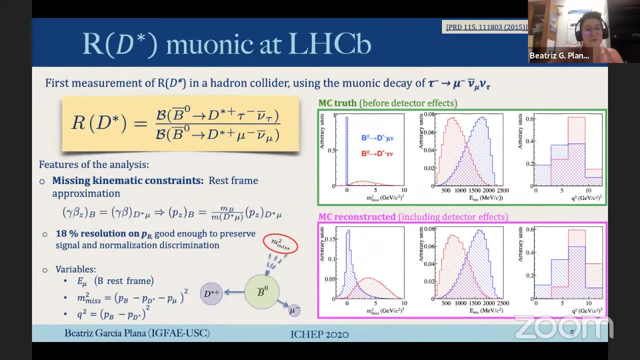 and the hadronic mode in which the tau decays in three pions, a pi zero and a neutrino. The first measurements of Rd star in a hadron collider was done using the muonic decay of the tau, So the tau going to mu and two neutrinos. 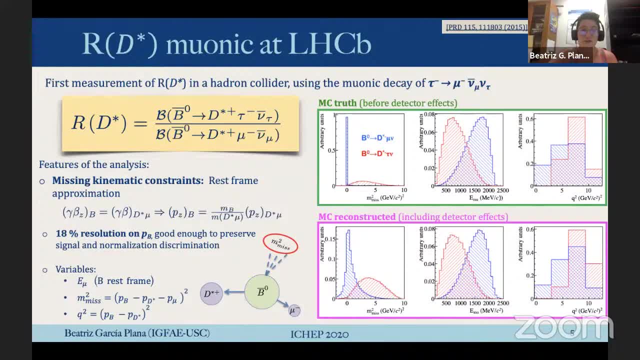 And here the coefficient Rd star is defined as the branching fraction of V zero going to the star plus tau nu, with respect to the same decay but with a muon. Some features about this analysis is that, since we have missing kinematic constraints, we have to make what is called the rest brain approximation. 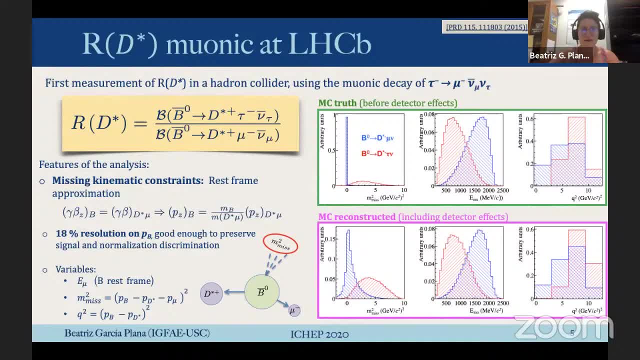 So here the momentum of the final visible state, so the d star and the muon, is scaled by the mass of the V with respect to the mass of the final visible state. With this approximation we obtain a resolution of 80% on the momentum of the V, which is good enough. 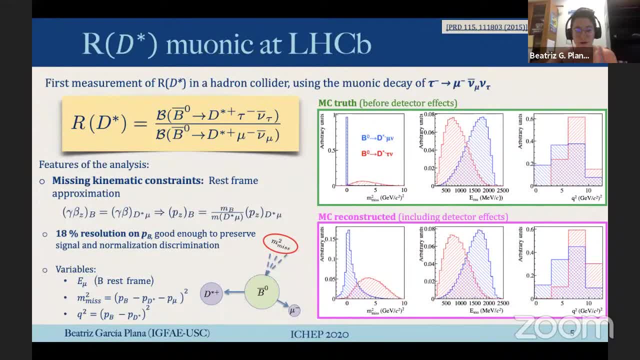 to preserve signal and normalization discrimination. We can see this on the right. So in green we have the projections of the variables in mass, the energy of the muon and q square, which are the ones with most discriminating power. So in green we have the Monte Carlo truth. 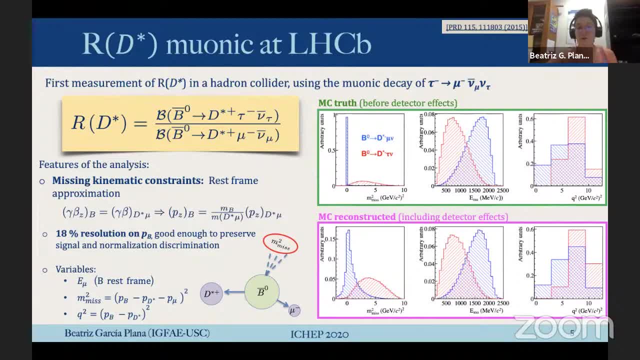 And in pink we have the Monte Carlo reconstructed. So it means after we include the detector effects. So here we can see that we can differentiate between the signal component and the normalization one, For instance for the missing mass. in the case of the normalization 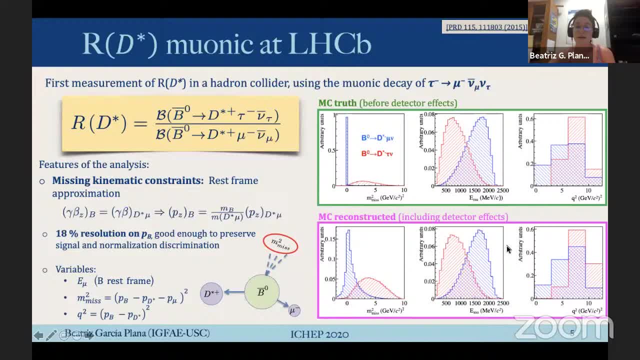 it's 0.5.. It's a spectrum. it's picking in 0.. In the spectrum of the energy of the muon, it's harder And it rains from 0. in the q square variable, In order to obtain our coefficients at the star. 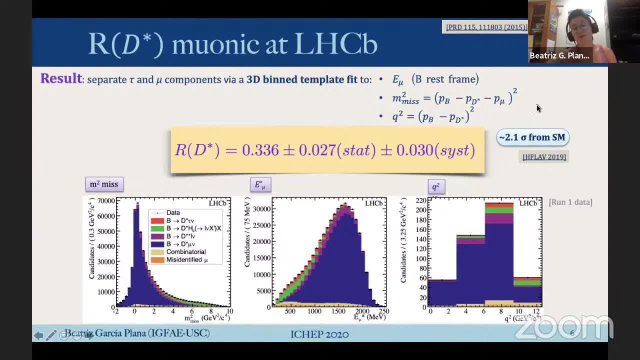 we perform a three-dimensional fit to the variables that I just present. so the energy of the muon, the missing mass and q square. And here we have the projection of the three-dimensional fit. In red we see the signal component. 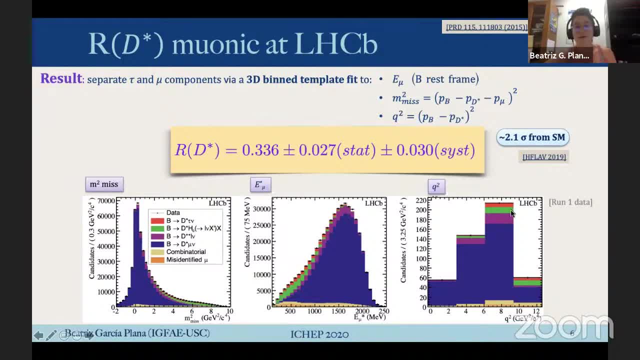 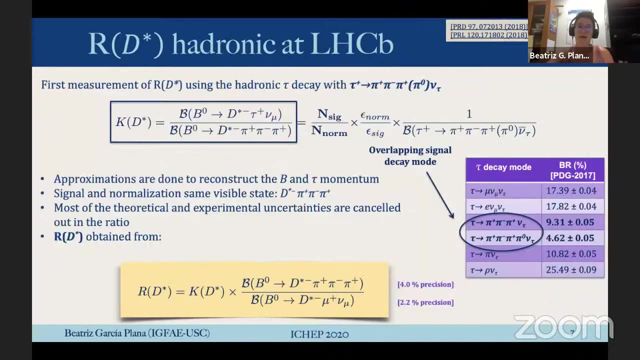 And in dark purple we see the normalization one. So this was the result that was obtained for the R1,1,, which is in tension with the standard model prediction at the level of 2.1 sigma. Let's move on now to the RDSTAR hadronic. 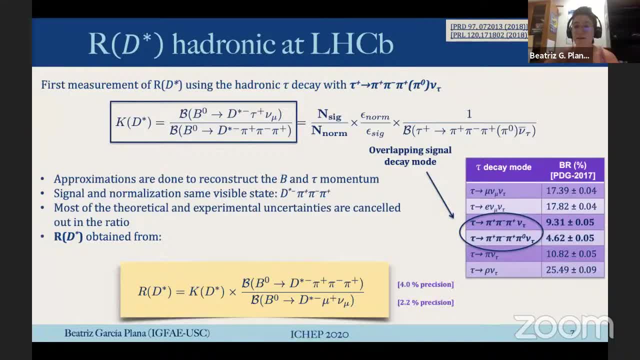 Here the tau decay is in three pions: pi zero and a neutrino. And this is the result. Let's move on now to the RDSTAR hadronic. Here the tau decay is in three pions: pi zero and a neutrino. 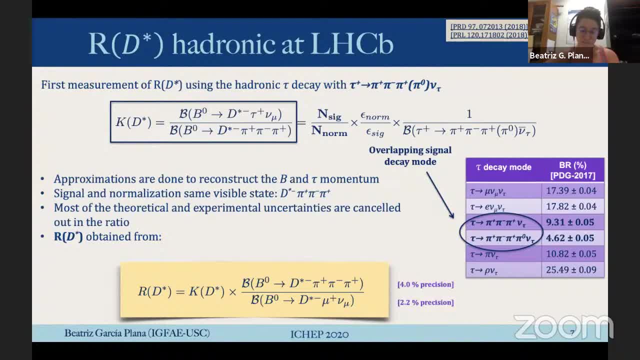 And therefore we have our overlapping signal decay mode. Actually, what is measured here is the coefficient that I call kappa, And in order to obtain it we need to measure the signal yield, the normalization one, and correct them by the ratio of efficiencies. 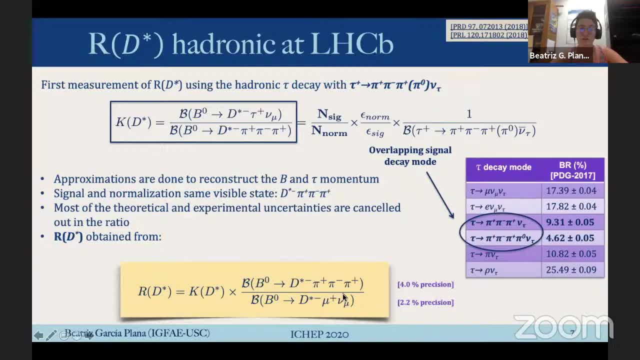 Again, we need to make some approximations in order to reconstruct the V and the tau momentum. An important feature about this analysis is that the signal and normalization time share the same visible state. So this star and three pions, And therefore most of the theoretical. 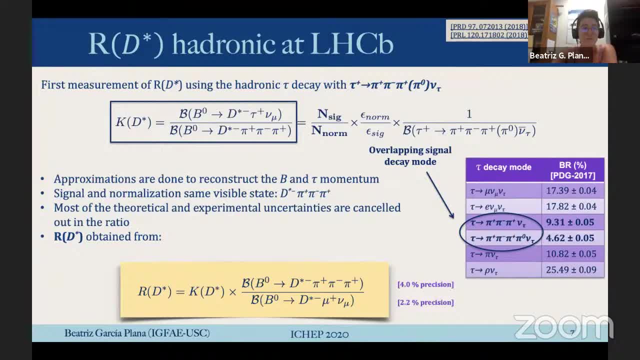 and experimental uncertainties are canceled out in the ratio. Once we have the kappa coefficients, RDSTAR is obtained by multiplying it by the external inputs, which are well known, with a four and 2.2 precision. So in order to obtain RDSTAR, 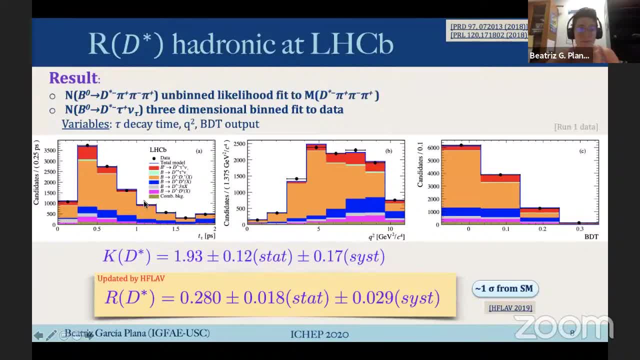 we perform a three-dimensional fit. We have here the projection of the tau decay time: q square and b dt. In red we have the signal component and in orange the main background. So this is the result that was obtained, which is in tension with the standard model prediction. 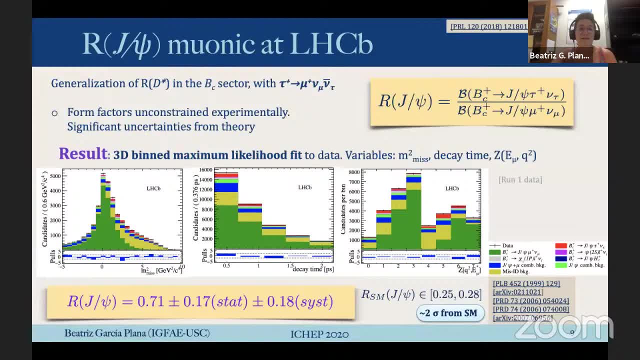 at the level of one signal. Then we can generalize the analysis that we have done for RDSTAR in the business sector And we obtained the RGPSI coefficient. The measurement that was done was done using the tau decay decaying in muon and two neutrinos. 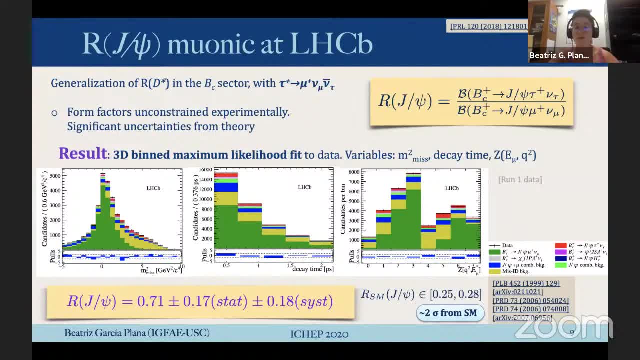 And in order to obtain our coefficient RGPSI, we perform a three-dimensional fit in the missing mass, the decay time and set, which is a variable that depends on the energy of the muon and q square, And the result that was obtained is in tension. 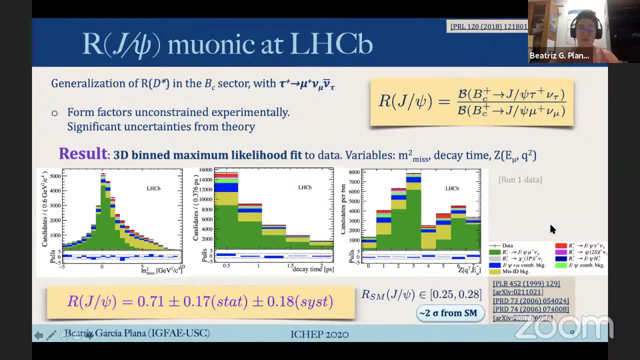 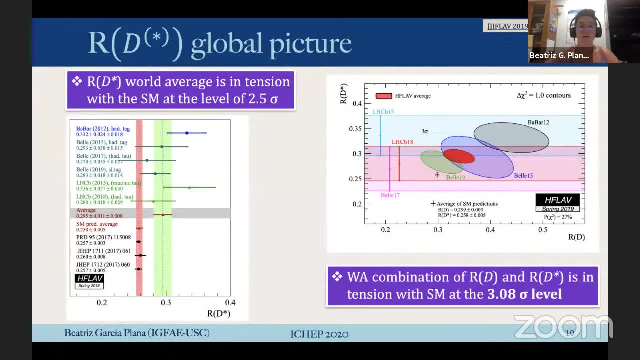 with the standard model at the level of two signals. So we have a three-dimensional fit in the missing mass, depending on which theory you are taking. So we may wonder now which is the global picture. In the case of RDSTAR, we have in the lab the different experimental measurements. 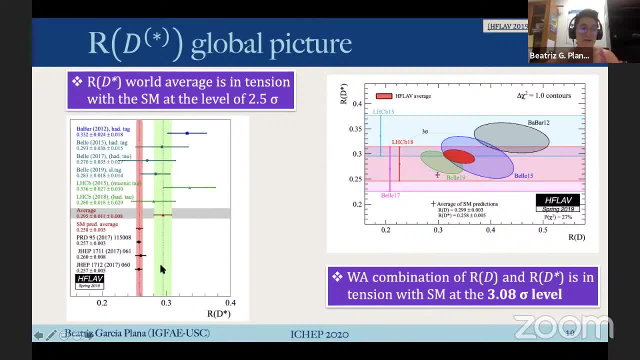 So the one corresponding to Babar, three from Bell and two from LHCb, which is the green bar, And then we have the standard model prediction, which is the red one. So the RDSTAR world average is in tension with the standard model prediction. 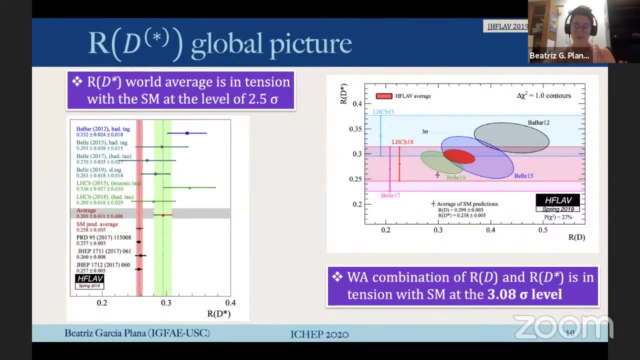 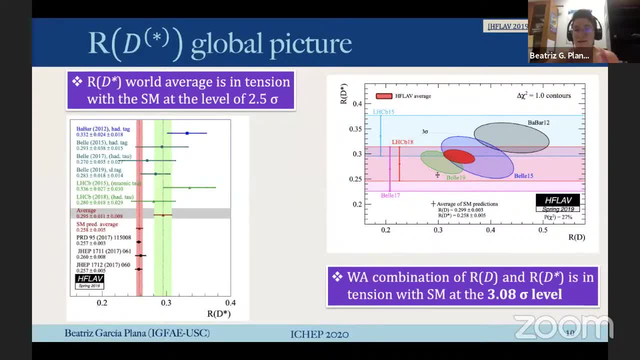 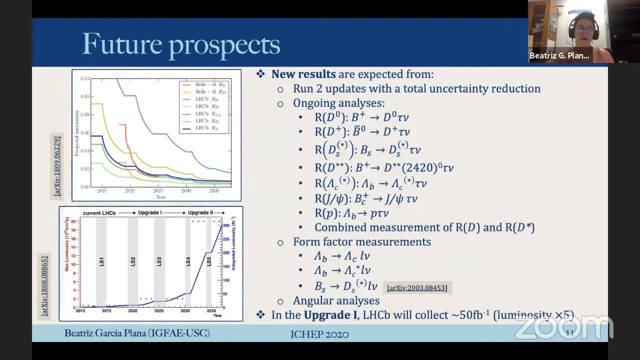 If now we take into account all the RD and RDSTAR measurements, we have the average in the red ellipse And if we compare it with the standard model prediction, we see that overall it's in tension at the level of 3.08 sigma level. 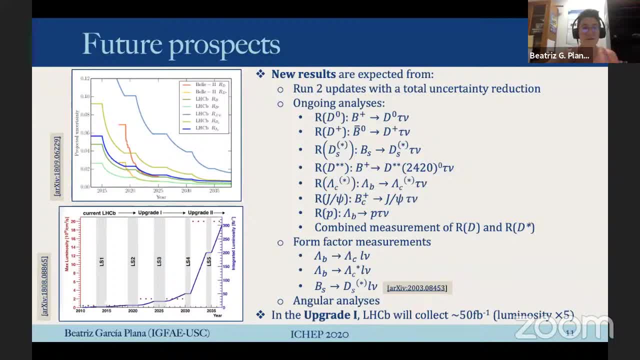 Some words about the future. Here we have the projected uncertainty for Bell and LHCb for all our our measurements. Here we have the projected uncertainty for Bell and LHCb for all our measurements. For instance, we can compare the two orange curves. 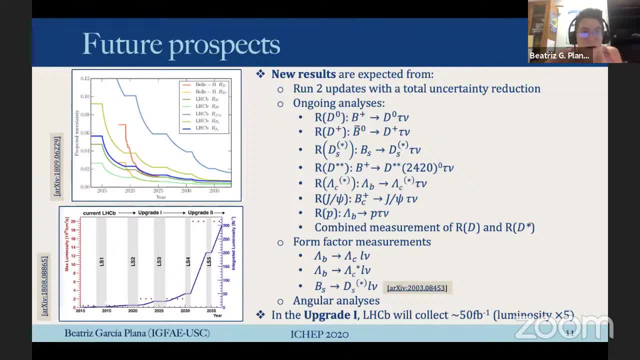 which are course, which correspond to the Bell RD and RDSTAR prediction, And we can compare it with the one from LHCb. that are the two green. So it's expected that both experiments will be comparable in the future. Then we are expecting new result coming from updates. 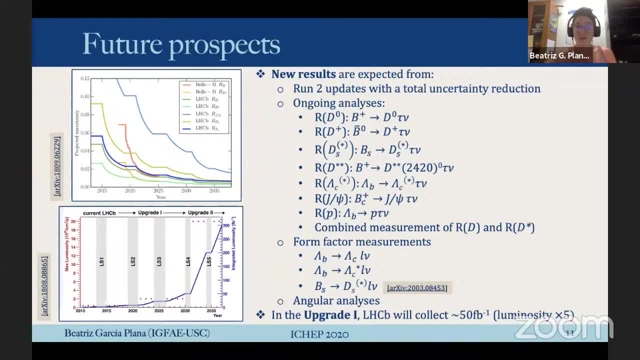 or using the RUN2 of all the analysis that I just present- And there are many analysis ongoing, So Rd0, Rd+, Rds, et cetera, And also combined measurements of Rd and Rd star for both the hadronic and the muonic mode. 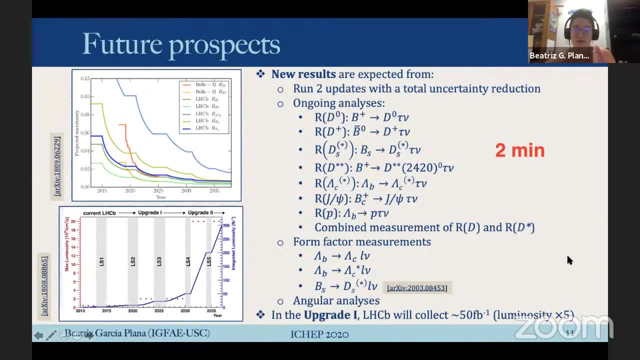 Then it's planned to perform some form factor measurements And in particular the Vs going to Vs star. it's already done. Then some angular analysis And in the future, after the upgrade one, it's planned that LHCb will collect 50 inverse Fentor. 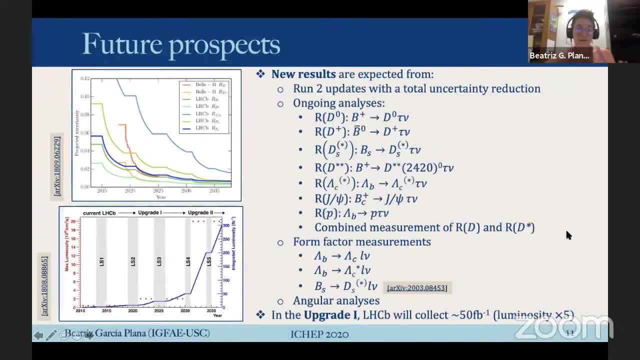 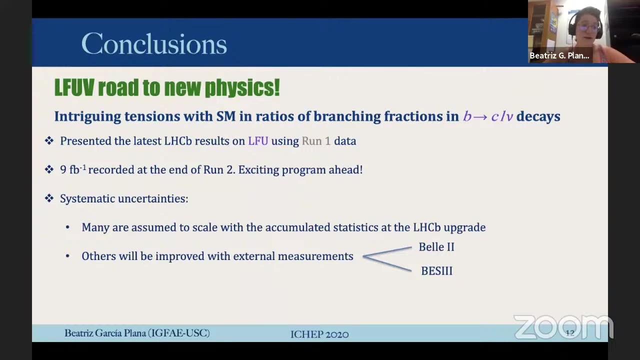 And we see here the projection of the integrated luminosity. So it means that we will have a five times more luminosity than what we have at the end of the RUN2.. Conclusions: we have seen that Leighton-free universality violation. it's a clean road to new physics. 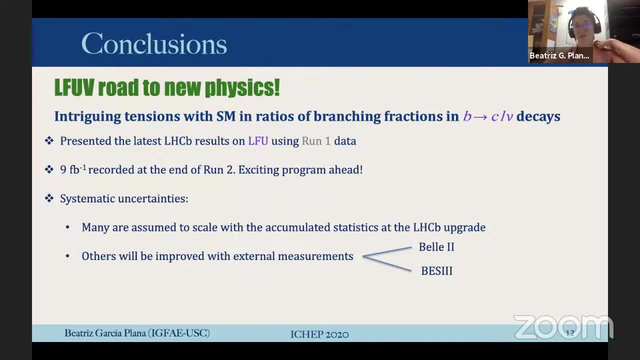 They're entering tensions with the standard model in the ratio of branching fractions in B2C leptoneutrino decays. All the results that they present here were done using the RUN1 data And we have nine Fentor bars in bed at the inverse. 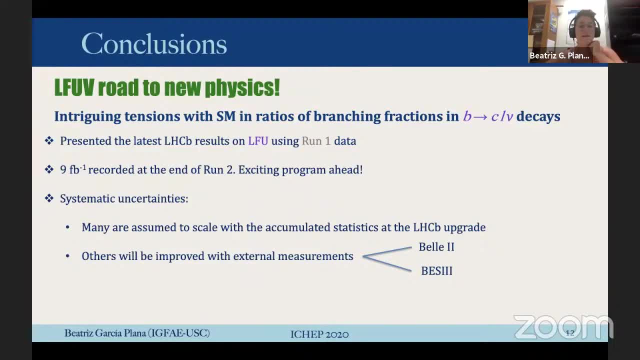 at the end of RUN2.. So there is an exciting program ahead. About the systematic uncertainties, many are assumed to scale with it. Some will scale with the accumulated statistics and others will be improved with external measurements, as the one coming from B2 or B3.. 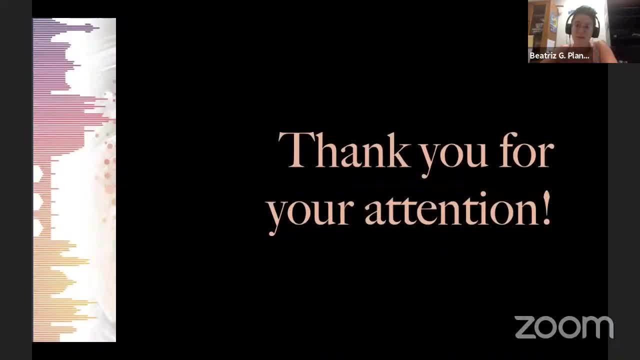 So stay tuned And thank you very much for your attention. Okay, thanks a lot. So any comments or questions from the audience? Hello hi, Yes, please. So I want to know if there are any updates on the experimental side. 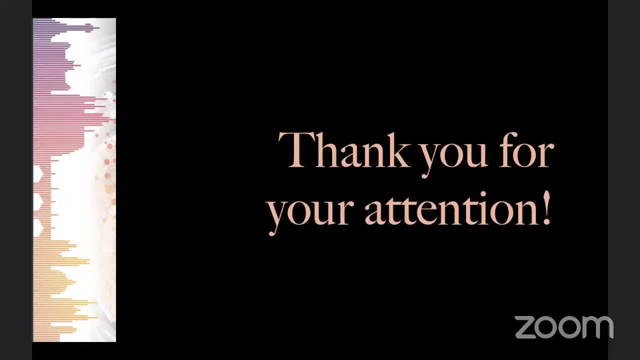 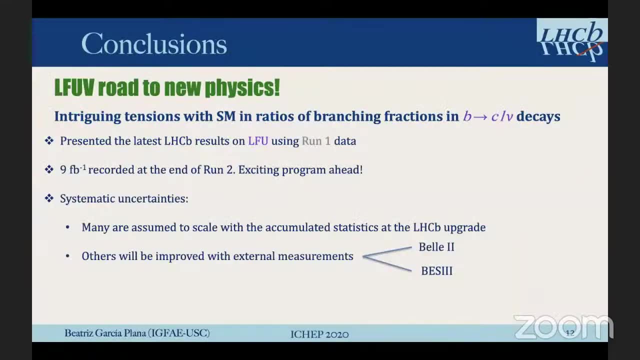 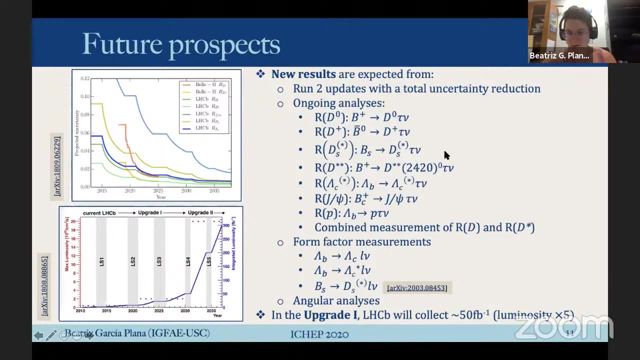 In the measurements of this BS2, DSTAR, the new leptoneutrino testing in those vehicles. I don't hear you well, but I think that you were asking for this coefficient, the RDS, right? Okay, so it's ongoing already. 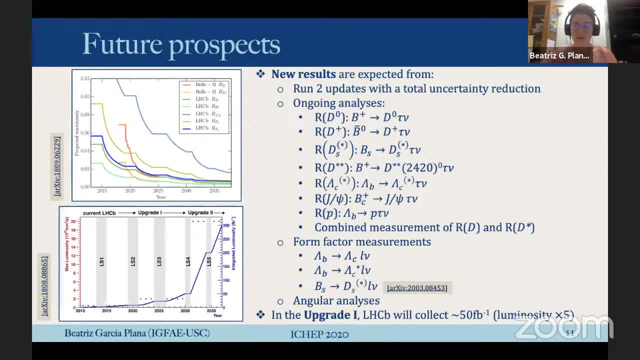 So I don't know exactly when it will be finished, but next year probably. Thank you, Okay. thanks a lot. If there are no other comments or question, I would move on. I don't see any other, So thanks again. 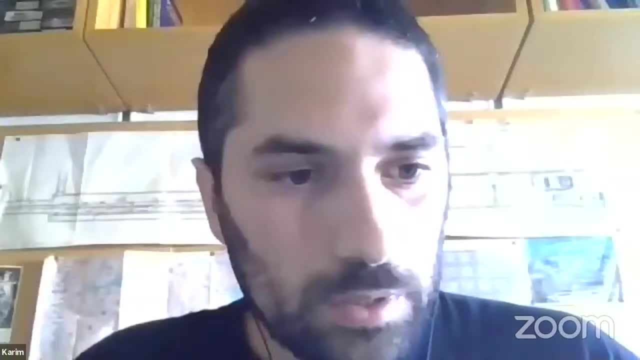 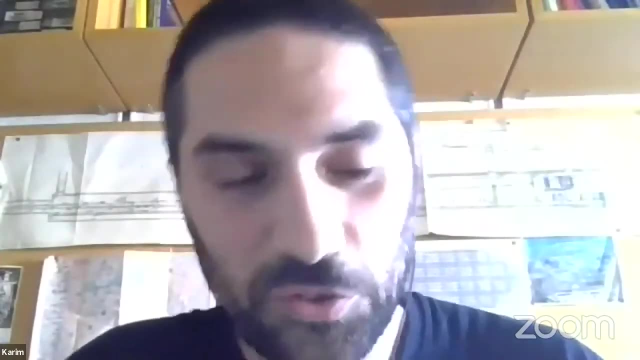 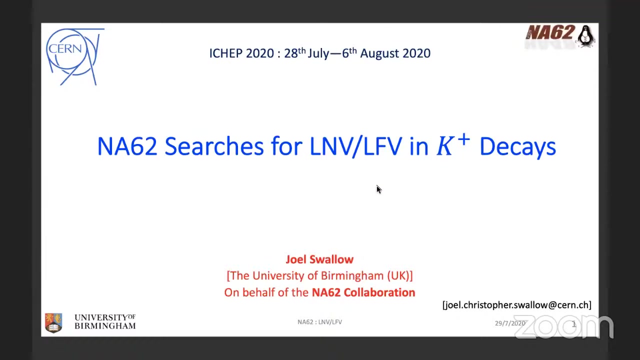 Thank you very much, And now we go to Joel Swallow, who will present the leptin flavor number. leptin flavor and number violation at the NE62X. Thank you, Thanks for having me. Hi, do you hear me and see the slides? 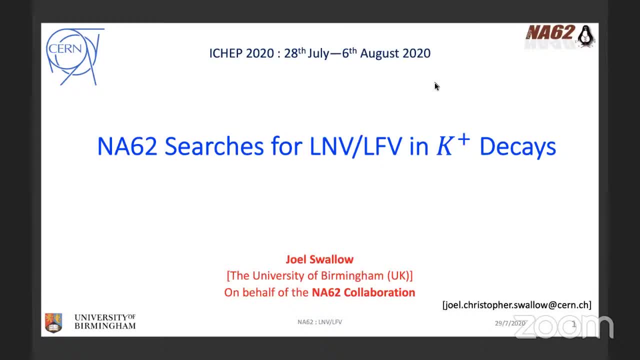 Yes, Okay, great, Let me know if there's a problem. Okay so, as Karim said, I'm going to be talking to you about NE62 searches for these leptin number and flavor violating decays. This is the quick overview of the talk. 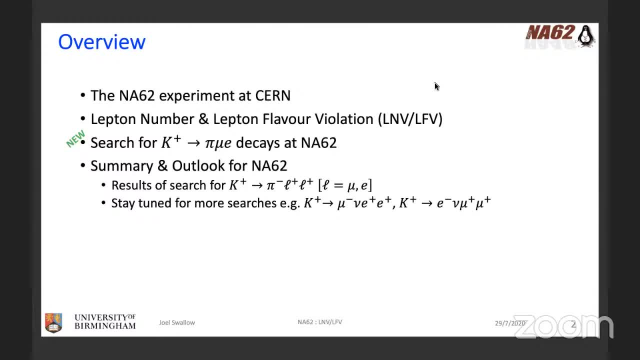 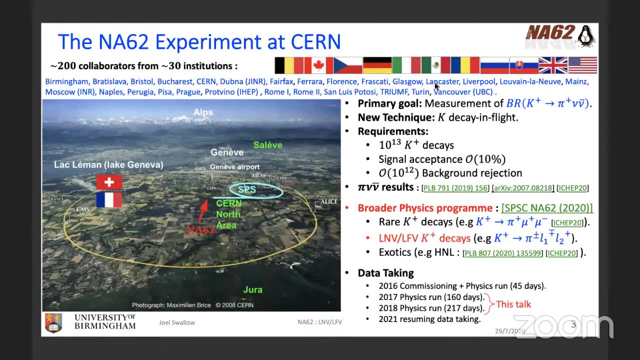 So I'll tell us you something about the NE62 experiment, and particularly the new result on the search for K goes to, and then some context related to the other searches that we're doing. So the NE62 experiment is based at the CERN North area. 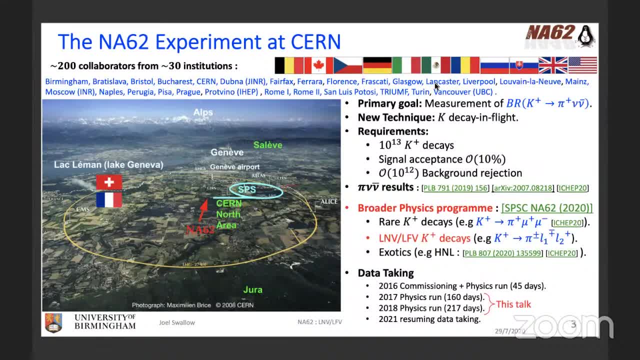 We're at the end of an extraction line from the CERN SPS And you can see on the left that we sit roughly at the center of the LHC ring And the primary goal of the experiment is the measurement of the ultra-rare K goes to: 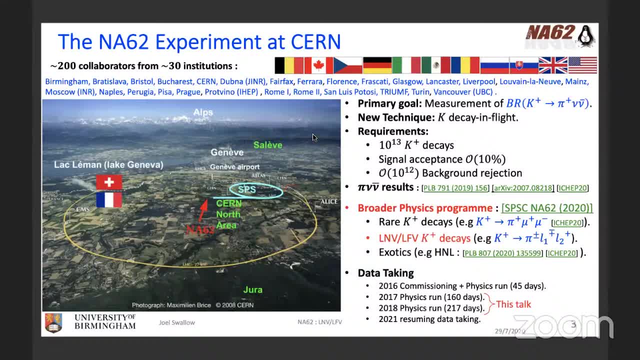 pineal, new bar, decay, But I won't go into any detail there because there's a very recent paper on the archive from the 2017 data analysis And there was a nice talk yesterday on our brand new result. Instead, I'm focusing on the broader physics program at NE62.. 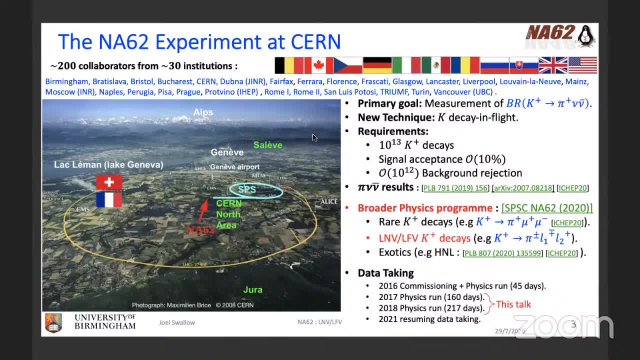 So this was also covered nicely in the last couple of days with the rare K on decay- K goes to pi mu mu covered yesterday- and also exotic searches, in particular for heavy neutral leptons, Also the subject of a recent paper and a talk, The run one data. 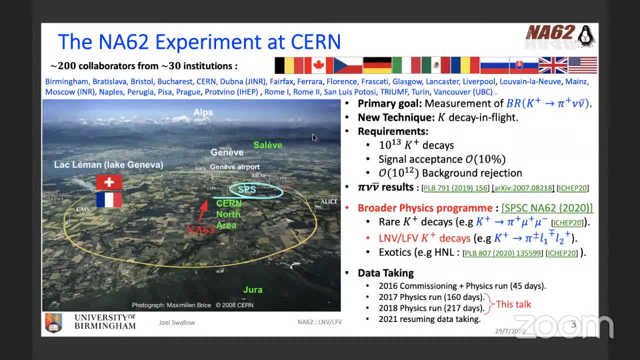 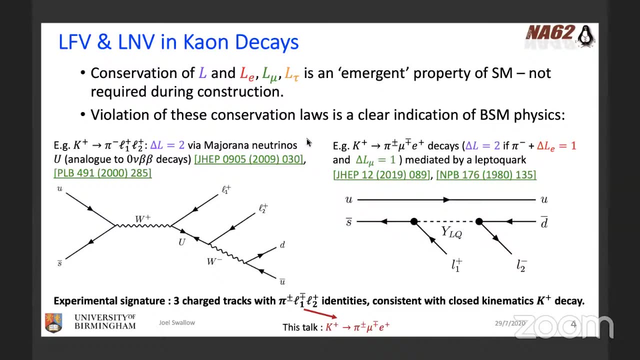 set was taken from 2016 to 2018.. And in this talk, I'm focusing on the data from 2017 and 18.. Okay, And as has already been covered quite well so far, and I won't labor the point- and in the standard model, 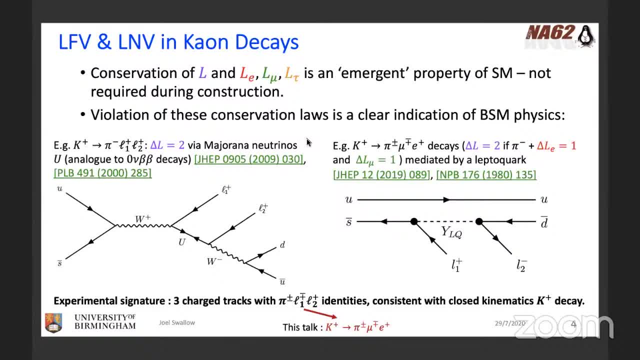 we have this conservation of lepton number and lepton flavor numbers, which is somehow an emergent property, but we've seen, in with the the neutrino, we've seen with the, the neutrino oscillations, that these individual flavor numbers can be violated. 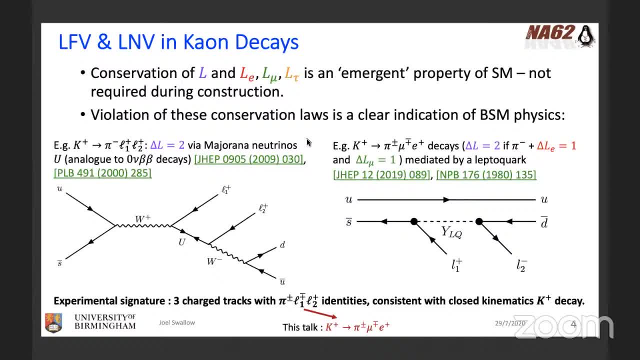 So it's worth checking to see if we can also violate them with the, the charge leptons as well. So in particular, you could have a scenarios with encounter case where you have a mediation via Majorana neutrinos, as you see on the left-hand side, or mediated by lepto quarks. 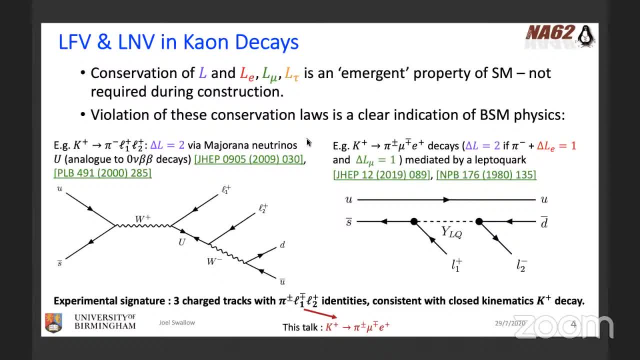 as shown on the right. In any case, the experimental signature here that we would look for is a pion And two leptons with the decay consistent with closed kinematics. If we then go to the next slide, you see just a picture on the left. 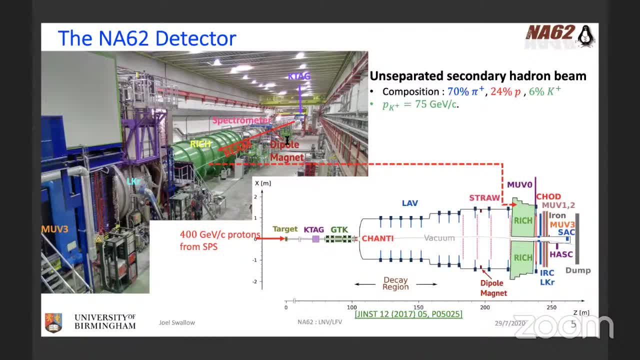 and the schematic on the right of the NA62 experiment. So we're using an unseparated secondary hadron beam that's produced when protons from the SPS hits a beryllium target. The experiment is very long, as you can get an idea of on. 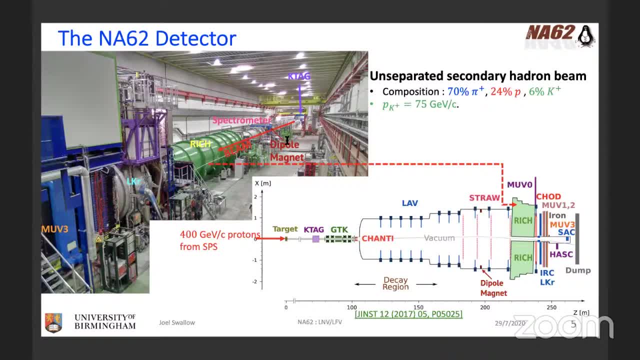 on the picture and then the schematic of the detector, And this is governed by the momentum of the K-on, which is 75 GV, and the Lorentz boost in the lab frame. I won't go into too much detail on the whole detector. 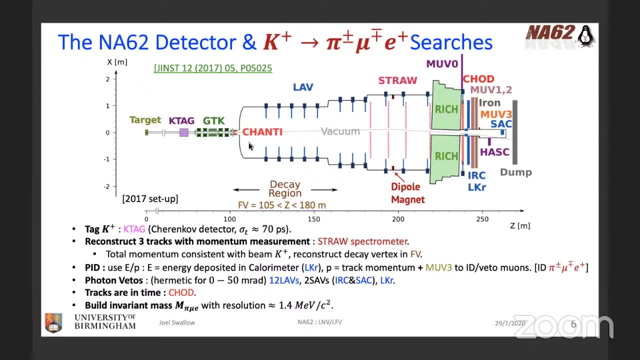 but just to comment on how it's used. in this analysis in particular, I told you that only 6% of the secondary beam is K-ons, So we tag these with the Cherenkov detector, the K-tag, with a very good time resolution. 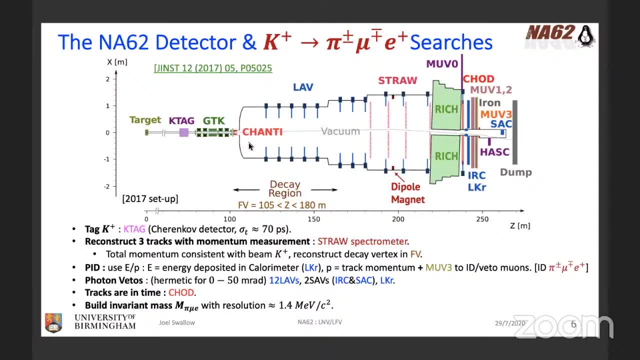 Downstream we're looking for a three track event and we reconstruct the tracks and measure their momentum with the straw spectrometer And we can then reconstruct a vertex in the fiducial volume. So this is indicated. It's a long vacuum tank region in which we're reconstructing this. 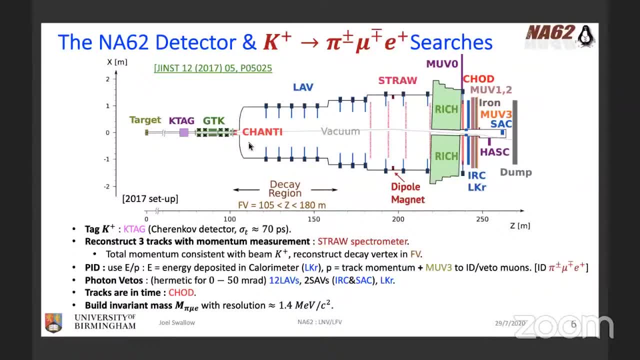 For particle identification we're using this ratio of E divided by P, where E is the energy deposited in the liquid krypton calorimeter and P is the track momentum. And then also we can use the muon veto 3 detector, which is at the very end of the experimental apparatus. 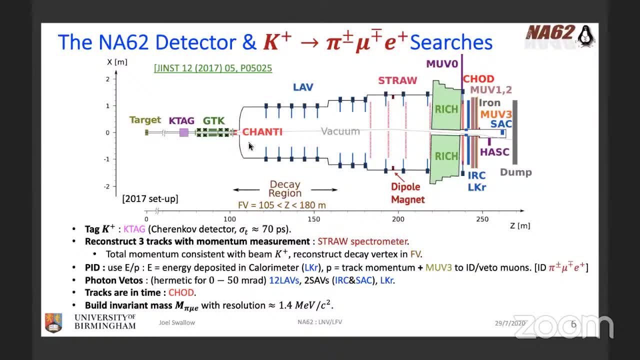 behind the calorimeters and an iron wall which is sensitive to veto or identify muons. There is a hermetic veto system at NE62 with 12 large angle vetoes surrounding the vacuum tank, small angle vetoes and liquid krypton calorimeter. 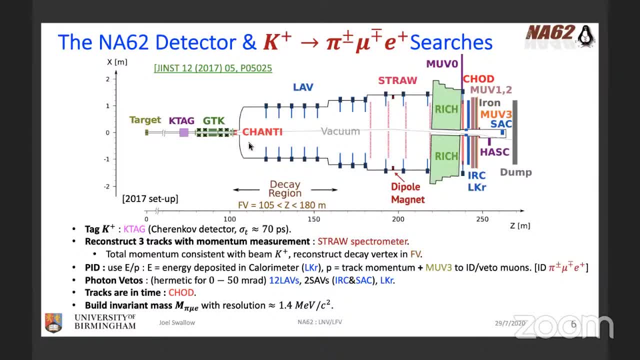 In this analysis, we're using the large angle vetoes to reject stray photons, The tracks must be in time, and we're using charged hodoscopes to make these timing measurements And, in the end, we're building an invariant mass of the primary candidate. final state. 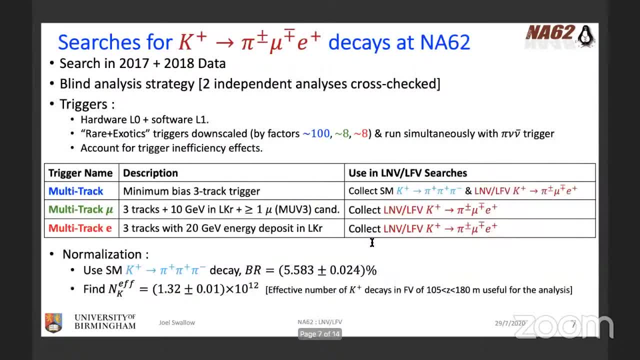 with the resolution of about 1.4 MeV. On slide seven you see the search strategy. We're searching with 2017 and 2018 data using a blind analysis strategy. There was actually two independent analyses and these were cross-checked for the. 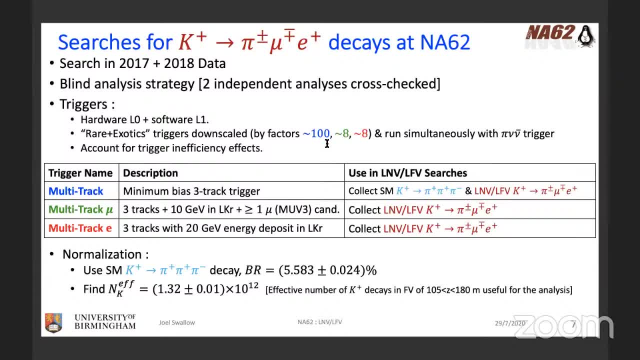 for the final result At NE62, we have a two level trigger system, with hardware level zero and software level one, And these triggers that we're using for this analysis, as shown in the table, are run concurrently with the pioneer bar trigger and downscaled by certain factors. 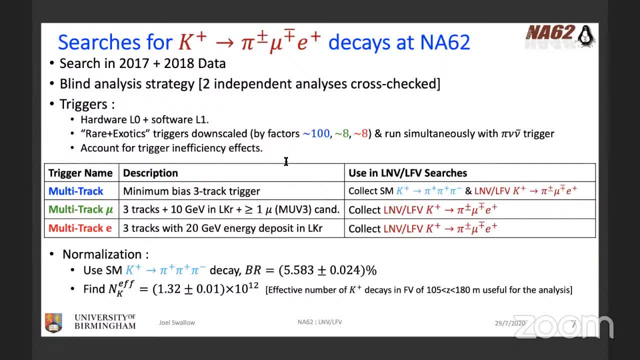 The inefficiencies of these triggers importantly need to be accounted for in the analysis. We're using a minimum bias multi-track trigger to collect the normalization channel, which is the k goes to three pi decay, which is the most common three track k on decay. 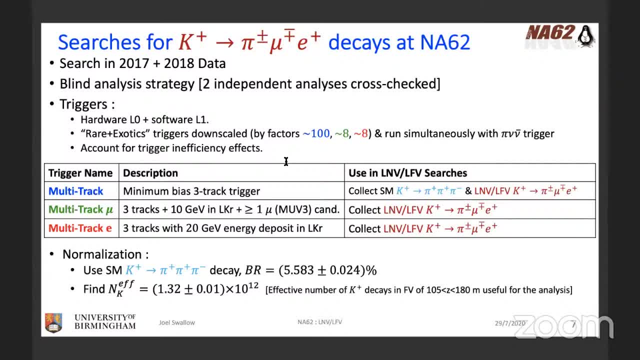 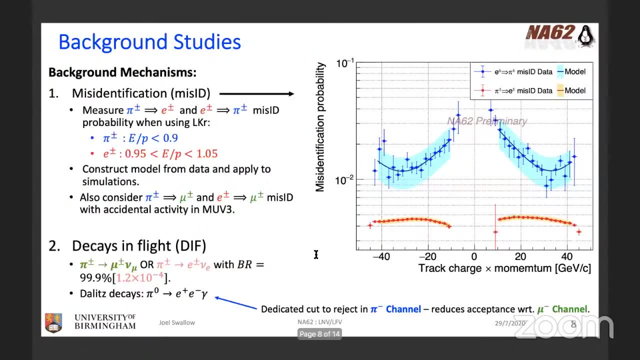 with a branching ratio about 5.6%. We're then using all three of these triggers to collect the signal candidates, and the overall effective number of k on decays in the fiducial volume that you can use then for this analysis is about 10 to the 12.. 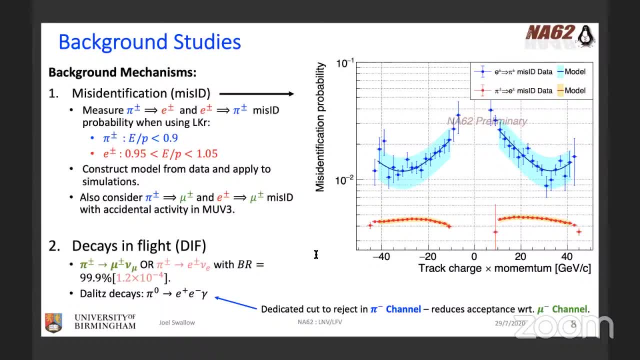 There's quite a number of backgrounds that have to be considered in the analysis and these enter by two ways: either by misidentification or decays in flight. Just to give a feeling for the misidentification. you see on the right, the misidentification probability. 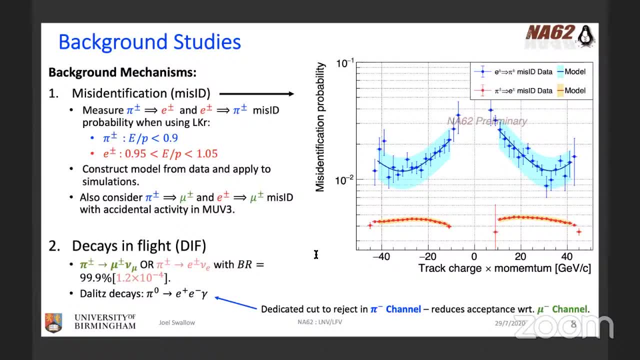 as a function of track charge times, momentum for the processes of pion, looking like electron or positron or vice versa, And this comes from using this e over p ratio that I was discussing before, where the electron is basically depositing all of its energy in the calorimeter. 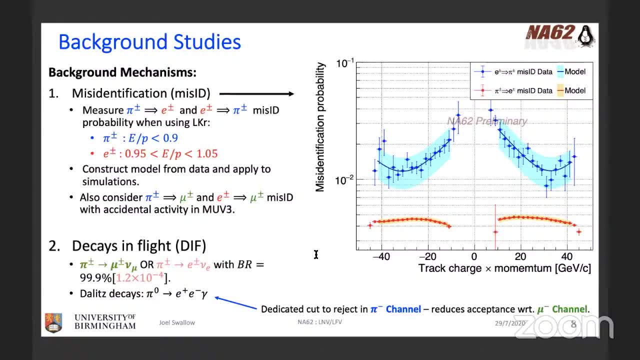 so you have an e over p ratio close to one. There is also the decays in flight that must be considered Importantly, the decays in flight of the charged pions, either to a mu neutrino or e neutrino, and the former is more important in general. 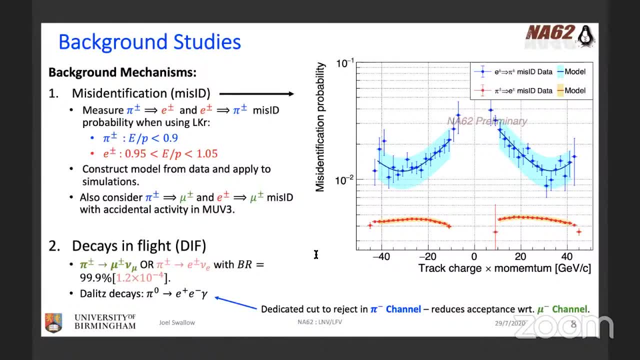 because it's much higher branching ratio is there. There is also the pi zero Dalitz decay, which is a particular nuisance in one of the two channels that we'll talk about in a moment, And this means there's a dedicated cut used for this. to reject this. 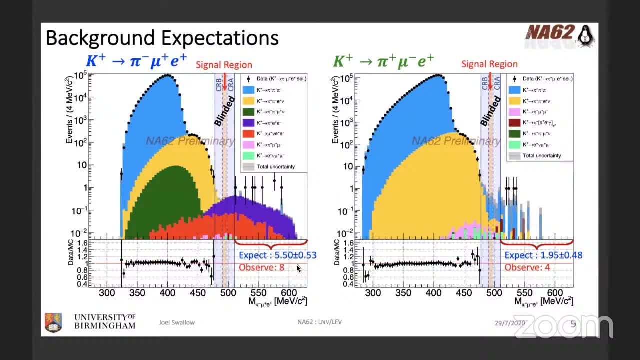 Here you see the invariant mass distributions on the left for the pi minus, mu plus e plus channel and on the right, pi plus, mu minus e plus. We have a blinded region which was kept blind for the optimization of the analysis, which is centered on the k-on mass. 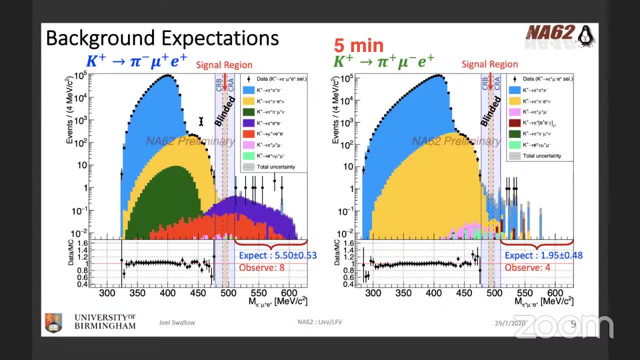 and the central signal region that you can see indicated sits at the k-on mass. We then have the sideband control regions that are also indicated Above this blinded region, you can see. we expect a certain number of events, as indicated, and the observations match quite well to these expectations. 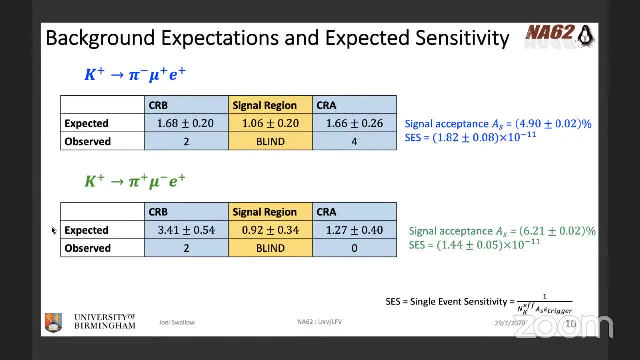 If we move forward now we look at the sidebands, We can see again that the agreement between the expectation and the observation is good. The acceptance for the two channels are also indicated on the slide. So for the pi minus channel it's about 5%. 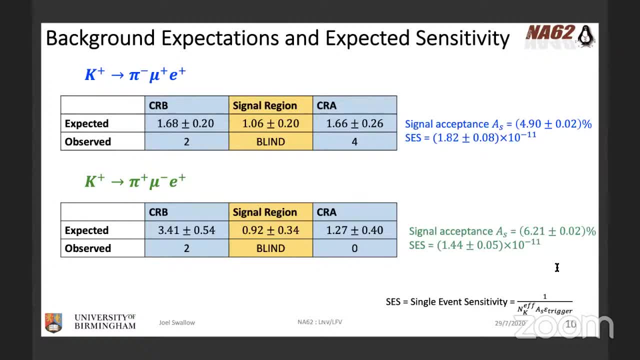 and it's about 6.2 for the mu minus channel And the main difference here is this additional cut to reject the Dalitz decays which I already mentioned. You can see also the single event sensitivity, which is calculated here at the level of about 10 to the minus 11,. 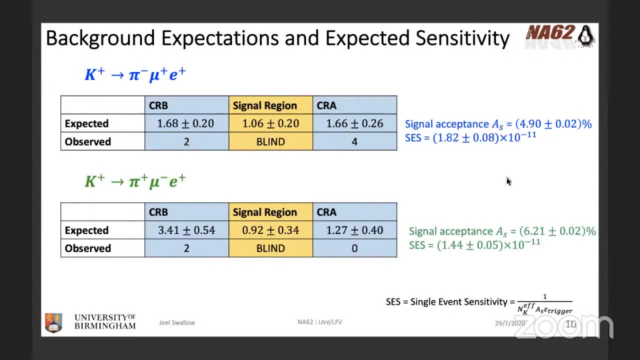 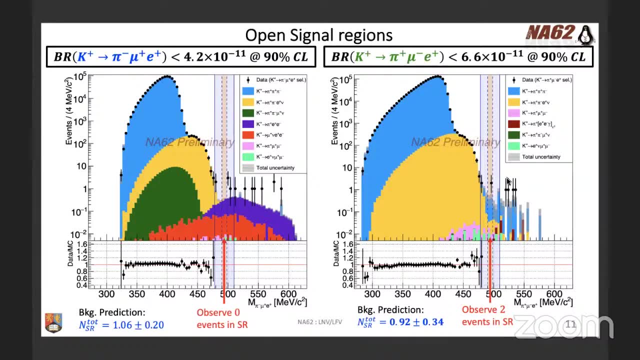 calculated using the equation at the bottom of the slide. Okay, so now we go ahead to the result And, as we saw, the expectation in both channels is about one event And for the pi minus channel, we observe zero events in the signal region. 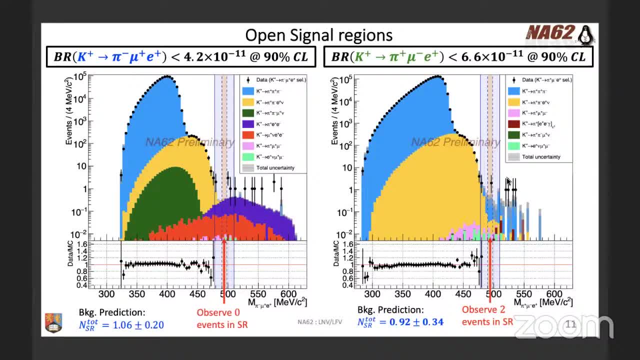 So we set an upper limit at less than 4.2 times 10 to the minus 11 and 9% confidence level And similarly in the mu minus channel we actually see two events and in the same way, we set an upper limit at less than 6.6 times 10 to the minus 11 and 90% confidence level. 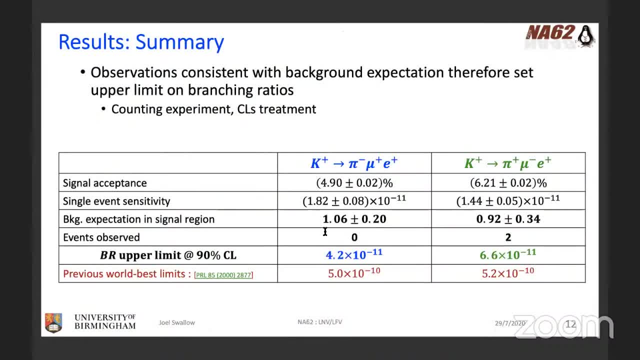 On the next slide. all I'm doing is summarizing the results. So we see the acceptance for the signal, the single event sensitivity and the expected and observed number of events. Takeaway message here is to compare these new limits that we've placed with the old, previous best limits. 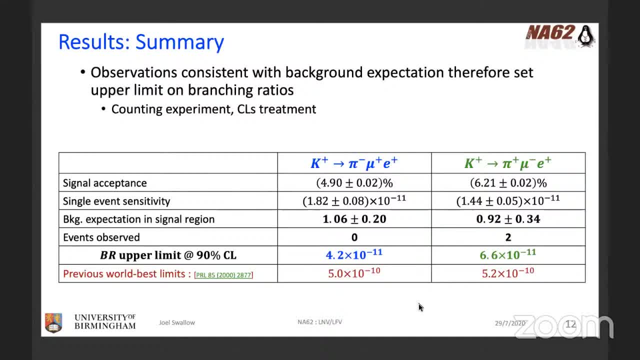 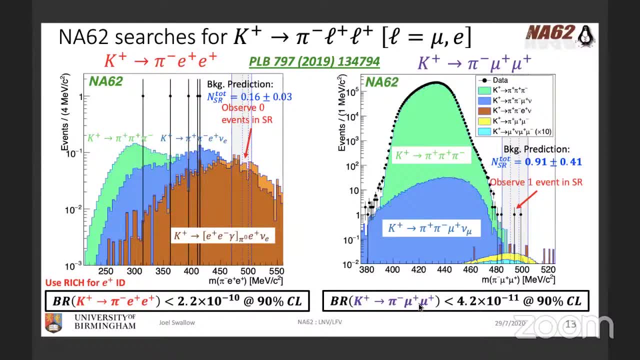 And we see we've improved by roughly a factor of 10.. This goes into the context also of the recent studies that we've published last year on the pi minus. and two same signs, nine same flavor leptons. So pi ee or pi mu and mu. 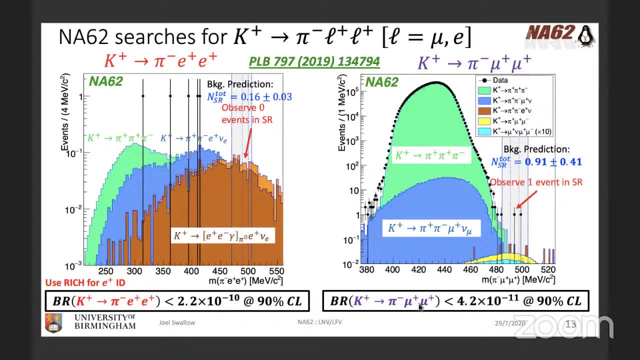 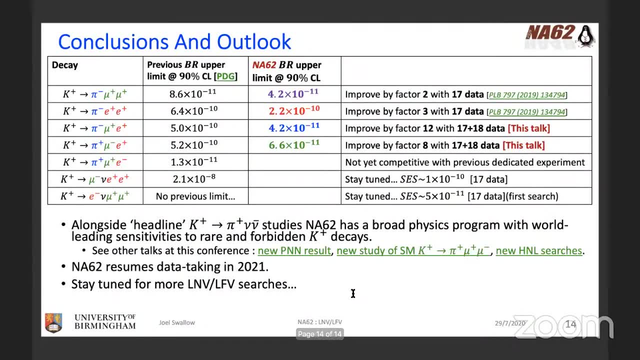 And again, using quite a similar analysis strategy, we observe these upper limits on the branching ratios of these processes. This brings me to the conclusions slide. So, alongside these nice headline pi nu nu bar studies at NA62, we have this broad physics program with the world leading sensitivity to these rare and forbidden k-under k's. 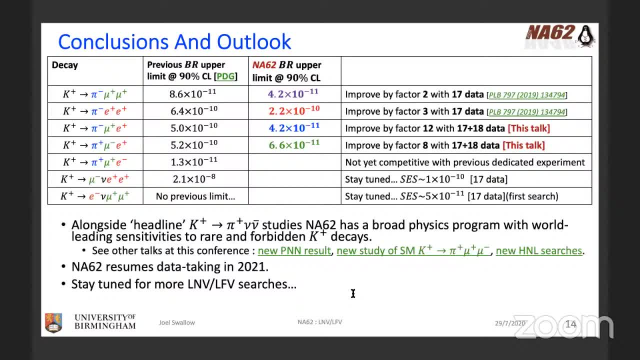 I invite you to see the other nice talks at this conference. In the table I summarized the picture for the lepton number of flavor violating searches at NA62.. So I've just shown you the top two where we've improved the previous limits using just 2017 data. 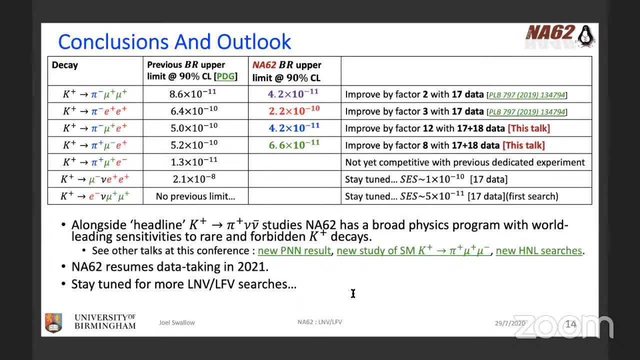 And this was published last year, And now in this talk, we're showing the improvement in the pi mu ee searches, which improved by a factor of 12 and eight for the two channels, Using both 17 and 18 data. We're going to resume data taking in 2021. 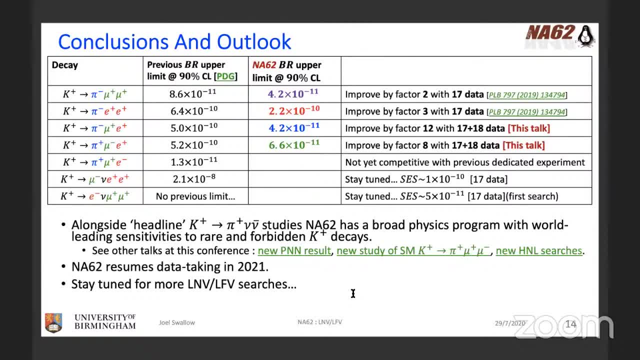 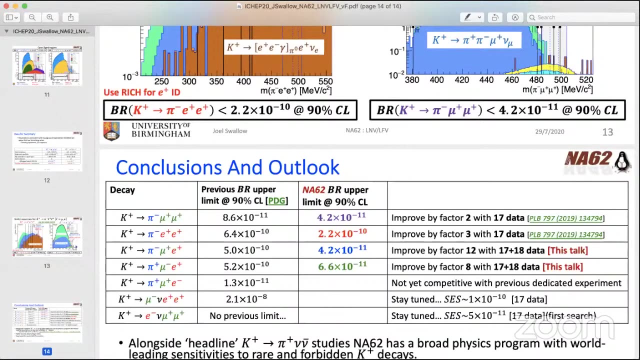 And already we have our eye on some of the channels, as you can see in the table. So stay tuned for future updates on this, Thank you. Thanks a lot to join. So any comments or questions from the audience? I don't see any. 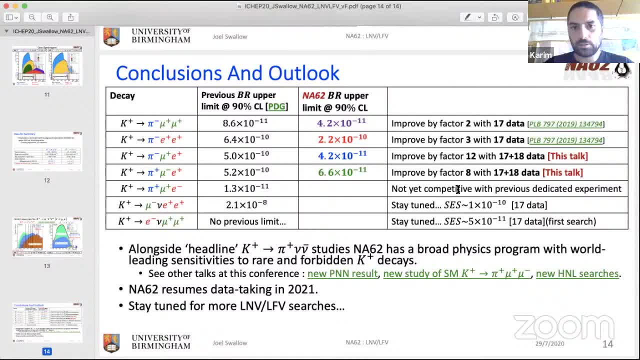 Okay, so maybe you can just tell us more or less. Do you have an idea on how big could be the improvement on these limits? Adding, let's say, the next data taking data. Okay, So when we resume data taking, the intensity will be a little higher. 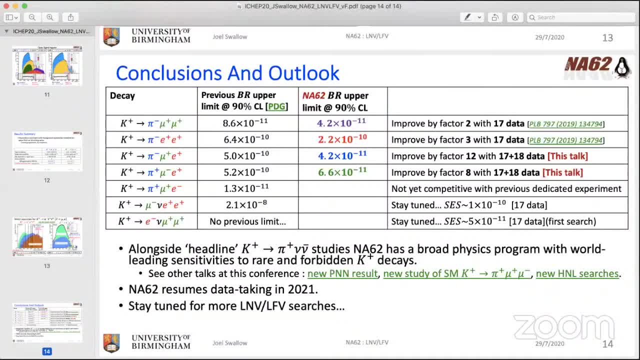 And so there's definitely potential to improve in terms of taking data, And we're not background limited in these analyses. So this is this is the good news, And one thing that we have to be wary of is that, because we're going to this higher intensity, 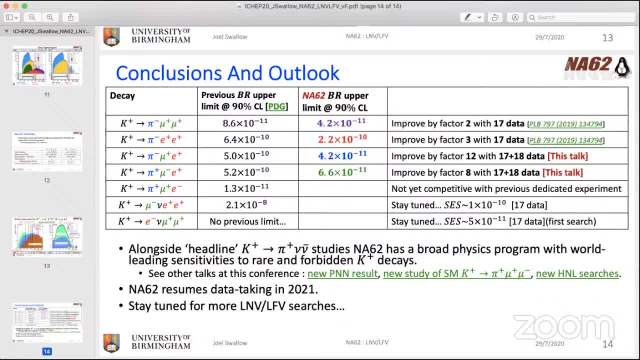 the trigger strategy might have to change a little bit, So this might mean that relatively we're taking less data for these kind of analyses In the future. But overall you make it could be possible to improve by a factor of order. five. 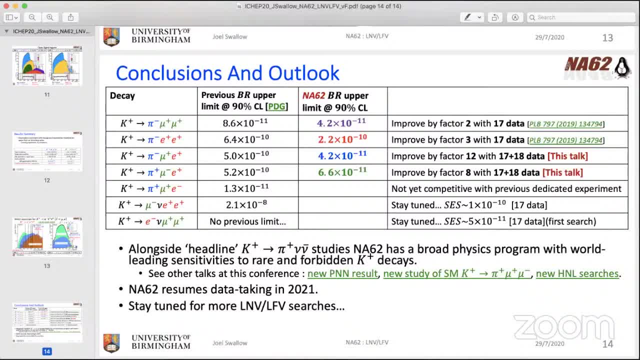 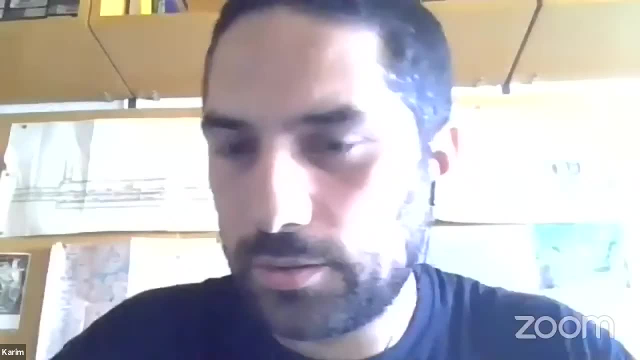 potentially with the next data set. Okay, that would be very good. Yes, Okay, Okay. Thanks a lot, Joel. I don't see any other comments or questions, So I would propose to move on And, of course, if anybody I remind anybody that there is a Mattermost channel. 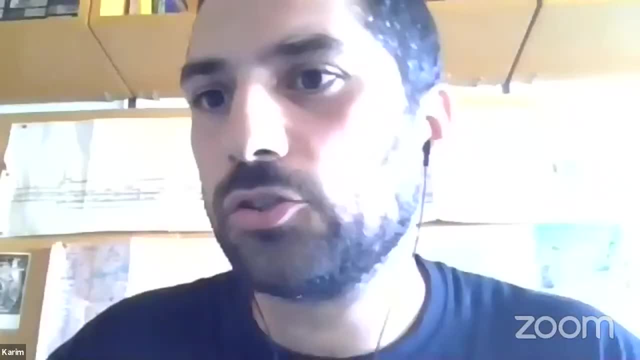 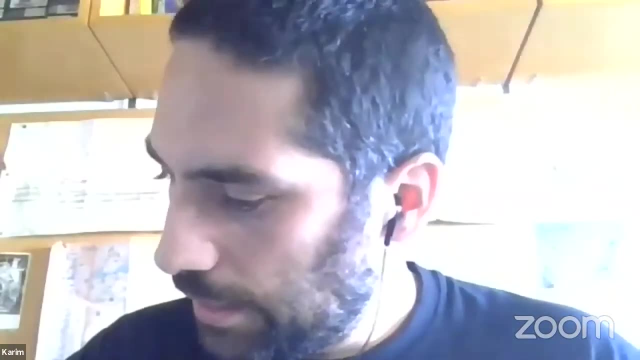 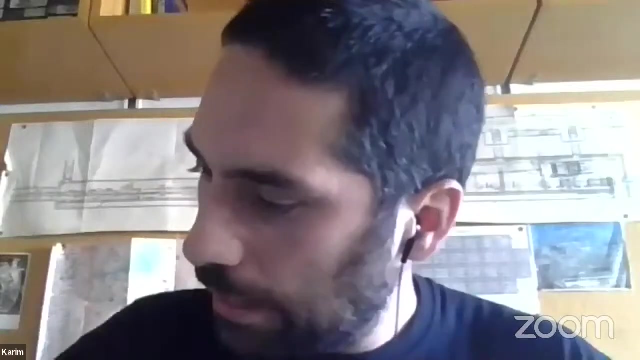 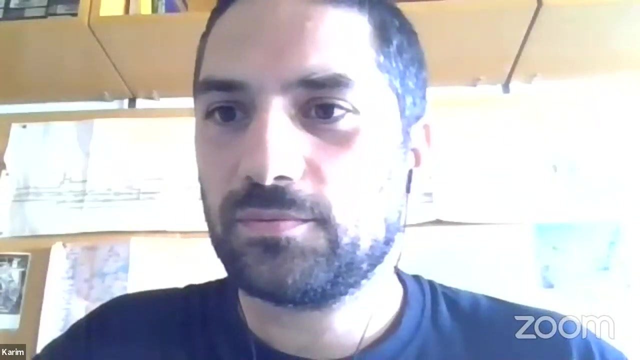 So if you want to have more, more discussion about some particular topic, please feel free to to have a discussion there. So now we go on with the next talk, which is by Amarizoni on the lepton flavor, universality violation and their repercussion. 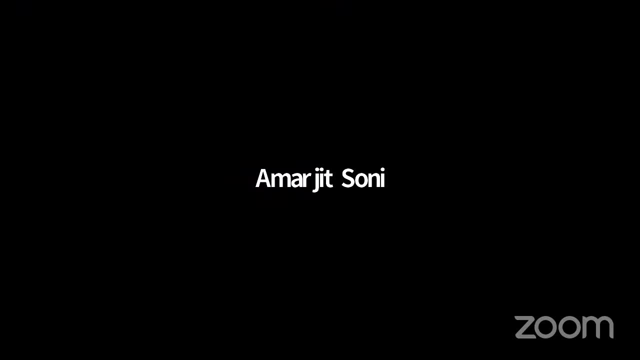 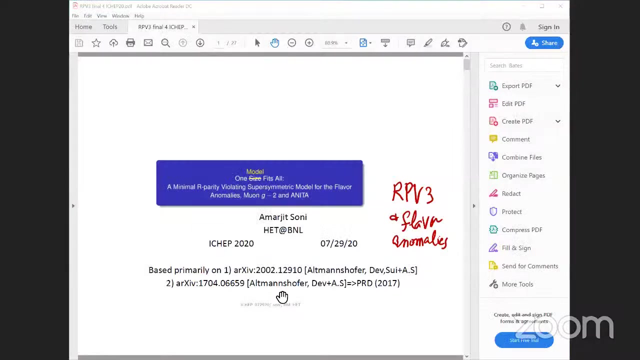 Hello, Yeah, So just Give me a second. I guess I'm going. Oh yes, So This is the video. Okay, Very good. How can I get the full screen here? All right, So can you hear me? 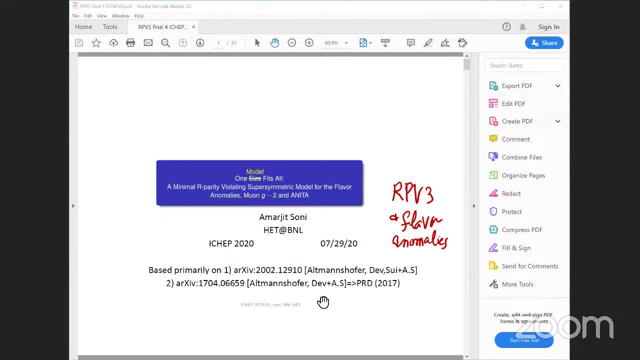 Yes, All right. So I'm not sure why I cannot use the full screen, but I think I'll go ahead with this. So, yeah, I will be talking about the flavor anomalies And, in particular, because of the shortage of time, in the context of our parity violation. 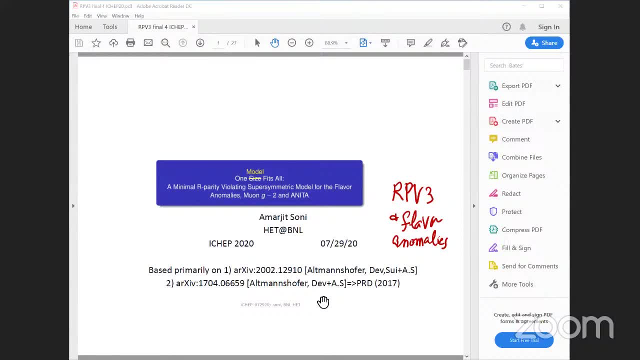 Susie and the 3D. I'll explain in a minute. So anyway, this is a paper with a word from working on Altman, Hoffer and Dave And for the last of three, four years. second, in a SQL district took place a couple of years to get all the pieces. 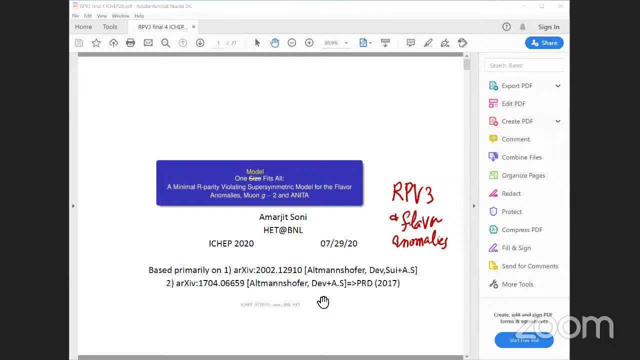 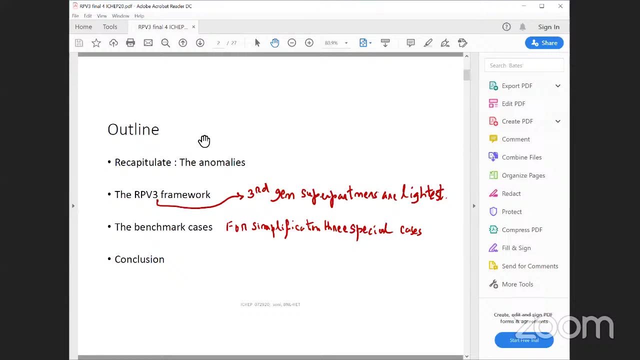 together. All right, Okay. So I'm sorry, I don't know why. the next, Okay. So here's the outline and I'm going to remind you the anomalies. And then the point is this: RPV Susie has lots of reasons for going after that. 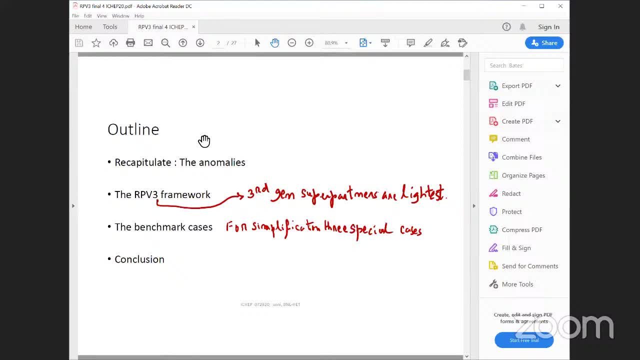 And we are putting the three there for the, the because of, starting from about 2017, your media. you know, for good reasons, that the third generation super partners are the lightest, And then I'll explain some three special cases for which we study this. 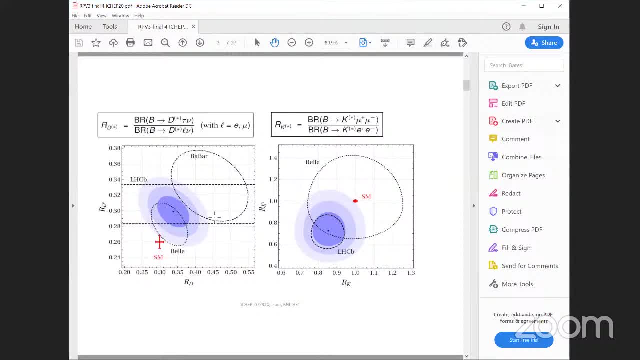 scenario. So of course you all know about the anomaly, the charge current anomaly and the neutral current anomaly, And there are all three experiments, B experience experiments showing some deviations in the in a simplest tree level charge current case on the left and amounting to 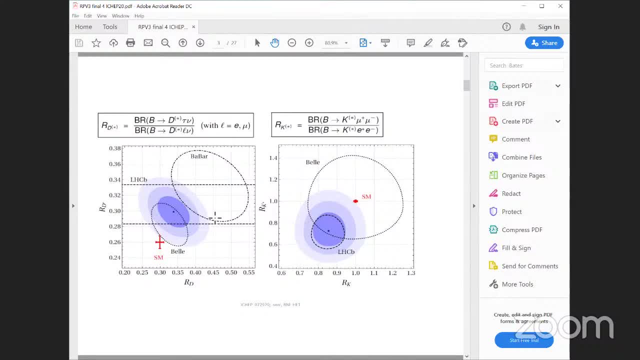 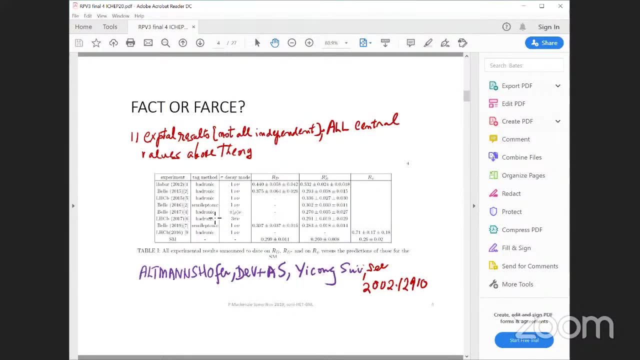 at the moment about three Sigma And on the right is the LACB RK RK star. This is about three and a half Sigma And the fact, of course, we always need to worry So many experiments from the charge. current case. 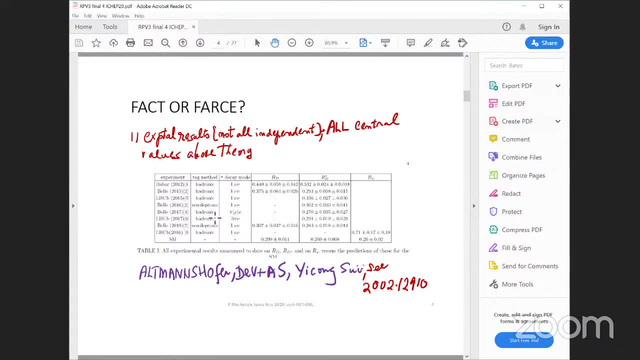 They're altogether 11 of them, And all 11 central values are higher than theory- And again, I don't have time to spell it- And this needs to be kept in mind. So it it seems as if you know. 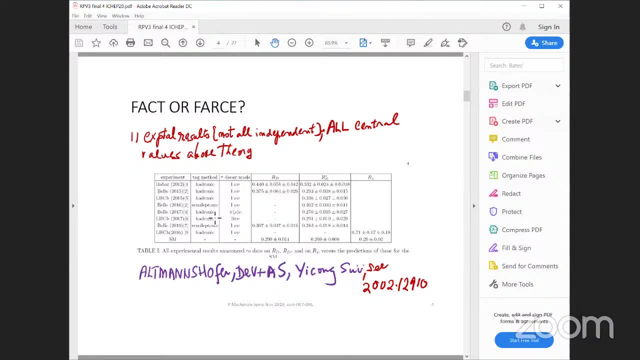 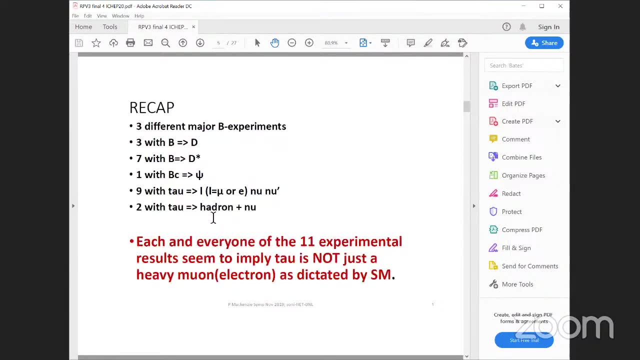 there is no way out And we have seen the breakdown of the standard model. but this is, in my opinion, not not. we cannot assume that that easily, because you know. so this is category of the experiment. three different experiments. major B: 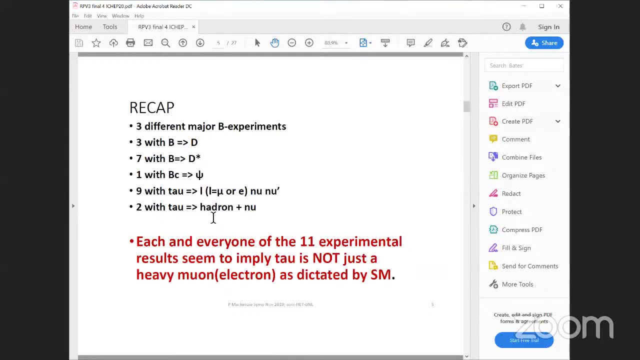 B experiments are involved: Three with B to D, seven with B to D star, one with BC to Psi, nine with Tau going to leptonically and two with Tau going pedronically. Each and every 11 of them show central value higher than a standard model. 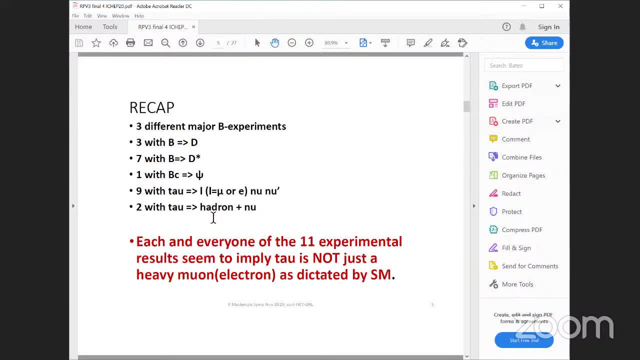 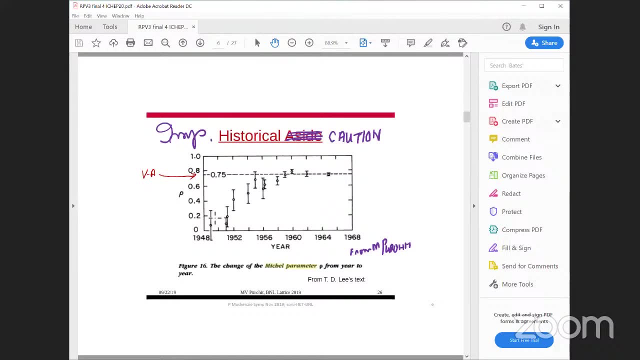 So it seems as if the universality is breaking down, but I think there are cautionary things that we have seen in the past, in our history- And this is a 10,, 12 years history- and long ago in the Michelle parameter, which is standard model. 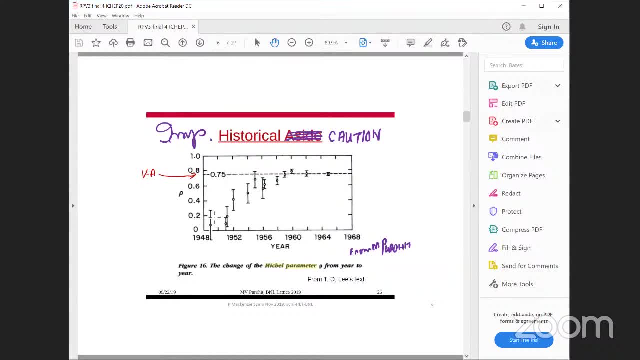 We might not say predicts 0.75 experiments for 10, 12 years, kept on seeing it below And then somehow magically it starts to come in agreement. So things like this can happen. They are there. Sometimes the systematics are there. 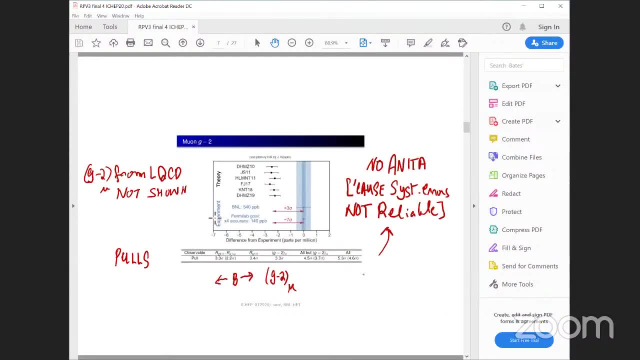 And I'll elaborate later on more. And so, anyway, then I also bring in here G minus two and G minus two. Booking. an experiment is deviating from theory by three and a half Sigma. on this slide only the phenomenology theory- dispersion relation is shown on the lattice- has made a lot of progress. 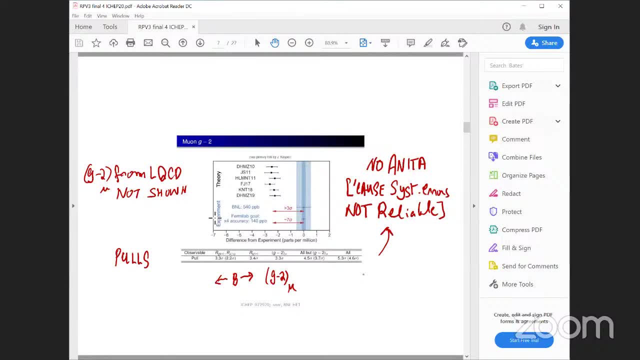 and- and it's about a factor of two larger errors at this point- And then the dispersion theory. but it will catch up pretty soon, in next year or two. And I'm also showing here- not showing here at the moment- the next slide for the balloon experiment called Anita. 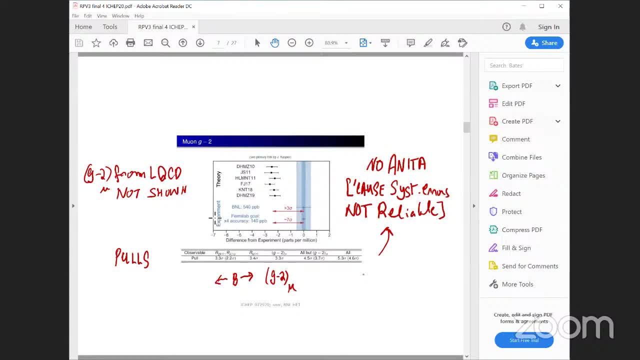 because the systematic errors are not under control. I don't like to show that. So in the book in the bottom are the pool for all of the three experiments that I talked about: RKR, RDRD star, RKR star. 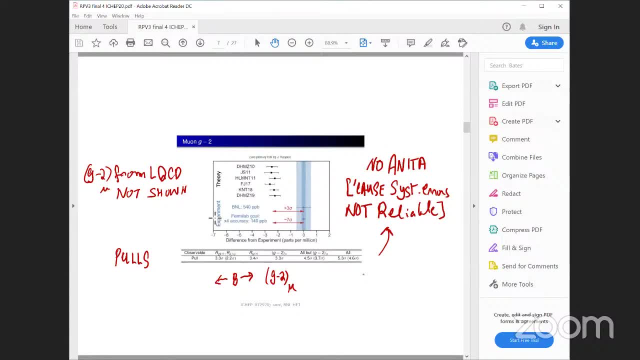 G minus two mu And whether there is some issues in RKR star. but in our mind is a theoretic theoretician, We take the Liberty or take license of leaving on Baba because it has a lot of deviation there. And if you leave out those, 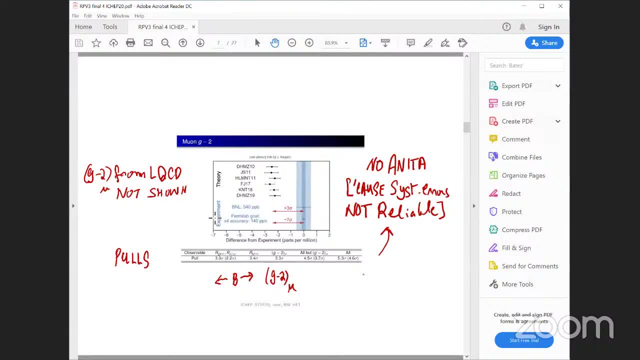 and you can see the when you take all of these three different types of experiments on the pool reduces to 4.6, Sigma, but otherwise it's over five Sigma. So it would appear as if this is compelling, but, as I said, 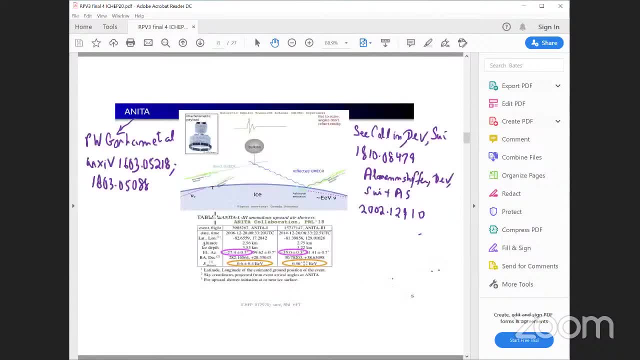 in each case there were some features, but in any case- and This is Anita balloon experiment, two gigantic energy, 10 to the nine electron moles, neutrinos, And both of these events people have argued cannot be understood from the standard model. 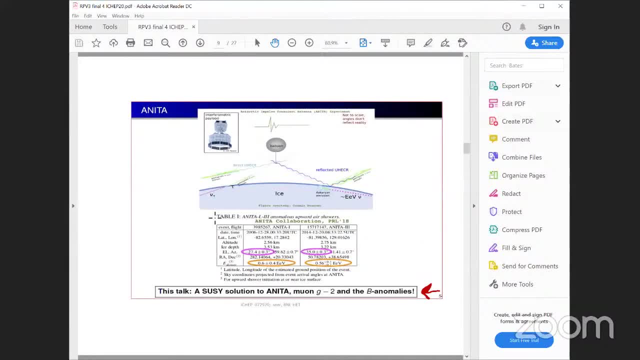 So I don't have the time to explain all of this, but systematic errors are worrisome. So we take Anita, along with the others that I mentioned, and we are looking for a SUSY solution, in particular RPV. The reason for that is the following. 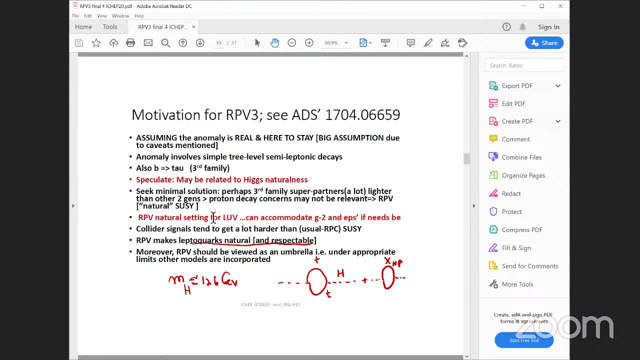 So, starting in 2017 paper, what we started, what we said, was the reaction B to D: star tau or electronic decays. is B going to tau? This is a third generation and perhaps it is all related to the problem that we have Higgs- naturalness. 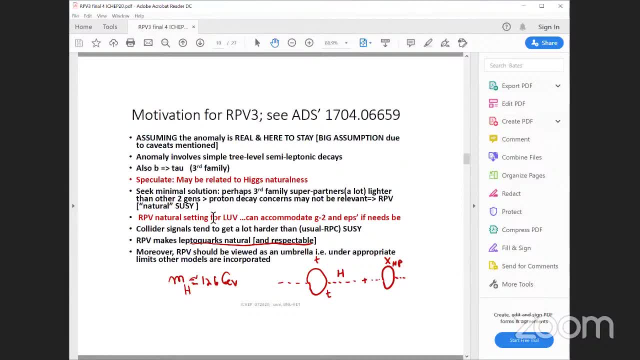 Higgs stability under radiative corrections, which is shown in the picture below. And so we wanna. we just proposed that the Higgs naturalness- let's consider the third family of super patterns partners- to be the lightest. If that happens, the proton decays. 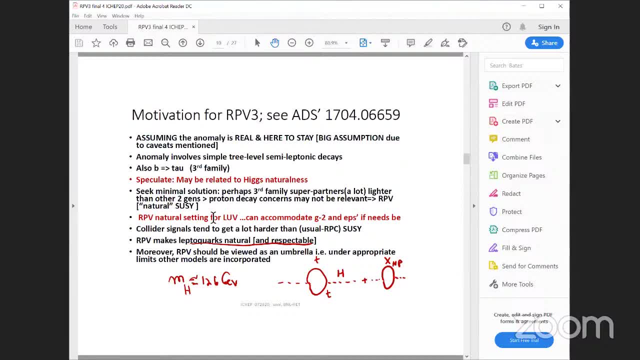 it becomes irrelevant and largely irrelevant. And so you go from the minimum MSSM to you can go to RPR evaluation. RPR evaluation is becomes, you know, a very good candidate. In fact, remember that RPR conservation just put in by hand. 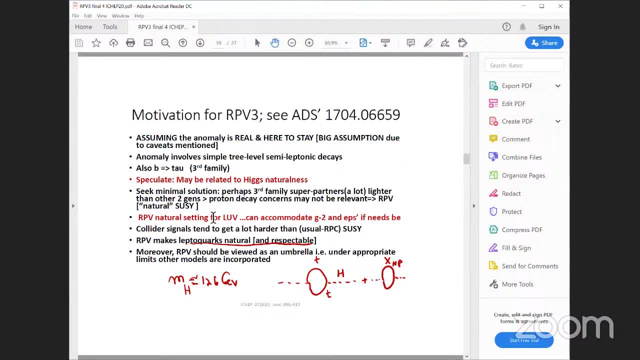 because you wanna protect the proton. But in this case, when the those super partners, first and second generation, are super, super heavy, Only the third generation is lightest, That proton decays are not really relevant. So we go, we RPV is very natural. 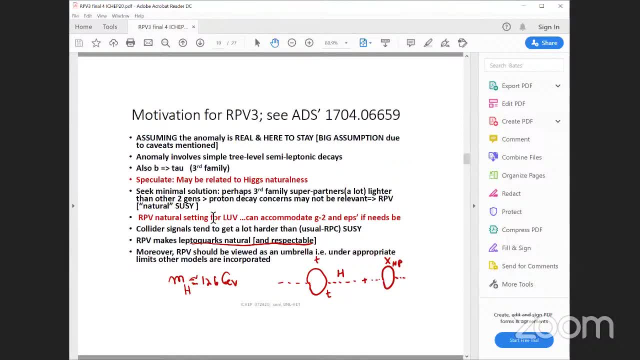 And in RPV, then lepton universality violation becomes natural And it lepto quarks become natural and G minus two, and if some prime thing like this you can accommodate, And the LAC looking for signatures for our and what's the prime thing for this? 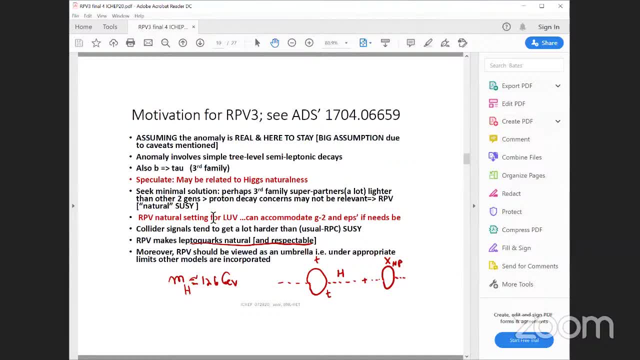 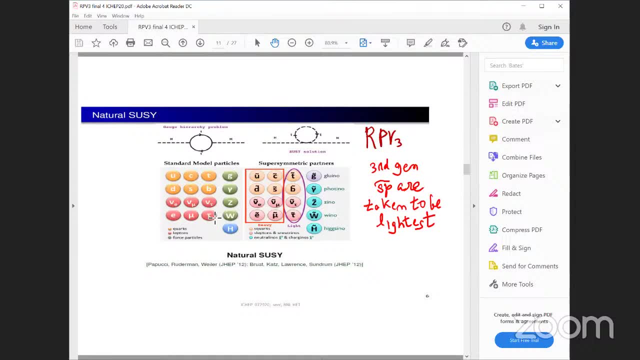 That's usually a very, very validating theory is a harder. So all of those reasons may make us wonder if this is, this is the way things are going, So, so anyways. so this is again saying that the third generation is. 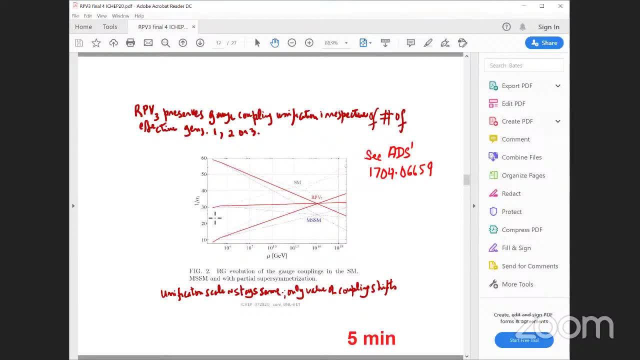 taken to be the lightest superpartners, and taken to be the lightest And a key point here is that one of the best interesting things about you know, Suzy, is that it gives you. you can see here, we show that explicitly- and whether you're one generation or three generation, 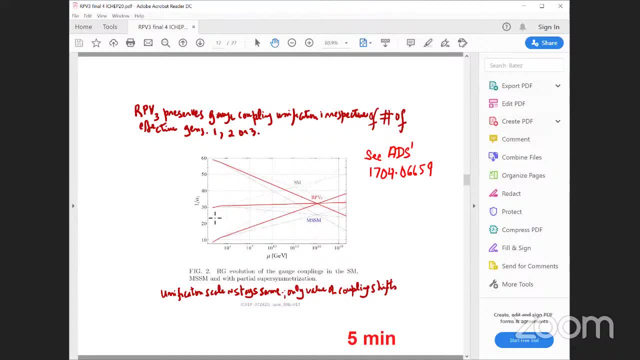 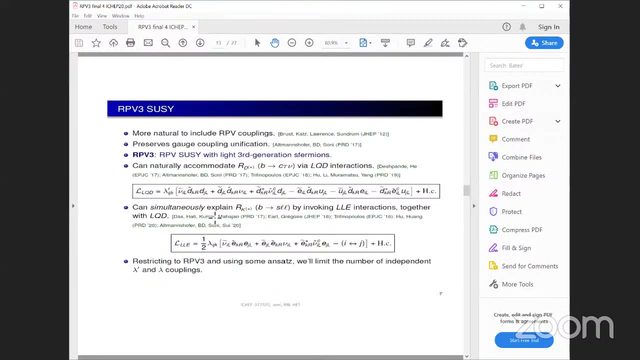 the gauge, coupling unification stays, it's just that the scale stays, just that coupling shifts a little bit. all right, so it has a nice feature too. so, uh, more on that, why it is so there are these effective logarithms that come in for our quark, uh, lepton interaction and lepton lepton. 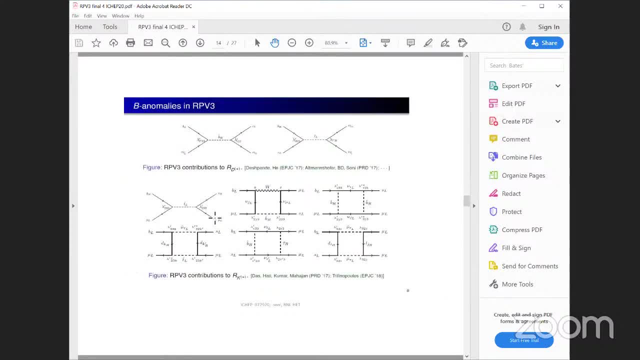 interaction and all that and we use those and there are a bunch of diagrams of this. charge current and this is a neutral government. for the neutral case, both tree level and loop level have to be capped because you want to get the sign correct for rk and rk star. the signs are correlated. 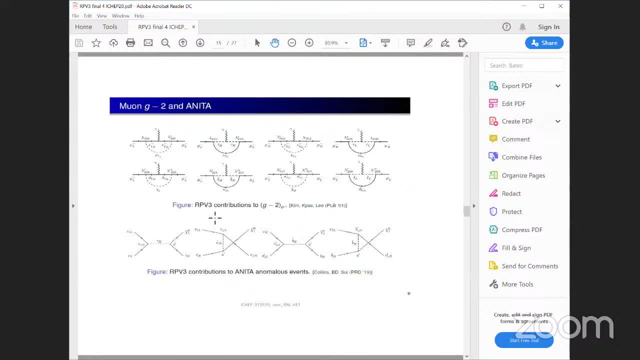 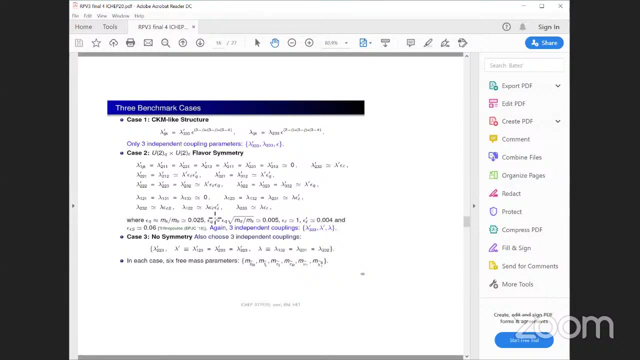 and having both tree and boxes are important. so then, this is for muon and also for g minus anita. i show you all the pictures and all a lot of the calculations are available in literature. we had to put them all together and the context of scenarios that we are studying. so then, to simplify things, we take three specific 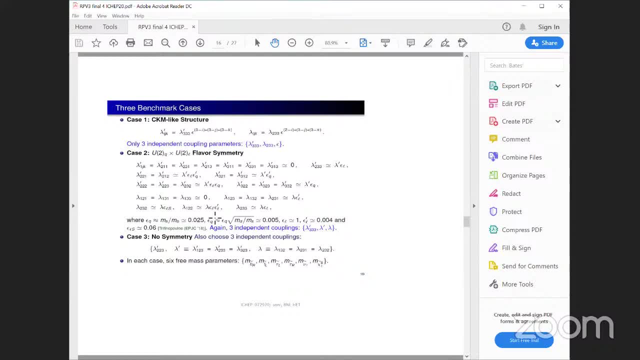 scenarios, benchmarks. one is very ckm, like in ckm. you know that first, if you, when you go to from first generation or second, you have to pay our price, and when you go from first to third, you have to pay even higher price. so we, we went to that and in so far as the third generation super, 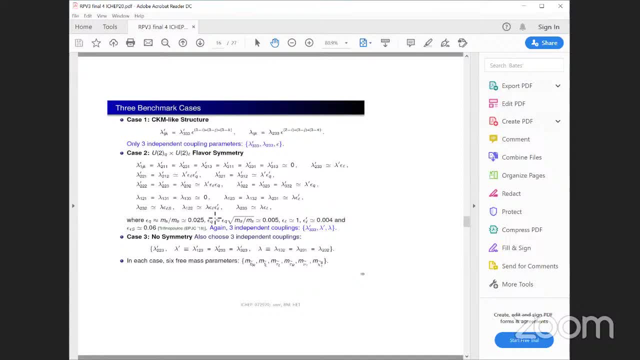 partners being lightest. uh, the. there was a very nice paper- i'll give the reference later- which formally put this in the context of youtube, youtube flavor symmetry, and this also has in each of these two cases there are three independent couplings and the third benchmark scenario. no such symmetry is imposed and again, they're not each of these three cases. 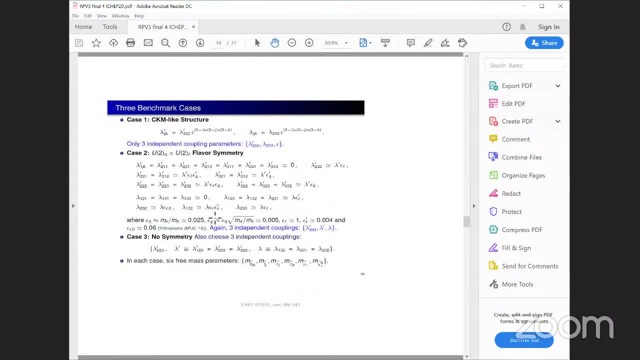 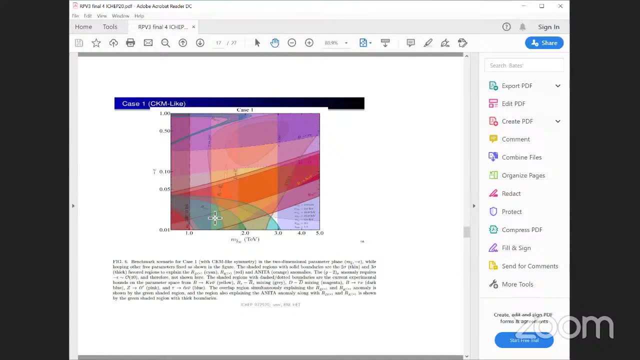 there are six, three parameters and three independent couplings are being used. so this is the case one that i mentioned, and you look for a common solution to all the anomalies and the common solution cannot be found. in particular, g minus two cannot be accommodated and the others perhaps could be, and then we look for case two. this is the reference for the very 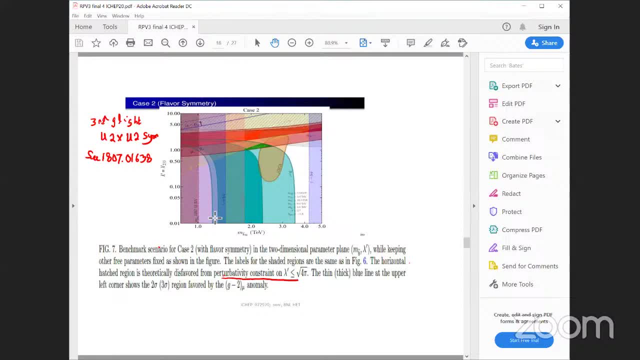 nice. uh, idea of making a third generation bottom lighter where the others are very heavy, and in this case you do find a solution in green there which overlaps, and there are some issues with perturbability in the horizontal scale up there, but you don't need to go there, it's just an. 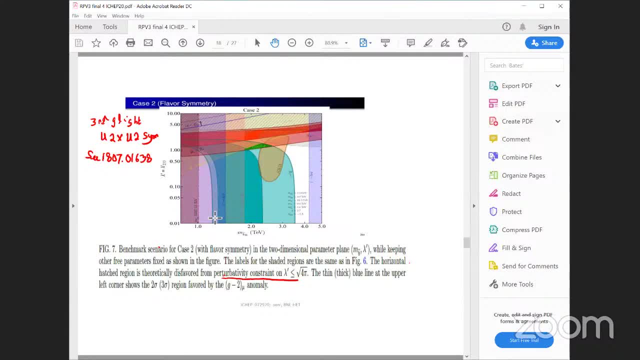 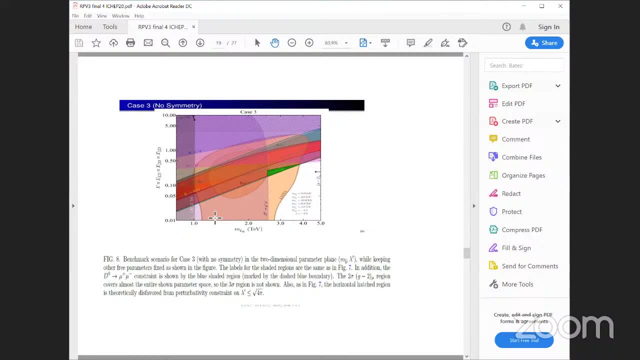 indication. all right. then the third one, uh, is, when there's no symmetry again, you are able to accommodate all of them. and there is an overlap, and this is pretty interesting, that, uh, you know, uh, that you are able to accommodate the things if the anomalies stay with you, of course, if you 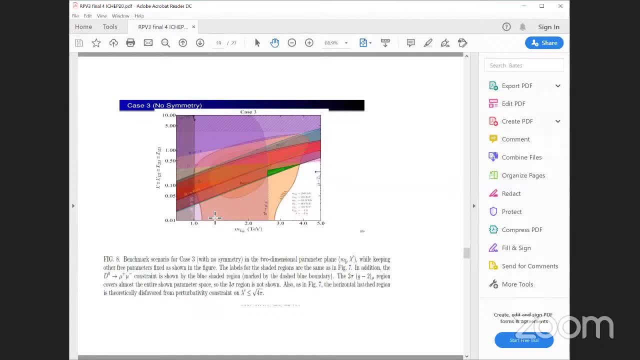 can you also have the capacity of taking? whichever one is, it does not for stand for the scrutiny, taking it out and see what happens. so it gives us a parameter space. the key point here is that that bottom mass uh has to be around, uh, you know, around two tb or or heavier, and then you know. 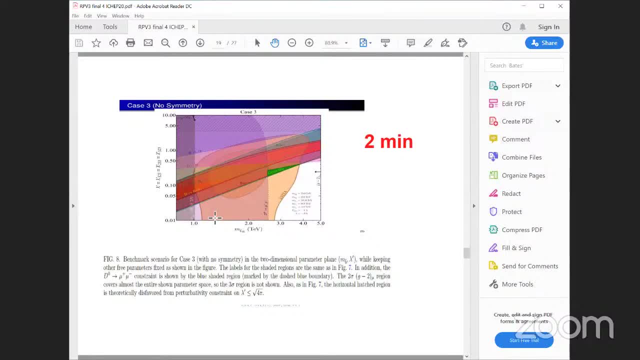 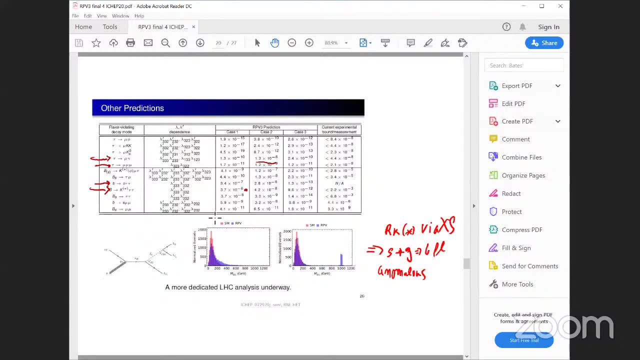 you have to look at our papers for other uh masses and so forth. i don't have the time to do that. so very interesting things happen in this kind of scenario for tau uh, flavor violation decays, in particular tartar, mu gamma is quite enhanced and b decays. the most interesting b decay is 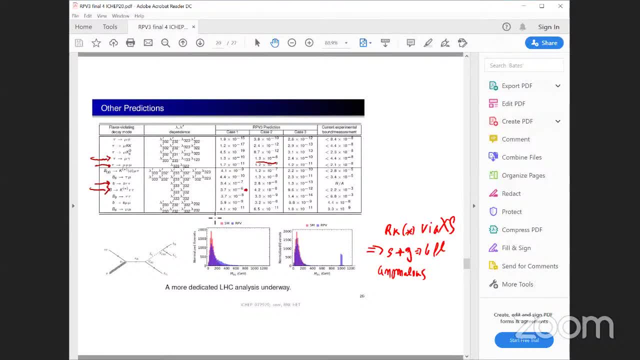 tau, tau, and it has a rather large spreading ratio, whether you go inclusive or exclusive. and that's pointed out, and it is it experimentalists ought to uh, go after them. this, uh, this would be a very important key. so what we are trying to do here is ask for repercussions of uh under this theory. 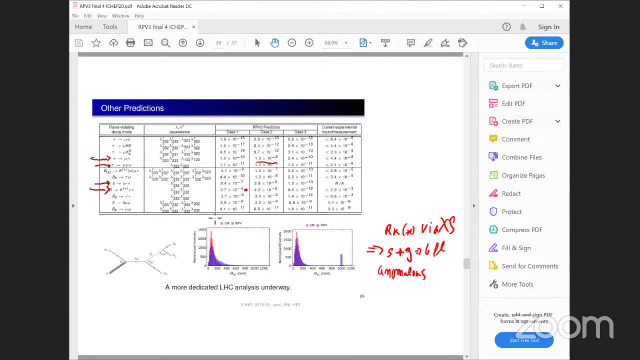 of the anomalies, and that's what we are doing, and and that's the first table in the bottom below shows what you do, what happens. you're making no theoretical assumption. this is crossing symmetry, you see? uh, rklk star, which means um b quark goes to s quark plus di lepton. 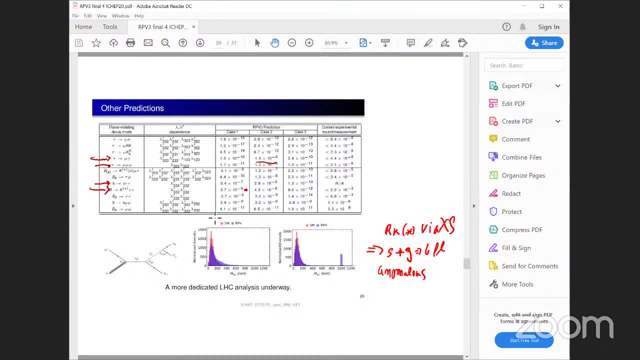 and that it automatically implies the reaction. the best reaction below um s quark plus gluon goes to b l, l and this should be anomalous. if the lscb result is correct, then in the atlas and cms and collider experiments they should be seeing an enhanced rate for this. 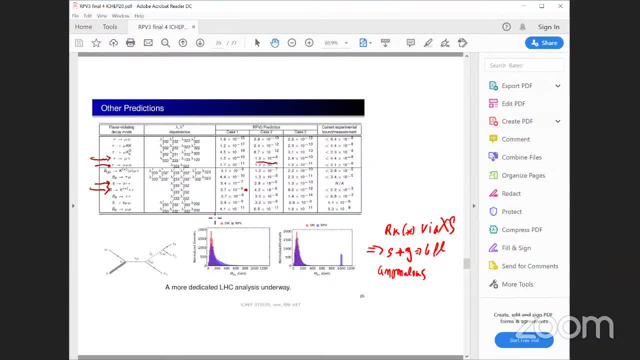 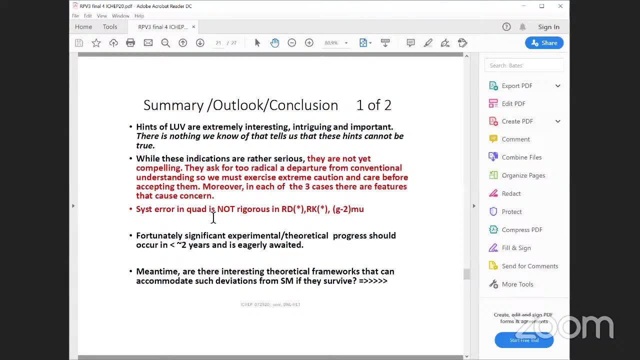 um b plus dilettantes, so anyway. so i'm going to summarize now. the hints of the lepton inversality violation are extremely interesting and intriguing, very important. there is nothing that we know now that says that these hints cannot be true, while these are rather serious. 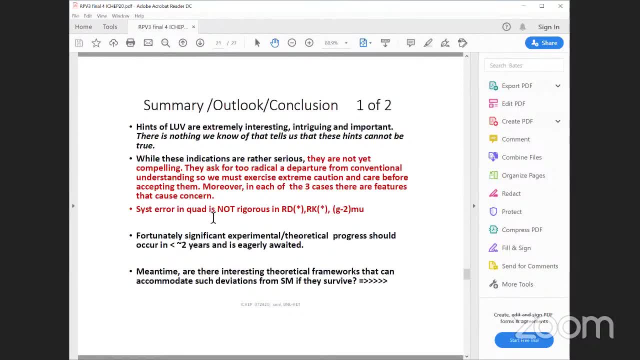 they don't appear to be compelling to me and in each case there are issues. for example, the rkrk star is just one experiment and g minus two is only one experiment and we have to wait for uh formula and one of the issues in all of these. 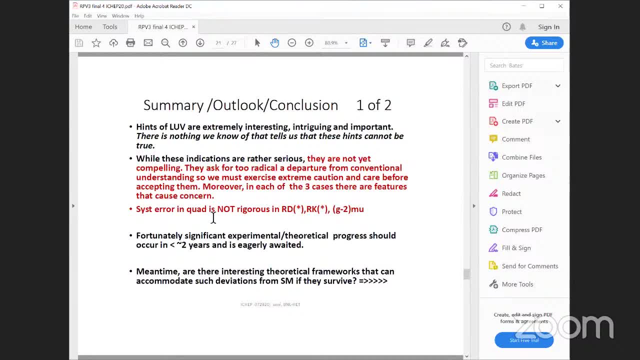 is that systematic errors are, uh, take, you know, taken to be in quadrature and i, i think, in all three experiments. this is uh, there's no rigorous theorem that you have to for to justify this. uh, in fact, even in my own experience, i have seen uh three or four cases in which, uh, you know, 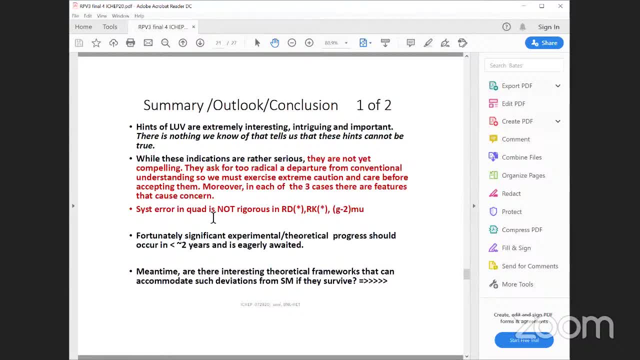 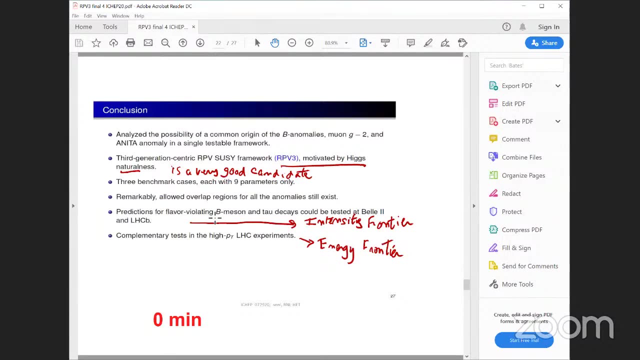 several, four different effects all line up in one direction: to cause an effect. fortunately, the progress will be made, both experimental and theoretical uh, in the next couple of years. so that's good. and then, as i said, um, the third generations. uh, assuming, assuming the third generation super partner, that the lightest is a very 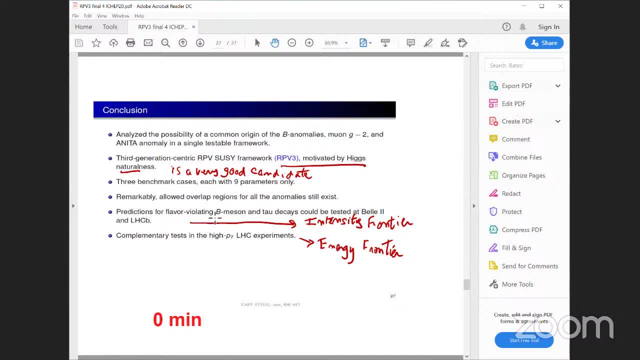 rpv becomes a very interesting candidate and it also gives us stability of higgs under radiative corrections. we showed three benchmark cases. each has nine parameters and a bunch of masses and we are. um showed some interesting signature predictions for the intensity frontier for b and target is the lepton flavor violation and they are complementary. testing our lec. 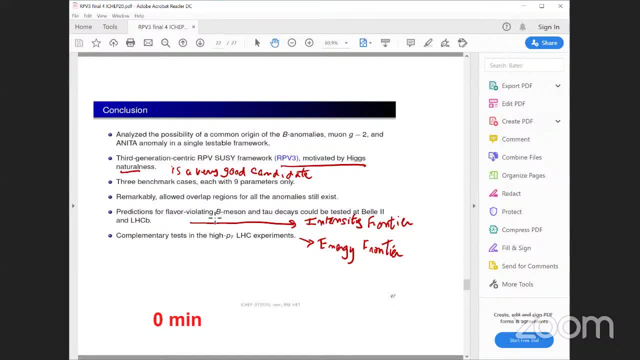 experiments and this. these are being followed. i showed one, and more will come in due course. i'm sorry about the phone. thank you very much. thanks a lot. so any comments or questions from the audience? i do not see any, okay, so i i just uh wondered because, okay, i missed uh the how, let's say, uh, this would explain the g. 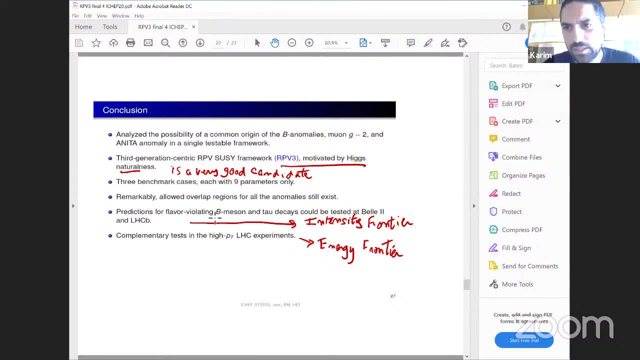 minus two uh muon anomaly, in the sense that what is exactly going in the loop? is there a muon to tau contribution or there is a uh supersymmetric particle? yes, so the muon goes to third generation b, for example. you know, and yes, okay, okay, rpv, there are things like that will happen, you know. 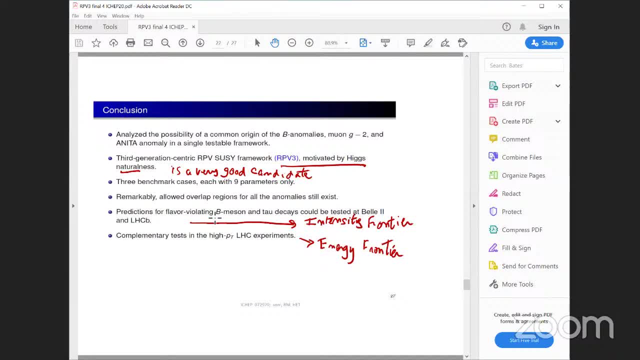 there are many graphs, and one of them then will be um lepton changing to uh, to to quarks and things like that, okay, okay, can i ask a question? sure, sony, can you also calculate the case of kaion's, not only b, with the same model, the same parameters? yeah, this is a very 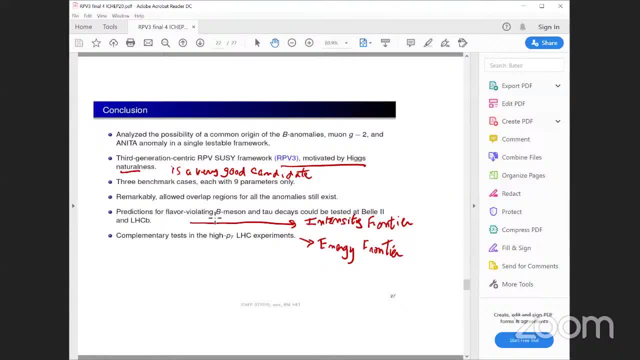 good question. i'm glad you asked. yes, you can do that and this is i was mentioning in some. in one case, uh, in fact you can. you can ask what happens to um k to 2 pi and epsilon prime and all that. of course, the setting here is suggest, uh, the the effects will be smaller. but you know there is. 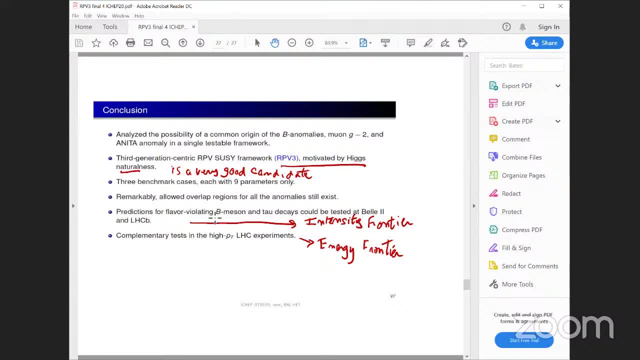 wealth of information and, rather than making a theoretical assumption, one can use that uh to to put better constraints. unfortunately, it takes time and our hands are full and you know this already took three years. someday, uh, it's. it's a very good question. we are trying to follow it up. 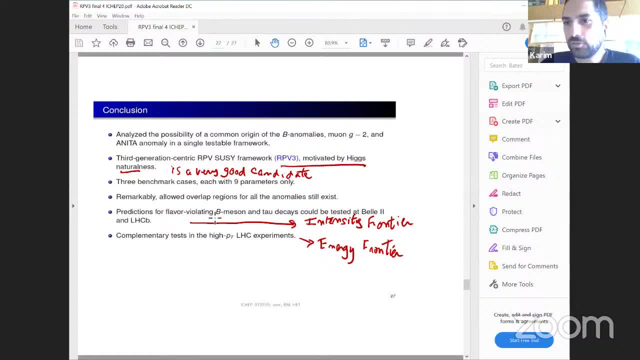 yeah, i agree, would be very nice, especially since there are also some uh- i mean count- experiments running uh also in the future. so it would be very interesting to have uh also that uh predictions, okay, uh, so maybe we can go on. if you have other comments or questions, 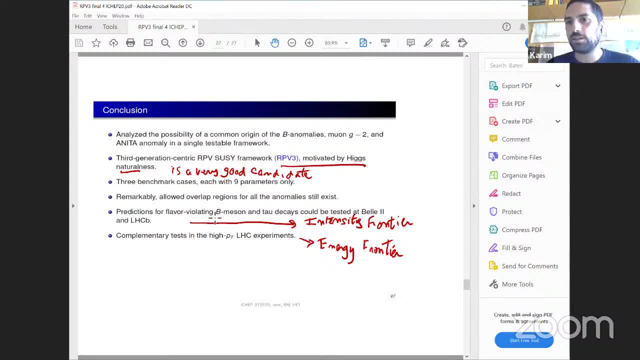 of course, as always, please uh use the matter most channel. so now the next talk uh is by alexey sividanov on the tau mu lepton flavor university universality in babara. hello, do you hear me? yes, could the previous speaker unshare yes screen. 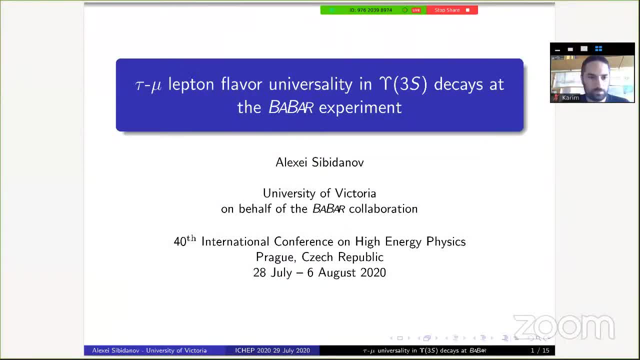 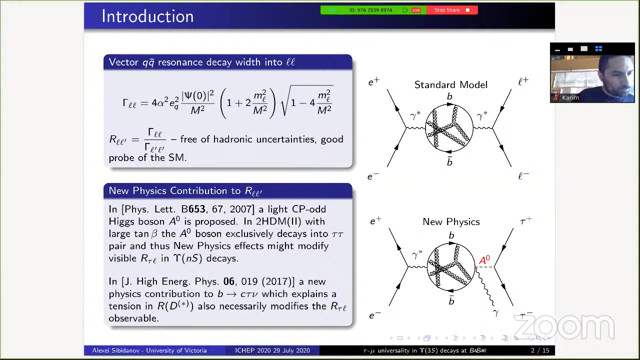 do you see spikes? yes, okay, today i will talk about uh tau mu, lepton, flavor universality, which is the one of the most common stoichiological newsperoads, or we call it the tectonic tectonic. what's the difference between the two? 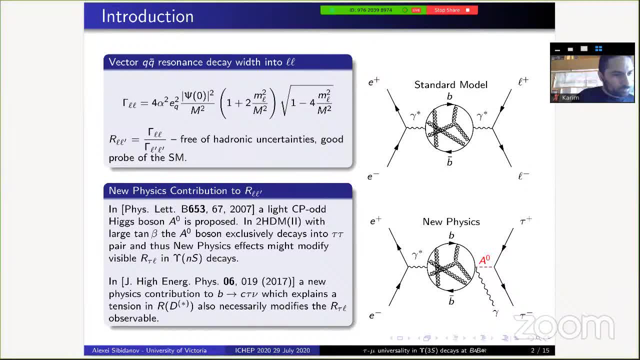 well as we have to understand this. so, for example, with the with, with the babara experiment: uh. in the babara experiment, uh, the ability in epsilon 3s decays: uh. And the width of this resonance was known since standard model exception, which is shown here. 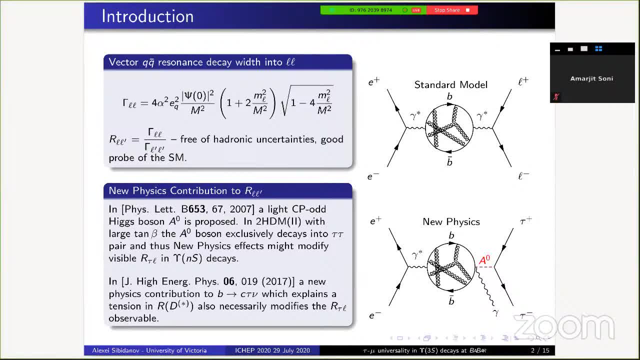 And so it's very clean and theoretically very well calculated. And so any deviation from this and ratio of those of those widths into different species of leptons are very well known and free of Hadrony uncertainties. So, and any deviation to this ratio, 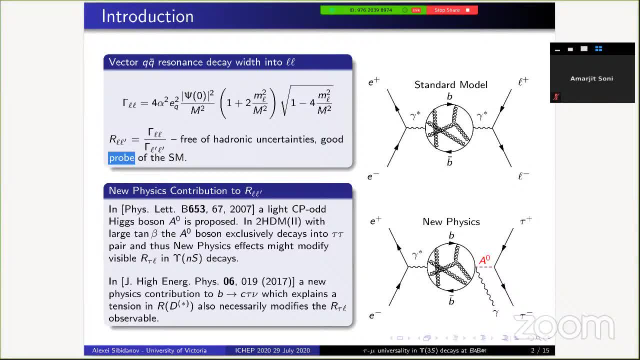 from the standard model prediction can give hint about new physics contribution. For example, in this work you can see that we have light CPO at Higgs boson And in this model is large tangent beta and this A0 boson exclusively decays into tau tau. 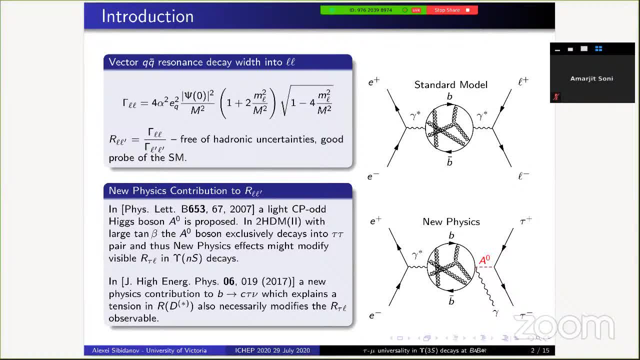 And thus, in presence of new physics, this ratio R tau mu will be enhanced And also in this work, new physics contribution to B to C tau nu, which explains tangent in R d star ratio, also necessary modifies R tau mu or tau E observable. 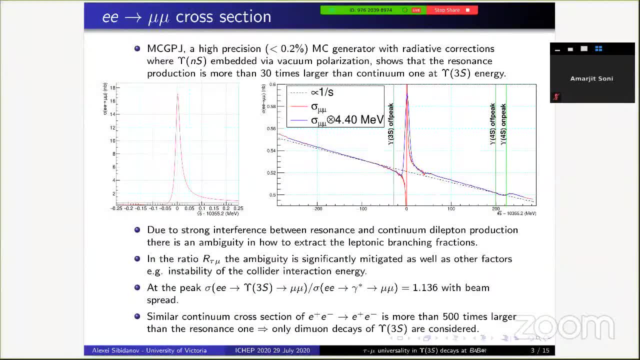 So why we are measuring R tau mu, not E R tau E? Here we can see a cross section of E plus E minus two mu mu, So you can see that at the peak it is about 30 times larger than a continuum production. 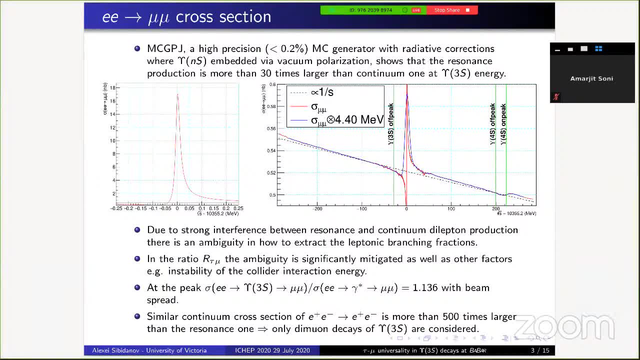 However, we have E plus E minus two mu mu. So you can see that at the peak it is about 30 times larger than a continuum production. This is because E plus E minus collider and we have beam energy spread. So, and this beam energy spread. 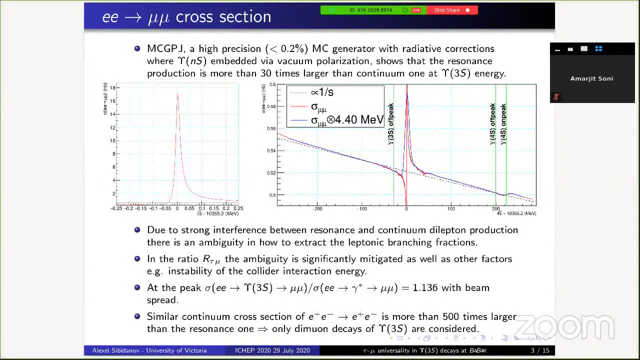 we have this picture here, So it's only a 15% larger than continuum production And similar continuum cross section for E plus E minus. three plus E minus is more than 500 times larger, So in this case only perovian production. 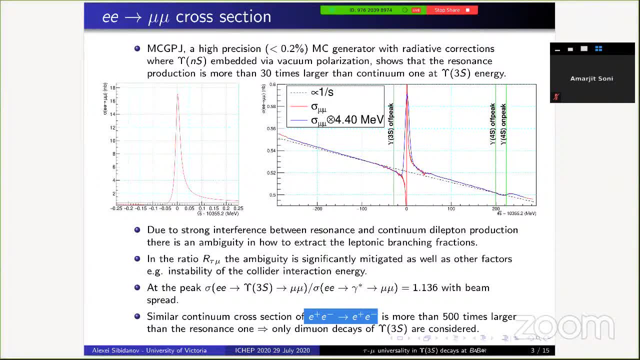 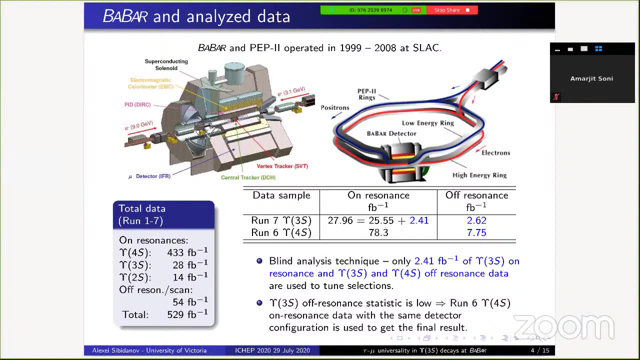 is possible to extract orợ, but I mean the case of epsilon 3s is possible to extract. so data for this analysis were collected at the babar experiment and the babar experiment operated at this dates at step 2 collider at slack and we use data from run 7 about 28 inverse hemtobarn on resonance and 2.6 inverse 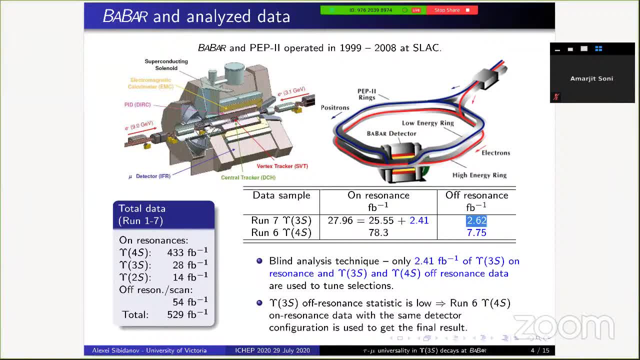 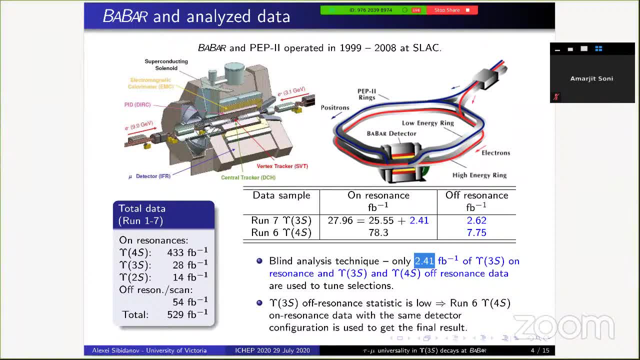 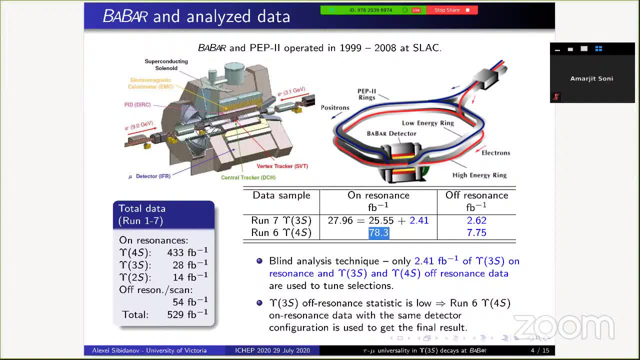 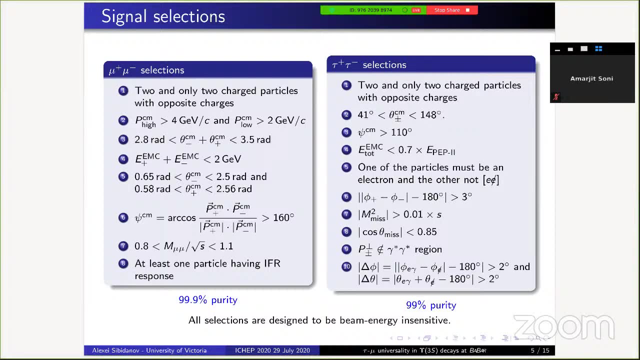 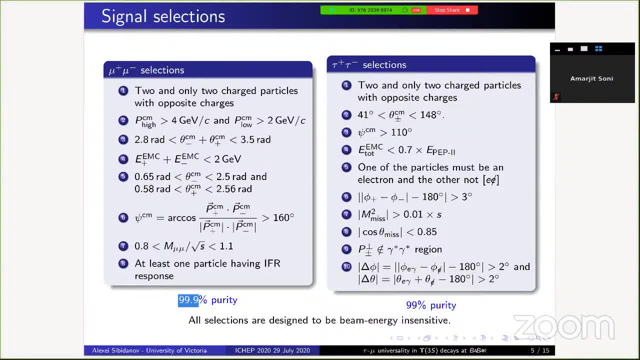 it doesn't have such obvious kinematics in the reconstructed kinematics in calorimeter. so a main feature of this analysis that we require that one particle have to be identified as an electron and other shouldn't pass or must not pass such electron identification procedure. so it's like electron and not electron. so it suppresses a lot of backgrounds. this. 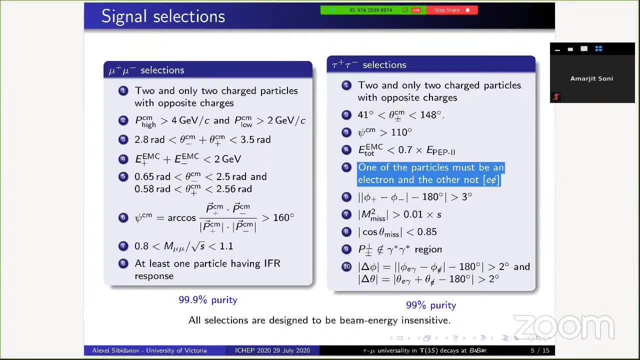 condition and with this we have 99.9% purity and all selections are designed to be beam energy insensitive, since we are trying to employ also epsilon 4s, which is about 300 muv higher energy. so we performed Montreal selection efficiency correction, which is shown here. so 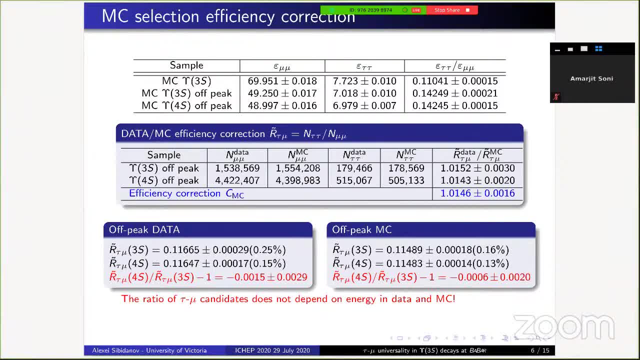 we did this on using only off-peak data in in off-peak y3s and off-peak y4s data and you can see that this very nice agreement between two, two data sets and we can apply such correction. so and conclusion, that this ratio of tau mu candidates does not be. 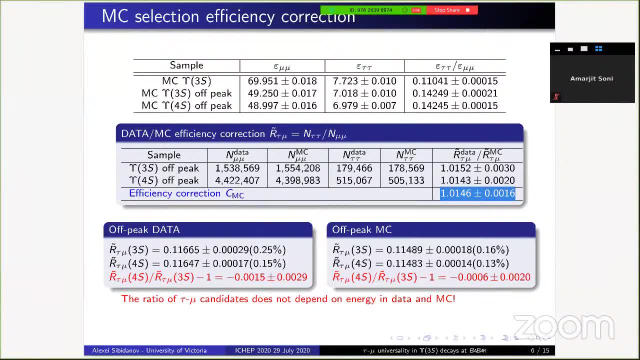 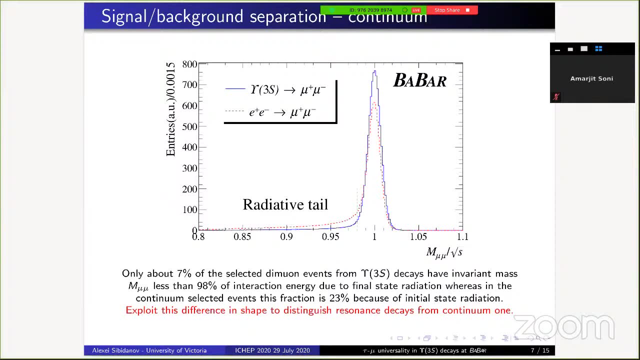 dependent on energy in data and Monte Carlo. so we can safely apply this correction to our on-peak analysis. so, and how to separate our continuum production and resonance production of muons. so we can see on this picture that here you can see simulation of epsilon stress to new mu and you can see that radiative tail due to 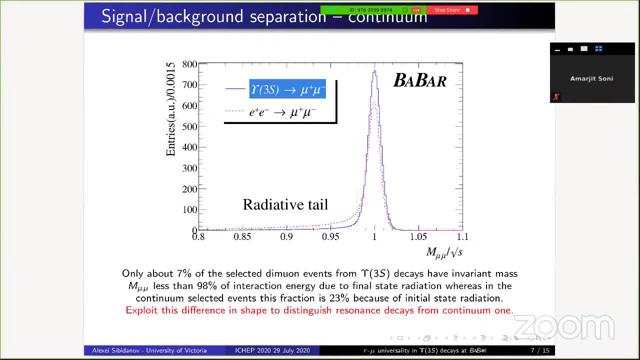 initial state radiation is highly suppressed in these decays, whereas for continuum production, you see that this radiative tail is much more prominent. and since babar detector has had excellent momentum resolution, we can exploit this difference in the radiative tail. so, and so you can see in numbers, because only seven percent are below three sigma resolution. 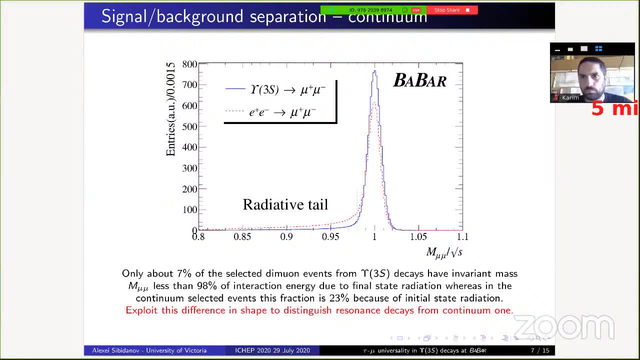 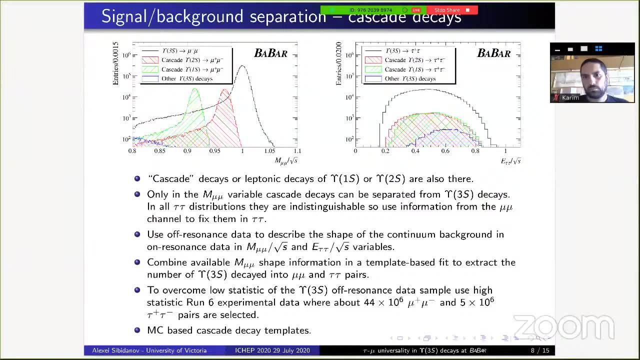 and whereas for continuum production about 23 percent of events have invariant mass less than three sigma resolution. another background is so-called cascade decays. when epsilon 3s decays, we have a decay chain where finally we have epsilon 1s or epsilon 2s, which 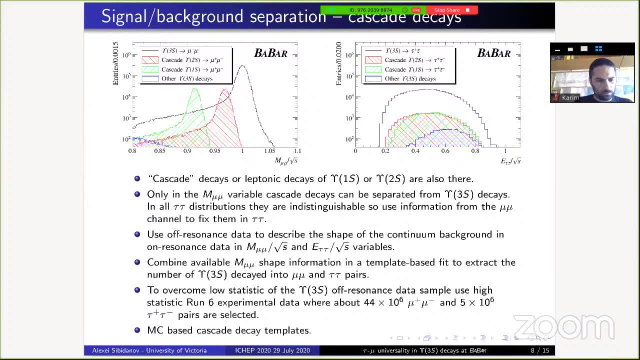 consequently decays into lepton pair. so in this case you can see that such decays are visible only in damion mass distribution. so we can fix amount of such events and assuming lepton flamer universality for epsilon 1s and epsilon 2s decays, we can somehow subtract them from our tau tau sample. 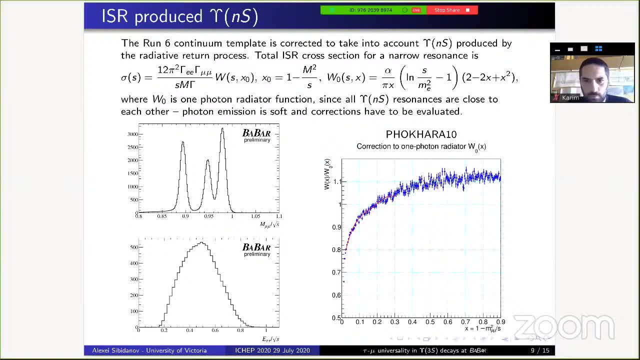 so another uh background is isr produced epsilon and s, so we use uh epsilon 4s data with so and this template contains also isr produced epsilons, so which are shown here. this is uh, our uh simulation. uh, we used fakara 10 to estimate this radiative function. 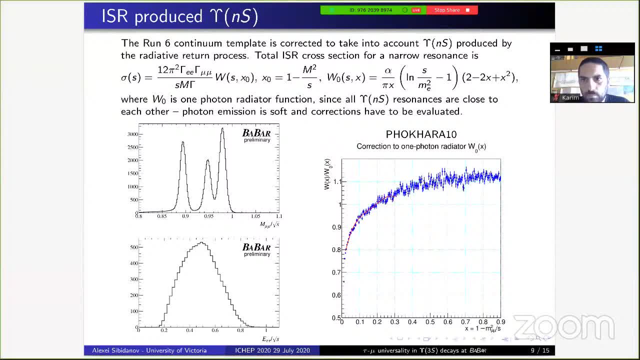 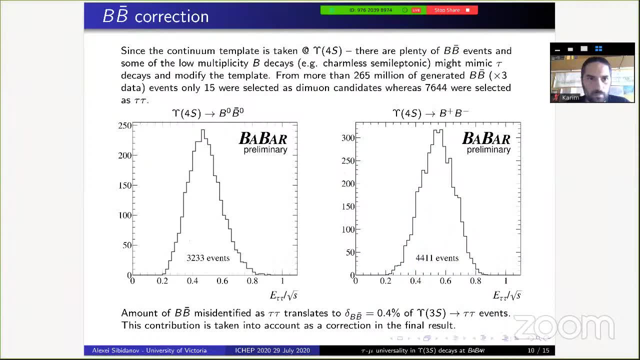 and uh and subtract such a background from our continuum template histogram. also, since we use uh, the uh epsilon 4s data, we have also bb bar contribution, which in case of new debut uh diamond production is negligible, but but for uh, for tau, we experience a particular4509. 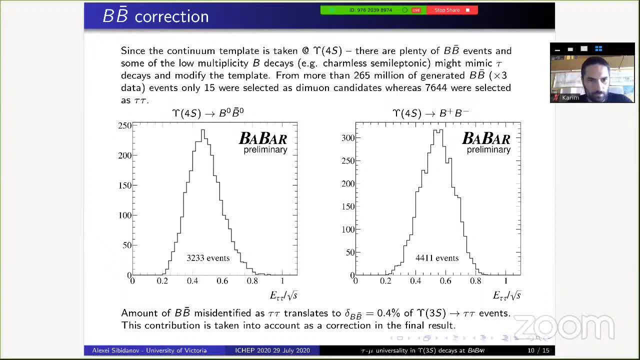 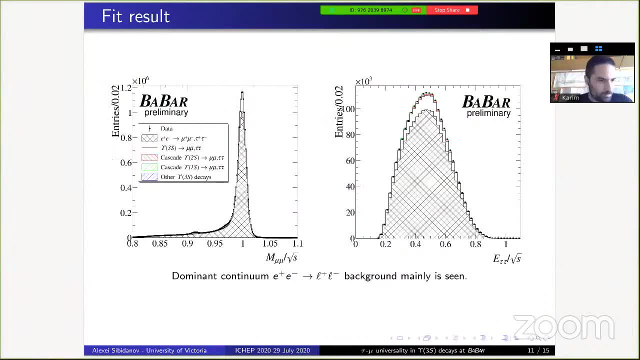 calculated possible contribution and apply this correction of 0.4 percent, which is quite small, so now you can see the fit result to the invariant mass distribution and to measure energy in the detector for tau tau and so and minor contribution. as you can see, this is crosshatch histogram, which corresponds to continuum production of muons and tau tau. 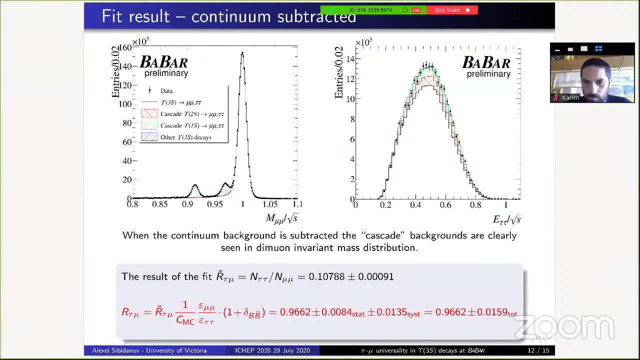 on this picture. you can see already continuum here subtracted and you can clearly see resonance peak and also cascade decays shown here. and also you can see how well we describe our energy deposition in the detector, measured energy deposition and the result of the fit shown here, that this ratio- number of tau, tau to number of 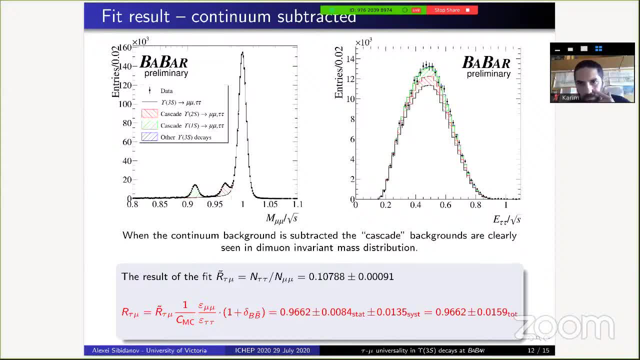 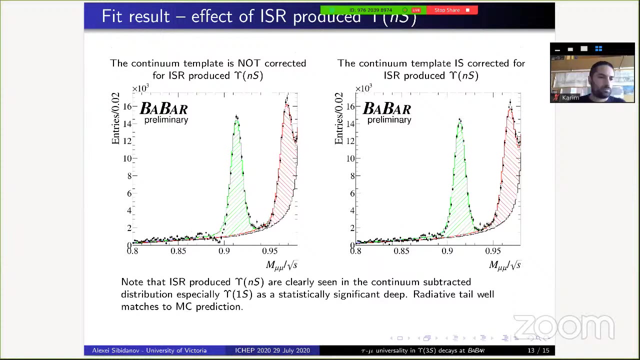 muons is shown here and this translates to this numbers shown in red and you can see that statistical error is quite small, less than one percent. so here you can see a result of isr produced y and s. so on this histogram you can see that continuity plate is not. 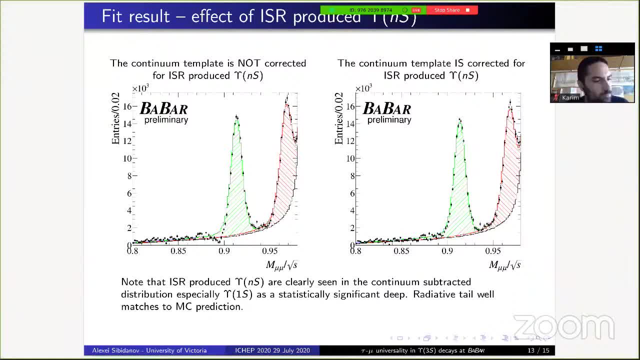 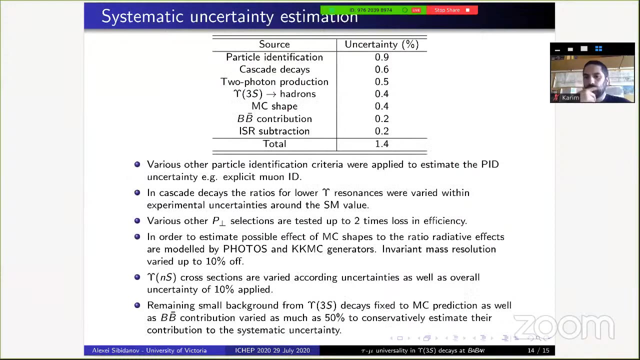 right for isr and you see this dip here and also this dip here, whereas this is isr correction. you can see very nice agreement between two plots. so systematic uncertainty estimation is shown on this slide. so minus the particle identification is shown on this slide. so minus the particle estimation and the rest are. 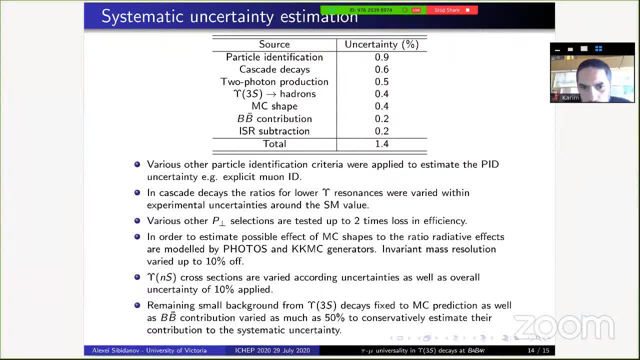 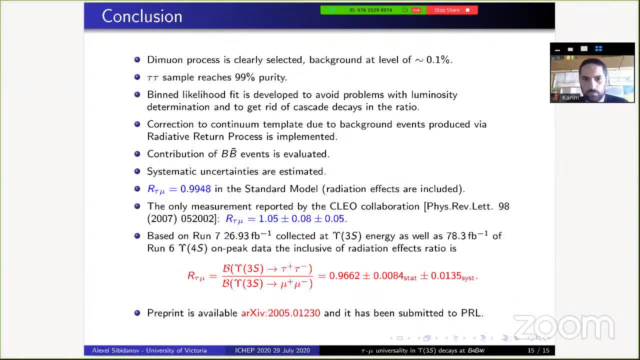 quite small and in total we have 1.4 percent total uncertainty. so here is a conclusion. so this analysis was done using bar data collected at y4s and and y3s resonances. We set up our selection procedure which yields finally background level at less than 0.1%. 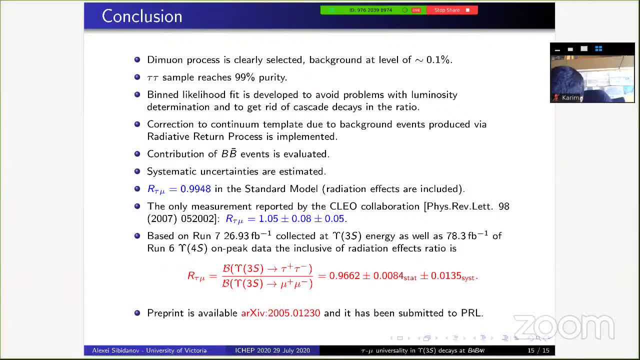 for mu mu and less than 1% for tau tau sample. We also developed a correction to our continuum template to exclude radiatively produced ipsilons And the result is shown here. final results shown here in red. And this result can be compared with the standard model prediction which is in blue here. and: 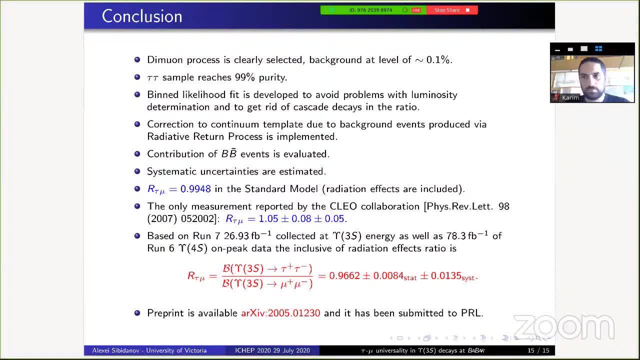 it is the only measurement reported by the CLIO collaboration And you can see that statistical uncertainty is 10 times better than the previous. the only previous measurement. Preprint is available. Okay, I, I'm done. Okay, Thanks a lot. 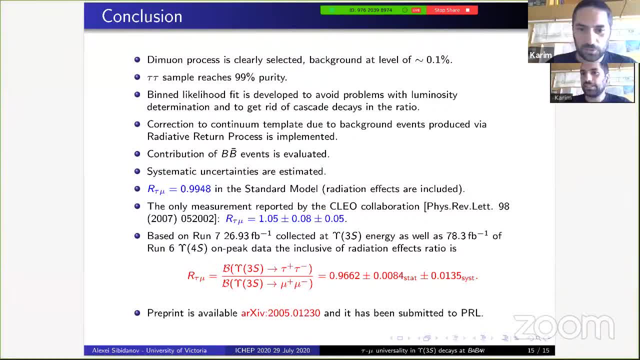 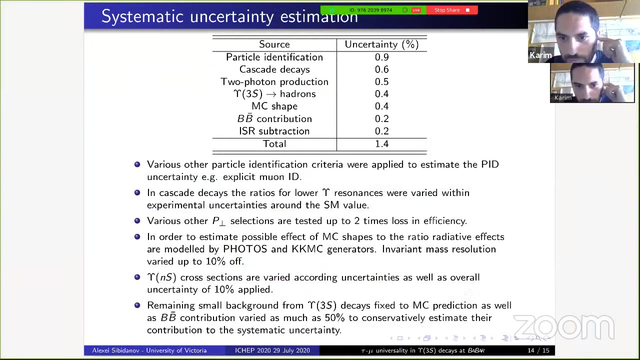 So any comments or question? I do not see any, Okay, So I well, I try to summarize, Okay, to follow as much as possible. so, basically, the what is the dominant systematics of your measurement, and I mean, do you have any plan on how to? 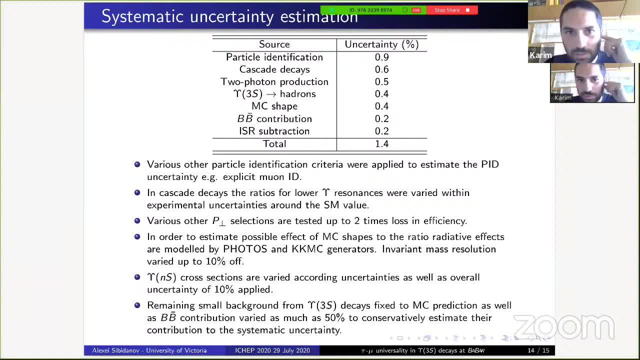 improve it or it's already. this is the mind. so identification so, and this particle identification is very hard to prove since it's limit of our knowledge- how we will model interaction with the materials detector. it's okay, I was wondering if, for instance, you can exploit the tau to mu decay. but this is 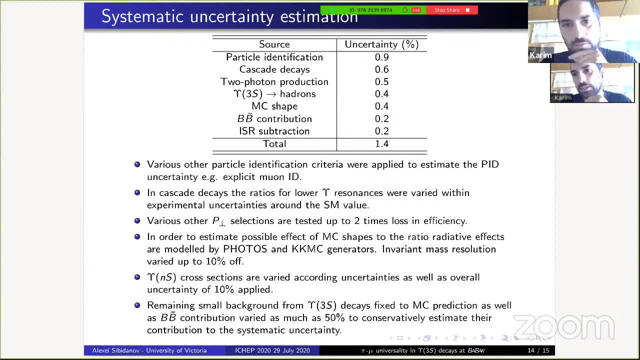 probably too complicated. yeah, because already all such tricks already you're exploring, exploiting this analysis, like all this Babar accumulated knowledge already in this analysis. okay, okay, thanks a lot. so I don't see any other comments or questions. in case you have some, please use the matter most channel and at this. 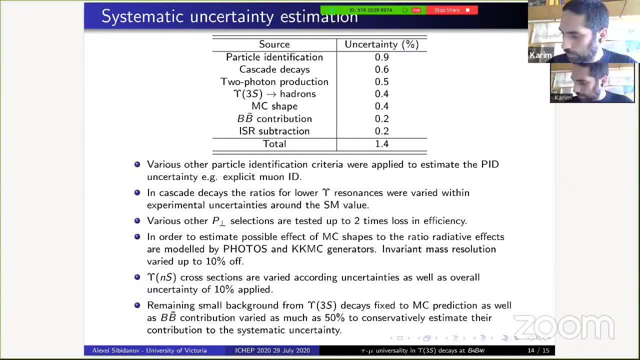 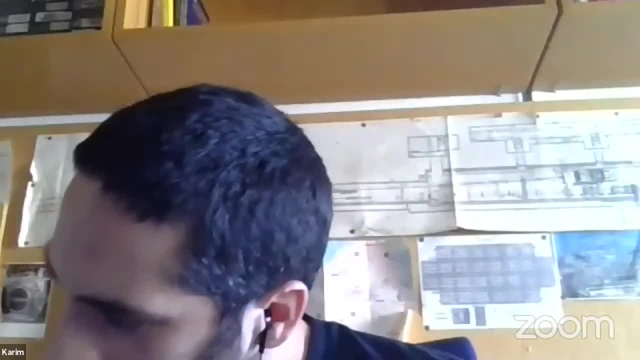 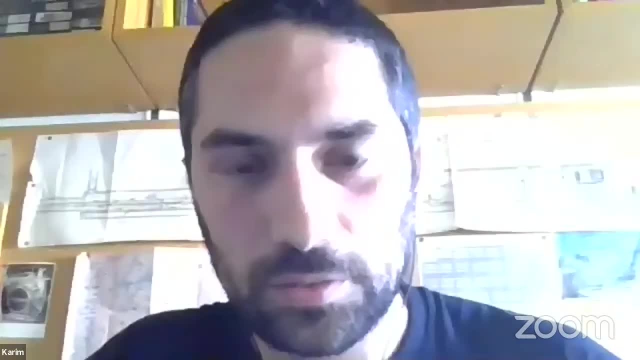 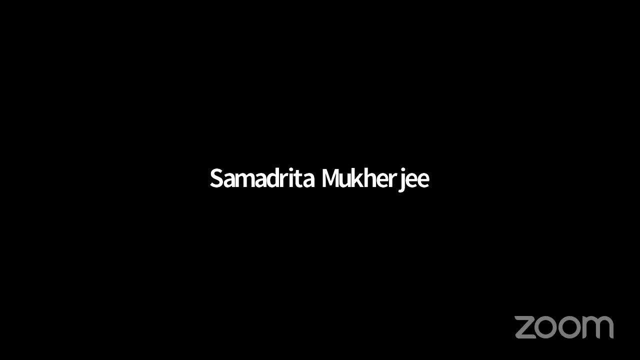 point. thanks again. I would move to the next talk. so, Samadrita Mukherjee, so, and the talk will be about probing. let them favor violation in minimal, supersymmetric, supersymmetric standard model. yes, can you hear me? hello, yes, yes, so let me share my screen and 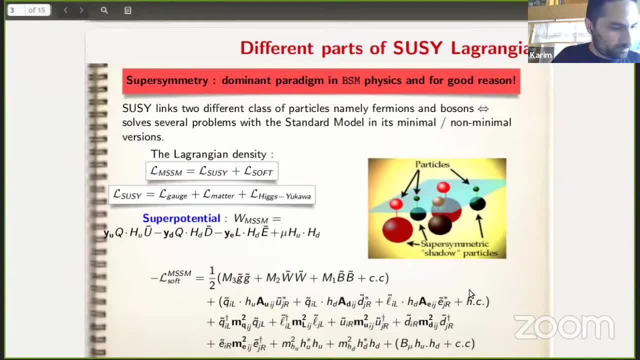 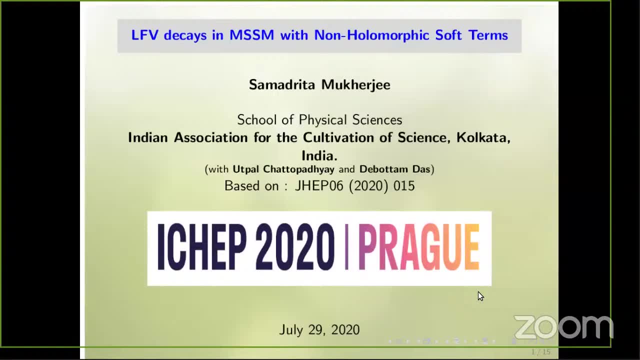 you, you, here you go, you, you, please. I hope you can see it. yes, yes, we can. so thank you very much. good morning, good afternoon and good evening to the people from all over the world, and we will be discussing leptin flavor violating decays in MSSM with. 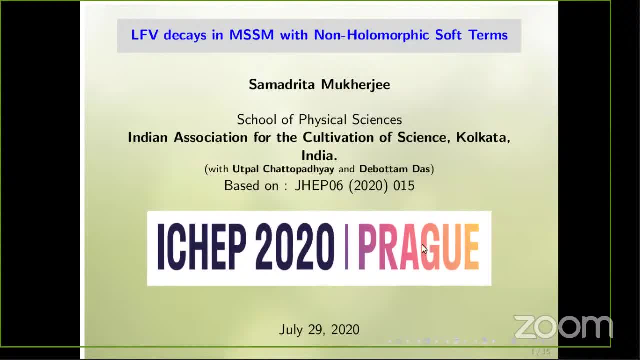 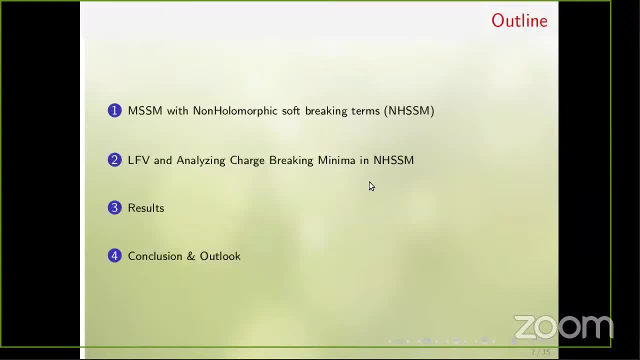 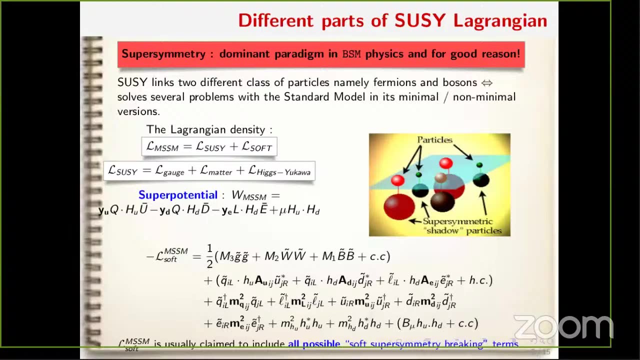 non-holomorphic soft terms, and this work is done in collaboration with Professor Upal Chattopadhyay and Professor Devuttam Dash, and based on this work, overviews are outlined in this slide, so let's see how it goes. among the many models of BSM physics, supersymmetry is a well-celebrated one for many years. 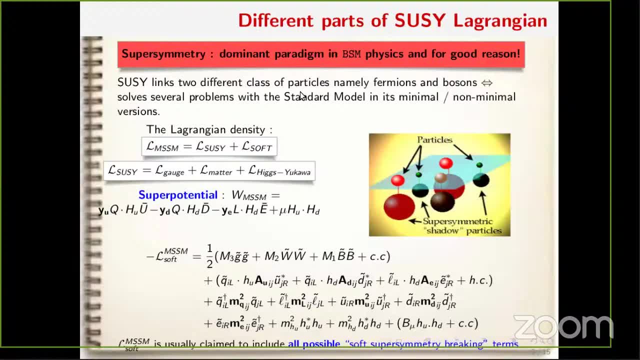 and since it's solved the hierarchy problem supported by the measurements of gauge coupling, strains consistent with precision, electric data and fixed mass. of course, now Susie links different class of particles known as bosons and fermions. now it must be badly broken in nature and in general, and Susie breaking Lagrangian consists of: 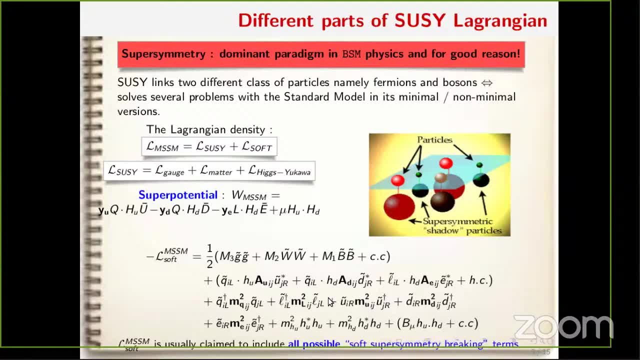 these gaugino mass term, analytic and non-analytic squared mass term and cubic scalar couplings. now, MSSM is usually claimed to include all possible soft Susie breaking terms, that is, the terms which plead for partners, but do not remove the protection against the quadratic divergence. 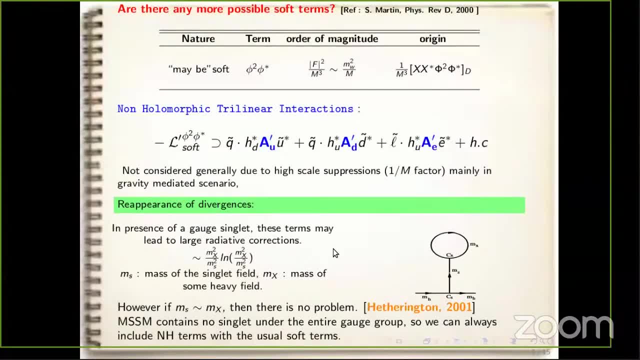 to the scalar mass, uh, but, however, are there any more possible terms? in a most general framework, it has been shown that certain non-analytic cubic scalar couplings also qualify as soft terms, that is, soft Susie. breaking sector is extended to include this phi square, phi star type of interaction. 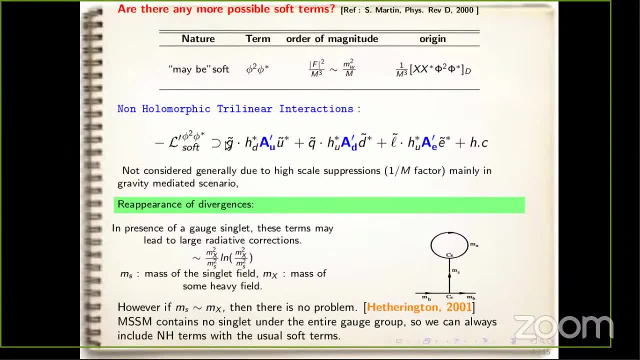 taking these interactions in the Lagrangian density we have this: q tilde times, HD star times au prime u tilde star and for the down type, squares and slepters and their Hermitian conjugate. now these terms are not generally considered because regimes. Firstly, there is high-scale separation. It comes from the 1 by m prefactor here in the 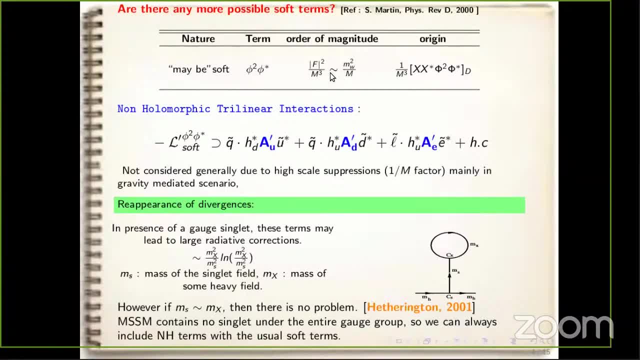 order of magnitude of these terms, which can be very large for gravity-mediated case as for the CMSSM type of scenario, And another is reappearance of the divergence What happens in a presence of gauge singlet, which is singlet under the overall gauge group. there can be quadratically large. 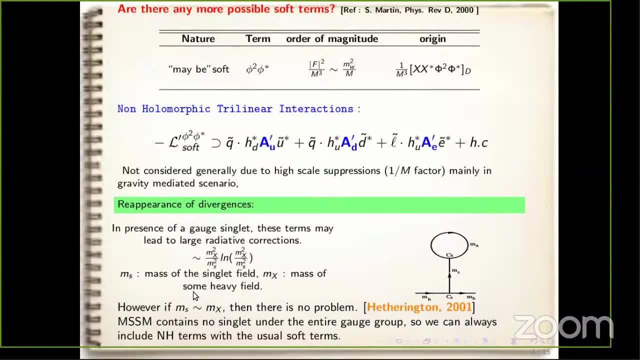 loop corrections depending on the masses of singlet fields. But however, the mass of singlet field and the chiral supermultiplate is of the same order, then there is no problem. And of course phenomenological minimal supersymmetric standard model evades these two reasons to not. 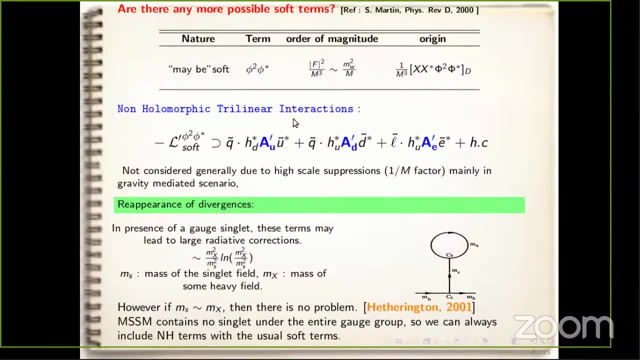 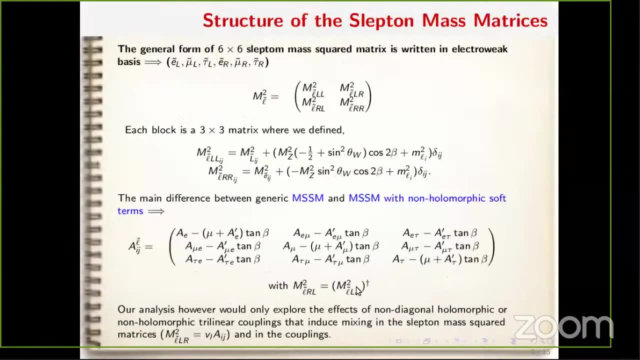 consider these terms. There is no separation, as we are considering all our input parameters in phenomenological scale, And there is no gauge singlet under the SU3 crosses, So there is no question of reappearance of this bad divergence again. Now let us see what happens. 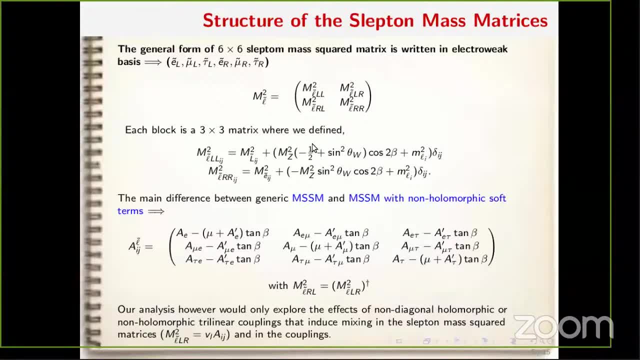 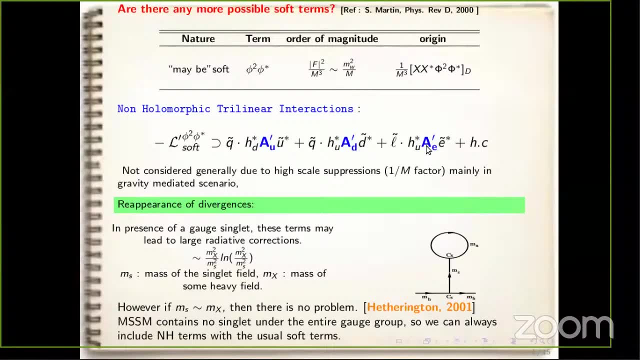 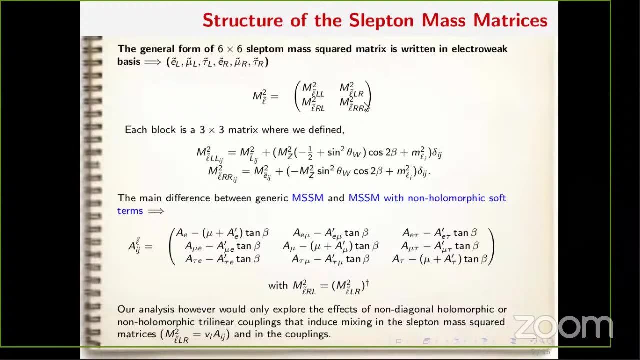 to the structure of Slepton mass matrices. if we consider these 5-square, 5-square terms, that is, this trilinear, non-holomorphic Slepton mass terms in the mass matrices. We are concerned with the mass matrix in the Slepton sector actually, So the general form of the 6 by 6 Slepton. 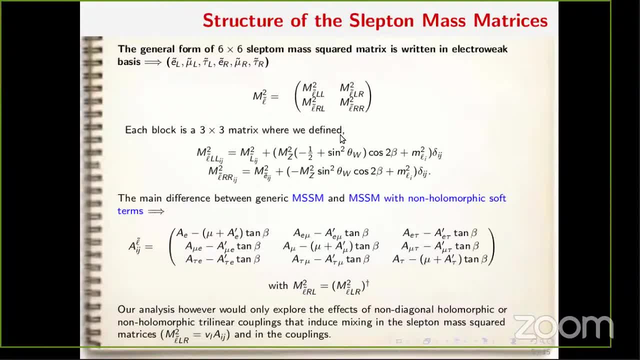 mass square matrix is given by this, where each element is a 3 by 3 block. The non-holomorphic trilinear coupling modifies mainly the Slepton left-right mixing. Here we have written the trilinear term explicitly And, as you can see, the term is here A minus mu plus A prime tan. 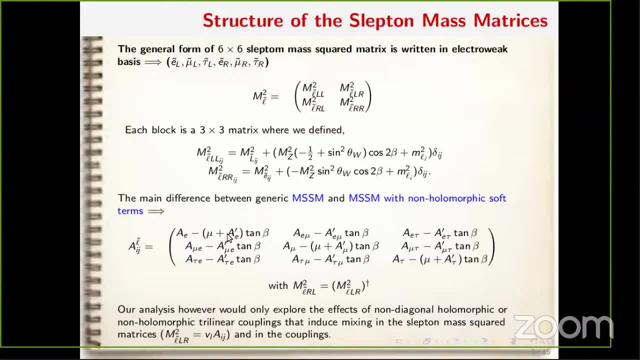 beta. In MSSM it was only A minus mu times tan beta. So both the diagonal ones and the off-diagonal ones are getting changed by this, A prime ij or A prime ii type of interactions. So our analysis, however, only excludes this non-diagonal holomorphic and 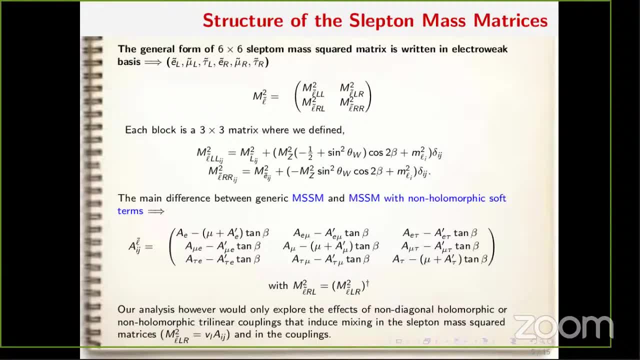 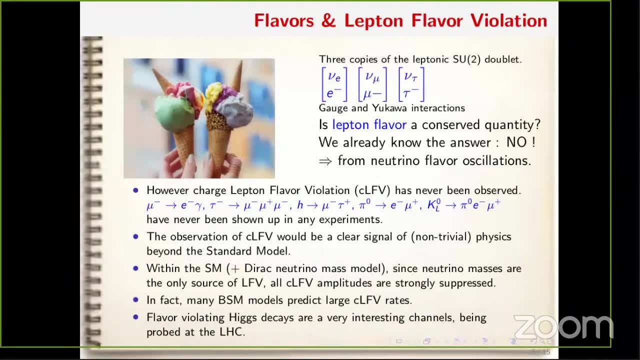 non-diagonal, non-holomorphic trilinear couplings to study the Slepton-Slevor violating observables. So what we know about the Slepton-Slevor violation? The observation of oscillation between neutrino flavor eigenstates implies that Slepton family. 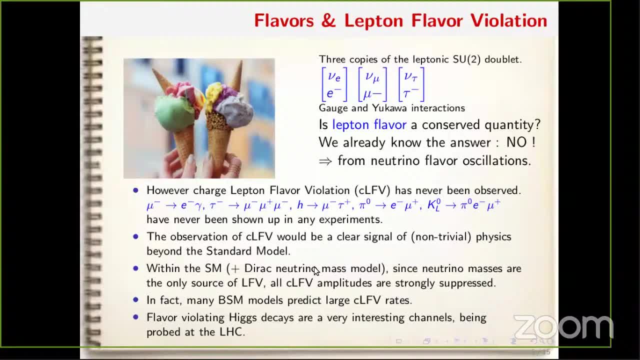 quantum numbers are not considered And, as a consequence, one can also explain the flavor violation in transition between charged Slepton. However, charged Slepton violation, flavor violation has never been observed in any experiment, which would have been a clear signature of the beyond-standard model. physics Now results from these experiments, indeed constrain the 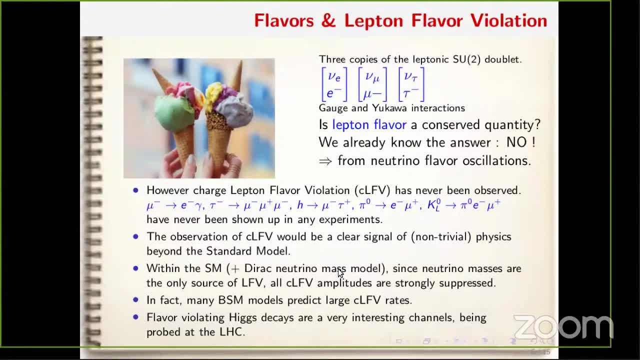 respective model parameters, And tremendous effort is currently being realized in to achieve unparalleled sensitivity to probe Slepton-Slevor violating decays at like Meg, Bell, Baber, LHCb and at all other experimental facilities. what is happening all over the world? 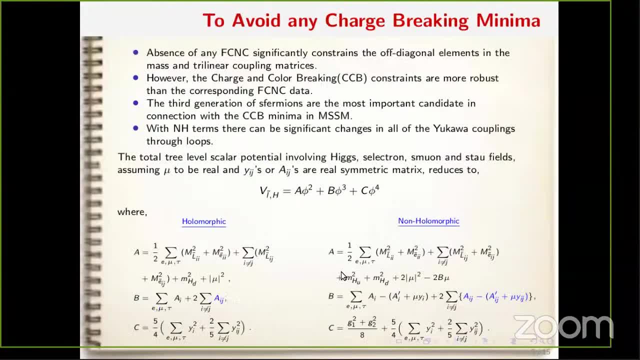 Now we will see that. we know that absence of any flavor-changing neutral current significantly constrain the non-sleptonic behavior of Slepton-Slevor. So we know that Slepton-Slevor is a non-sleptonic element and that Slepton-Slevor is a non-sleptonic element But charged and 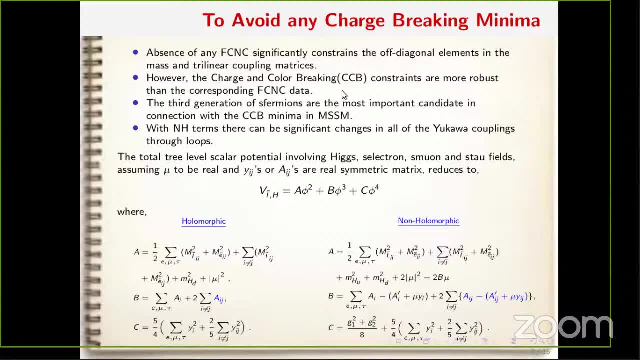 color-breaking minima aspects are more robust in this aspect. Now in the left-hand sector there is no color-breaking context, So we will study the charge-breaking minima here In a theory with multiple scalars, choice of desired electric one puts restriction on. 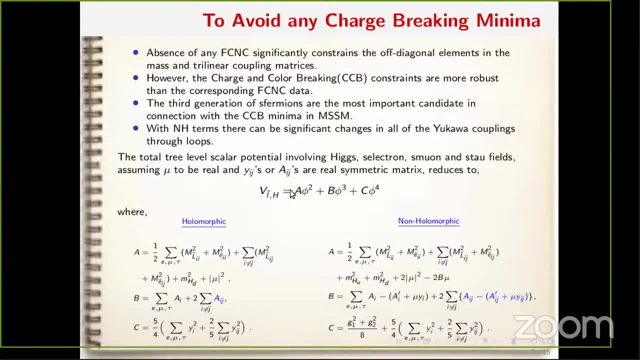 the allowed parameter scale. The total pre-level potential is given by this equation involving Higgs, electrons, muons, tau Efficient A, B, C for two cases are here. Please note the presence of both diagonal and the off-diagonal trilinear couplings in both cases. Now, considering all the three generations, 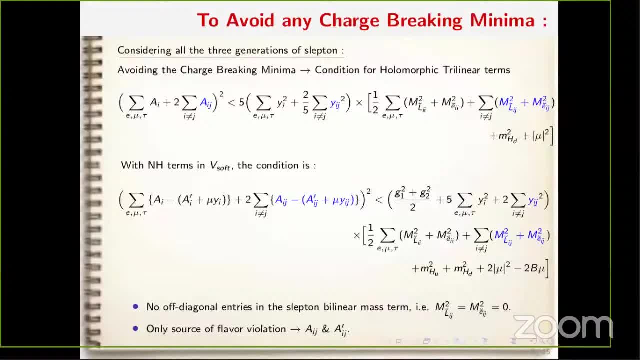 the condition to avoid any charge-breaking minima is derived as follows: For the first one is for the holomorphic trilinear couplings- Note the presence of Aij here- and the corresponding off-diagonal Yukova coupling element- And the one with non-holomorphic and holomorphic one is: 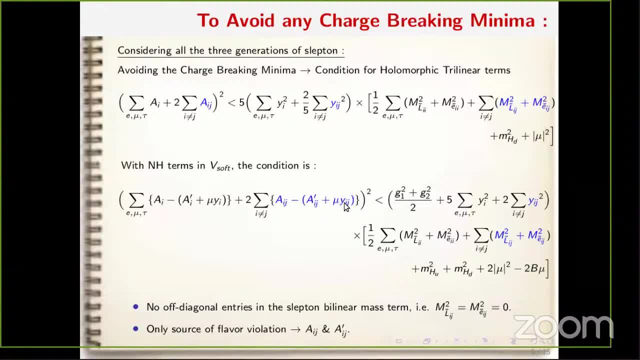 given by here. So Aij minus Aij prime mu times Yij is present, So in. okay, I will hurry up, So in, as I have five minutes more. So here in our numerical analysis, we will consider these: 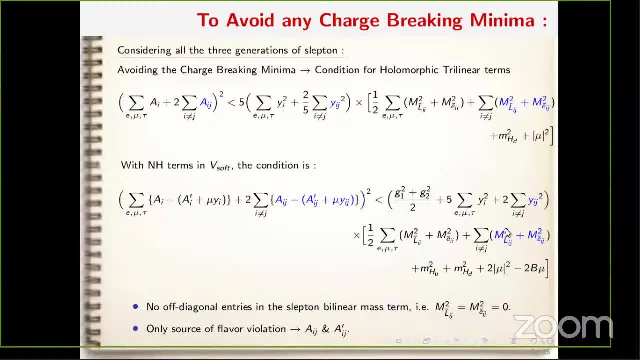 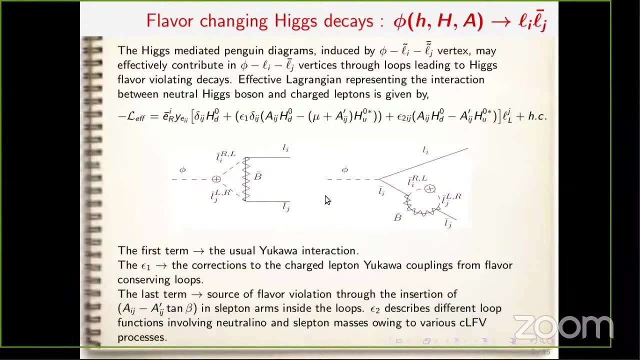 uh, bilinear, soft-square-square lepton mass matrices element to be exactly equal to zero. So whatever be the flavor violation, that will be due to the Aij and Aij prime. So let us see how the results come out. comes out to be Flavor-violating. Higgs stickers play a significant role for 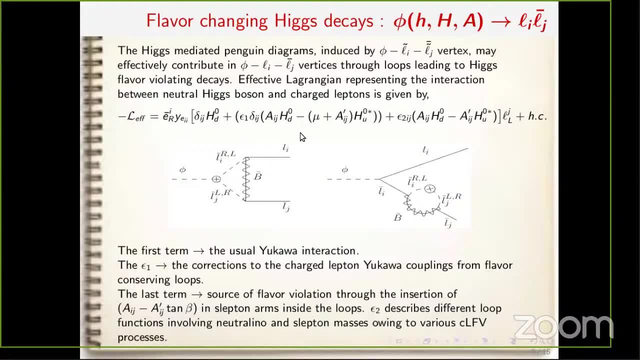 investigating lepton flavor violation. The effective Lagrangian-Phi-A-Li-Lg vertex has three parts. The first part is the lepton-flavor violation. The second part is the lepton-flavor term denotes the Yukova interaction, where epsilon-1 encodes the correction to the charged. 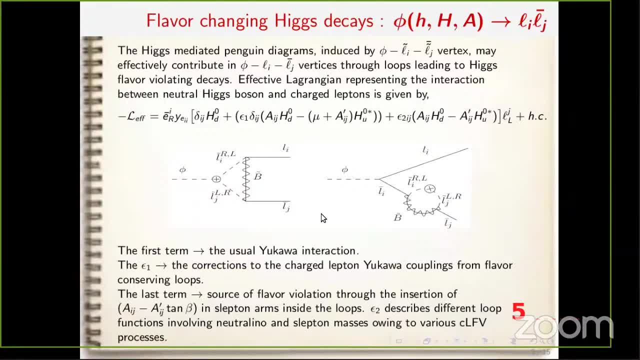 lepton-Yukova coupling from flavor-conserving loops- And the last term corresponds to the source of flavor violation- And epsilon-1 and epsilon-2 arise out of loop function involving neutralino and leptons. This effective Lagrangian essentially generates all the off-diagonal Yukova. 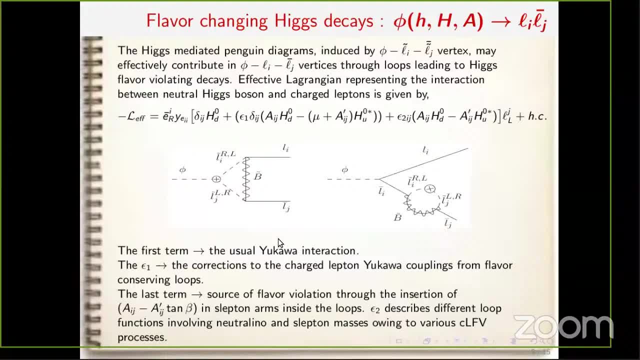 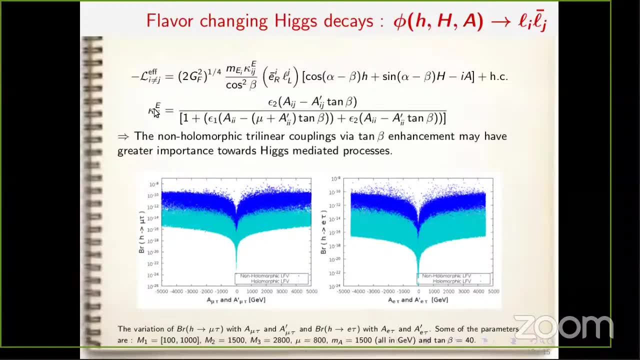 couplings radiatively in the respective trilinear coupling is non-zero. Now strains of physical Higgs boson to the leptons are given here with kappa ij factor. Typically dominant contribution comes from the Cp-even heavy Higgs and Cp-odd heavy Higgs which are evident from the factors in front of them. 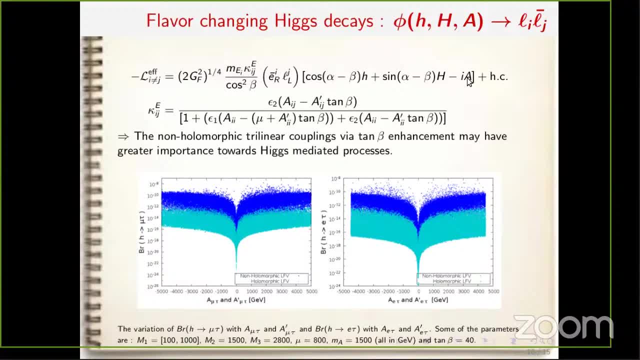 That is sine alpha minus beta in the decoupling limit is close to 1 and for Cp-odd heavy Higgs it is 1.. The scatter plot shows the branching ratio H2 mu tau and H2 e tau as a function of Aij in cyan and Aij prime in blue respectively, And appropriate non-Hodgkin's Higgs boson. and Cp-odd heavy Higgs are given here with kappa ij factor. Typically dominant contribution is from the physical Lagrangian essentially generates all the off-diagonal Yukova couplings. radiatively in the respective trilinear coupling is close to 1 and for Cp-odd heavy Higgs 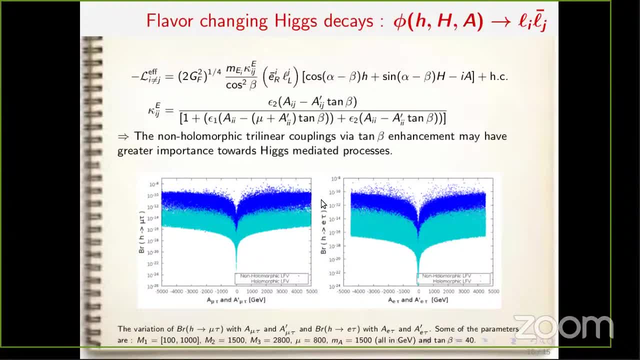 but the scatter plot shows the branching ratio H2 mu tau and H2 e tau is a function of Aij prime, in blue respectively, And appropriate: non-Hodgkin's Higgs boson and Cp-odd heavy Higgs b of the non-Hodgkin's Higgs boson and Cp-odd heavy Higgs b of the non-Hodgkin's Higgs. boson and Cp-odd heavy Higgs b of the non-Hodgkin's Higgs boson. So this is a non-holomorphic coupling that is in the blue. additionally multiplies with tan squared beta, leading to an enhancement by a factor of 10 to the power 3 compared. 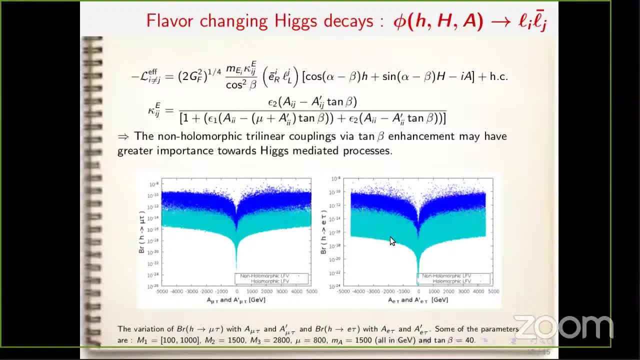 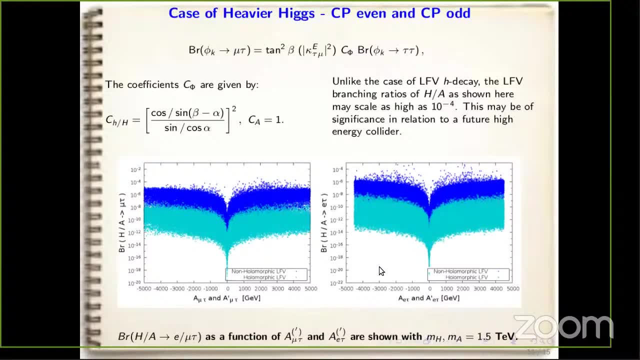 to the MS system values. As mentioned earlier, the heavier Higgs are dominant, one in the LFBD case for decoupling limit. Straight up the branching ratios are shown for 1.5 TV heavy Higgs mass. All points here satisfy the upper mass bounds for various masses which 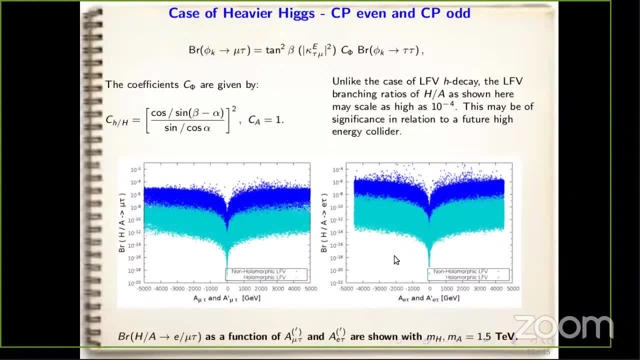 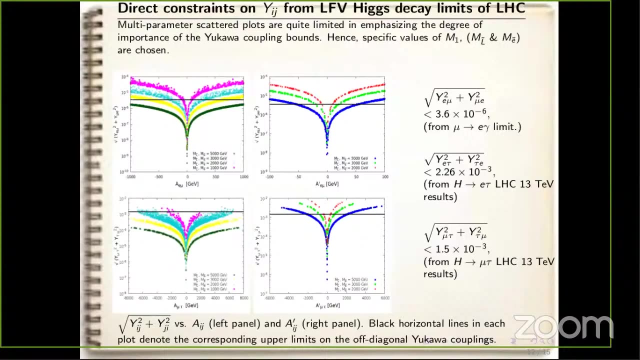 have been searching in the LHC the various LFBD case like mu 2e, gamma, mu 2, 3e and other flavor constraints and mass bounds from LHC and of course avoid deeper charge breaking minima than the electric one, Now with the identical U-cover couplings that MSSM inherits. 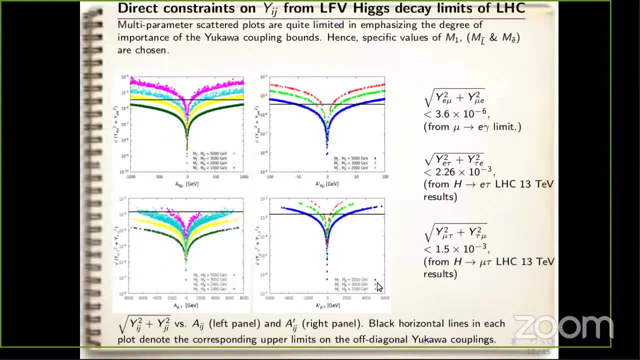 from standard model. we will use constraints of LHC on relevant off-diagonal U-covers to restrict the trilinear parameters. To draw this bounds we need to fix the neutral renewal and slip-turn mass at some fixed values. Clearly, the larger radiative correction are induced. 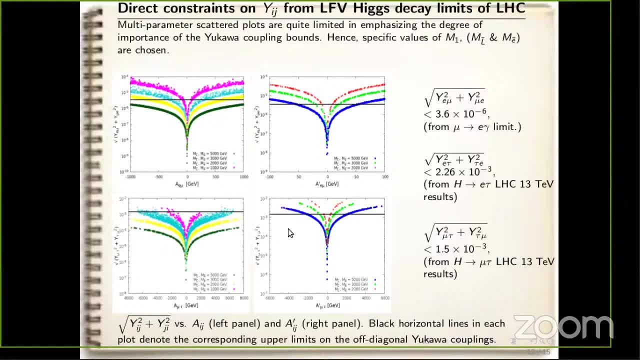 in the LHC. So we need to fix the neutral, renewal and slip-turn mass at some fixed values. So we need to fix the neutral, renewal and slip-turn mass at some fixed values. Clearly, we will use constraints of LHC for operator information as the 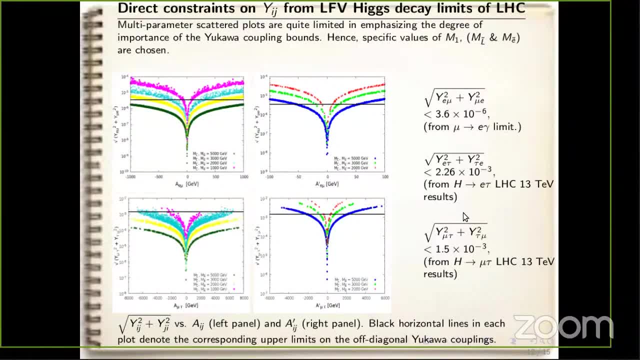 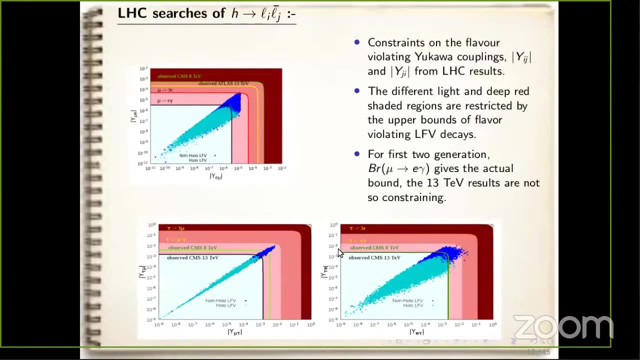 final stores into UV data And here you can see the extent of variation due to the non-holomorphic couplings is much more larger. Actually it is 10 to the power, 3 times larger. Now, with the understanding on how up-diagonal U-couple couplings can directly influence the 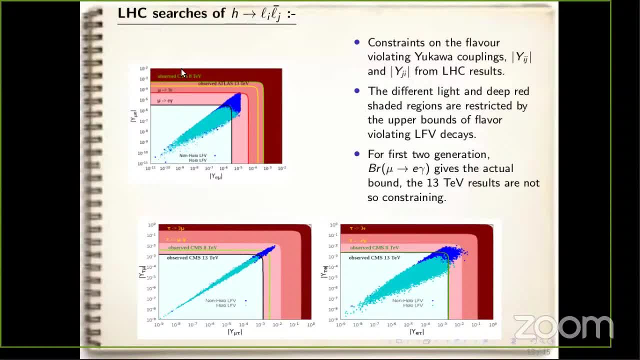 free rise of trilinear coupling. we have shown here the bounds in the mod YIG and mod YJI plane And here the different light and deep redsheds region are restricted by the upper bounds of labor, violating LFPT case. Again it is shown that for first two generation mu2 igama is the 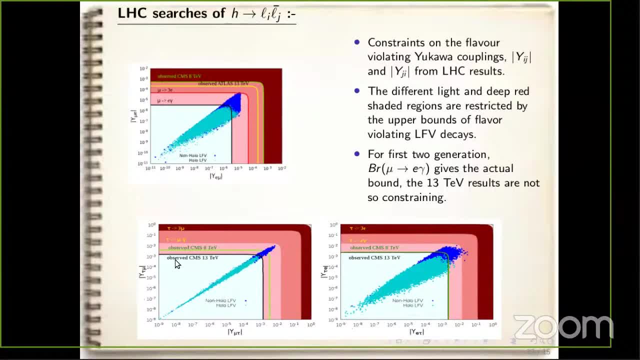 most constraining one And for the other two generation it is the CMS and ATLAS 13 TV data Blue points are derived from the non-holomorphic couplings And, as you can see, the large extent of non-holomorphic couplings are excluded from the 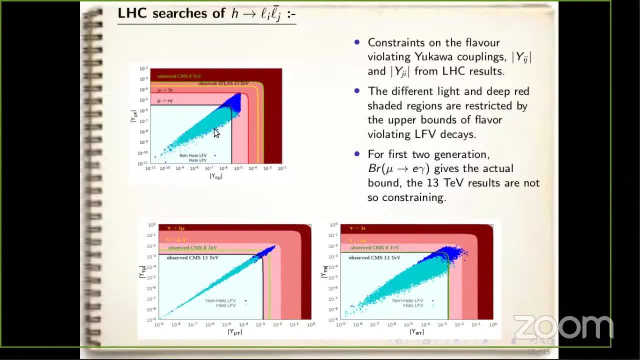 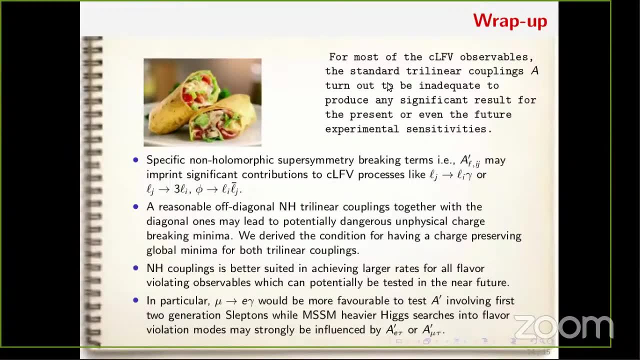 search of the LHC and null results from the mu2 igama. So let us wrap up quickly. For most of the charge, length and flavor violating observable, the standard trilinear coupling A, that is, the holomorphic one, turn out to be inadequate to. 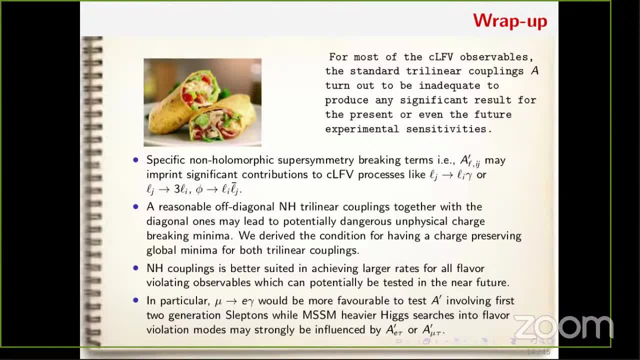 produce any significant result for the present or even the future sensitivities. So we have two class of. We have classes of non-holomorphic coupling. One of them is AIJ prime may influence significant contribution in these processes. A reasonable amount of half-diagonal couplings, together with 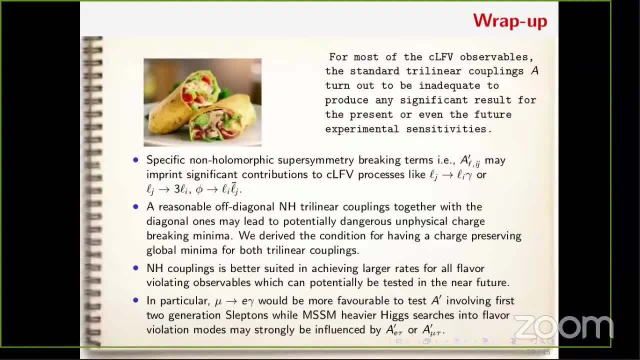 the diagonal one may lead to potentially dangerous charge-breaking minima And we derive the condition analytically to preserve the global minima which is charge-conserved And non-holomorphic. coupling is always better suited in assuming large rates than compared to the holomorphic. 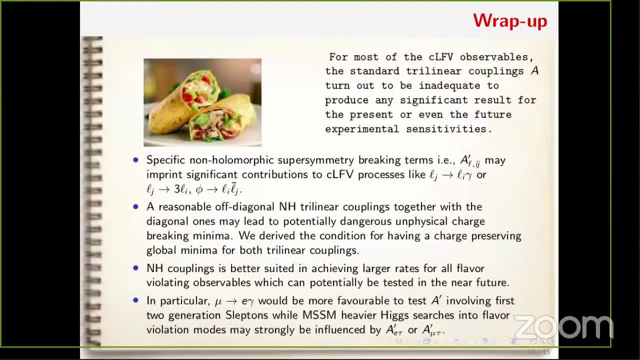 couplings And, as we discussed, from the results that mu2 igama constraint more favorable to test AIJ prime for the first two generations and the LHC limits are more favorable to test the second, third and first generation of diagonal couplings. So with this, 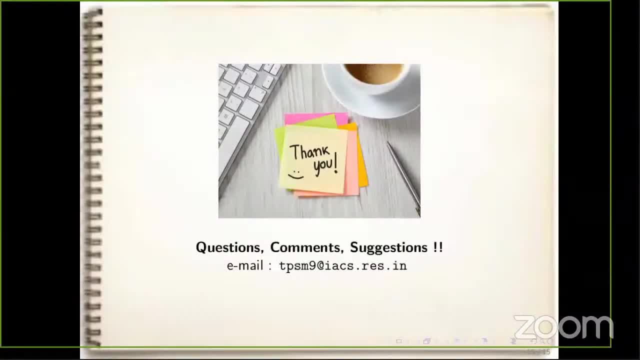 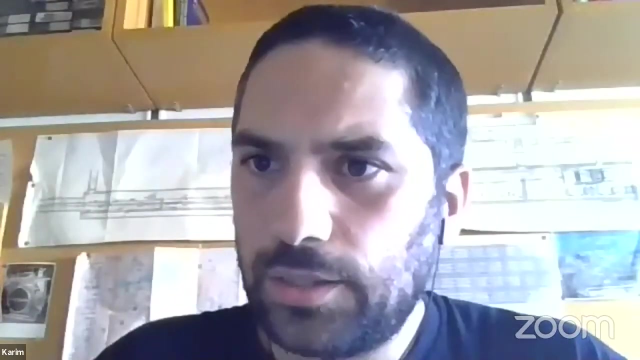 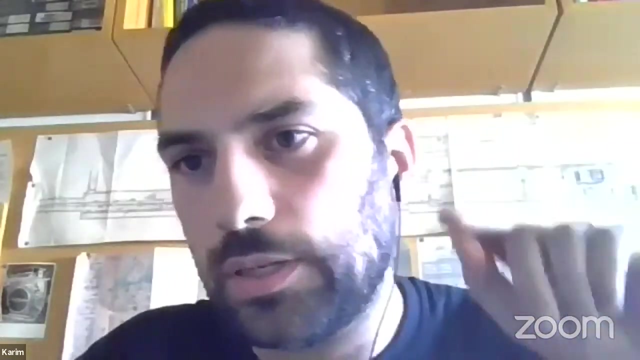 let me thank you all for your attention. So that's it, Okay. thanks a lot. Any comments or questions from the audience? I do not see any, So I just wanted to ask you. So I've seen you are mostly discussing about 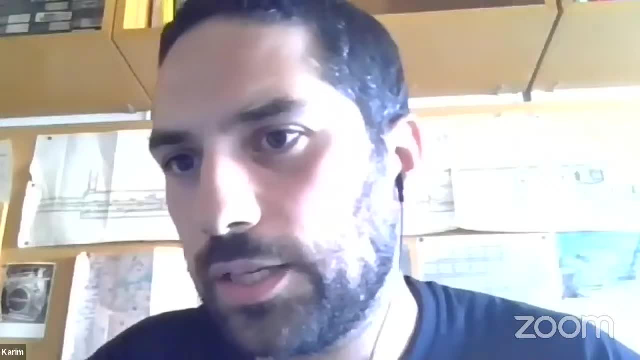 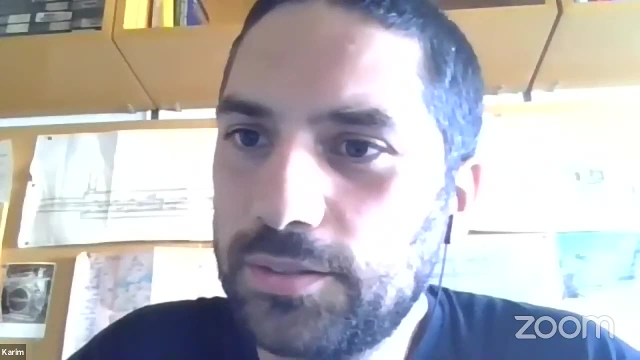 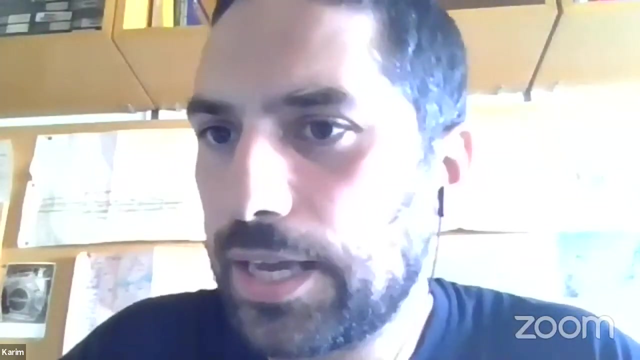 lepton to lepton, gamma decay or to lepton-lepton. But do you think that I mean, is there any, let's say, possible constraint coming from the meson, let's say lepton flavor, violating the case or it was just not considered? I mean, is it? 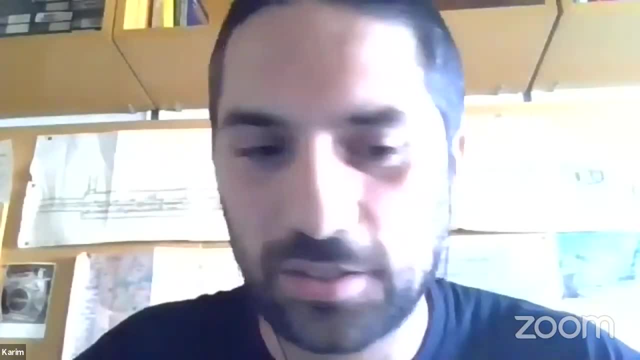 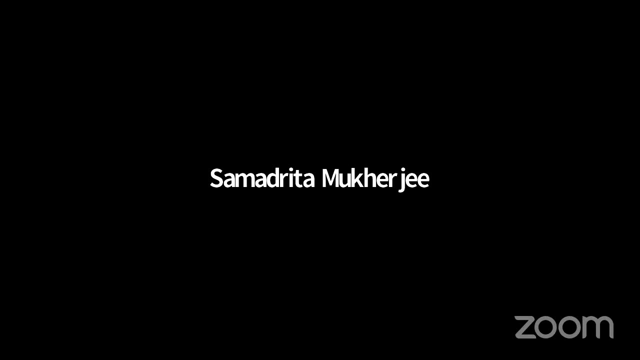 sensitive, not sensitive or was just not considered. Okay, we have not studied these mesons to lepton flavor violating decay in this analysis, but I think it will be sensitive because we have considered this lepton-left-right mixing And for quarks- quark sector also- we can have the non-holomorphic of diagonal elements. So 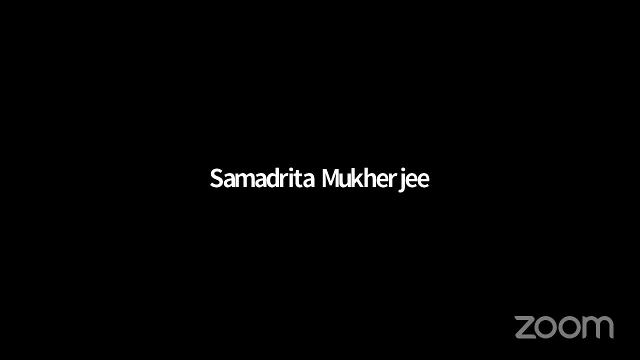 meson containing like QD bar or some K mesons etc. Then if we consider the non-diagonal couplings, non-holomorphic in the squark sector, then we can have some imprints of them in that decays also. That may be a. We can have their imprints. 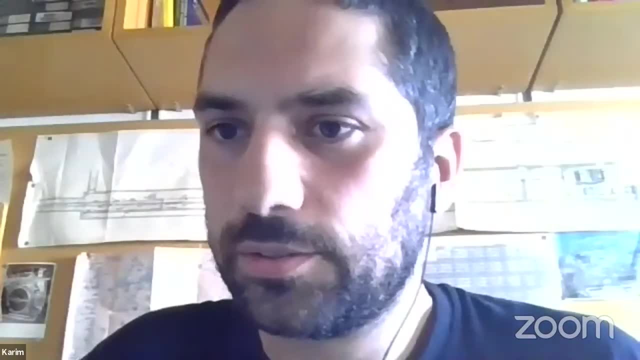 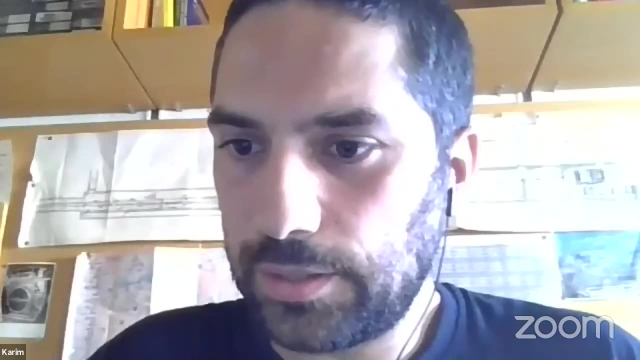 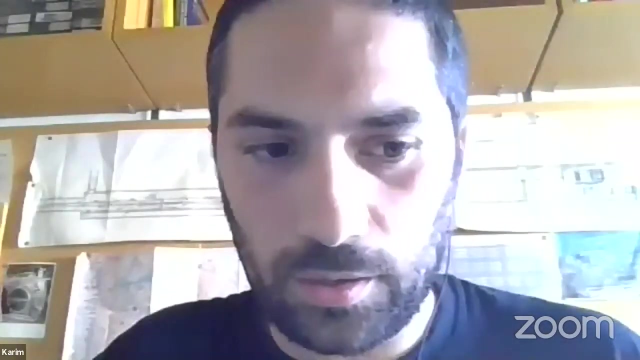 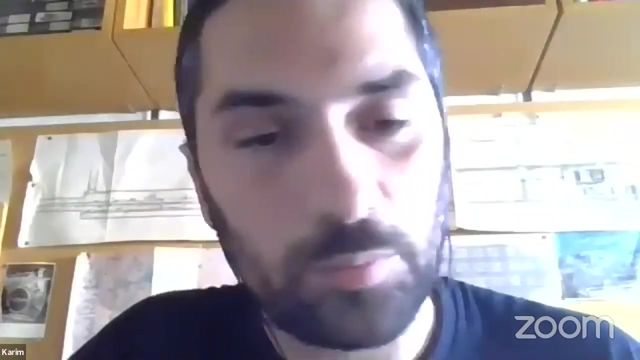 Okay, so it also can occur there. Okay, very nice. Okay, thanks a lot. So if there are no other comments or questions, I thank you again and I would move to the last talk of this session before the coffee break. And we have met Yusel about the mu2e experiment. 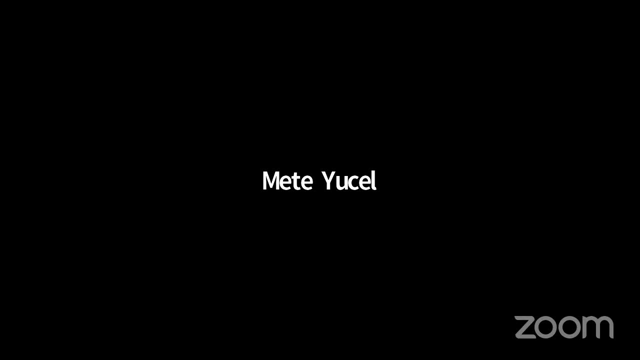 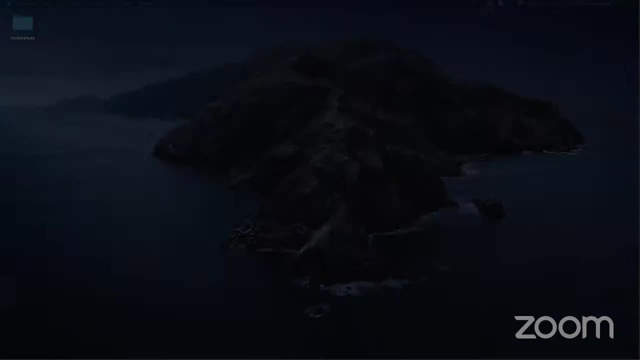 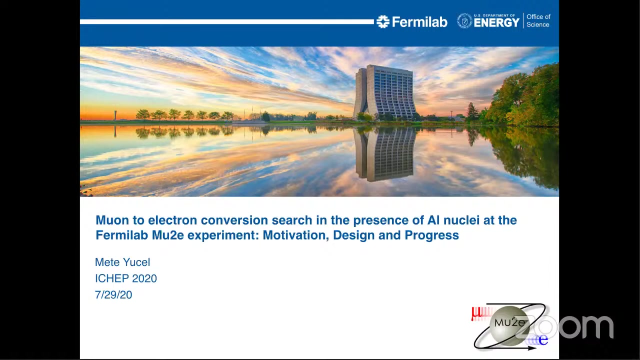 Hi, I will share now, Yes, please, And then I'll start the presentation. Can you see this? Yes, Okay. So I'm going to talk about the mu2e experiment at Fermilab, our motivation, the design of the experiment, and I'm going to report on the 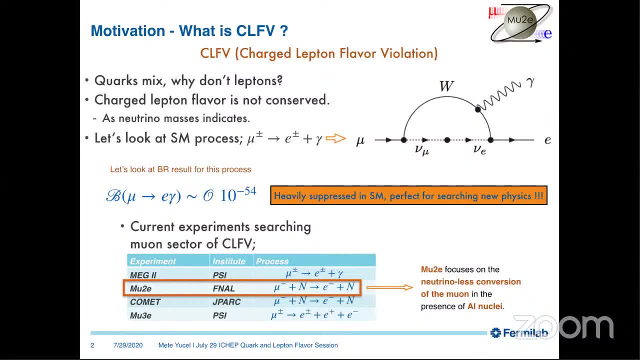 progress. So we'll start with what is a charged lepton flavor violation. We know that quarks mix, but why don't leptons is the actual question. So, as discussed in other talks today, the charged lepton flavor is not conserved, as you know, indicated by neutral masses. So 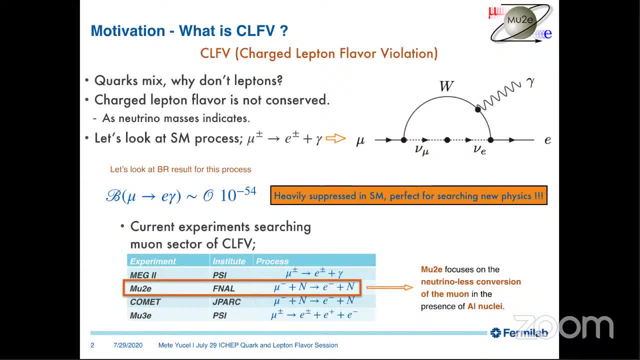 let's, you know, use that and let's look at a process which is mu2e gamma and in the standard model and calculate the branching ratio. That turns out to be 10 to the minus 54, which is heavily suppressed. So that means, if you point something here, 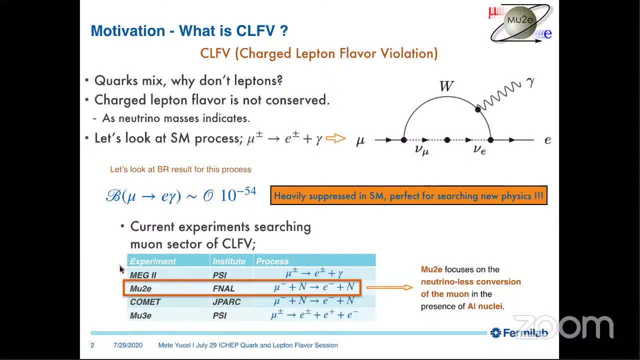 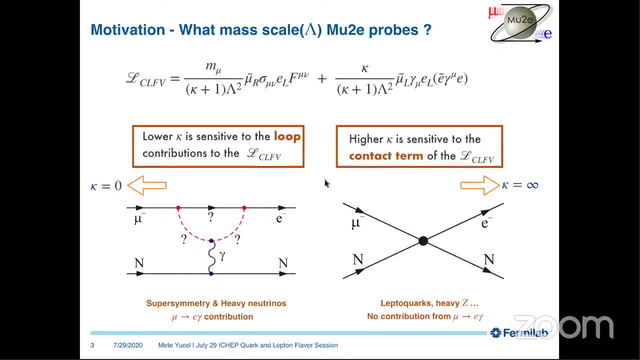 it will indicate in the new physics. So here I list some newer experiments focusing on the muon sector, And of course we're going to talk about mu TE, which is the neutrino-less conversion of the muon. So which scales mu TE probes? 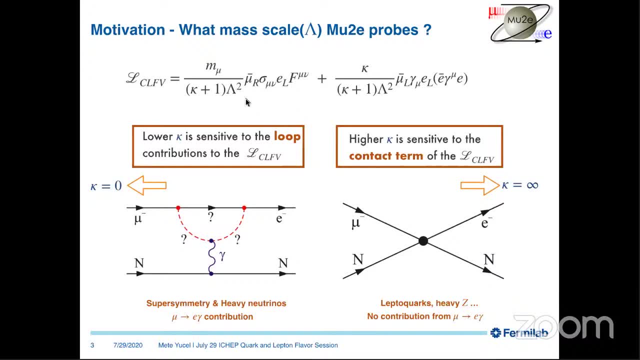 here's our effective Lagrangian. Here is the Lambda is the mass term and the Kappa is a scale factor between the first and the second terms of this Lagrangian. So if the Kappa is low you get effects sensitive from the loop contributions. 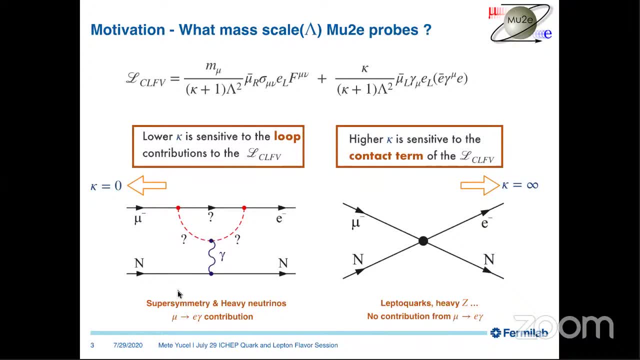 So the Lagrangian is indicated here. Now these can be supersymmetric model heavy neutrinos and all those things, And if you increase the Kappa, then your second term dominates and this is sensitive to what we so-called contact term and these couplings interactions. 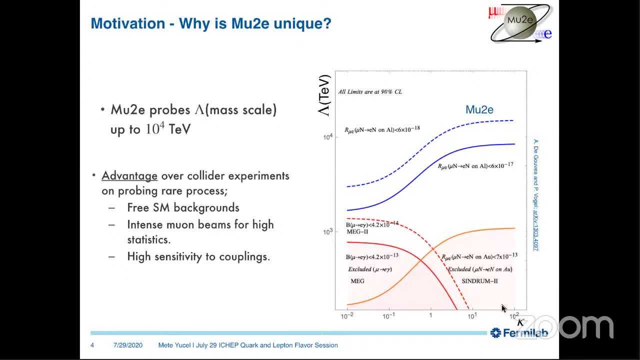 So why is mu TE unique? So let's try to understand that while looking at this picture, the plot of Kappa versus the mass scale- here you can see the mass scale mu TE probes. Let's start with syndrome two, which is the older experiment. 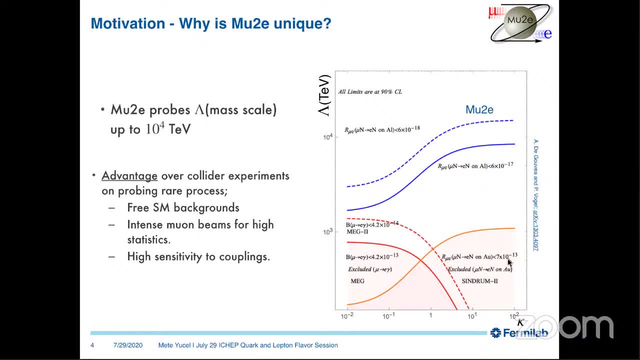 This puts our conversion limit at 10 to the minus 13 and covers this region of the spectrum. And we have mu TE gamma experiment, again at 10 to minus 13,, covering this sector. So in comparison, mu TE can probe up to 10 to the four TEV. 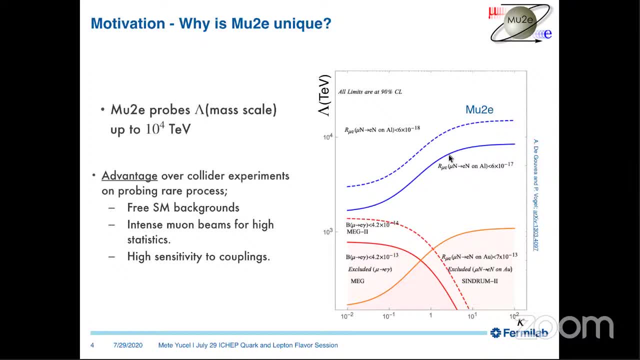 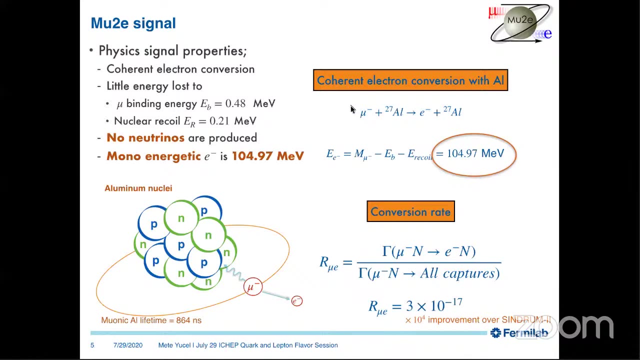 And not only that, like for in comparison to collider experiment, mu TE is free from standard model backgrounds. You can also have intense muon beams for high statistic, which you can't get in a general collider experiment. So let's look at our signal. 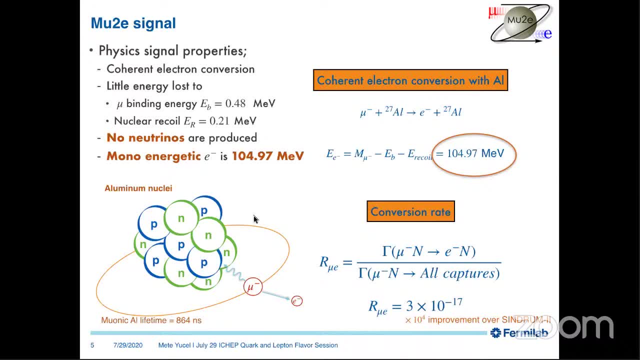 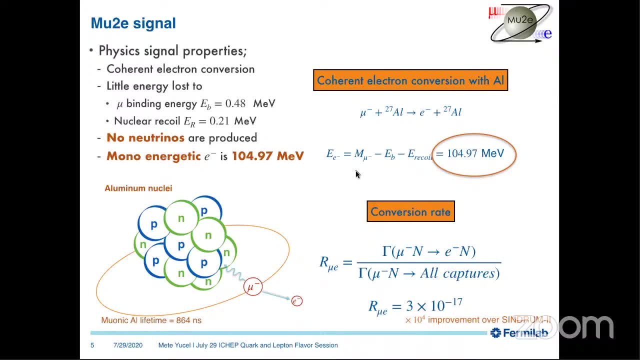 Some to the binding and some to the nuclear recoil. So you put that in and you can calculate the this mono-energistic electron of 105 MeV. So what we're looking for is the rate of this conversion divided by all the other captures. 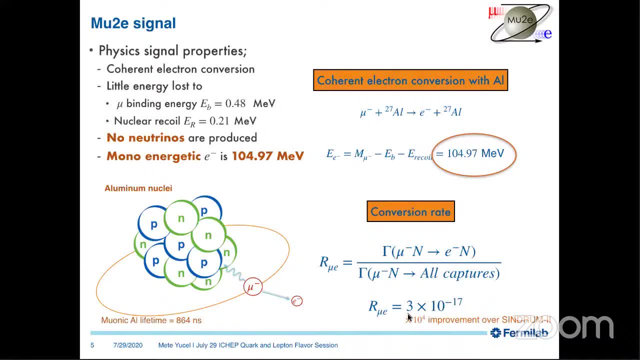 And this will give you your conversion rate, which we aim three times 10 to the minus 17.. And this will be a 10 to the four improvement over syndrome two, the last experiment. So let's talk about our brain, Let's talk about our backgrounds. 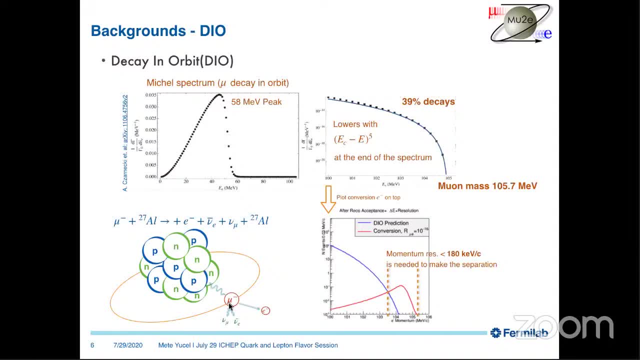 The biggest background we have is decaying orbit electrons. Here again the same picture: muon goes in around the aluminum, It's this time- regularly decays into electron with neutrinos which then, you know, shares the momentum with the electron. 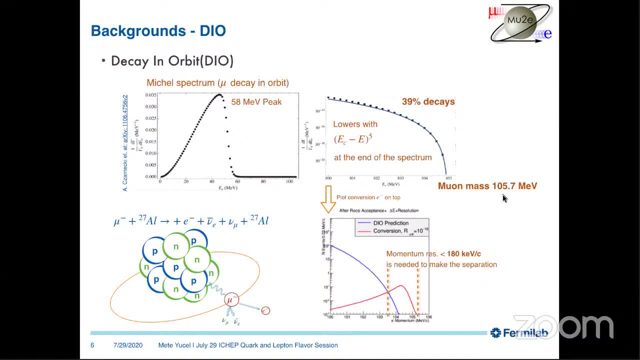 This means it has a lower energy peak compared to our muon mass. So the spectrum- let's inspect that tail end of it- It decreases sharply. But if the, if you plot our conversion, the electron on top of this decay, the background will get this: 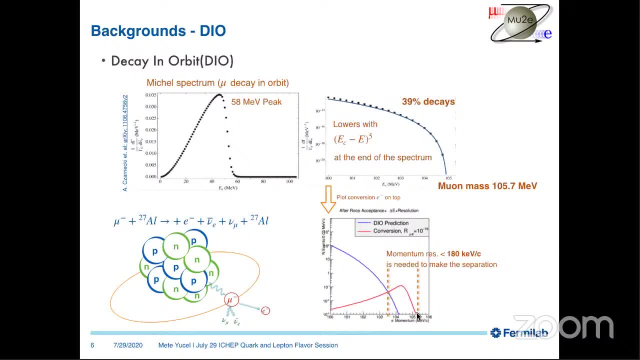 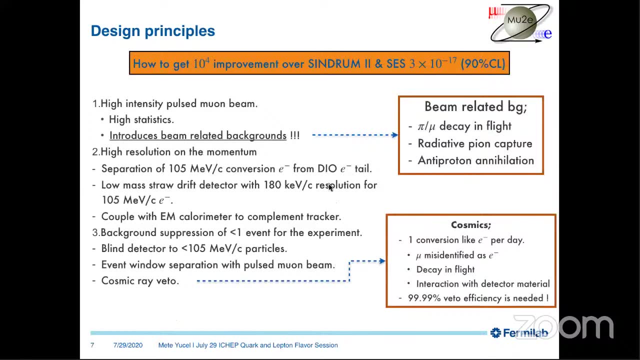 So the media experiment tries to separate this red signal from the blue background, And to get that we need a good momentum resolution. So let's summarize our design principles. So when I get 10 to the four- improvement over the last experiment- the question is how to get there. 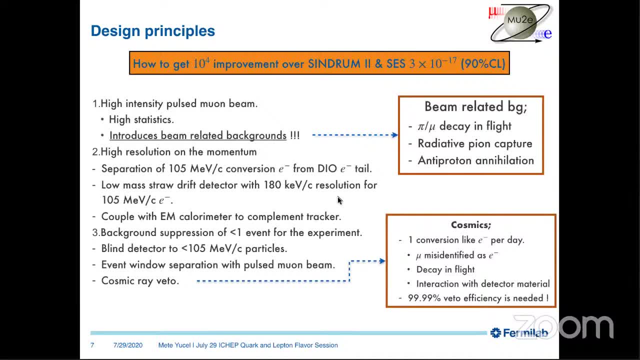 So, firstly, we get there by having a high intensity pulsed muon. This provides you with high statistics, but also with the beam. it introduces beam backgrounds. So what are those? Like pions and muons coming with the beam and then decaying in flight. 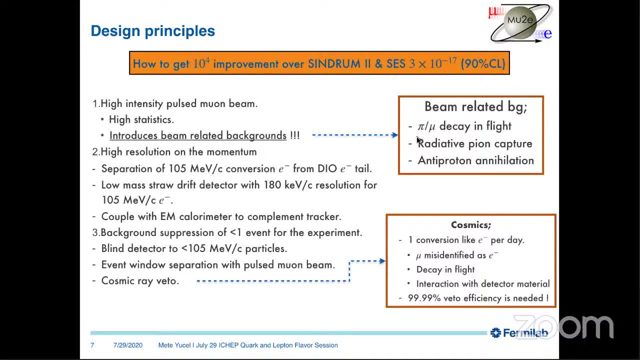 Radiated pine capture or antipodal annihilation. These are some examples. Secondly, we need high resolution on the momentum to be able to separate 105 MeV conversion electrons from the DIOs. to achieve this, We have to be able to separate 105 MeV conversion electrons from the DIOs. to achieve this, 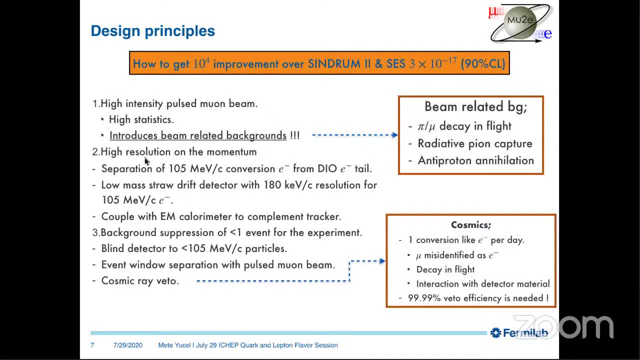 We have to be able to separate 105 MeV conversion electrons from the DIOs. to achieve this We have a tracker and electromagnetic colorimeter, And then to get a discovery, we need a background suppression of less than one event for the whole experiment. 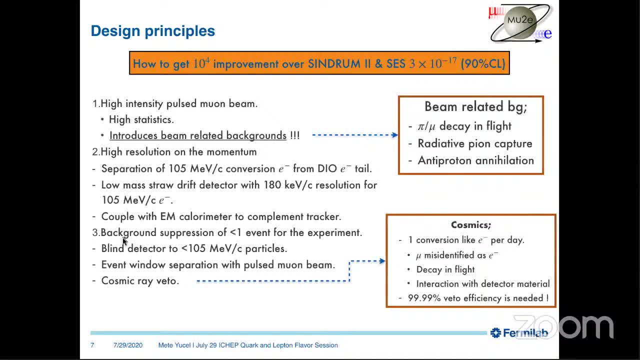 So that means making the detector basically blind. to lower energy particles. We're going to use an event window separation with pulsed muon beam. We need a way to veto cosmic rays because they're also a big part of the background. It produces one conversion-like electron per day. 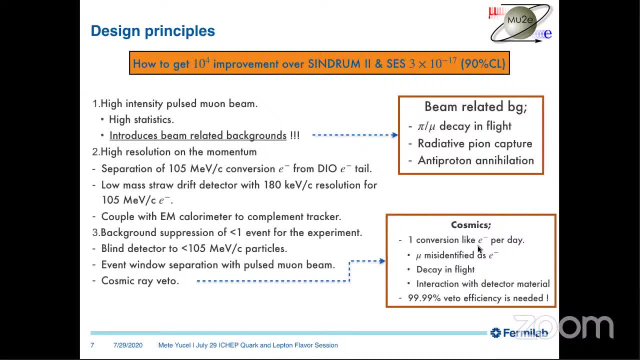 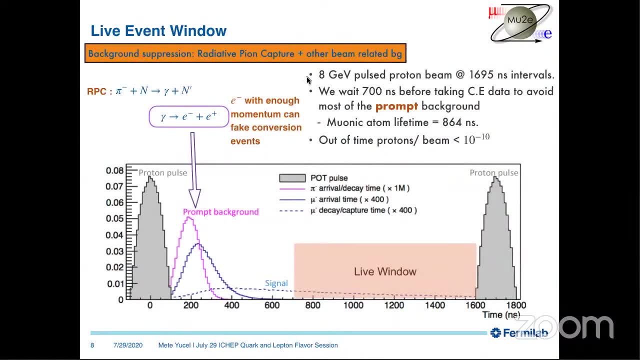 It produces one conversion-like electron per day. And so the discovery we need: we need 99.99 veto efficiency, which is pretty hard. We need 99.99 veto efficiency, which is pretty hard. So let's talk about our live event window. 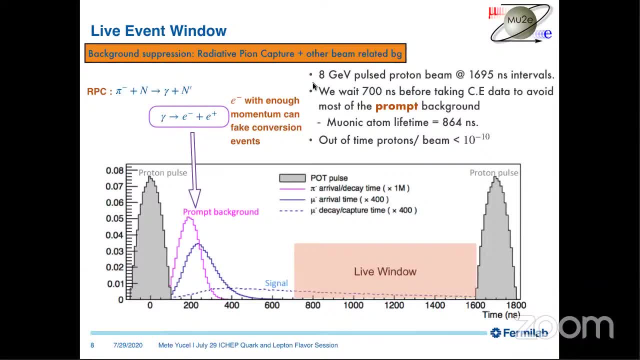 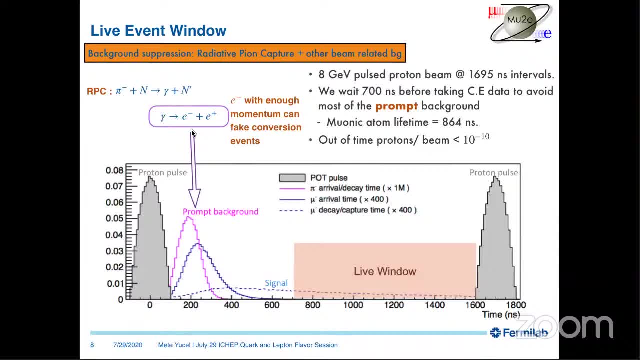 to die out even before we start taking beam data. So here's an example. radiative pine capture. one of the biggest Pine- is captured by the aluminum releases, a gamma, which then converts into an electron and positron pair. Here you can see that it just dies out. 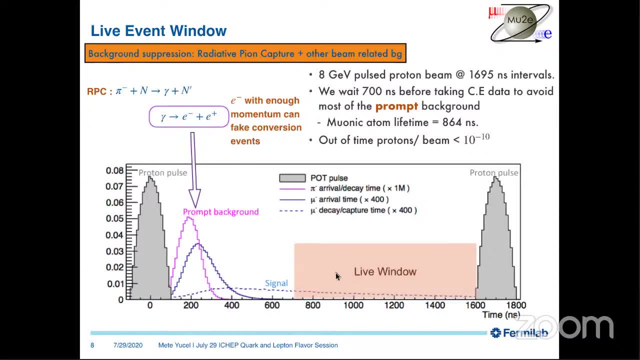 while we're taking signal, 700 nanoseconds later You can ask: what about out-of-time protons? Well, out-of-time protons per beam: we limit that to 10 to the minus 10.. we limit that to 10 to the minus 10.. 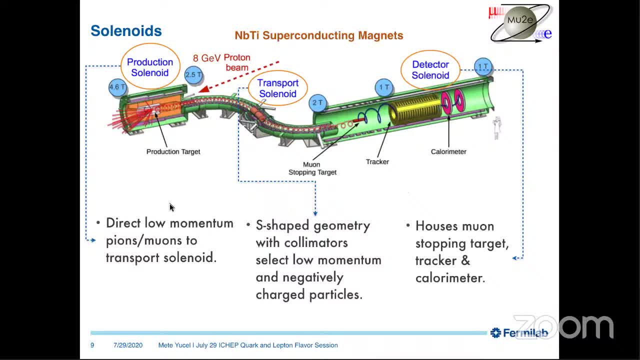 So here's the overall picture of the experiment. It has three superconducting magnets. There's a production solenoid. a two proton beam comes here and hits the production target housed in the production solenoid, which produces muons. We direct them to the transport solenoid. 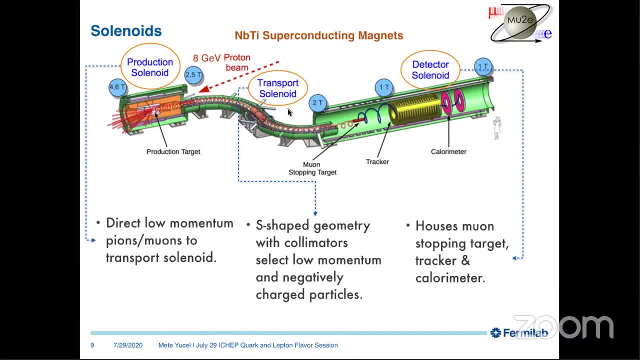 where they transfer into the muon stopping target. So this transport solenoid has an S-shaped geometry which selects a low-and-medium solenoid, a low-and-medium solenoid and negatively charged particles, And then these go into the detector solenoid. 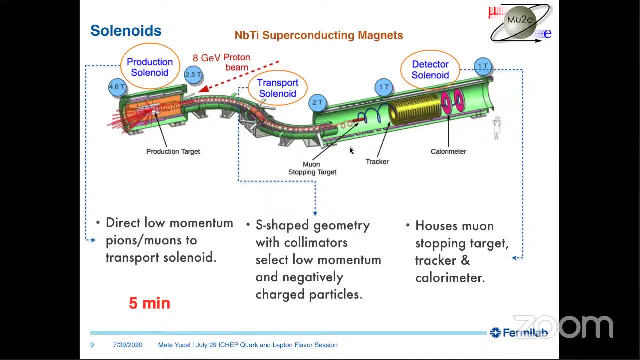 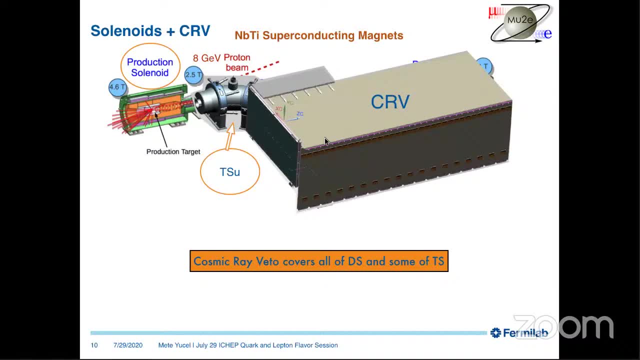 the conversion electrons go into a helical orbit, hitting the tractor and the colorimeter. So all of that is covered by our cosmic ray-achiever system. Here you can see these are like giant scintillators. Here you can see that it is covering. 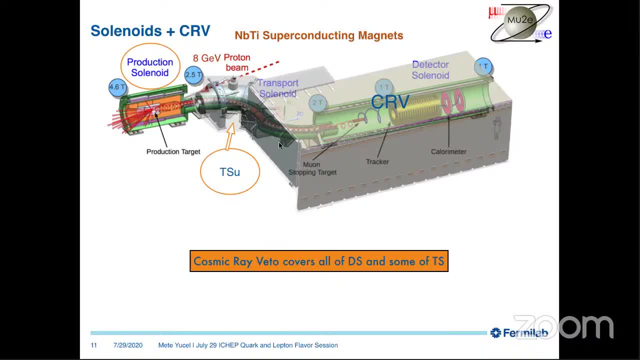 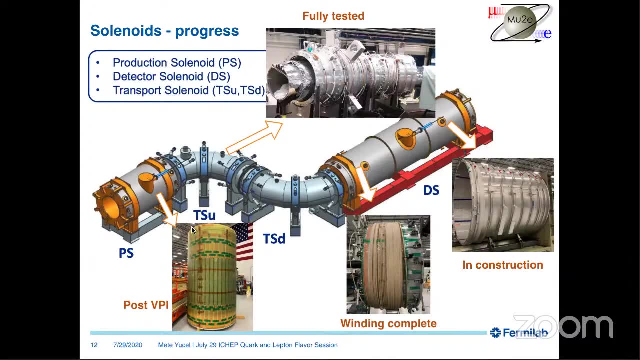 the whole of the detector solenoid and some part of the transport solenoid. So our progress on the solenoids. here is a picture of the Mio and BM line showing where different parts of the solenoids are at. I would say the transport solenoid is the. 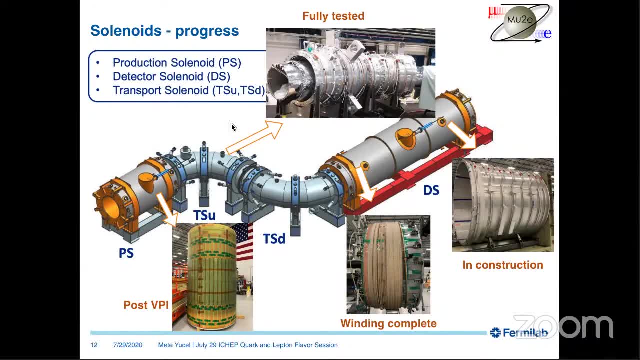 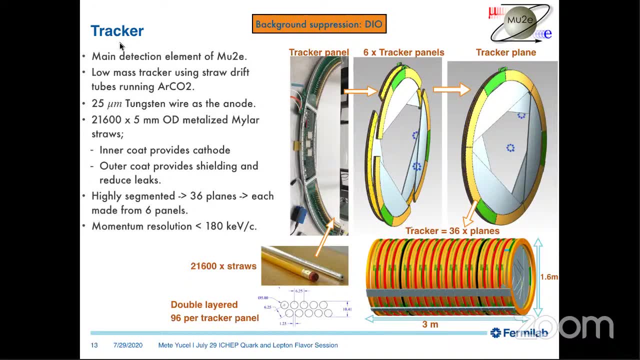 farthest one apart in terms of completion. So let's talk about the tracker which I work on. This is the main detection element of MuTe. It's a low mass tracker using straw drift tubes running argon CO2.. Here's a picture of the straw: five millimeter in diameter, We have a 96 per. 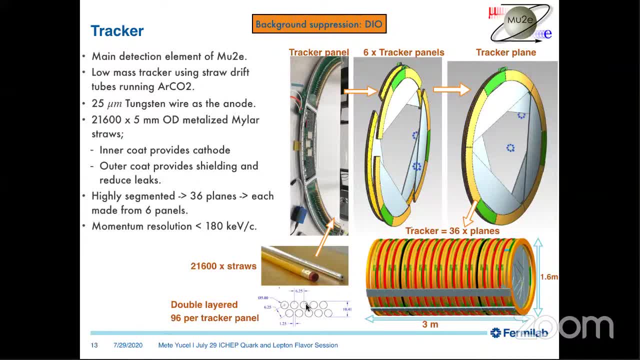 tracker panel staged in double layer configuration like this. Here's a panel. We put six of them together to produce a plane and the whole tracker consists of 36 such planes and it is three meters in length. This highly segmented nature of tracker helped with the particle identification and our 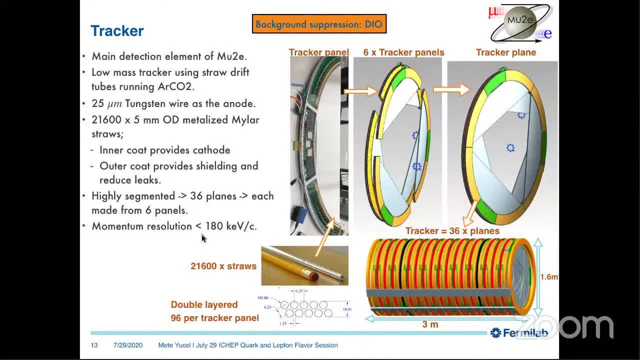 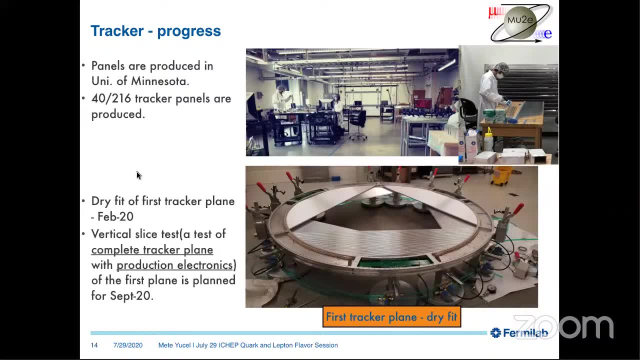 momentum rate. So our progress. the tracker panels are produced in the University of Minnesota. 40 out of 216 are produced. In comparison, planes are going to be produced at Fermilab. We did a trial at the back in February before quarantine. Now we're planning to do a vertical slice test. 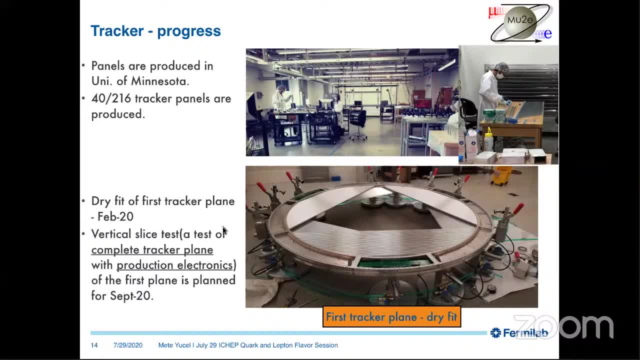 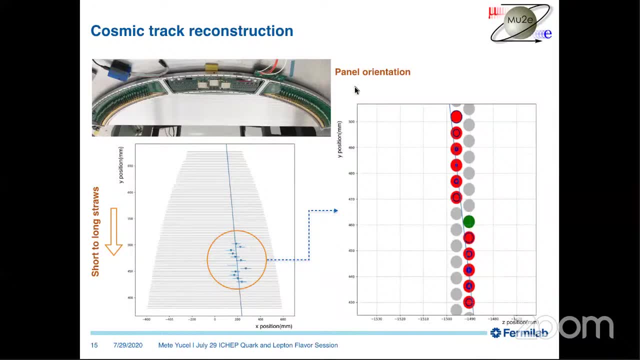 which is a complete test of tracker plane with the collection electronics, and this is going to be done. Here's an example of the tracker construction Panel. upside down. particle comes down and then you can see that it hits both layers and we calculate, we determine the distance of close approach on each straw to construct our track. 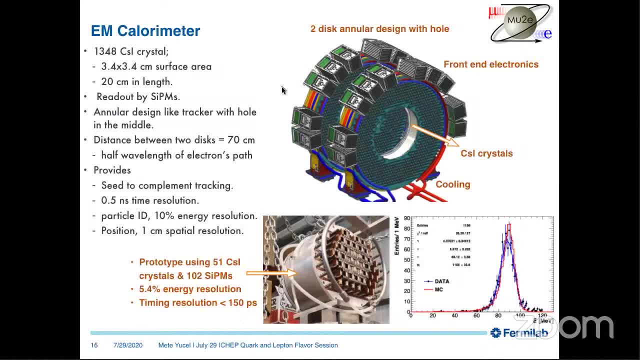 So let's switch the electromagnetic colorimeter. We have 1348 cesium iodide crystals. These are all read out by silicon photomultipliers. The design is similar to tracker, with this annular structure with a hole in the middle. Here you can see a prototype from 2017. 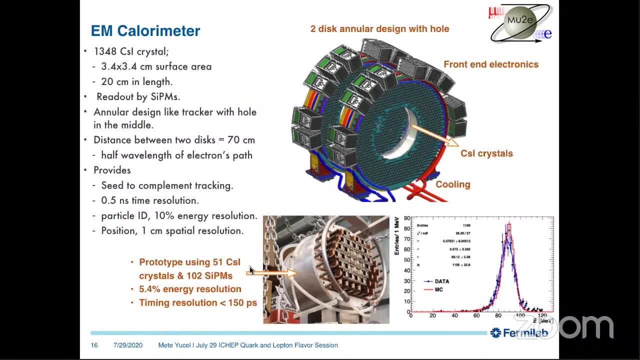 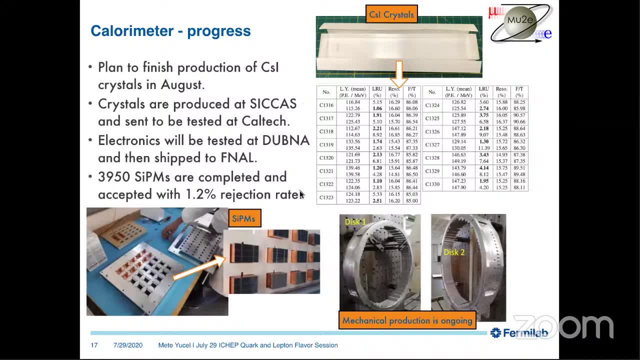 which you know achieved all the experiment's goals, like the time resolution, energy resolution and spatial resolution. So the progress. on colorimeter, we have cesium iodide crystals expected to be done by August. They're measured at Compton. 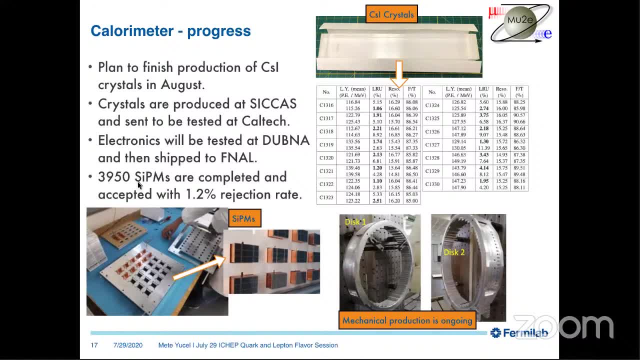 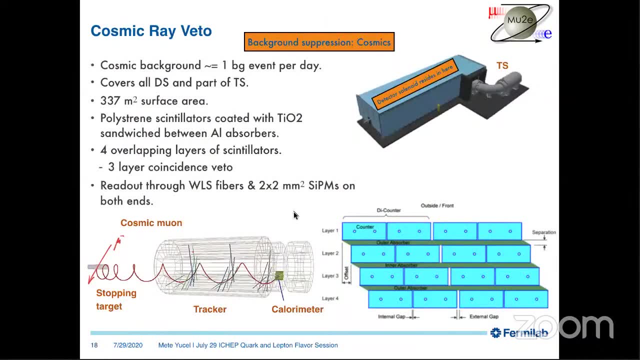 For light yield and resolution. all the systems are completed and assembled into these plates, which will be then installed into the colorimeter, A cosmic ray veto. we talked about this. It consists of this: polystyrene scintillators layered in this four-layered staging. 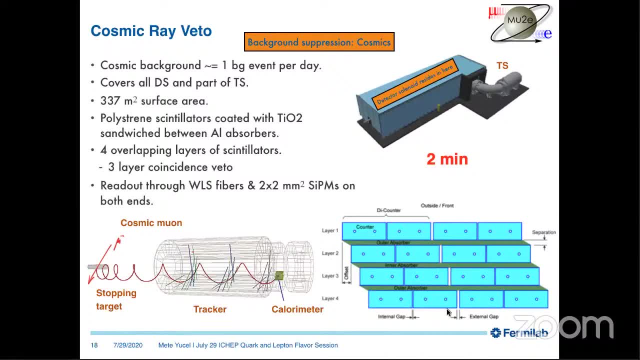 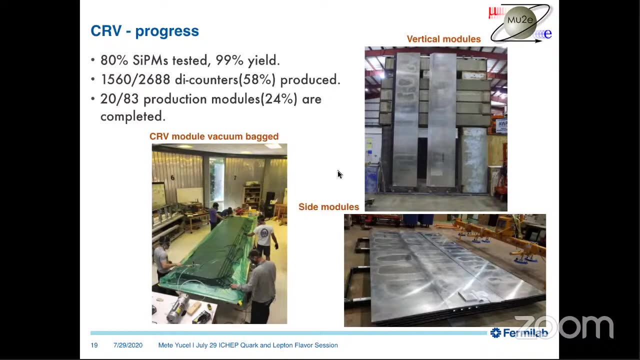 and it covers all of the detectors on it. Whenever a particle, a muon passes by it is. we do a constant test to see if there's any evidence of three out of four and eliminate the cosmic ray on it. For the progress, all of the systems, eight percent of the systems, are tested. 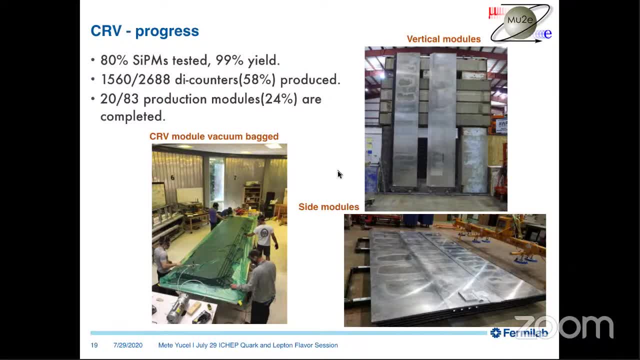 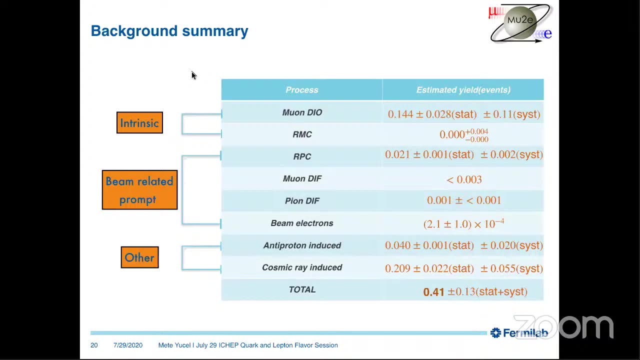 The die counter is 58 percent of them produced. Then they're being assembled into modules. Here you can see a picture of a vertical one and here you can see a side one and two out of 20 out of 83, 24 percent is completed. So all of that design and detector elements. 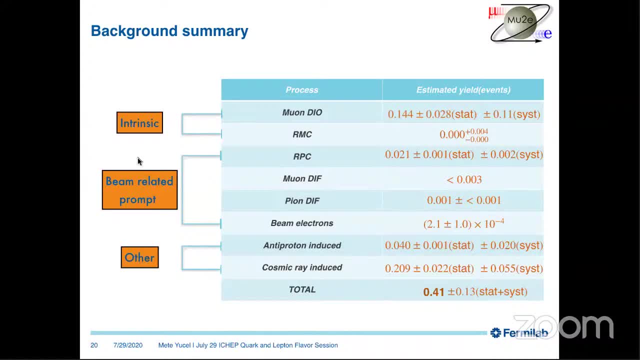 combined into this background summary table which lists intrinsic this prompt, beam related prompt and the cosmic ray backgrounds, And in total we have we achieved 4.41 event per day per experiment lifetime. So let's talk about our sensitivity. 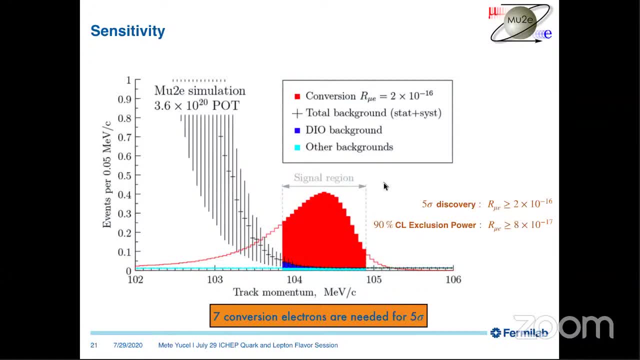 So this is what we want to find: to get the five sigma discovery We need our MUTE two times times minus 16, if we have, if the conversion is above that, we get five sigma discovery with nine, 90 confidence, the 90 percent confidence level. 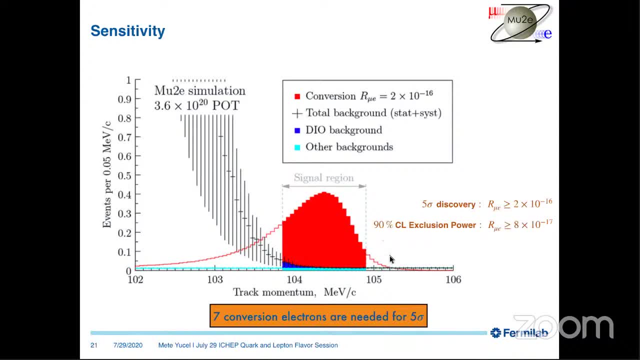 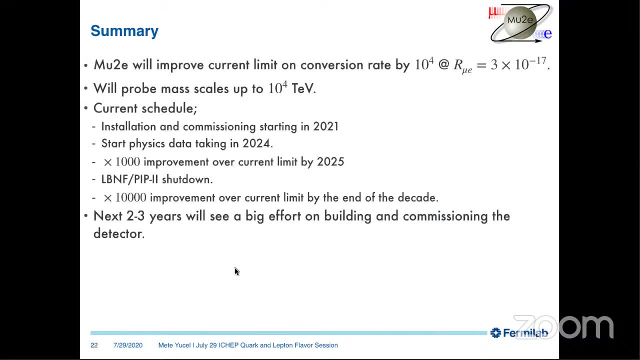 for the exclusion at eight times times minus 17.. This interestingly means to get this we need we only need seven conversion electrons. So, in summary, MUTE will improve current limit and conversion rate by 10 to the fourth at the single electron sensitivity of three times. 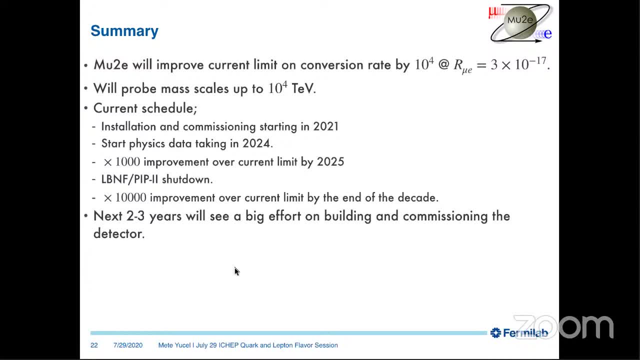 10 to the minus 17.. It will probe mass scales up to 10 to the fourth TV. Our current schedule is the installation commissioning starting in 2021, the physics in 2024.. This means a thousand times improvement over the current limit by 2025. Then there's going to be a shutdown and it will 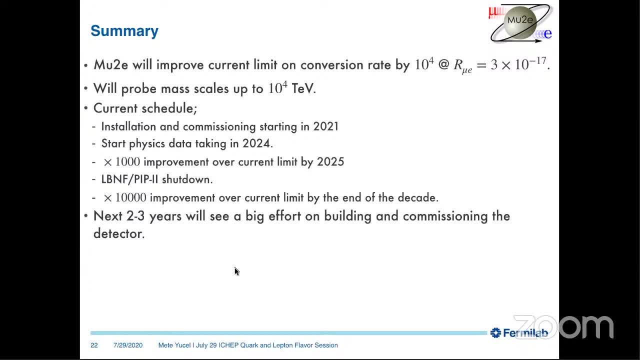 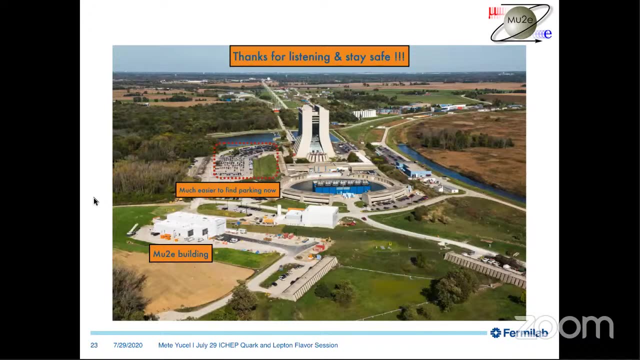 it will. we will then, by the end of the decade, hopefully get a 10,000 improvement over the current limit, And the next two, three years we'll see a big effort on building and commissioning the detector. So thanks for listening. Here's a nice picture of Fermilab campus with a MUTE building. 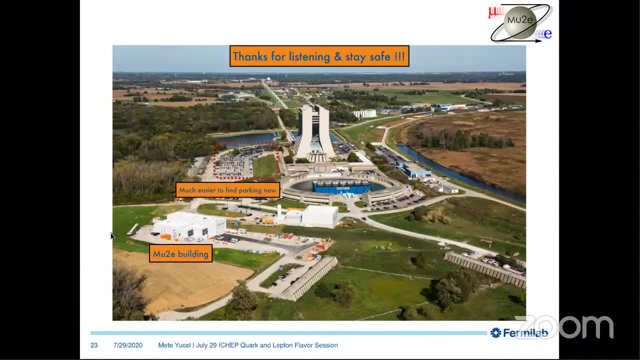 in the lower left corner. So that's all Okay, Thanks a lot. Any comments or questions from the audience? Hi, thank you for a good talk. I have two questions. The one is that if there is a, if there is any plans for upgrade or something else during the PIP2 shutdown. 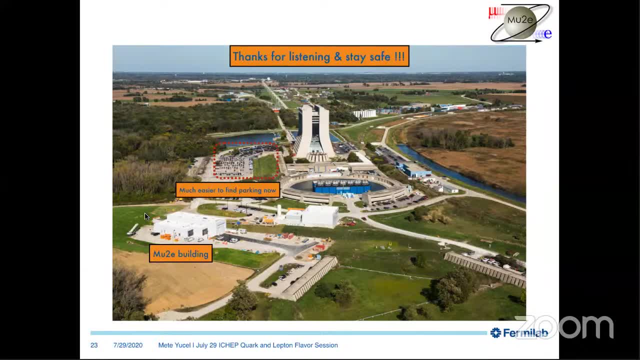 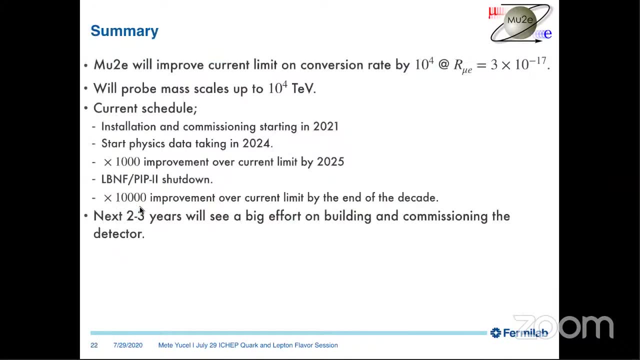 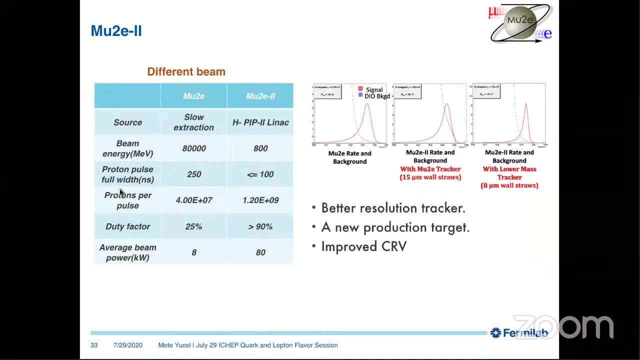 Next question is that if there was any chance to measure the extension directly, So for the first, first one, let's do So. yeah, so there's an upgrade already planned: MUTE2.. The schedule is, you know, is not solid yet, But this of course uses the PIP2. 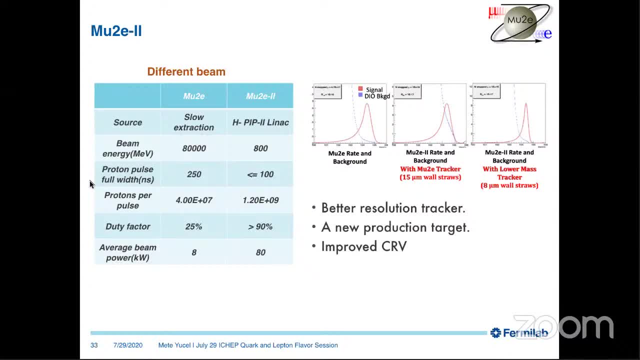 beamline to get a better beam for the experiment, which in then you know, know, increases our resolution. Of course you know this has to come with, like all the upgrades to the tracker and and saunas and you know, or the improved CRV. So the studies are. 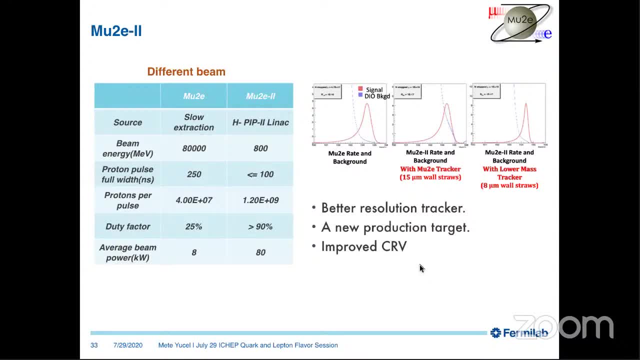 currently, you know, being done on how to how to upgrade those for the next generation, but it is planned. What was the second one? Your second question was that if there was any chance to measure the beam extinction directory, Yeah, so not here on my slides, but we have an extinction monitor, Let's go here To get. 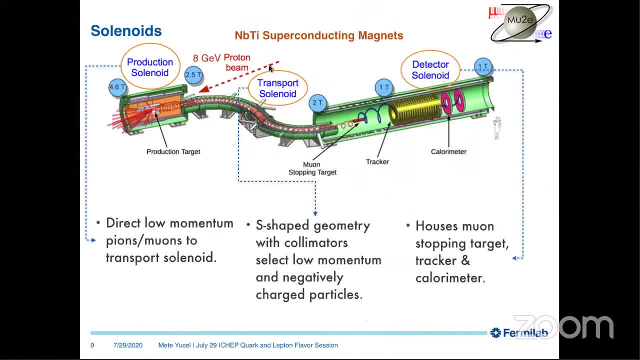 a picture of the experiment. Yeah, So right around here, before the beam comes to the production solenoid, we have an extinction monitor which you know measures the out of time particles, and then collimators that limits, limits that number to 10 to minus. 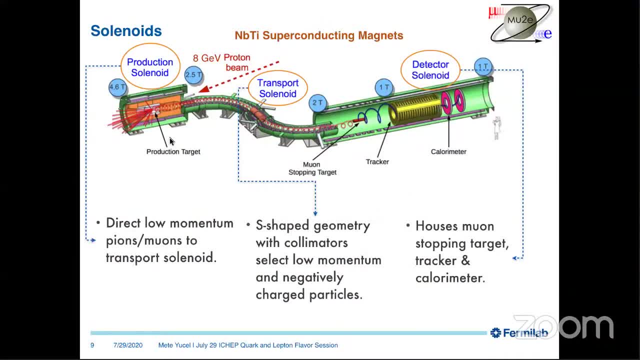 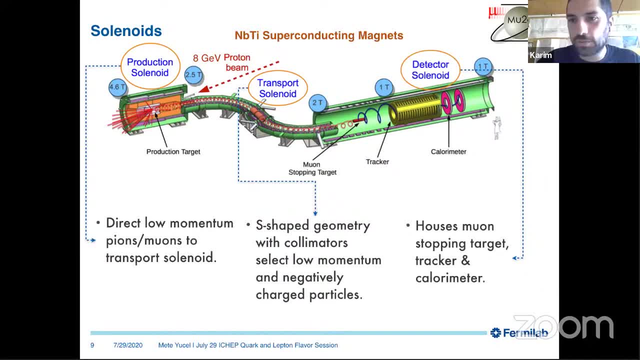 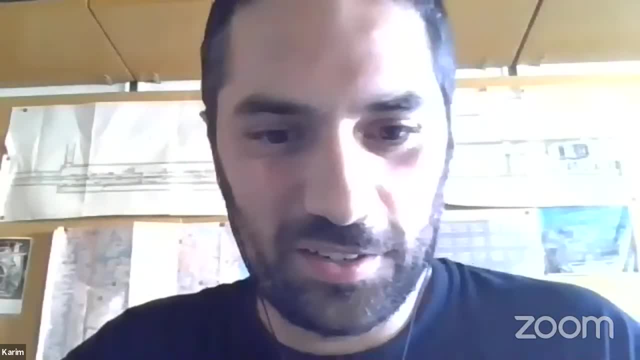 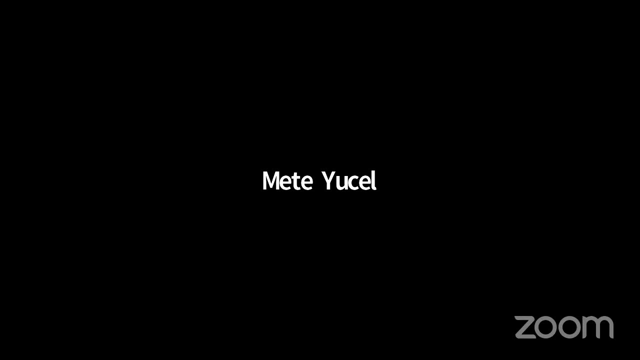 Thank you. Thank you, Like you said, it happens often, like you know, one of the main problems because that just another mechanism. in some situations it happens. I don't see any more questions Sorry to take on. I don't see any questions when I do have a burning arrays here. 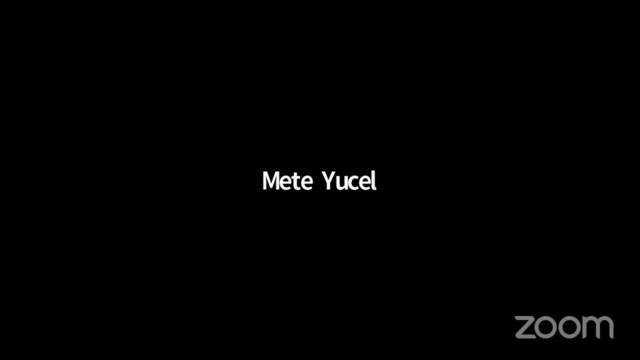 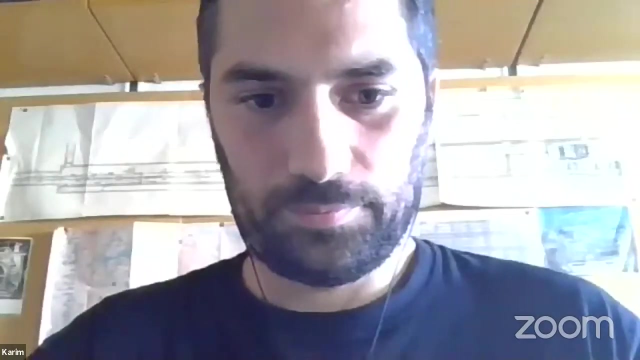 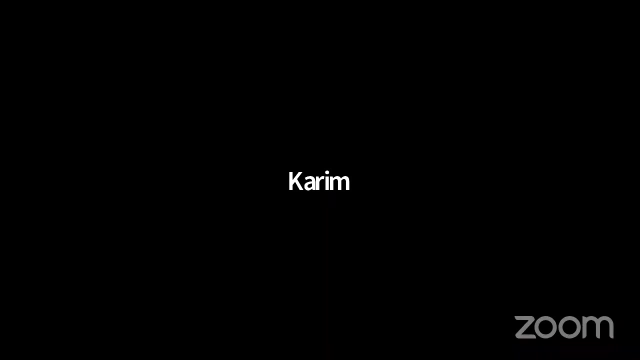 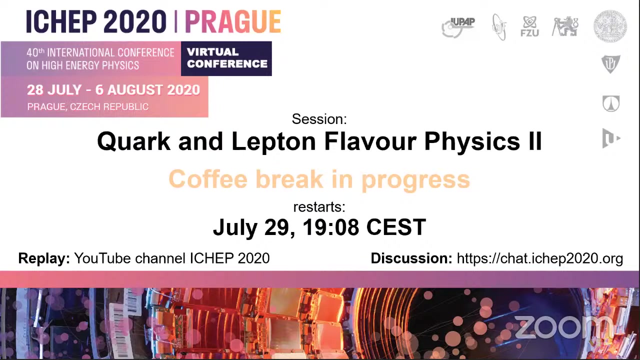 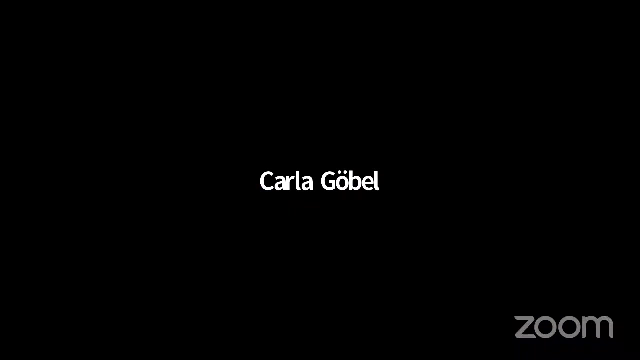 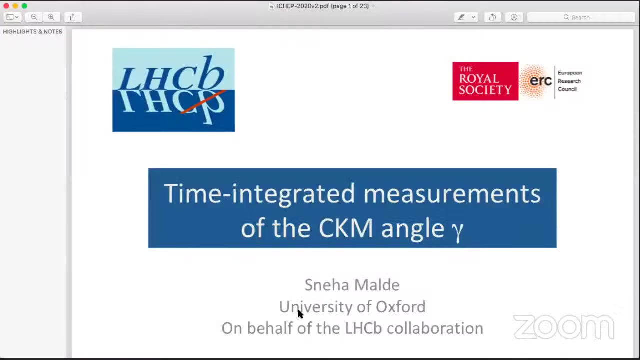 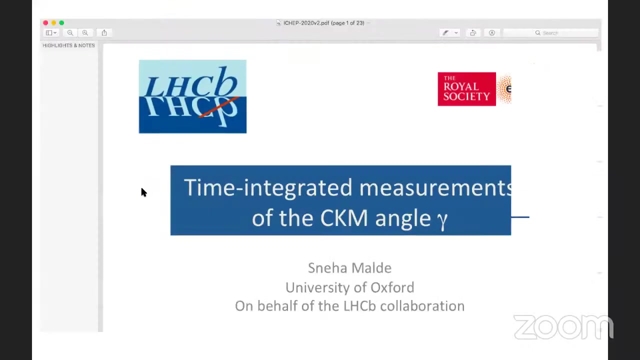 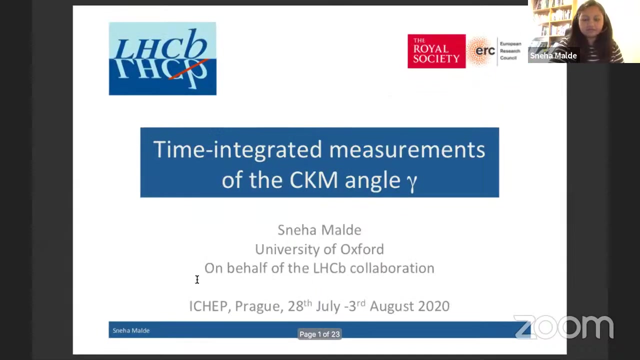 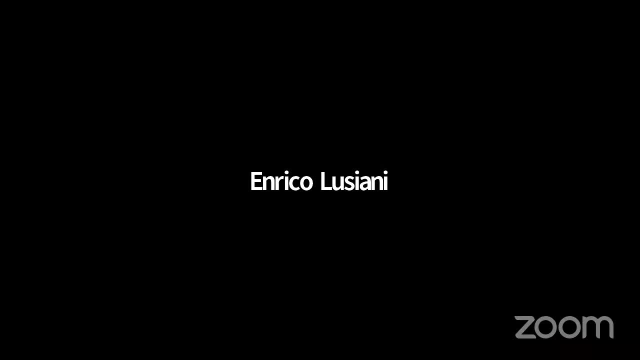 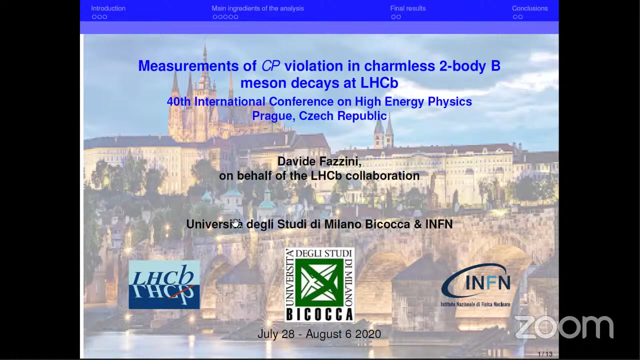 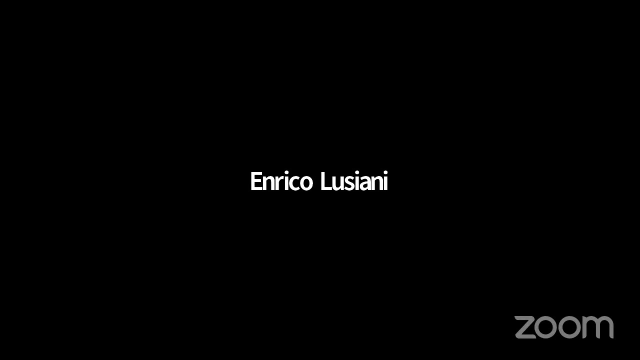 Anyone else? Yes, Okay, Someone else before? I will test later. Okay, And just Can you see them? Yes, Okay, Great Next. Yes, That will be me One second. Can you see them? Perfect. 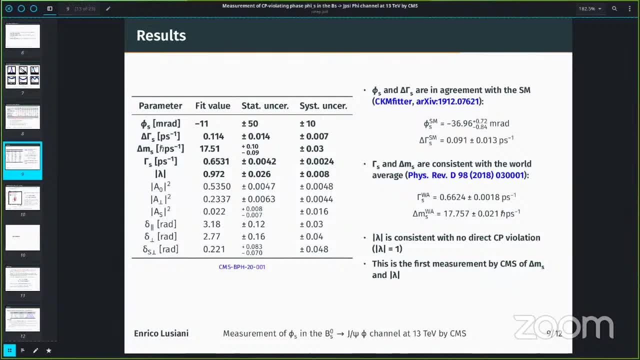 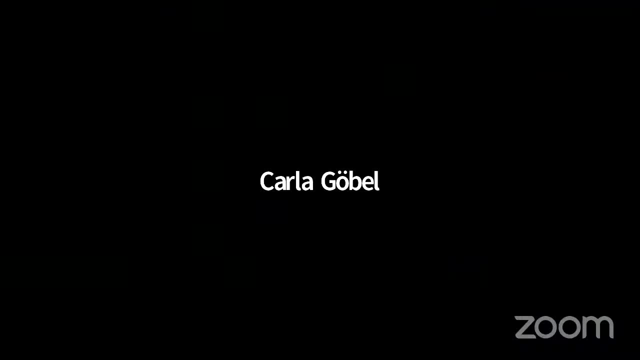 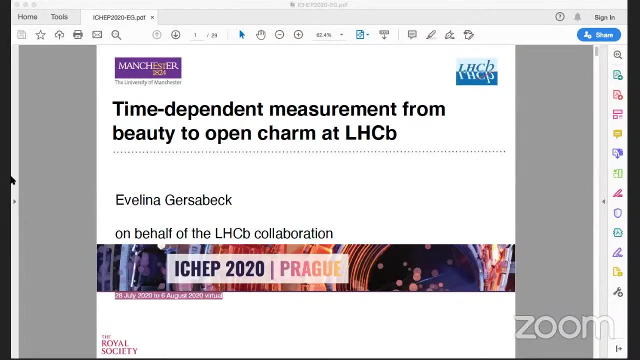 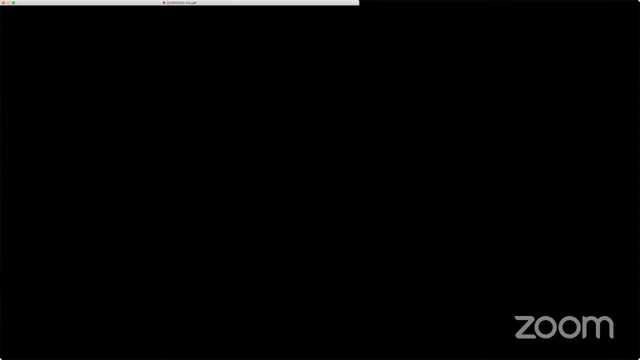 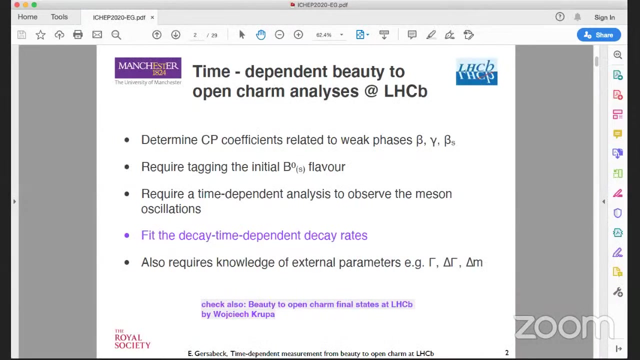 Yeah, Great Thank you. Can I also try? Anyone Try? Yes, Sure, Okay, Okay, Can I try Just a moment, Eva, I can't see yours on full screen. Yeah, I can see that way. 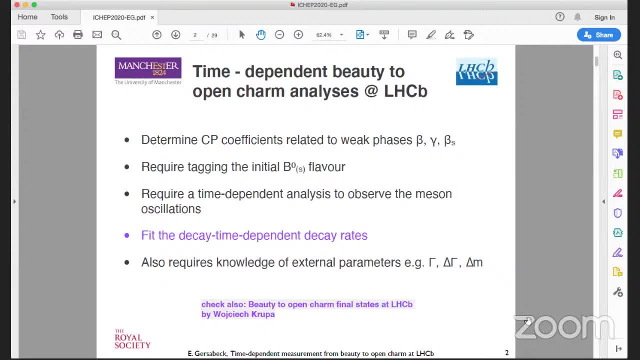 Maybe I can see you just use one there. Can I try to speak, Eva, Sorry, yes, Ah, okay, just to test. So anyone else? I'll stop sharing now. Yeah, probably you need to pass from there. 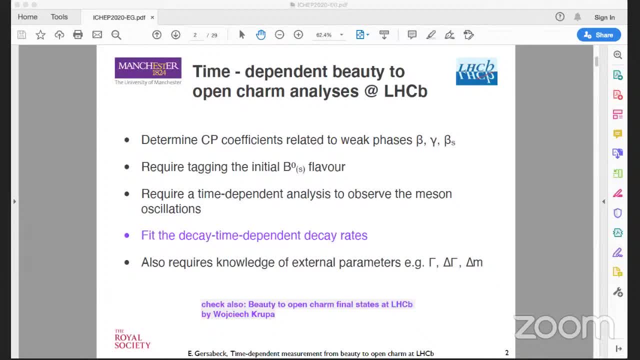 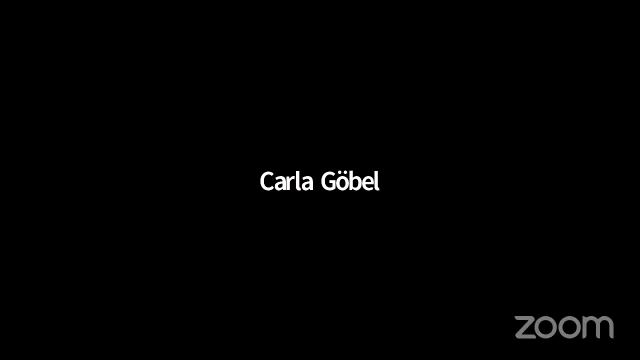 I couldn't see the other way. We can try later, but just be No. no, I'll just keep it like that. Okay, Can you stop sharing. Okay, I'll just stop for you. Well, it's time to restart so. 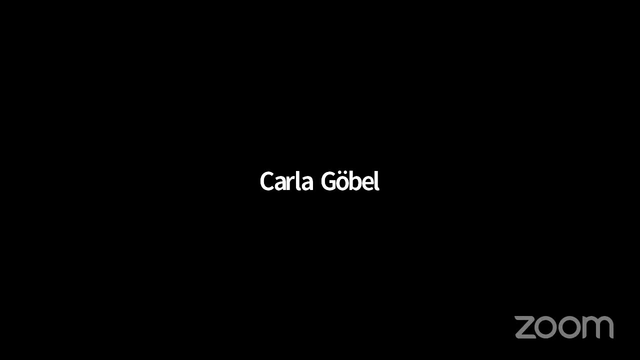 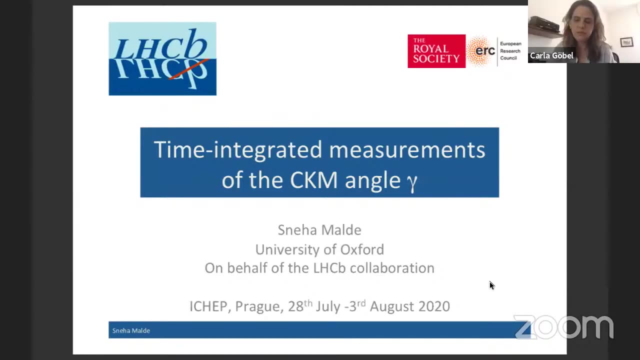 Otherwise we won't be able to be on time. So we are resuming the last block this evening of the session two of the Quark-Lactone Flavor Physics, We'll have seven talks on CP violation from Atlas, CMS and LHCb. 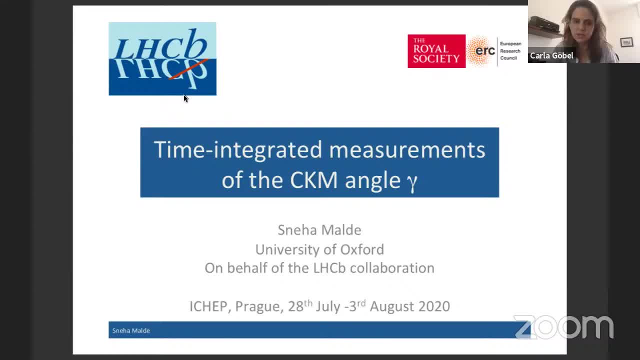 and the last talk from the DIPO-B project. So we start with Suneha with time-integrated measurements of angle. Please go ahead. So good evening. I will be telling you about our latest measurements of the CK-mangle gamma from the LHCb experiment. 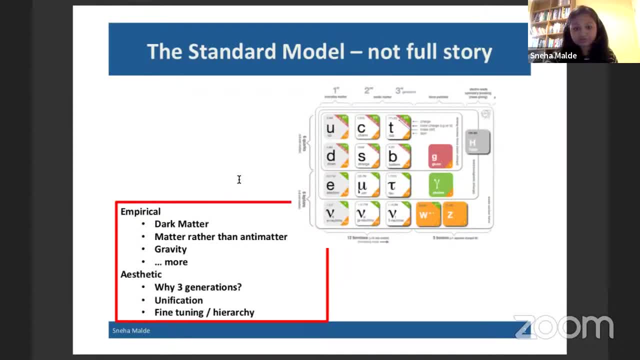 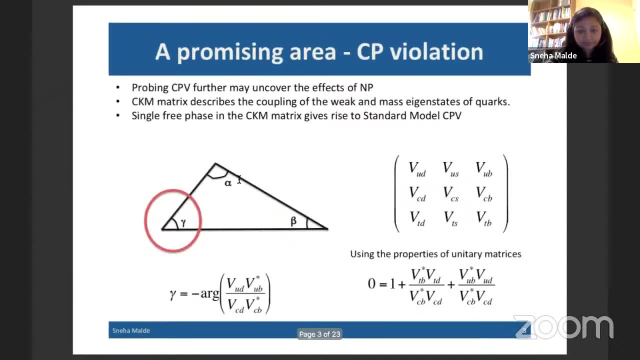 So we know that the standard model is not the full story. There are empirical and aesthetic reasons to expect there to be physics beyond the standard model. A promising area that we can explore to try and look for the effects of new physics is CP violation. 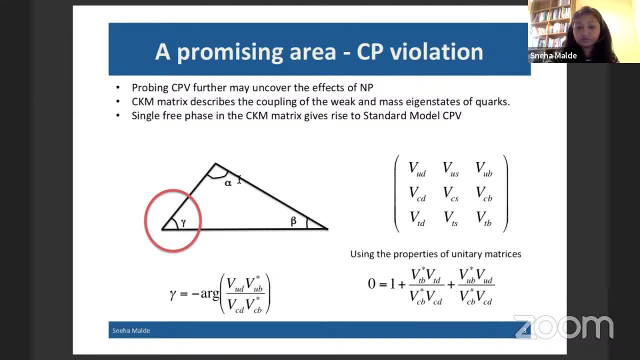 Within the standard model, the CP violation in the quark sector is encoded within the CK matrix, which describes the coupling of the weak and the mass eigenstates of quarks. Using the properties of the unitary matrix, we can represent that matrix as a unitary triangle. and we can use that matrix to represent the unitary matrix as a unitary triangle. and we can use that matrix to represent the unitary matrix as a unitary triangle and we can use that matrix to represent the unitary matrix as a unitary triangle. 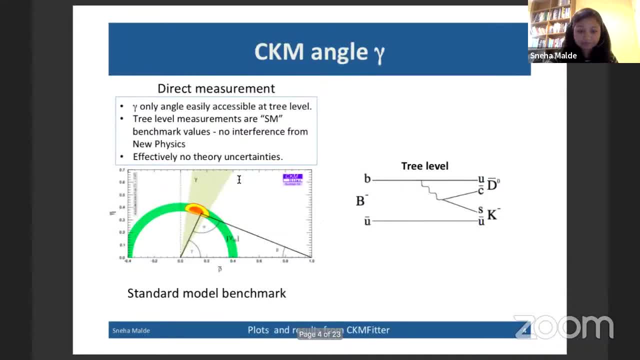 and the angle gamma is of particular interest at the moment. So gamma is interesting because it's the only angle which is easily accessible in processes that only include tree-level decays. Tree-level decays basically mean that they are standard model benchmarks, because it's very difficult for new physics to interfere and change the values. 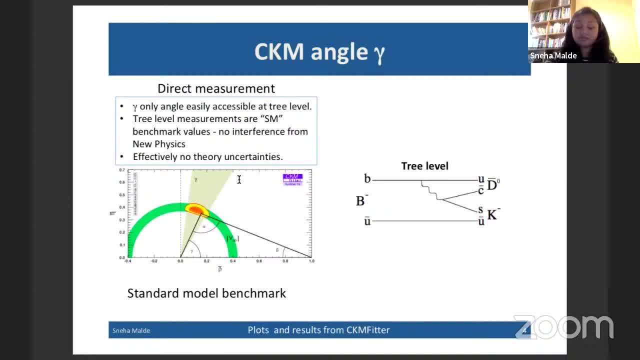 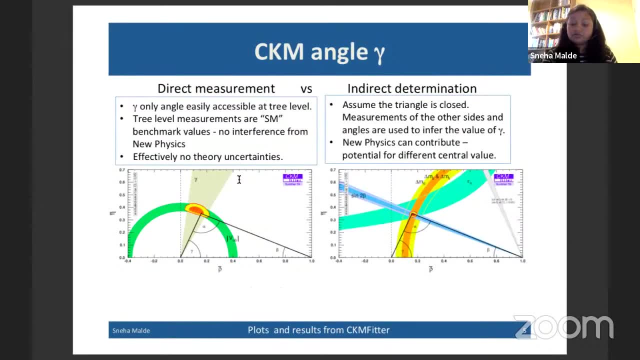 Also with gamma, we have effectively no theory uncertainties. So how would you go from a standard model benchmark to new physics? Well, you can also make indirect determinations of gamma. So here one assumes that the triangle is closed and we make measurements of the other sides. 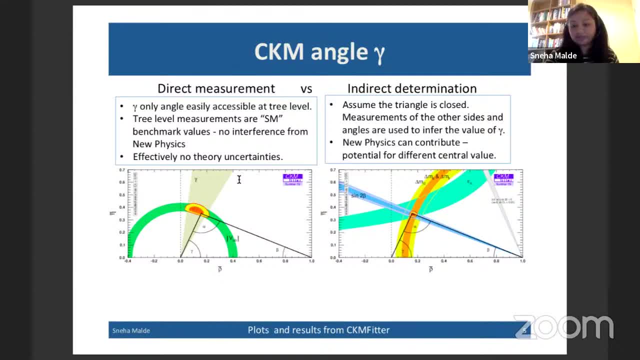 and we use measurements of the other sides and angles to infer the value of gamma. Here new physics is more likely to contribute, because a lot of these processes have loop decays in them, And so there is a potential for a different central value. 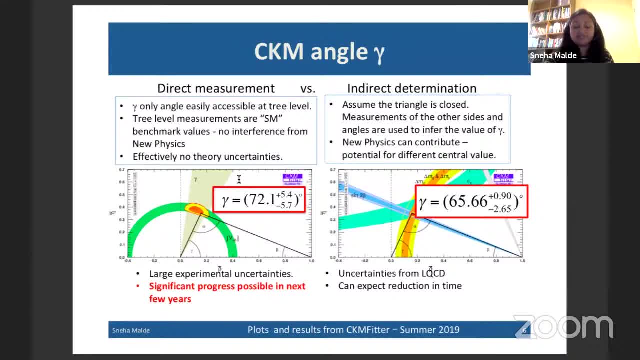 If we take a look at the current values, we see that the direct measurements and indirect measurements are a little bit different. It used to be about two sigma different. That's a bit less so now, But nonetheless the uncertainties on the direct measurements of gamma are still very large. 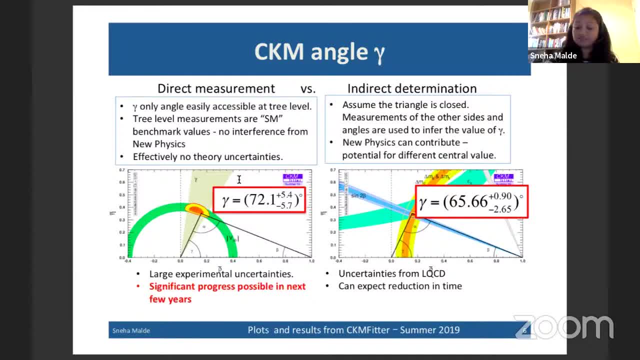 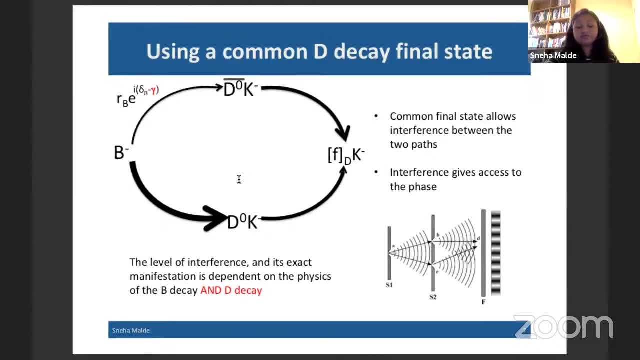 and significant progress is possible in the next few years, And that's one of the reasons why this is so interesting at this point in time. So time independent measurements of gamma are typically made in beta decay decays: There's a favoured decay and a suppressed decay. 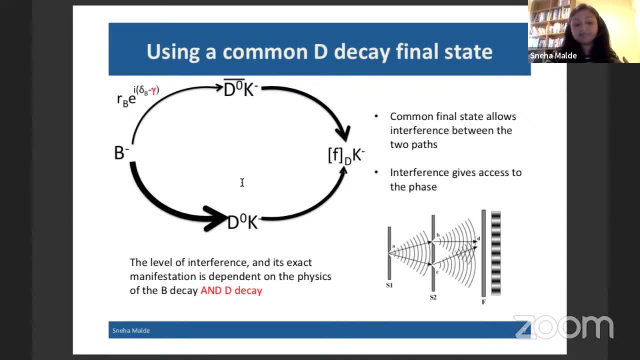 And the amplitude ratio between them is dependent on some hydronic parameters, from the strong interaction RB and delta B, and then the weak phase, which is the one that we're interested in Now. in order to access the phase gamma, we need to have a system that has interference. 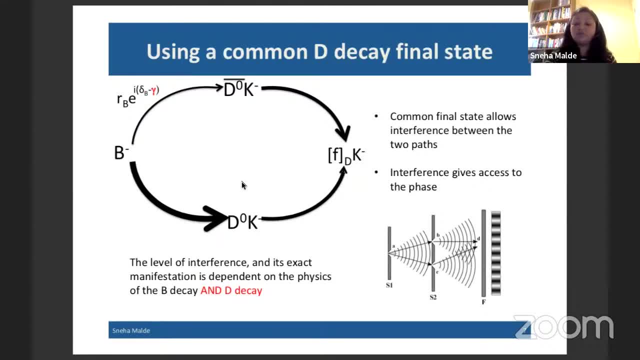 which means that we need to have the D0 and the D0 bar mesons decay into the same final state So that we can have access to the phase from the interference. The level of interference and its exact manifestation is going to be dependent on the physics of the B decay. 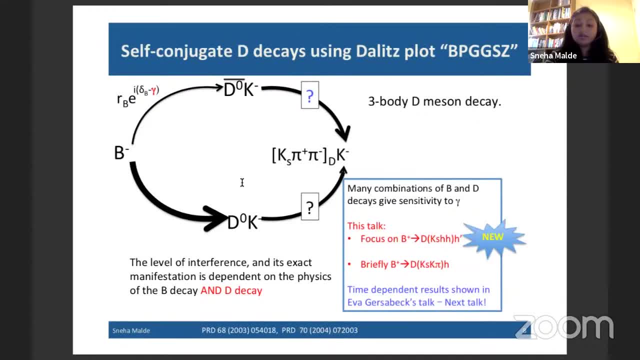 but also of the D decay. The measurements I will be telling you about today will mainly be our new result, shown here for the first time, on B to D k, where D goes to k- short pi pi or k- short k k. I will briefly show you the results from: 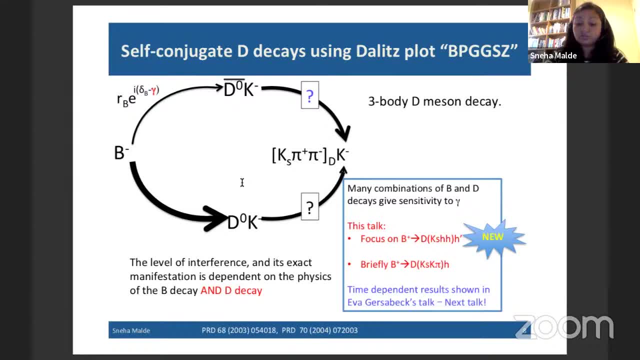 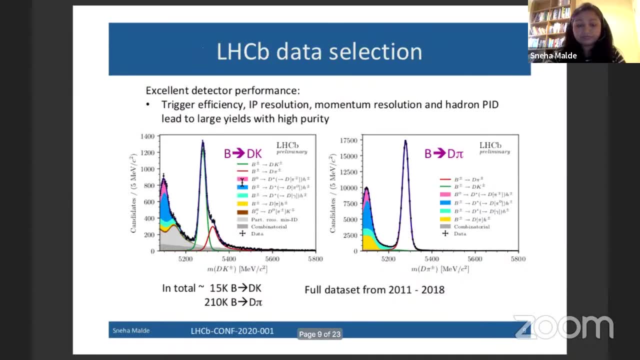 a similar analysis where the D decays to k, short k pi, And Ava will tell you about some of our time dependent results in the next talk. So if we take a look at our data collection for B to D k and B to D pi, 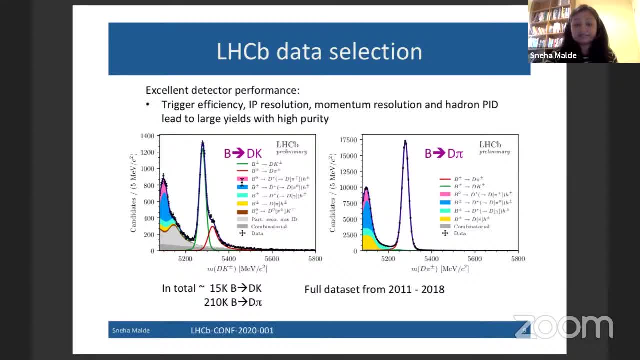 this is our full data set from 2011 through to 2018.. We can see that the excellent detector performance has given us great- you know it's given us great performance here, So we have very large yields. So 15,000 B to D k and 210,000 B to D pi. 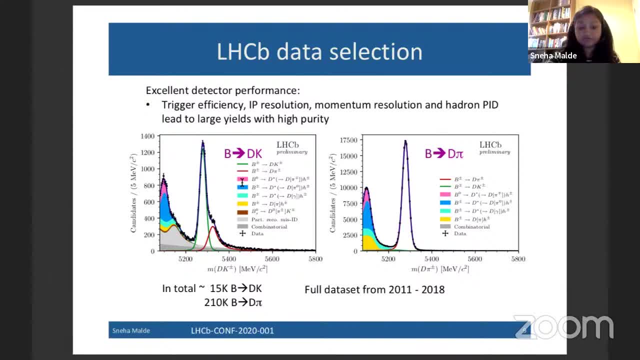 And this is a result of having excellent hadronic trigger efficiency. The IP resolution that we have means that we can really beat down those combinatorial backgrounds And the momentum resolution means that we can separate this partially reconstructed background on the left hand side from the signal very well. 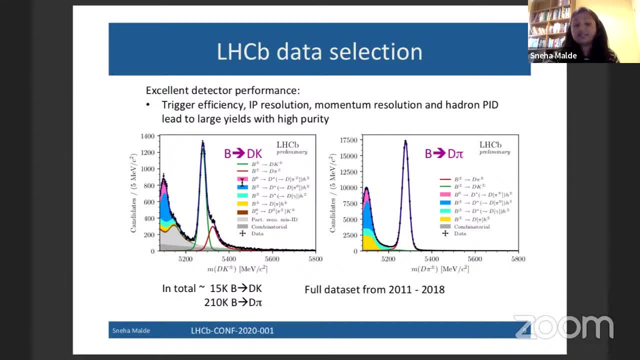 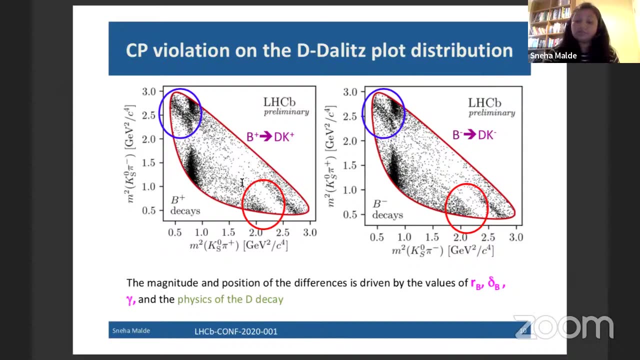 And finally, our hadron PID means that we can select out B to D k very cleanly from B to D pi, which has 12 times the branching fraction. So if we were interested to see what CP violation would look like, we would take a look then at the Dalitz plots of the D decay from B plus and B minus decays. 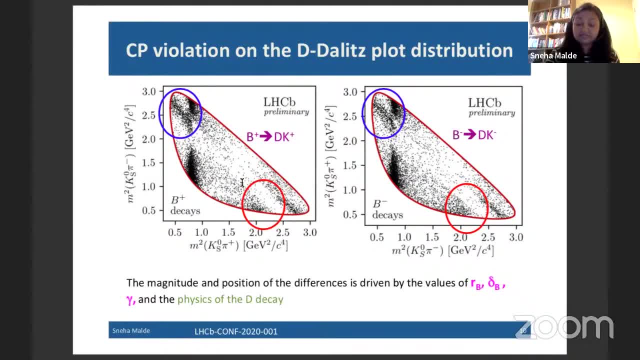 You can see that already with the statistics that we have. these differences are visible by eye. So, for example, if you take a look at the red circle, you will see that the points in the left hand plot are more constant, concentrated than the ones on the right hand side. 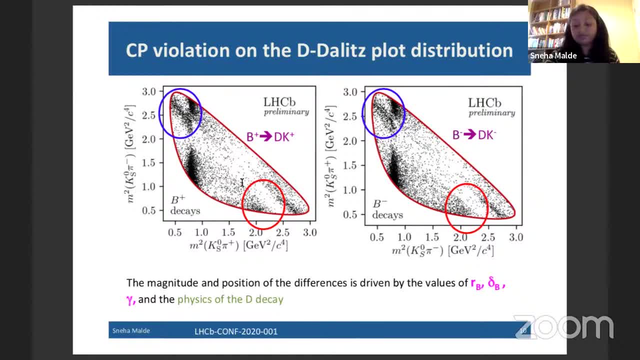 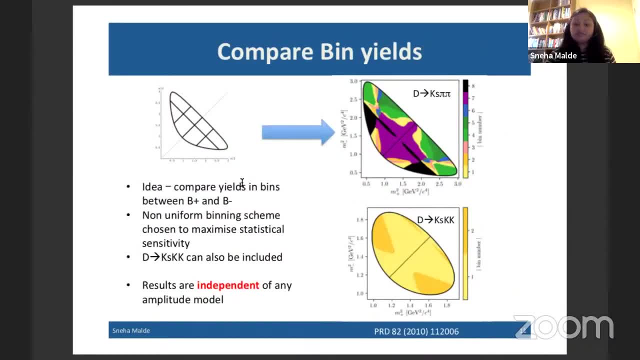 And the magnitude and position of these differences is driven by the values of gamma and also these other hadronic parameters. So the idea of the analysis is quite simple. We just want to compare the bin yield between B plus and B minus decays. We don't use a standard rectangular binning because we know that this is likely to dilute our statistical sensitivity. 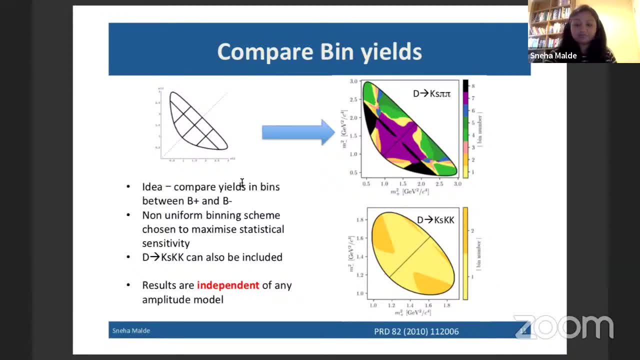 So we use these highly non-uniform binning schemes for k-short pi pi- and we can also add k-short kk- And these have been designed to maximize our statistical sensitivity. The key point here is that the results are independent of any amplitude model. 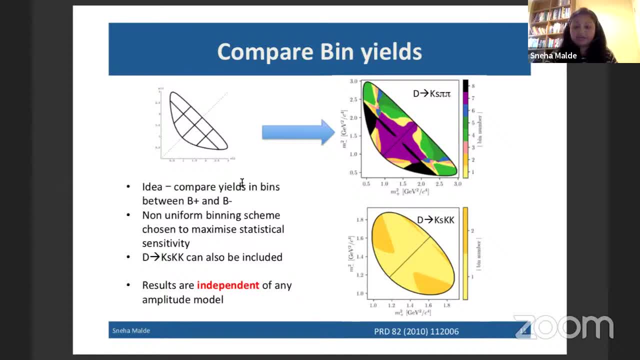 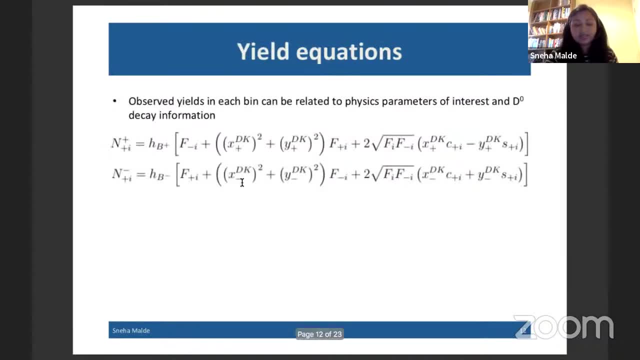 And this means that we don't have to worry about how we are assigning our systematic uncertainties, which is important when it comes to precision measurements, So we can compare the yields to um, um a number of parameters, So the equation looks complicated. 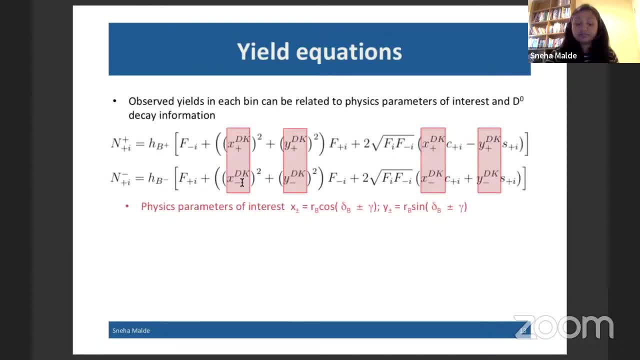 but it boils down to these x and y parameters, which are our physics parameters of interest, and they basically parameterize the real and imaginary parts of the amplitude and they have the sensitivity to gamma. We then have the ci and si, which are essentially strong phase parameter measurements of the d decay. 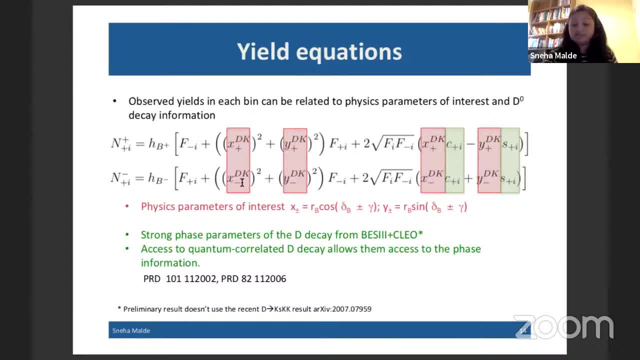 So this is the information that we need about the d decay. It comes from BEST3 and Clio, and the reason why it has to come from another experiment is that we need um, a system that can access these parameters, And one of those systems are quantum correlated d decays from the ci double prime. 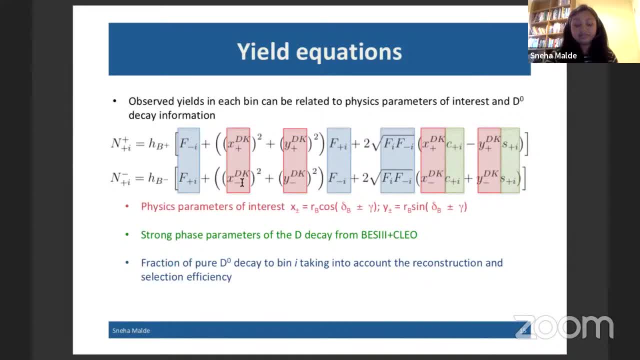 Um, and finally we have um, the, these, these F parameters, and this is just the fraction of the pure d zero decay into a given bin, taking into account reconstruction and selection efficiency. One of the key parts of the analysis is: 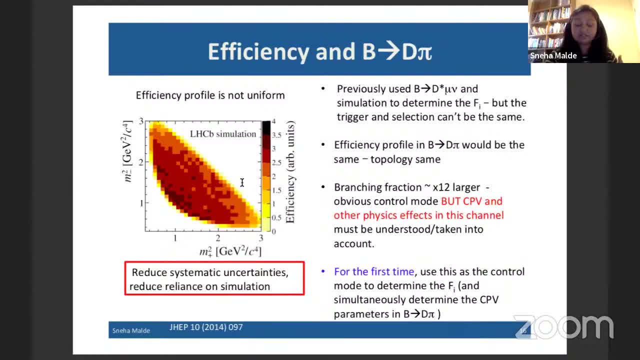 is is um attaining these Fi to measure them. We know that our efficiency profile is not uniform at LHCb um and previously we've used b to d star mu nu as a control mode to determine the Fi. But the trigger and the selection can't be the same. 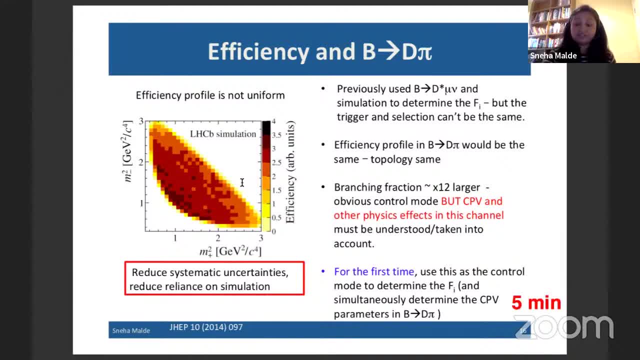 and it was becoming clear that we would be leading, for you know, very large systematic uncertainties if we continued to, to, to follow the same path. Ideally, um, the, uh, the, the best control mode would be b to d pi. 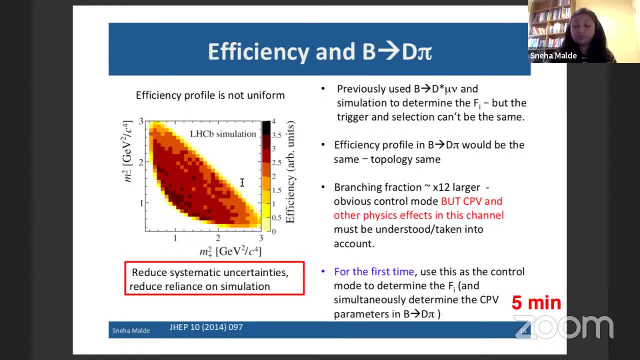 It has the same efficiency? uh, because the topology is the same and we can apply the same selection. Also, the branching fraction is 12 times larger than b to d k. So there are enough statistics there to to to control, But it. 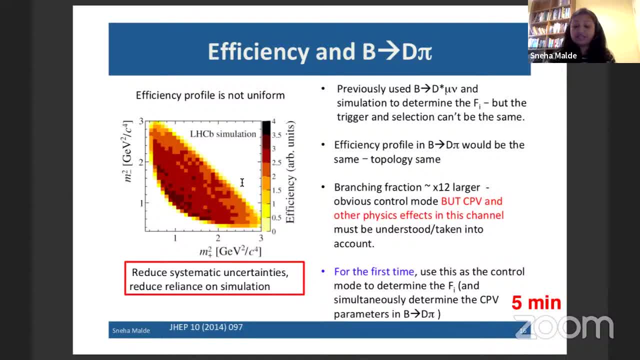 it. it will always been a worry that the CP violation in the decay mode and other physics effects in this channel may make um uh, a problematic- maybe problematic in the actual execution of the analysis. However, we've understood these physics effects much better now. 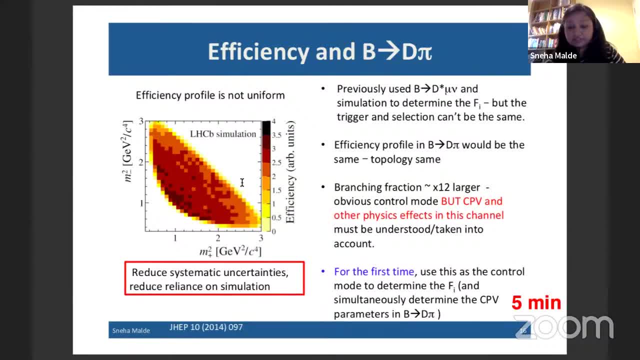 And we also know how to take into account the CP violation, And so, for the first time, we use this as a control mode to determine the FI and simultaneously determine the CP violation parameters in b to d pi. So we perform a fit which is essentially the fit to the invariant mass model. 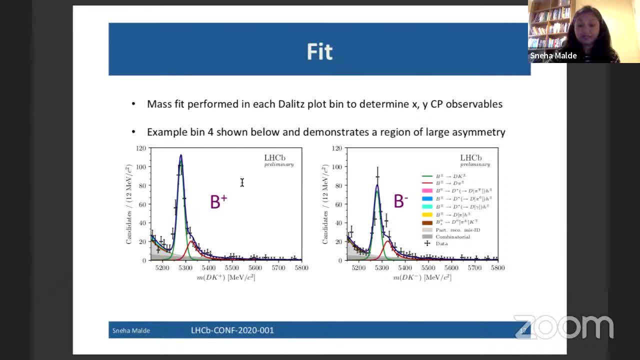 um, the invariant mass spectrum in each bin. separate um simultaneously And we use that to determine the X and Y CP observables. What I've shown here is um been plus four Um, so we've got a fit of four. 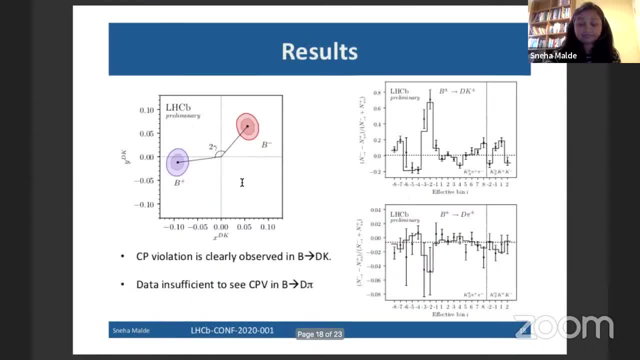 which is one that exhibits um a large amount of asymmetry. If we take a look at the results, we can plot X and Y, And the signature for CP violation is that these two blobs are separated, And so you can see that they clearly are separated. 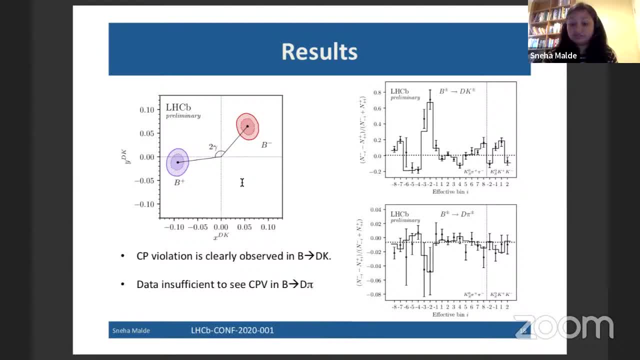 And if we take a look at the bin by bin pair asymmetries, you can see that we do in b to d k see some very large asymmetries and that the fit predictions match the data very well. Um on b to d pi. 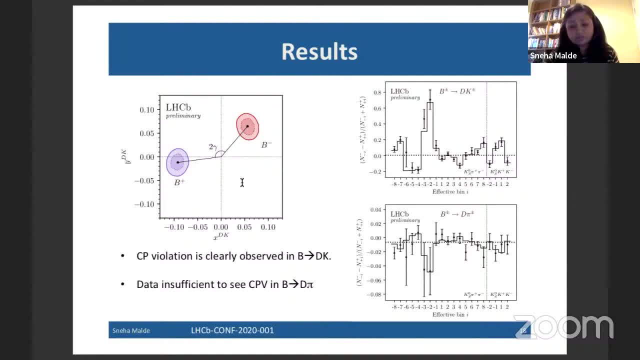 the CP violation is expected to be an order of magnitude smaller, So the asymmetries that we're expecting are much smaller And for this reason the data is not yet sufficient to be able to um say that we can see CP violation in this decay mode. 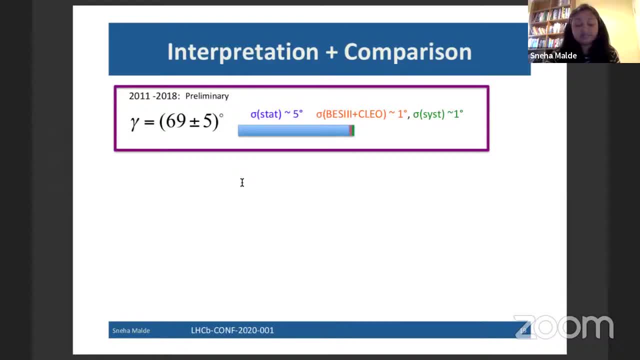 We can compute um the value of gamma from these CP observables, And so we measure gamma to be 69 plus or minus five degrees. That is nearly all um that is dominated by the statistical component um, which is about five degrees. 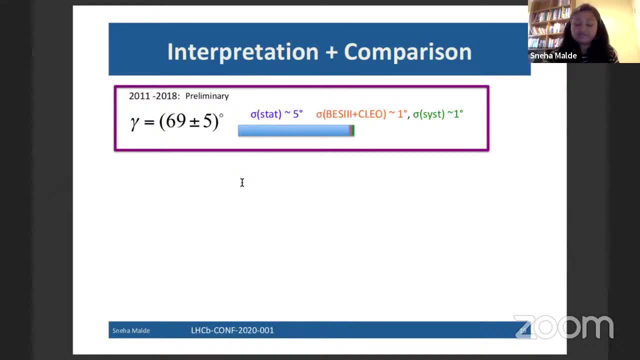 And then we have two sources of um. well, we have two classes of systematic uncertainty. One comes from the propagation of the uncertainty on the strong phases, which are the measurements from best three and clear, And you can see that they um. 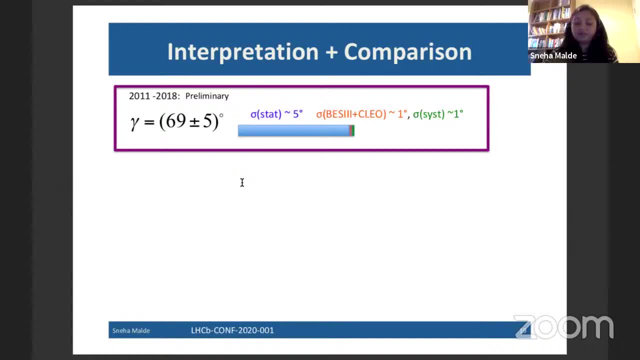 have an uncertainty of around one degree, And then we have um a number of systematic uncertainties from the experimental side on LHCB And these add up to about one degree as well. We can compare that to our previous measurement that used uh. 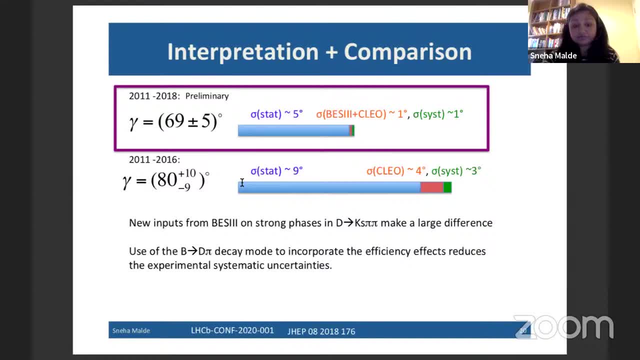 2011 to 2016 data And you can see that this is um a substantial improvement. Um, we've gained in statistical uncertainty by adding the two years of data and some small improvements to the selection, But one of the key points here is that the old 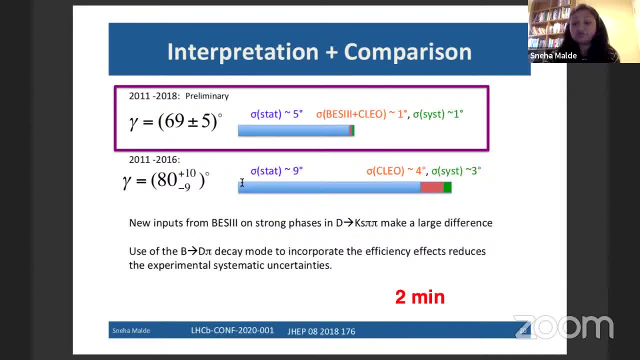 um, uncertainty from clear, which was about four degrees, is now shrunk to about one Um, and this is um. and you can imagine that if we still had a four degree uncertainty, we w you know, there is no way we could reach a precision of five degrees. 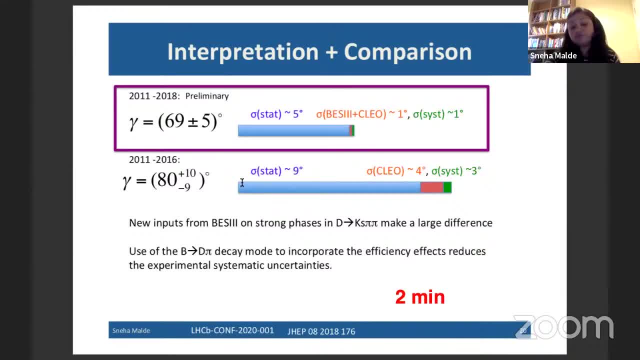 Um, and so these new inputs from best three have made a big difference. And then, secondly, we've been able to very much reduce the systematic uncertainties from the experiment by using this B to D pi mode um as the control We also measure. 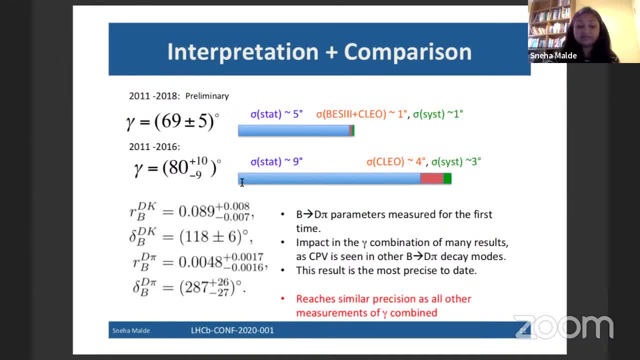 um. a number of hydronic parameters and um. the B to D pi. hydronic parameters are measured for the first time and they will have impact um when they go into the full gamma combination. The measurement of gamma reaches a similar position. 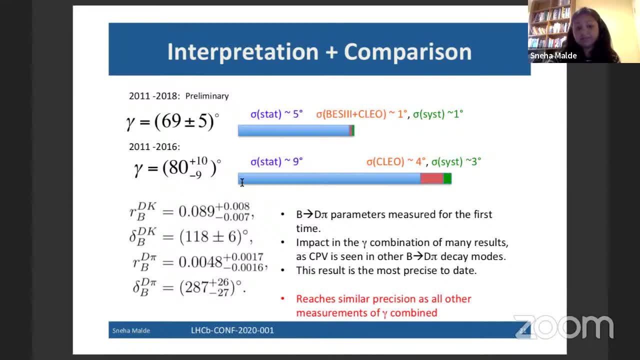 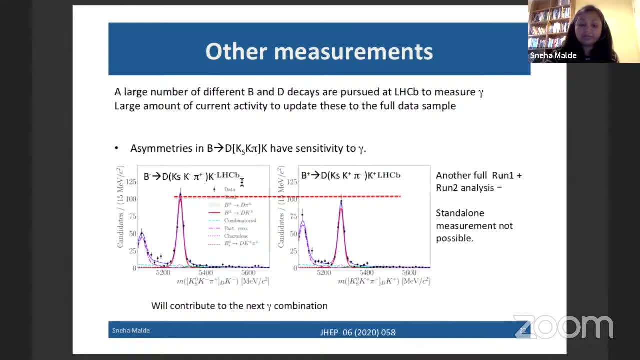 uh similar position as all other measurements of gamma combined. As I said, we have a large number of B and D decays are being pursued at LHCB to measure gamma And um. a large amount of. there is a large amount of current activity to update these to the full data sample. 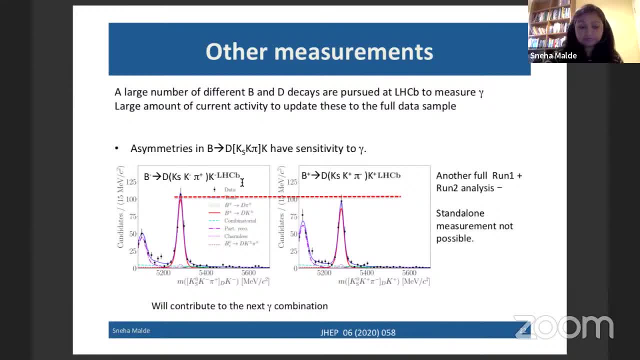 um, or even introduce new methods. I show here another decay mode, which is B to D, k, where D goes to k, short k pi, Again asymmetries, um, and so on. So, um, this is a. 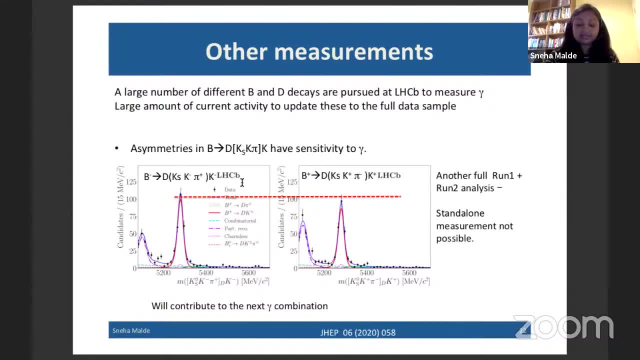 um, as as a standalone measurement, this doesn't have direct sensitivity, Uh it, it can't make a measurement of gamma on its own, but it? uh does contribute to, uh uh, a combined measurement of gamma. 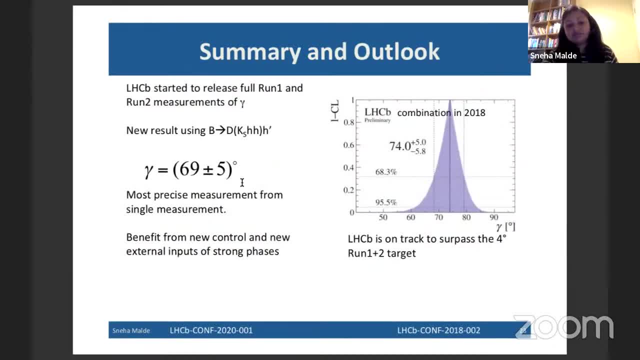 which will be put into the next combination. So to to summarize, LHCB have started to release full run one and one team measurements of gamma. We have, um, a new result, um which has um a precision of. 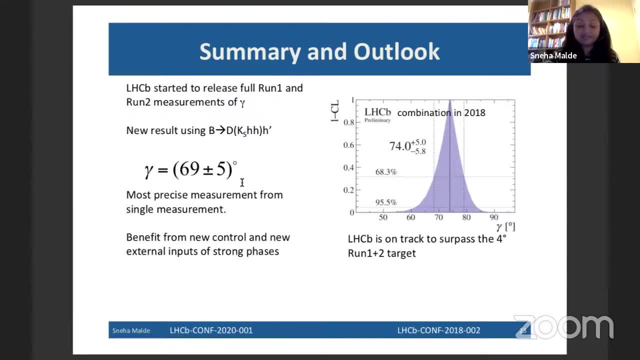 of about five degrees And it's the most precise measurement from a single measurement, And we have benefited from new control modes and new um external inputs of strong phases If we take a look at how the LHCB combination looked in 2018,. 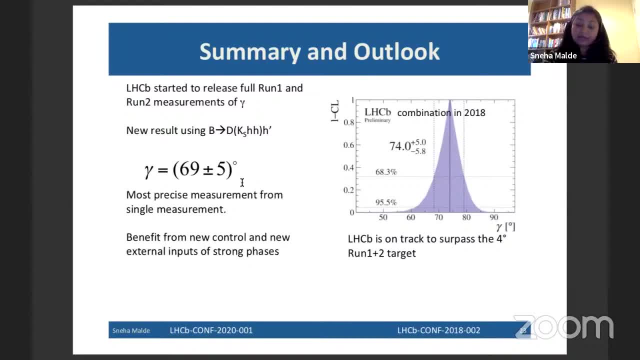 you can see that once these measurements are added to it, the LHCB is is well on track to to to surpass the four degree- one one plus root, one, two target- And so we put ourselves in a very good place for the upcoming upgrade. 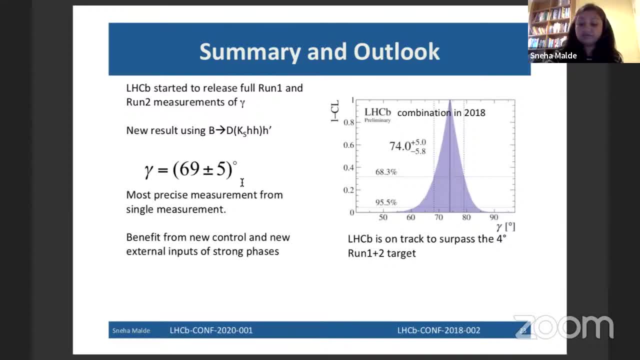 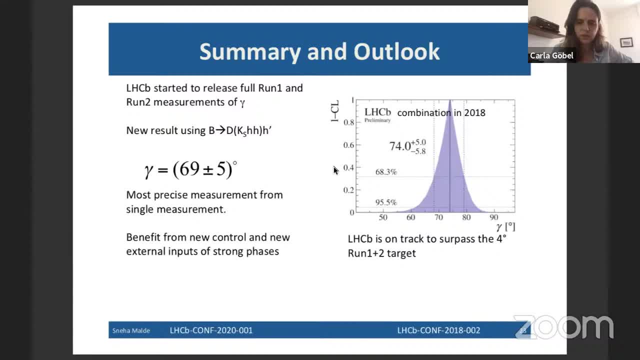 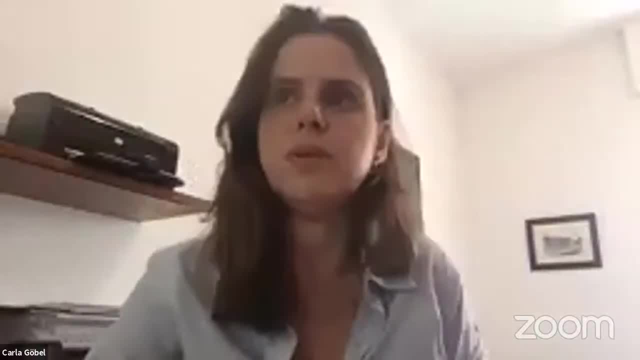 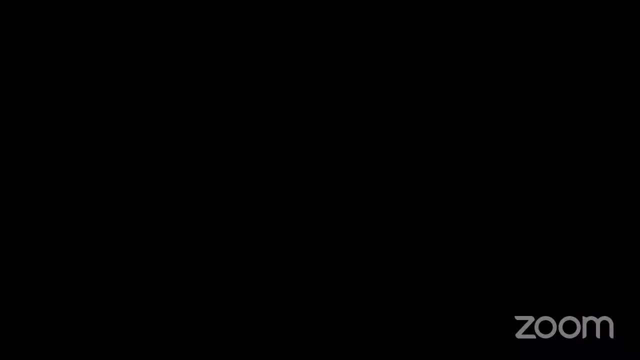 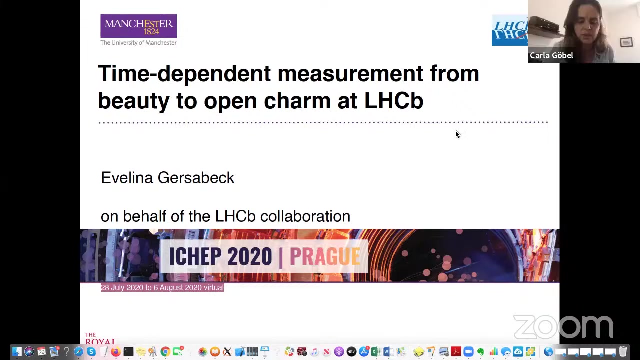 uh continue with. uh ever gets our back with uh the time. dependent measurements from B2D, LHCb. so I think that is uh. that is all I can uh apply to. Thank you. Can you see my screen now? 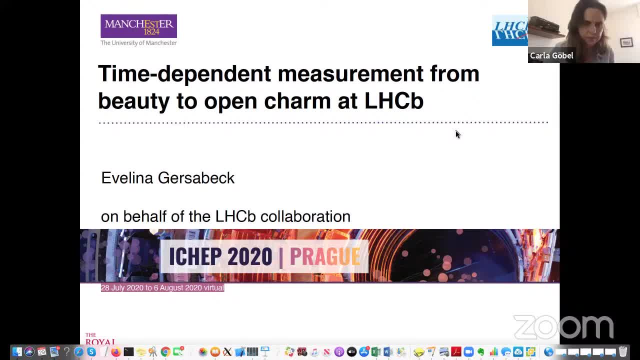 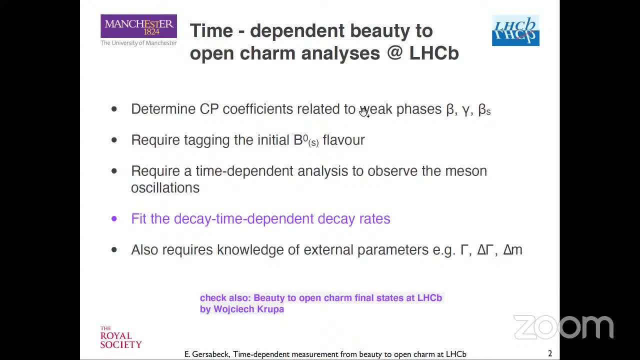 Not yet. Yes, now I can. Okay, thank you very much for the introduction, So what I will speak about now is pretty much complementary to what Sneha presented. I'll be speaking about the time-dependent beauty-to-open-charm analysis we do at LHCb. We're interested in them because they are sensitive to the weak phases. 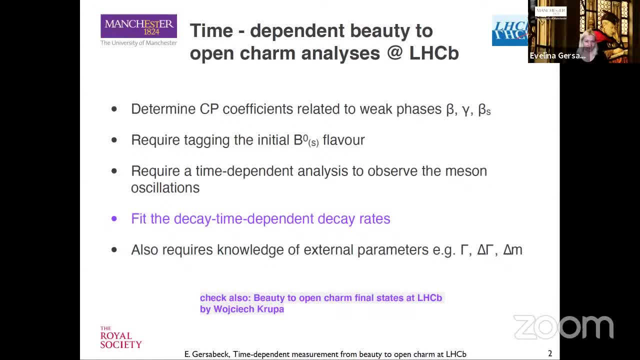 beta and gamma and beta s, and we do them in a time-dependent way. When we deal with neutral beam mesons, this we do in order to resolve the beam meson oscillations, and to do that we fit for the decay- time-dependent decay rates and we extract the parameters of interest. So these measurements also require 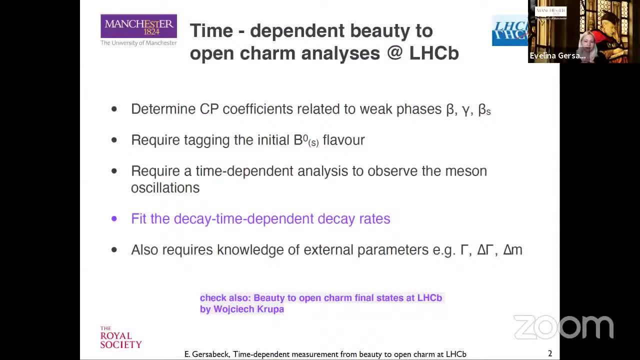 a knowledge of the external parameters: gamma delta, gamma delta m and a few others you will see in the slides thereafter, And to check for further updates on these charm final states at LHCb, you can check the talk by Wojtek tomorrow in this. 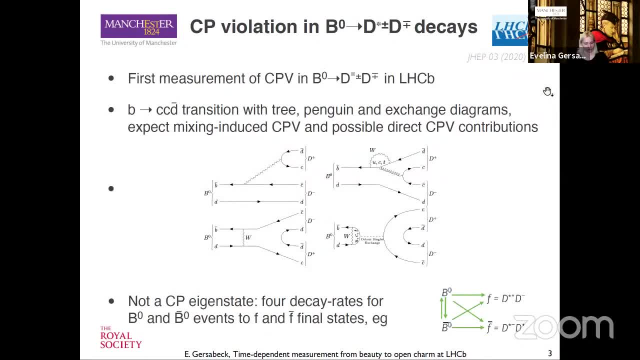 session. I'll start with the B0 to d star d decays where d, star and d are charged, and this is the first measurement we do in these decays at LHCb. It's been done previously by Bell and Babar. Here we're dealing with a B2CC debark transition where we have three penguin. 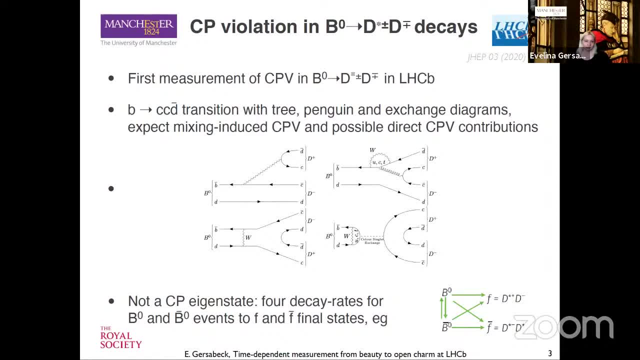 exchange and annihilation diagrams. Therefore, in addition to the mixing induced CP violation, we also expect possible direct CP violation contributions. And in the little sketch in the corner you see the possible decays of the B0 and the B0 bar decays. These decays are all accessible from all states. in addition to that, you 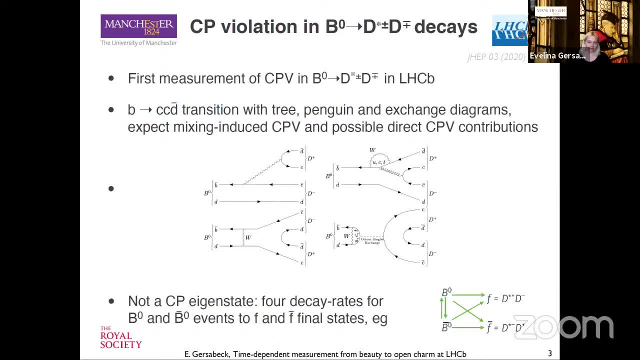 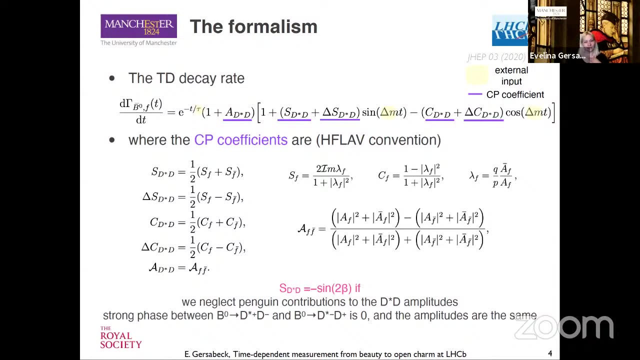 have the B0, B0 bar oscillation. Therefore we're sensitive to CP violation. as I said, interference, and also the direct one. On these slides you see the time-dependent decay rates. I've highlighted with yellow the external coefficients we used or the decay time. 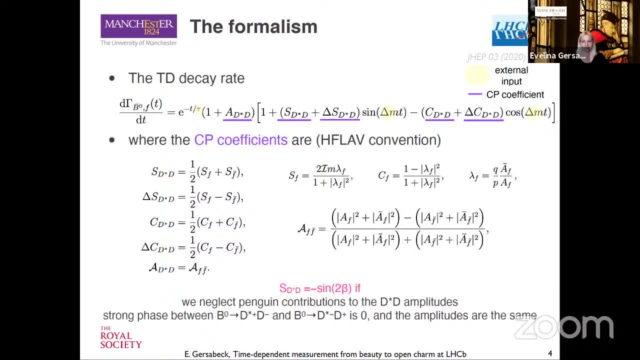 and I've underlined with purple the CP coefficients which are of interest to this analysis And you see the definition also of these coefficients using the H-fluff convention and their relation to the, for instance, lambda f, the CP parameter, and the overall asymmetry between the F and FFR final states. So the one 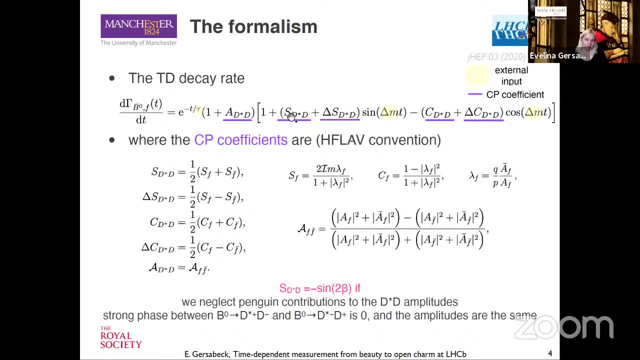 CP coefficient which is of most interest to us in this case is the S d star d which, if we assume, no, if we assume that we can neglect the penguin contributions, which are known to be about a few percent, and we can essentially assume there is no direct CP violation, if we can assume 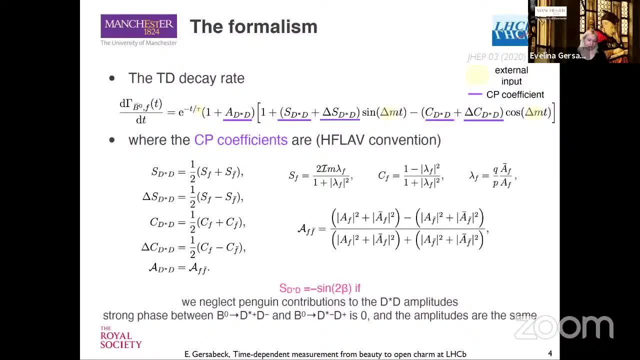 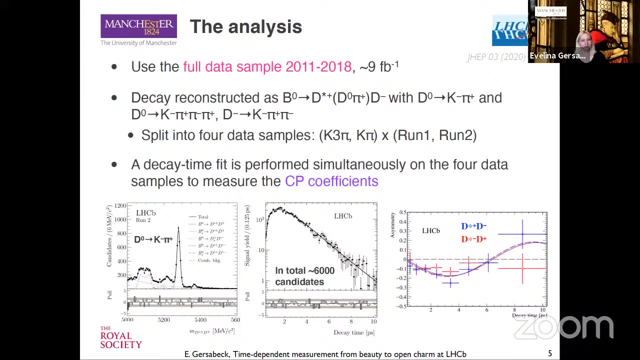 that Then the S d star d would be a good approximation of the sine two beta, which is the angle of the unitary triangle. So for this analysis we use the full sample of run one and run two, which is about nine inverse time. 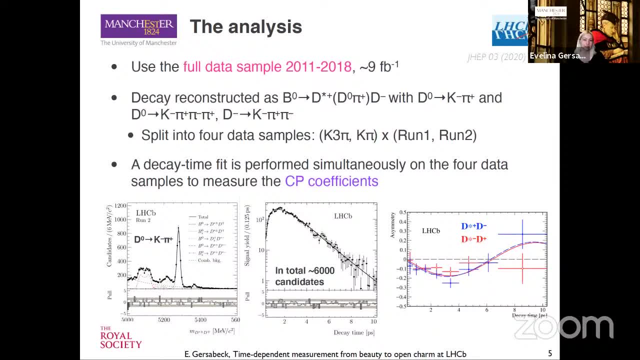 to bond. And here we split our data into four subsamples, according to the decay of our intermediate, the zero mass, and according to the LH run. And we fit that. You see on the left plot the fit to the invariant mass of one of those four subsamples. 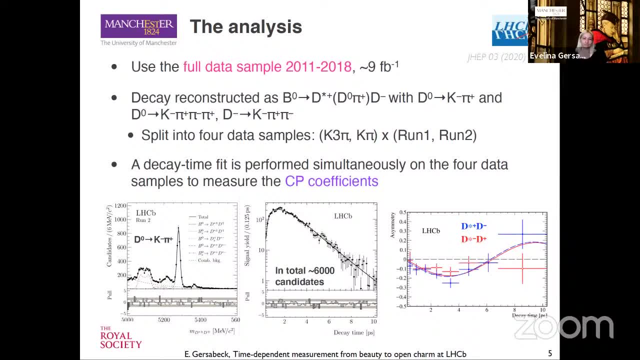 And then we fit simultaneously all the four subsamples and we perform a decay time fit And we use about a total of six thousand candidates to measure the CP coefficients of interest. on the plot On the right you see the asymmetry between B zero and B zero bar decays, And actually on this slide you see the results for all. 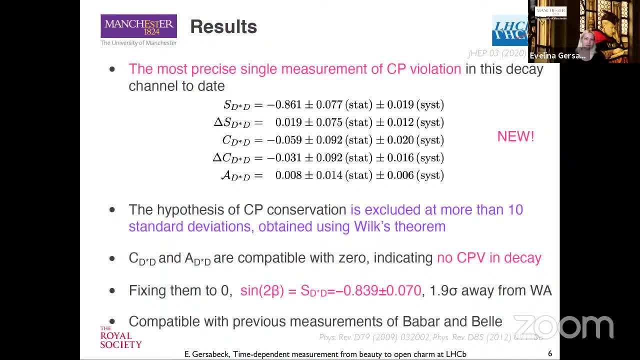 five coefficients And this is the most precise measurement of CP violation in this decay channel today. This is relatively new, So the publication went out this spring And the hypothesis of CP conservation is excluded with the great significance in the decay channels. What you note here is that 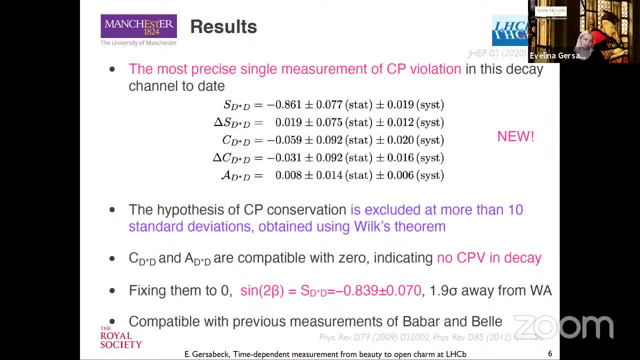 the coefficient c and the coefficient a are compatible with zero. therefore this indicates no CP violation in the decay, And then we can make this assumption that there is no direct CP violation. we can fix them to zero and we can repeat the fit, and then we get a value for sine. 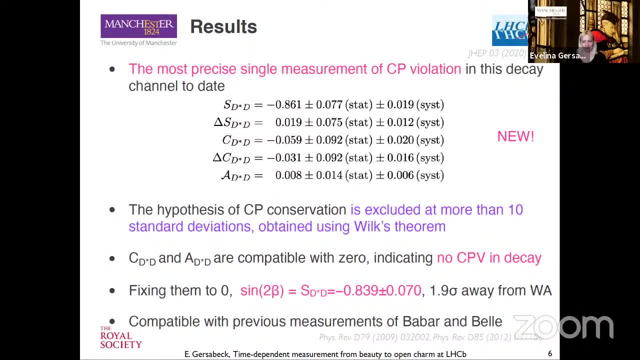 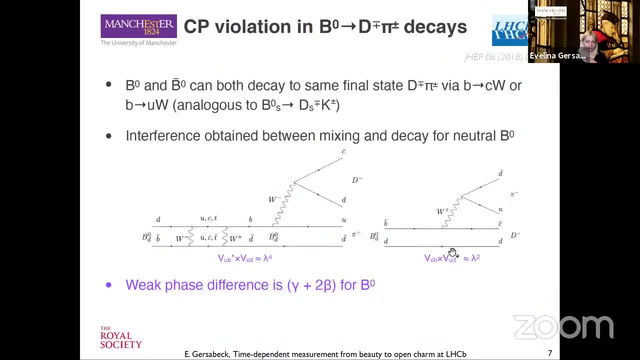 two beta which you see here, and this is about 1.9 sigma away from the world average. Okay, I'll move to the next decay I'll discuss. This is the second out of three time-dependent measurements. So here we have neutral B0 going to charge the meson and the pion decays. 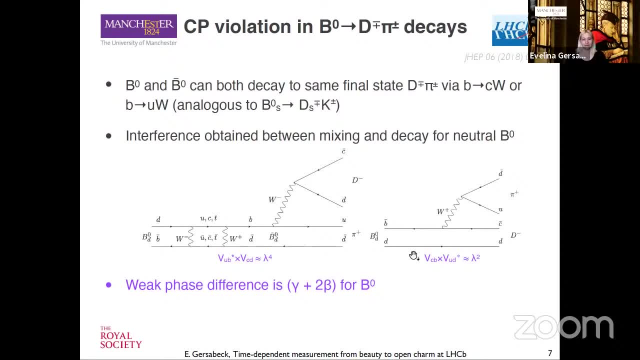 The two leading Feynman diagrams contributing to the interference in this decay channel. are the two leading Feynman diagrams contributing to the interference in this decay channel. are the two leading Feynman diagrams contributing to the interference in this decay channel You see below: we have a transition of B2CW and another one of B2UW. 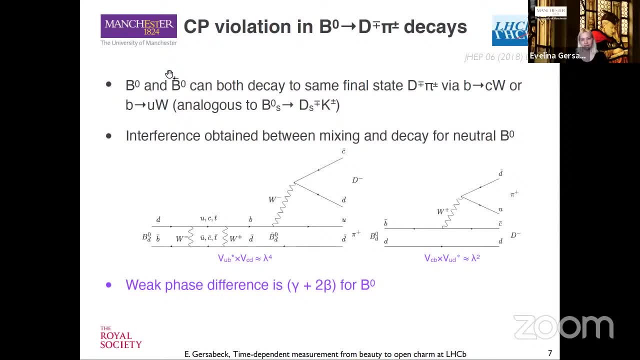 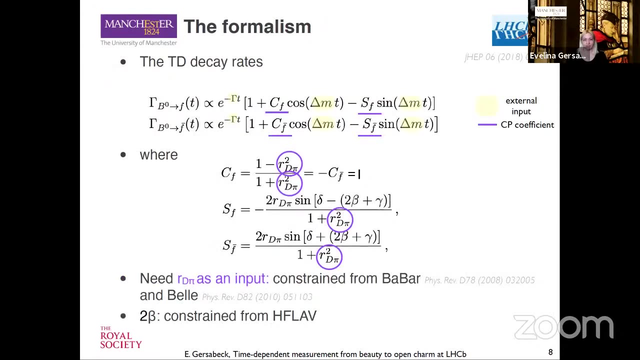 This is analogous to the last decay I'll discuss later B2DSK decays. So I mentioned we have an interference between them and the weak phase. difference between these is gamma plus two times beta. Again, we have time-dependent decay rates. so the correlation between these two, the top and bottom, is actually much higher than what we've experienced. 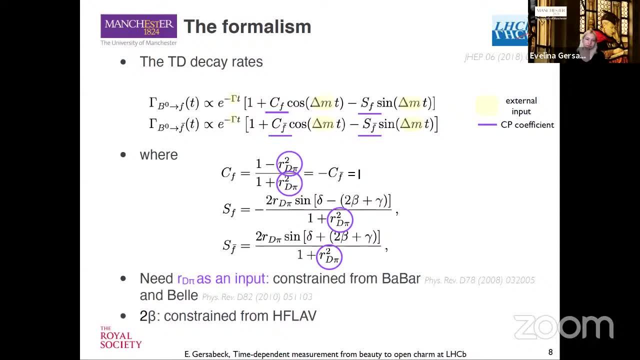 in a random configuration of b1 to b2.. We can set it to one because we know that the magnitude of RDP is quite small. it's below two percent. So, thank you, We basically effectively remove this out of the equation and we set it to one. 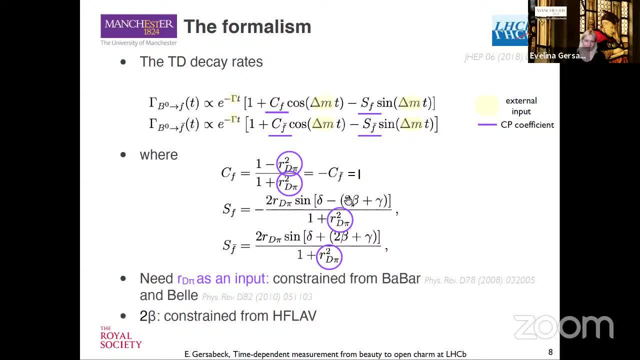 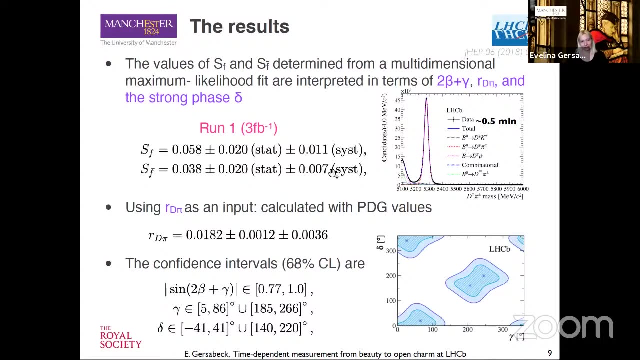 RDP would also be used in the other as an input and we can constrain that from the bar and bell Two times beta. we would constrain from the H-flow. Therefore we extract the values of Sf and Sf-bar from a multidimensional fit. 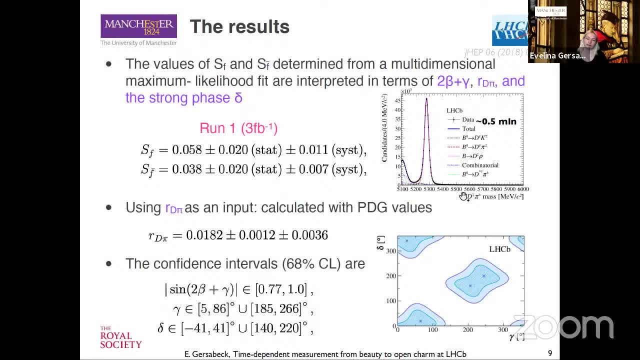 One of the components, one of the fits we perform is to the invariant dpi mass which you see on the top plot. We have a very, very clean, peak, very significant data. We have close to half a million events And you see our results. 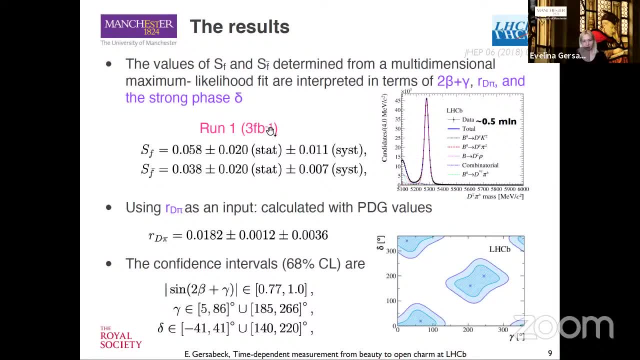 This is the result for Sf and Sf-bar using our RUN1 sample, And then we use this CP coefficients to constrain further the strong phase delta and gamma. And you see the intervals, the confidence intervals, for these variables, delta and gamma. 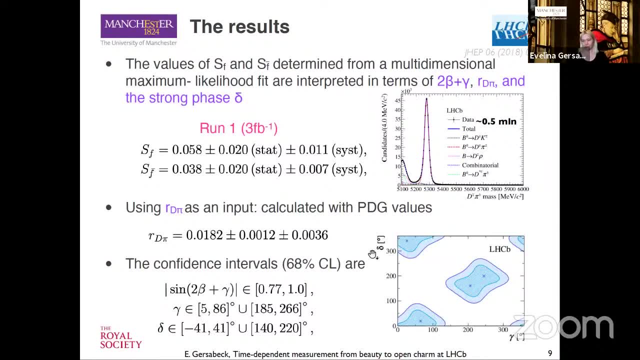 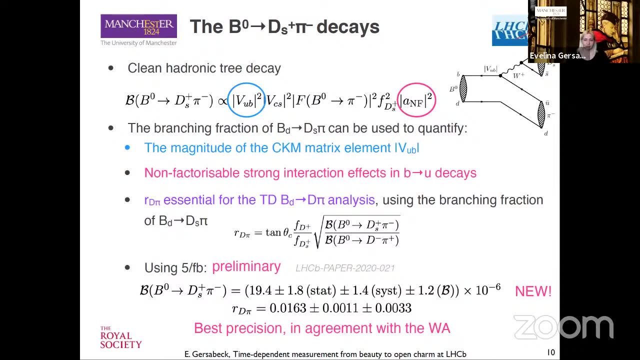 and also the two-dimensional scan at the bottom plot of delta versus gamma. As I mentioned, we need the RDP as an input. We are able to calculate it And for the analysis I just presented, that's been done using information from the PDG. 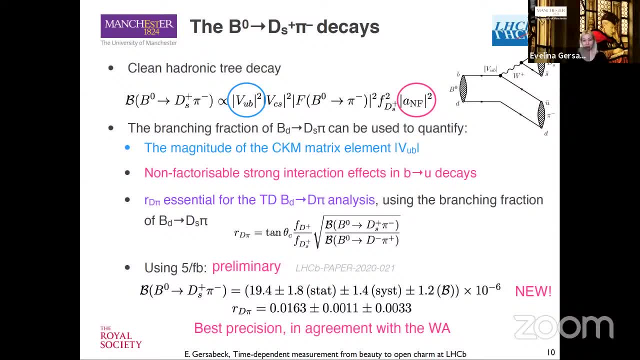 using measurements of Bell and Babar, But we can also measure it at LHCb and we're doing it using B0 to dspi decays. We can do that because we have a clean hydrometer. We have a clean hydronic 3-decay. 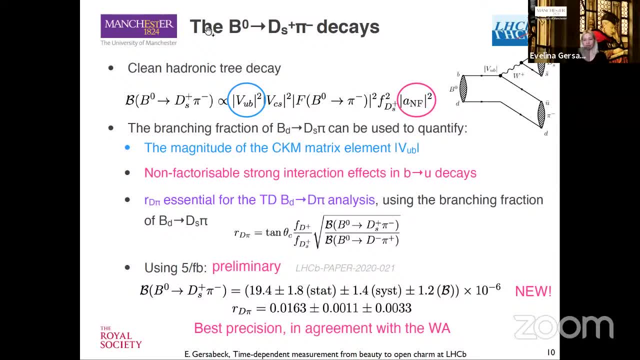 You see the Feynman diagram here in the upper corner, And the branching ratio of these decays is interesting because it's proportional to the CKM element, Vub and also to some non-factorizable strong interaction effects in BTU decays. However, what's most interesting for us in this case is that we can use this branching fraction to calculate RDP. 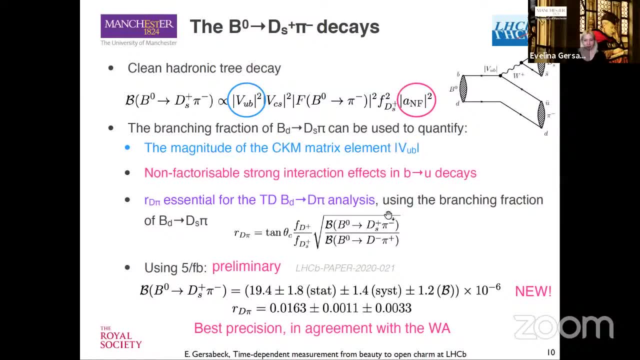 using the second formula on this slide here And here it's how this branching fraction enters. So, using 5-inverse, 5-to-Barn RUN1 plus part of our RUN2 data, we're able to measure this branching fraction and RDP. 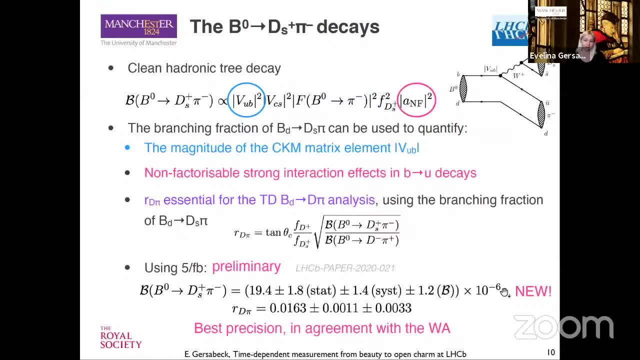 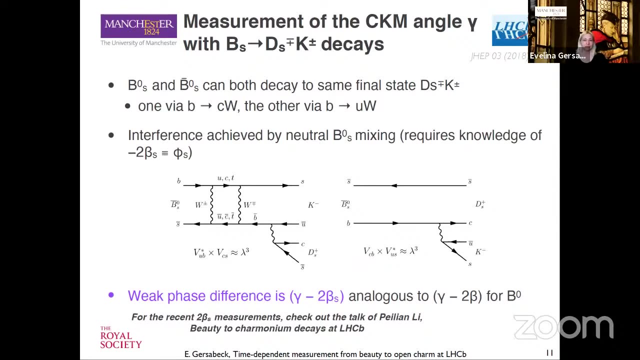 This is a new result, which is also preliminary, and Vojta will discuss it in more detail tomorrow. And here we have the best precision in this data And here we have the best decays, in agreement with the world average. OK, I'm at the last time-dependent measurement I will discuss. 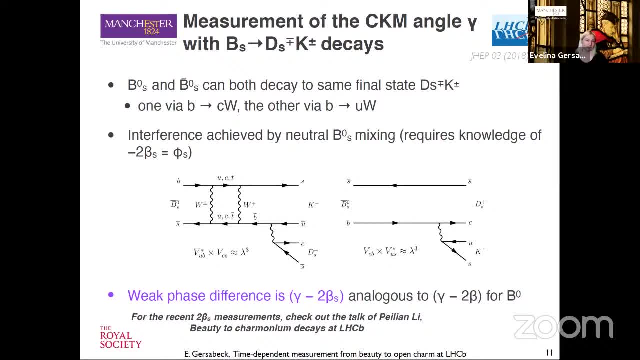 This is the measurement of the CKM angle gamma with a BS2DSK decays. This is very well known. Here, essentially, we have a similar situation. We have two leading diagrams with transitions of the B2CW and B2DW. 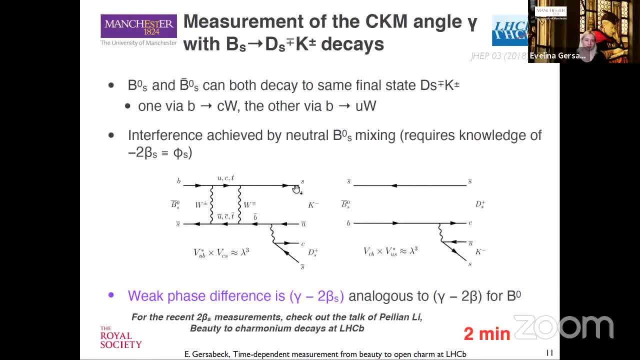 So here, in contrast to the B0-to-DPy, we have two amplitudes that are both proportional to them. The amplitudes are of the order of lambda to the third power, And here we have the weak phase difference of gamma minus 2 times beta. 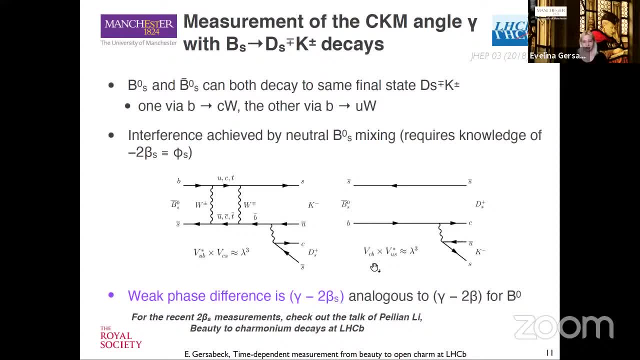 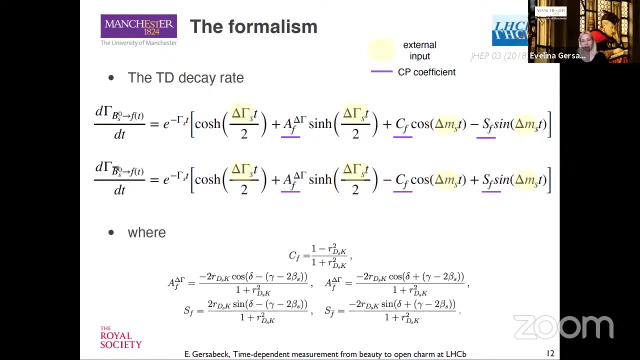 analogous to the gamma minus 2 beta. So beta S we take from other external measurements And if you're interested, check out the talk of Pei-Liang Li on the recent BS measurements with the LHCB experiments. Again, we have a time-dependent decay rate with external inputs. 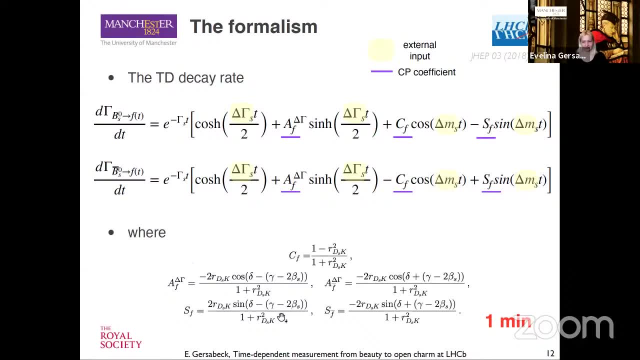 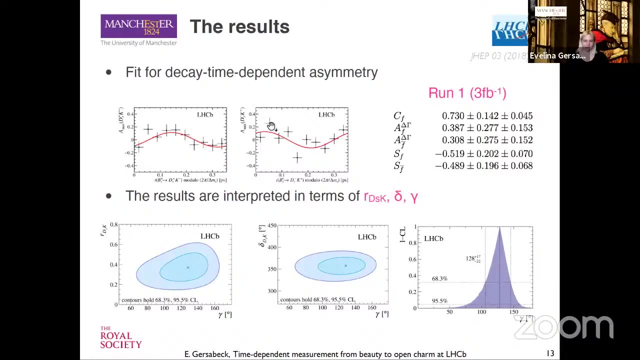 and the Cp coefficients. You see their relation to the thank you to the strong phases and the weak phases and the ratio RDSK. Here is what we determine with our run-1 data sample And using that we can actually also plot the asymmetries. 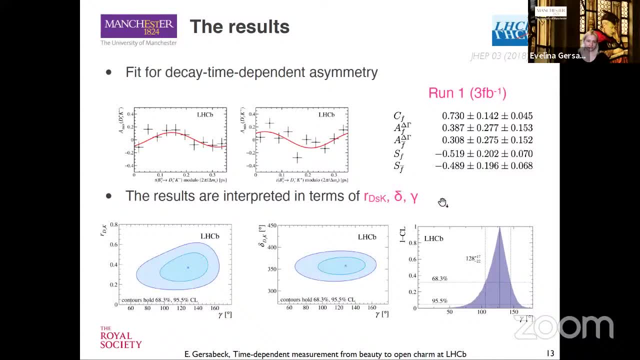 shown here above. We can also interpret these variables in terms of RDSK, delta and gamma. You see the two-dimensional scans of RDSK and gamma, the strong phase versus gamma, And then the single measurement of gamma, which is at about 128 degrees. 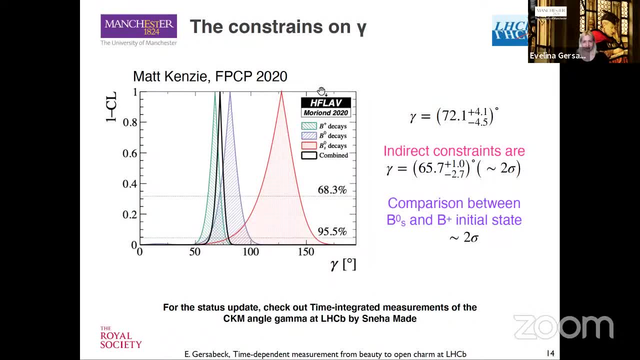 which is very nice. Then we use those as input to the combination of gamma, And Matt Kenzie has shown this plot at FBCP. So here the BS contribution is in red And you see it's a bit far away from the results. 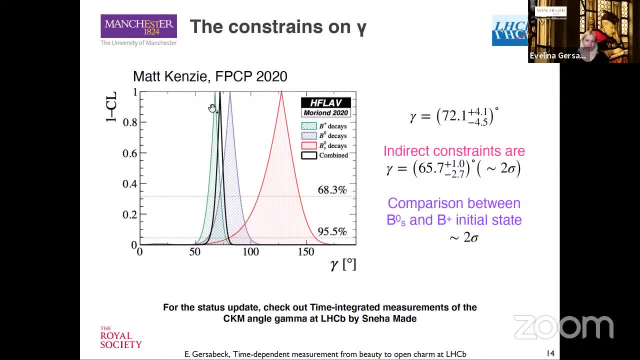 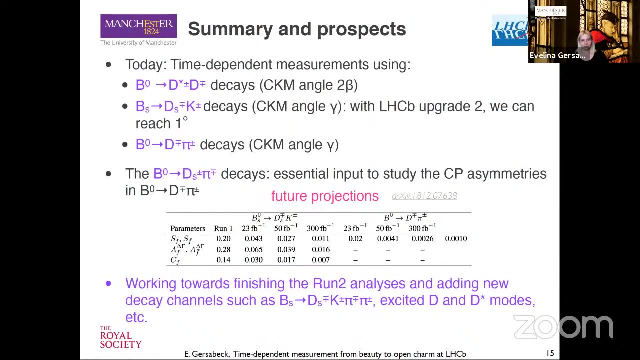 with using B plus and B zero decays, B plus being the results that Sneha just discussed, and probably this would be updated now after the results that Sneha updated. So there is a certain tension. We are very curious to understand where we have this tension from. 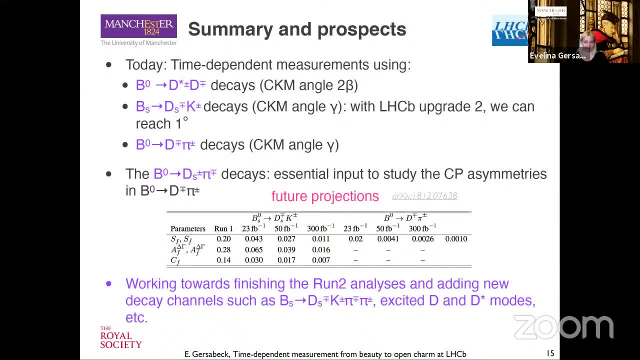 And I arrive at my summary and conclusions. I've presented three time-dependent measurements, The LHCb. they are sensitive to the CKM angles of two times beta and gamma. We've done some future projections what we can do with 50 and 300 inverse femto-Barnett LHCb. 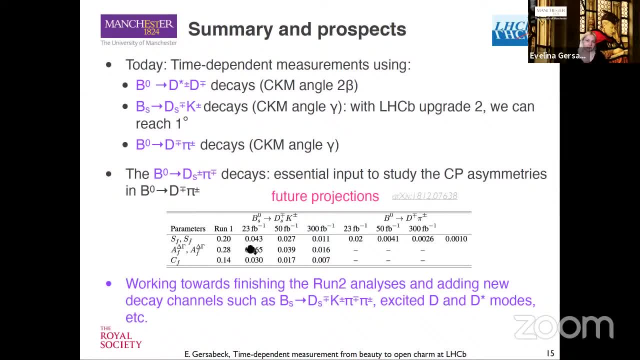 And probably, if there is one number to take from this slide, this is that with the LHCb upgrade two, we can reach a precision of about one degree with DSK decays, which is very nice. We are also working towards finishing our round two analysis. 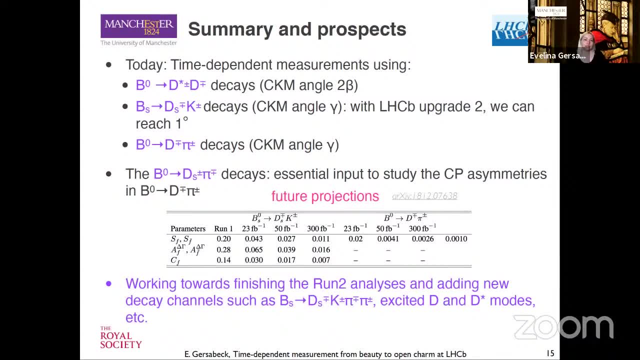 and adding a new decay channel, such as the BS2DS, KPI or some new states, including excited D and D star modes. So hopefully this will be available soon. Okay, that's all for me. Thank you, Eva. Questions from the audience. 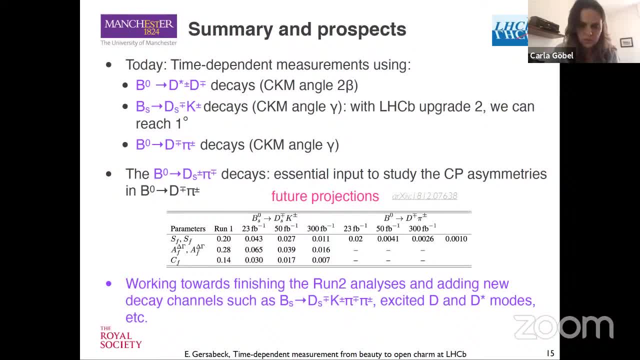 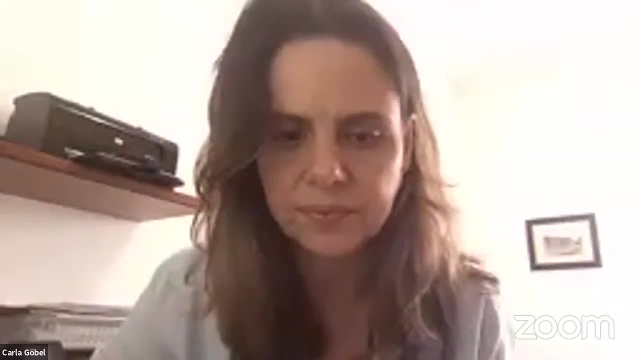 I don't see any. Please don't forget to use the Mattermole channel So you can if any question arises later. the discussions proceeds there, Thank you. Thank you, So we can move to the next two talks on FIAS. 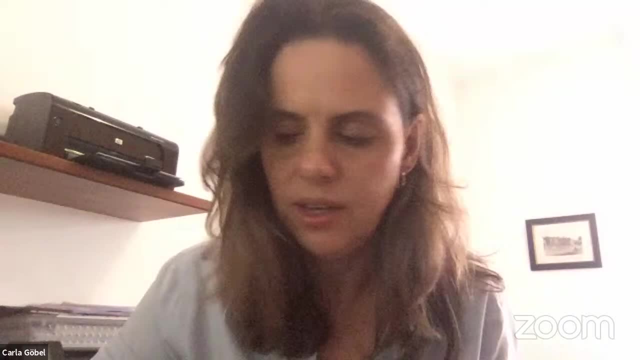 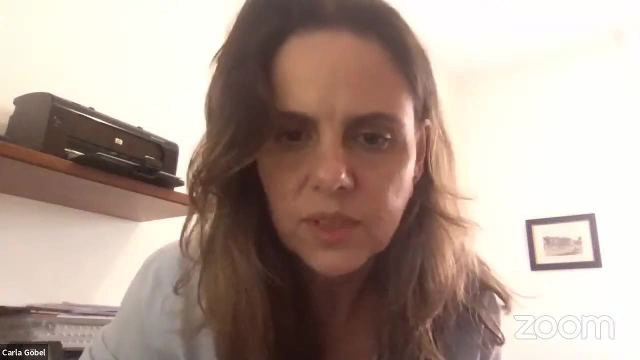 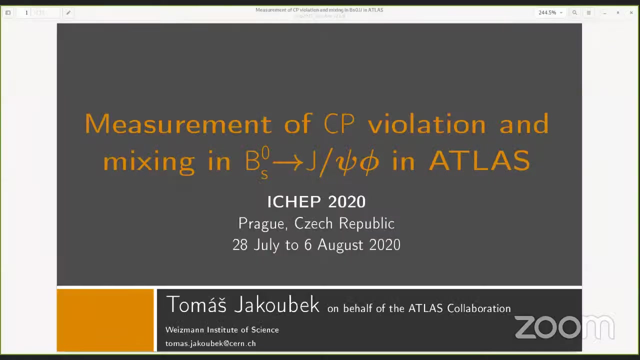 The first from Atlas Results on FIAS. from Thomas Back: Yes, hello, Do you hear me? Not so loud? Okay, Give me a second, It's better. It's better now, yes, Okay, So do you see my slides? 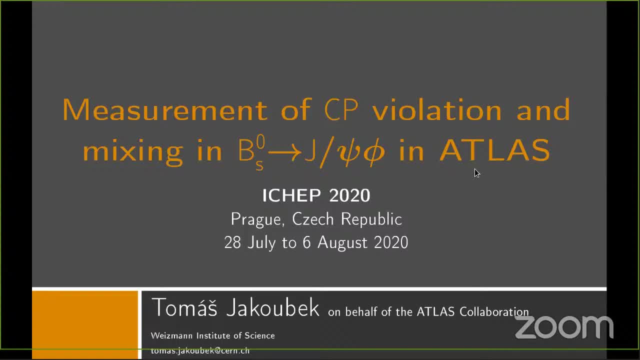 Yes, Okay, great, Thank you very much. Hello everyone. Good afternoon. So yes, I'm Tomáš, Tomáš Jakoubek, It's Czech name. I'm from the University of Czachornik. 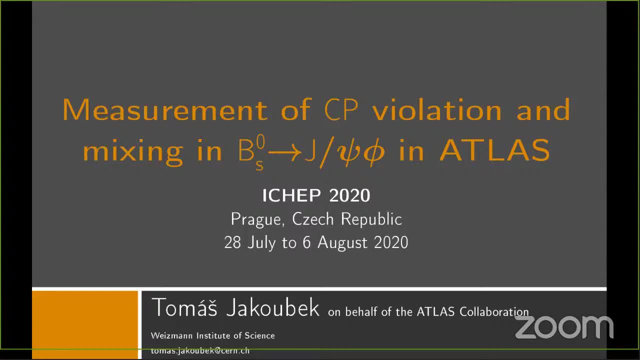 And I'm here, almost here, in this conference. So, on behalf of the Atlas collaboration, I'd like to show you the latest, or the updated results of our measurement of CPI violation in the BS2GiPsi phi decay channel. So this channel is expected to be sensitive to new physics contributions. 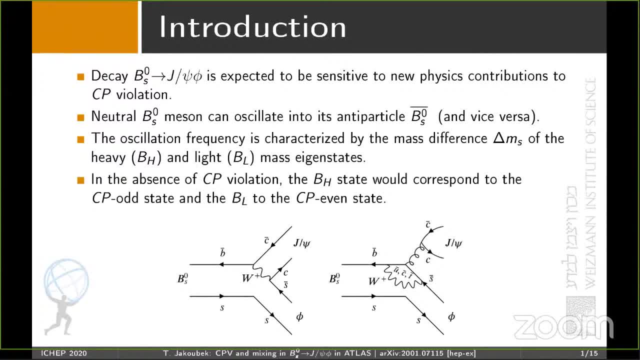 to CPI violation, and it's often called golden channel by the community Before the decay. the B meson can oscillate into its antiparticle particle, and this oscillation can characterized by by the mass difference between heavy and plus light mass eigenstates. if, in the absence of the cp violation, these states would then correspond to: 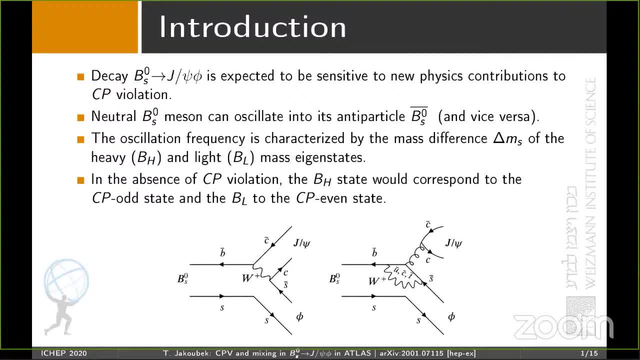 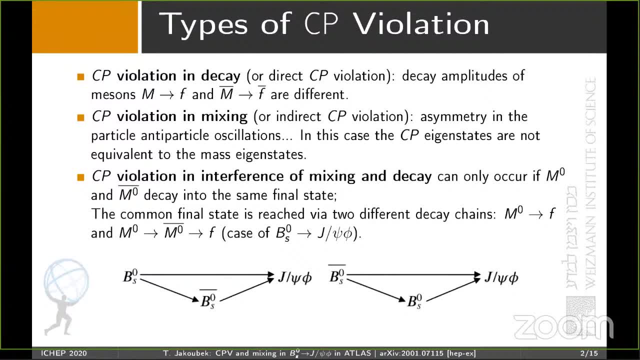 the flavor eigenstates. so in general we define two types of cp violation: violation in decay, where the amplitude of meson to the final state is different from the decay amplitude of an anti-meson to anti-final state, then there is a violation in mixing. in other words there's asymmetry in the 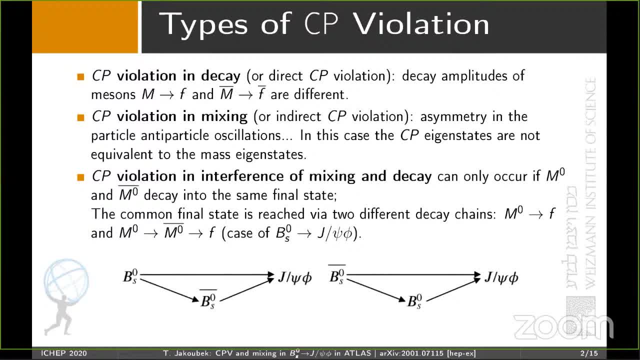 part in the particle antiparticle oscillation, and these two processes or these two types of violation can interfere, and so we define cp violation in the interference of mixing and decay. this one is only possible if meson and its anti-meson decay in the same to the same final 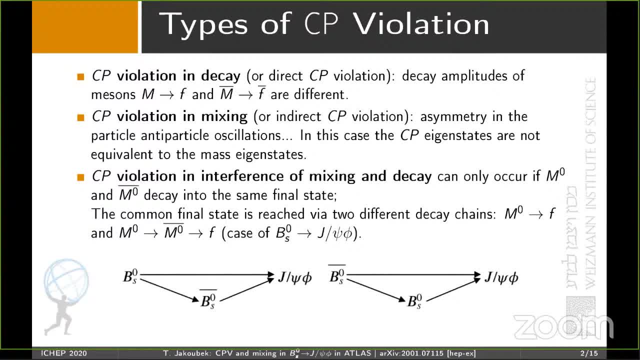 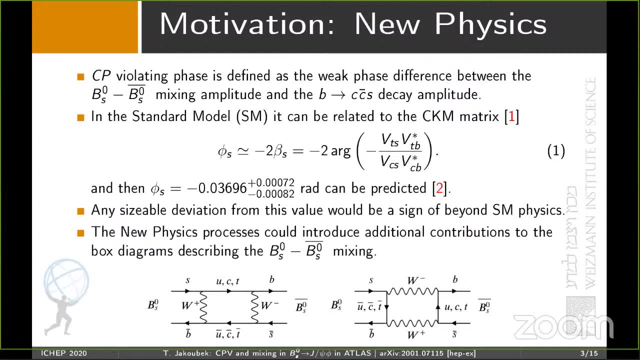 state. in other words, the oscillation can occur before the decay. this is of course the case the bs2, jpe, sci-fi decay channel. so what? what define the cp violation in this channel is a weak phase. a weak phase difference between the mixing amplitude and b to c c bar s transition amplitude. 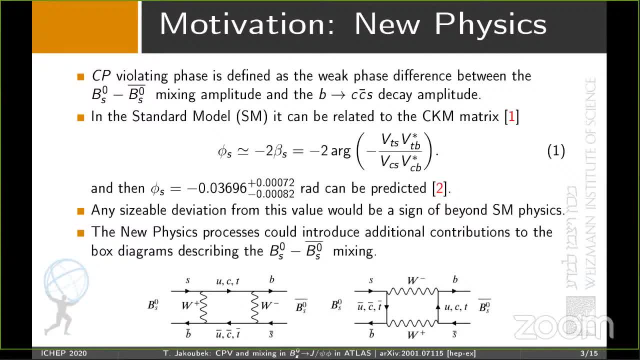 in the standard model, this phase can be related to the Kavibo-Kobayashi-Maskawa quark mixing matrix and thus can be predicted very precisely to the b minus 0.037. let's say so: any size of a deviation would be a clear sign of beyond. 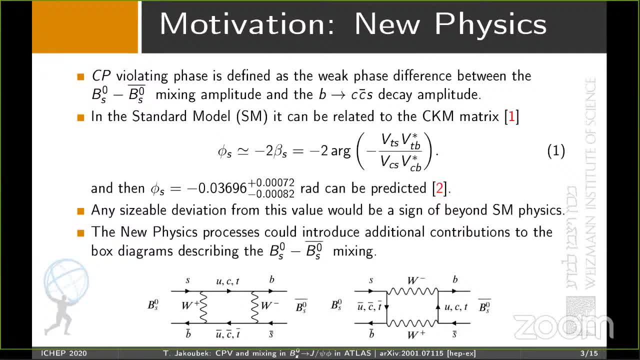 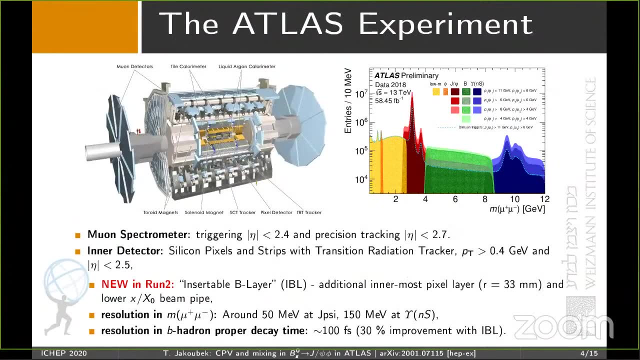 the standard mode of physics, because these processes could then introduce a contribution, or contributions to the box diagrams describing the bs mixing, so to our measurement in atlas. so it was done using the data collected by the atlas detector. of course, this is one of the multi-purpose parameters of the LHC. from all the important parts, let me mention the muon spectrum is used. 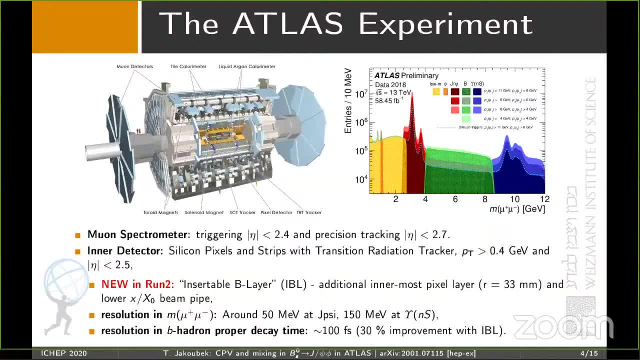 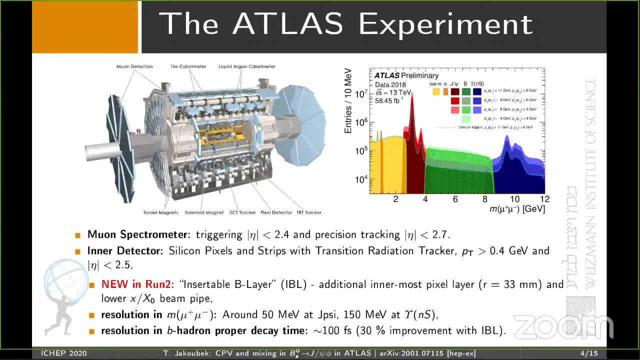 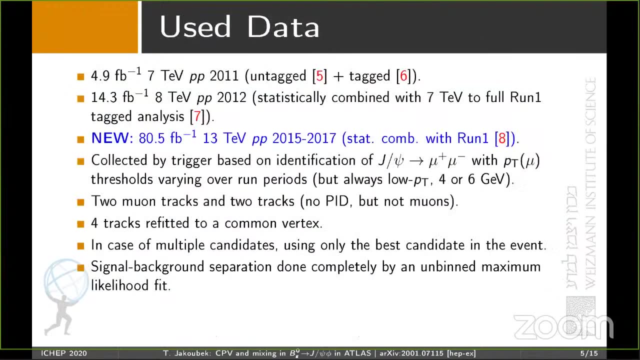 our typical diameter triggers with vario invariance, invariant mass windows are shown on the on the right plot. basically all our triggers are four or six GeV diameters. our analysis started many, many weeks ago. the first paper was based on five inverse phentabaron slice of. 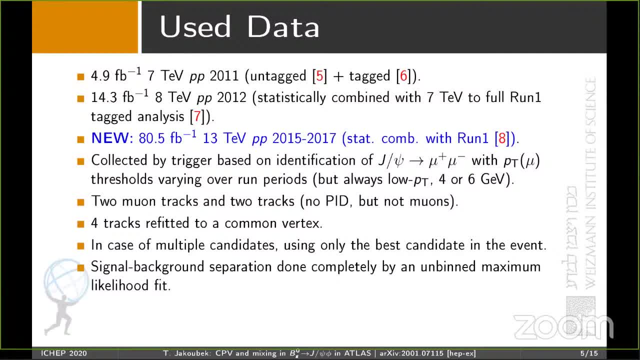 70 EV data. then we published the full round one analysis with additional 14 inverse Fentobarns of ATEV data, and today I'd like to show you the latest result and its update. It's our partial run-to analysis using ATEV inverse Fentobarns of 13 TEV data from years. 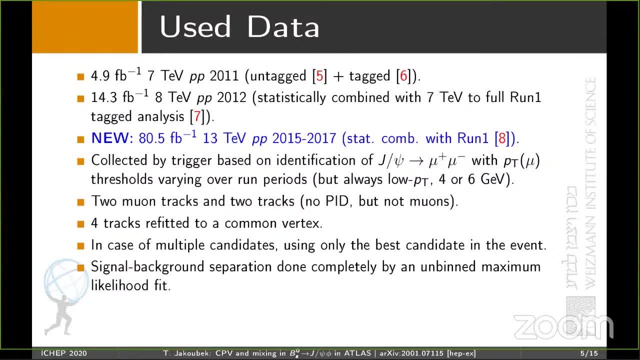 2015,, 2016 and 2017, so without the last year of data taking In our analysis we require at least four tracks, in the event two muons and two other tracks. so we do not have any particle identification atlas, but because of the muon spectrometer we 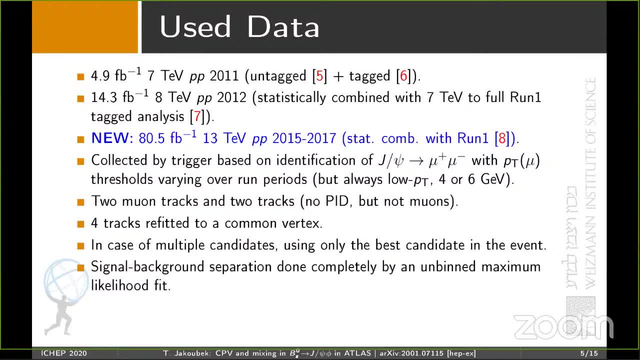 can of course exclude muon tracks from the set. Then we refit the vertex, or we refit these four tracks to the common vertex under the K-on-K-on hypothesis for the remaining tracks, And by refitting these four tracks we can then obtain the secondary vertex. 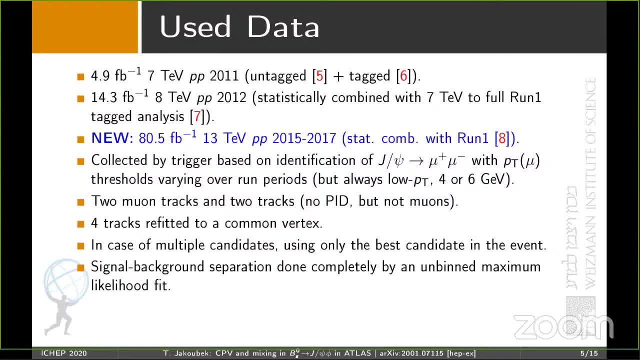 and the decay length or the lifetime of the B particle. If it happens that there are multiple BS candidates in the event, then we take the one with the best vertex fit. All signal background separation is then done completely by an unbind: maximum likelihood fit. 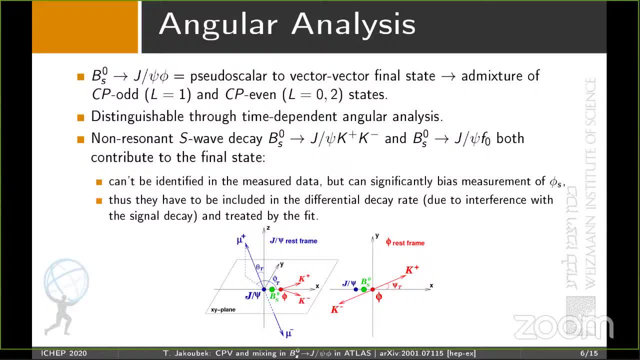 So BS is a decay length of the B particle. B is a decay length of the B particle. B is a decay length of the B particle. B is a decay length of the B particle. THERE IS- 맛이 Binaresing GRU. 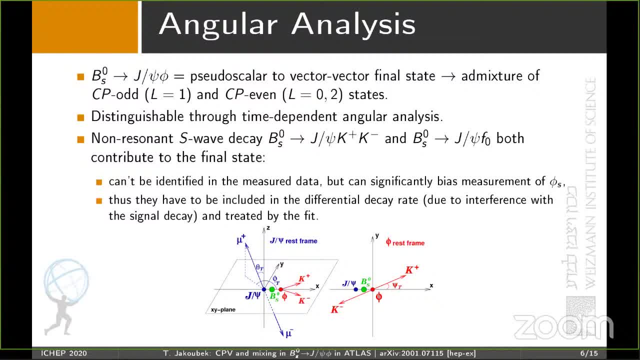 and you can follow the 442-V 🔡, this state of decay, and you will understand the situation much better. Again, we SaltWinds also show you that the state of decay of pseudo-scalar to vector-vector final state, which is thus the world's 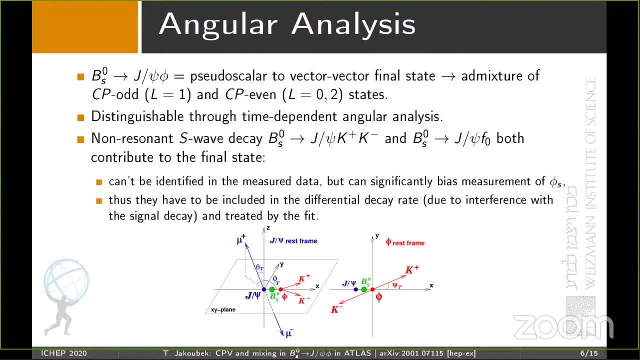 own motion. matriculation pattern of RST SC to vector-vector final state, which is thus a mixture of C0M and C0M events states. we can distinguish this state through time dependent angular analysis, and our data are still polluted by Non-Resonant S wave decay B, K and K. 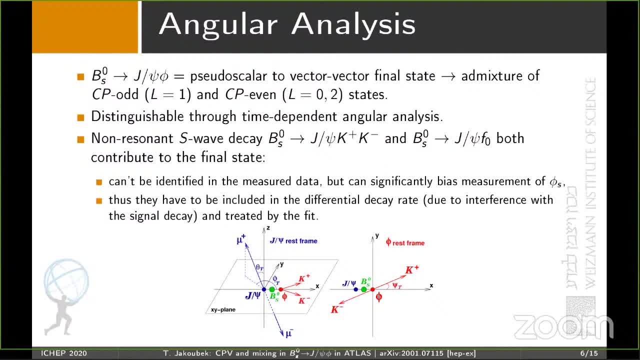 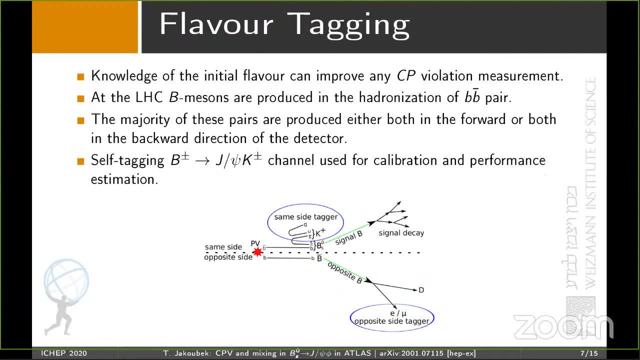 the data and thus can significantly bias the measurement of the weak phase. they also interfere with the signal decay, so we have to include them in the differential decay rate, and everything is then treated by by the fit. so few words about the flavor tagging, which is of course very important. 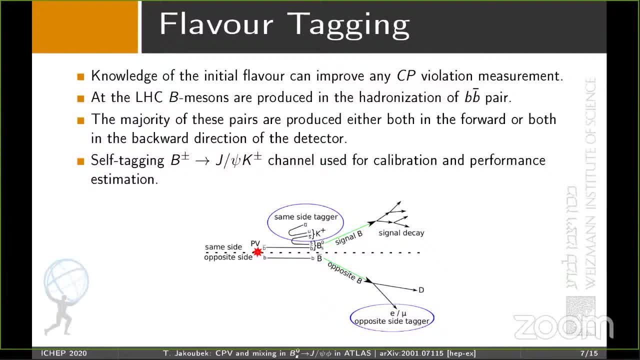 in every cp violation measurement we use so-called opposite size tagging, where we try to deduce the, the flavor of the signal b meson from the flavor of the other b meson produced in the. in the event, for a calibration and performance estimation we use a self-tagging channel b plus minus to j psi. 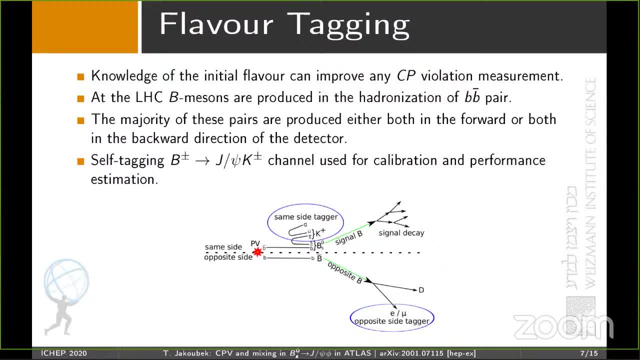 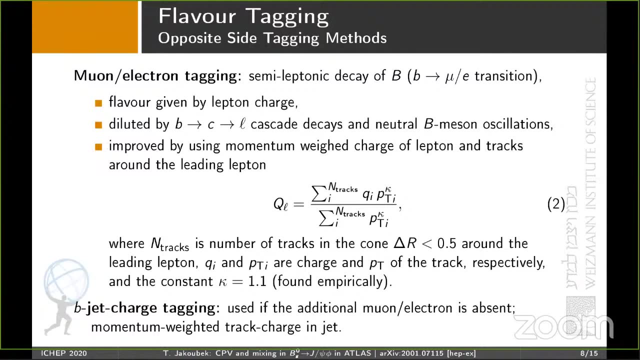 k plus or minus, where the flavor of the v meson can is given by the, by the current charge. so to identify- sorry, yeah, so to identify, uh, the flavor, uh, we use a lepton, uh, lepton tagging where it's. this is based on the semilatonic decay of b meson, where the flavor is given by the lepton charge. but 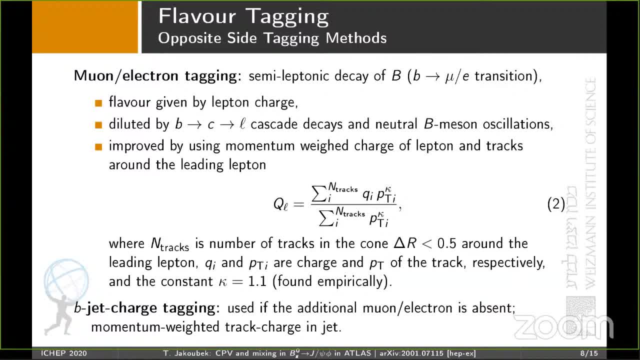 of course it's diluted by the b to c quad transition as well as as the oscillation itself. this this fact can be improved by the moment weight charge of the lepton and tracks in the cone around the leading lepton uh if there is no additional muon or electron uh. in the event we try to use a b jet charge tagging. we calculate the. 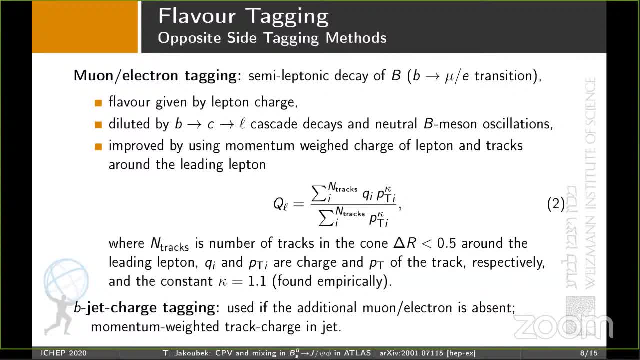 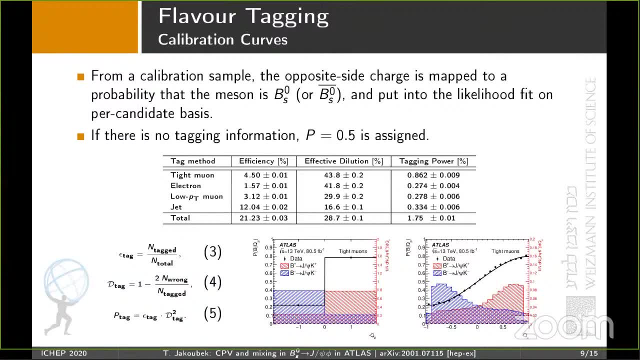 moment-weighted track track charge in the in the jet um from the calibration calibration b plus to minus sample uh. we can map uh these charges to the probability that the given candidate is bs or anti-ds and these these. this probability is then used in the fit on the per candidate uh basis if. 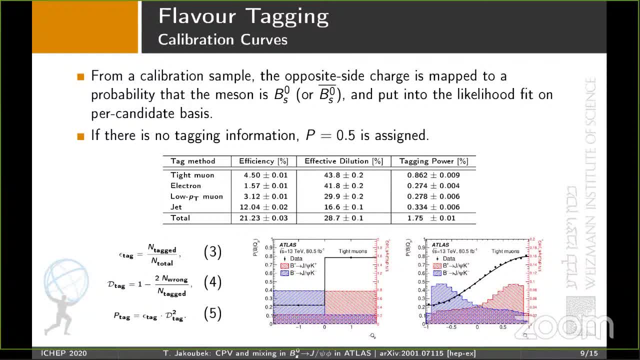 there is no tagging information. uh, we assign a probability 0.5. uh, in this way we can take, we can. we can take about 15 of all bs candidates. uh, yeah, so you can see the comparison of our tagging and also the mapping. uh, from the charge, the probability on the bottom plots, uh, as an example, 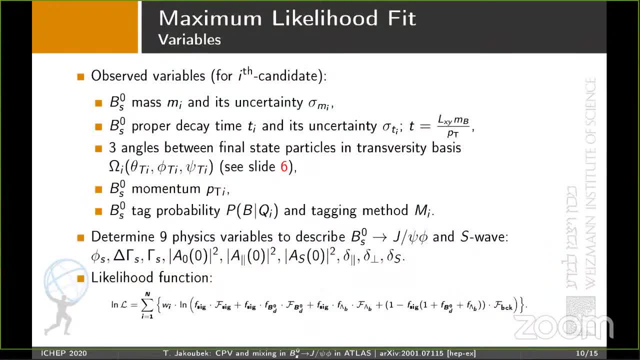 um. so to obtain the physics parameter population in the decay we use the maximum likelihood fit uh, which takes all possible information about the event. so the mass and its uncertainty property, decay time uh, angles between final state particles, bs, momentum and the tag probability and the fit and. 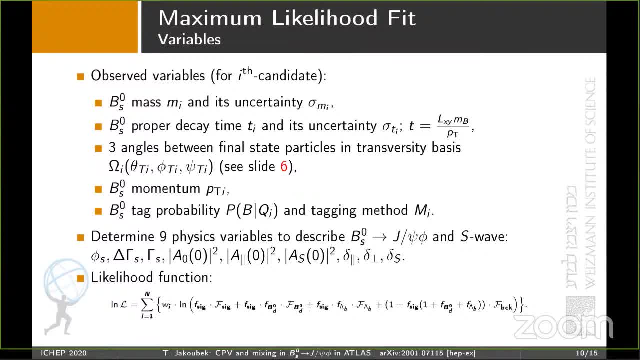 this is the Unity function of theveCity function, which defines nine variables: uh the weak phase, uh decay, width of heavy and plus uh light mass eigenstates and three amplitudes and relevant strong phases. so the likelihood function consists of four main parts: the signal part, 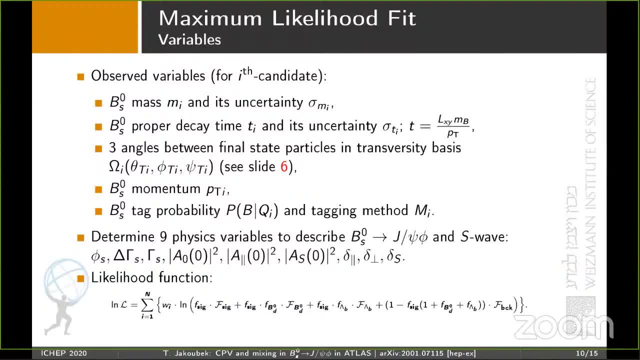 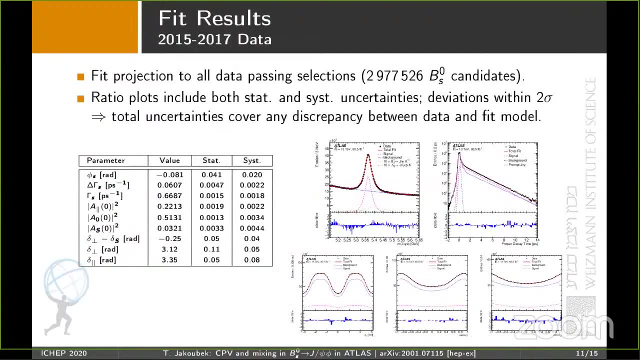 two specific backgrounds from misreconstructed BD and lambda BD, decays of the BD case and uh combinatorial background, um, and then all these probability density functions are weighted for a proper decay time. uh, efficient mixing is important. Here you can see the fit results of our partial run-to data analysis. 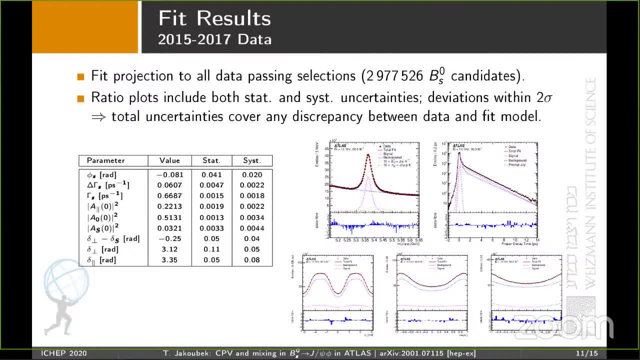 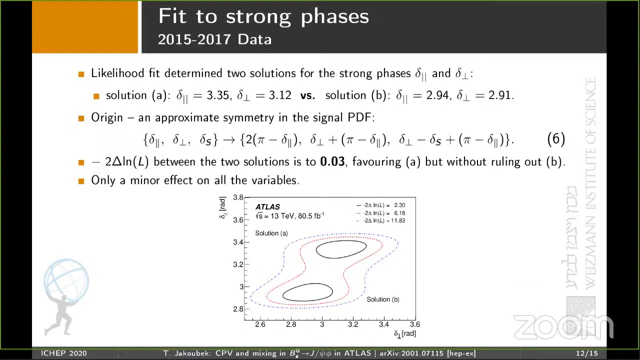 This is a fit projection to all data passing the selection. The ratio plots below each figure include both statistical and systematic uncertainties And you can see that these plots cover all the differences between the data and the model. During the analysis of the full run-to data set, we observed that there is a secondary minimum with respect to the two variables. 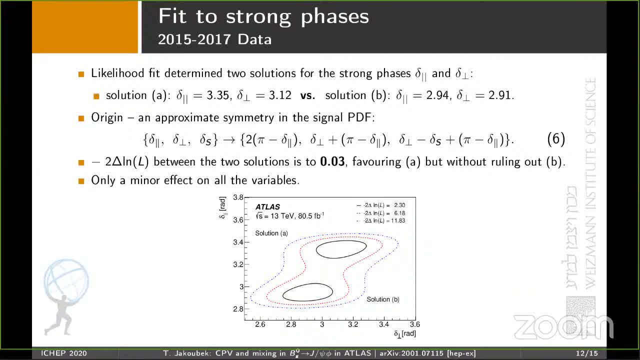 It's a delta parallel and delta perpendicular. We have both solutions here. The origin is anonymous And the approximate symmetry in the signal properties of this function, And we measured the two solutions as a difference of 0.03, favoring A but without ruling out B. 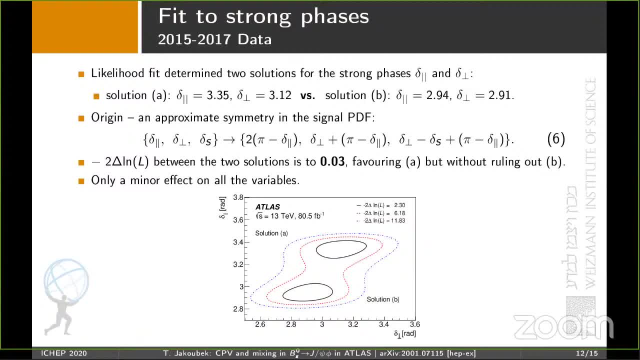 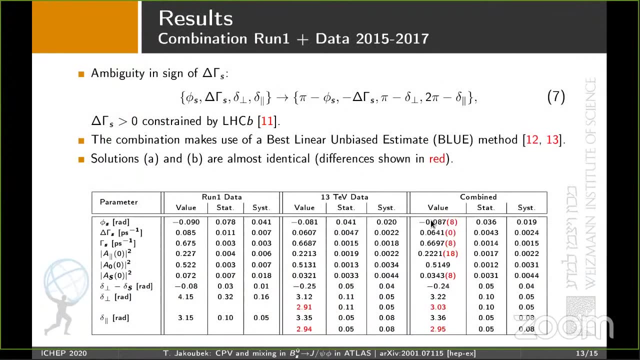 So we are including both solutions for analysis And you can see the likelihood contours of all the 1,, 2, and 3, let's say sigma- intervals On the plot on the bottom. Then there are results of our combined analysis of run 1 plus partial run-to data set. 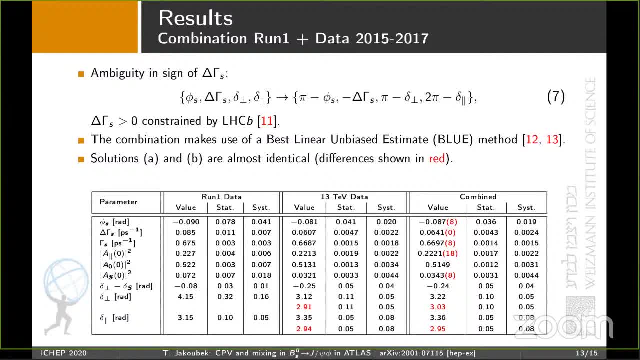 The ambiguity of the delta gamma sign is constrained by the measurement of LHCb experiment. For the combination we make use of the best linear amperes estimate method And you can see that both solutions or the differences between the two solutions. 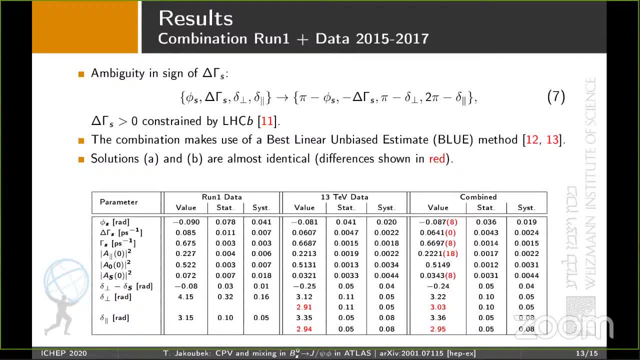 are negligible, even in the combination. So in the table below in the three right columns the red curves show the different number for each value. So for example the phi s for the combination of solution A is minus 0.087.. And with solution B it's minus 0.088.. 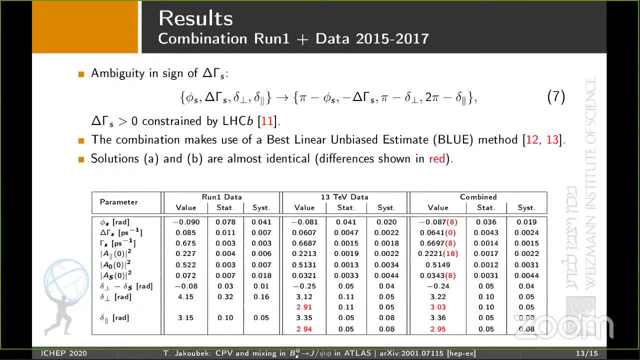 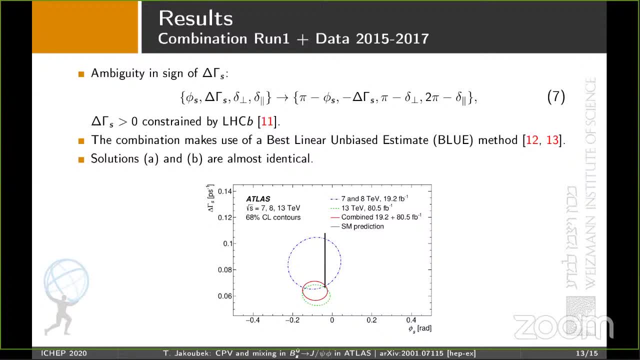 So all the differences are negligible. The combination is better shown on the plot on the next slide, where you can see the 7 and 8 TeV result in blue, Then in green the 13 TeV result And then in red the combined measurement or combined result of run 1 plus partial run-to analysis. 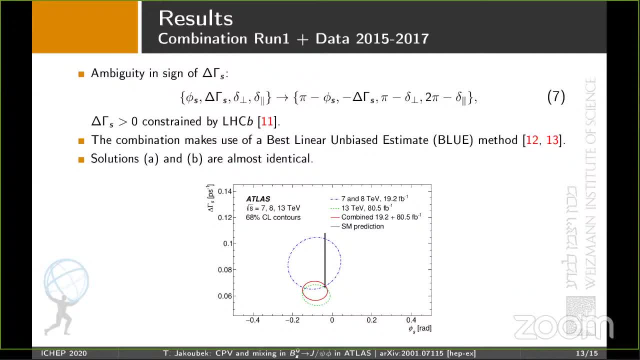 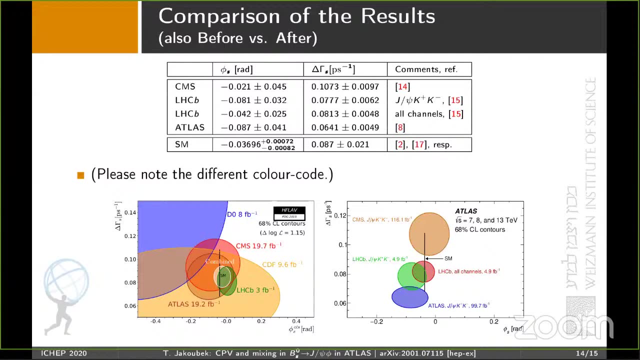 These are one sigma confidence level contours for the most important parameters: the weak phase, phi s, and the difference of the decay length, delta gamma s. So there is a small comparison before and after and also between the experiments. I'm very sorry for the different color code of the plots. 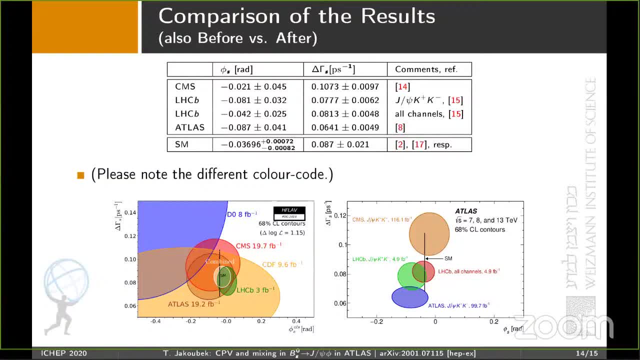 The left plot is made by HFlap group before the latest LHC results from all the experiments. The right plot is the comparison of newest results from, I believe, all three experiments from the LHC. You can see we are still compatible with the standard model prediction and with the LHC-B-Gypsi-2-k-plus-k-minus channel. 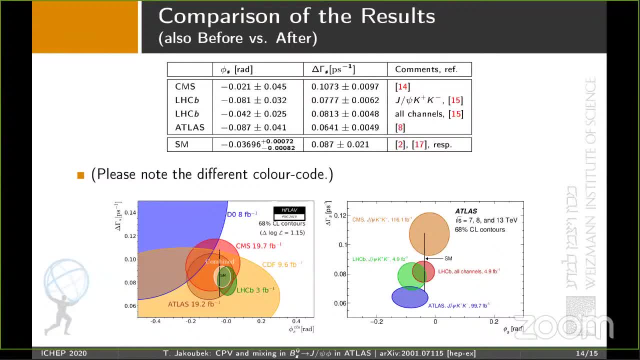 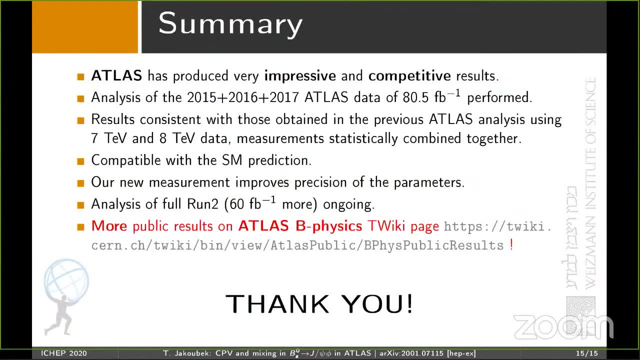 We are slightly away from the combined LHC measurement and also from CMS. So to summarize that we are not the B-physics experiment, but we can still produce very impressive and competitive results. I've just shown you the latest update of the partial run-to analysis of the data from 15,, 16 and 17,. 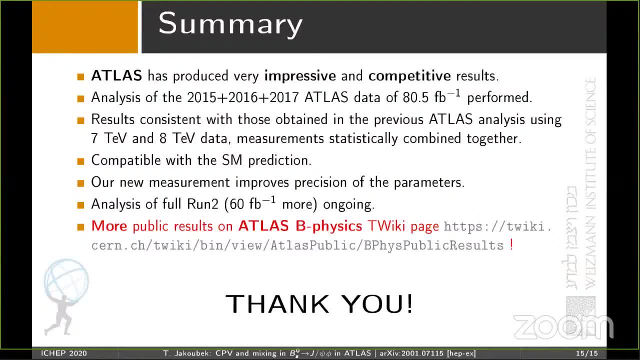 which is together 80 inverse femtobarns, And the results are consistent with those obtained in the previous ATLAS analysis using 7 and 8 TeV data, So we can combine them together. All our results are consistent or compatible with the standard model prediction. 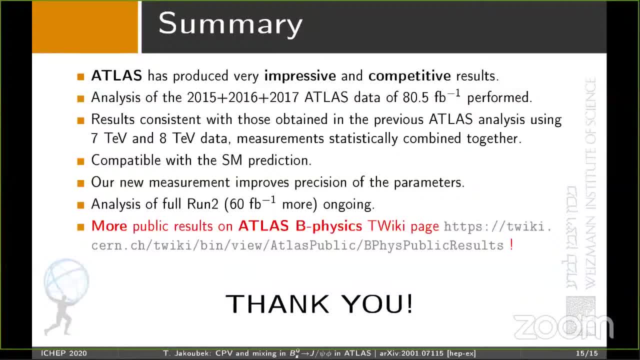 The analysis of the full run-to data- so another 60 inverse femtobarns- is currently ongoing, And please visit the TDK page for our B-physics public results. Thank you very much. Thank you, Tomas, Really impressive. 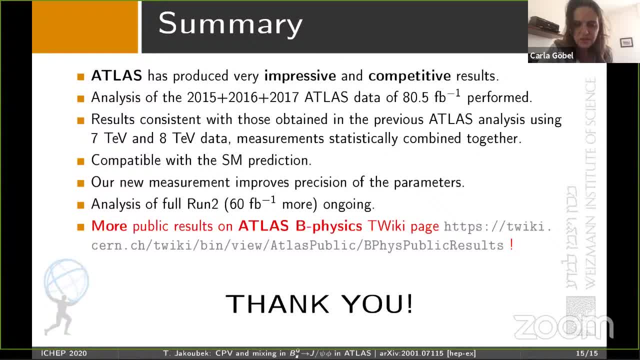 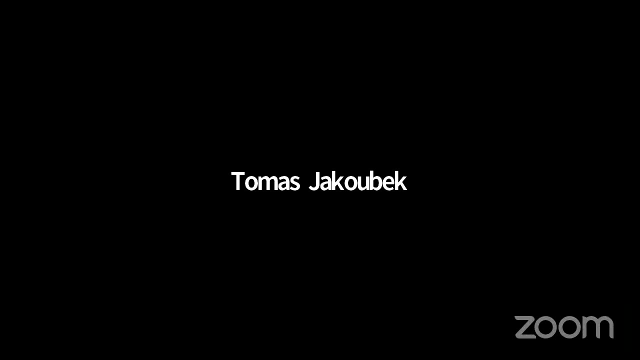 Do you have any questions? Any questions from the audience? Otherwise we move to the FIAS measurements from CMS. now, Okay, thank you very much. Let me stop the share. Could people see the hand-drawing of the time? The text wasn't working when I wrote in the slide. 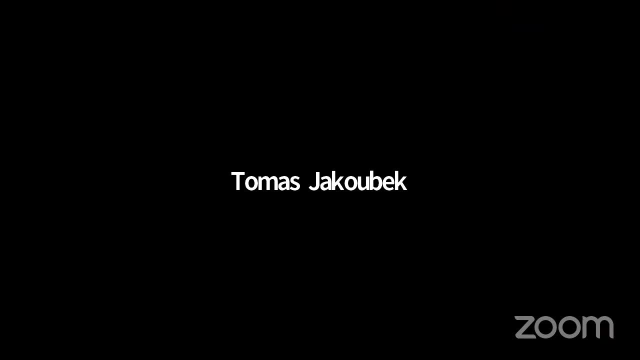 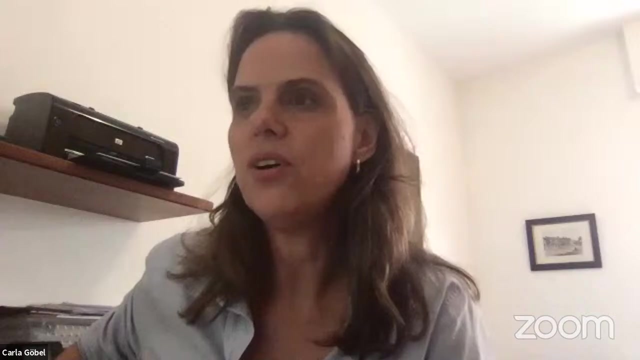 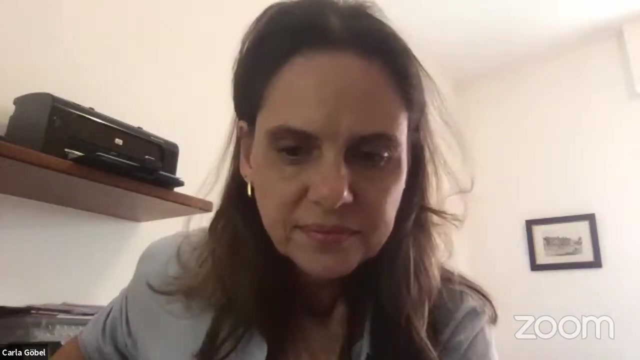 Sorry, Could you see the time that I wrote? Yes, Okay, Yes, it was very nice. I see the first five minutes and then the handwriting. Okay, Yeah, So we can move on then with Enrico. Yes, Let me share the screen. 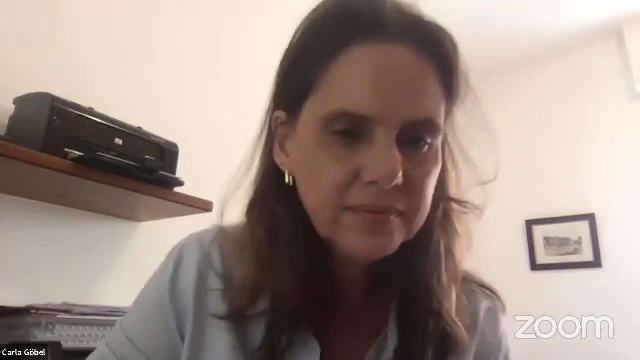 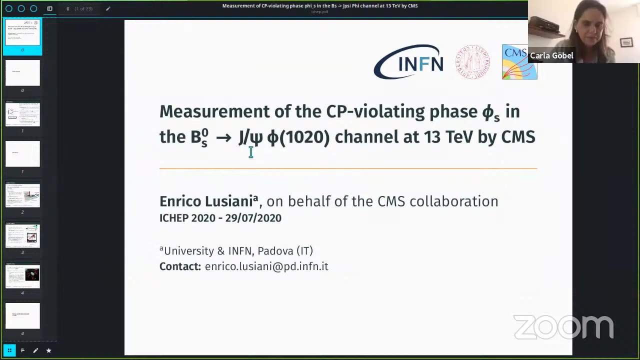 Can you see the slides? Yes, So hello. My name is Enrico Lusiani And I'll be presenting the measurements. I'll be presenting the measurement of the CP violating phase FIAS In the BS to JPSI-5 channel at 13 TD by CMS. 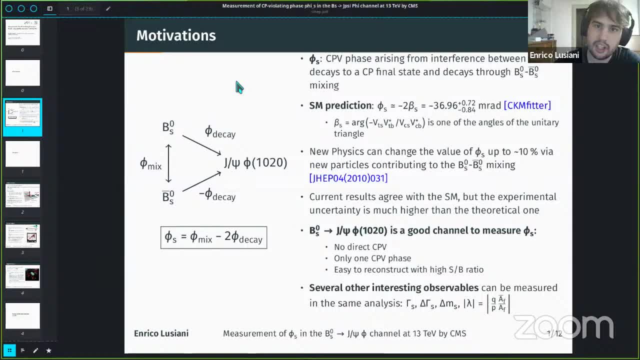 So let's start with a brief introduction. FIAS is the CP violating phase arising from the interference between direct decays to a CP finite state And decays through the BS anti-BS mixing. The standard model predicts this to be close to minus two beta-S, where beta-S is one of the angles in the unitary triangle. 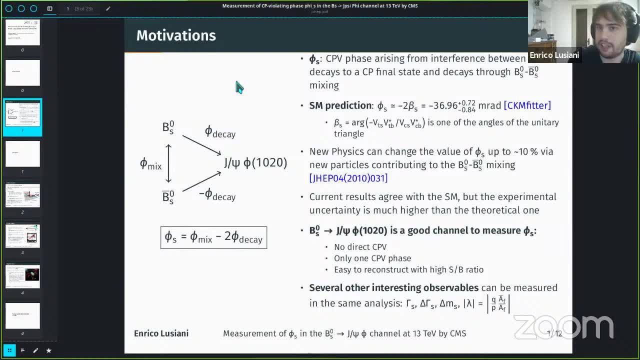 And equal to about minus 37 milliard, with the uncertainty below the milliard. However, new physics can change the value of FIAS up to 10% via new particles contributing to the BS anti-BS mixing. Currently, the results agree with the standard model. 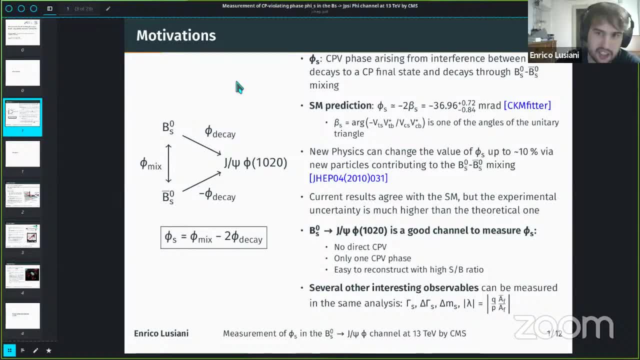 But the experimental uncertainty is much higher than the theoretical one. The decay of FIAS into JPSI-5 is a good channel to measure FIAS Because there's no direct CP violating predicted, Only one CP violating phase, And it's easy to reconstruct using the two muons and two K. 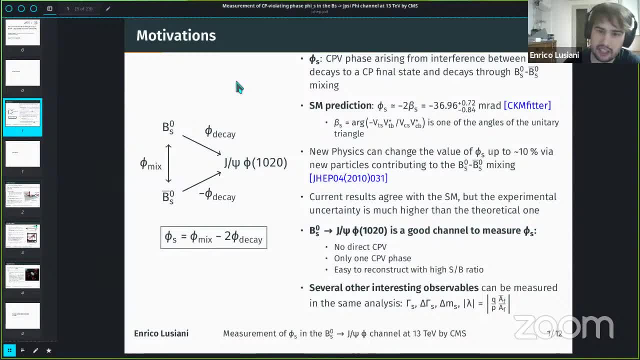 Also, in the same analysis, we can extract several other interesting observables, Such as the decay width, The decay width between the two eigenstates, The difference in mass And the module of lambda, which is a parameter quantifying the CP violation. 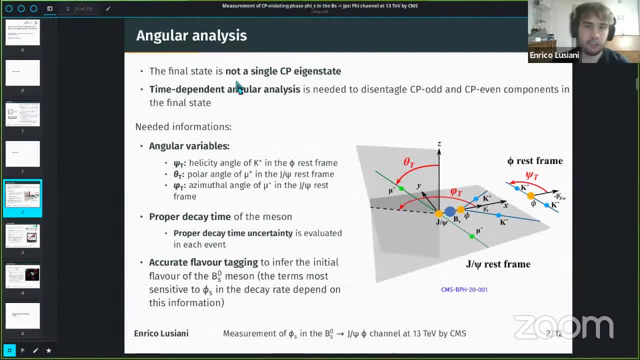 Let's now go to an overview of the analysis. The main issue in the analysis is that the final state is not a single CP eigenstate, So we need a time-dependent angular analysis to disentangle CP of the CP-event components. For this we need a parametrization of the angles in the decay. 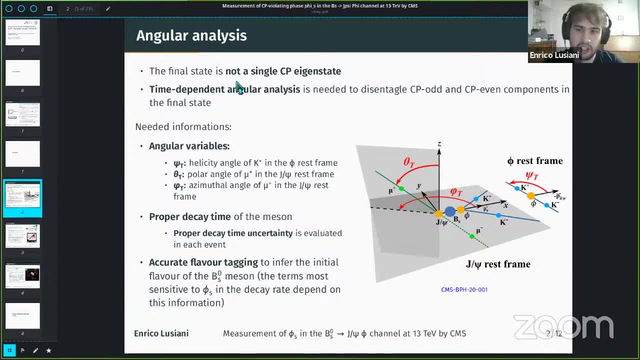 On the right we can see the one used by CMS, Which uses CP, which is the LCT angle of the K-ons in the FIAS frame, And theta and phi, which are the spherical coordinates of the muons in the JPSI-res frame. 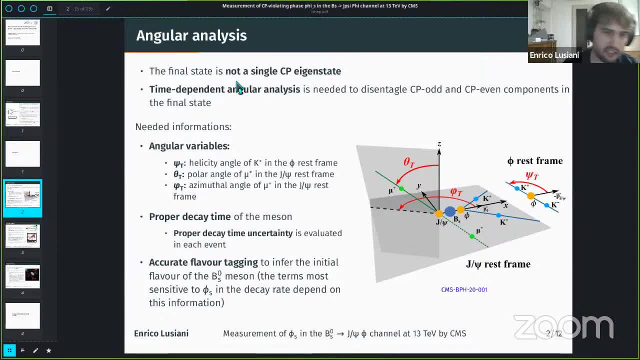 We also need the proper decay time of the meson And its uncertainty, which is evaluated in each event. Finally, we need an accurate flavor tagging to infer the initial flavor of the BS meson As the terms most sensitive to FIAS in the decay rate depends on this. 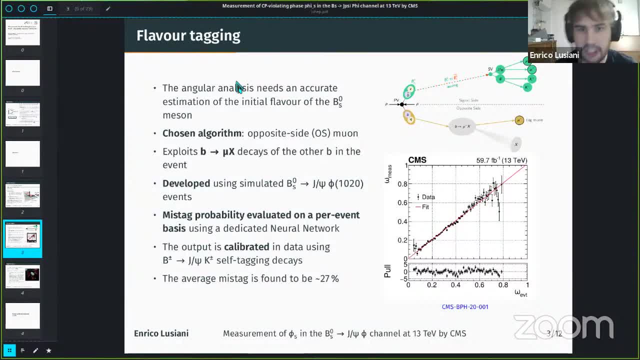 So for the tagging we use an algorithm based on the opposite side, muon, Which uses the semi-leptonic decays of the second B. in the event, For the analysis it's important to not only have an accurate estimate Of the flavor of the meson. 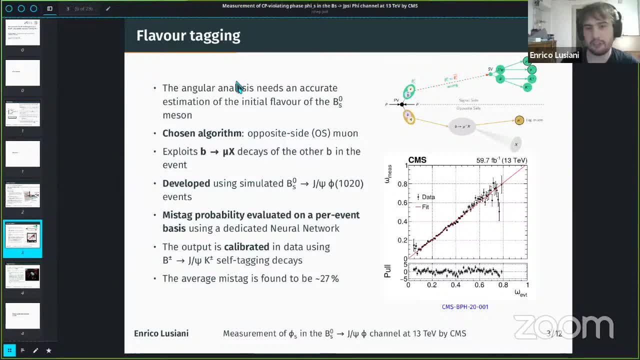 But also a measurement of the accuracy for the flavor. For this we trained our neural networks So that the output is directly the missed probability on each event, And we calibrated this output on data using B plus to JPSI, K plus In the case, as we can see in the slide. 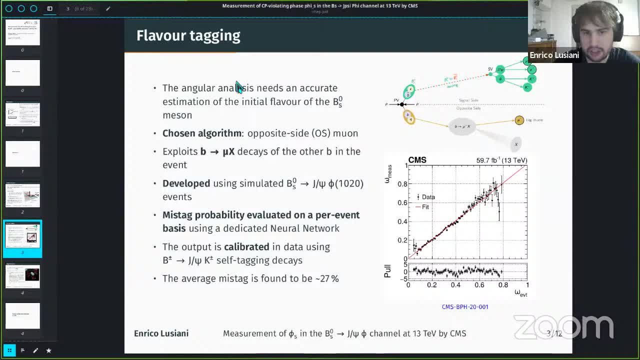 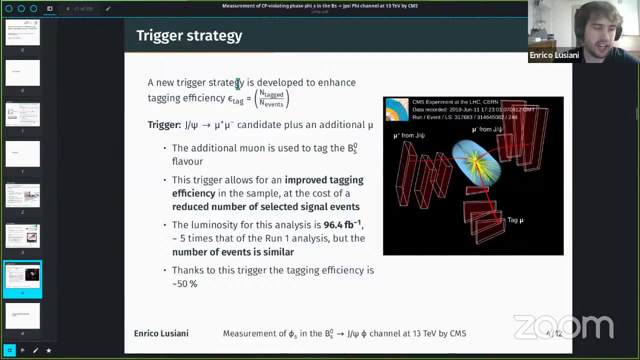 The plot. on the right Post calibration, the average mistag is found to be close to 27%. Since we need a muon for the tagging, We developed a new trigger strategy To enhance the tagging efficiency, Which is the number of tagged events. 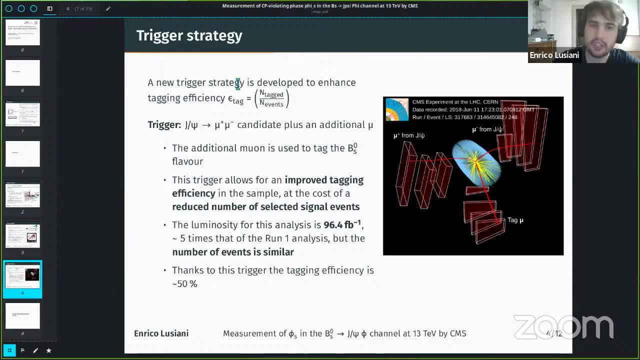 Over the total number of selected events. Our trigger requires a JPSI decaying to two muons Plus an additional muon Which is used for the tag. This trigger allows us to improve the tagging efficiency, But at the cost of a reduced number of selected single events. 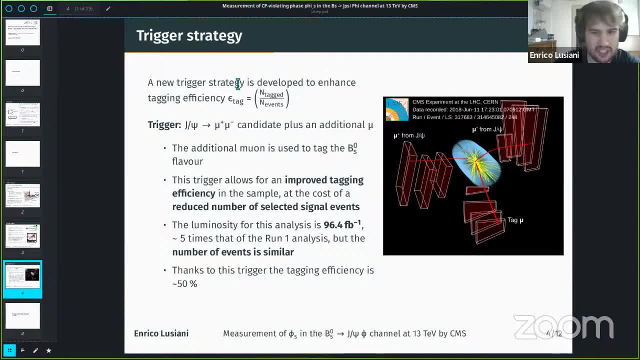 For example, the luminosity of this analysis is about five times The one used in a previous run. one analysis, But the number of events is similar. We will see that this has important consequences In the precision of the measurement, Thanks to this new trigger strategy. 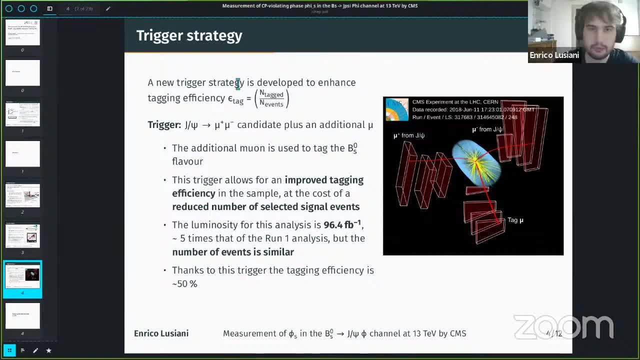 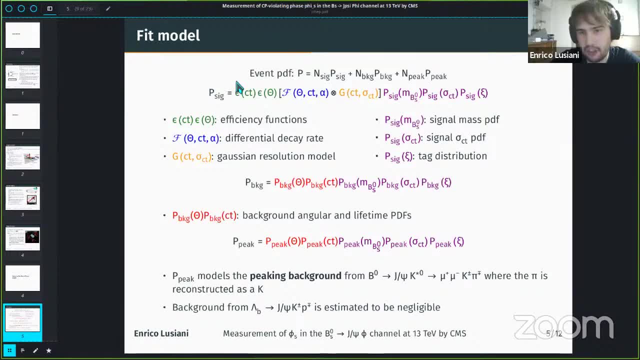 The tagging efficiency is close to 50%. Let's now look a bit at the model. Without going into details, There are three main terms. The first is the signal, Which contains the decay rate, Of course, The efficiencies And the PDF of our nuisance parameters. 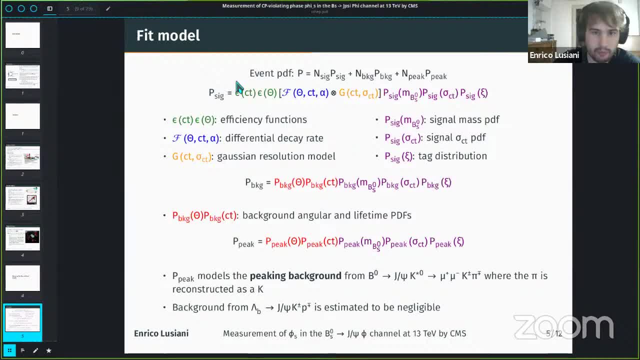 Then we have the combinatorial background And then the picking background Which comes from the case of B0 into JPSI K-star, Where the pion was reconstructed as a K-on. Another possible source of background Will be the lambda B to JPSI K-on proton. 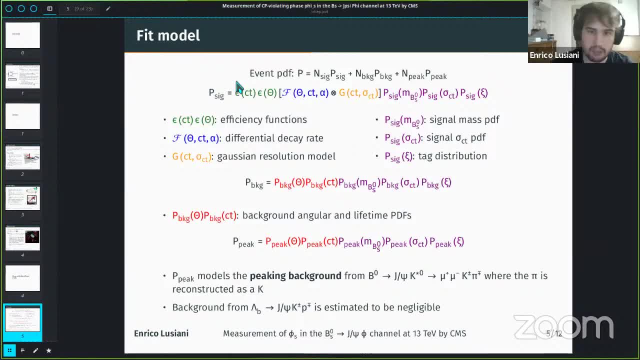 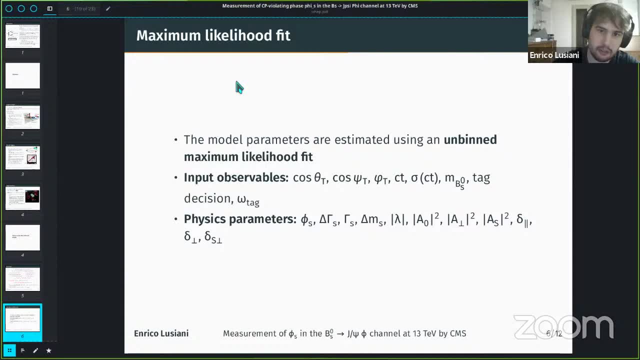 But we estimated this to be negligible in our sample. The model is fitted to the data Using the maximum likelihood fit With inputs, The three angles, The proper decay time. Its uncertainty, The mass, The tag decision from the tagger. 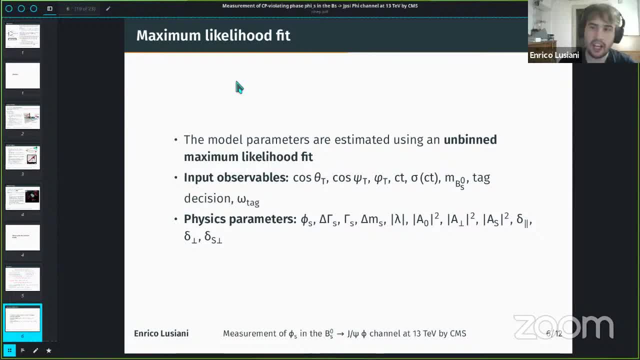 And the mistag probability. And from the fit We can extract the physics parameter, The decay width, The different decay width, The difference in mass lambda, Three amplitude for the difference, final state And three strong phases. Here we can see the one-dimensional projection of our fit model. 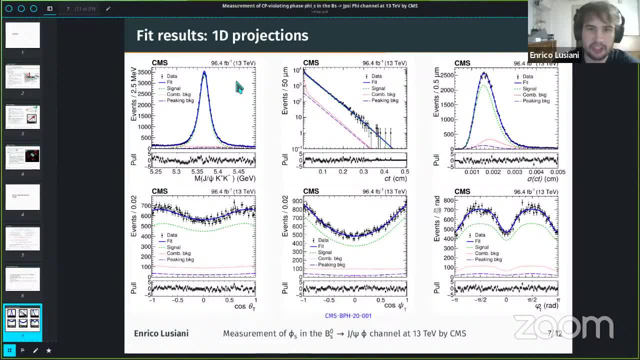 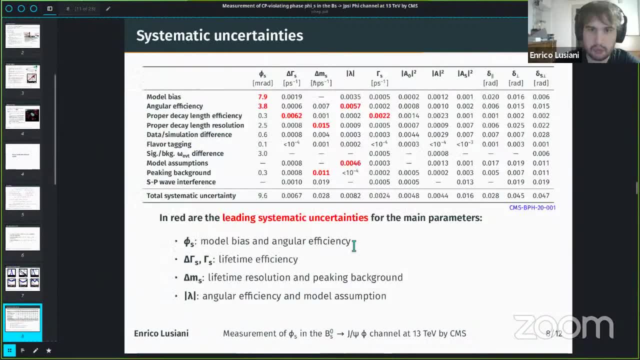 We can see the mass, The proper decay time. Its uncertainty And the angles. Here we show the systematic uncertainties for all the parameters In the fit And in red We evidence the leading systematic uncertainties for the fit For Fies. these, for example, are the intrinsic bias of the model. 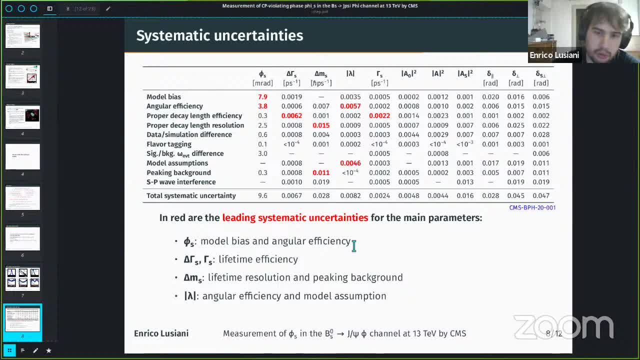 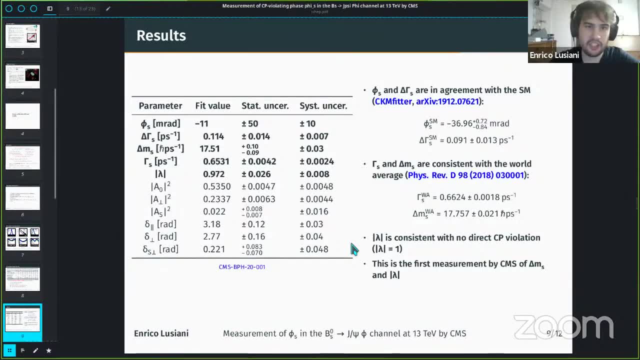 And the systematic uncertainty associated to the limited statistic we used to compute the angular efficiency. Here we can see the results of the fit For Fies. We found it to be equal to minus 11 millirad, With a statistical uncertainty of 50 millirad. 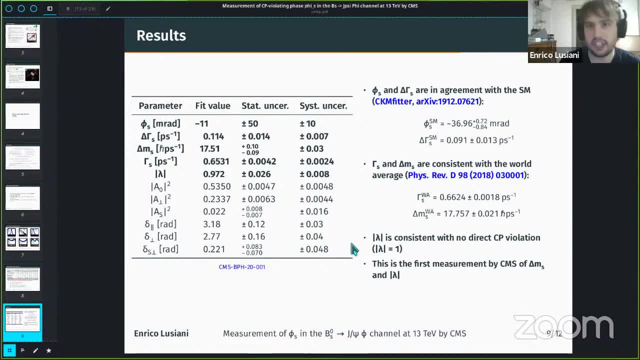 And a systematic uncertainty of 10. Which is in agreement with the standard model. We also measured the difference in decay width, Which again is in agreement with the standard model, The decay width and the difference in mass, Which are consistent with the world average. 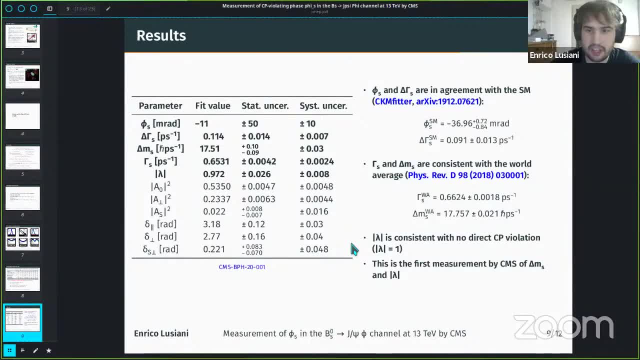 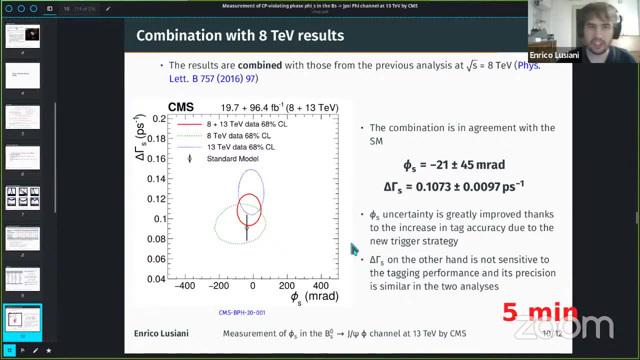 And the module of lambda, Which is consistent with having no direct CP violation, Which will force its value to 1.. The results are combined with those from the previous analysis And the result of the combination are shown in this slide. We can see from the plot that the uncertainty of Fies is greatly reduced. 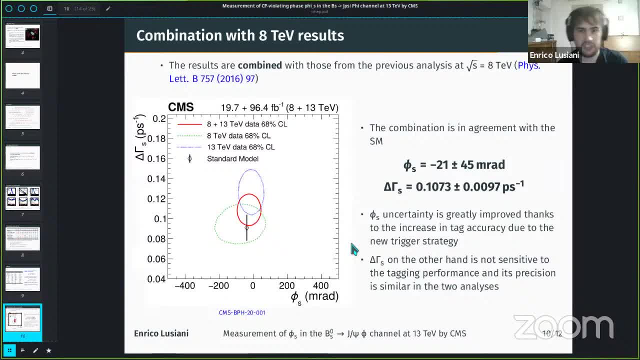 Thanks to the increase in the target accuracy, But delta gamma S did not improve Because it's only sensitive to the total statistics And not to the target accuracy. Another thing to note in this plot Is that the standard model prediction for delta gamma S 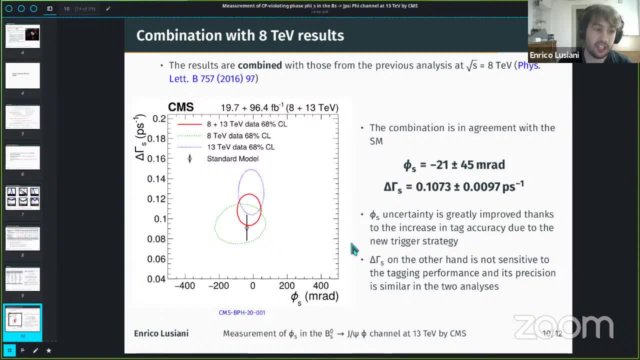 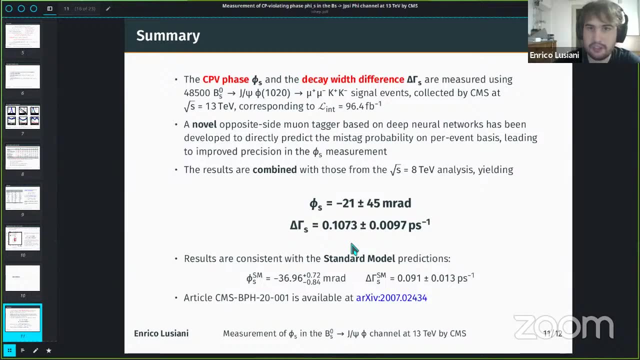 Shown in the plot Is a fairly recent result Which greatly improved the uncertainty. In conclusion, We measured the CP violating phase Fies And the decay width difference, delta gamma S, Using roughly 50,000 single events Collected by CMS at 13 TV. 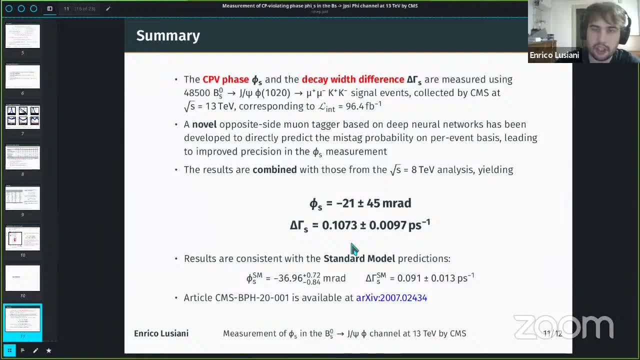 Using an integrated luminosity Of about 96 inverse. We developed a novel opposite side target Based on deep neural network Which can predict the missed probability on each event, Which led to an improved precision in the Fies measurement. We combined the result. 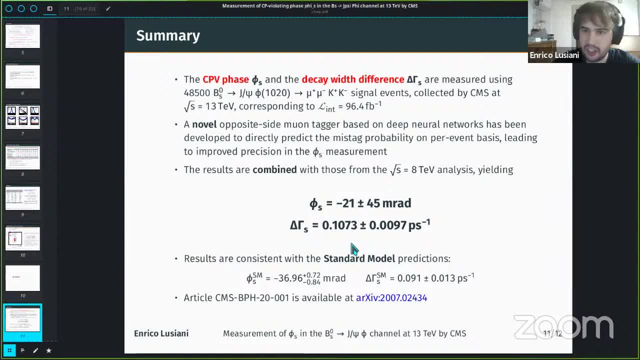 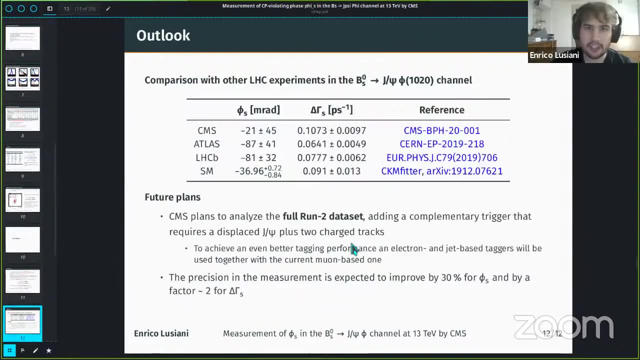 With those from a previous analysis Yielding the result shown here, And both are consistent with the standard model prediction. The full article is available at the link shown here. Here is a small comparison with other LAC experiments. In the future we plan to analyze the full RAN2 dataset. 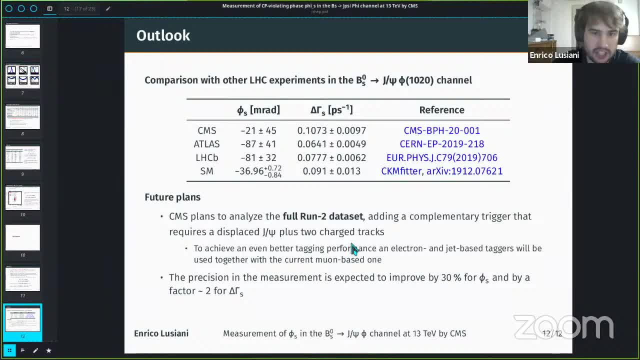 Adding a complementary trigger That requires a JPSI plus two charged tracks, And to improve even further the tagging performance, We will deploy an electron and jet based taggers Together with the current beyond base one. After this new trigger, We expect the precision of the measurement of Fies. 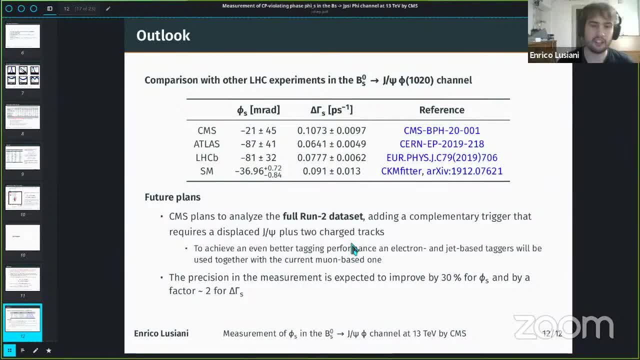 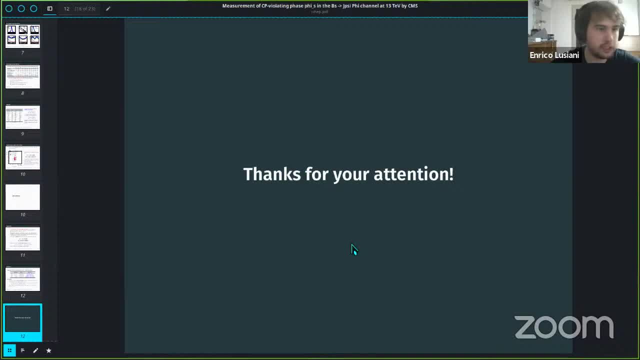 To improve by about 30%, And of Delta Gamma S about a factor of two. Thanks for your attention. Thank you, Enrico. Questions from the audience. Yes, Nils, Go ahead. Hi hello, I'm Nils from LACB. 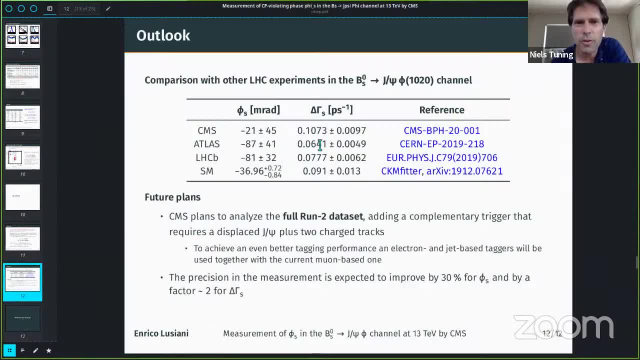 Thanks a lot for your interesting talk. I'm not sure if this is a question to you Or maybe to the previous speaker, But can you maybe comment on how you see the difference in the Delta Gamma S, The decay width difference Between ATLAS and CMS? 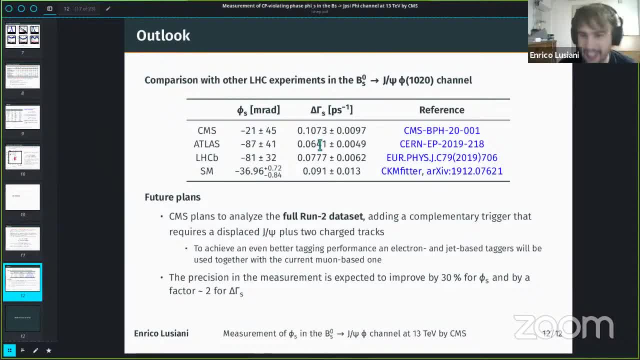 Yes, we have noticed it, But we have no comment on it. We hope that the continuation of this analysis With the full RAN2 dataset Will shed some light on the difference. Okay, Thank you very much. Any other questions? 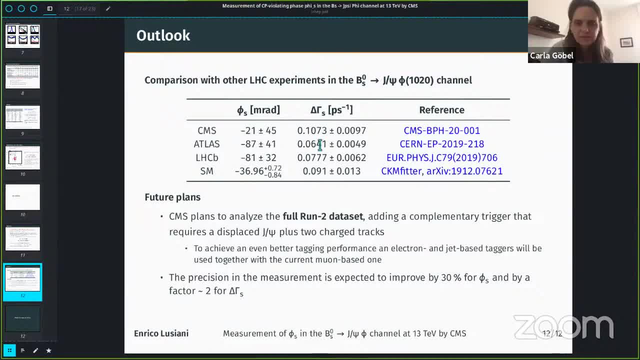 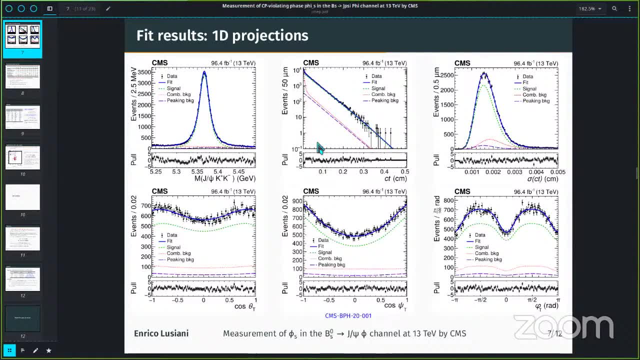 Sorry, just jumping. I have a question on the FIT projections That you have on page seven. Do you have a comment on how good they are? There seems to be some shifting around In, for example. Sorry, could you repeat This FIT projection? 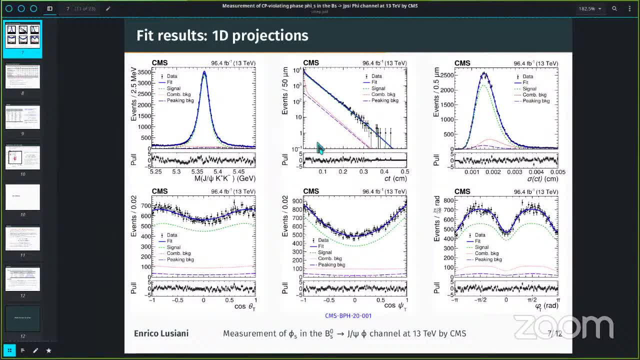 I know they don't tell the whole story, But there seems some shifting, For example in the FIT, In cos, theta, t, Where there is like a linear trend, For example, Or the low mass, The part of the JSI. 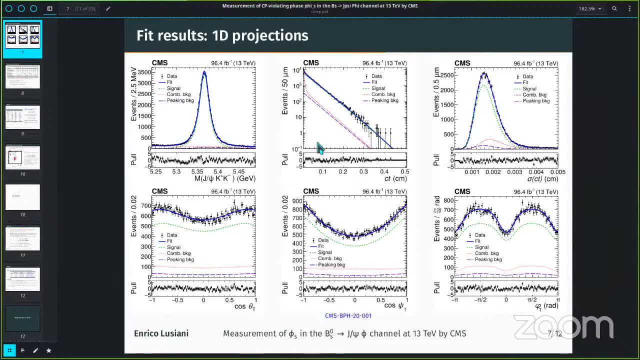 Yes, Of course, as you said, These are just projections, So we cannot infer too much For the mass. We tried We optimized the FIT In one dimension And it showed No issues there. We don't think We also tried the different mass models. 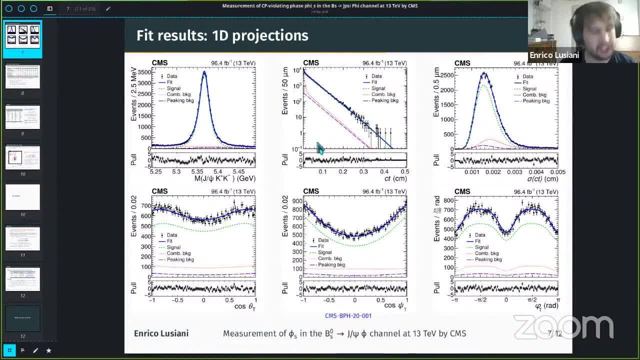 In the And use them as a systematic. We don't think it's an issue For us. They're not too good projection. Yes, Yes, We can do it, But we don't know What the T-shape is. 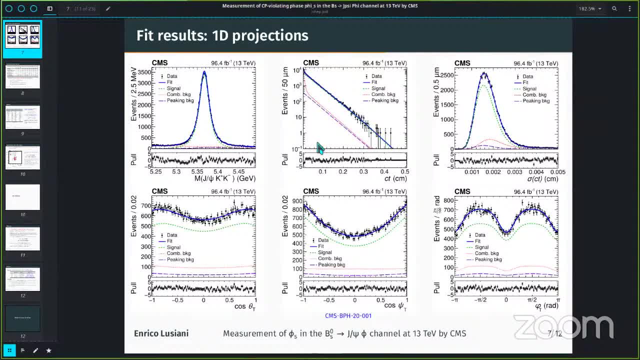 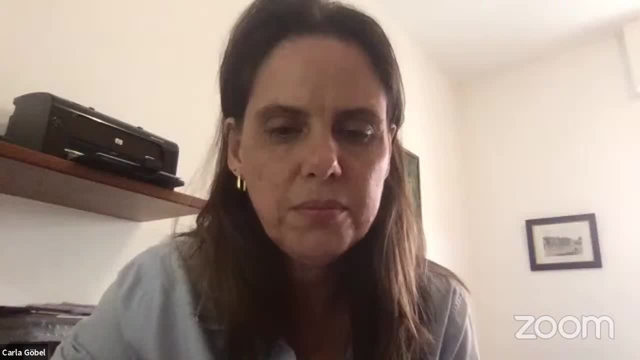 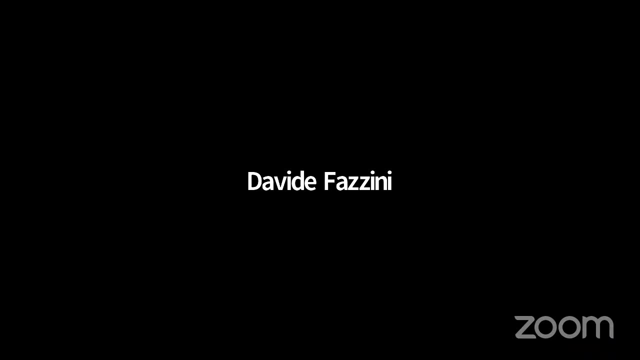 Yes, Yes, Yes, Yes, Yes, from Davide Fazzini. Yes, can you hear me? Yes, Let me shut the slide. So good evening and- I can't see yet your slides. Oh, okay, Now you can see. 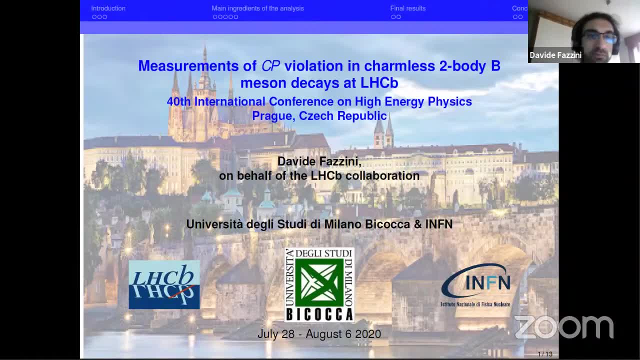 Yes, Perfect, Good evening. Today I will give you a talk on the latest results of the measurement of CP violation in charmless to body B meson decays at LCB. And so the motivation of this analysis is that the CPU of cerebral are sensitive. 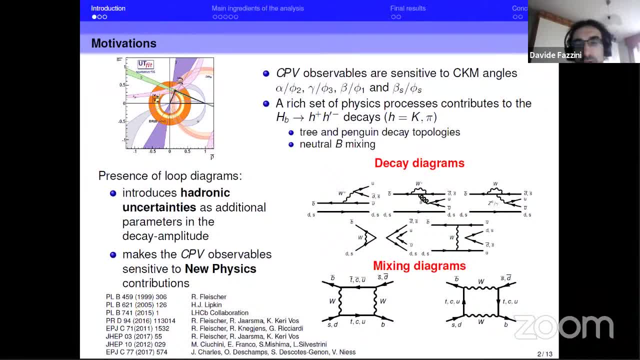 to the CKM angle, alpha, gamma, beta and beta S, And there are a rich set of physics processes that contribute to the generally called HB to HHD case. that is small H stand for K. on our time We have three and Pinguin decay topologies. 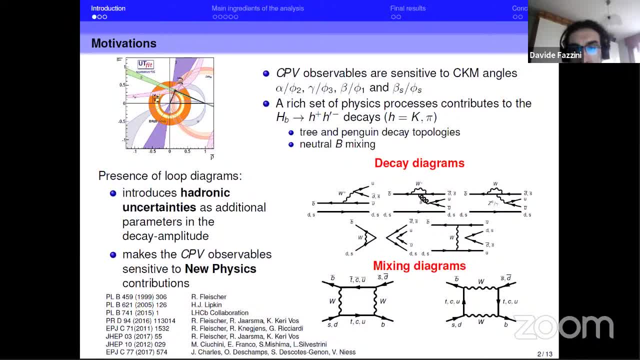 and also neutral B mixing, as you can see from the diagrams in the bottom of the slide. So the key point is that in many of these diagrams there are loops And the fact of this loop is introducing adrenic uncertainty as additional parameter on the decay amplitude. 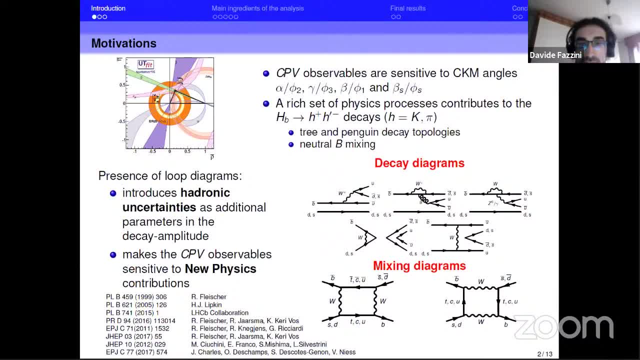 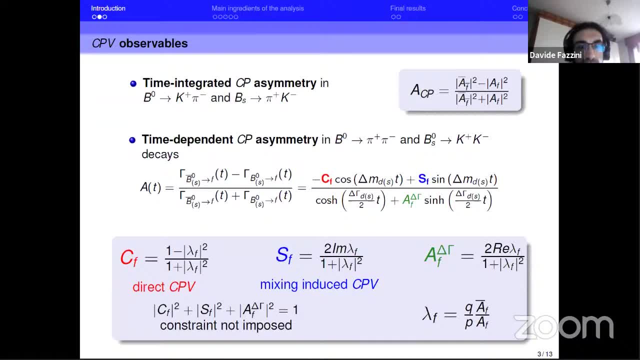 and also make the CP the several sensitive to the new physics contribution. So what we want to measure in these analysis are the time integrated CP asymmetry in B0 to K pi and Bs to pi, K decay which are determined as reported in there. 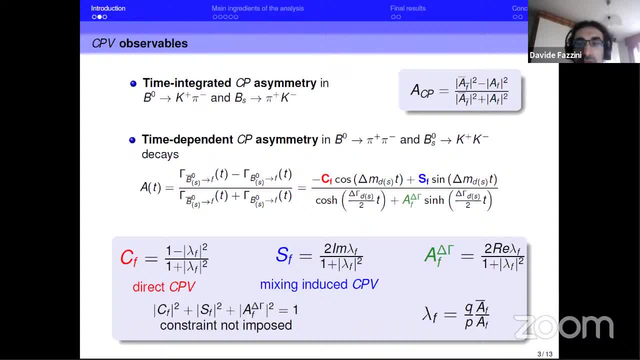 in the top of the slide. So the as the difference between the amplitude squared to the F bar and F state divided by the sum of the two terms. And also we want to measure the time-dependent CP asymmetry in B0 to pi, pi and Bs to KK. 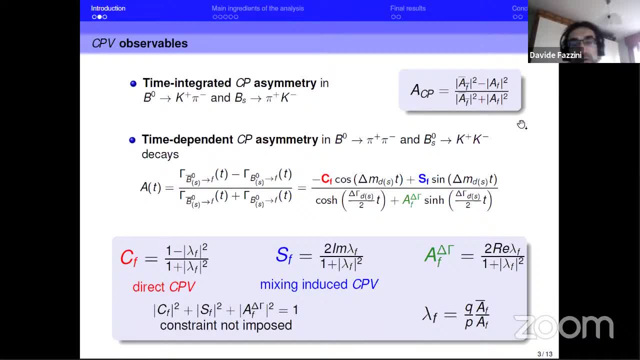 which are defined and reported in the middle of the slide, And in particular, we want to measure the three coefficient Sf, Sf, Sef Sf and Af delta gamma, which are related to the direct CP violation, mixing induced CP violation. 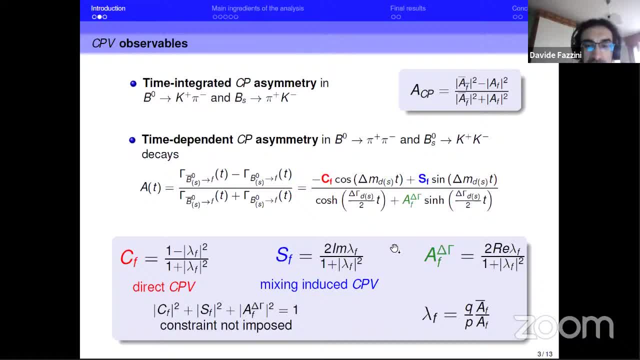 And they are symmetry related to the different in a lifetime between the two mass eigenstate. So these three coefficient satisfy a unitary constraint which is not imposed in the analysis but you use it up posteriorly as a cross-check to check the final results. 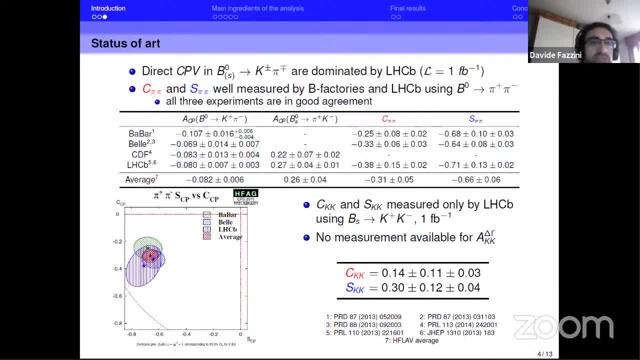 So at the moment, the measure of the direct CP violation, the B0 to K pi and Bs to pi K decay, are dominated by the LSCB measure and perform it at one inverse 10 to one, As you can see from the table. 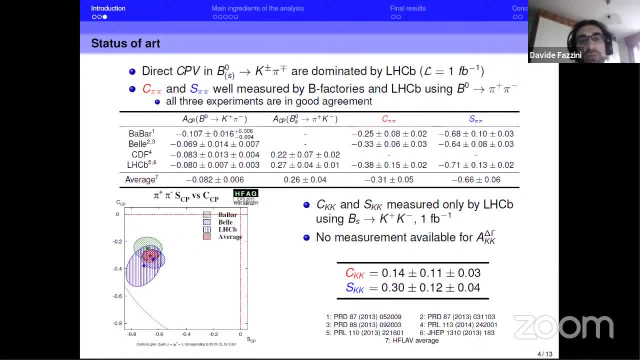 And while the measure on C pi pi and S pi pi are well measured by both the B factories and the LSCB, using the B0 to pi pi decays and the results between the three experiment are in very good agreement, as you can see both from the table. 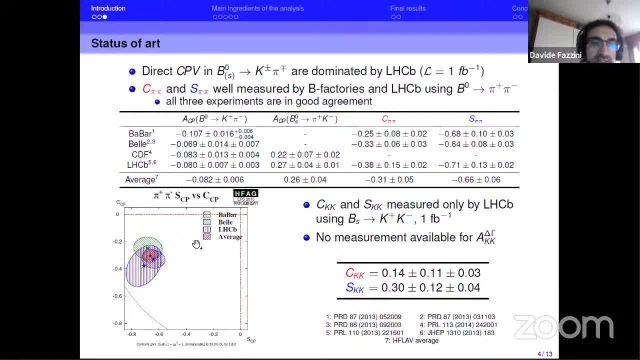 and also from the typical SCP versus CCP plot reported in the bottom of the slide, where there are shown the results of the three measurements, the three experiments and also the world average. So LSCB performed also a measurement of CKK and SKK using one inverse 10 to one on the Bs to KK sample. 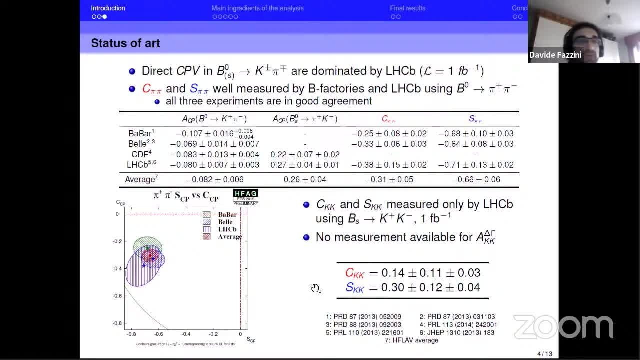 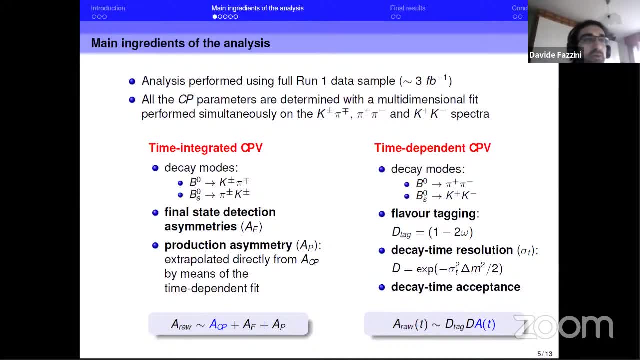 And the results are reported in the bottom of the slide. But for the moment we don't have a measurement for A delta kappa KK, So the analysis that I'm going to present today is performed using the fuller and one data sample corresponding to three inverse, 10 to one. 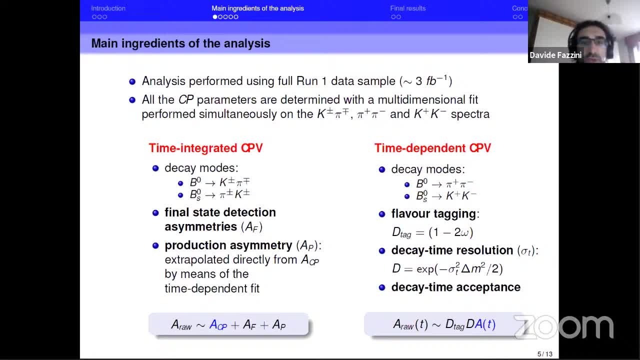 And the CP parameters are determined simultaneously using a multidimensional fit to perform on the three different spectra: K, pi pi pi and KK. So in this slide, In this slide I point to the most important ingredient for the evaluation that I integrated. 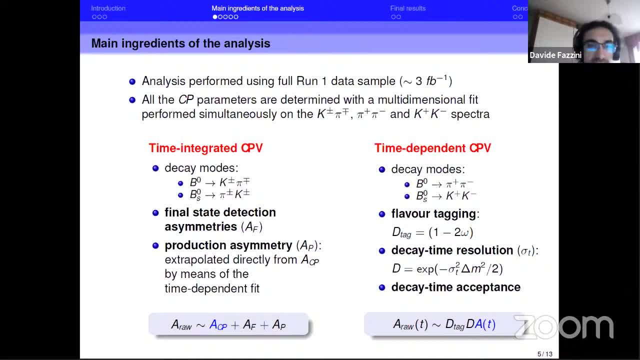 the time-dependent CP parameters. So for the first group, as you can see from the bottom of the slide, the raw asymmetry can be determined in the sum of the three components: one related to the CP asymmetry, and then we have a symmetry due to the final state detection symmetry. 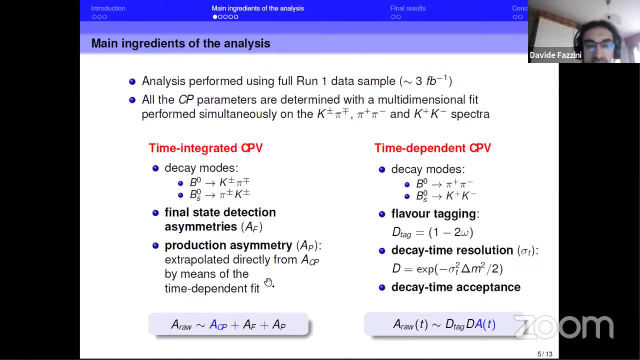 and the production asymmetry. The first term is used as external input, while the second terms can be extracted directly from the SCP by means of a time-dependent fit For the time-dependent CP relation. instead, the key points are the flavor tagging and the key time. 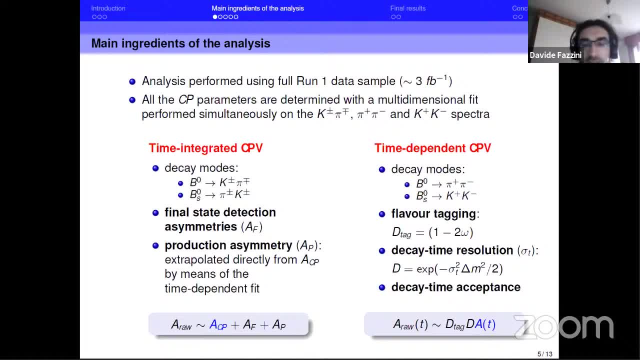 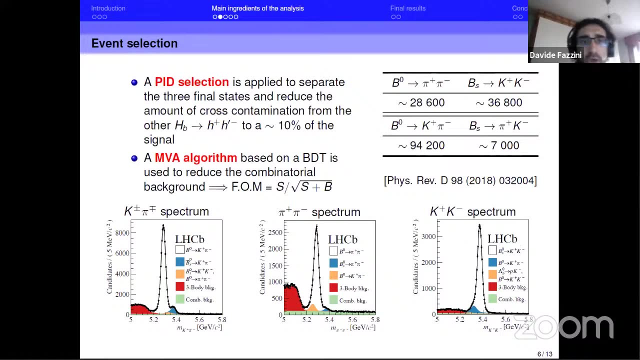 resolution which indeed diluted the true asymmetry, introducing two factors and the dedicated acceptance which had large effect on the KK parameters, in particular on A delta kappa KK. So, starting from the event selection, this is based on two different steps. 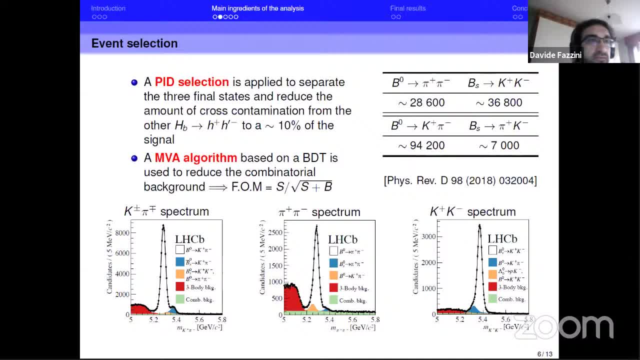 The first is based on P, the selection which is used to separate the three final states- KK, pi, pi and K? pi- in order to reduce the amount of cross-feed background contamination up to 10% of the signal yield. And then we perform a second step. 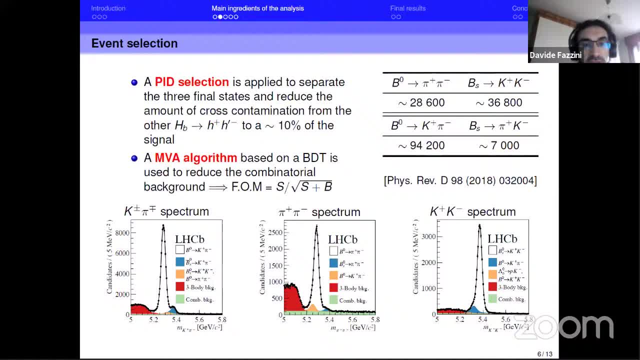 using a multivariate algorithm based on the boost decision tree, used to reduce mainly the combinatorial background, And then we optimize using the signal divided, the square root of signal plus back. So here on the right you can see in the table: 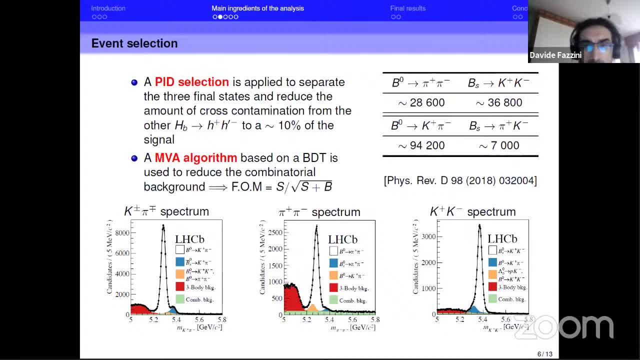 the final yields for the four main signal mode And in the bottom instead, you can see the invariant mass distribution for the three different spectrum. In white, you can see the signal which is clearly visible. In green, the combinatorial background. 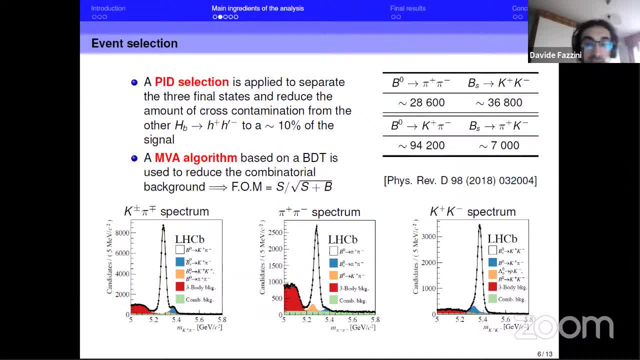 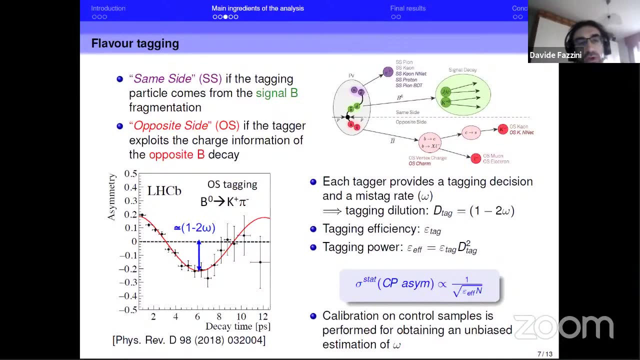 which is very small, And then, in red, the free body, partially reconstructed the mode, And in orange, the cross-feed, which are very reduced. So, starting from the flavor, going on with the flavor tag, which represents a key feature for the time-dependent analysis, 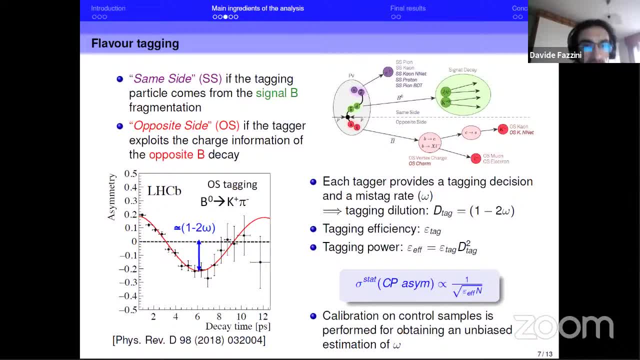 And in LCB we have two different kind of algorithms: the same side taggers which exploit the charge of the particle coming from the signal B fragmentation, which on the right. there is a sketch with the flavor tagging algorithm available In LCB and the top part is the one related 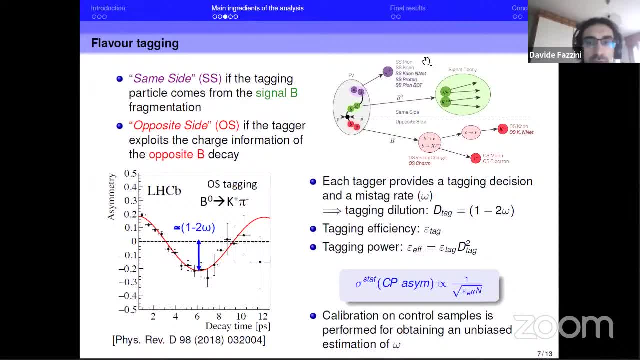 to the same side taggers. So we have the algorithm that exploit the pion, proton and ancheon, And then we have the opposite side, charmer, which exploits the charge information of the decay of the opposite bit, which is in the bottom part of the sketch. 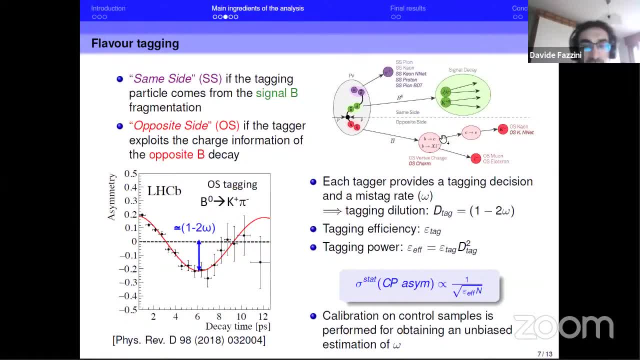 So each of these algorithms provide the tagging decision and the mistag rate, which is quite important since enter directly in the dilution term that I mentioned before, And the performance on these algorithms can be estimated using the tagging power, which is the product of the tagging efficiency and the dilution. 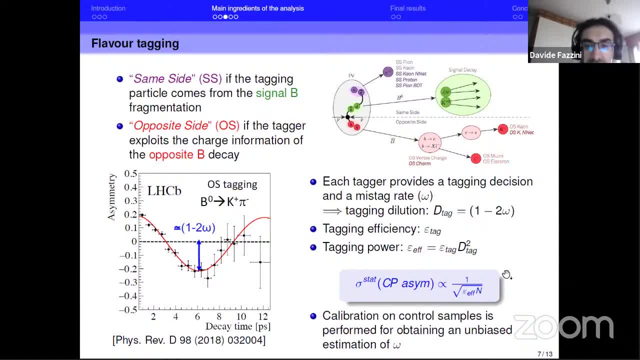 factor squared, which is also quite important, since it is inversely proportional to the statistical uncertainty of the Cp parameter asymmetry that we want to measure. Of course, in order to have an unbiased estimation of the mistag probability, we have to calibrate the information provided by the tagging. 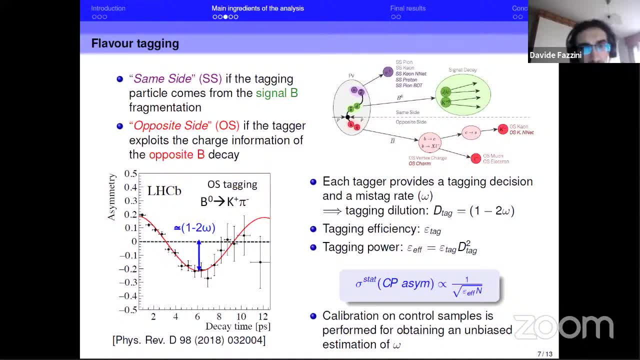 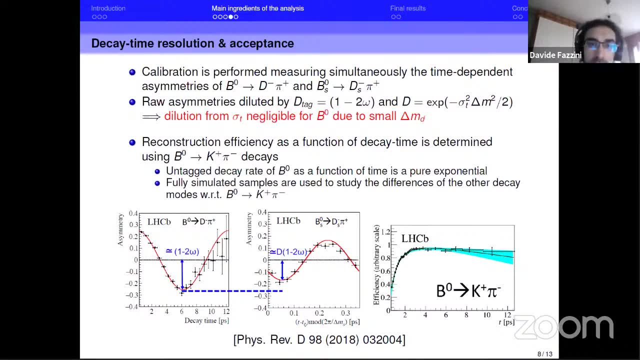 algorithm And this is performed on a specific control sample. Going on with the decay time resolution, this is calibrated using simultaneously the b0 to dpi and bs to dpi decay, performing a time-dependent fit. So, as you can see from the plot on the left of the slide, 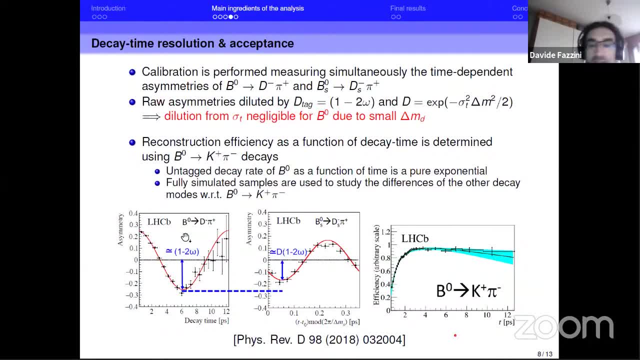 the symmetry in the b0 to dpi is basically reduced only by the dilution factor coming from the flavor tagging, since delta md is very small And so the dilution from the decay time resolution is negligible, While for the bs we have both the b0 to dpi decay. 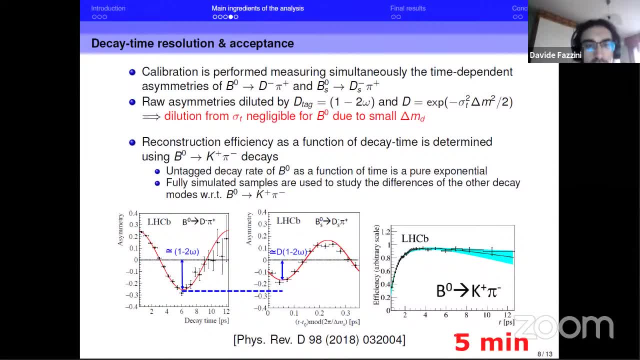 and the bs to dpi decay. We have both the dilution factor. So from the first sample we can estimate the dilution for the flavor tagging And then, looking at the difference, estimate the dilution from the decay time resolution and then performing a calibration. 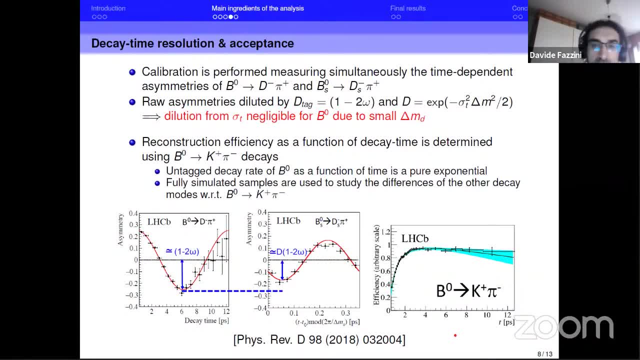 Regarding the reconstruction efficiency, this is determined as a function of the decay time using the b0 to dpi decays Indeed. for these decays, the unpacked decay rate can be expressed as a poor exponential. So it's quite easy to retrieve the related reconstruction. 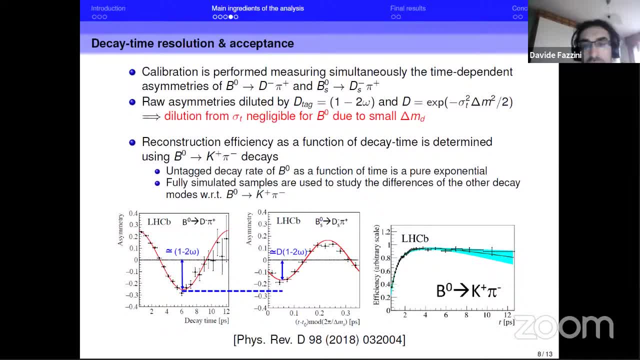 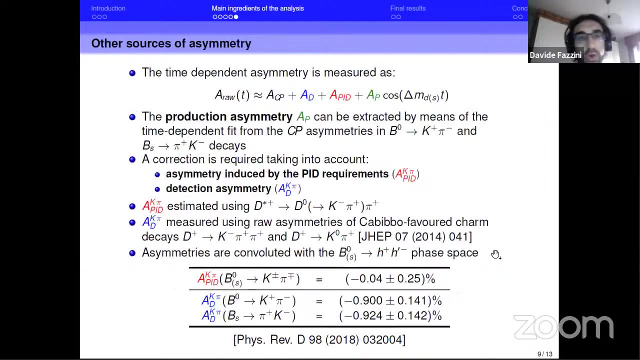 efficiency And then for the other decay signal mode, we basically correct the acceptance for the b0 to dpi for some factors that are estimated from fully simulated sample. Yeah, on the right on this slide you can see the acceptance function for the b0 to dpi. 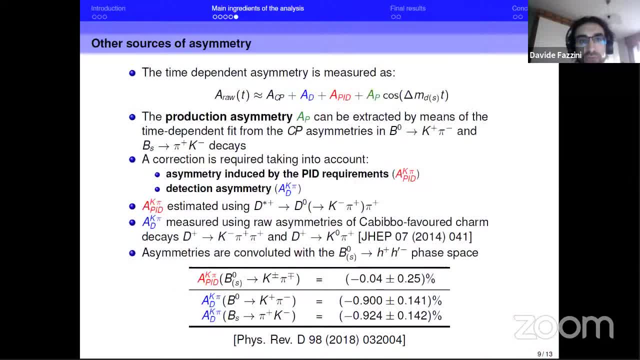 Going to the last ingredient that I mentioned before, that are, the production and the final state detection of symmetry. So the time-dependent symmetry can be measured as described here on the top of the slide. So we have different contribution, a term related. 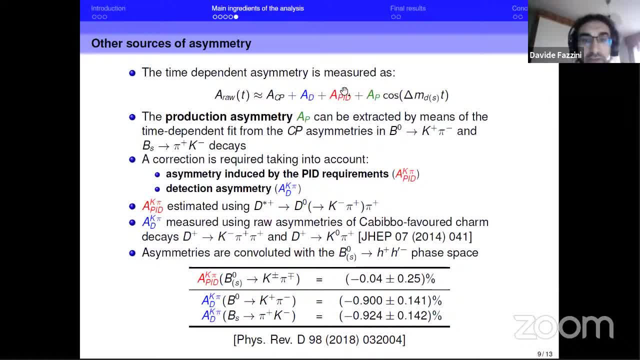 to the CPS symmetry, then a term related to the final state. two terms actually. One term is related to the detection of symmetry and then another term related to the PID requirement applied to select the free spectra, and then the production assent. 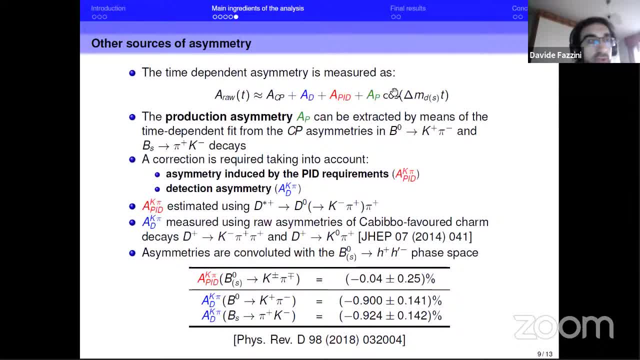 As you can see, this last term is multiplied by a cosine term, So it can be extracted by means of time-dependent symmetry. So we have two terms and we have to take their value as external input, And so the PID assymetry is estimated using the d star. 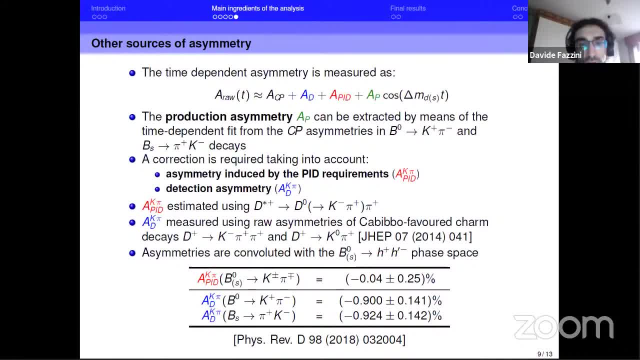 plus to d0 pi dk's, while the detection assymetry is measured using the raw assymetry of Kavipo-Faberet charm dk's, d plus in k pi pi and d plus in k0 pi dk's And of course, at the end, these assymetries. 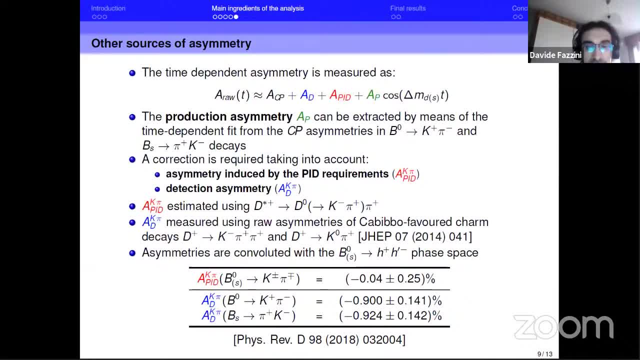 are convoluted with the b0 to d0 pi dk's. So we have two terms and we have to take their value as external input. They are convoluted with the b0 to hh phase space. in order to have a proper correction. 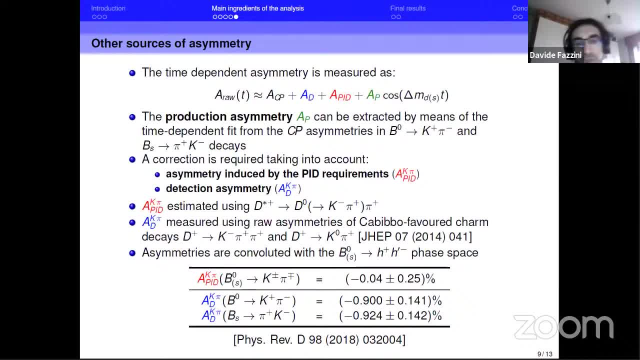 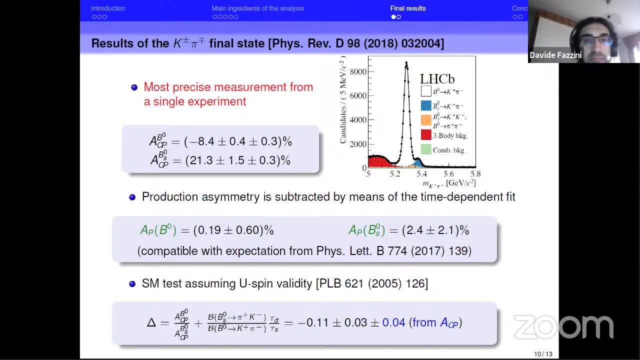 Here in the bottom of the slide, you can see the value for this assymetry for the b0 to d pi and for the ds2 pi, k dk's. So going to the results, these are for the k pi, final state. We obtained the most precise measurement. 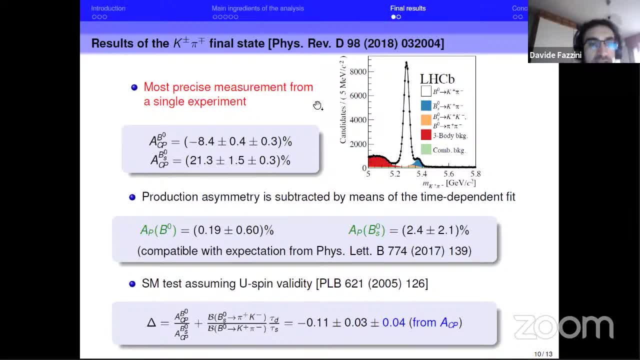 from a single experiment. Here in the first box you can see the value for the direct CPS symmetry. On the right there is the environment mass distribution for the k pi spectrum And, as I said, the production assymetry can be determined directly by means. 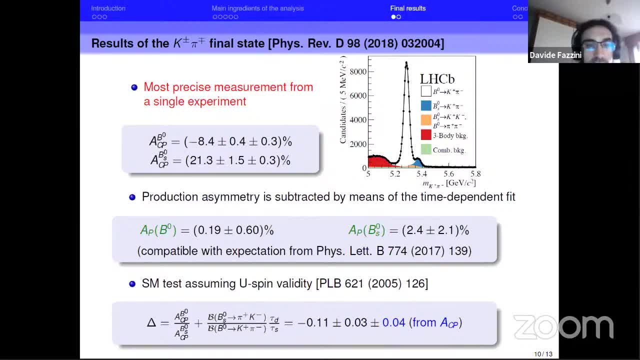 of the time-dependent fit, And here I report also the value that we obtained for the b0 and the bs, And these are compatible with expectation. And we also perform a test on the standard model validity, assuming they use spin symmetry. So we evaluated this discriminant delta. 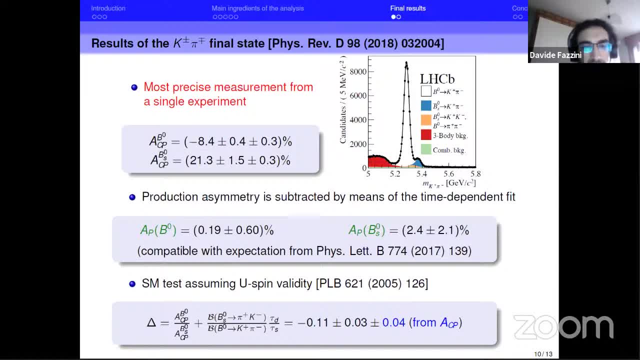 which is defined as the ratio between the SCP asymmetry between b0 and bs, plus the ratio of the branching fraction of the 2dk mode, times the diffraction, The ratio between the lifetime of the b0 and the bs, And we obtained the results reported here in the slide. 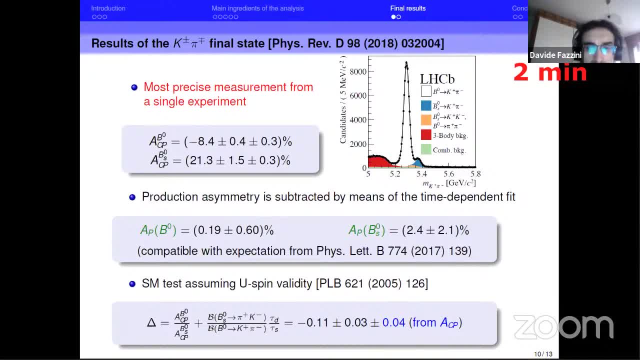 We have. the first error is related to the fixed parameters, to the fixed value report used for the evaluation, And the second term is related to the CPS symmetry, And this is found to be compatible with the standard model expectation, which is 0.. So, moving to the pi pi and kk final state, so for the pi pi, 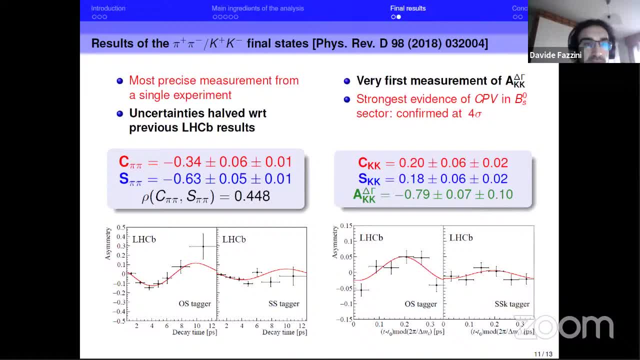 we have the same error. We have the same error, And for the pi pi we have the same error, but we are using the same data to find the case, And then we have the same error And we have the same error. 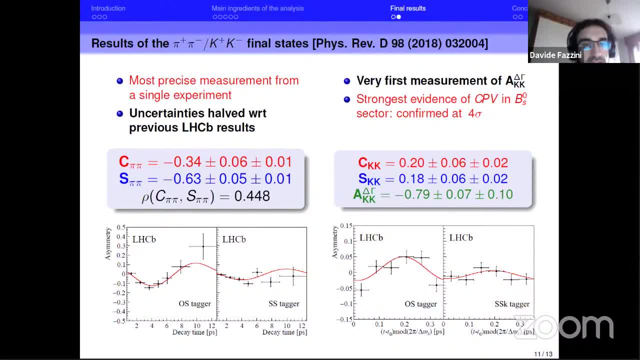 So in this case we obtained the most precise measurement from a single experiment. We basically have all the uncertainty, both statistical and also systematic, obtained in the first LSTB analysis. Here you can see the results for c pi pi and s pi pi. 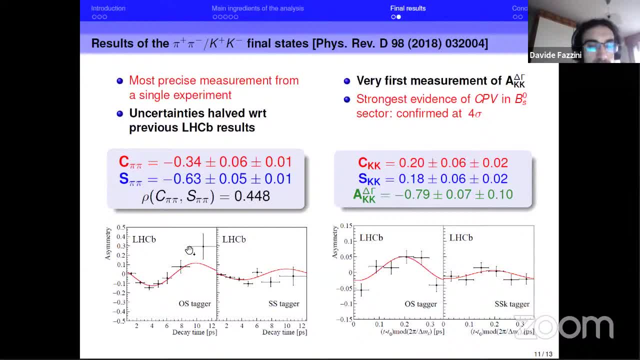 where the first uncertainty is statistical and the second is systematics, along with their correlation back Going to the KK final state, this was the very first measurement of a delta gamma KK and performing a chi-square test, we obtained the strongest evidence of CP violation in time. 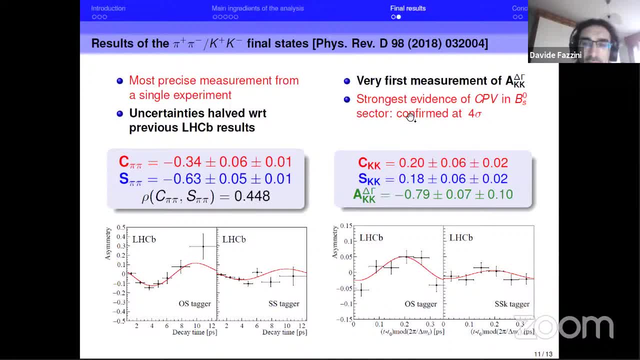 dependent analysis for the BS sector, confirmed at more than four sigma. And here you can see the results for the various CP parameters with their statistical and systematic uncertainty and, as before, in the in the box in the bottom of the slide you can see the, the asymmetry plot for obtaining using only the opposite side and only the same side attack. 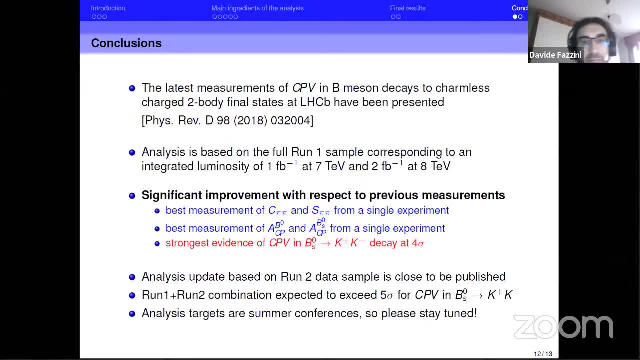 Going to the conclusion, the latest which today I will. I show you the latest measurement of CP violation in B Maison. B Maison, the case to charmless charger to body, final state, perform at the LCB and this is based on fuller and one corresponding to integrate luminosity. 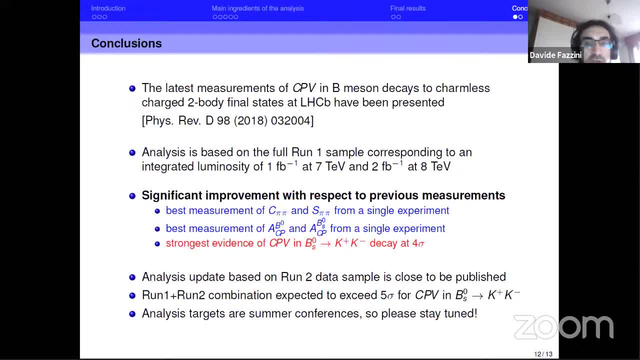 on one inverse phantom at uh, collected at seven TV, and two inverse phantom and collected at eight TV. we get- we got a significant improvement with respect to the previous measurement. we obtained the best measurement for CPI and SPI perform it from a single experiment obtained from a single. 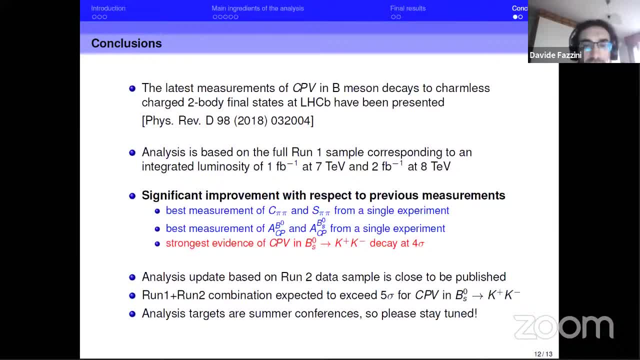 experiment, as well as for the direct CP violation in B zero to KPI and B2PiK. and we also get the strongest evidence of relation in the BS sector at more than four sigma. So the analysis, the analysis of data based on run two data, is close to be published. 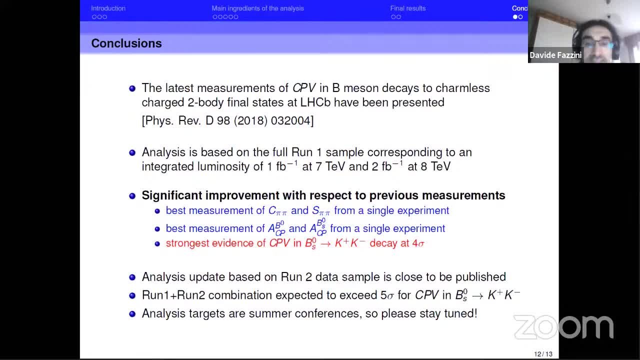 We expect that the, the combination of one plus run two, exceed the five sigma for the CPI, CP violation in BS2KK. and then the target of the analysis are the summer conferences. so in the next few months you should see the new presentation with the new results. so please stay, stay tuned. 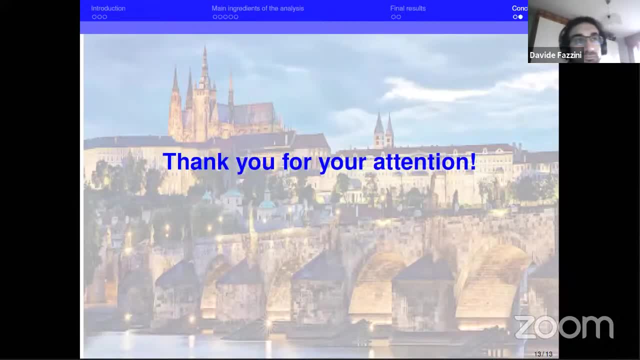 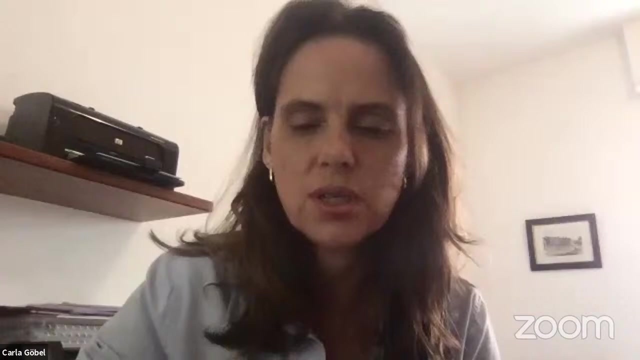 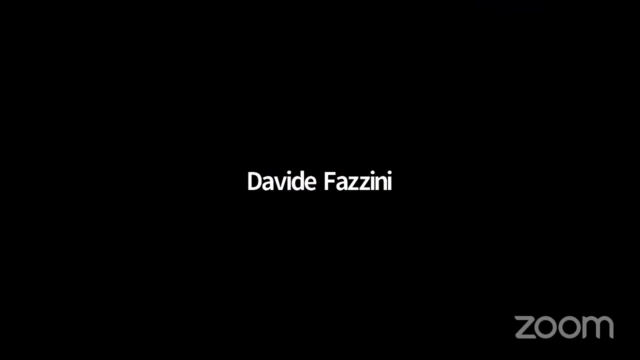 and that's all from my side. so thank you for your attention. Thank you, Davide. Questions, Comments. Otherwise, thank you again and remember to make questions at the Mattermost channel. So now we move to three body charm: charmless BDKs. uh in LHCb, uh from uh Tomas Grammaticum. 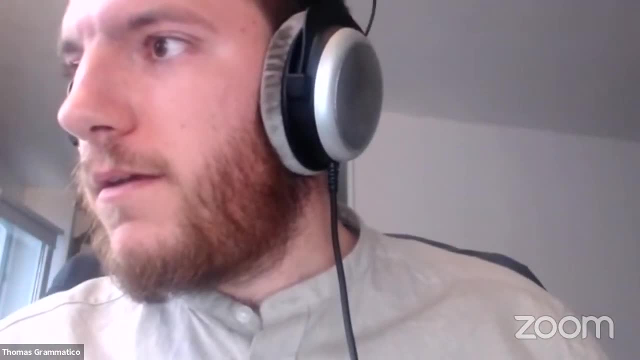 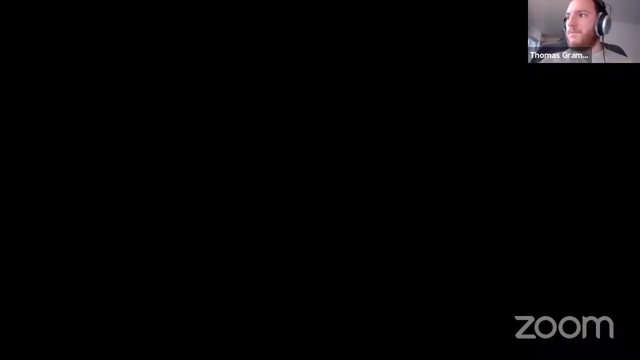 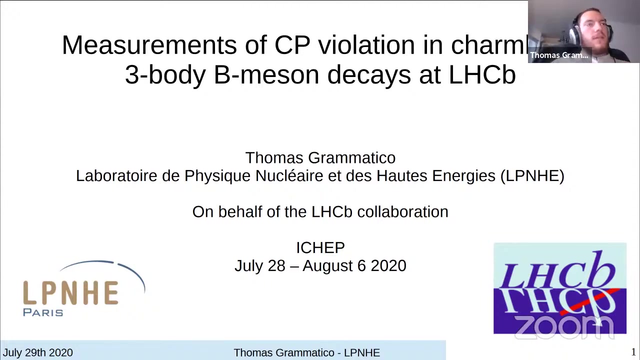 Hello, can you hear me? Yes, Okay, great. Let me show my slides. Okay, is it working? Yes, Okay, great. Okay. so today, good evening everyone. Today I'll be discussing the recent measurements of CP violation in charmless 3 body beam isn't. 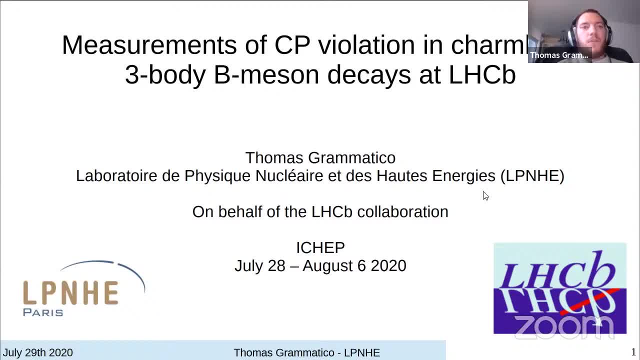 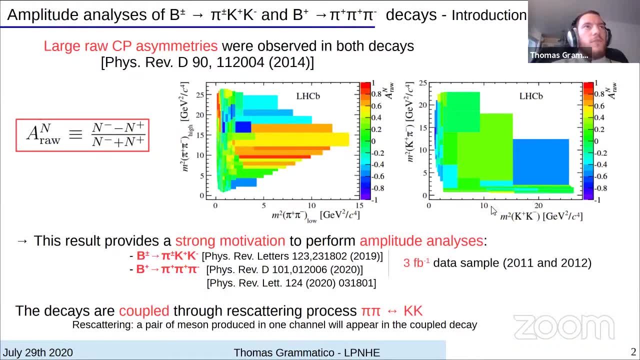 decays at LHCb. uh, I'm Thomas Grammaticum and I'm talking today on behalf of this, a member of the research team and our participants. Toma Grammaticum and I'm also talking about both LHCb collaboration. Today I will focus on two amplitude analysis: the amplitude analysis of 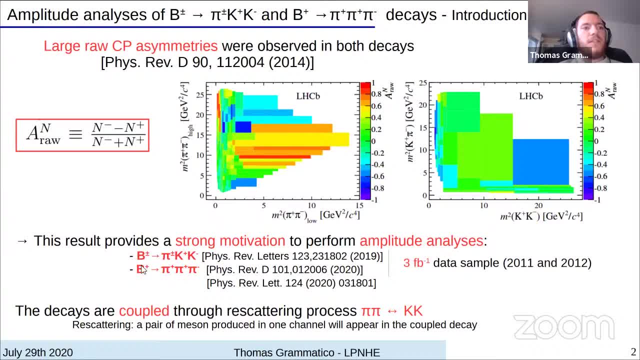 b2 pi kk decays and the amplitude analysis of b2, 3 pi m decays. Why is it interesting to perform such amplitude analysis If we take a look at those two plots here. so those are the row asymmetries represented as Dalitz plane four. on the left, b2, 3 pi m and on the right 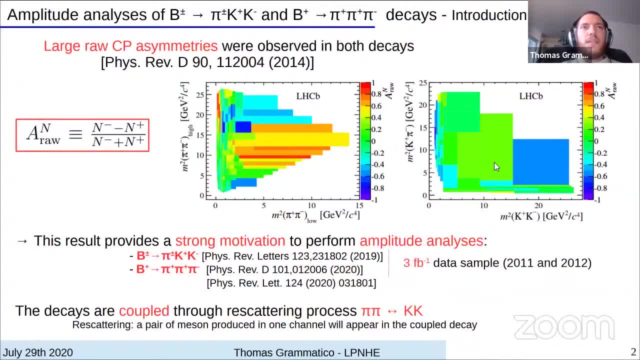 b2 pi kk, and what we can see is that we can see the large row asymmetries. In the case of b2, 3 pi m, there's even asymmetries where there is no known resonances, And so for those reasons it's quite interesting to have a look at the to perform the amplitude. 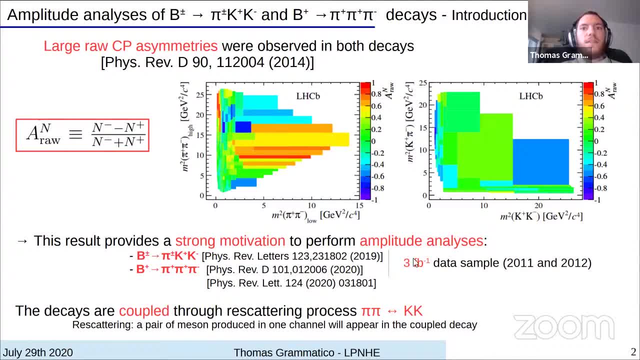 analysis of that, And so for those reasons, it's quite interesting to have a look at the to perform the amplitude analysis of b2, pi m analysis, And also so this analysis will use three inverse phantom bounds of the data sample, And the decays are coupled: 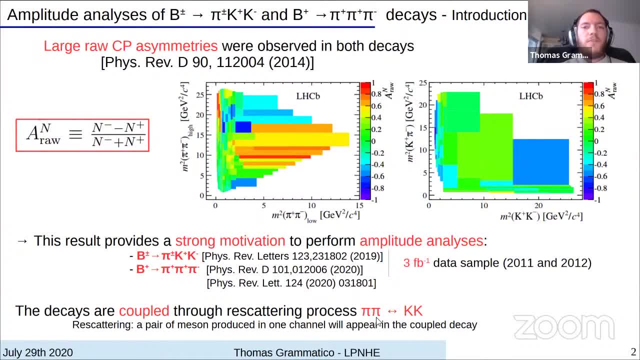 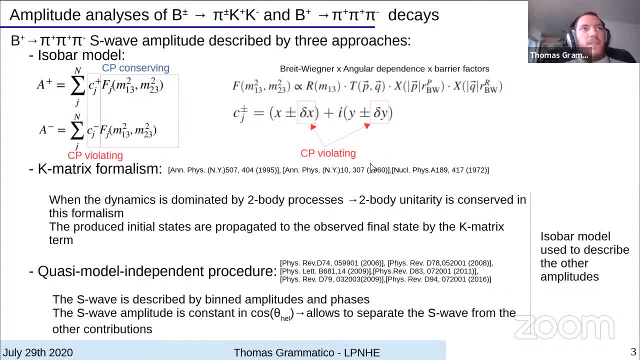 through rescattering processes between a pair of bion and a pair of kaon. In both amplitude analysis the Isoban model will be used to describe the amplitude. So the Isoban model consists of some of products over the different contribution to describe the 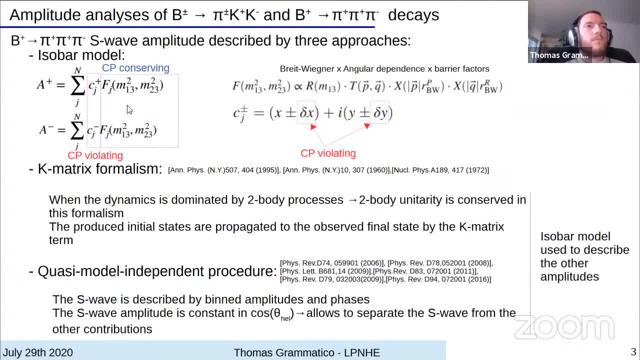 amplitude. The product contains the C term, which is CP variating, and contains the weak dynamics and the F term, which is CP conserving, And it's a product of a nice line shape most of the time to be a Bragg-Degner with an angular dependence and the barrier factors. 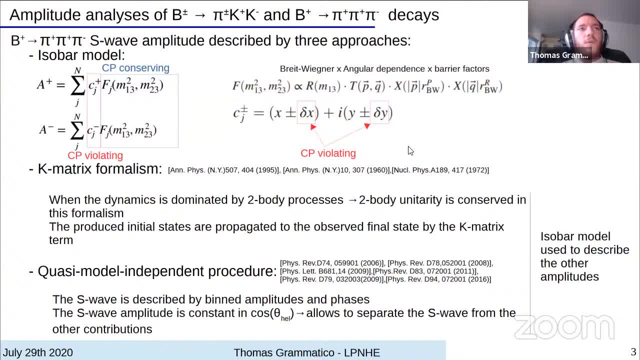 In the case of b to 3 pion, the S-wave amplitude will be described by three different approaches. The first one is the Isoban model we just discussed. Next, there are also the K-metrics formalism that will be used. 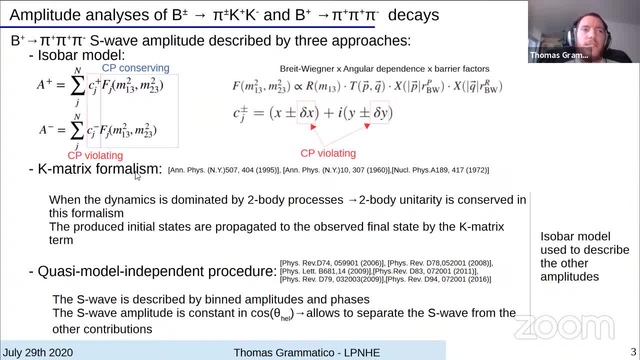 This formalism conserves the two-body unitarity when the dynamics is dominated by two-body processes. And the third approach would be the quasi-model independent procedure, in which the S-wave- sorry- will be described by bin amplitudes and phases And to separate the S-wave from the other. 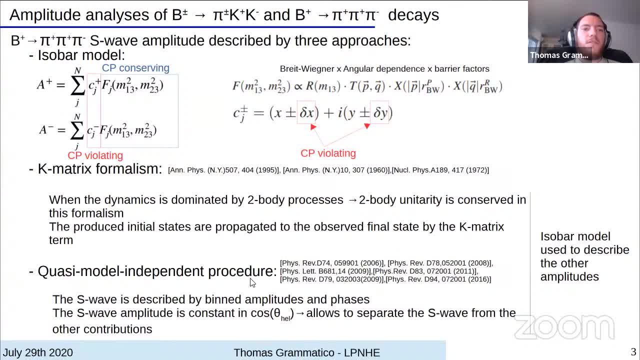 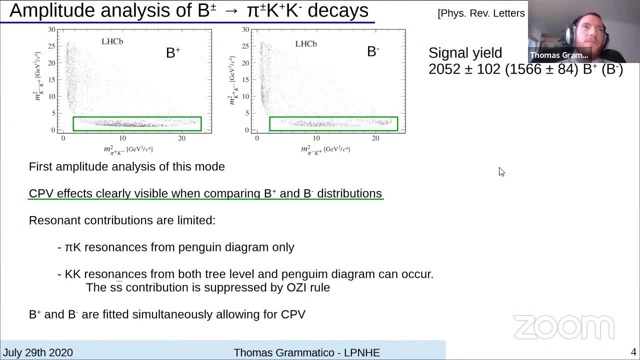 contribution. we use the fact that the S-wave amplitude is constant. Now discussing further the amplitude analysis of b to pi k k, the signal yield is about 2000 events for the b-plus decay and 1600 events for the b-minus. This is the first time that the amplitude 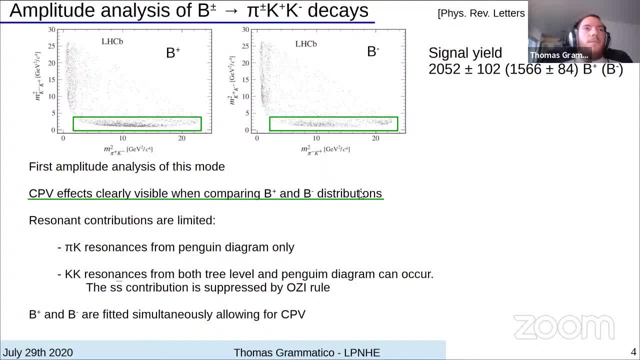 analysis of this mode has been performed. If we take a look at this diagram, we can see that the amplitude is about 1000 events for the b-minus and 1000 events for the b-minus, And we can see that the amplitude is about 1000 events for the b-minus. 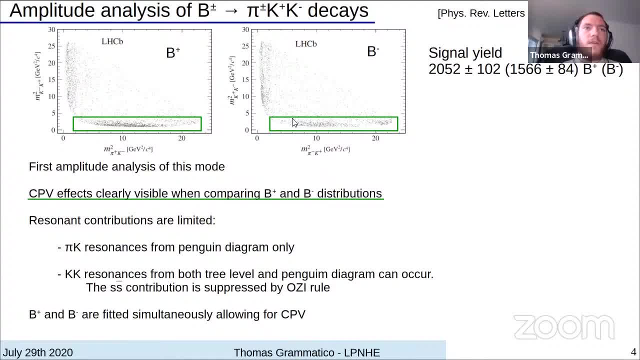 and 1000 events for the b-minus. We can already see, for example in the green boxes a clear CP variation effect when we compare the two distributions. The resonance contributions here are limited In the pi-k channel this can occur only through the penguin diagrams. For the k-k resonances they can come. 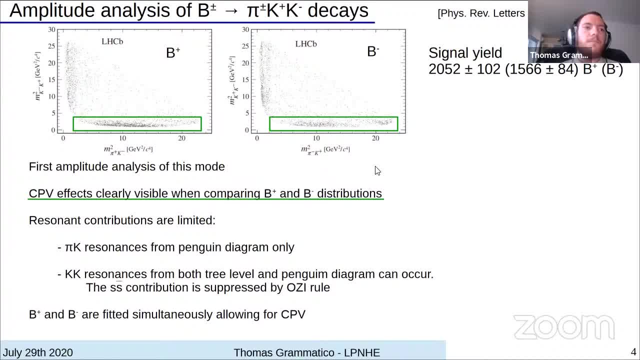 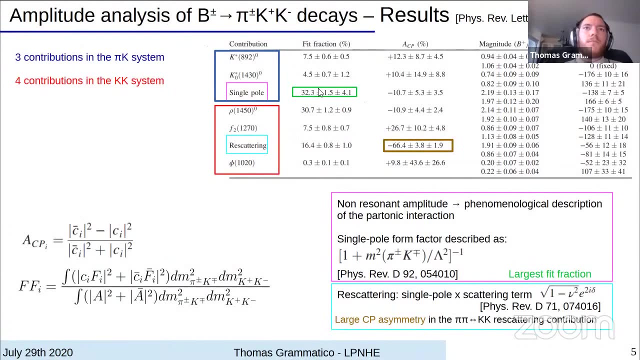 both from the tree level and the penguin diagrams, And the ss-bar contribution is suppressed by Aussie rule And the b-plus and b-minus are fitted simultaneously, which allows for CP variation. The Dalitz plane model that best describes the Dalitz plane is described here in this table. 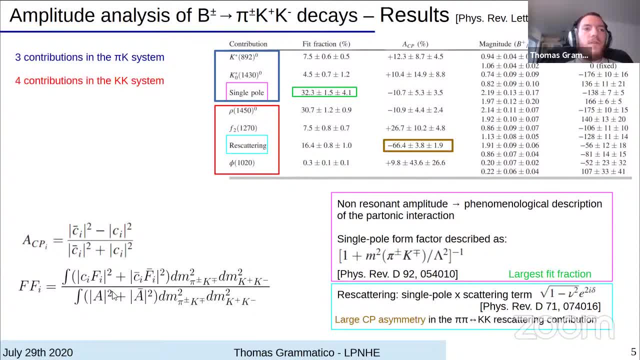 and I've put on the bottom left hand corner for the description of the fit fraction and the amplitude and the CP asymmetry. What we can see is that the main contribution comes from the single pole. The single pole is a non-resonant amplitude, which is a phenomenological description of the 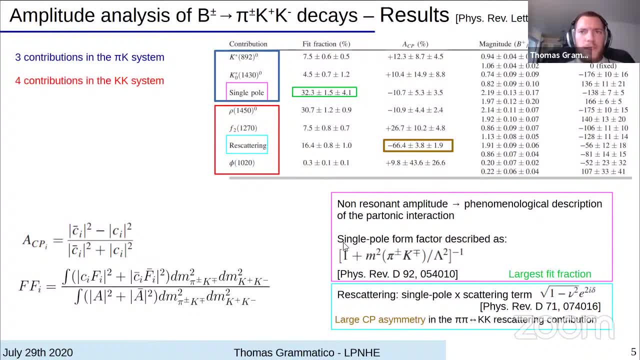 partonic interaction. Here's a description of the form factor, And another thing which should be mentioned is that the CP asymmetry of the rescattering is about minus 66% and it's the dominant CP asymmetry that has been measured here. 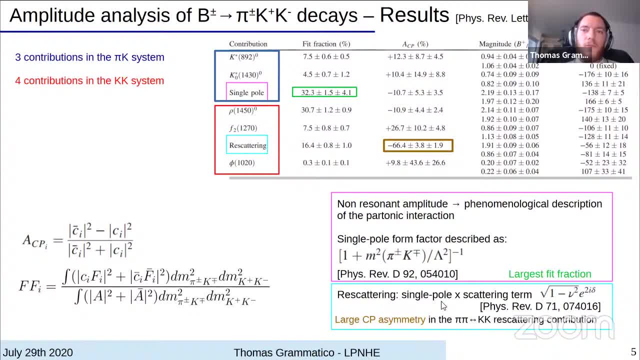 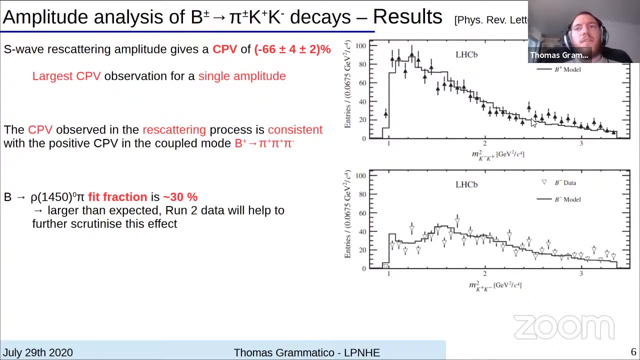 And the rescattering is described as a product of a single pole with the same description as above, with a scattering term here, where nu is the elasticity and the inelasticity- sorry- and delta is the phase shift. We have here, on the right, the projection of the number of entries on the invariant mass square of 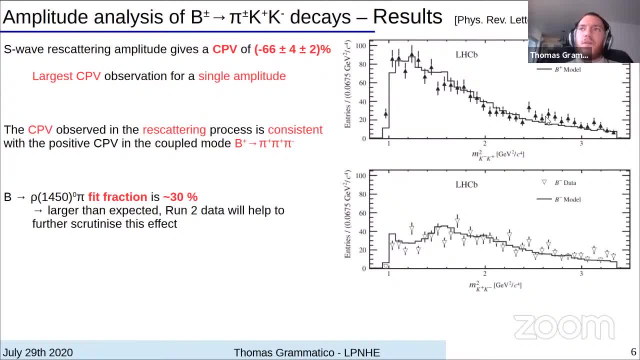 the pair of KM And looking at both the b-plus results on the top and b-minus on the bottom, we can see that the data described as triangles is quite well modeled, the model being the line, And also, again, when we compare both distributions, the CP variation is. 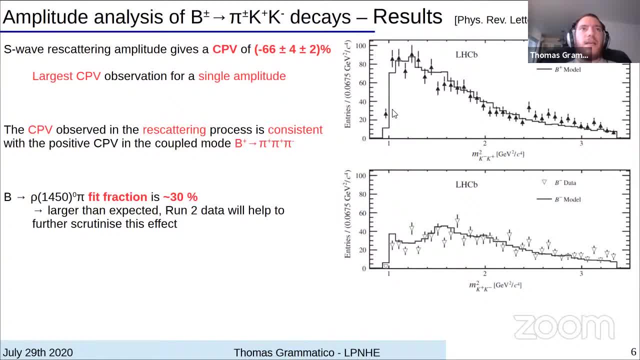 clearly visible. And so, yeah, as I mentioned, in the S-wave the CP variation is around minus 66%, which is the largest CP variation absorption for a single amplitude, And this result is consistent with what is observed in b-plus to 3-πn. Another thing is that 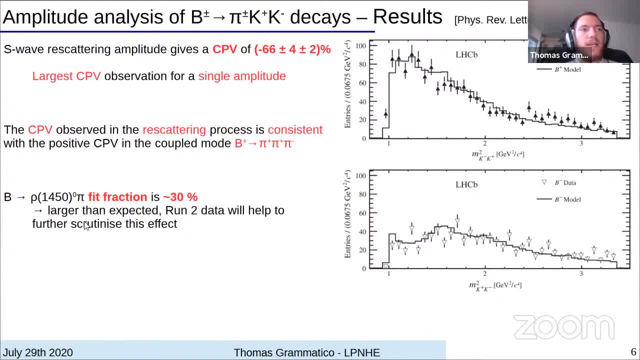 the b-to-Rho-1450π filtration is quite large, at around 30%, which is larger than expected, as the Rho is mainly decaying to 2πn And its contribution to the 3πn delta-explain is not so high. We hope, though the Rhen2 data. 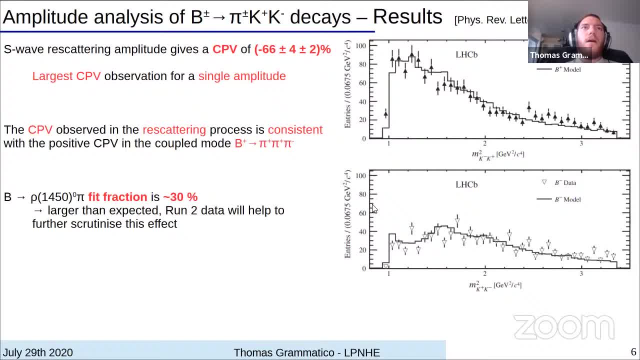 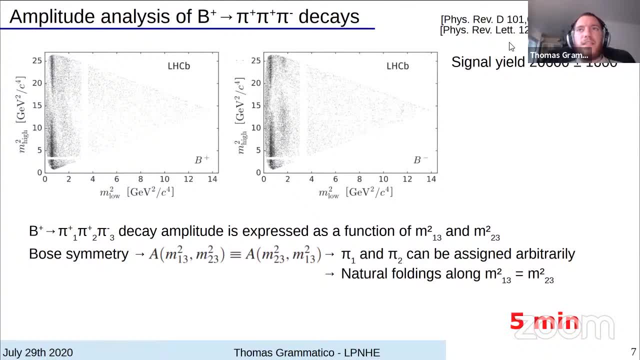 will help to understand this effect. We can move now to B2-3 pion decays. The scenario here is of about 20,000 events. We have here the Dalitz plane distribution for the B plus on the left and the B minus on the right. Here we have two positively charged pions that can be 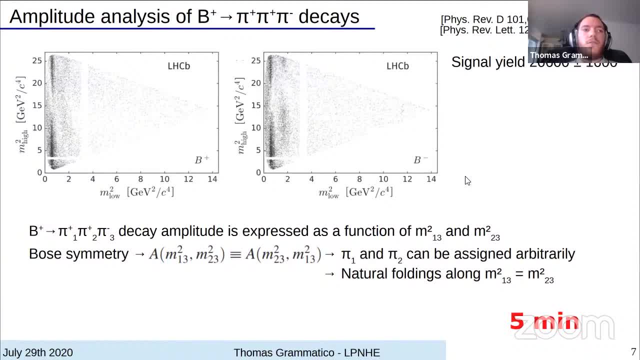 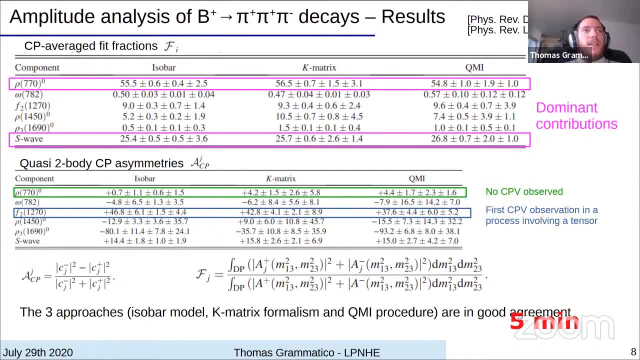 assigned arbitrarily Both. symmetry applies here. The model that best describes the Dalitz plane has as main contributions the rho zero, 770 and the S-wave. No CPU violation was observed in the rho zero case. Another thing that it was mentioning is that the F2-1270 has a CPU violation of around 40%, which is the first time that CPU violation is. 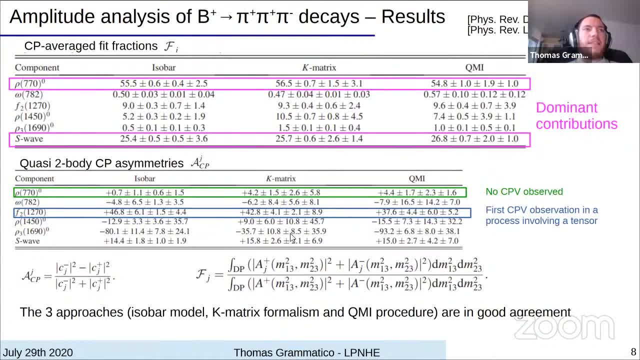 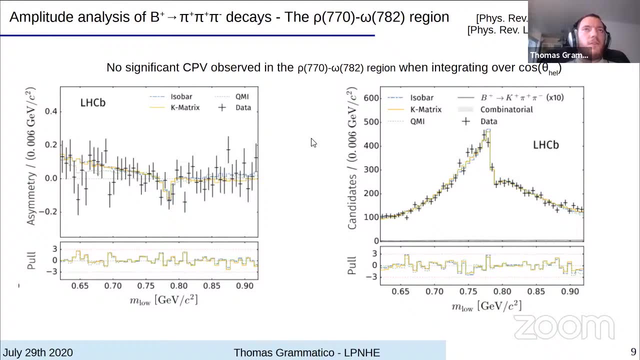 observed in a process involving a tensor. Also, the three approaches are in good agreement, as you can see on those tables. If we take a closer look to the rho omega region, we can see that there is no CPU violation observed when we integrate over cos theta L. 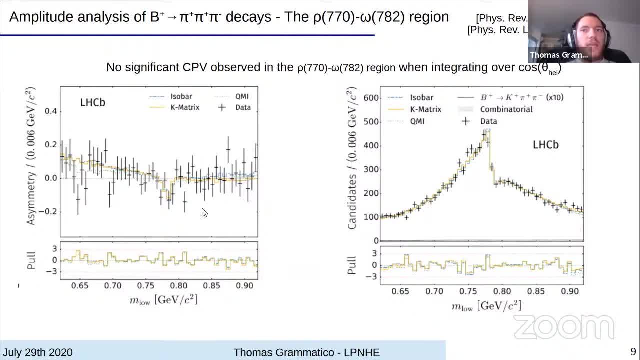 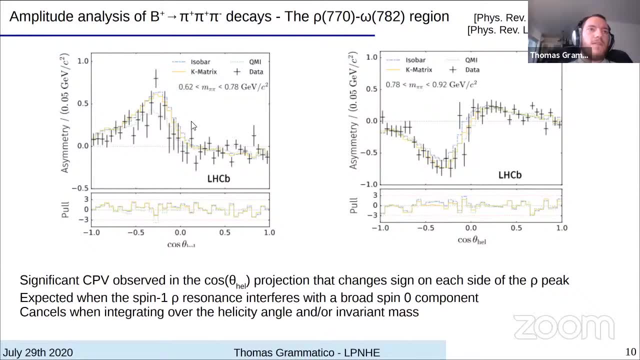 as you can see on the projection here of the asymmetry on M-low. But when we look at the asymmetry projected on cos theta ECT for the mass of the power pion, below 0.78 giga electron volt here and above this value here. 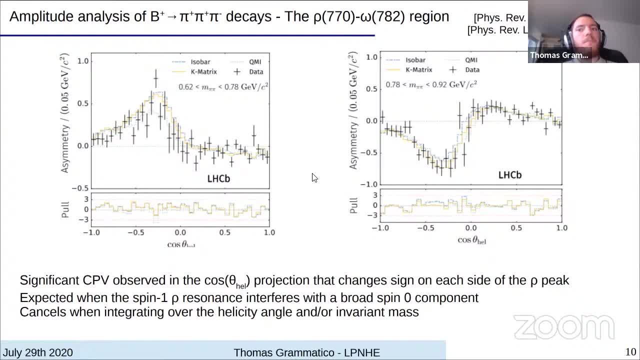 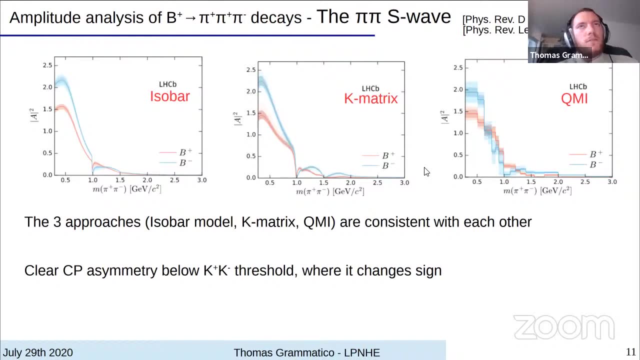 we can see that there is a significant CPU violation which changes sign on each side of the rho peak And this effect, mediae effect, conserves when we integrate over the AECT angle and all the invariant mass In the pipe-by-sweath case, we can see from those projections of the amplitude square on the mass of the power of pion, the invariant mass of the power pion and the mass of the authoritarian mass of the pion. The H-s-wave of the polarity of the mass of the power pion is just the coefficient of the weight Thepta pion of the mass of the polarity of the power pion is the various data and local mass of the pion. 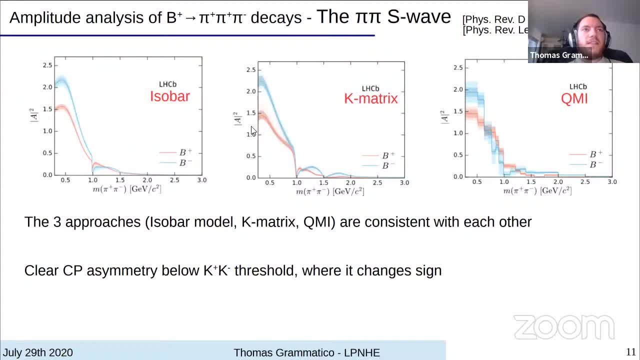 The delta of the pion is the average of the vector mass of the pion. The delta of the pion of the pion management is the value of the pion on the invariant mass of the perfpion. we can see that the three different approaches. 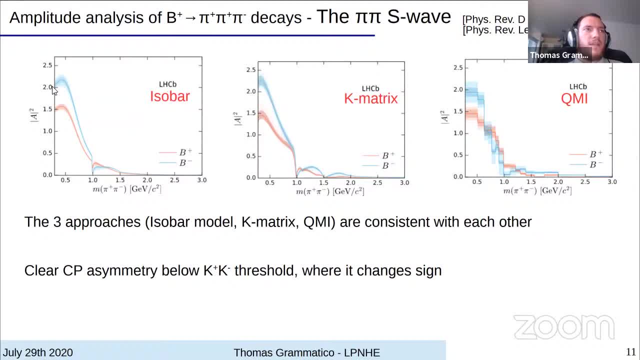 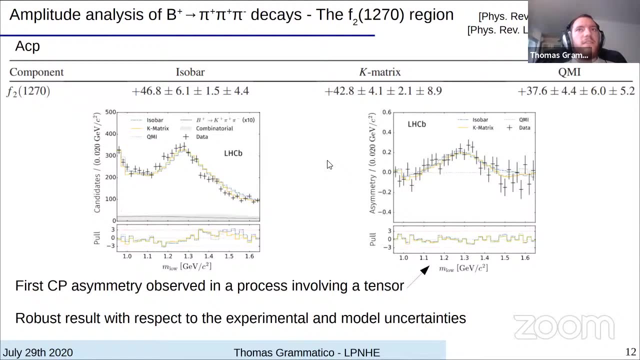 are quite consistent with each other. And also there is a clear CPI symmetry below the K plus, K minus threshold where it changes sign. And yeah, in the F2-1270 region, as I said, there is a CPI symmetry result of about 40%. 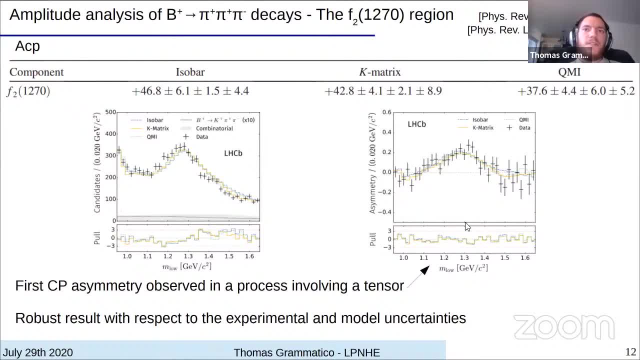 As we can see also on this plot, which is the asymmetry projected on the M low. This is the again the first time that such an asymmetry has been observed in a process involving a tensor, And this result is robust, with respect. 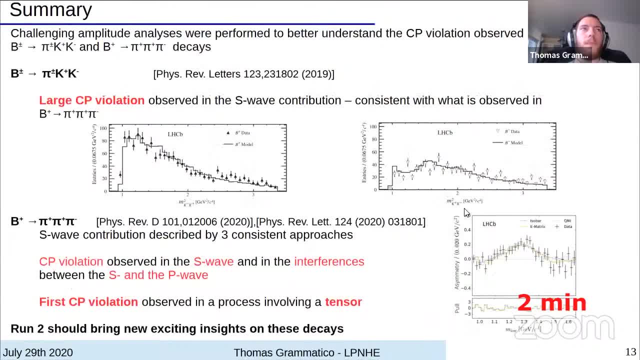 to the experimental model uncertainties. To summarize, to better understand the raw asymmetries that were observed in B2piKK and B2-3piN decays, challenging amplitude analysis were performed In the case of B2piKK, as you can see on those plots. 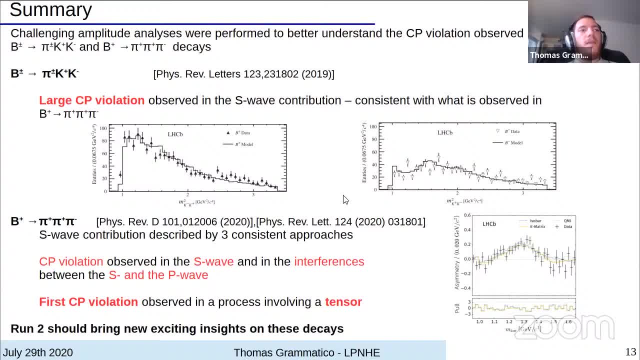 large CPI variation was observed in the S-wave contribution, which is consistent with what is observed in the B2-3piN. For B2-3piN, the S-wave contribution that is included in the model that described. that explain is well described by the three approaches. 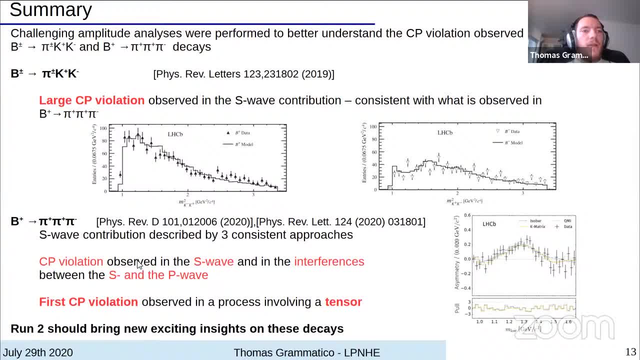 and they are consistent with each other. And there are three sources of CPI variation that I would like to mention now, which are the situation in the S-wave, in the interferences between the S and the P wave in the S-wave, and also separation in a D-wave, which is the first time that this has been observed. 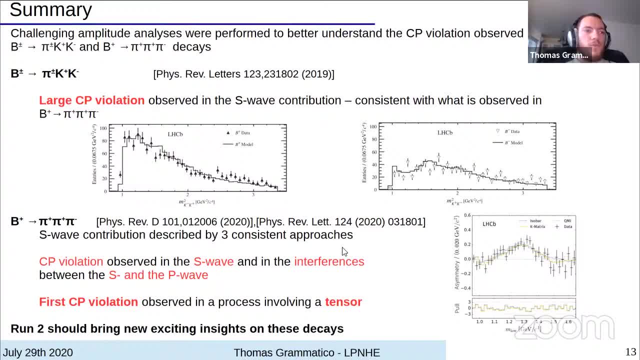 And so, yeah, we expect that the RUN2, we hope that the RUN2 will bring new, exciting insights on these decays. Thanks for your attention. Thank you, Thomas. Questions, Comments: I don't see any, So in that case, thank you again. And now we move to charmless B-Barrions. 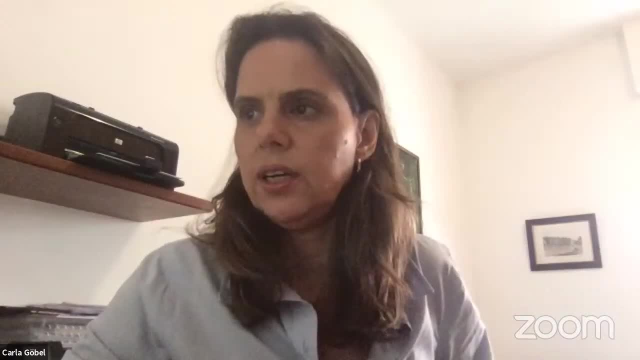 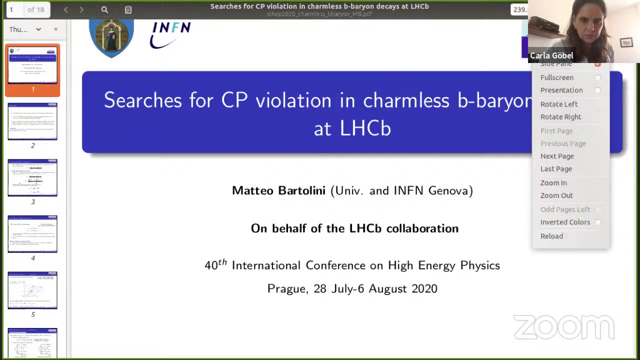 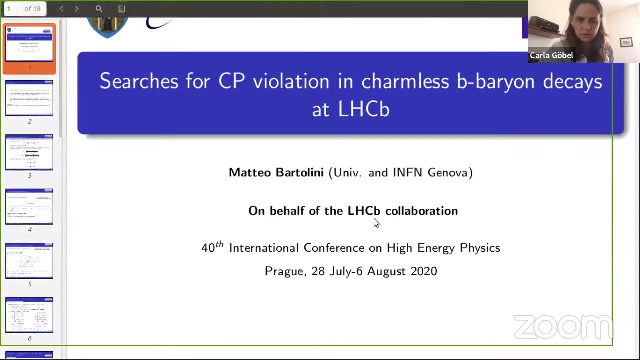 Thank you From Matteo Bartolini. Okay, I see the slides. You're muted. Okay, Can you hear me? Yes, Thank you. So good afternoon, So I will. in this presentation, I'll be talking to you about the latest results from LHCb concerning the search for CP violation in charmless B-Barrion decays. 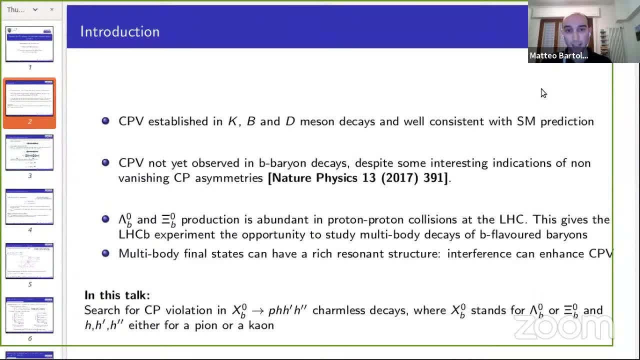 As you know, a CP violation is well established in K, B and D-Mason's decays and is well consistent with some of our predictions. But it has not been observed yet in B-Barrion's decays. Also, Lambda-B and Xy-B production is abundant in LHCb. 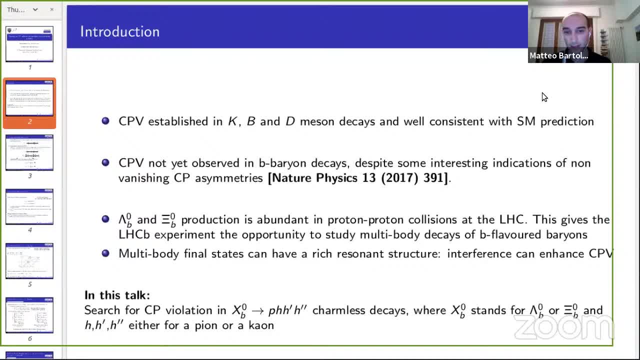 And this gives the LHCb experiment an opportunity to study multi-body decays of B-flavored biomes. Multi-body final states are a very interesting place to search for CP violation because they can exhibit average resonance structures and therefore which can cause local CP violation effects. 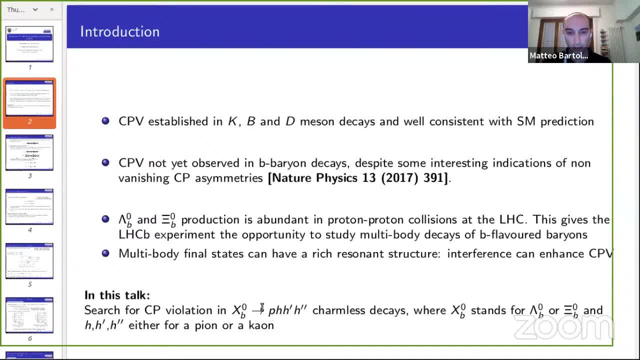 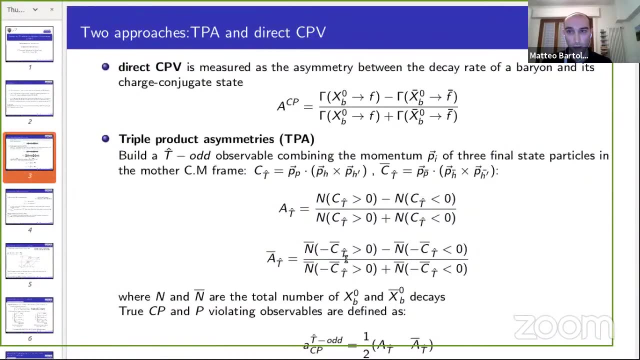 So in these talks I'll be talking in particular about this case, with this topology, where either Lambda-B or Xy-B decays to a proton and three mesons which can be either pines or kaons. So to this talk, two approaches will be used. 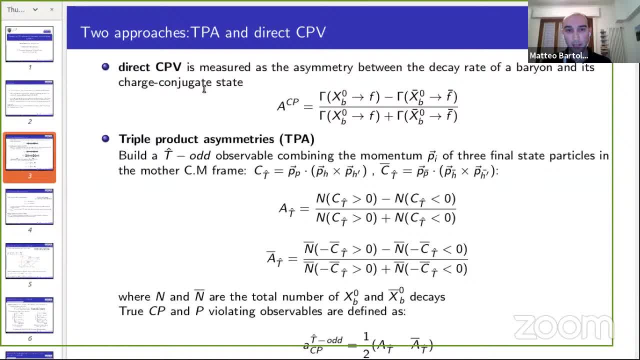 It will be shown on the standardized CP evaluation methods, which measures the asymmetry between the decay rate of a baryon and its charge conjugate, and a complementary approach which is called typical product asymmetries, where one builds a fjord observable. 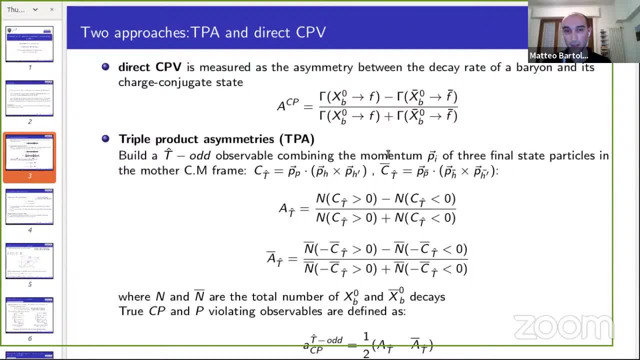 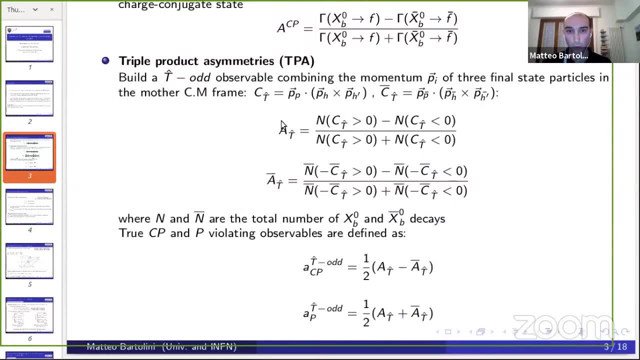 by combining the momentum of three final state particles in the mother rest frame And by splitting the data samples according to the sign of this C variable and the flavor of the baryons, one can measure these two CP violating asymmetries and also these two P violating asymmetries. 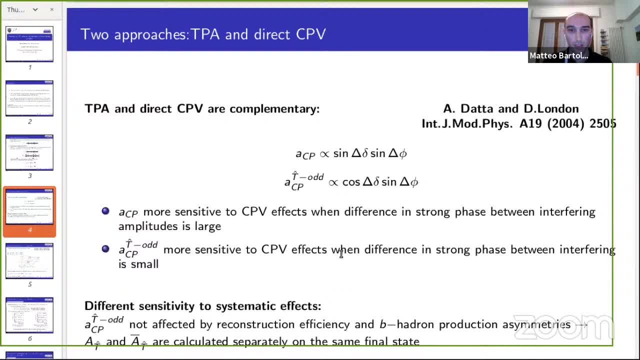 These two approaches are complementary in the sense that they have different sensitivity to the physics. The standard CP evaluation is more sensitive to CP violating effects that have when the difference in strong phase of the interfering amplitude is large. On the contrary, the CP et of the asymmetries is more sensitive to effects. 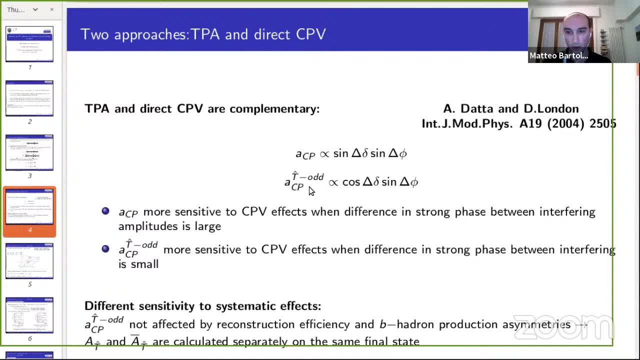 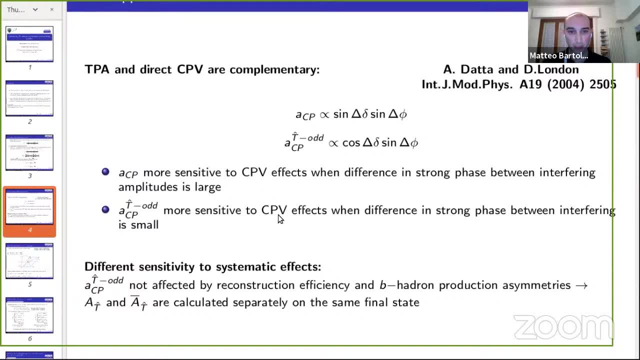 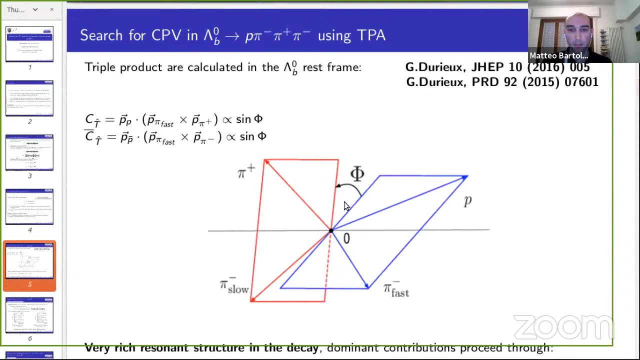 where the difference in strong phase is small. They also show different sensitivity to systematic effects because by definition, the CP et of the asymmetries is not affected by the construction efficiency and the potential baryon production asymmetries. Let me first start with the first experimental results. 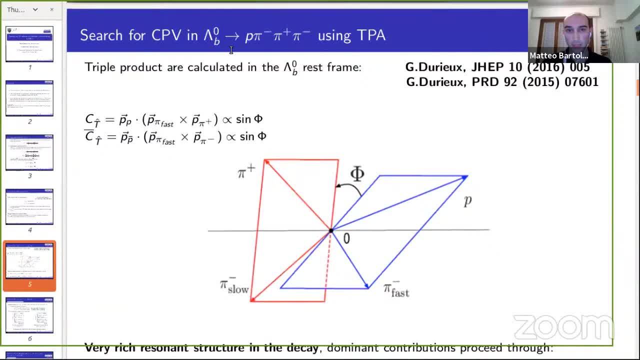 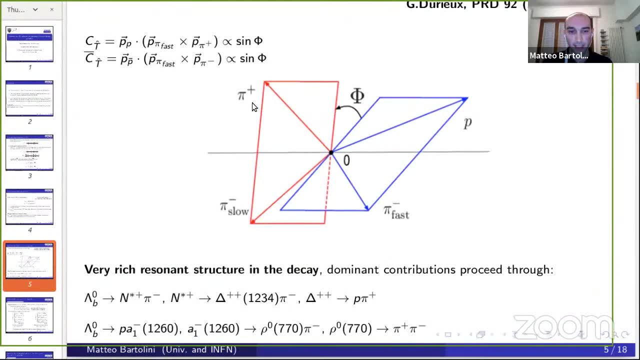 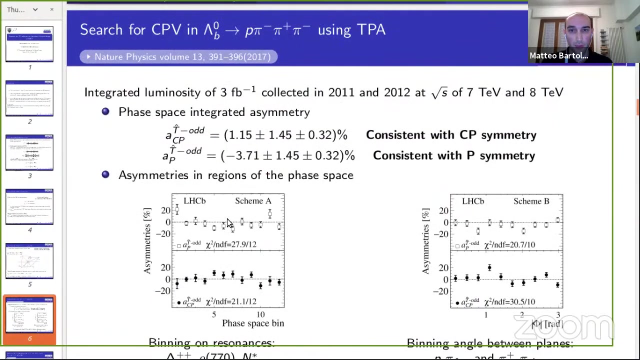 concerning the central CP relation in λv to protons and triplines, using typical product asymmetries, These decays are very rich in restaurant structures, where contributions proceed mainly through these quasi-to-body decays listed here. The first measurement was released by LHCb in 2017. 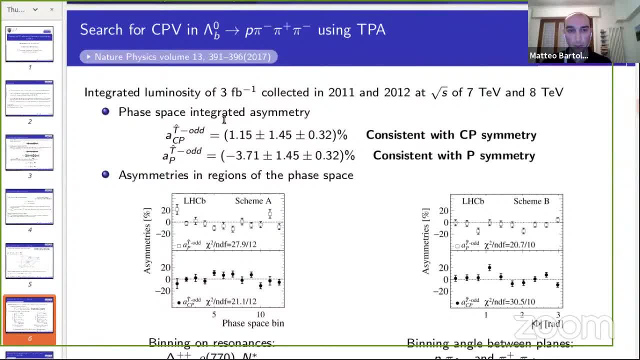 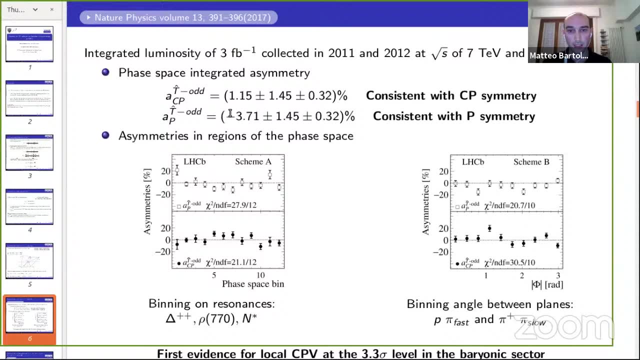 by using a sample of corresponding material luminosity of 3-inverse femtobar in run 1.. And So both the phase-based intermediate asymmetry was measured, where both the CP and P asymmetries are consistent with 0, and also asymmetries in the regions of the phase space. 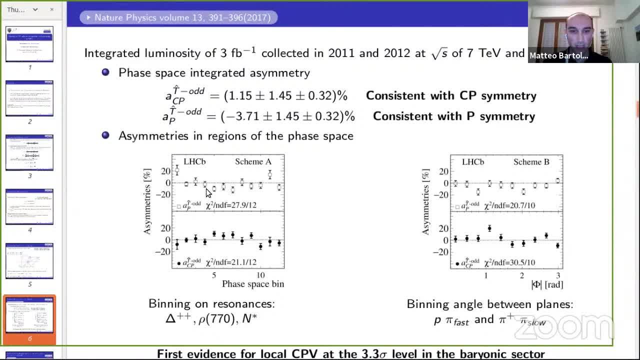 to be more sensitive to local simulation effects. So two schemes were defined: Scheme A, where one bins on these resonances mainly, and also on the PHI, which is the angle between the angle defined by the planes of these combination of these two particles. 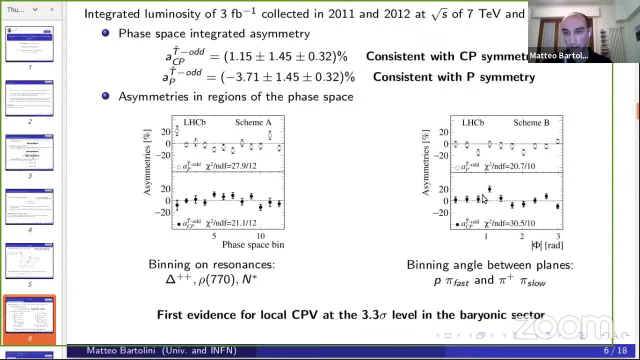 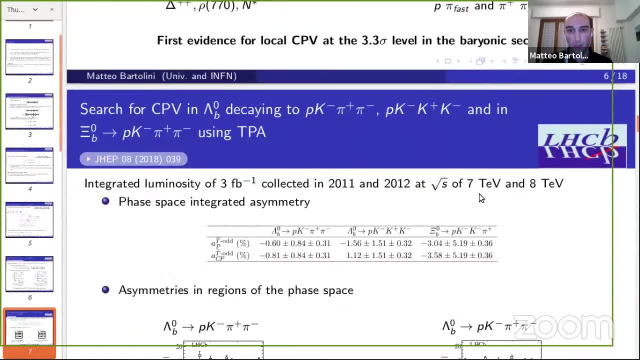 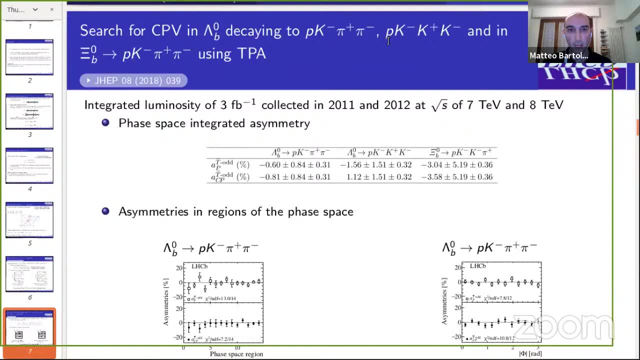 And one series here that for the first time one sees the first evidence of local CP relation effect at 3.3 signal level. A similar approach, same approach but with slightly different decays listed here was used. was measured in using run 1 of a set. 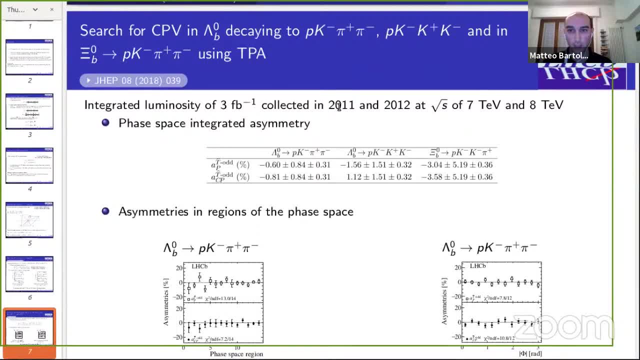 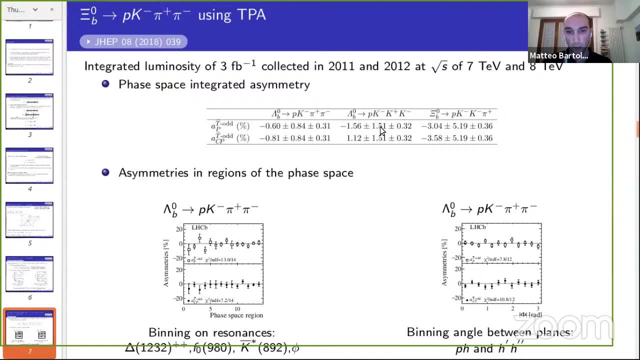 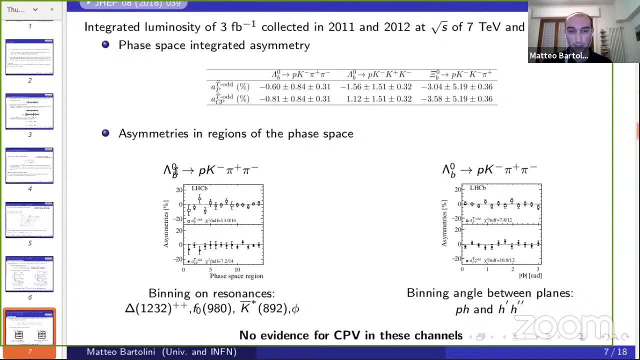 in 2011-2012.. And both the phase-based intermediate asymmetries for the three channels are consistent with 0.. And also the asymmetries in regions of the phase space, like, for example, this decay binning on. 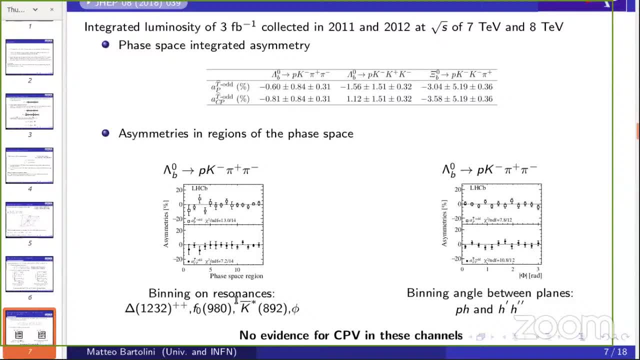 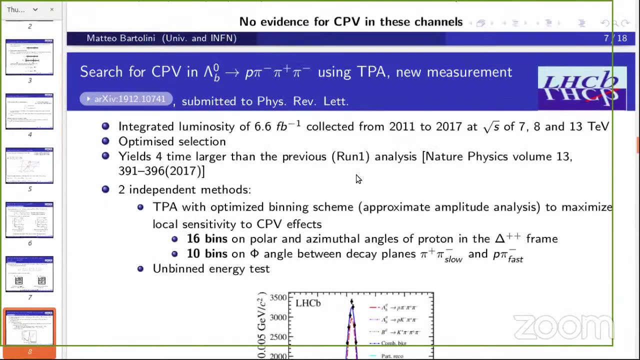 binning was done on these resonances, renouncing contributions of the resonances, and also on the angle defined by the this particle And no evidence for CP variation is found. Now the this decay lambda b to proton as n of 3 pines. 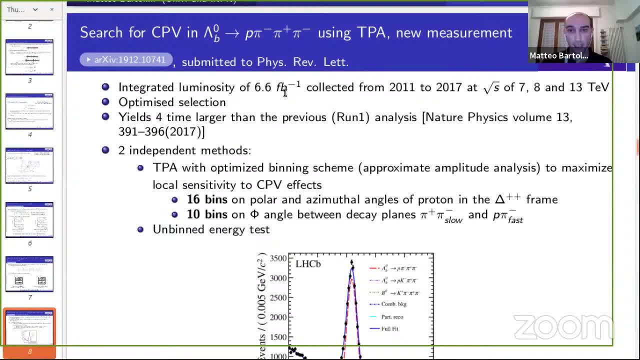 was recently updated by adding also run 2 of a sets corresponding to the luminosity of 6.6 inverse femtoburn. Also, an optimized selection was used, which led to which is 4 times larger than the previous analysis. 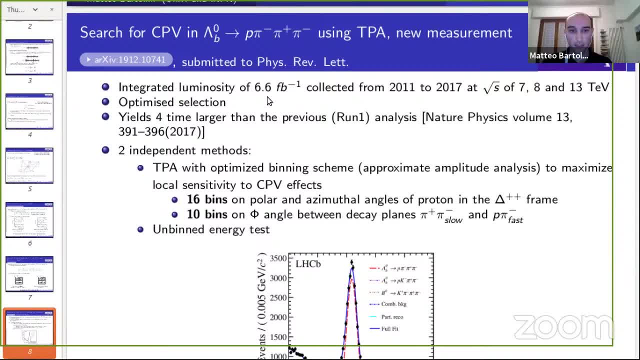 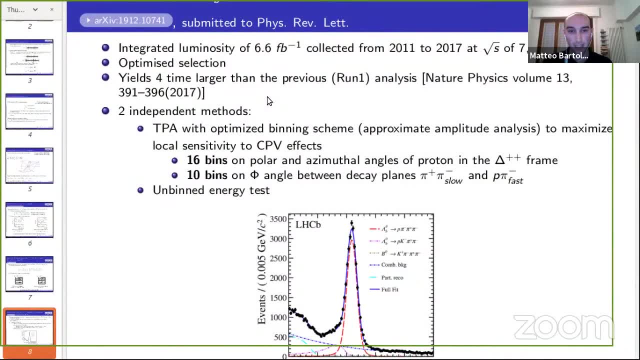 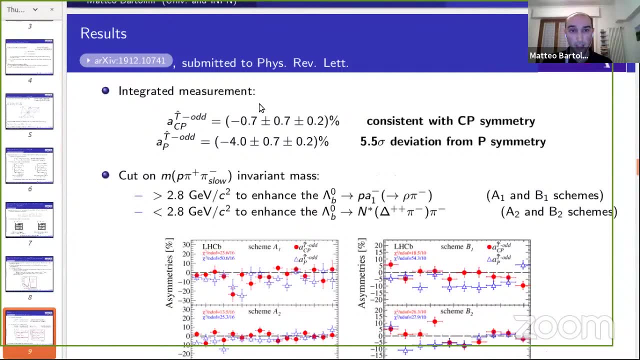 Two methods have been used: the standard, typical parallel asymmetries and with optimized binning scheme and also an ambient energy test. So going to the moving to the results for the phase-based intermediate asymmetries, we see that for the CP asymmetries, 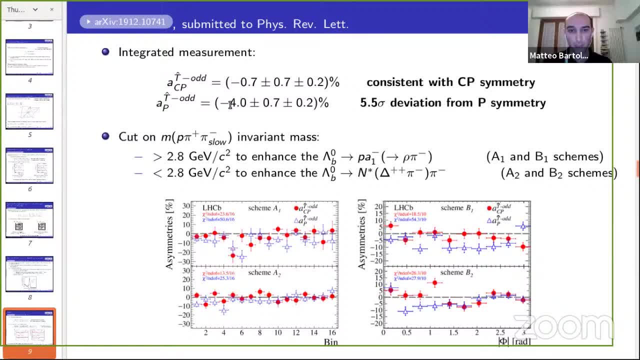 it is consistent with zero. but for the but we see a difference, or we see a deviation of the 5.5 sigma level for the peak symmetry And whereas for the symmetries in the, in the specific equations of the phase space. 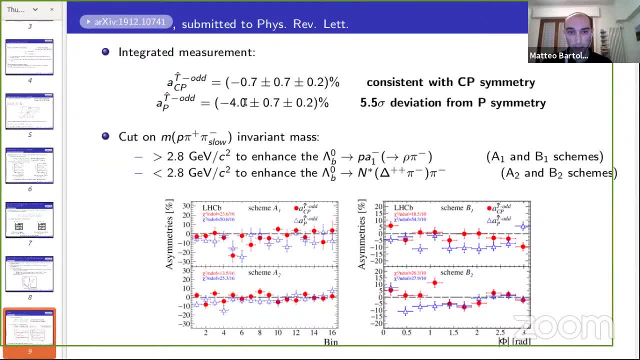 the scheme A and B previously defined were also, in this case, were separated by a cut on the on the environment-mass combination to enhance these particular contributions, And what we see here is that we see also no evidence for CV violation. 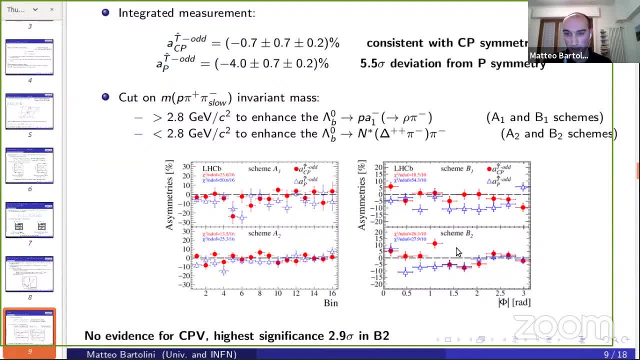 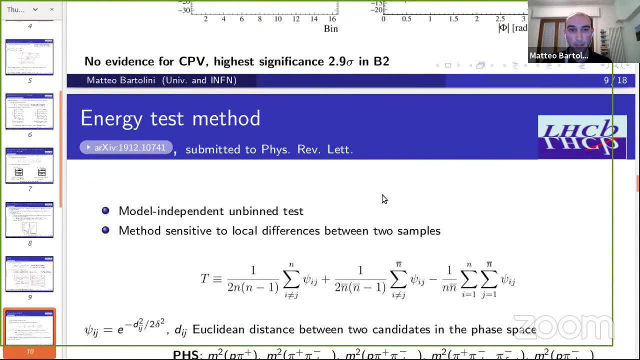 where the high significance is reached in this, let's say, in this scheme- scheme B2,, where the high significance is 2.9, and it which is slightly reduced with respect to the previous analysis. Now, complementary method. 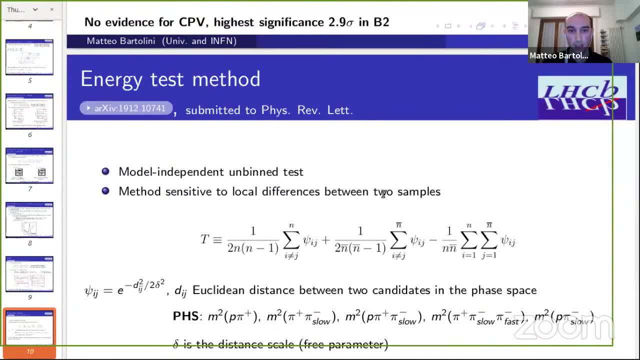 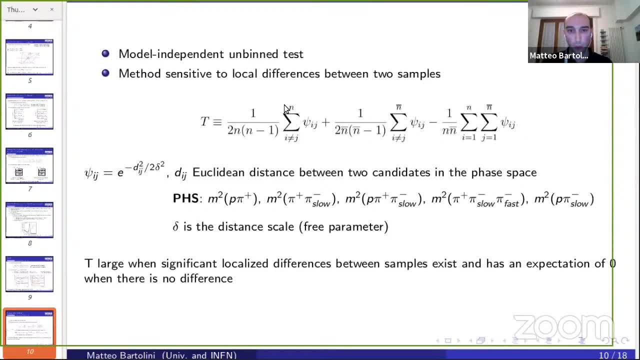 is known as energy test method, which is, let's say, a model-independent approach and is massively sensitive to local differences between two samples, And the test is defined here. where this psi is is defined as follows: where d is the 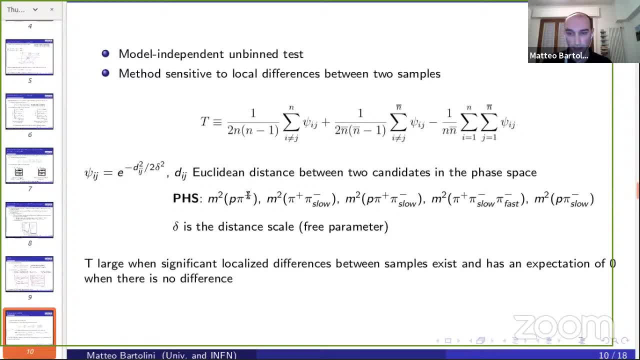 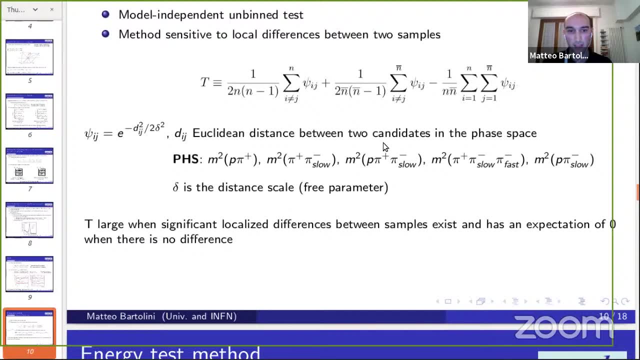 distance between two candidates in the phase space defined by the combinations of by these coordinates in the phase space. Delta is a distance in scale in the in the phase space and is treated as a few parameters. 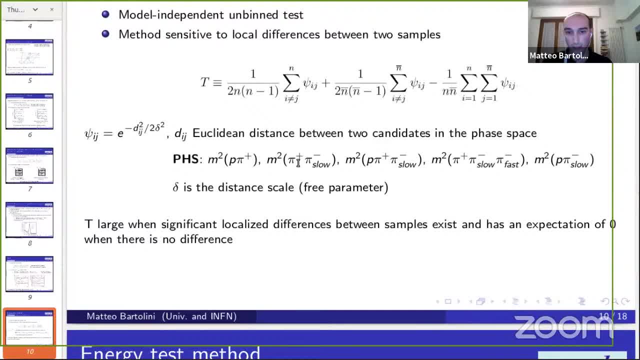 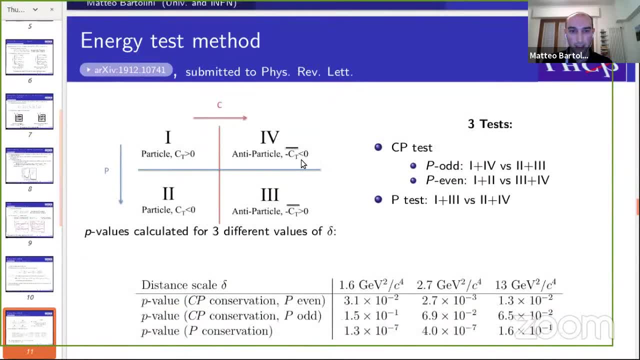 So d is large when there is a significant localized differences between two samples. So, going to results, what? what was done is that the sample was divided into four sub-samples, which are linked to each other according to the. 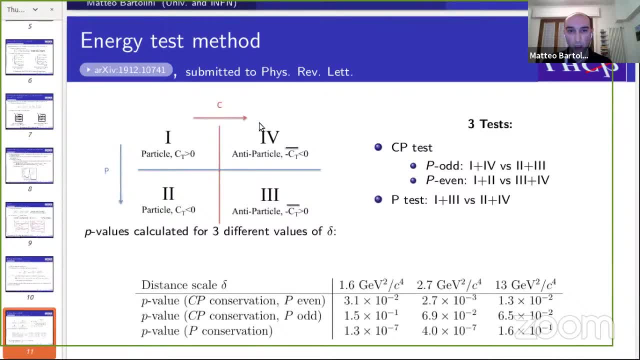 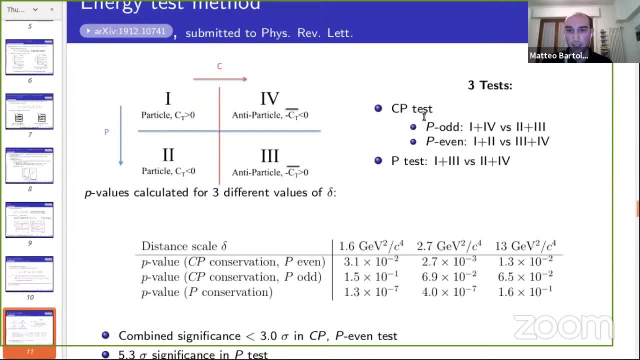 following P and C transformation And and the four, one can say do three tests, Cp. P of the test by combining the one and the four sub-sample and also the two and three as the second sample. 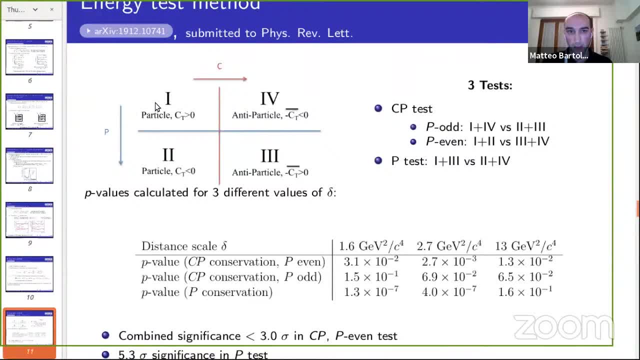 Cp: P of the test, when the first sample is done by by adding one and two and three and four, And a P test where, where the first sample is obtained by adding one and three and two and four. 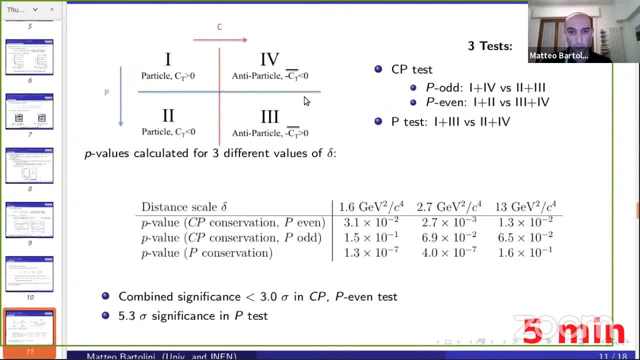 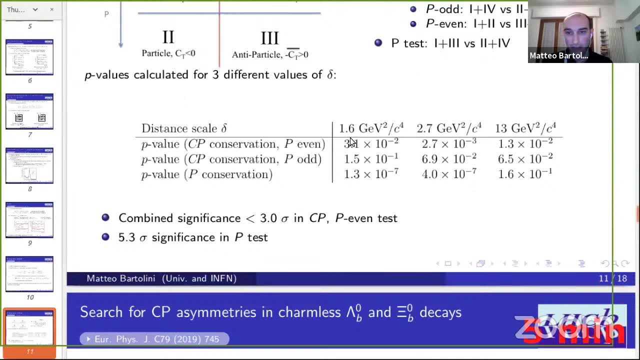 And the results show. it was calculated for three different values of the of this delta And results shows that we have the highest significance in the Cp given tests, but the combined significance is less than three sigma, whereas for the. 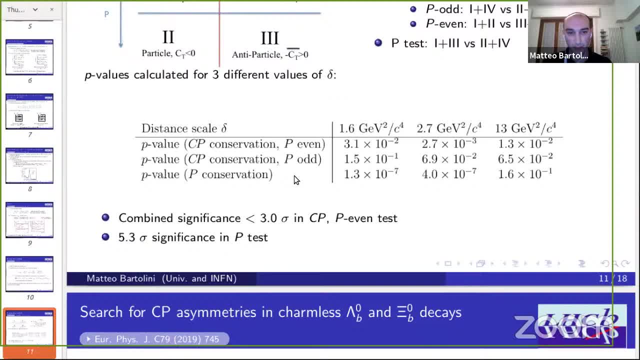 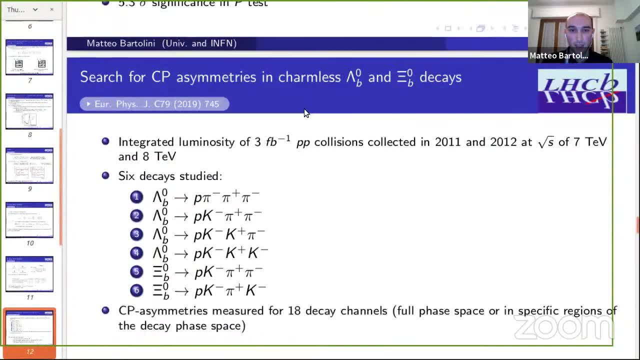 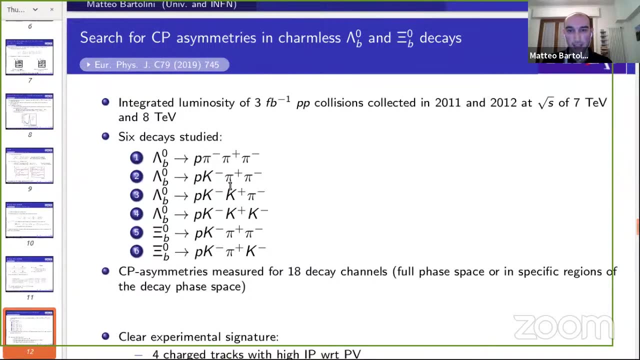 P test, we see a 5.3 sigma deviation from the P symmetry. And okay, now the search for Cp violation was also performed in these channels, but by using the, the standard Cp. 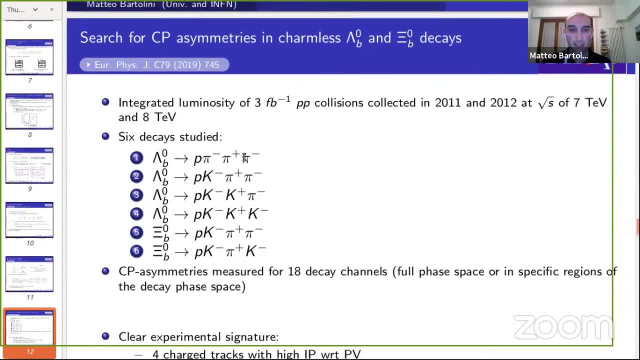 asymmetries, and so the data sample also corresponds to three inverse van-to-varn collisions collected in 2011 and 2012.. And the so these are the cases that have been studied. 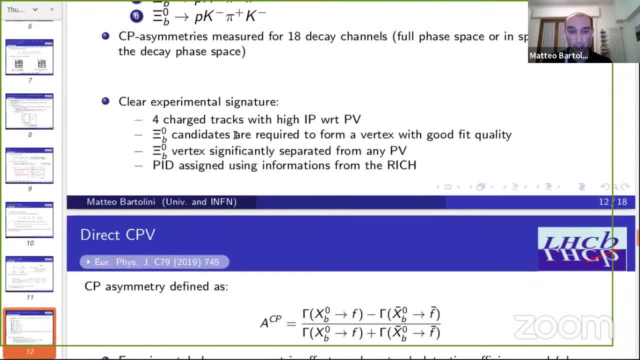 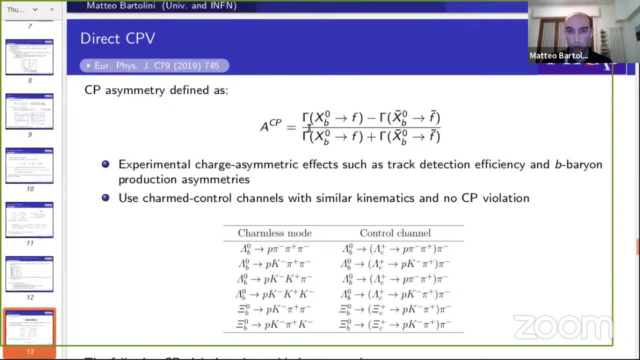 And okay, and the the method is the direct Cp asymmetries, which which is as far as you are familiar with and, but this is, this is a symmetry which can be say affected by. 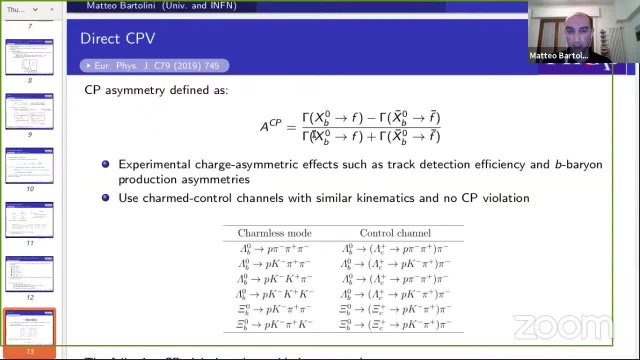 track detection efficiencies and the atom production asymmetries And therefore, in order to get rid of it, we use, we use the, the we use what we use, what they use is is a control. 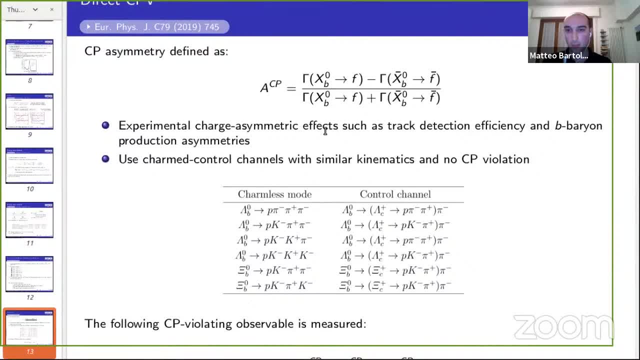 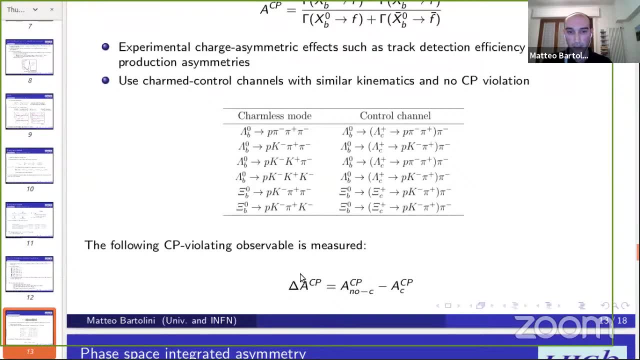 a channel, a control channel, with similar kinematics and no speculation expected in the standard models, And so one measures the. so the following Cp asymmetries, two Cp asymmetries where the fake Cp asymmetries. 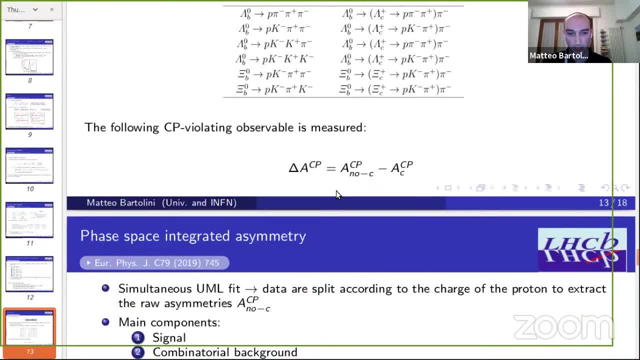 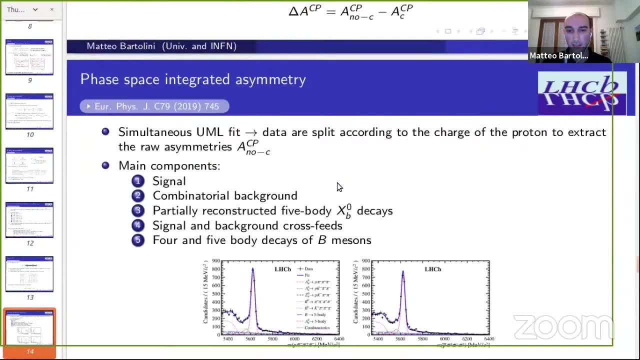 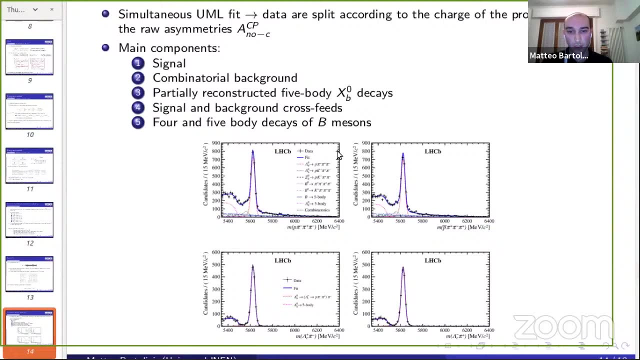 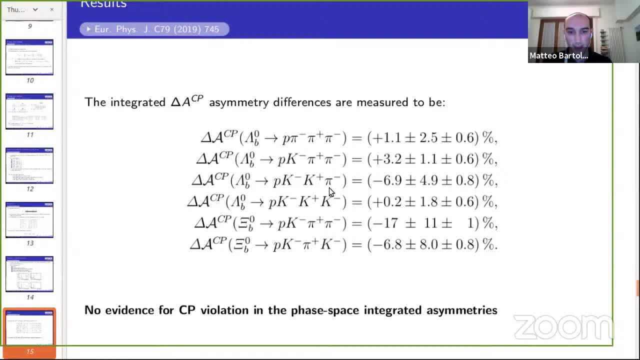 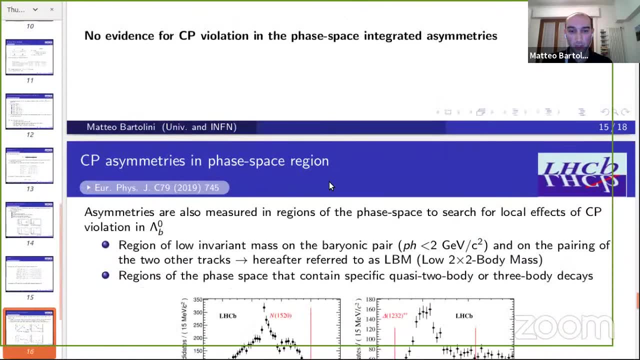 Now adding up to So the Cp, Cp, Cm, Cp, Metateful Results are: are they minor? because it is, rather it is below Cp, but it is a minor that gives us the, the, the. 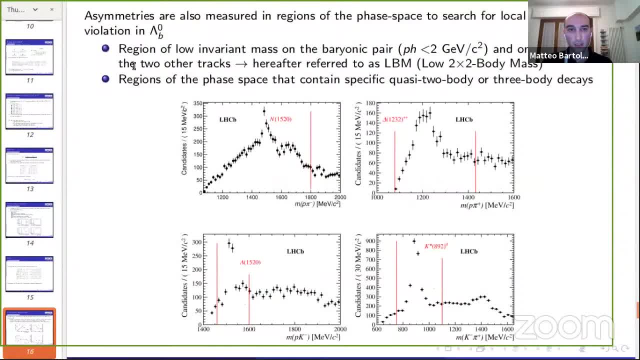 the Cp and mainly uh. two regions were defined are regions of the low environment mass and the baryonic pair, where the where we place a cut on this combination of problems and mesons, and also in the specific regions of the phase space that contain quasi two body or 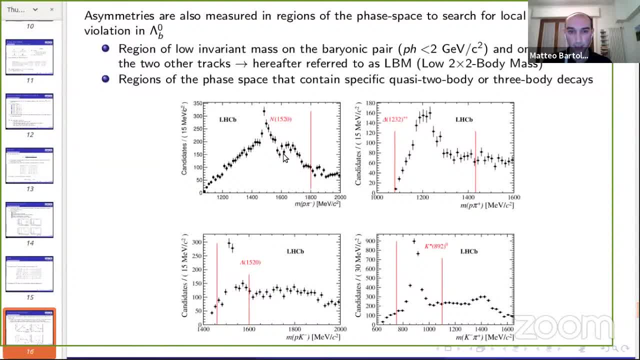 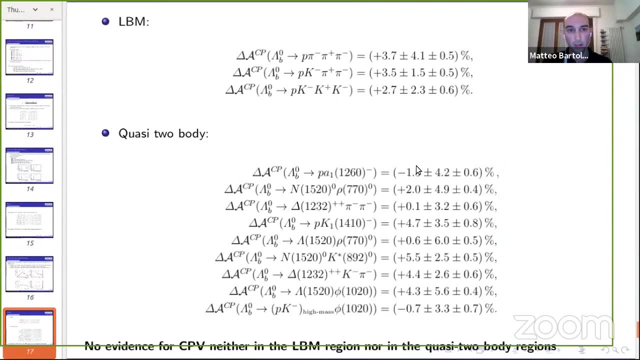 three body decays. now you see here the assuated distributions of the of some combination of environment masses and you can see the resonance is well known resonances and the results also for the, both for the low body mass regions and the positive body region. leads shows that there is liabilities neither for the lower body mass regions. 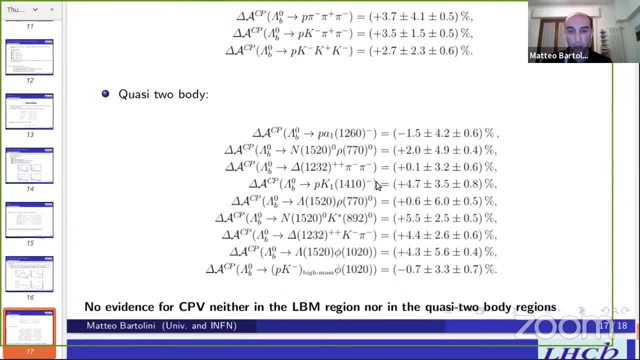 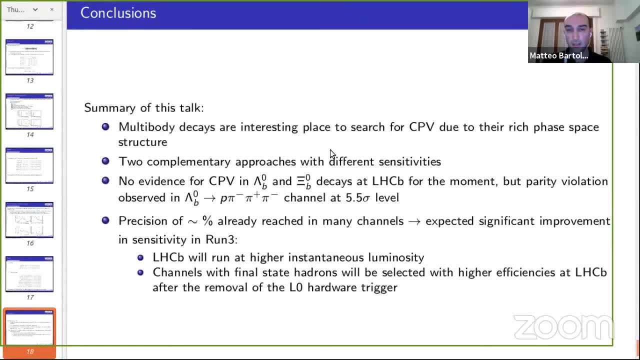 and in the positive body regions. this brings me to the conclusions of this talk, where i've shown you that the multivariately case is a very interesting place to search for situation due to the the fact that they have a rich phase-based structures. um, so for the moment, we have no evidence for civilization in both in. 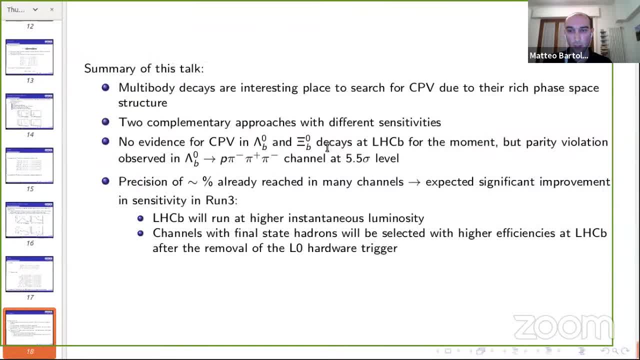 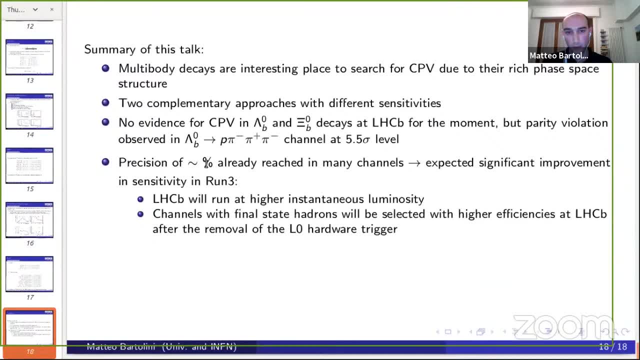 lambda b anxiety decays, but uh, cp violation was found in this particular decays at 5.5 cinema level. what, what is interesting to note, is that we we already reached a precision of few percents in many, many channels and a significant improvement is expected for one, three, because, uh, actually we 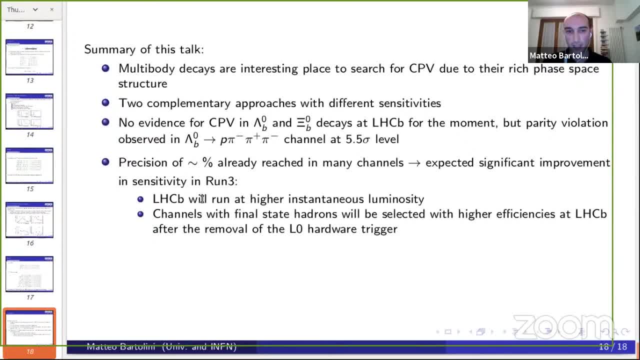 run out much uh high luminosities and also because, uh, in particular, the channels with finite state hydrants will benefit a lot from the removal of the zero arbor trigger. so that's all and thank you very much for your attentions. thank you, mateo. any questions? 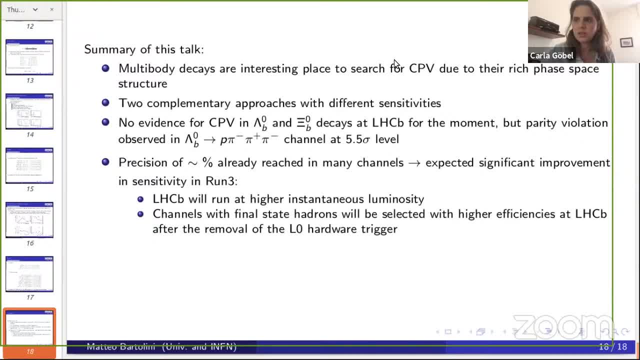 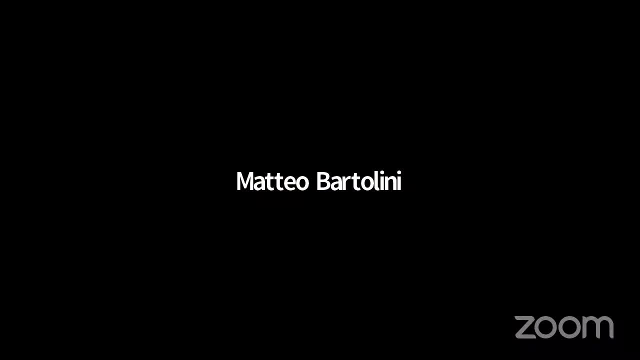 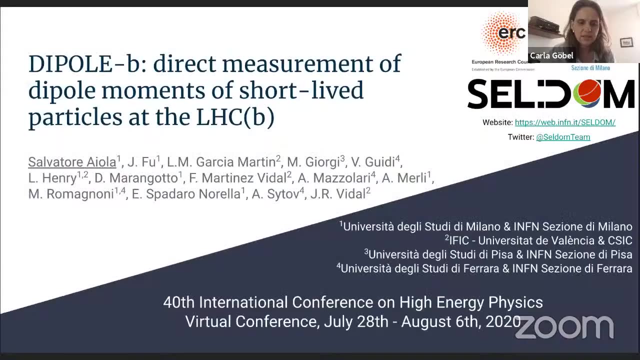 okay, you don't see any. so we finished the cp violation block and we move to our last talk of this block and of the session with uh, salvatore ayola on the dipole beam experiment. hello, can you hear me? well, yes, okay, do you see this link? 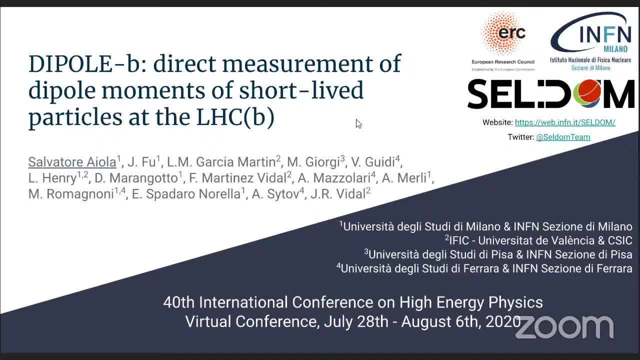 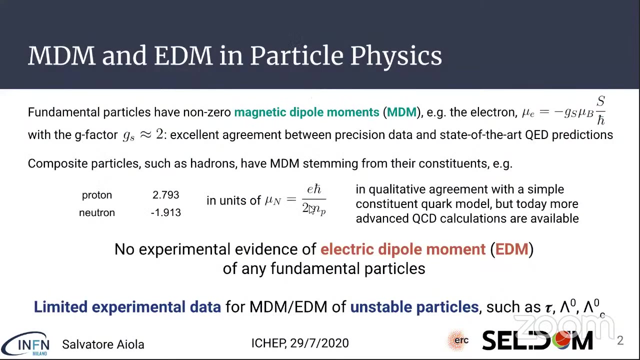 slides: yes, okay, um so good evening everybody. i present today the that will be project, which is a project aiming at measuring, measuring the diaper moments of electromagnetic moments of short-lived particle at the lhc. um so first just a quick introduction about the electromagnetic double moments in particle physics. 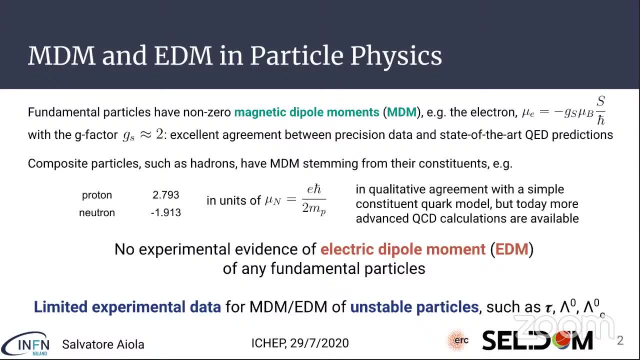 we know that all fundamental particles have non-zero magnetic double moments. well, most, not all, there are from the particles with non-zero many double moments, for example the electron and and all most of the particles that we know of, composite particles such as hadrons, have a magnetic development that is stemming from their constituents. 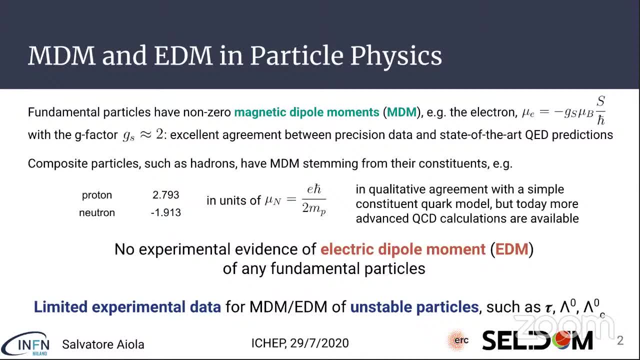 and, for example, for the proton and neutron. the values that we have from the theory are in qualitative agreement with the experimental measurements. however, we have no experimental evidence of electric double moment of any fundamental particle and we also have a limited experimental data for electromagnetic moments of unstable particles such as the tau, the lambda zero and the lambda c. 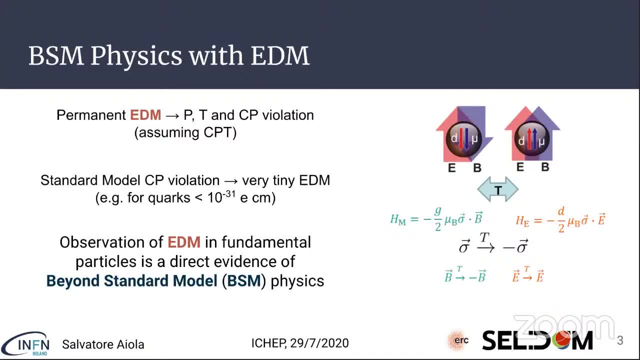 um, so why there is no electromagnetic moment in fundamental particle. this is due to the fact that the permanent edm violates both parity and time reversal symmetry and assuming that the cpt theorem holds, this means that the permanent dm violates also cp um. this can the according, since we know that there is a cp violation standard model. 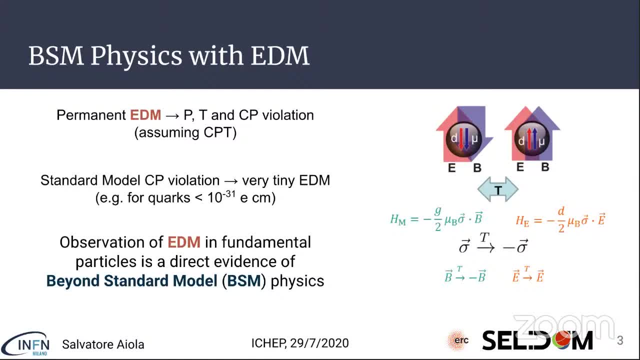 This allows for a very tiny electromagnetic dipole moment, but this is so small that it's very far away from what we can experimentally probe. So if we do see an electromagnetic dipole moment in any fundamental particle, this is a direct evidence of beyond standard model physics. 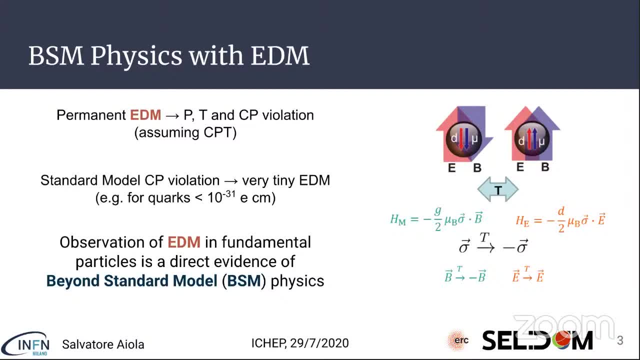 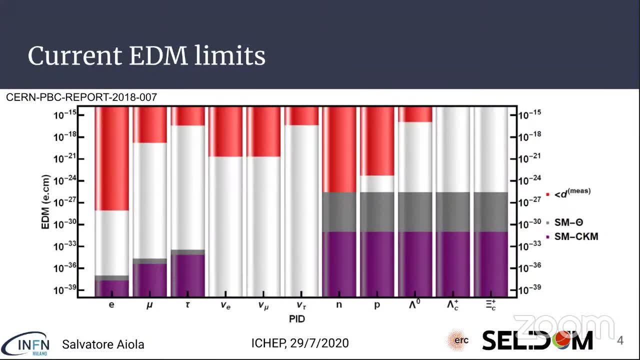 because it requires additional city violation beyond what is in the standard model. So these are the current limits on the electric dipole moments of some of the particles. So the magenta bars from low are the limits coming from the expected values from the standard model. 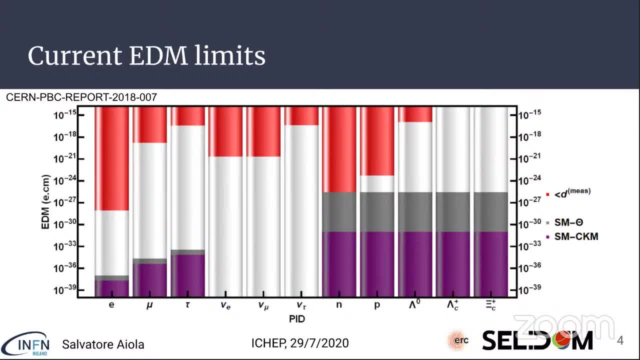 From above the red bars indicates the current experiment. So these are the experimental limits And we see that there is a large gap between the experimental limits and the standard model prediction. So there is a large region for potential discovery. In particular, I'm gonna focus on some unstable particles. 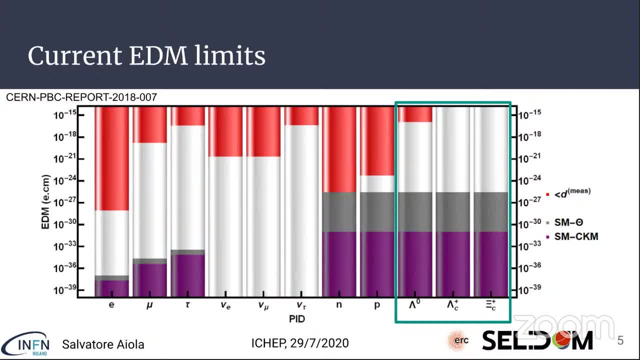 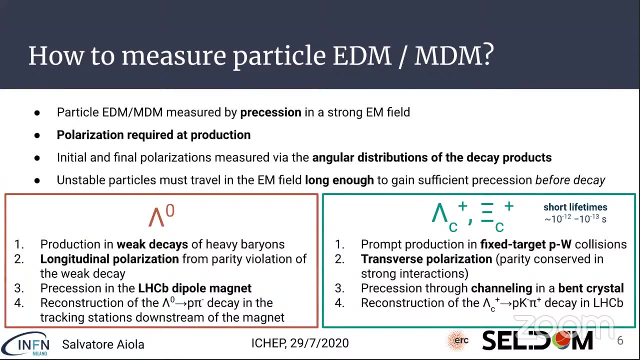 so, particularly the lambda zero and the charm variance, where we see that indeed, the separation between the limits, the experimental limits and the standard model prediction is quite large. So how do we measure a particle electromagnetic dipole moments? We do this by measuring the precession of the particle. 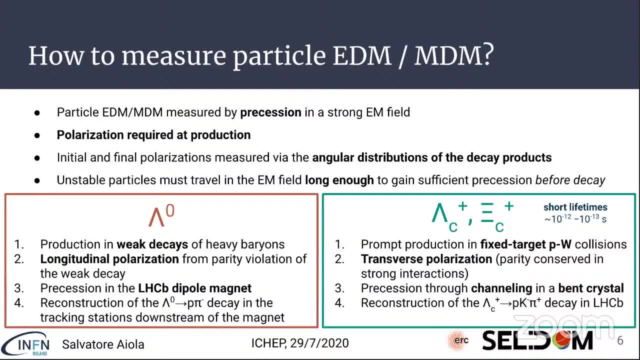 dipole moments in a strong electromagnetic field. Of course, in order to observe precession we need to have polarized beam of particles And we must measure the initial and final polarization, so before and after the precession of the magnetic field. 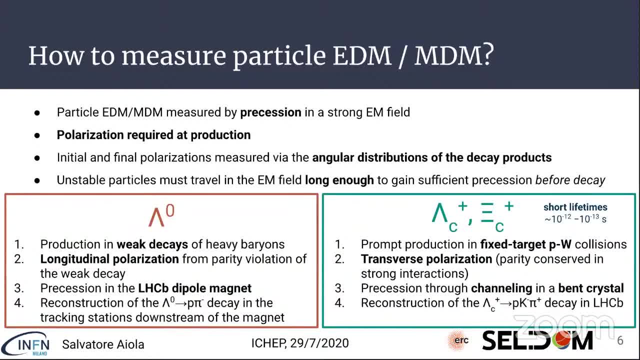 via the angular distribution of the decay products, since these are unstable particles. The tricky part of this measurement is that, since these are unstable particles, they must travel in the electromagnetic field long enough to gain a sufficient precession before decaying. So I'm gonna talk about two different measurements that we plan to do. 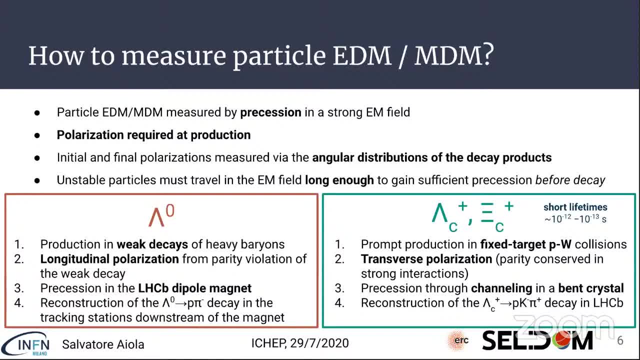 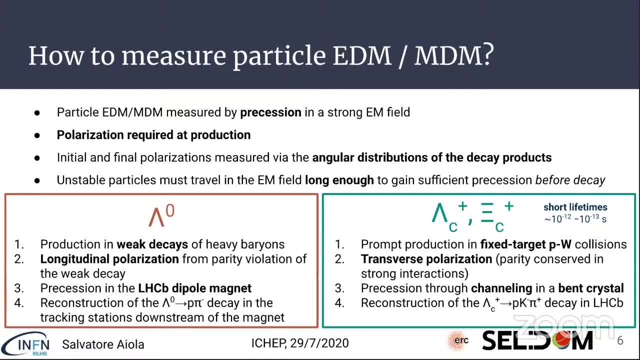 In this case we look for production in weak decays of heavy baryons where the lambda zero is produced with the longitudinal polarization because of the relation of the decay. Then we will look for precession in the LHCb dipole magnet. 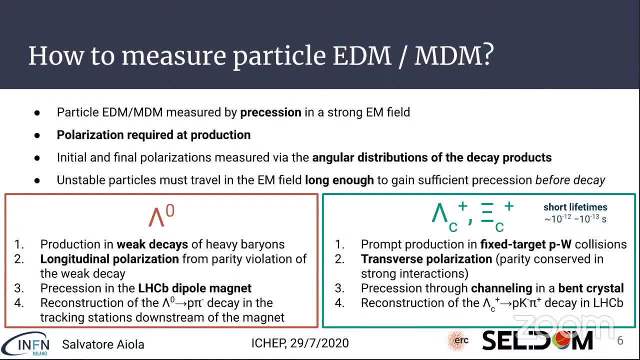 And we reconstructed the lambda zero, looking at decays that occur after the magnet, before the tracking stations that are placed downstream of the magnet. The second part of the presentation will be related instead to another measurement that aims at measuring the electromagnetic moments of charm baryons. 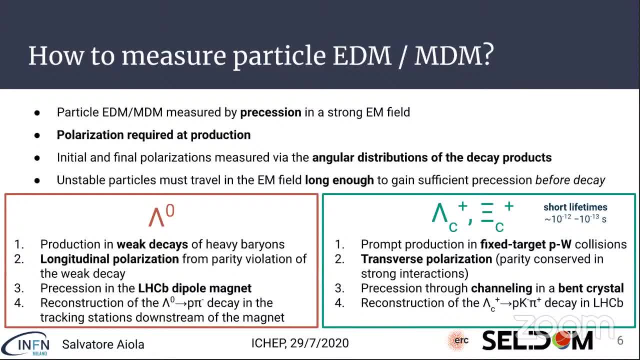 In this case, we will look for charm baryons produced promptly in fixed-target proton tanks. in fixed-target proton tanks: In this case, we will look for charm baryons produced promptly in fixed-target proton tanks. In this case, we will look for charm baryons produced promptly. 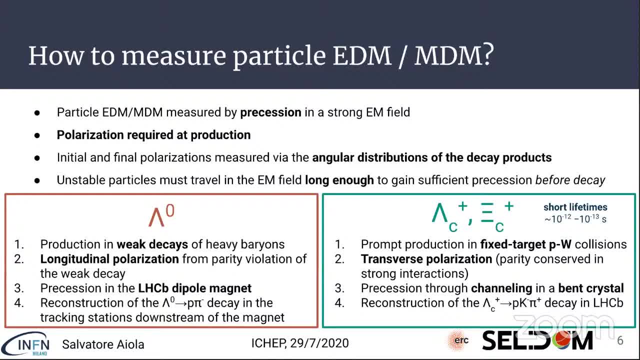 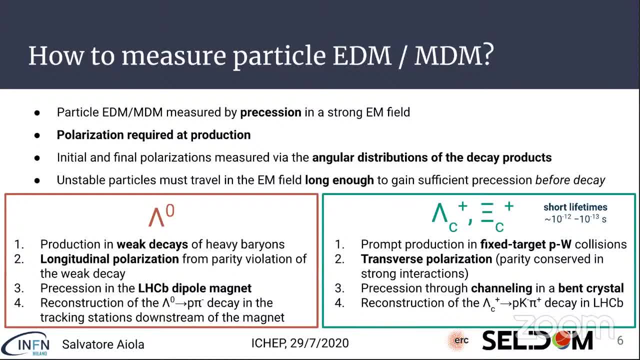 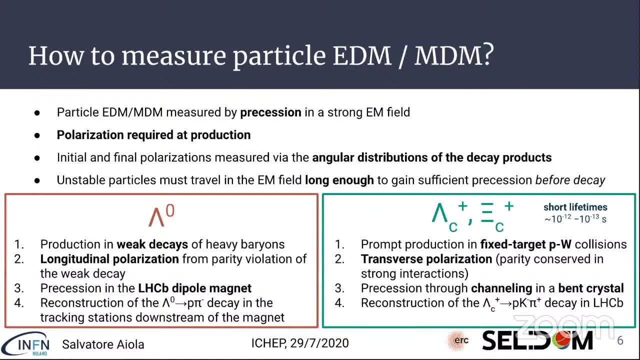 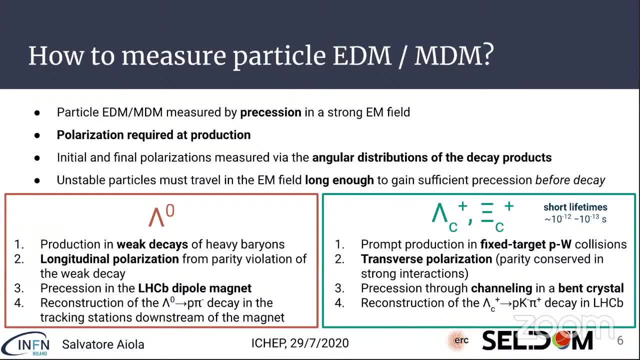 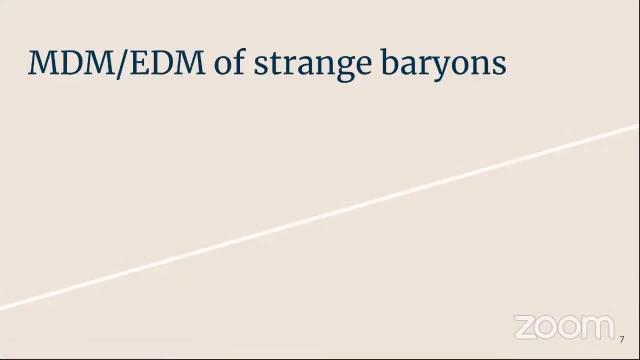 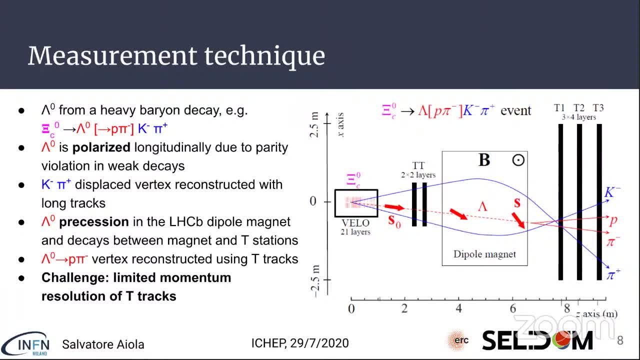 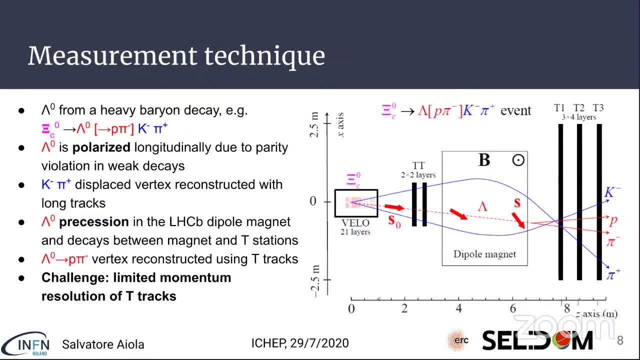 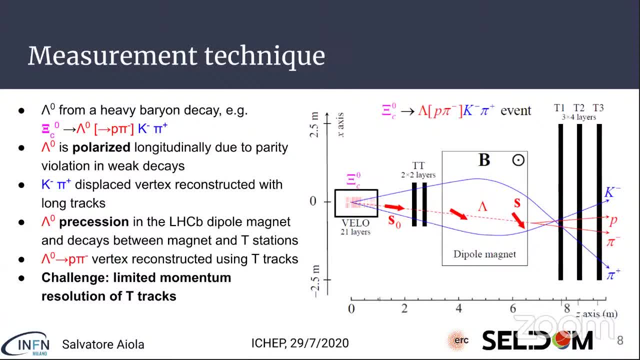 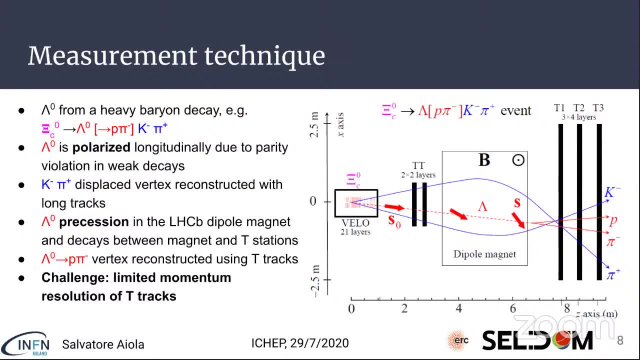 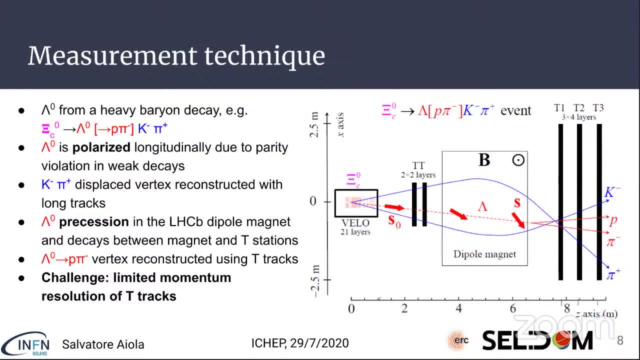 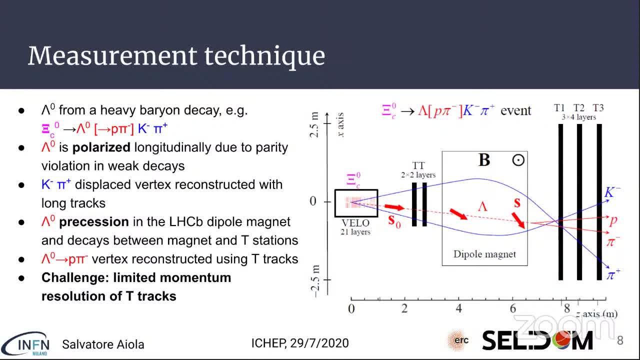 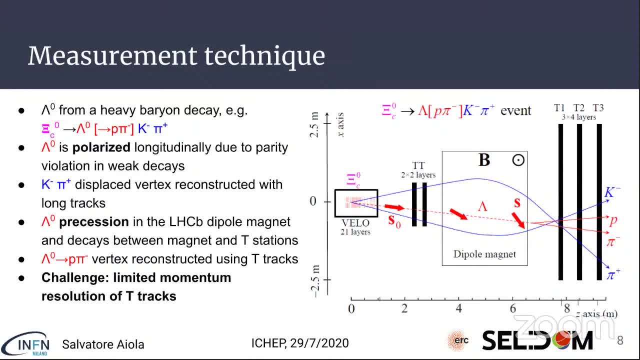 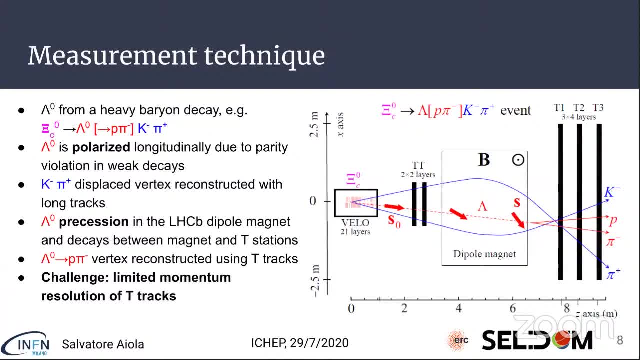 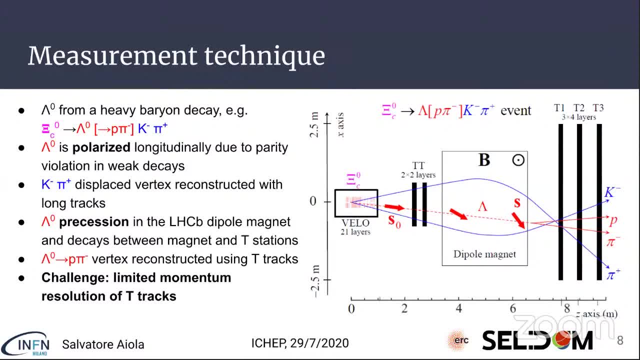 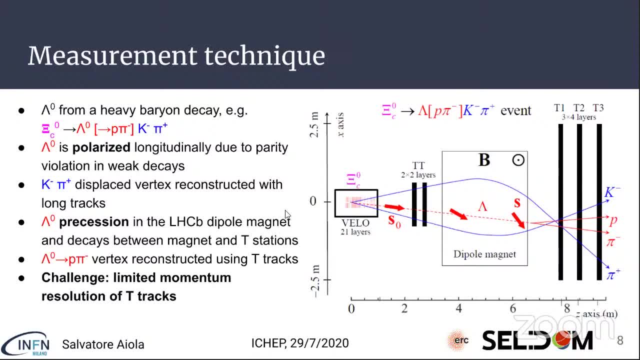 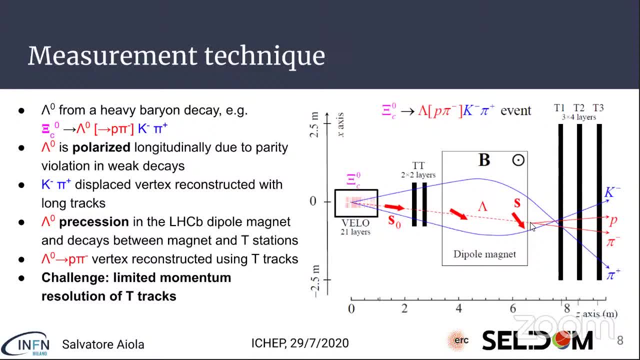 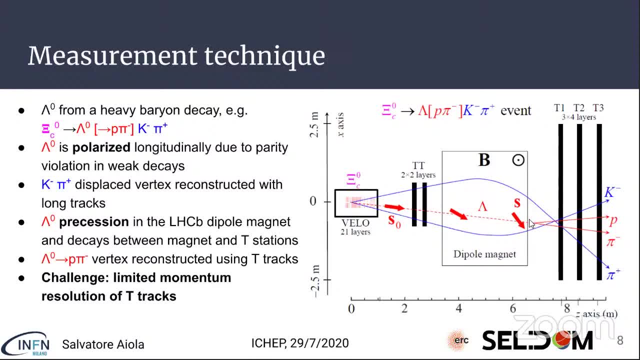 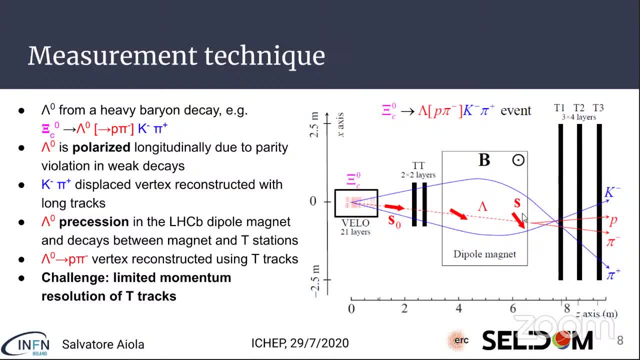 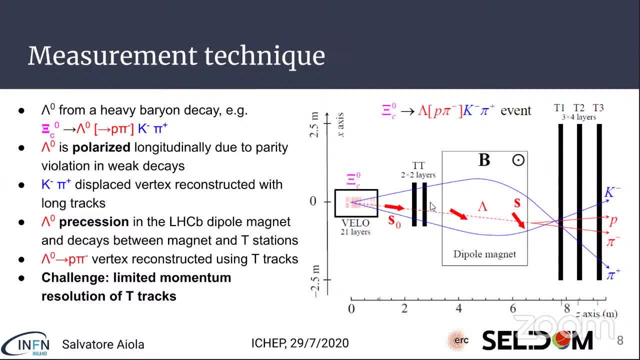 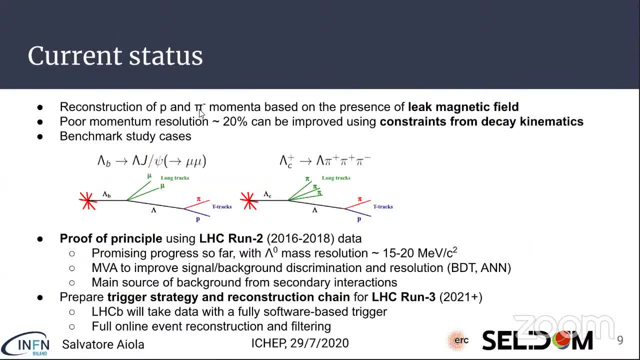 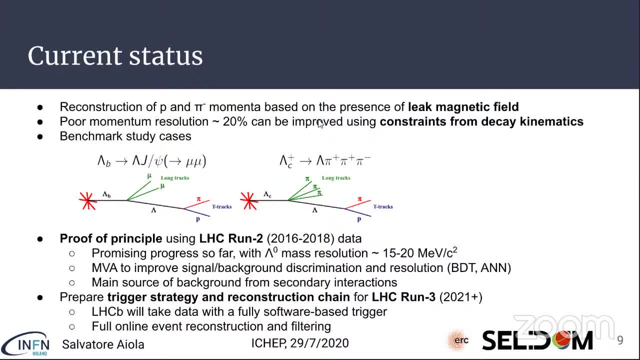 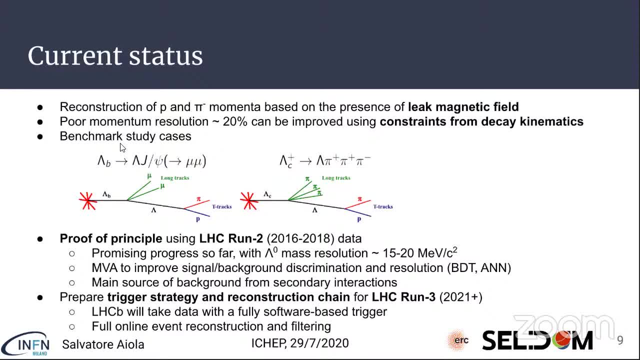 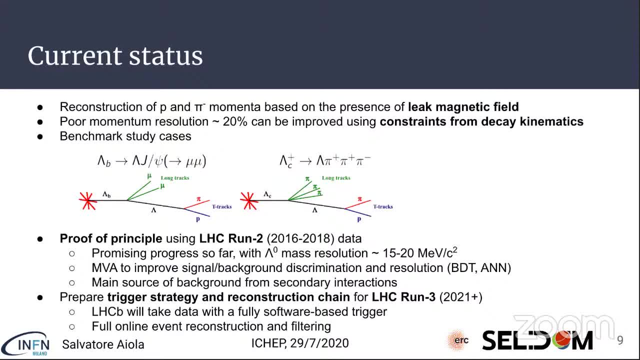 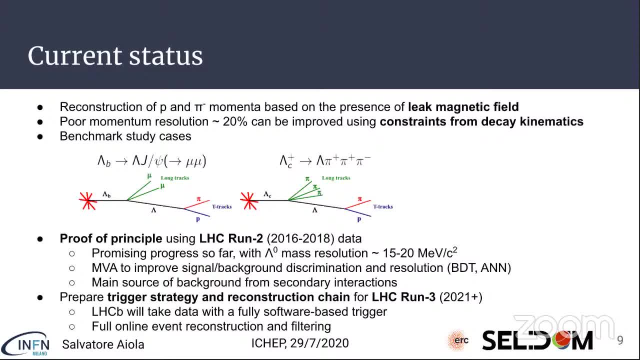 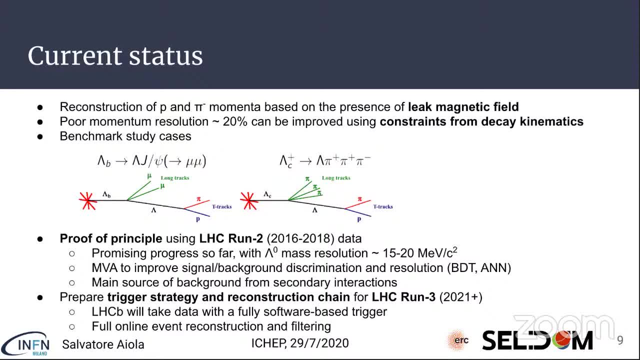 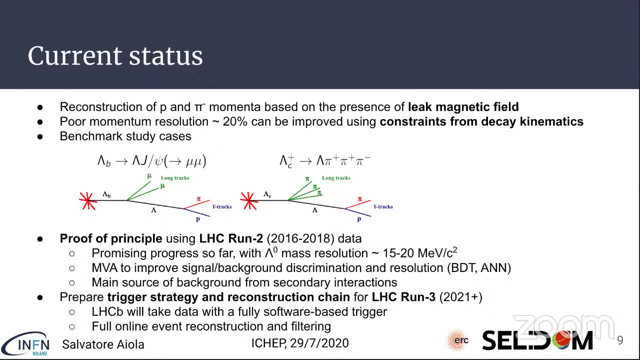 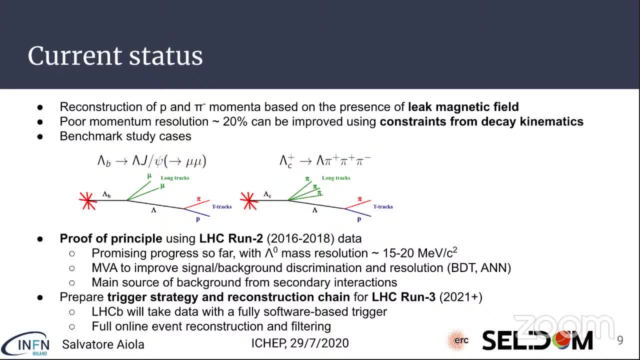 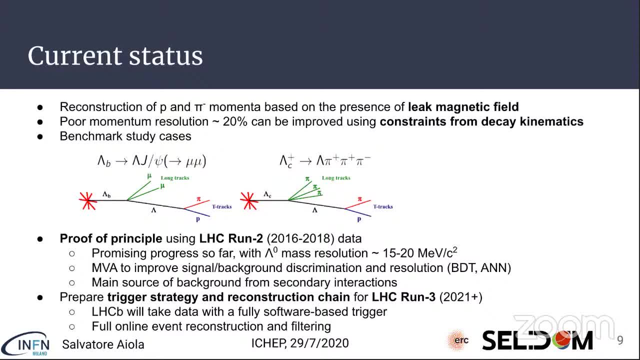 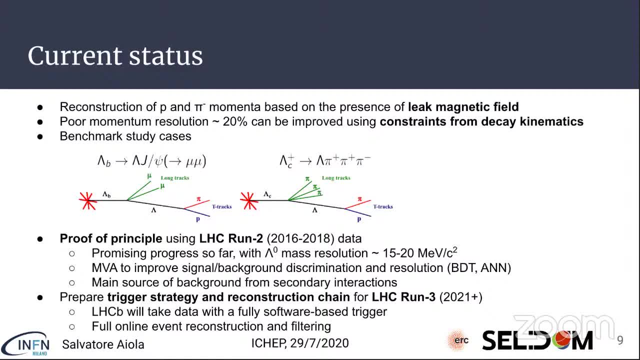 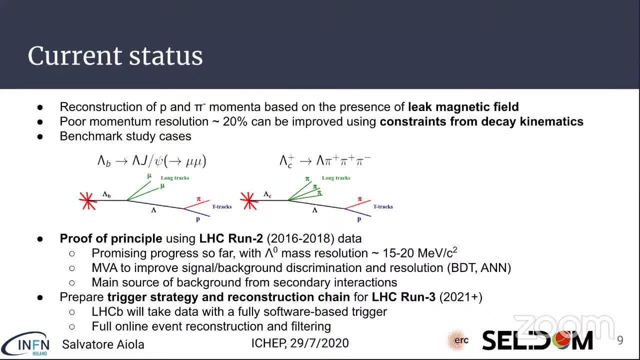 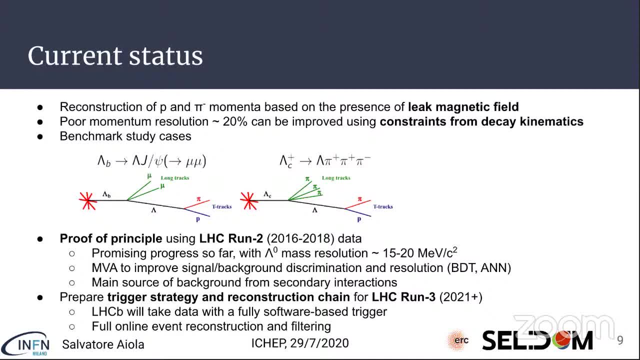 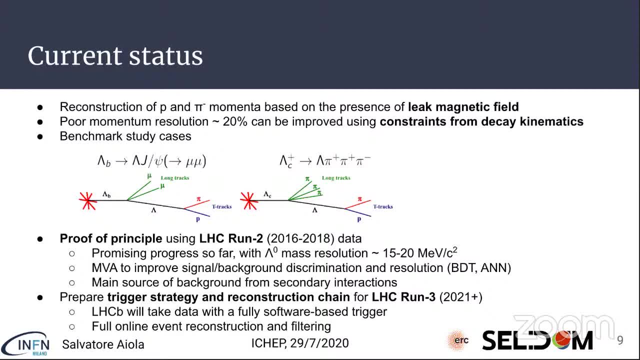 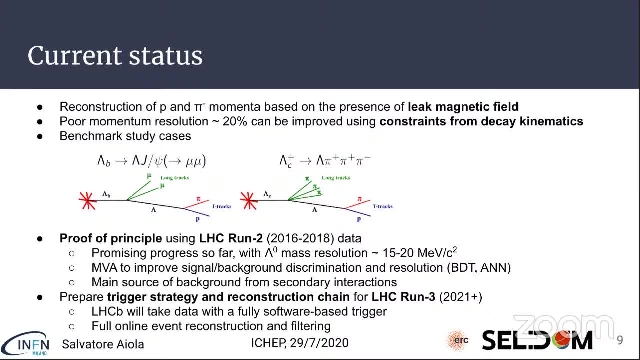 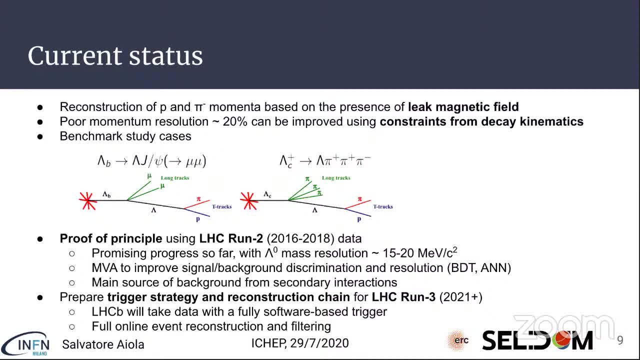 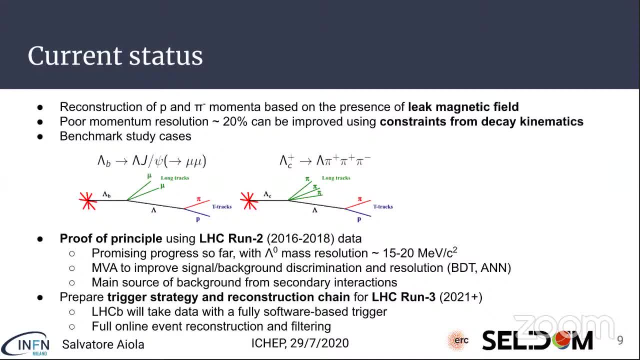 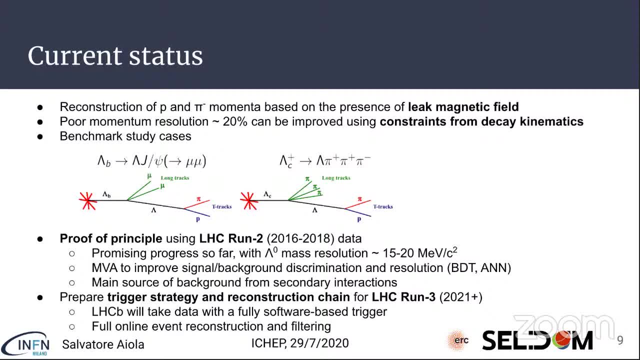 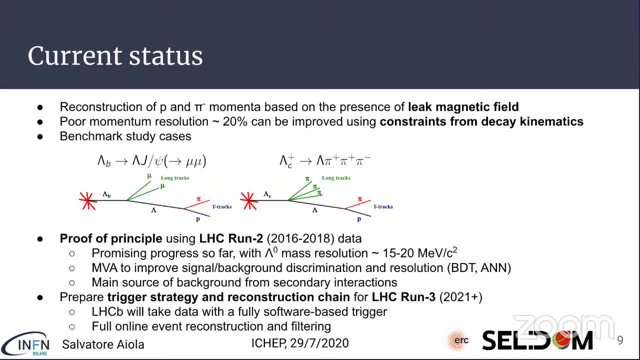 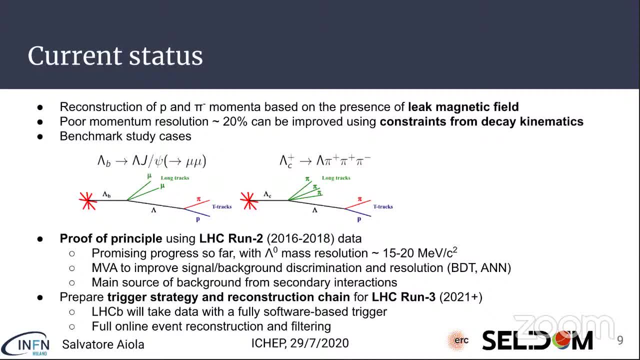 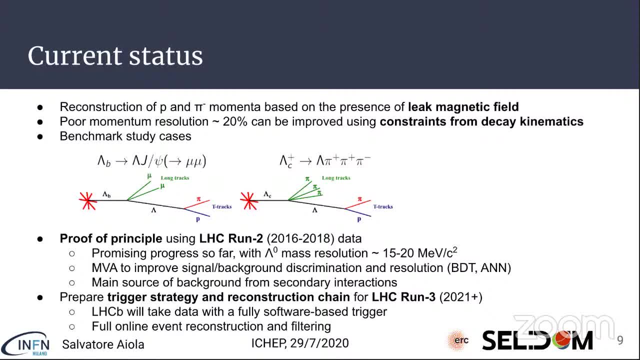 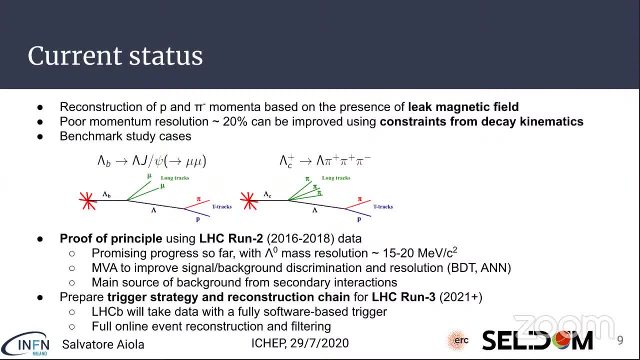 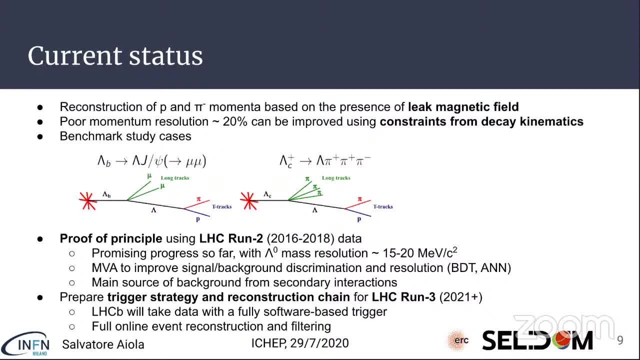 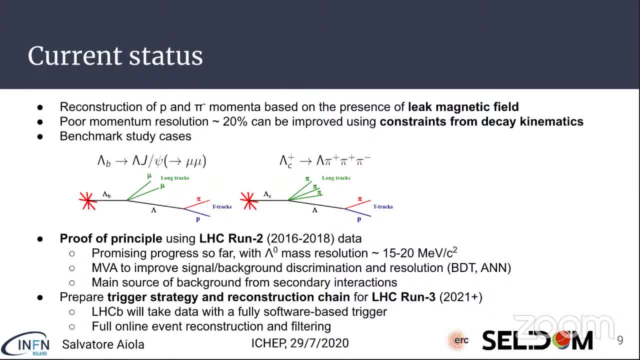 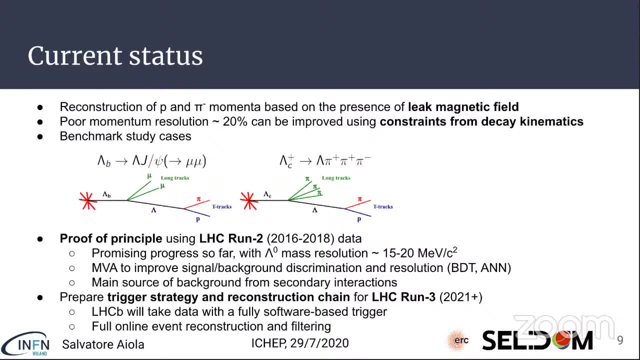 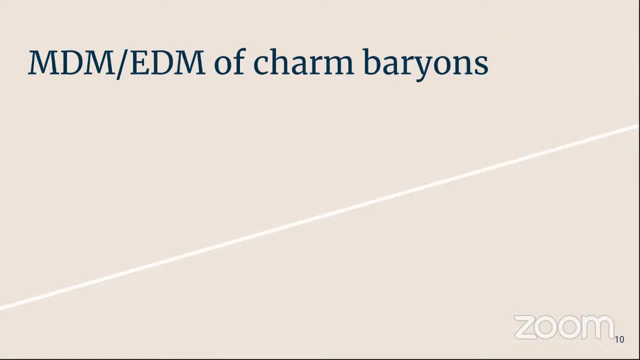 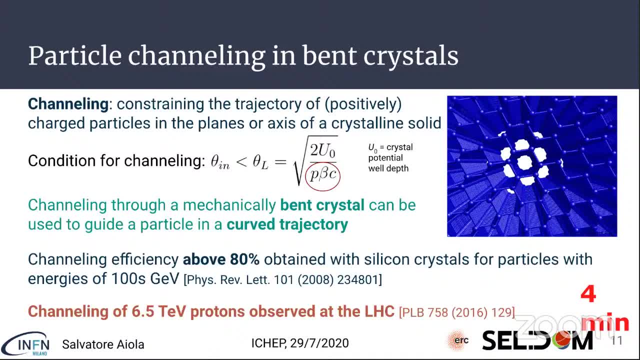 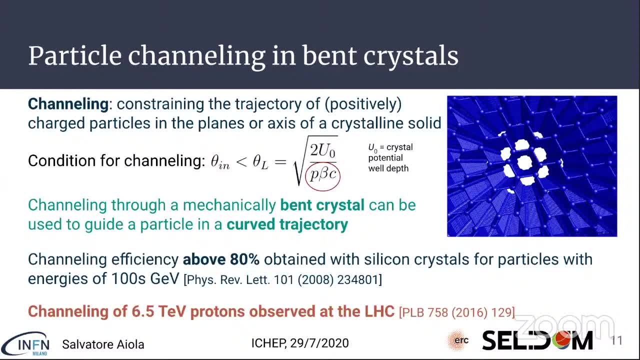 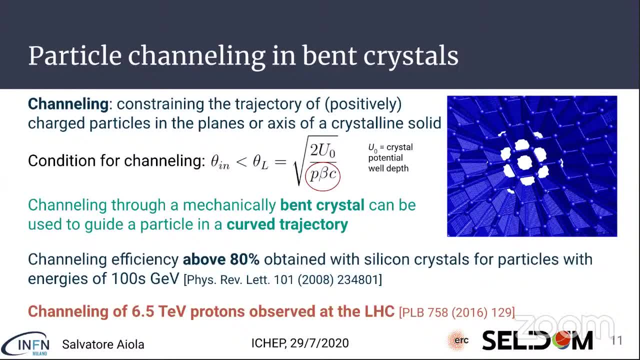 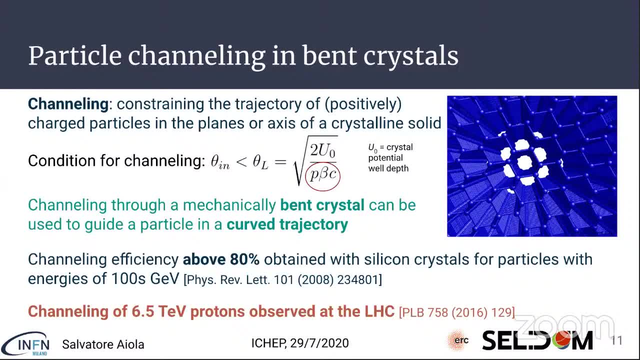 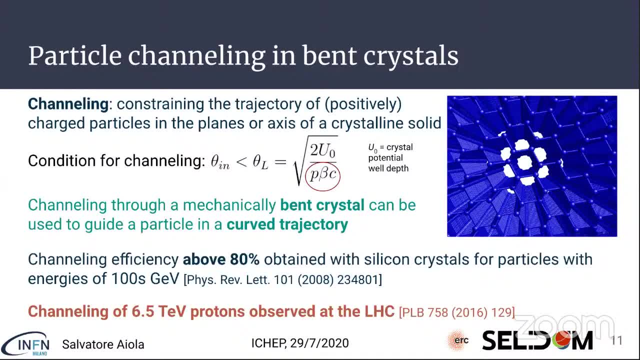 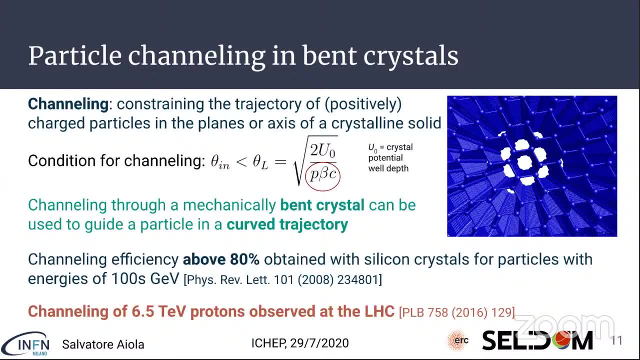 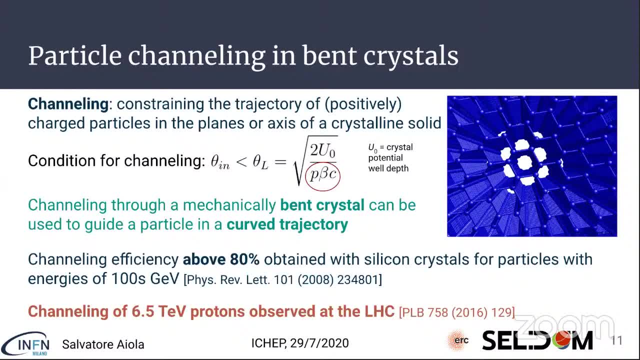 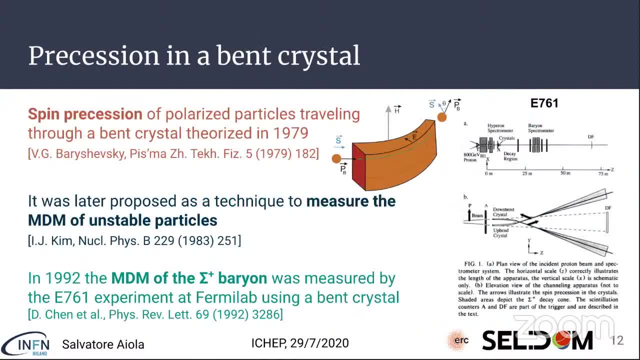 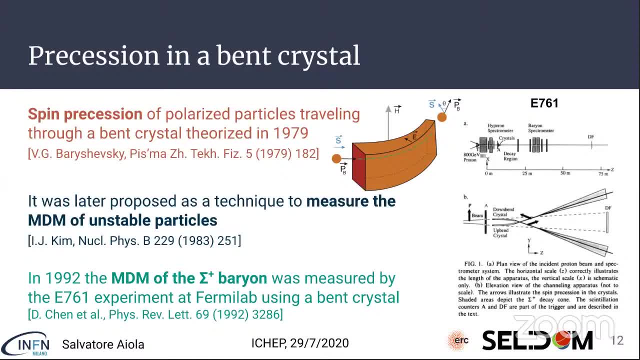 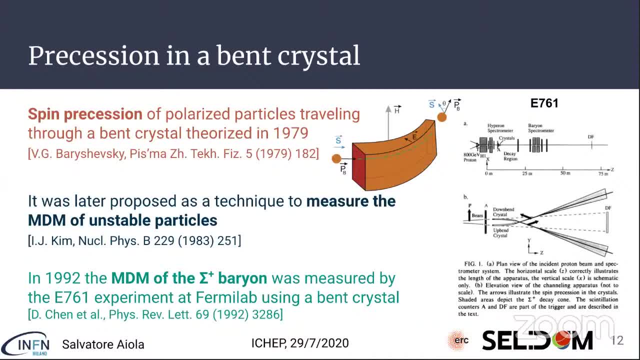 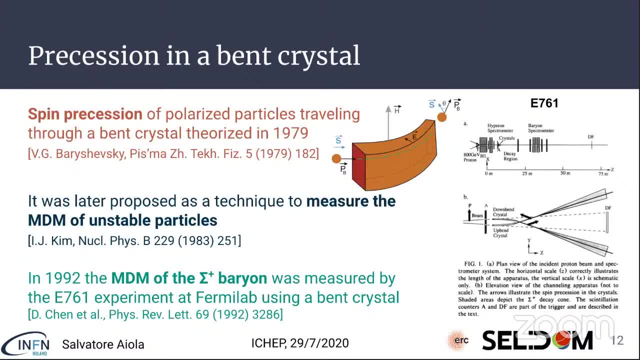 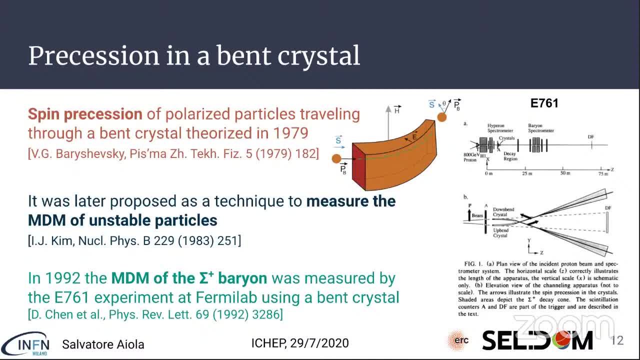 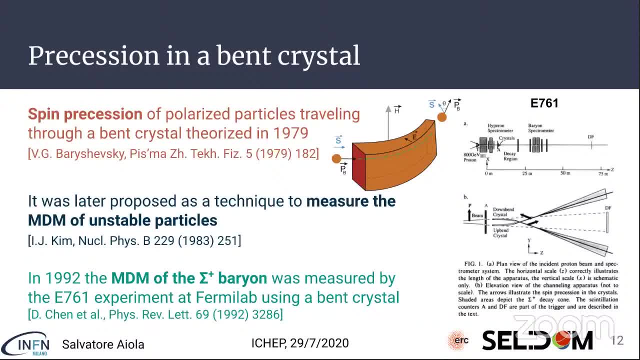 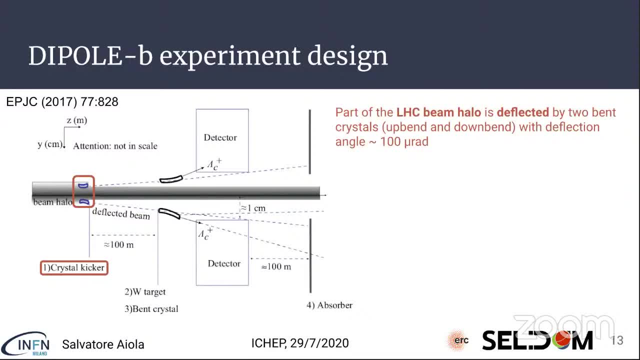 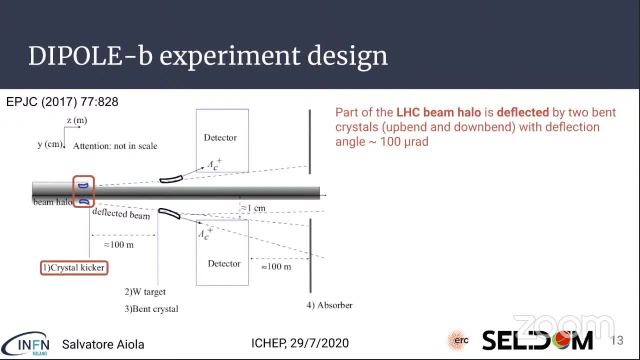 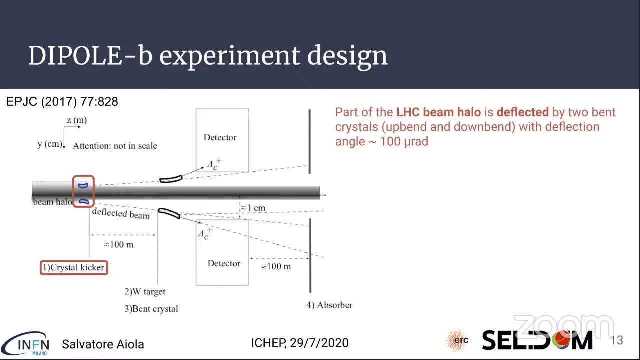 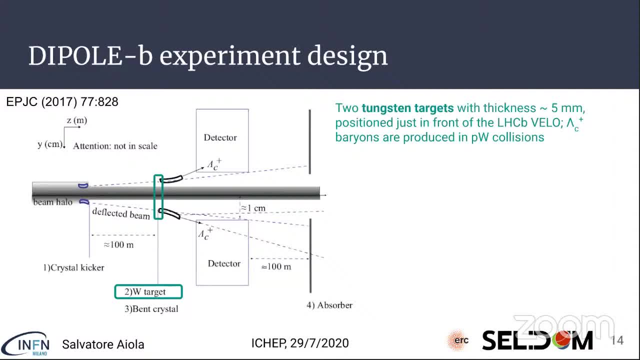 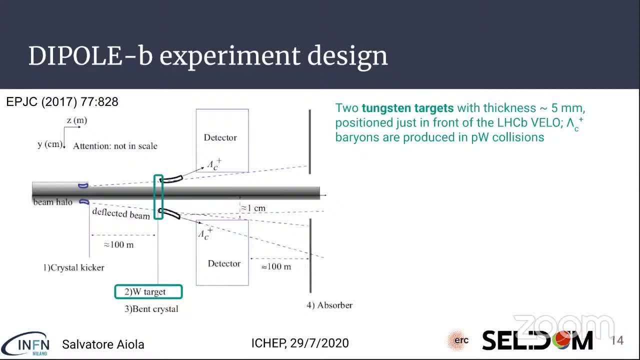 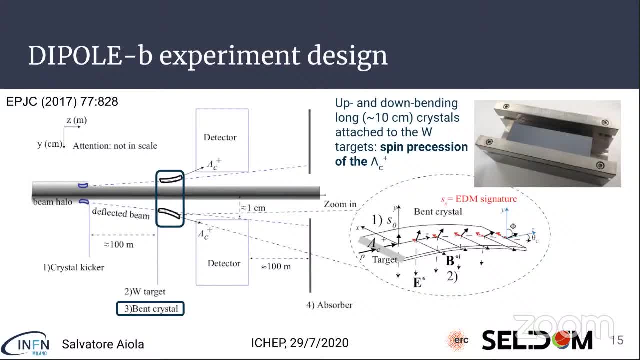 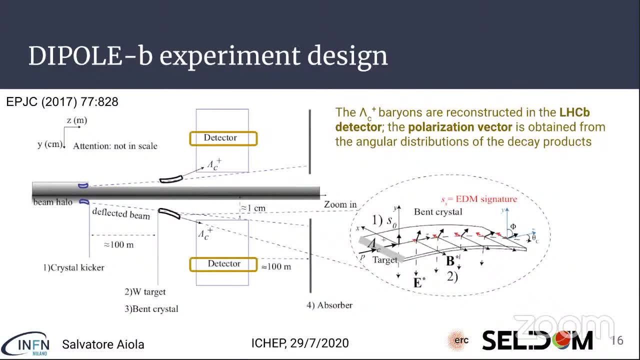 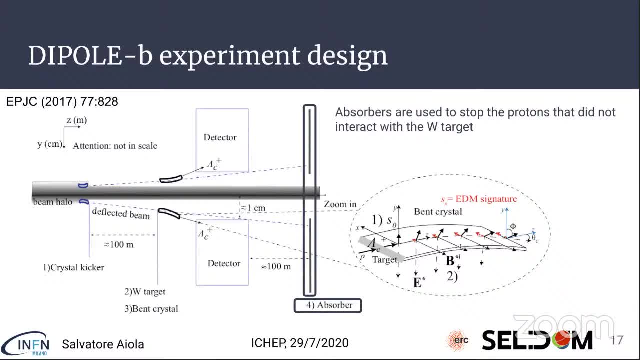 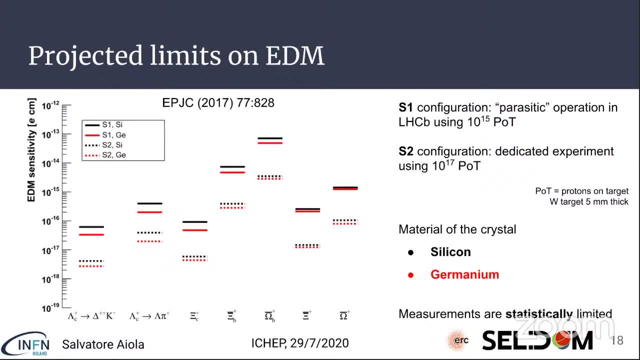 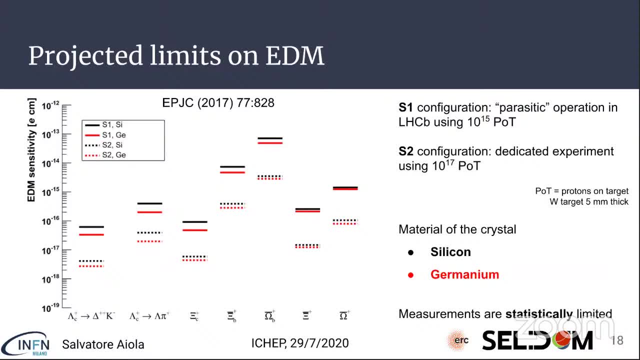 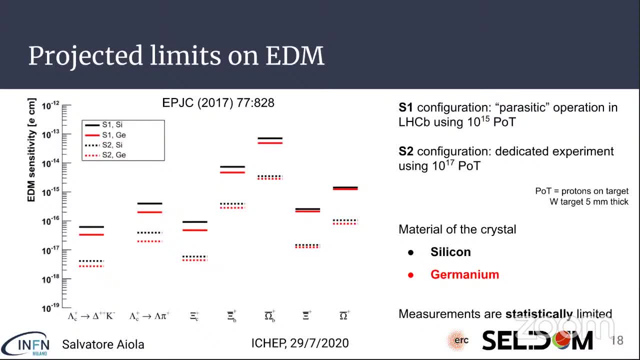 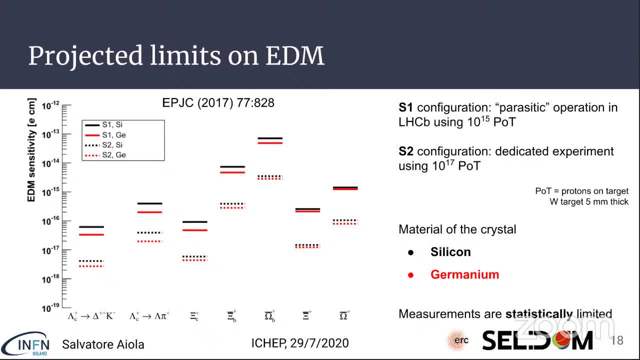 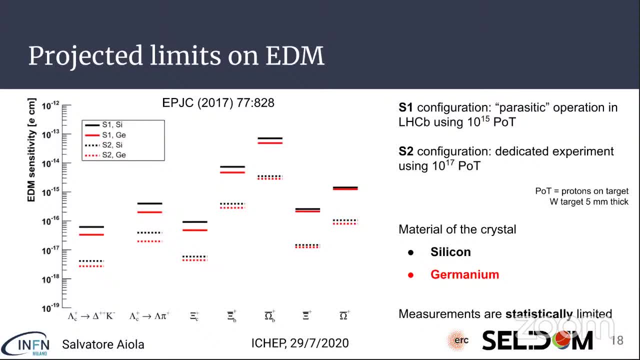 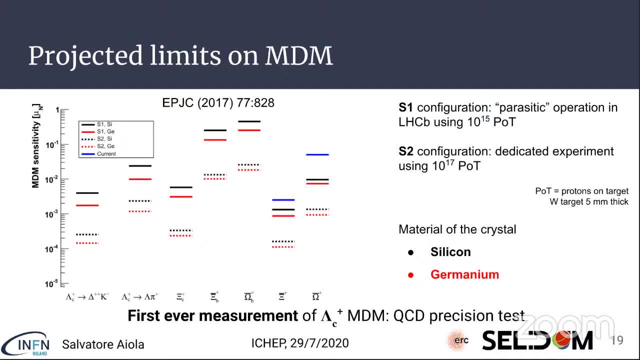 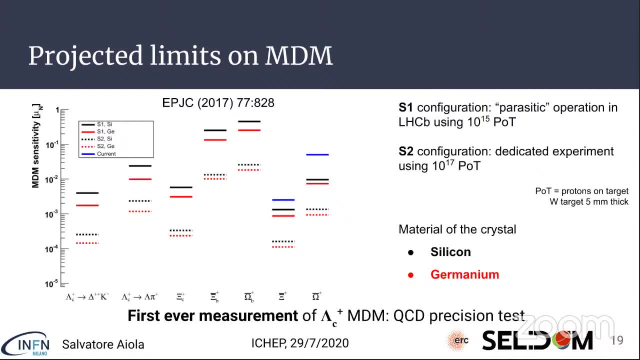 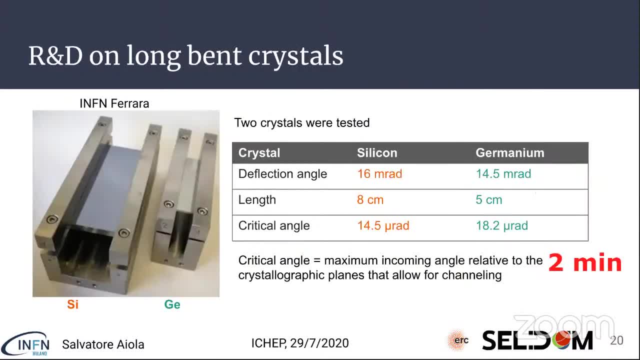 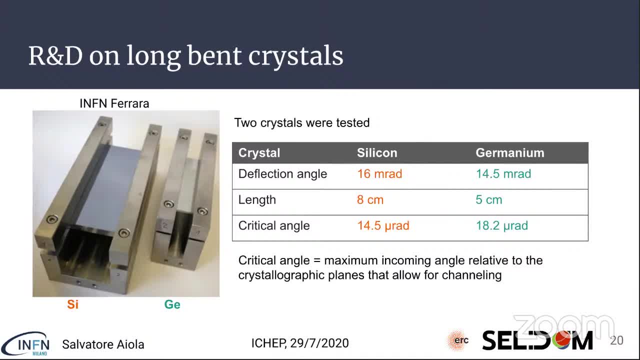 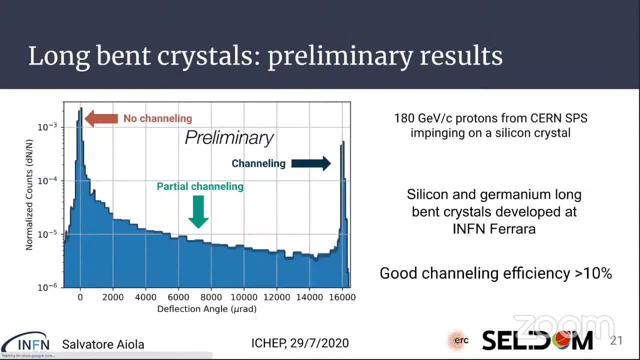 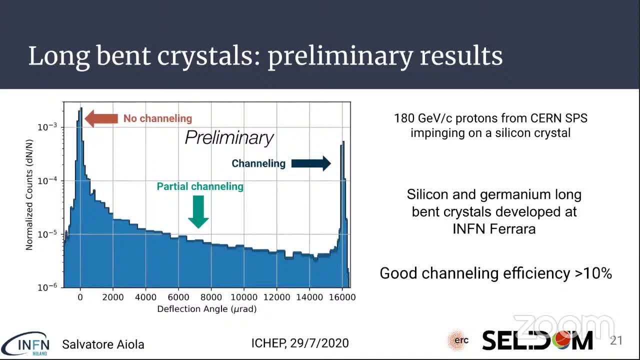 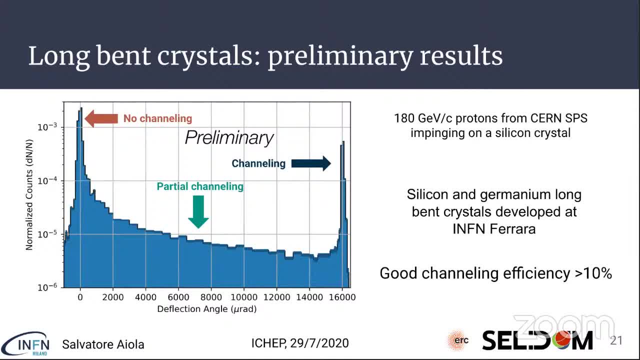 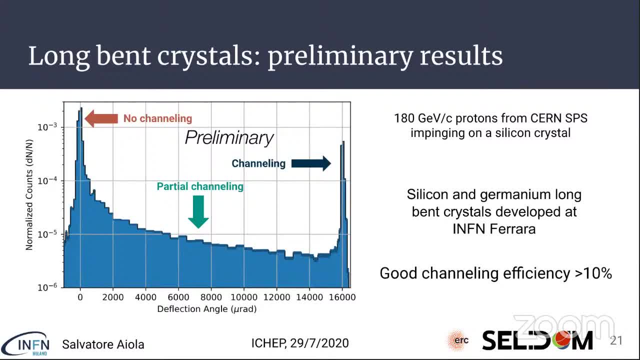 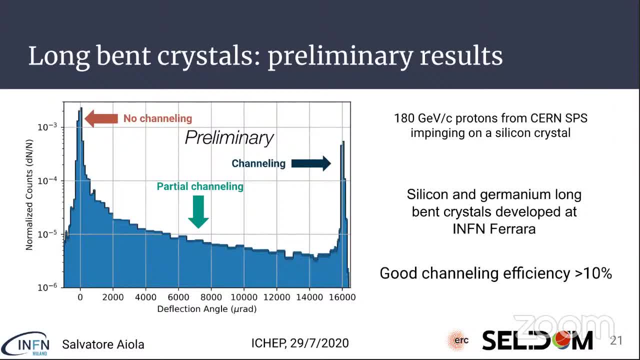 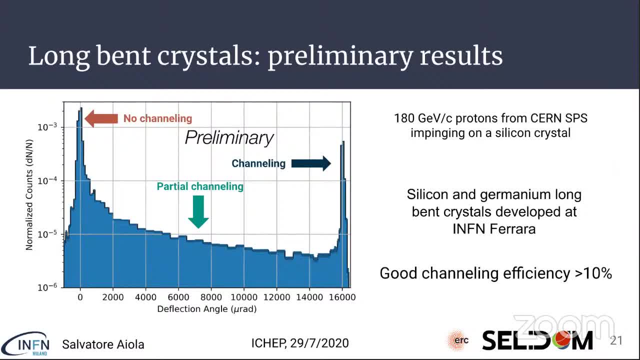 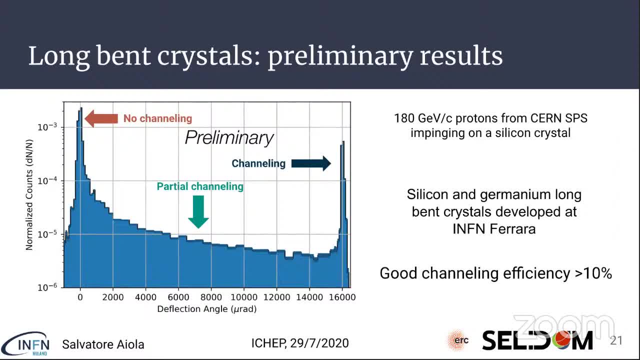 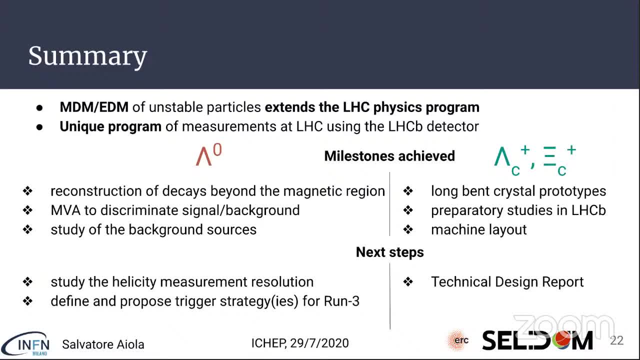 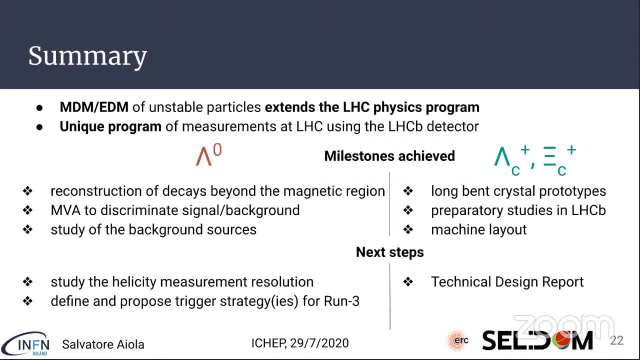 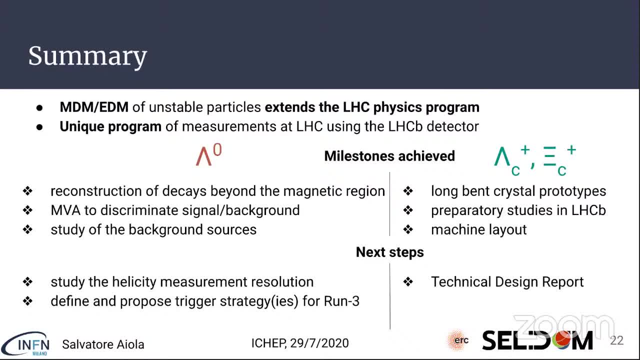 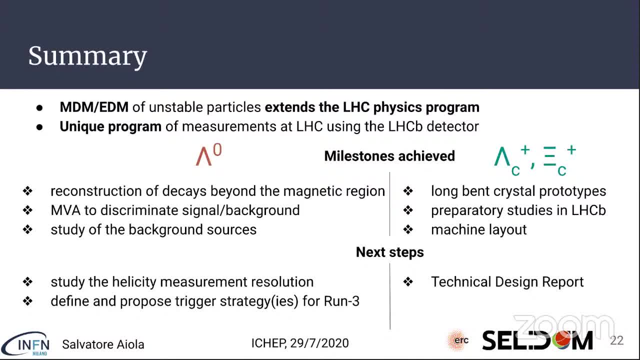 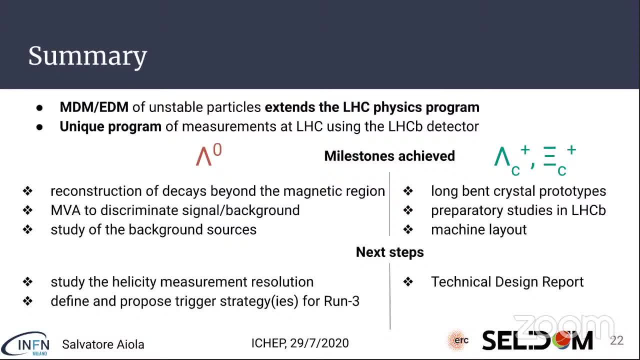 in fixed-target proton tanks. In this case we will look for charm baryons produced promptly in fixed-target proton tanks. In this case we will take the trusted persistence of an NCI teaspoons based today like the CMT- good candidates for this experiment. Then we have done some preparatory studies and simulations in LHC-B. 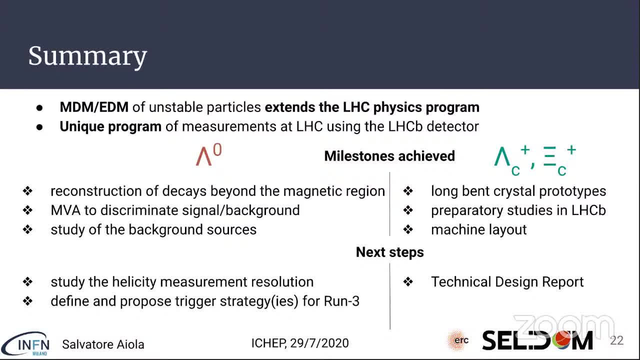 A machine layout has been designed by the experts of LHC of the accelerator, And so the next steps will be to prepare a technical design report, And this is all I have for today. Thank you very much for your attention. Thank you, Salvatore. Questions- Comments. 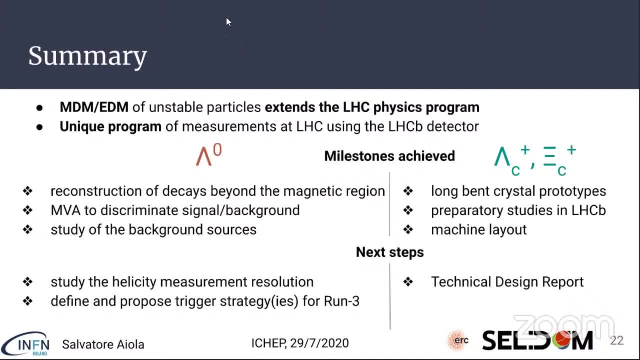 This is Alexey Petrov. Go ahead, Hi. So this, the channeling. I'm not a specialist in channeling bent crystals, but this seems to be quite an exciting technique. Would it work for leptons as well? I mean, for instance, if I would like to measure, you know, MDMs of tau leptons, for instance. 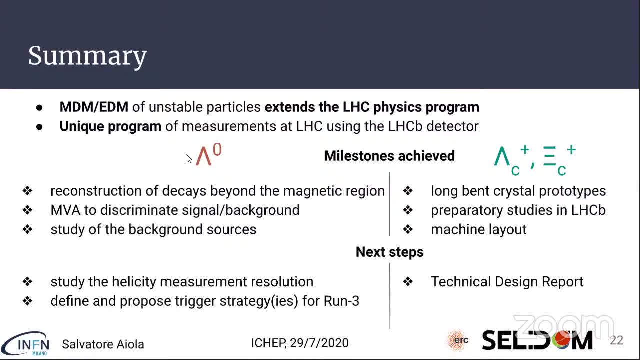 Yes, Certainly. In fact, I didn't talk about this because of time constraints, but there is indeed a proposal. I can send you a link to a paper that was published a few months ago about the proposal to use a similar technique to apply it to the measurement of the tau electromagnetic double moment. 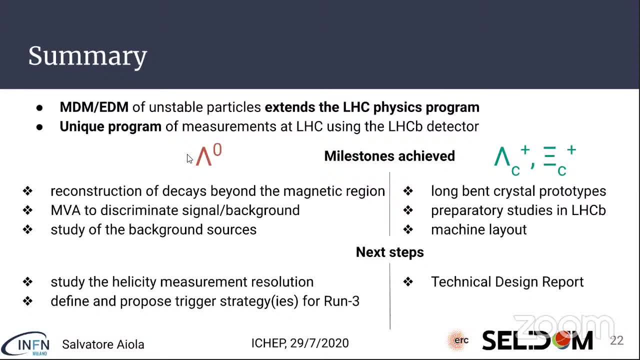 It is more challenging because of how the tau decays, So it's a more challenging measurement. It requires a lot more statistics. But yes, certainly it can be done also for leptons. Cool, I would appreciate it. Thank you, Yeah. 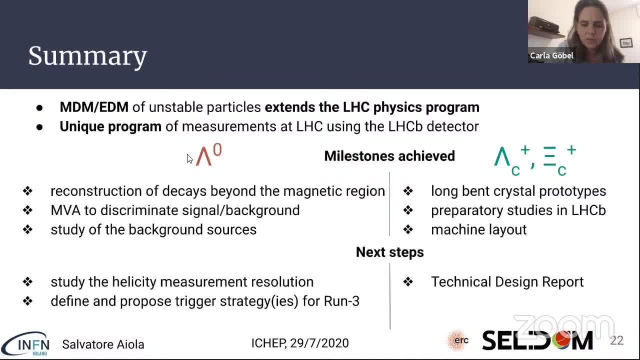 Another question. I have a couple. So the idea is to start by the start of RUN3, then No, The idea is to start perhaps during RUN3.. So maybe to install this equipment should be possible. maybe I mean with this we have to still negotiate with the accelerator expert. 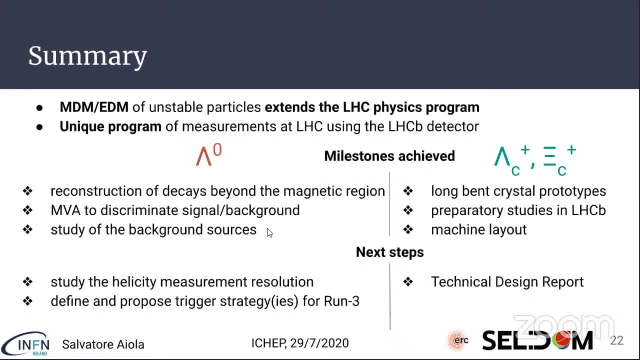 But certainly we will not be ready for the start of RUN3.. So, if we manage, we do it in one of the technical stops- end of year technical stops- during RUN3. Otherwise it will be done in RUN4.. Okay, And another thing due to my ignorance. 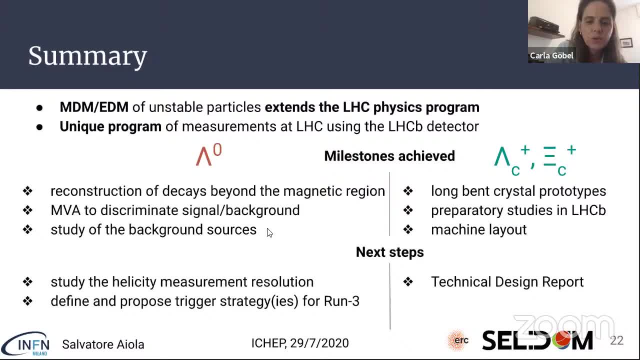 So can you comment on possible new physics models that would lead to EDM? I think there could be many. I mean it just requires additional CP violation in the standard model. So I think pretty much any model that adds CP violation to the standard model. 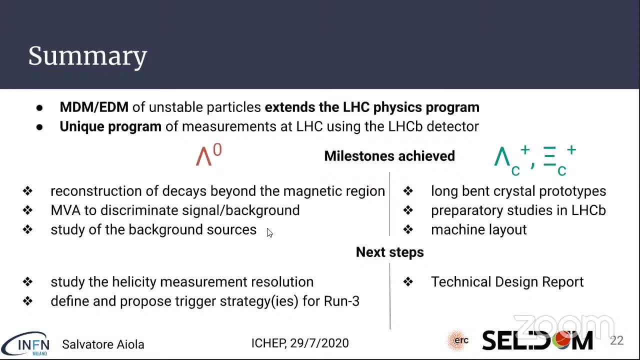 could have an EDM. I think it's not difficult to have this in a model, It just requires more CP violation, More CP violation, Okay. So are there any other questions? So otherwise, this is the finish of the session. two of the quark and lepton flavor track. 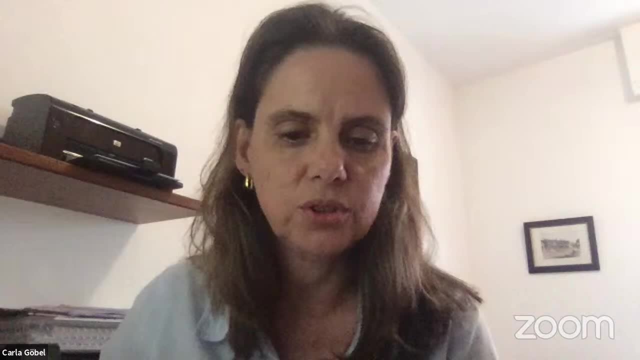 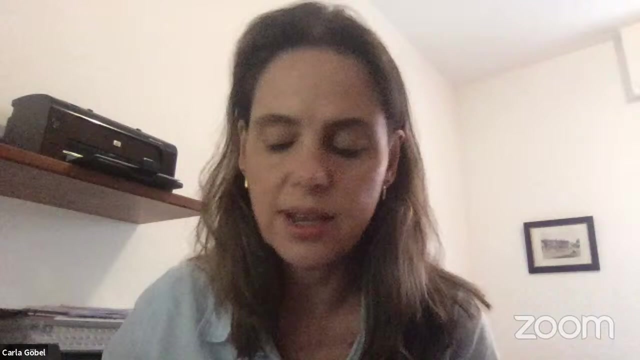 Tomorrow, the third session. the premiere will be in the morning, starting at 8 am European time. So we move to the morning for Thursday and Friday. So see you tomorrow, Thank you all. For those who want to stay here to discuss further, the Zoom room will be open for a while. 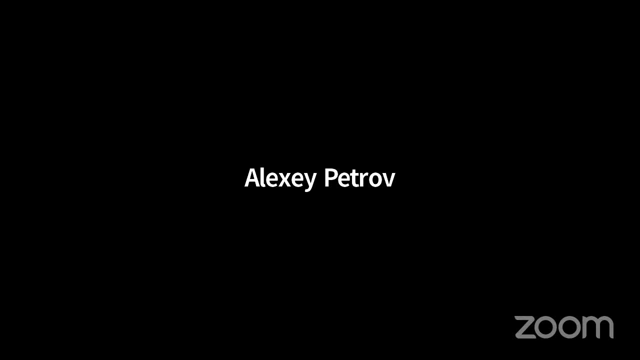 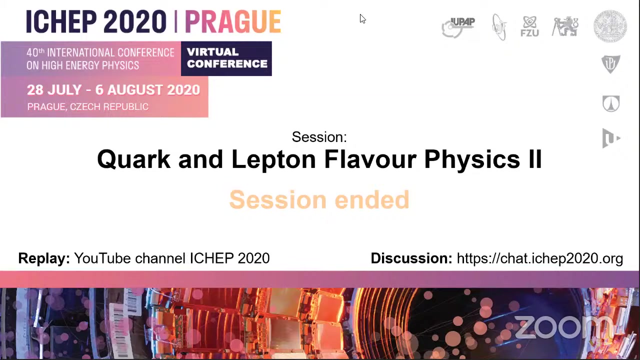 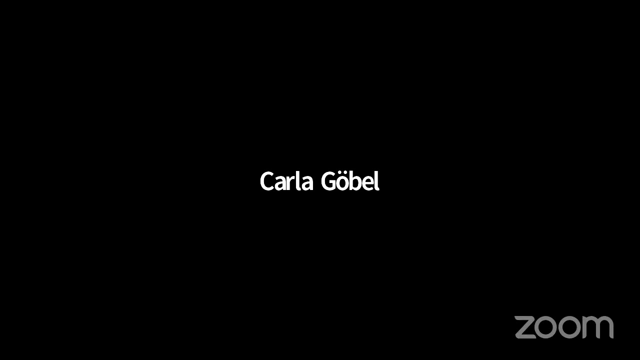 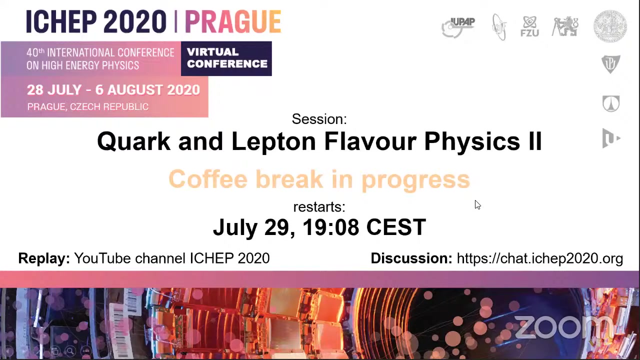 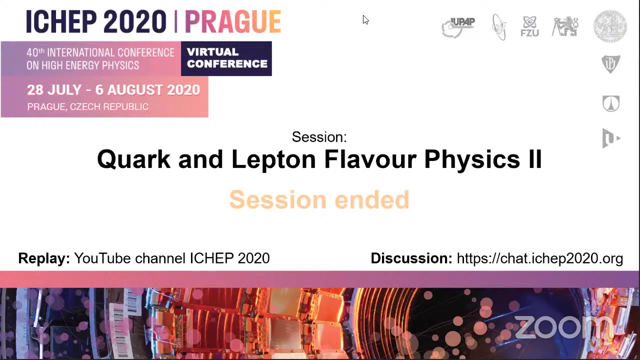 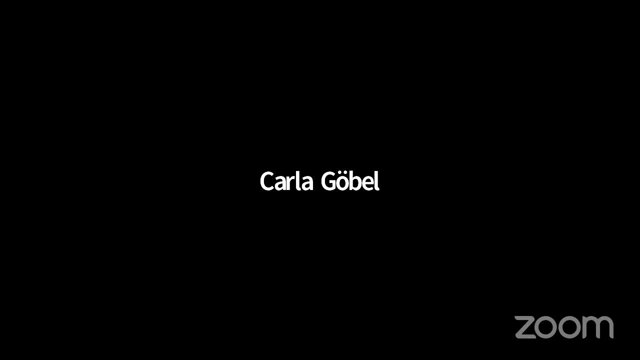 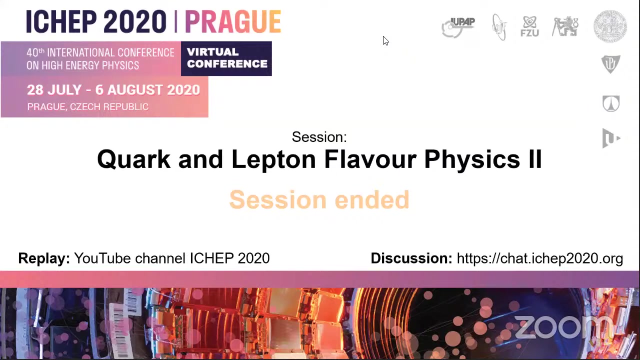